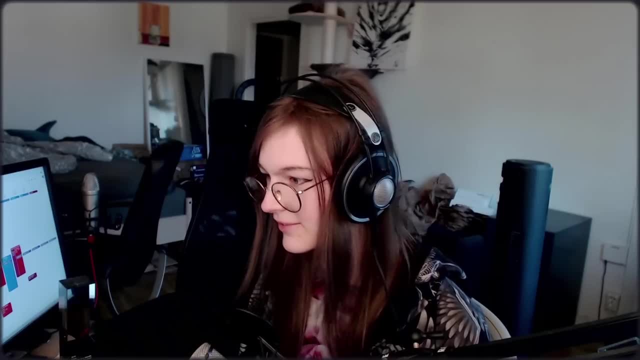 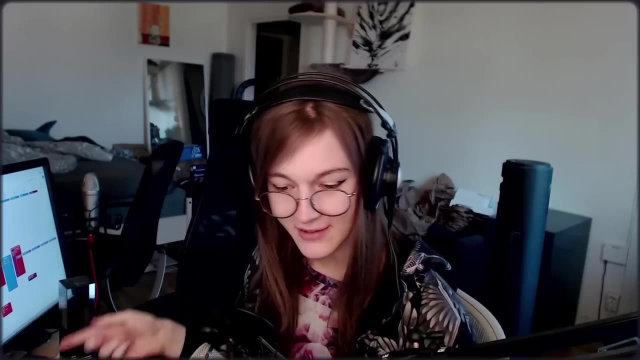 because then I could make ShaderForge. So I sold ShaderForge on the Asset Store, which made like enough money to be two full time salaries, pretty much. So me and another student at Future Games we started a studio. So we started an indie game studio called Neat Corporation. 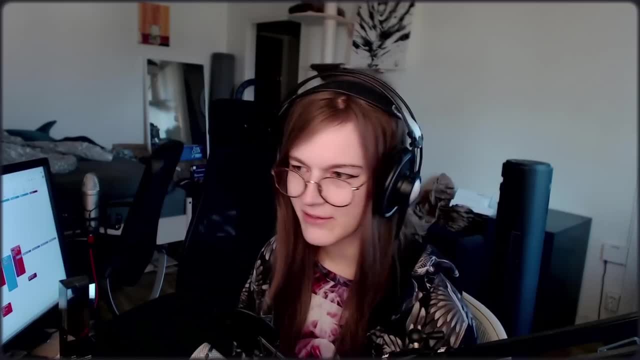 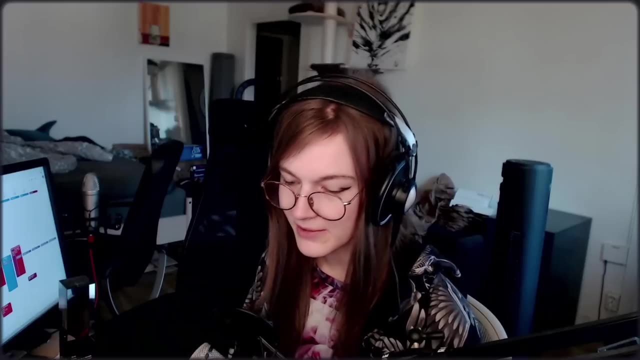 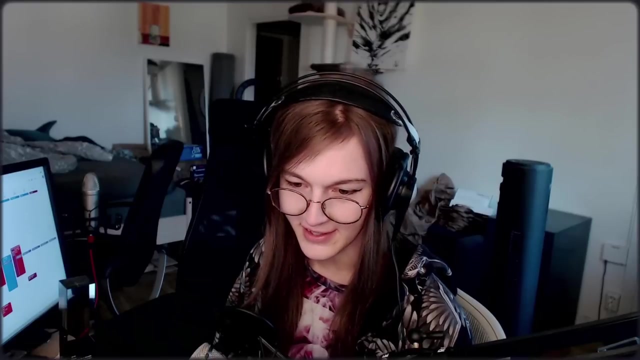 So at Neat Corporation we kind of started out wanting to make our own like very specific indie game. But then at GDC we were sort of we sort of like bumped into Valve right as they were releasing their HTC Vive headset. So we got kind of inspired by VR as soon as that kind of happened. 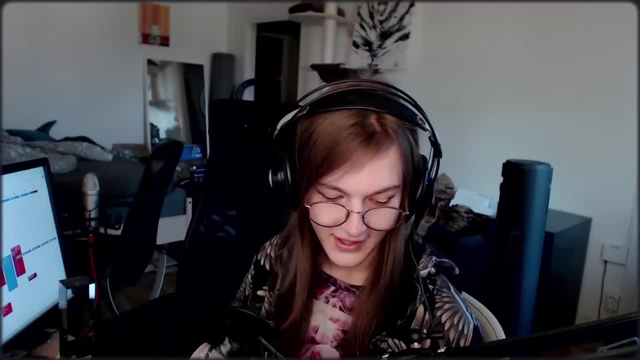 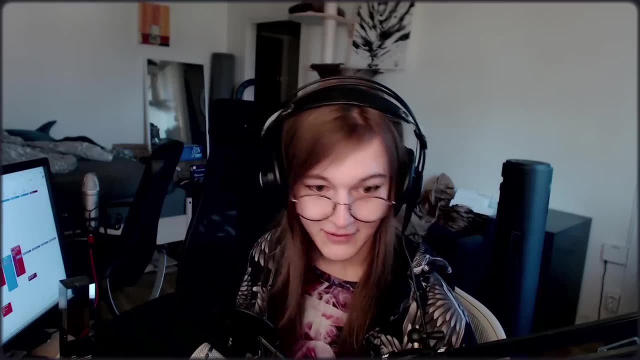 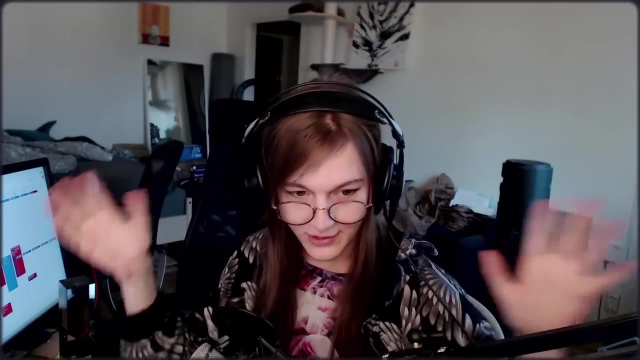 So as that exploded, the whole VR scene- we got to be there like at the very, very beginning, when everything started like growing, which was really cool And also made us realize how, like going to GDC and just talking to industry, people can lead you down so many paths. 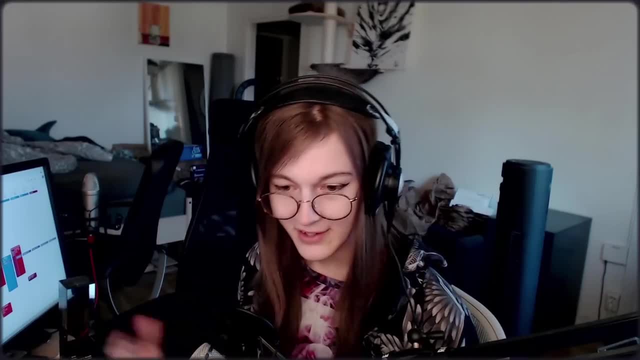 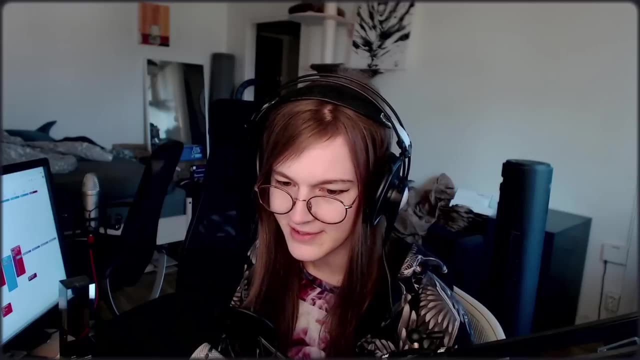 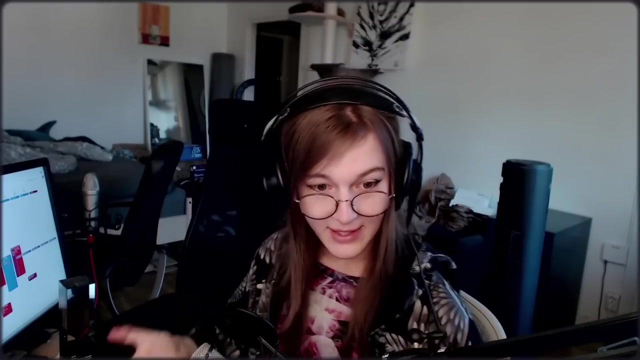 And like just that connection with people is so important if you want to like make connections in the industry, start new opportunities and whatnot, And all it takes is kind of like you have to try to be available for all of these things. Anyway, that was the story of NICORP, how we sort of started NICORP and started working on the game called Budget Cuts. 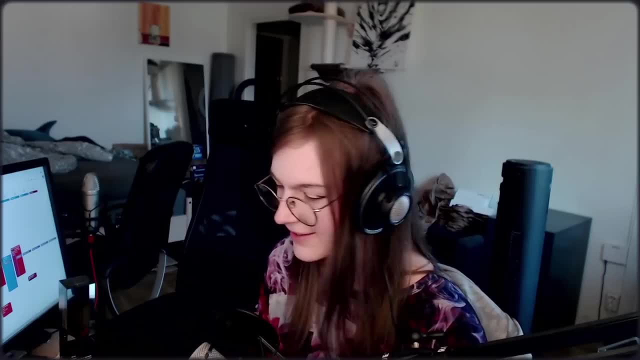 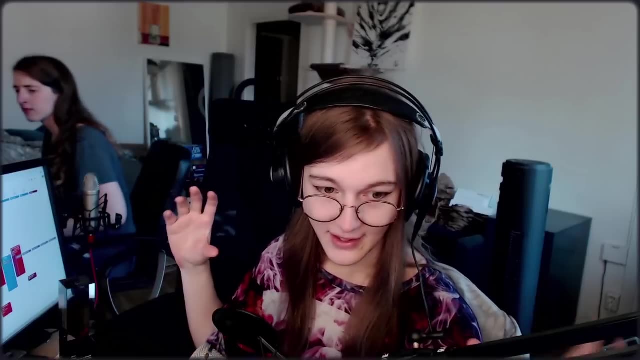 So that was our first kind of flagship release title, One thing that I just need to mention before we get started in terms of, like, my approach to teaching, like my goal is that I'm here to help you learn- Right, That's kind of that's kind of it. 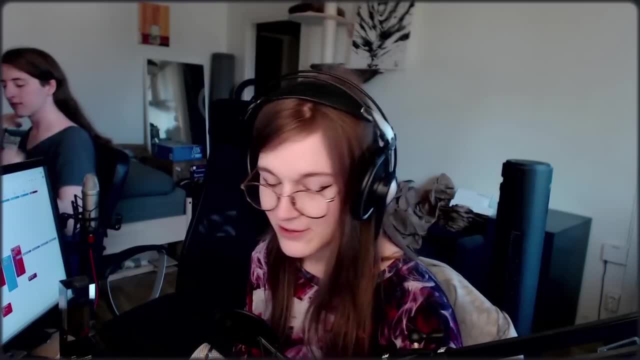 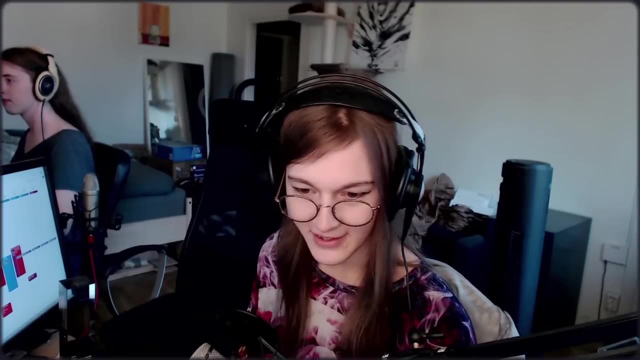 So you usually get a lot of questions along the lines of, like you know, do I have to do this assignment, and so forth? And The short answer is yes, because you're going to have Krister do all the grading and all that stuff. 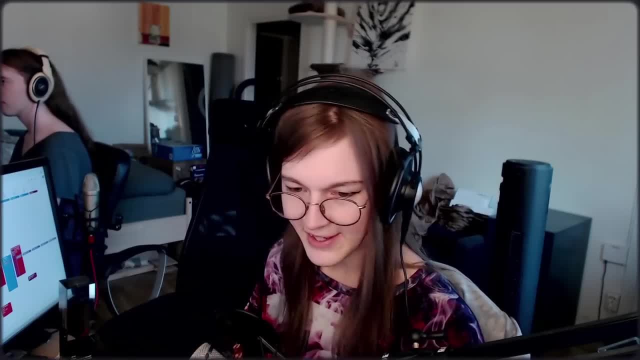 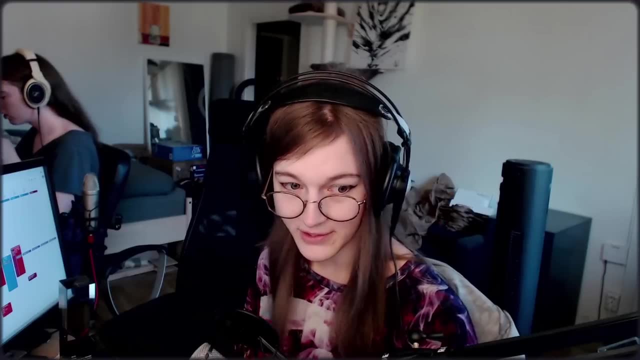 But the long answer is that I personally- I don't care what assignments you do or don't do, or anything like that- My goal is that you should learn the things that you want to learn Right, And I'm here to help you do that. 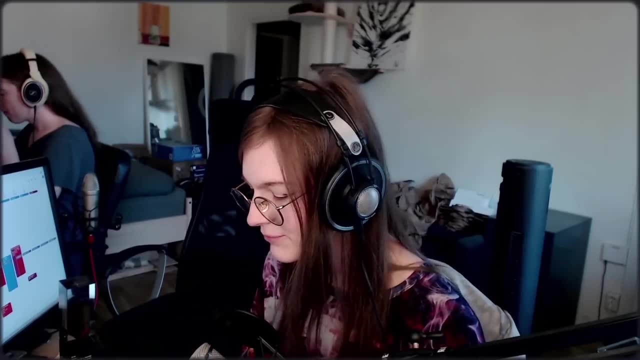 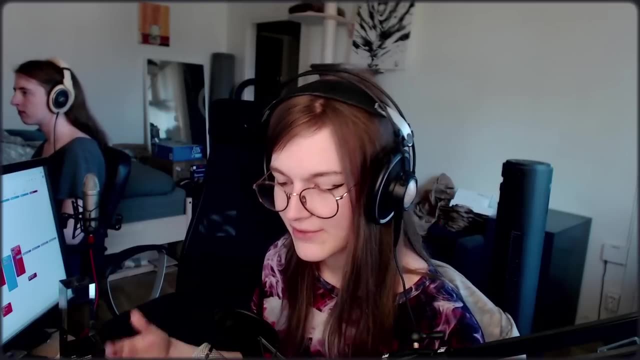 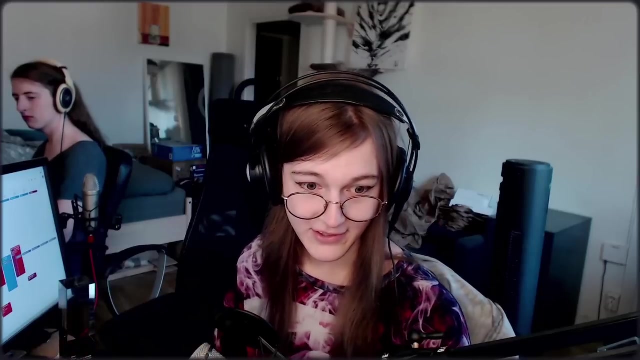 But I do, I do want to stress that it is important, though, like what kind of like, what kind of standard you're setting, not only for yourself in terms, So like what goals you have and what you want to learn and how you learn, but also how that reflects on you in the eyes of your, your fellow students. 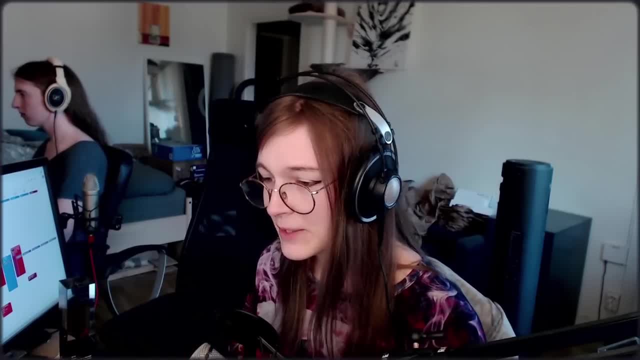 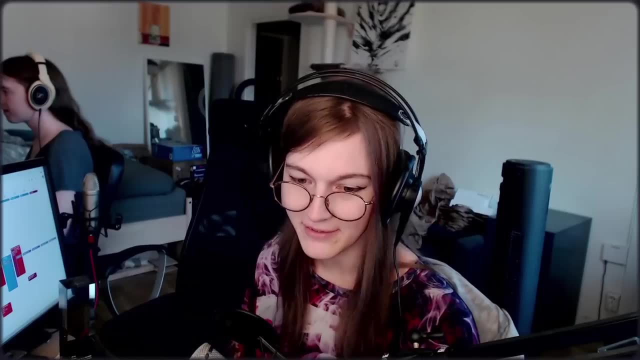 Right, Or even in the eyes of me, Right. If I, if people around you notice that you are someone who is like doesn't do any assignments or like show up late, effort every lecture, then I think a lot of people like are going to think of you as that person that's always late and doesn't like deliver or whatever. 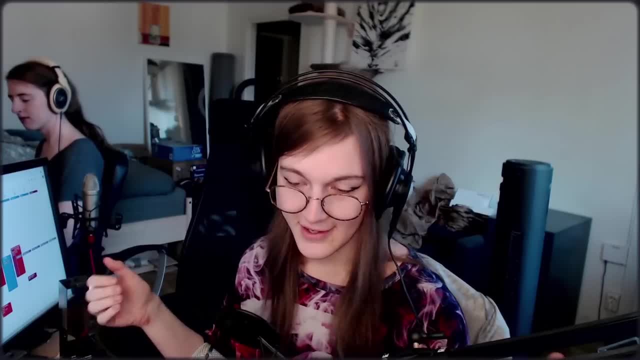 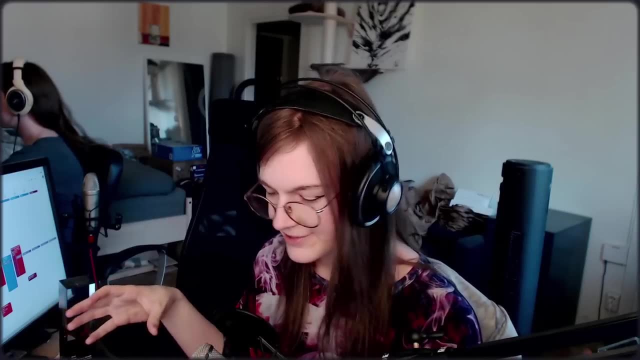 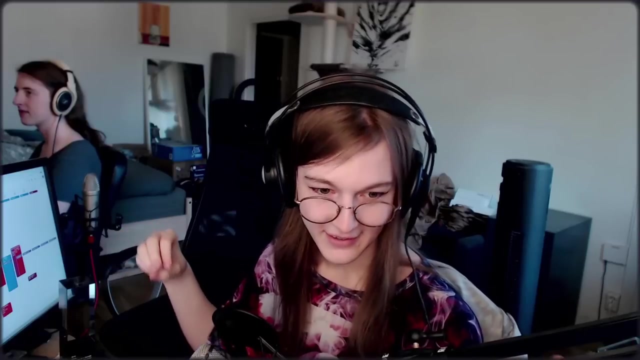 And you're all going to be in the industry soon, Right, Like? if you think about my classmates, pretty much all of them are in the industry now. So you know I will remember people who were kind of like not great, So like it's important to kind of like be a good person and be like kind of project the image of you that you want others to see once you're in the industry. 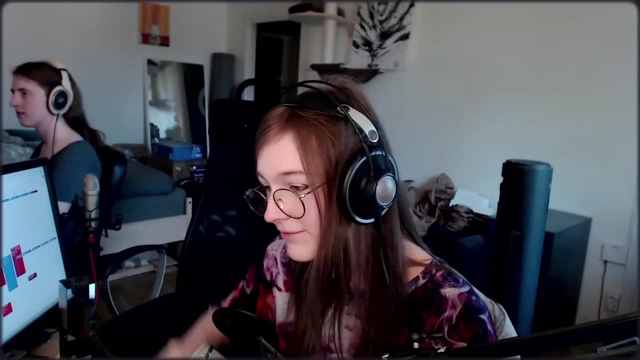 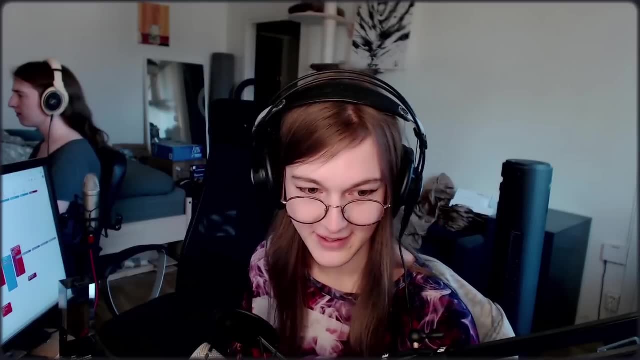 Right. So I think it's important for like from that, from that point of view, to actually do do assignments and whatnot, to at least be the person who did the assignment Right. But then again, personally I don't care that much. 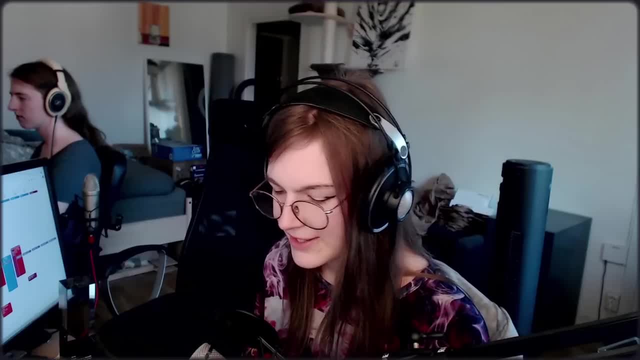 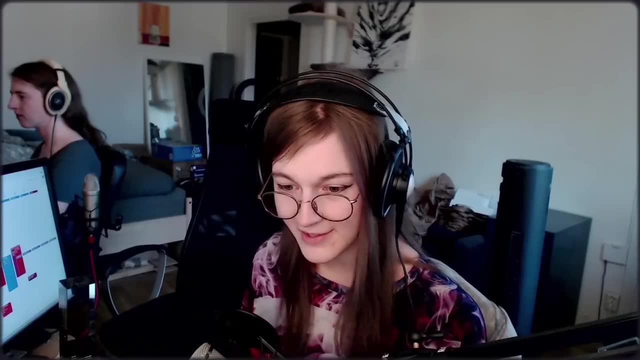 I just want you to be able to learn the things you want to learn, Right? If you hate math, you don't think it's going to be useful, Then then Sure, Feel free to not do anything, Right? But I think it would be detrimental for you, especially if you're, if you want to do a lot of coding. 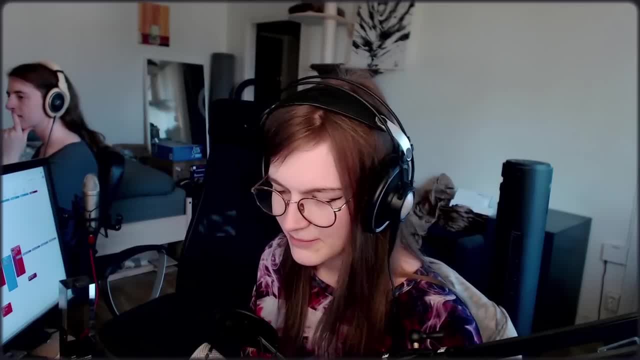 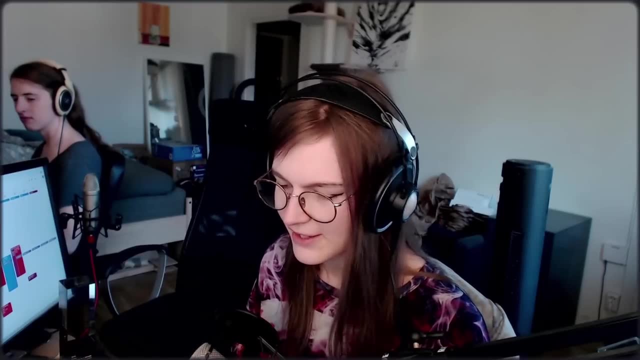 What will the assignments look like? The assignments will be mostly to do some mathematical thing in unity. It's not going to be very unity centric. Unity is mostly going to be there as oscillator, our platform and rendering engine. So it could be things like: 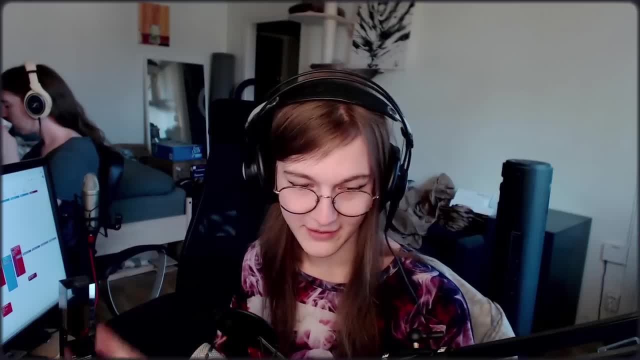 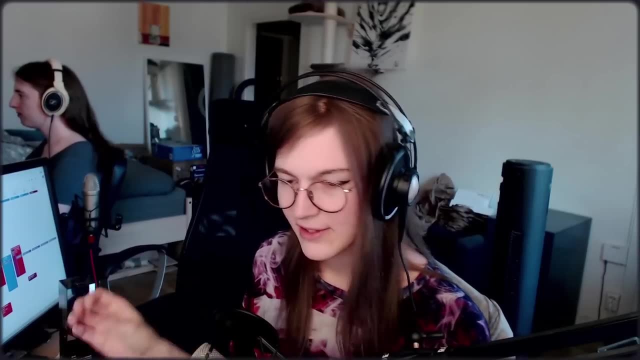 I would do the math for the spread of bullets in a shotgun or whatever like that kind of stuff. So they're gonna be pretty short. I intend to do more than one assignment per day, So you can have three tier assignments, like one easy, one medium and one harder task. 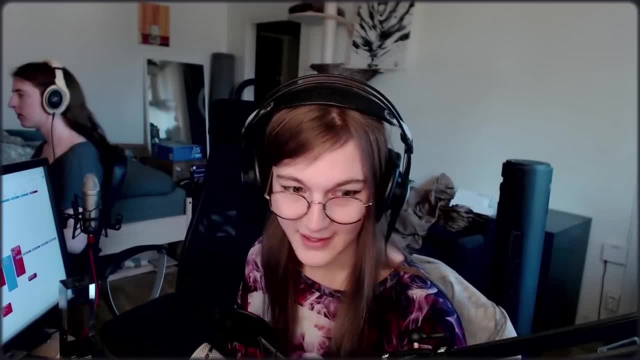 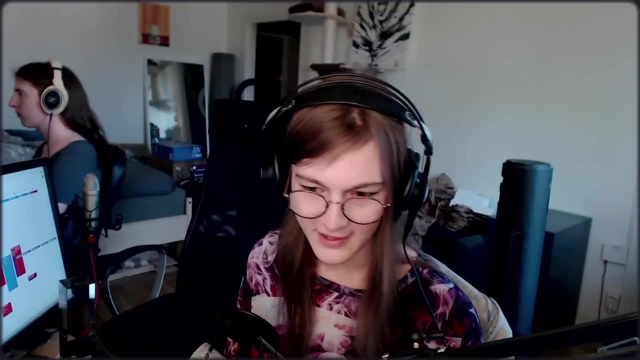 And then you can sort of do however many you want, I think, depending on how Krister wants to grade this. I'm just gonna send the answers to Krister and he's gonna work on the grading and stuff. I usually like having a tiered like assignment thing. 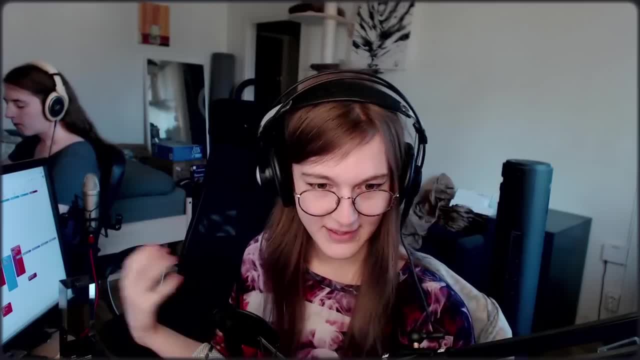 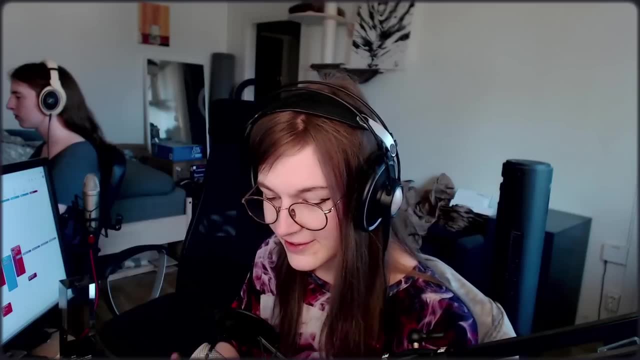 because it tends to be more flexible and you can sort of do things step-by-step, which I like All right. another very important thing: please ask questions. There are no stupid questions. I think it's like one of the most detrimental things. 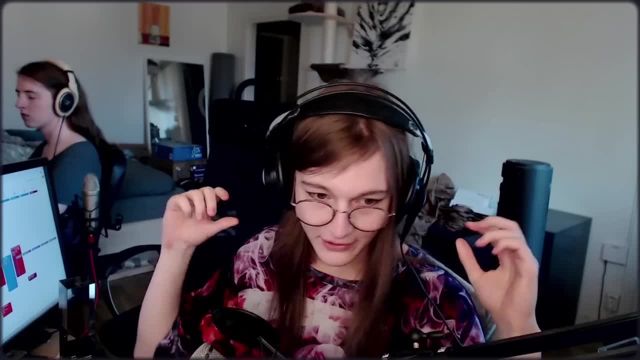 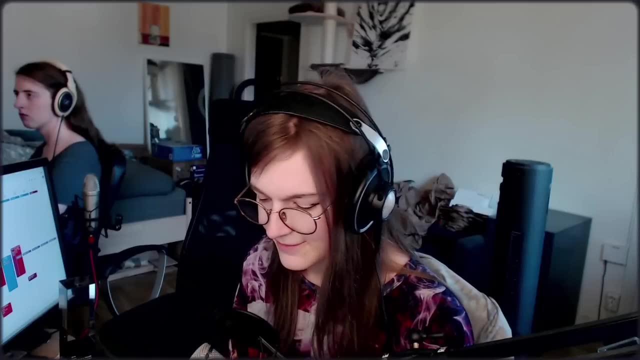 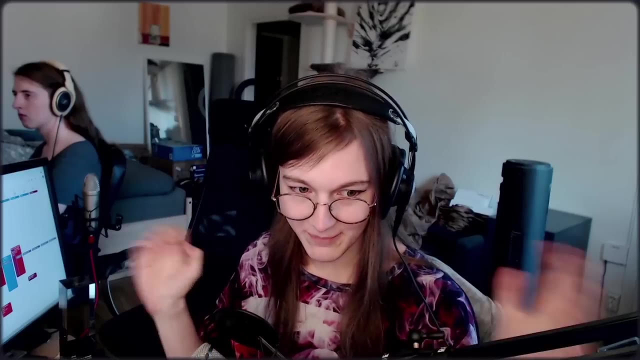 for you to do is to, like you have a question in your head or something I said was unclear. please ask that question that you have in your mind. It's so important because, like usually, when people like almost every time, someone says this might be a stupid question. 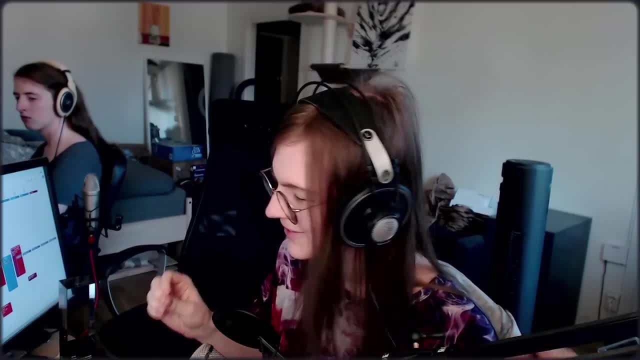 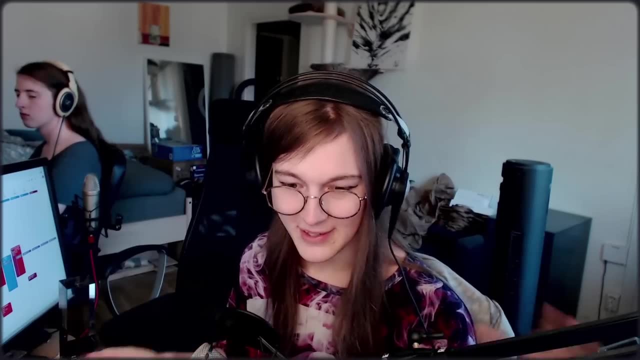 but they ask a really good question. So please keep that in mind: ask questions. Don't be afraid to ask questions. Asking question doesn't mean that you're stupid. It means that you're actually smart because you actually want to learn the thing. 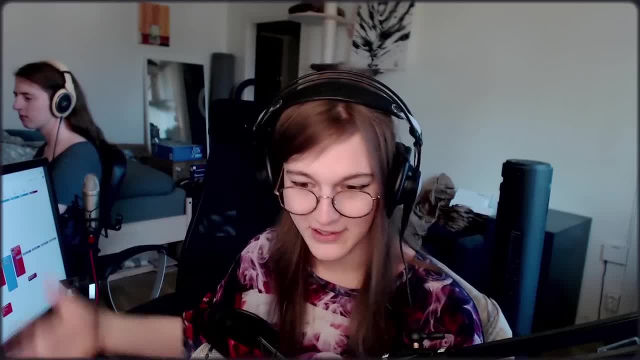 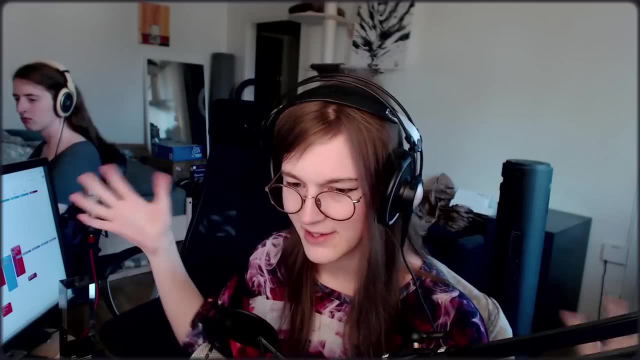 and want to understand the thing that you are observing and trying to pick up right, But of course try to stay on topic, Like don't go like too far off. We're going to have a lot of breaks, So we're probably we can do like you know. 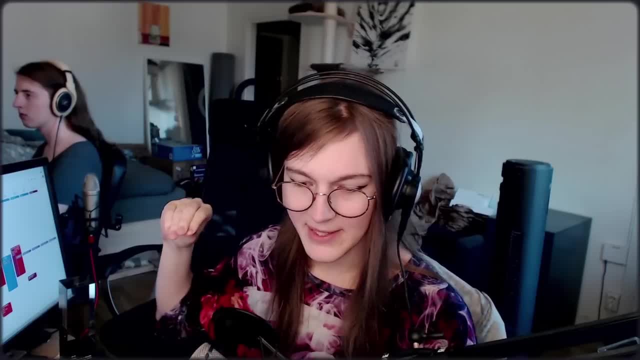 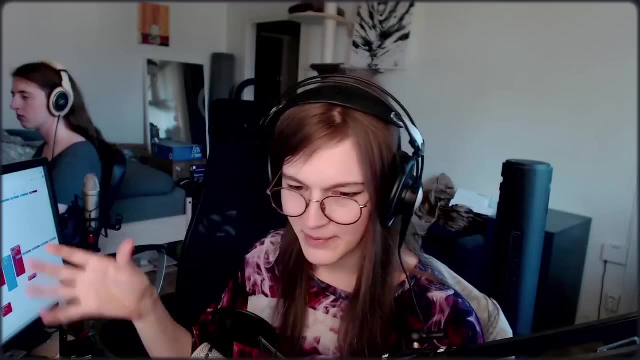 random Q and A stuff during breaks, if you want. Okay, oh, obviously, sometimes, like some people can get very stuck on one thing. In that case, if, like one person gets very stuck on something, then we can probably like talk about that after the lectures to like clarify any anything. 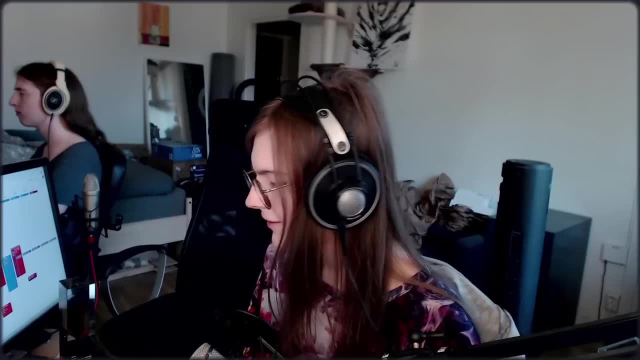 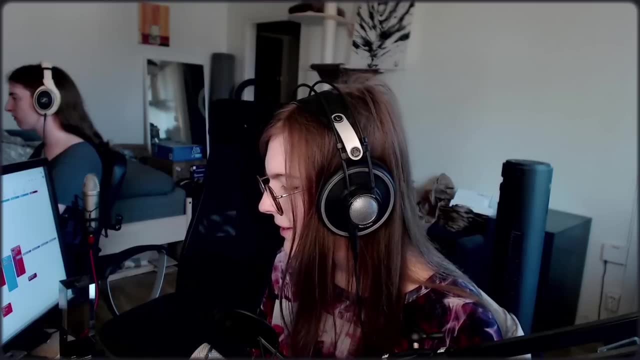 So in case it like takes too long to like try to hash that out. All right, any questions so far? Sorry, we haven't like started the actual lecture. I've just been rambling about random stuff. Will there be any linear algebra? 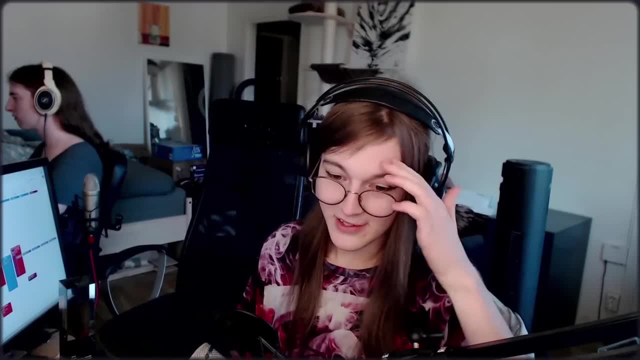 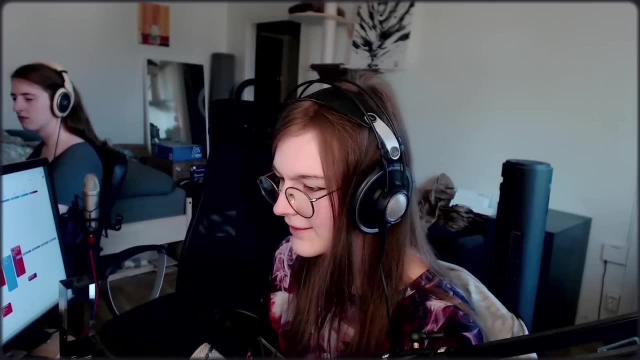 I believe. so yes, I mean yes, We're going to talk a lot about vectors, dot products, cross products, all that stuff, And matrices too. All right, So let's see shuffling around my notes. Oh, if you want to, we could look over some of the things. 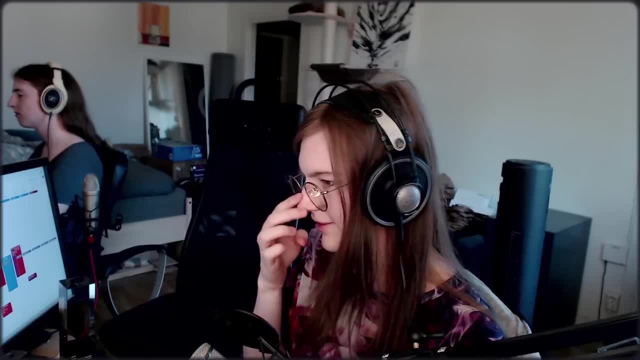 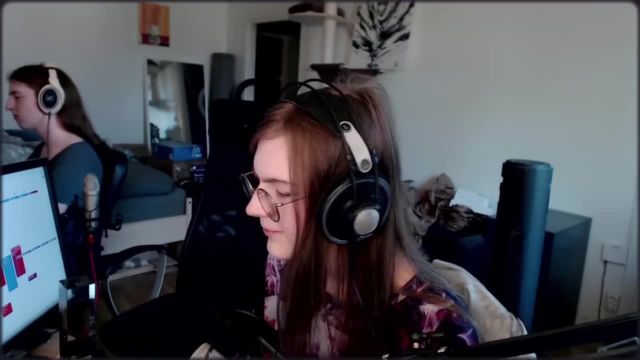 you're going to see in math papers. I don't know if you want to like have some tool sets for like being able to parse papers. I could plan that in- probably not for today, but some of the others. I could plan that in the other days. 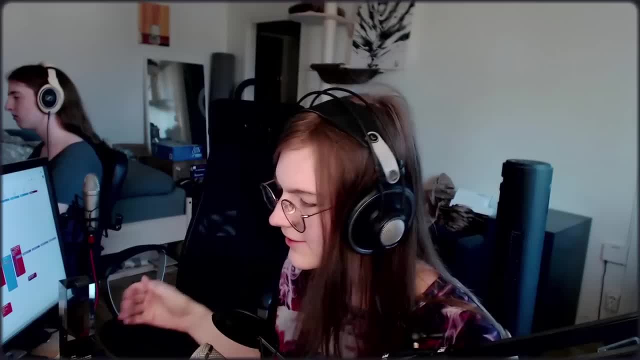 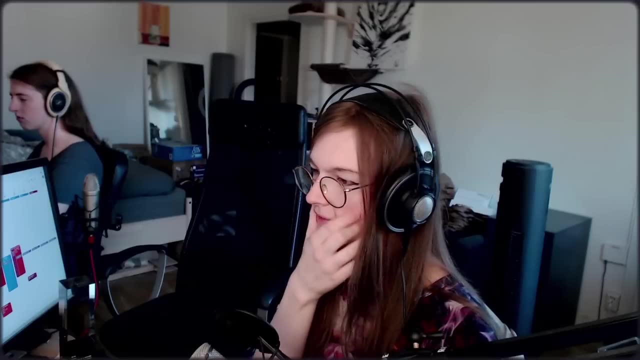 Cause we do have- I do have- a bunch of like time that I haven't like planned in, because usually things take longer than you expect, Sometimes they're way shorter and so forth. All right, So I first want to talk a little bit about like why I think 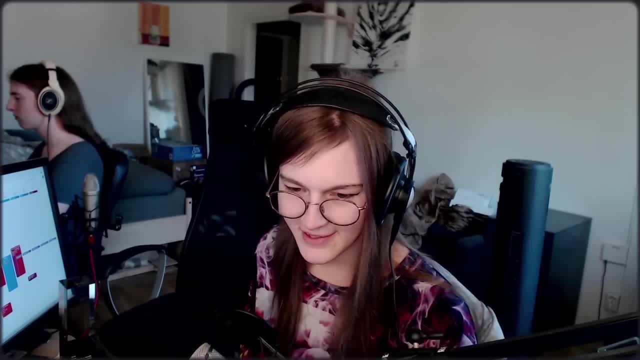 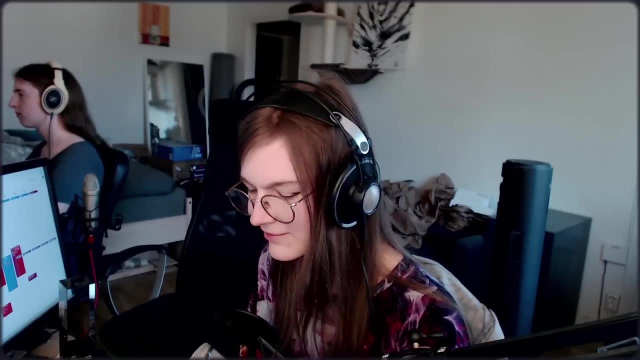 math is cool. I think math sort of has this bad reputation Cause I think a lot of, in a lot of cases it's taught as kind of just the boring thing you have to do in school that has to do with numbers and you have to like 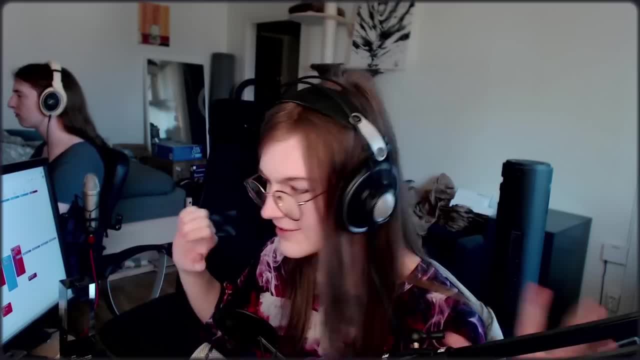 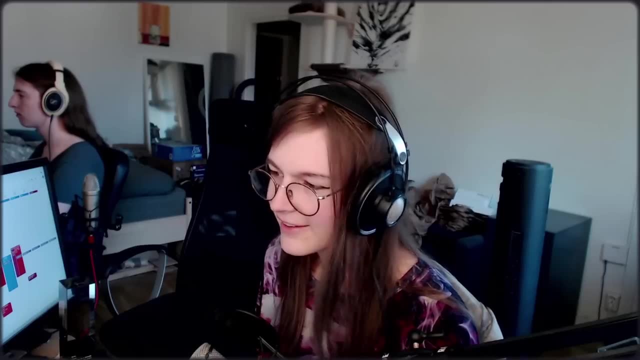 I don't know. It's very esoteric And the most common question that students ask is: like: when am I ever going to use this in my life? Right, Like, when do I need the cosine? You know, like that, that is extremely common for people. 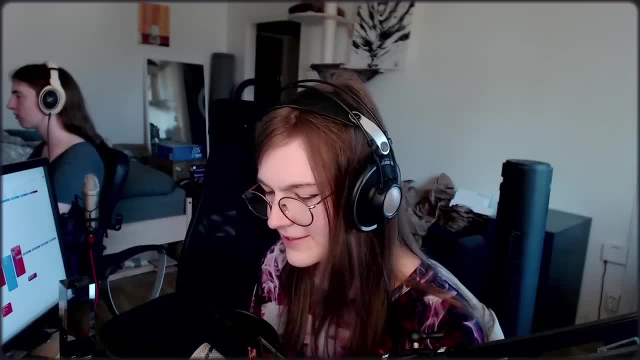 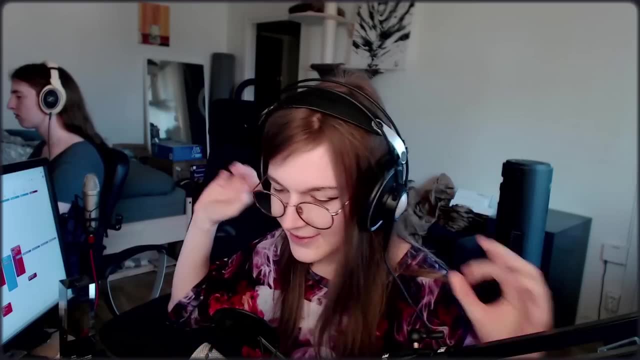 to to feel like that And when it comes to math, but I feel like game development is sort of one of the like, one of the strongest cases where math is just like extremely useful, like absolutely everywhere in in doing game development. 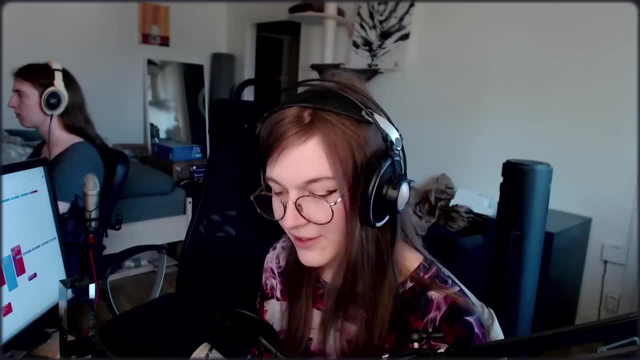 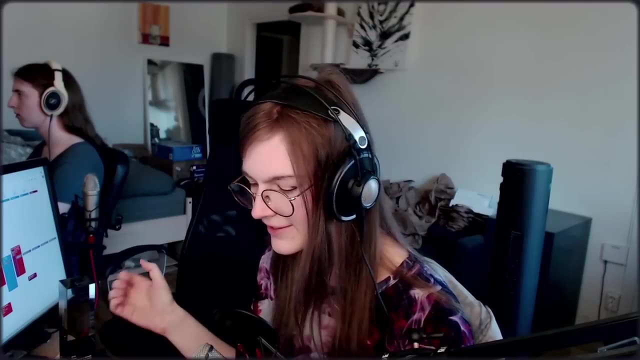 Not only like in terms of gameplay code, but also like a lot of it is in like rendering and all of that stuff Right. But I think the the problem with teaching math in general is that I feel like people who teach math are sometimes like excited about. 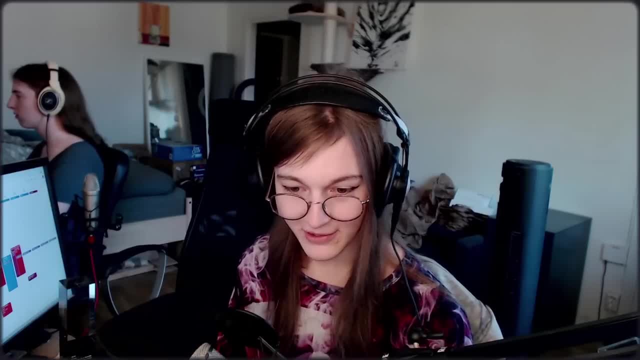 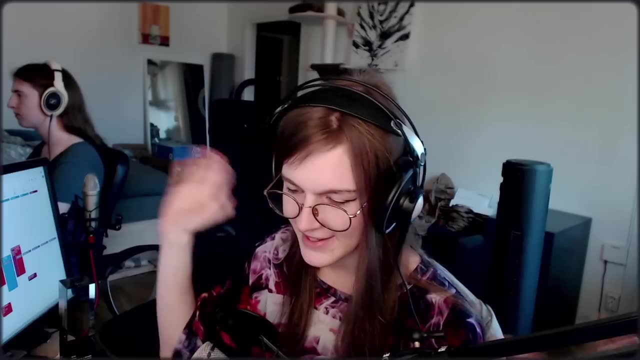 math, but they don't really. they kind of presume that other people are already excited about math and then they don't really like show it in an exciting or interesting or visual way. So then it just becomes this esoteric thing where you have to trudge through a bunch of numbers and it's just boring. 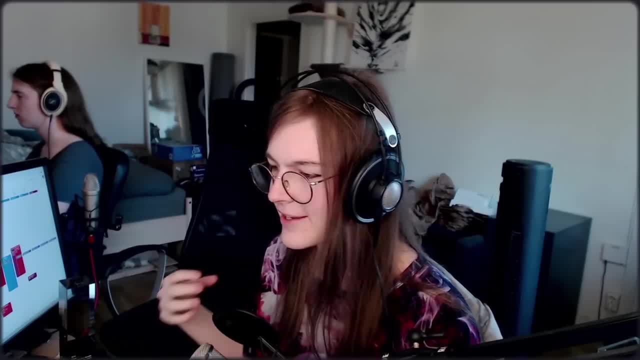 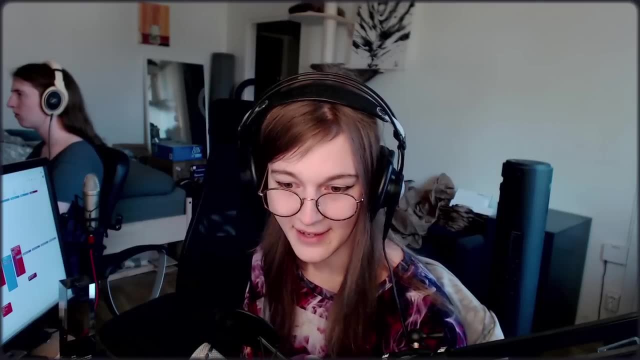 Right. So I think that's a that's a shame. I feel that, like mathematics is incredibly fundamental, It's like one of the most fundamental fields of study that we have. Like they're like it kind of doesn't matter where you are in space. 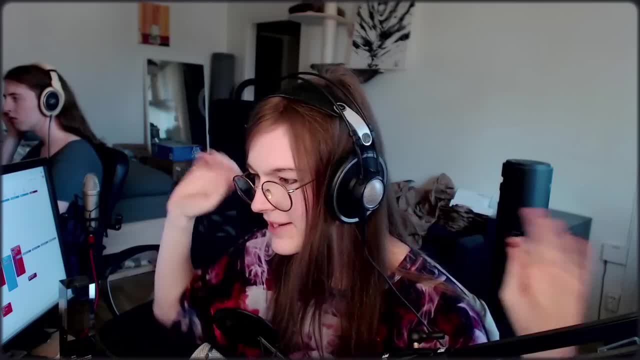 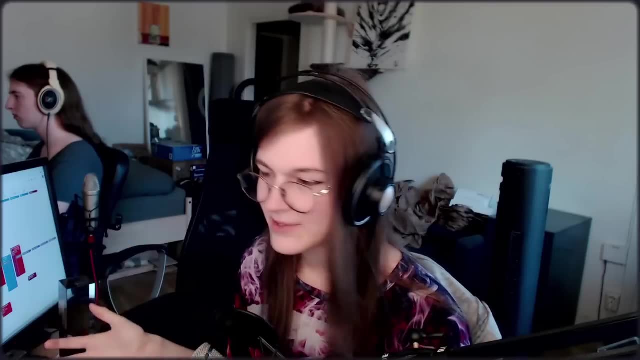 Like you could be an alien species somewhere. You could be like absolutely anywhere, It doesn't matter, It doesn't have to be on earth, Doesn't have to be this society. You can have other numbers of dimensions, but math is still. 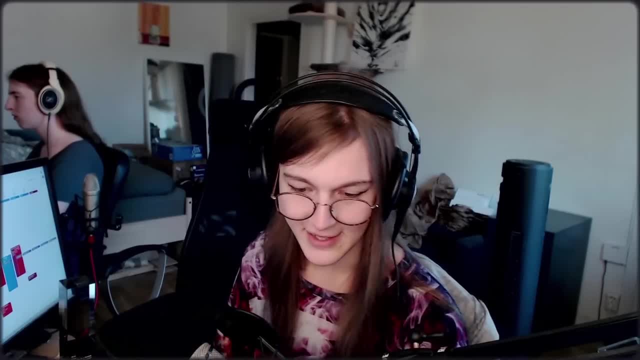 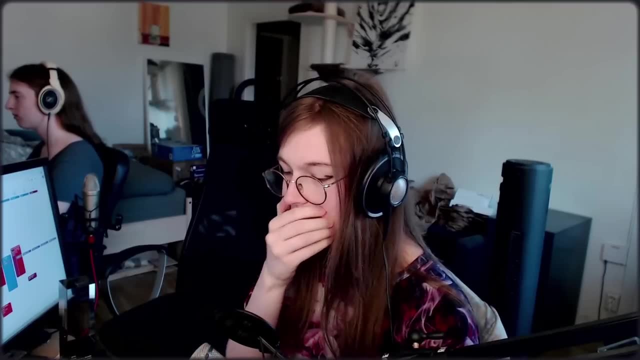 still gonna exist. right, It's going to be called something else. Numbers are going to be presented in a different way, People are going to use different symbols, but math in and of itself is going to exist because math is, like it's the like- the study of quantity. 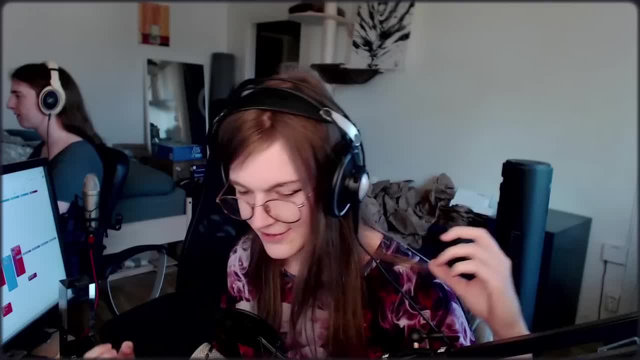 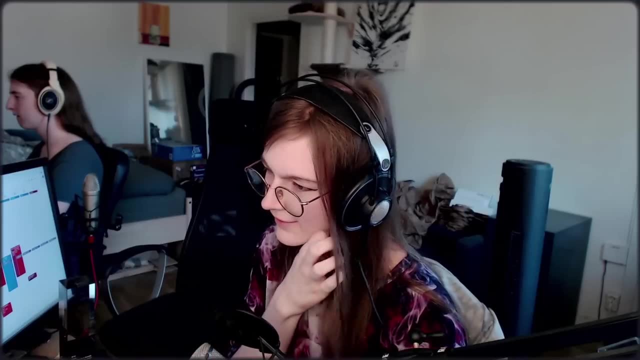 It's a study of space, It's study of structure, It's a study of change, And it's kind of hard to imagine a universe where any of these things just don't exist. Like what does it even mean to have a? 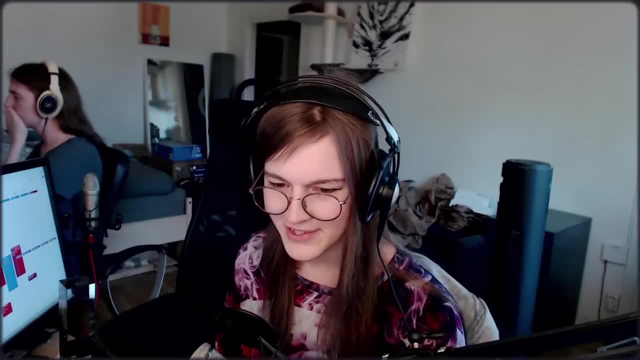 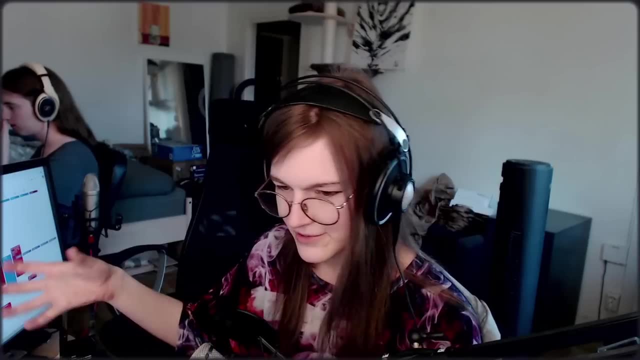 like: what does it even mean to have a universe that doesn't have quantity as a concept? right, And I think that's really cool. It's kind of this like field of study where you can sort of co-discover things. like you know, the 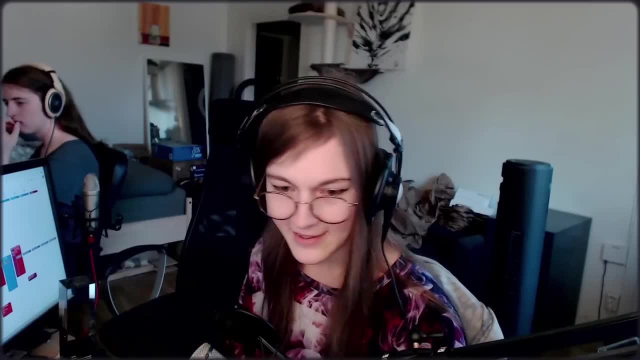 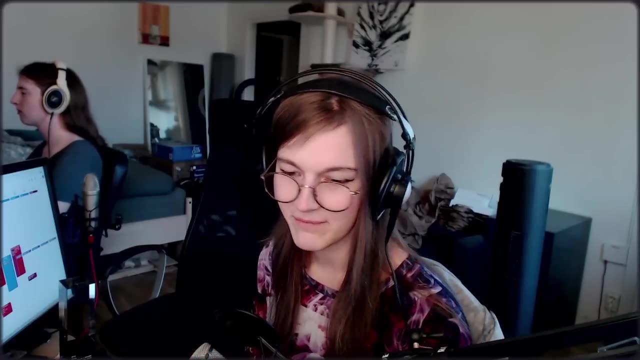 the circle constants like pi and tau, E, the golden ratio, like all of these things are probably discovered in other societies, presuming they exist, even though we're entirely disconnected from each other. just because it's this study of the very fundamentals of kind of 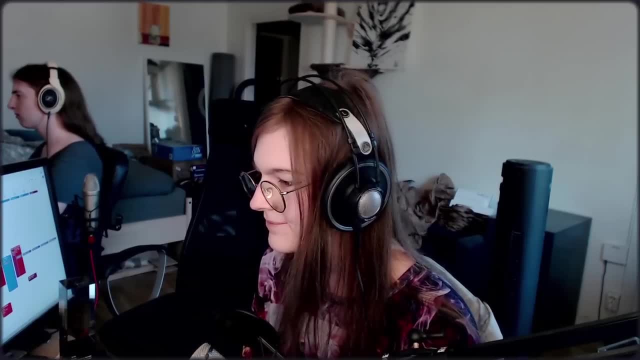 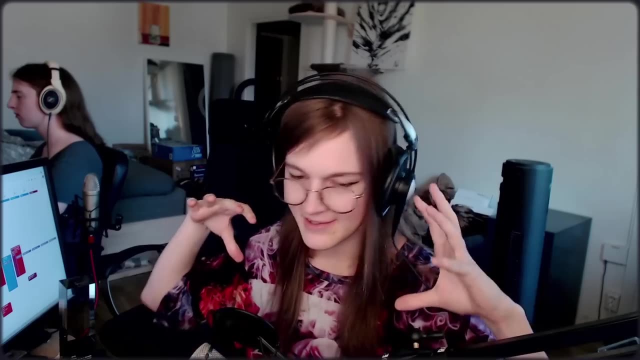 structure and change and that type of stuff, Yeah, And so so. so for me I feel like the it kind of underpins like physics, It underpins chemistry, biology. none of these things would really exist without math working as. 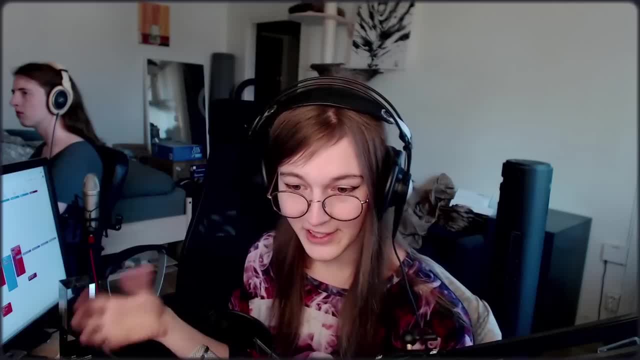 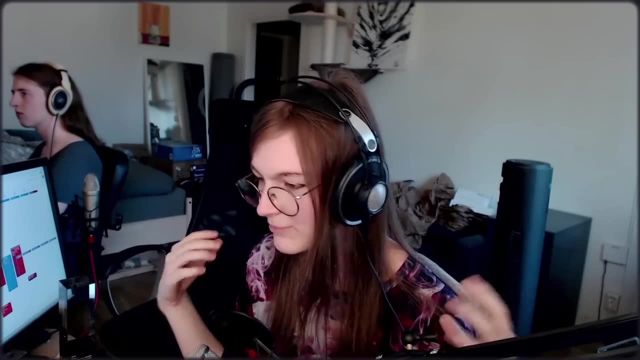 well as it does and being applied to these fields. Right, It's similar to philosophy. I feel like philosophy underpins everything in like social sciences, It underpins morality, ethics, politics, ethics, ethics, politics, ethics, ethics: It underpins everything. 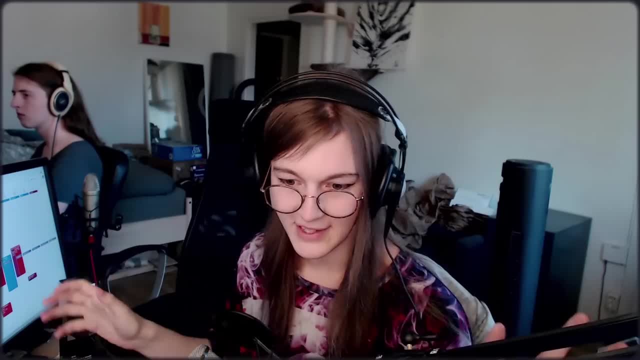 It underpins everything. It underpins everything. It underpins morality, ethics, politics. It underpins everything. philosophy is sort of the groundwork for all of those things, and that's kind of why I also like philosophy, um, but I think it's really cool that this is so fundamental, and that's why I think. 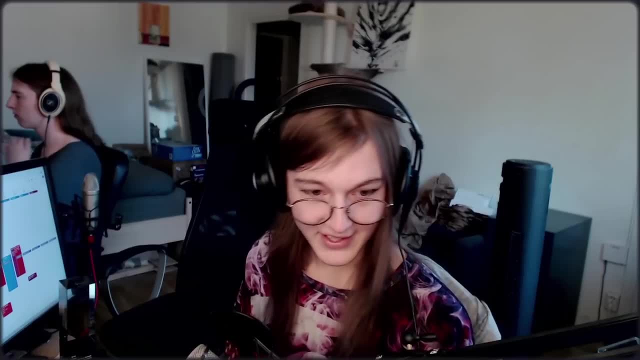 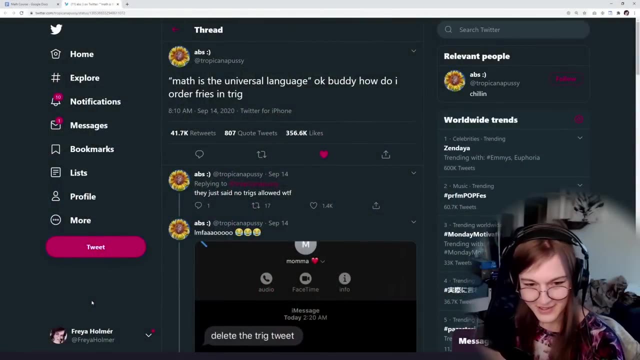 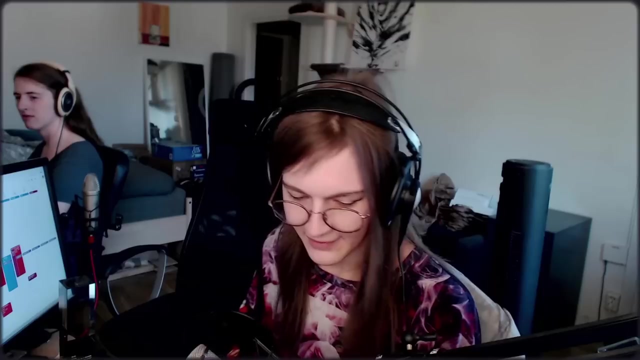 math is cool, um, they're also like you, of course. can't like apply it to absolutely everything, um, because usually people say stuff like math is universal language, uh, but you know, it's kind of not universally applicable to every situation out there, uh, anyway, so that's all well and good, but 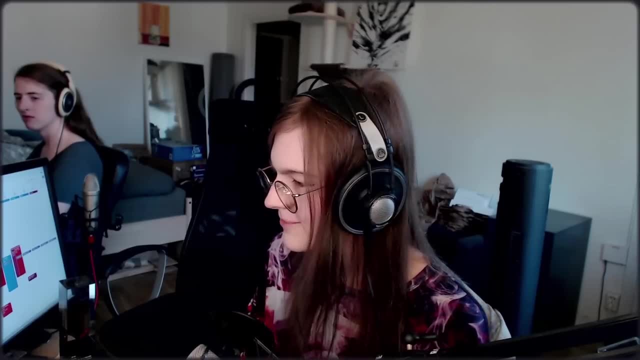 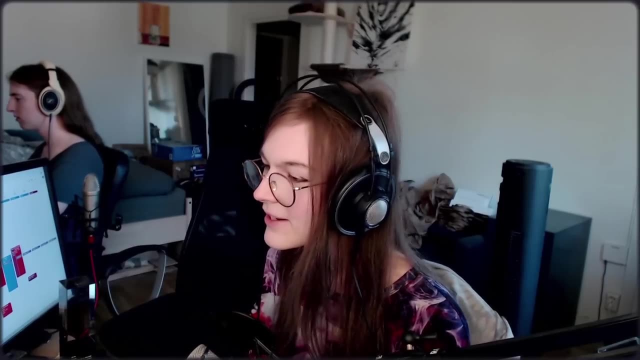 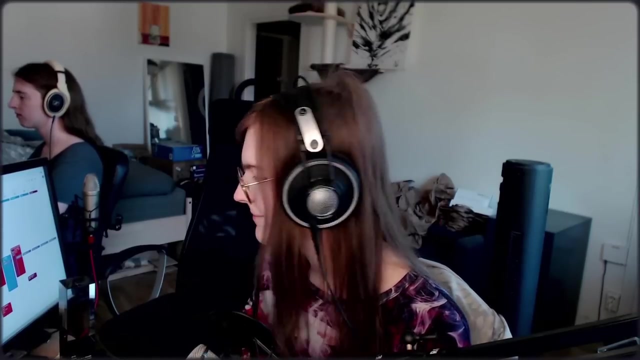 I'm already. I'm already interested in math, and you might not be um, so I feel like we should go into the like practicalities of what it actually means to use math in, in games, um, and how everything works. I also think people overestimate how much math you need to know to do cool shit you can get. 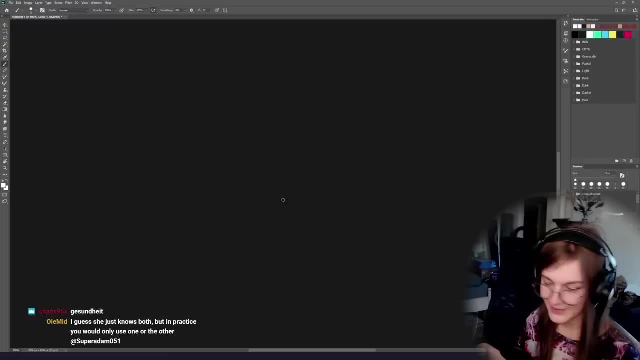 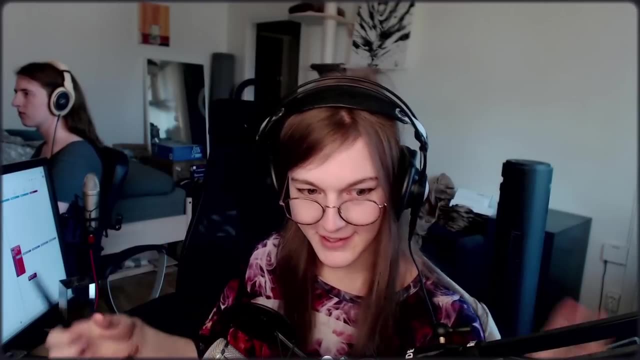 so far with a few basic principles. in some time, yes, um I I keep saying that you don't need to know that much math to do game development. uh. if you um want to like make an engine, you need more, uh. but if you just want to do gameplay coding or even. 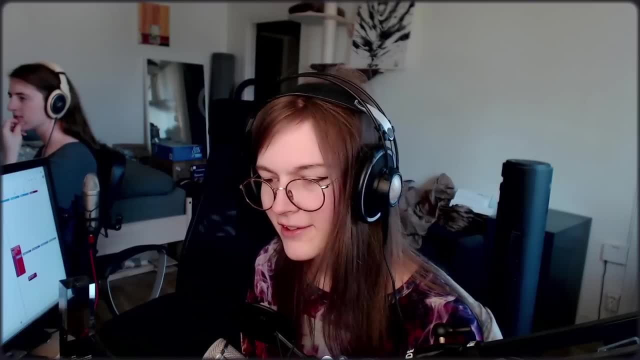 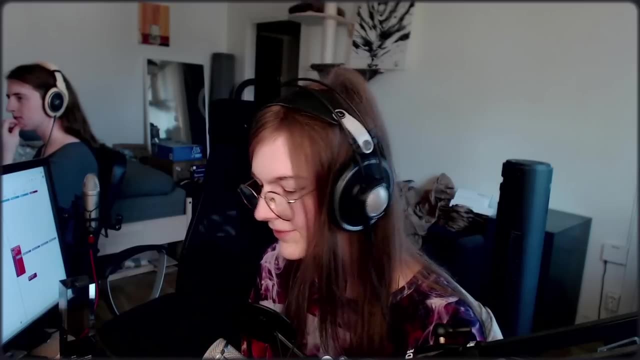 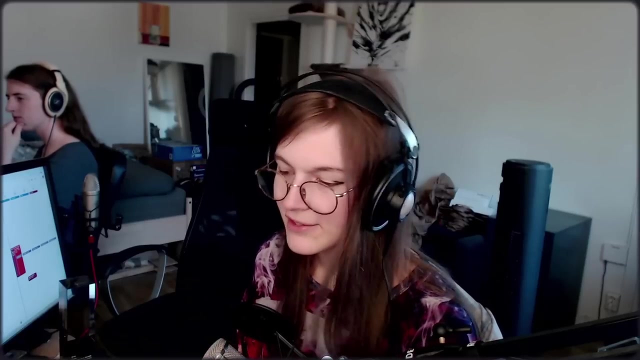 shader coding. to some extent you don't need that much math. uh, so I'm going to go through most of the like, the very essentials of um game development. math, um like even things like derivatives or integrals- they are kind of rare in game development, even though they're very fundamental in teaching. 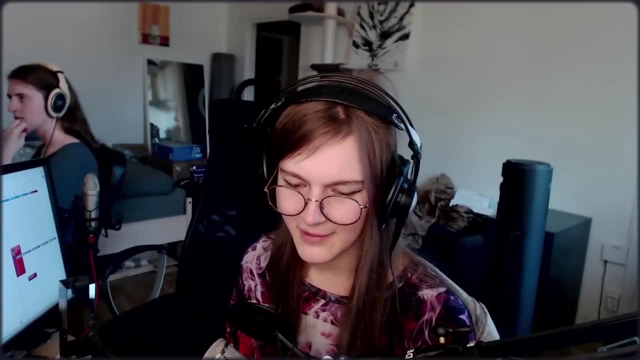 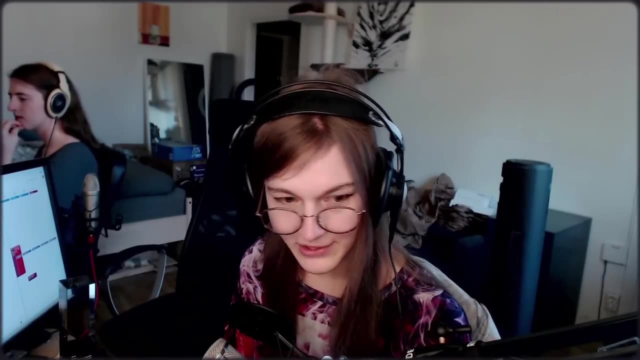 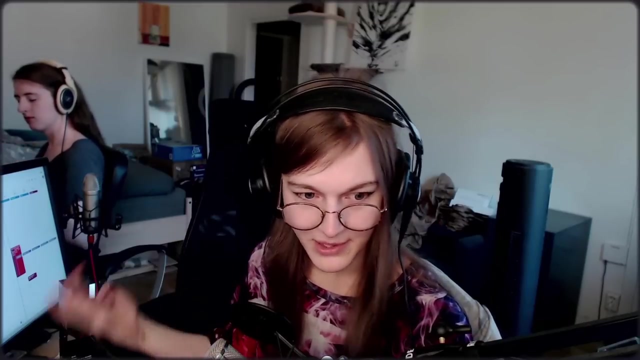 math in game dev. you don't have them very often, um like. mostly if you're doing some very like um very math heavy rendering stuff, that's when you start running into um, especially integrals, but otherwise like generally like, linear algebra is like most of most of game dev math. understanding derivatives and integrals is really useful for anything. 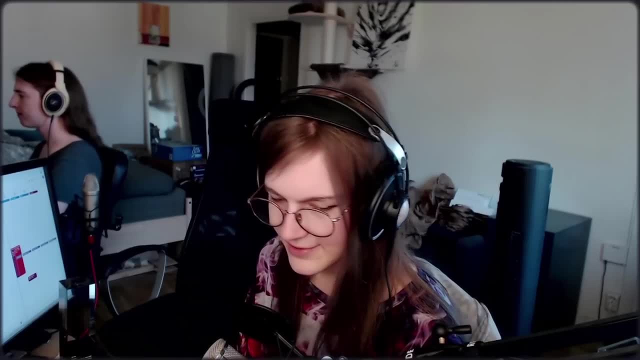 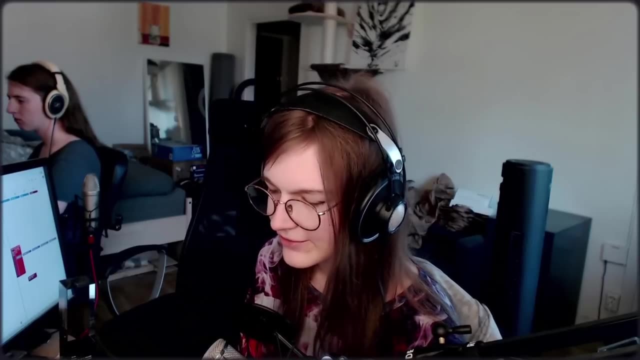 related to implementing physics. yeah, so there's the idea of what a derivative is is really important, but you don't really need to know how to derive equations and derivatives are really important to you. can learn how to do them, but you don't really need to know how to do them, but you don't really. 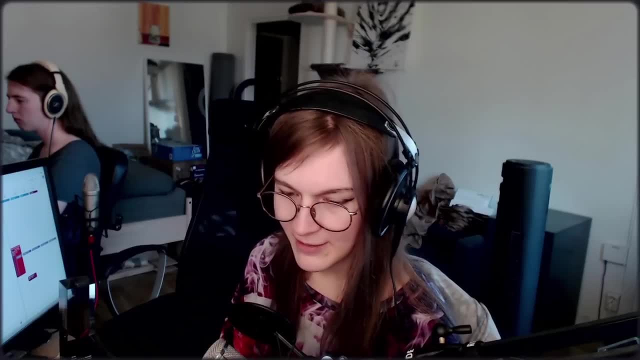 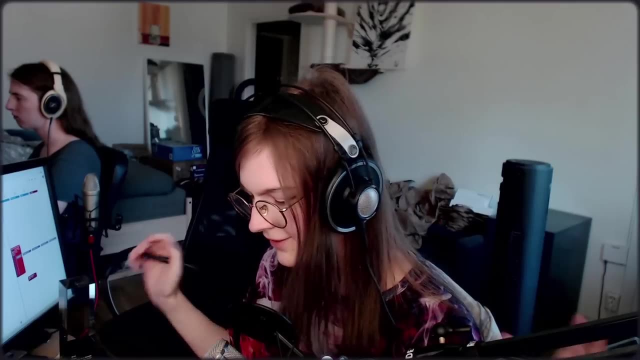 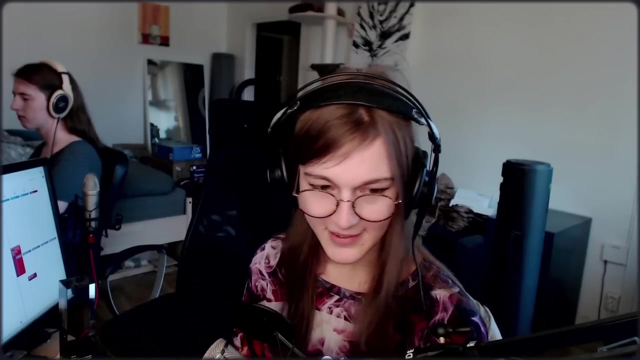 So, like generally in game dev, unless again you're coding a game engine, you're going to be using existing physics packages. you're generally going to do things on a per-frame basis. so like, the understanding of it is really important, but to actually derive equations isn't that important. 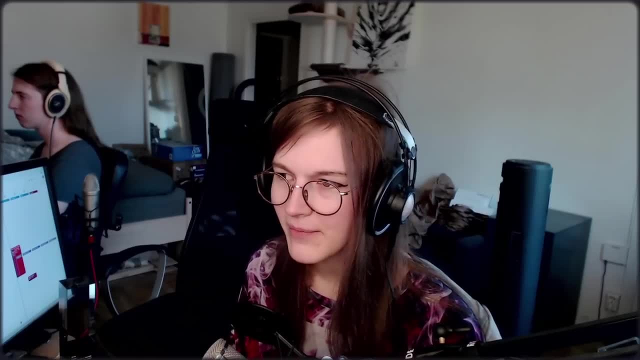 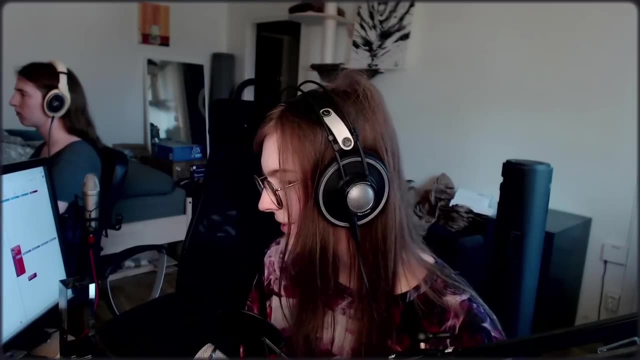 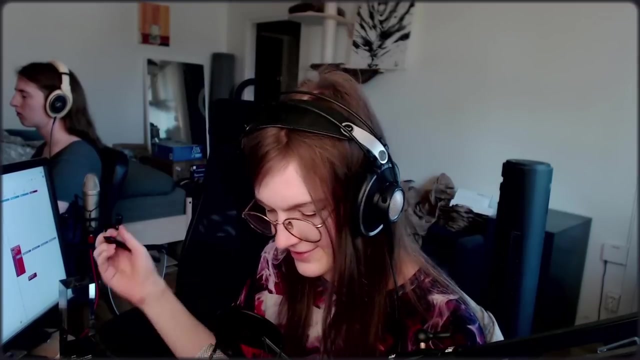 Sometimes you will run into it, but I don't think I think I might have run into it like once or twice throughout my career. but, yeah, understanding it in terms of like- yeah, like you mentioned, like timedeltaTime that we're going to go through because that's really important- but in terms of like actually deriving equations, eh, you don't really do that much. 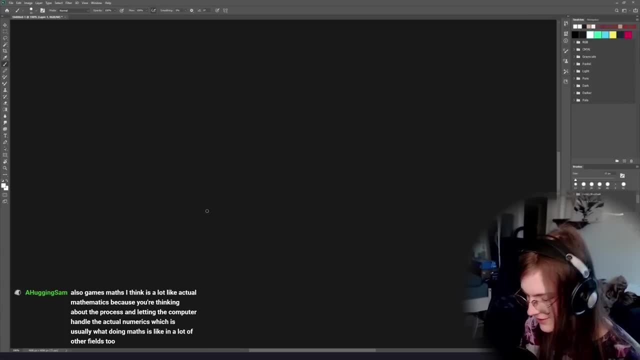 So I feel like there is a concept that is talked about very early on in your math course. Usually it's referred to as the number line, So you can imagine this Like one-dimensional space. We can just move along this one line, right? 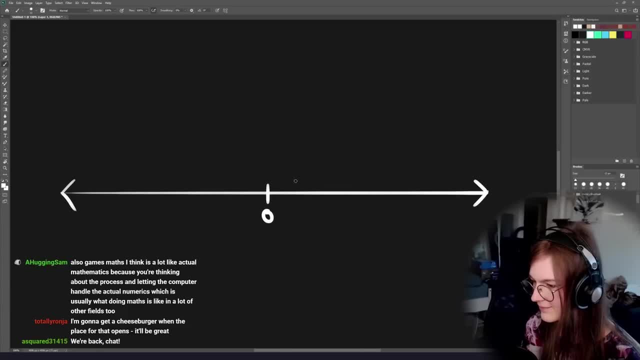 And in the center we can put the number zero right, And then you can sort of imagine a space where these numbers are kind of put along this whole line right. All right, so we have one, two, three, so all integers are on these little notches. 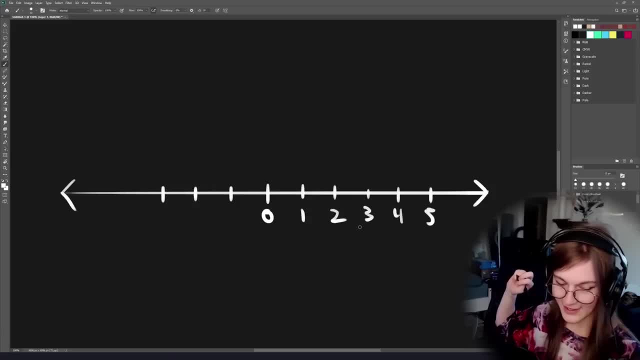 All right, cool. So this is a number line, It's like I think it was. like usually This is mentioned very early on in your math courses and then it's kind of like forgotten. But I think it's an extremely useful place to be because it very like beautifully illustrates kind of the continuity of numbers and like where the integers are and so forth. right, 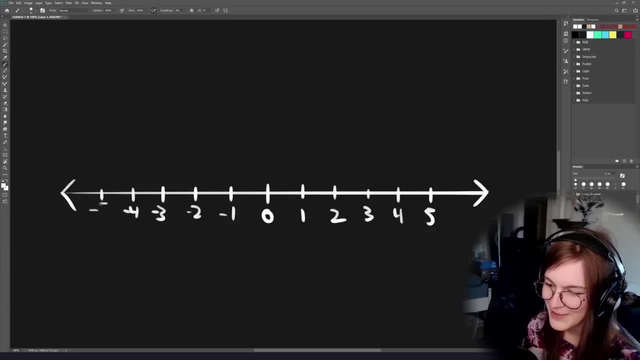 I hope I got these numbers right. I feel like I'm going to make so many weird mistakes. So, all right, This is correct. right, Okay, cool. So we have zero in the center, And then one, two, three. 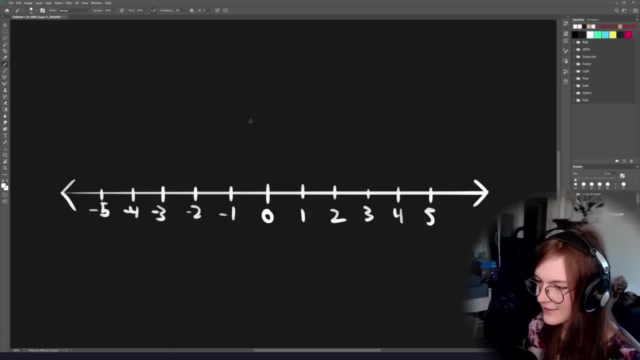 Four five. So we have our positive numbers on this side and negative numbers on this side, And this continues to positive infinity. This continues to negative infinity, right? So this is a useful way of thinking about it, because you can have numbers that are between the integers, right? 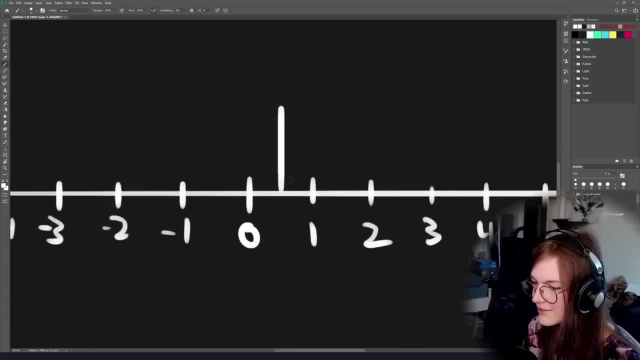 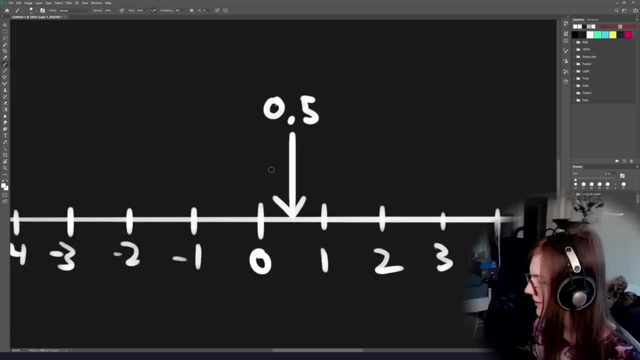 So these whole numbers are integers, And then between those you can have decimal numbers, right? So you have 0.5 here, So that's halfway between zero and one and so forth, right? Okay? So now one thing that's very important whenever you're working with math. 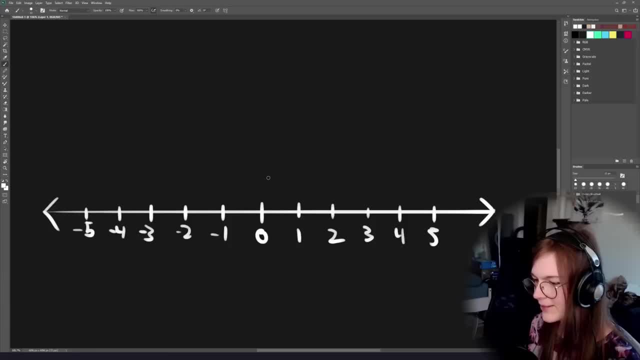 especially in game dev is not to really think about numbers in terms of just being numbers, Because numbers is only there to represent something else, right? So then you can ask like okay, what is this number? What is it like? what is it a substitute for right? 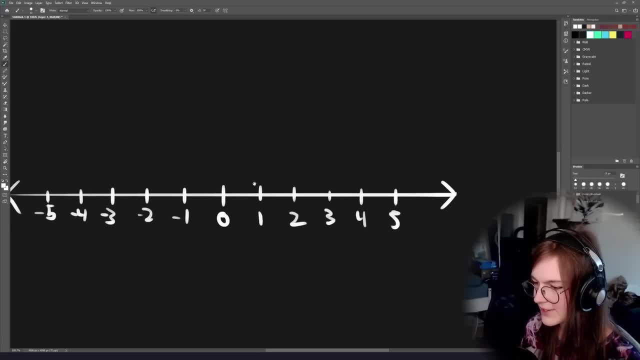 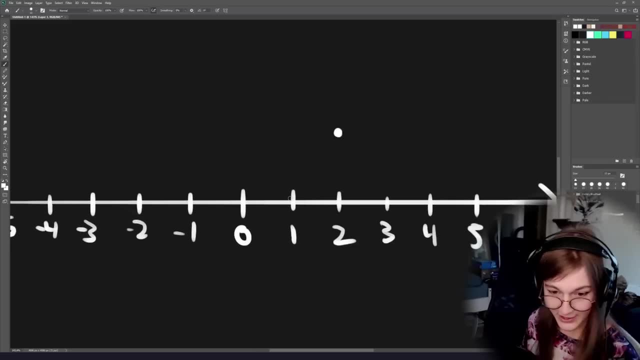 And what is it representing? So usually if we have a number, let's say we have number two And we can mark it with a dot there. So what does two mean here? Well, we could interpret it in many different ways. 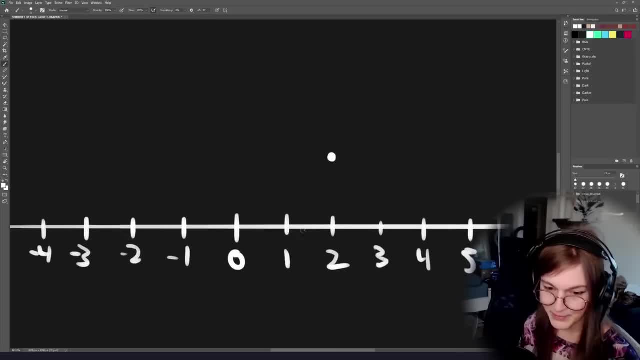 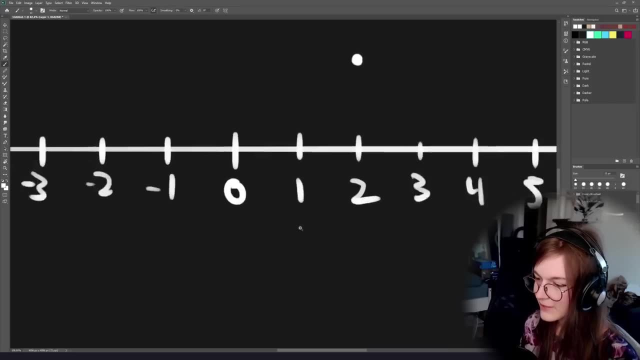 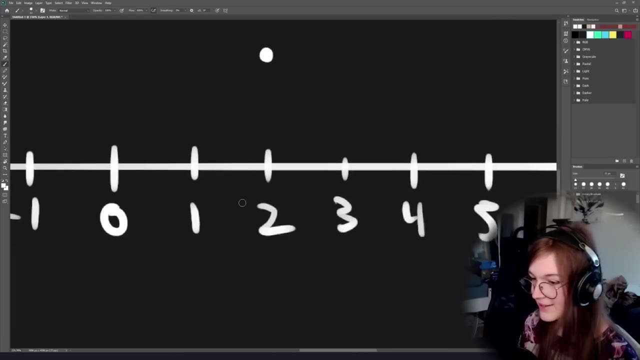 Two could be. it could be a position, right. Maybe this is the position along this line, In which case this is going to be a coordinate system, right, Where every number says the position on this one dimension right, So we could call this the one x-axis right. 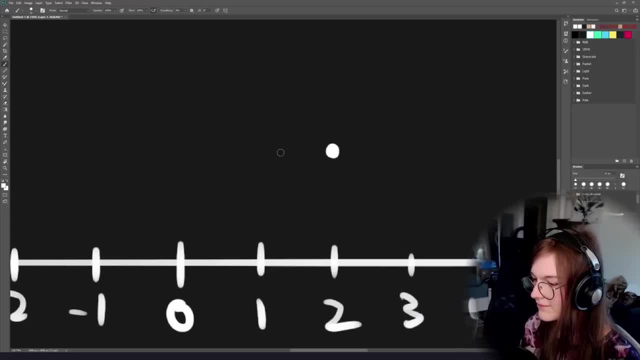 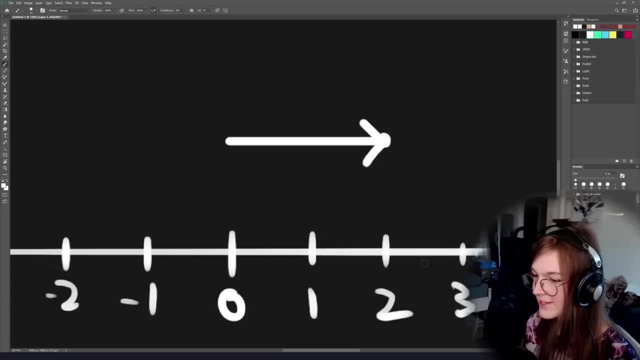 So this could be interpreted as a position. We could also interpret it as a vector right. It could be an arrow, usually going from zero, because vectors don't really have a root of quote-unquote the arrow, They only have a single point right. 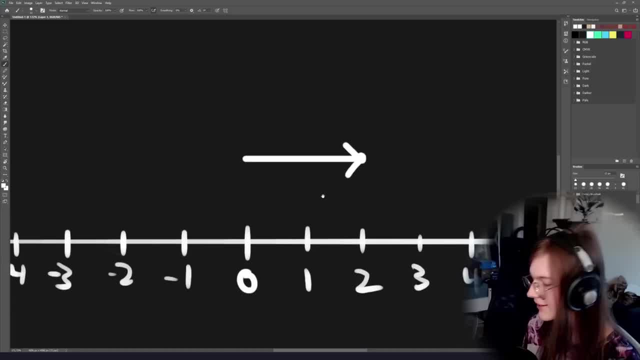 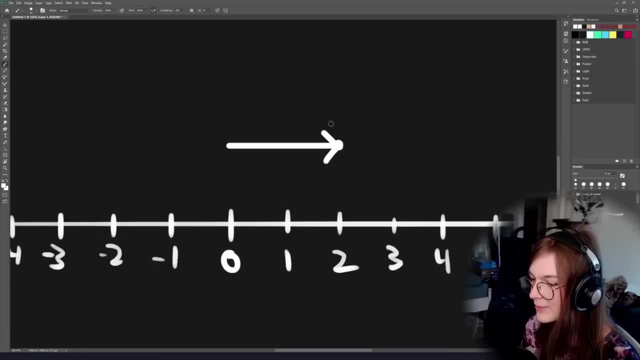 So this is a vector. It just has the value two right, And because it's one dimensional, we can only have vectors that point either to the right or to the left right, So we can interpret two as a vector. 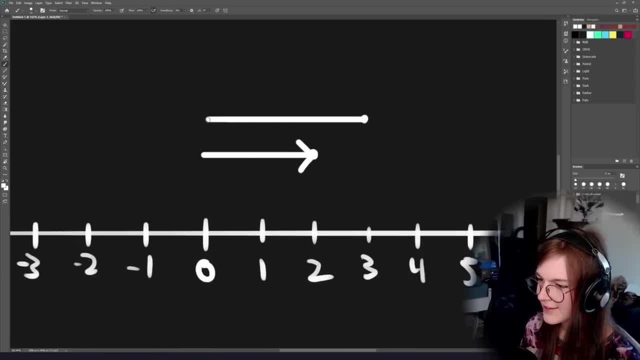 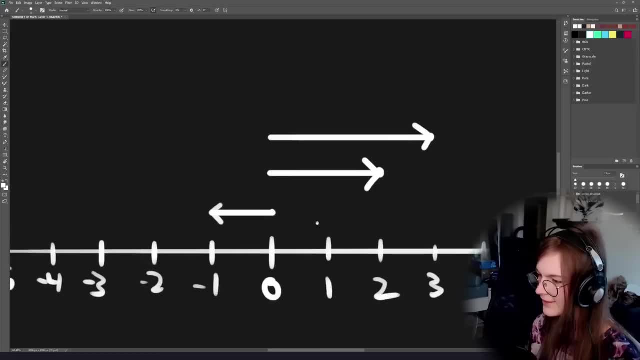 We can do another number, Let's put three here, And then this is another vector. We can do another vector for negative one, right? So this is one, So this is one. So this is sort of a one-dimensional interpretation of vectors. 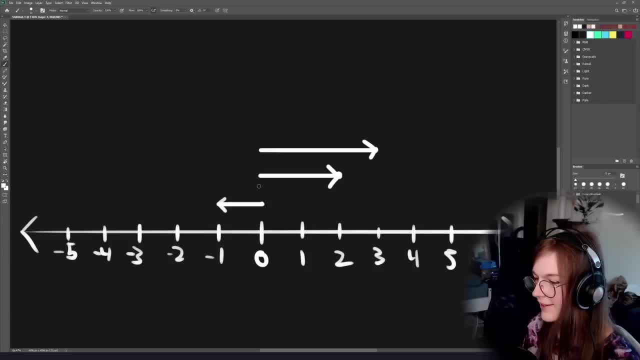 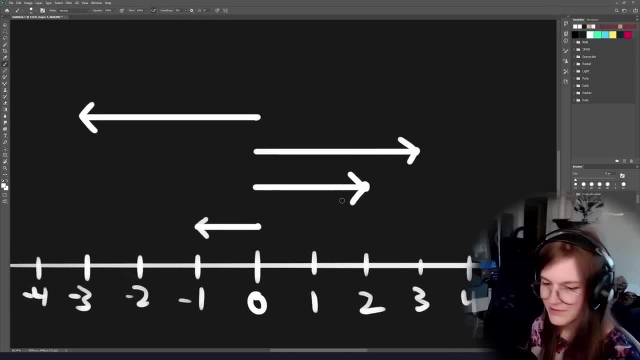 But then we can ask like lots of questions about these, right, We can ask how Let's do another vector. actually Let's do negative three, Okay, So usually when you work with vectors, you work with a lot of concepts. 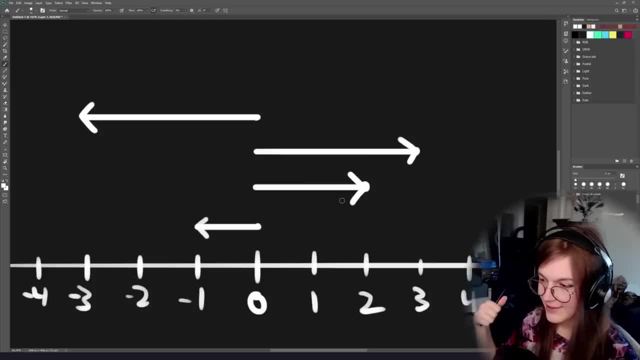 in terms of like, length and direction and that kind of stuff, And usually you kind of start doing that once you go to two dimensions. But all of these things exist in one dimension too. This is not exclusive. This is not exclusive to like two dimensions and above right. 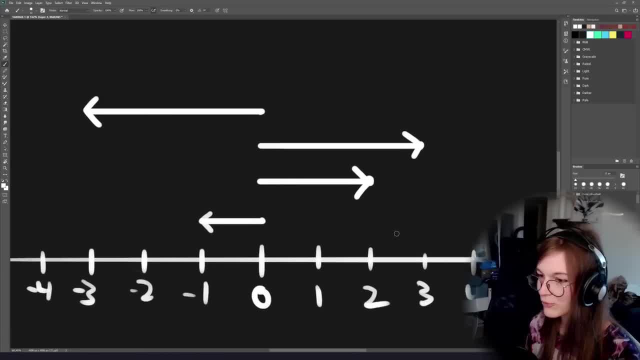 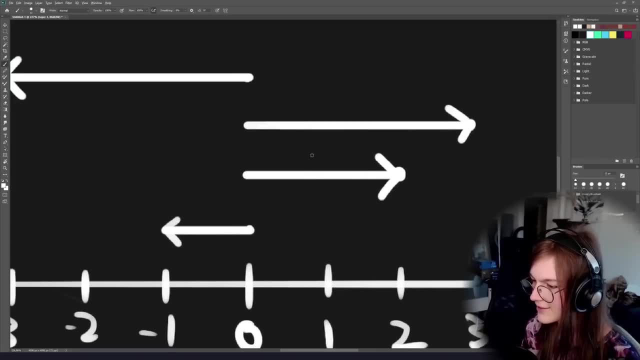 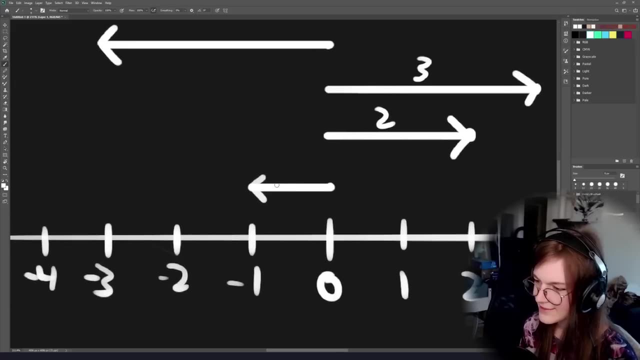 So, if you look at these vectors right here, what is the length of these vectors? Well, this one that's pointing to two, this one has a length of two, right, This one has a length of three. But if you go to these, these also have a positive length, because lengths are always positive, right. 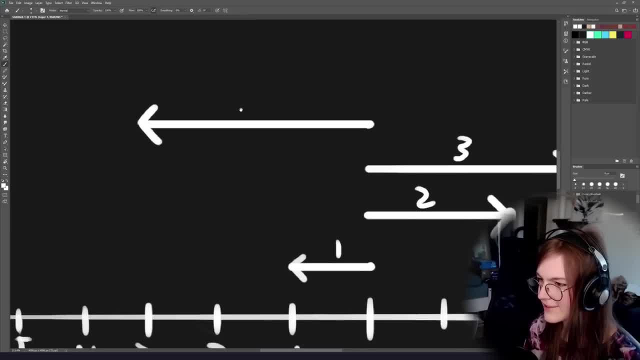 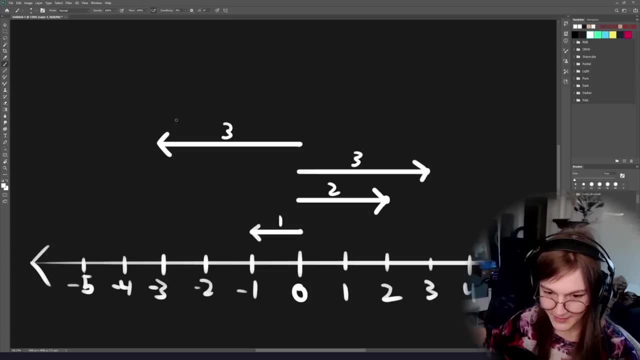 This has a length of one. This one has a length of three as well, So, yeah, So this is basically just a one-dimensional interpretation of what vector length is right. Also, I didn't draw these exactly the same size, but you know what? 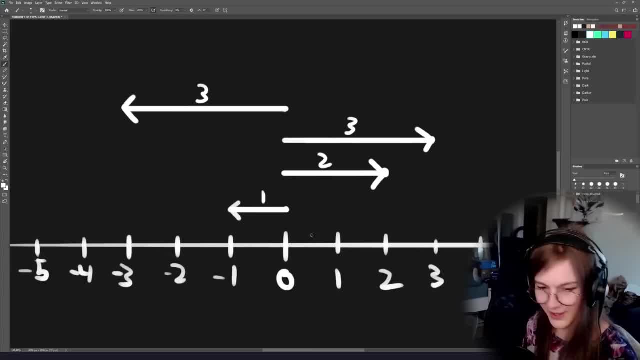 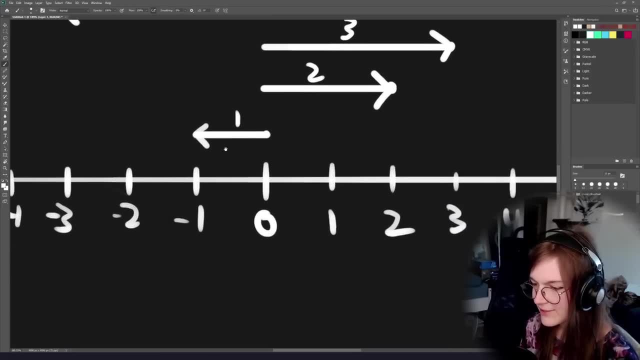 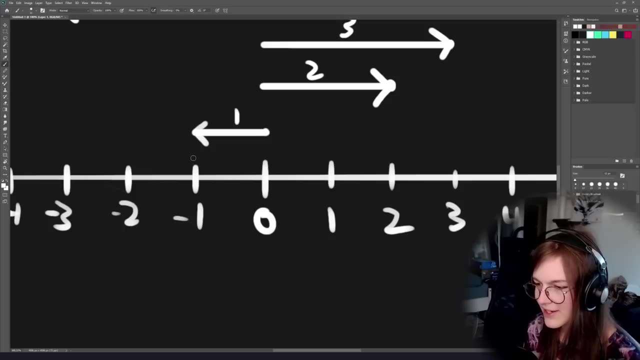 That's okay, You get the idea, I hope. All right. So what about direction? What is the direction of these vectors? Well, if you think about direction in one dimension, usually directions have a length of one. So in one dimension you can only have direction. 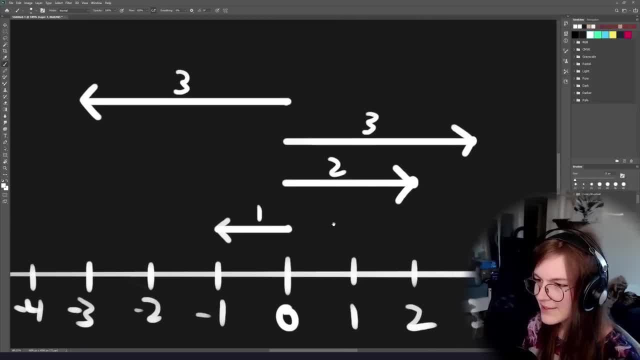 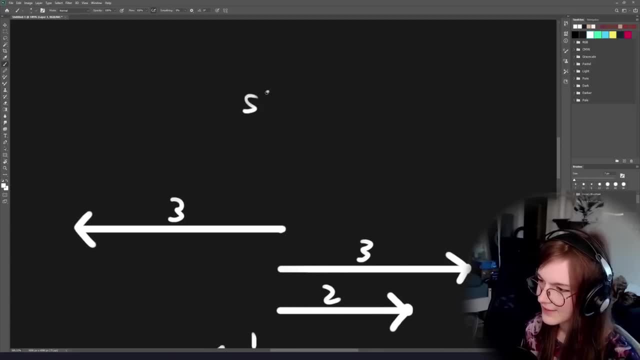 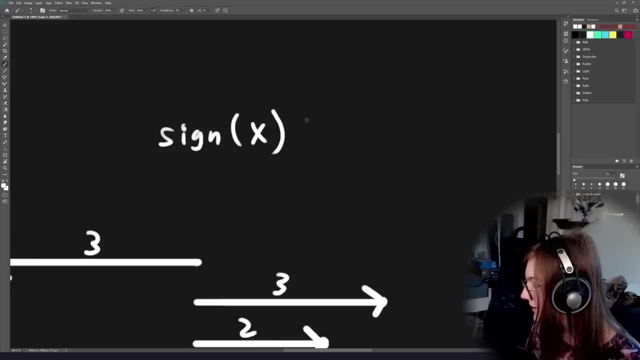 So you can only have directions that are either negative, one or one. Sometimes that's usually called a sign. When you're working in one dimension, usually it's called a sign Sine of x. So usually this is the one-dimensional direction, right. 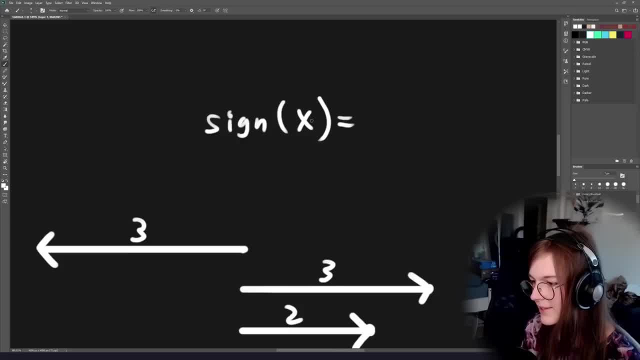 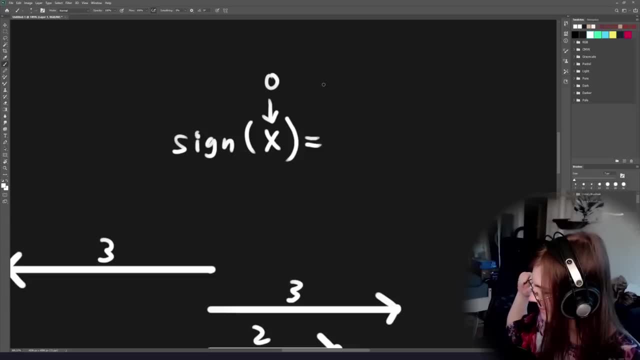 Basically it's only positive one or negative one. There are some exceptions, if x is zero. If x is zero, then it kind of depends on the implementation. In some cases it's going to throw an error, In some cases it's just going to return one, and so forth. 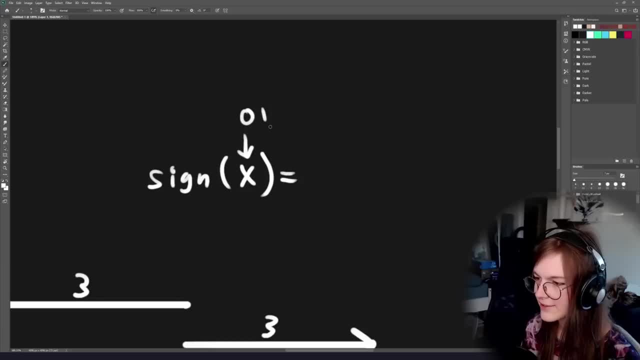 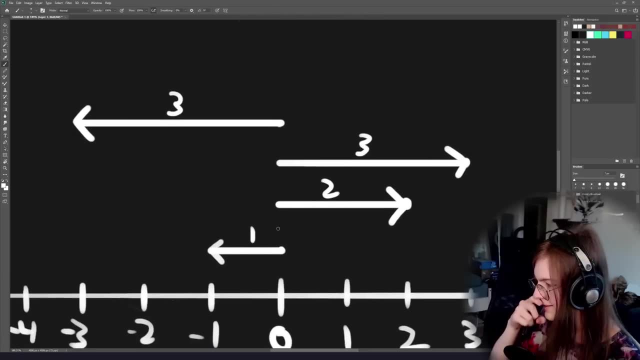 But usually it'll either return zero one or an error when you pass in a zero Anyway. so the sine of these numbers is the direction it's pointing pretty much, And if you want to get the length of these actually, maybe I should keep the sine of x. 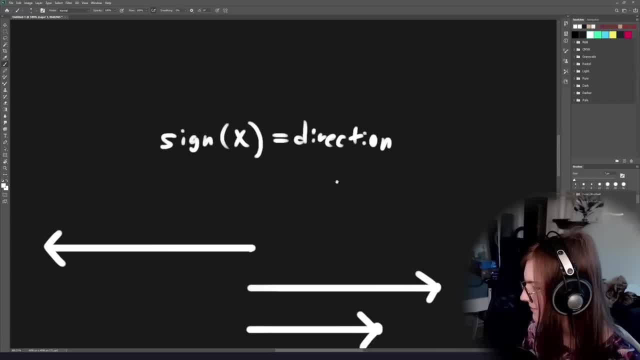 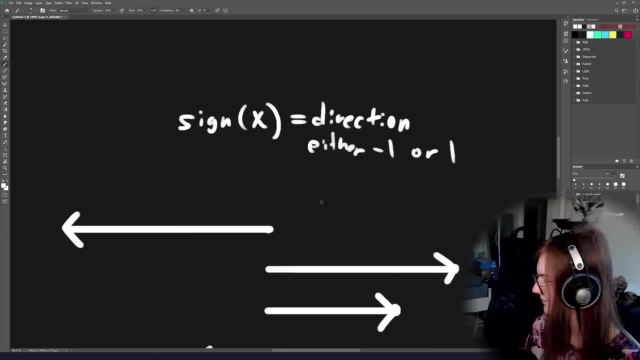 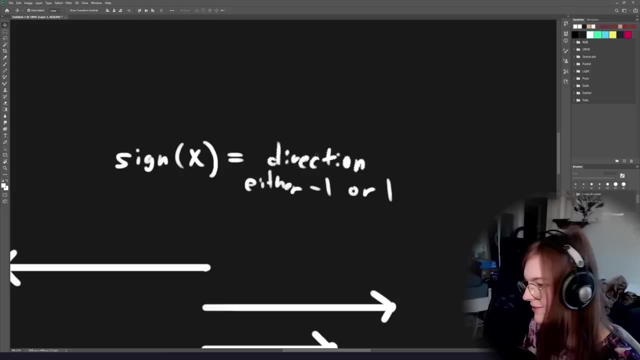 This is basically the direction. So this is e Either negative one or one Mostly random rambles in the student chat. No questions yet. So zero vector has no direction. Yes, It sort of like. depends on your implementation and interpretation of like what it's used for. 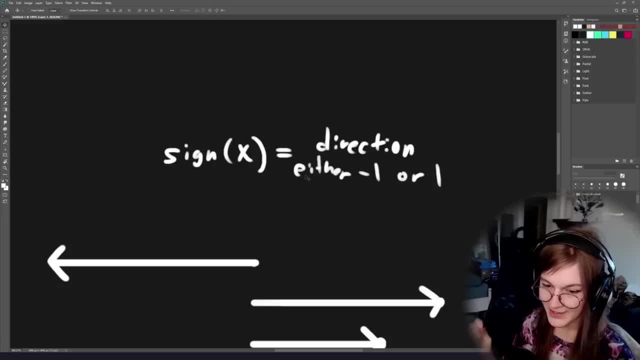 Like. in some cases it is useful to interpret the sine of x to be one, Because quite often you use the direction to multiply something, To like sort of change the direction and then scale it by some value And sometimes, when the value you're checking the sine of is zero. sometimes you want it to be a one. 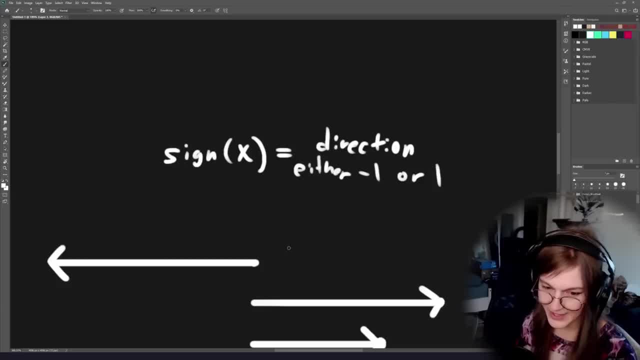 But generally it depends on, generally it depends on like the case, right, But again the like, purely mathematically, a zero vector doesn't have a direction. as far as I'm concerned, All right. 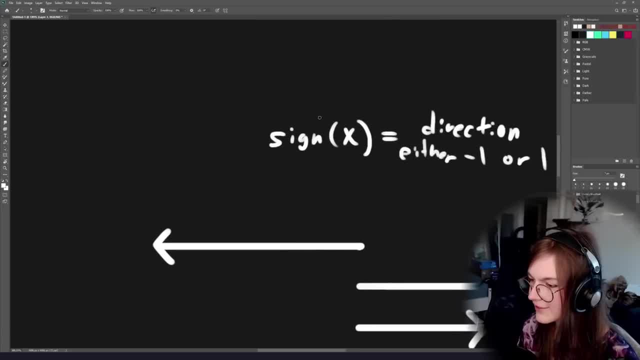 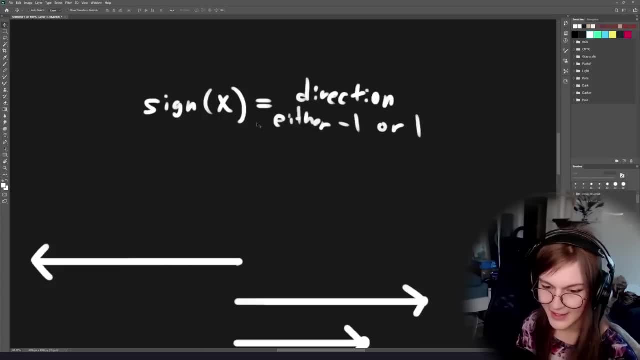 So this is kind of the direction of a one-dimensional vector. It's usually called a sine, Again, for one dimensions These are sometimes called scalar, scalar values and so forth. Then again, the length we talked about like the length of these vectors. 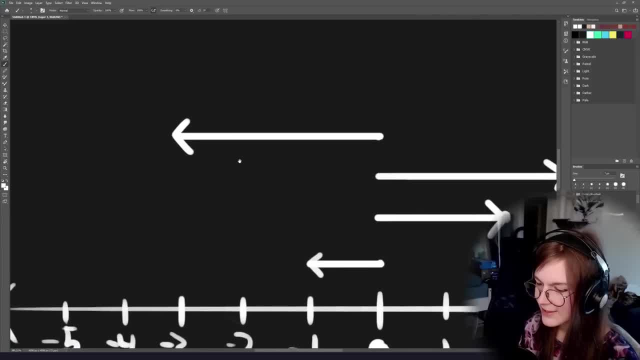 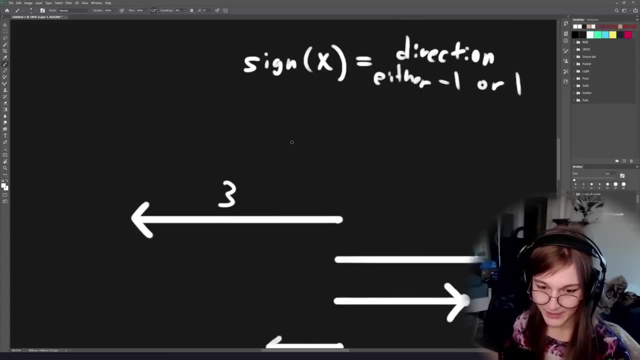 Because the actual values of the vectors, like the value of this one, is negative three, right, But the length of it is three. So to get the length of a number, you basically just you get what's called the absolute value. 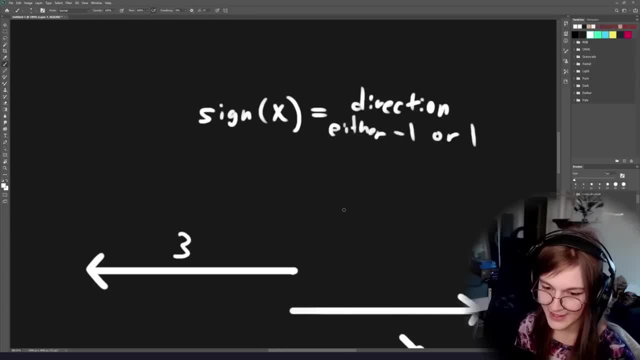 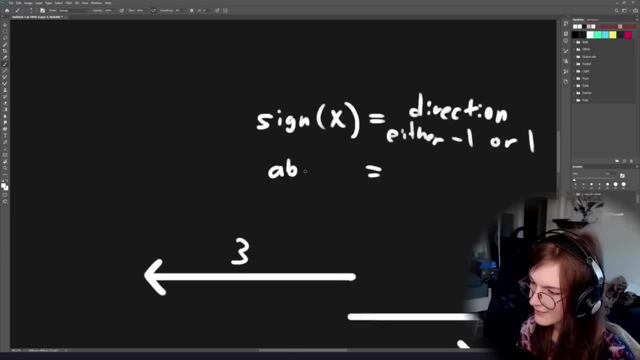 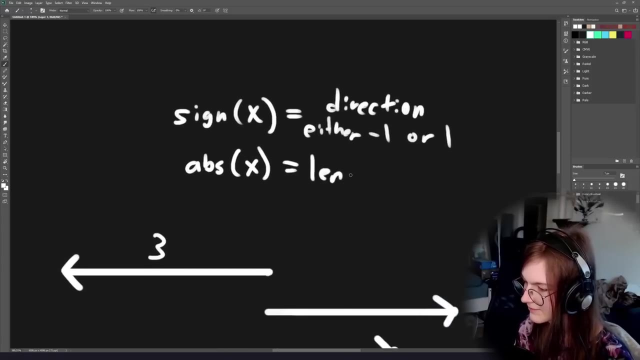 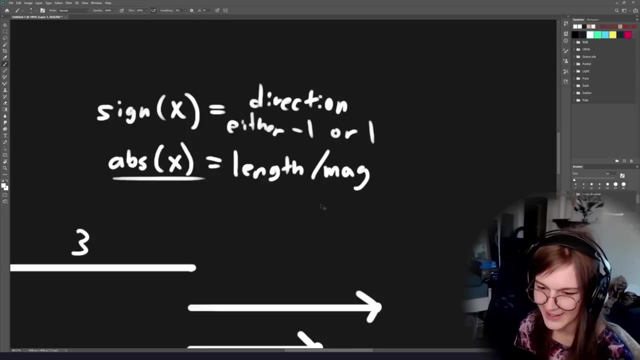 Which is just a fancy way of saying: if it's negative, make it positive Like that's it. So the absolute value Usually abs. in your math libraries. That's the, that's the length, Sometimes called magnitude, But I feel like I'm the only person in the world that calls abs for scalars magnitude. 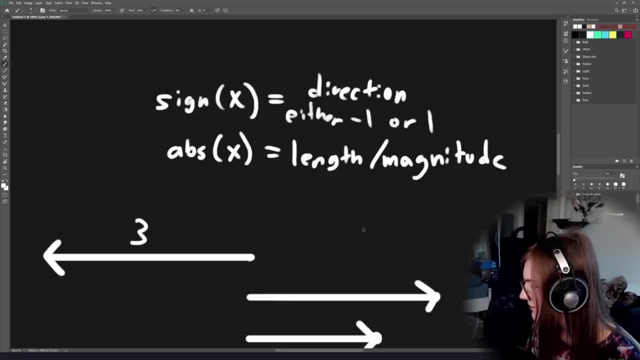 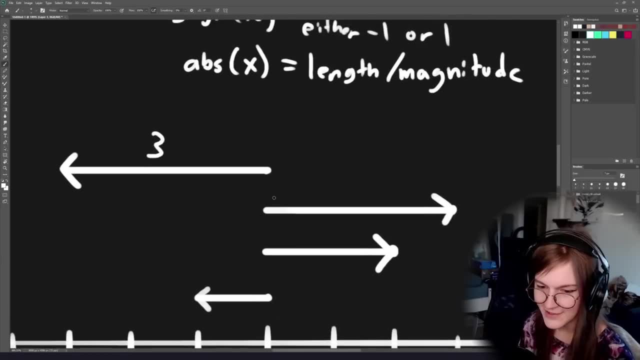 But I think it's funny: If sine x can only return one number, why not use a float? It does return a float. We are not talking about two-dimensional vectors yet. We're only talking about one-dimensional values, which is floats or a scalar or a single value. 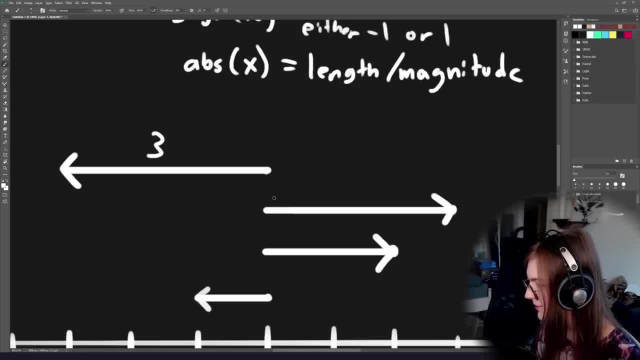 So we're not. we haven't gone into two-dimensional or three-dimensional vectors yet. Can you sine a 2D vector? What if the vector has one negative value and one positive? So generally the general case of a sine is that it gets the direction of the vector. 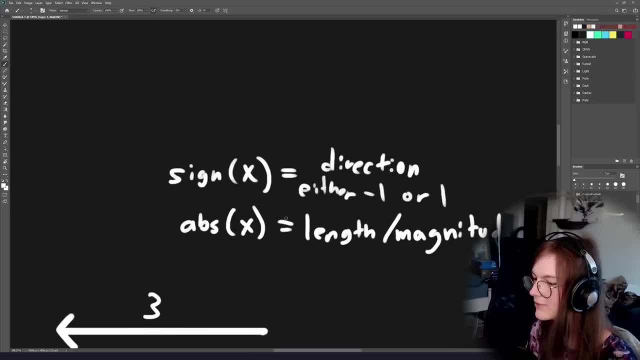 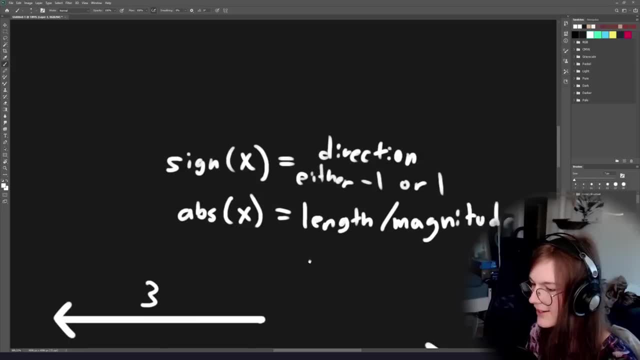 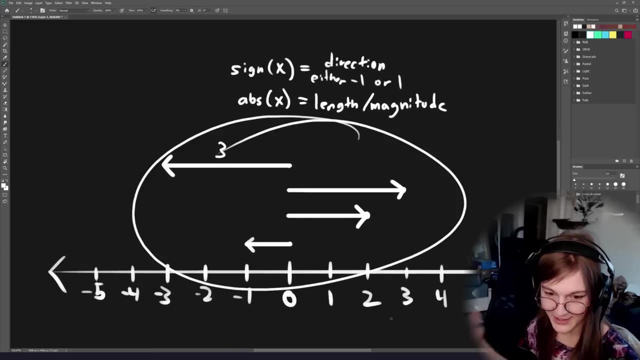 The sine of a two-dimensional vector would be itself a vector, right, Because it's a two-dimensional direction. But we're going to get into 2D vectors. I just want to start out with one-dimensional stuff, But I think it's kind of neat that you can have a one-dimensional interpretation that is still vector-based. 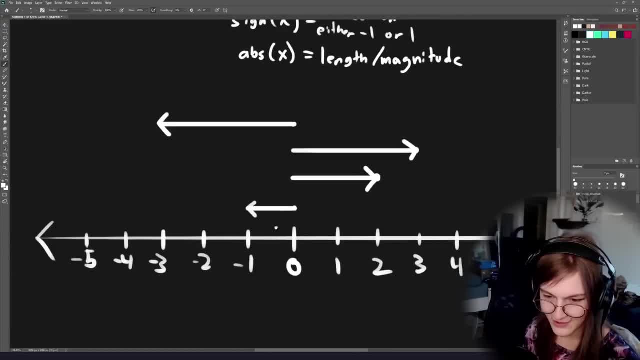 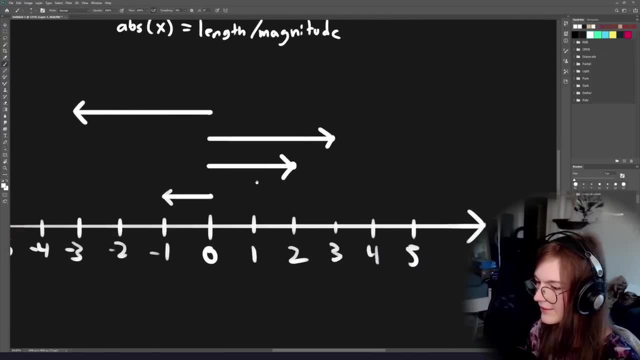 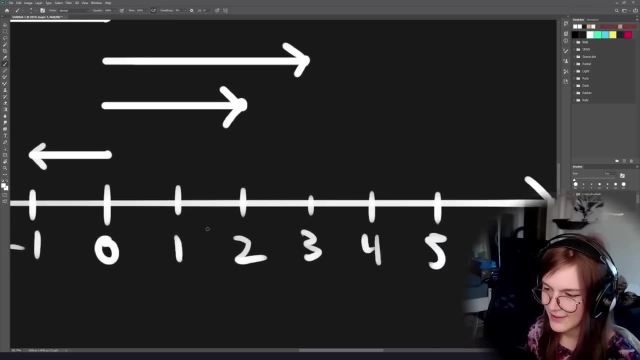 So we're still just on the number line. We don't have any two-dimensional vectors here, All right. So then we can ask a lot of questions Like: what does it mean to, let's say, you ask some question like what is the distance between? what's the distance between 1 and 3?? 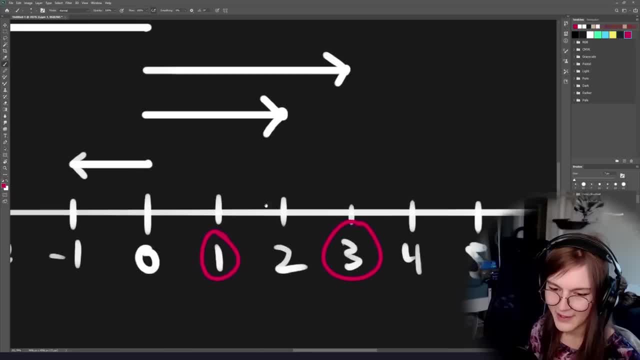 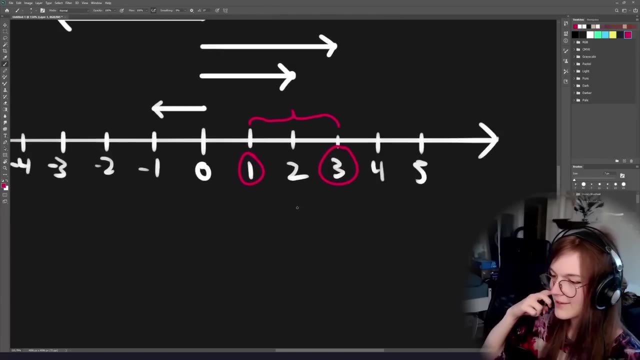 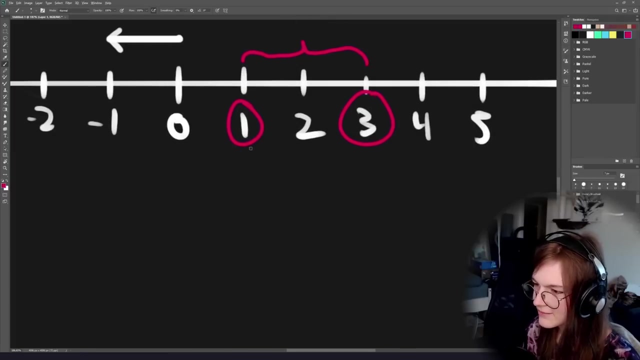 Like, what does that question mean? Well, generally a distance would be: we want to get this length here between these two numbers, So that would be a way to get the distance right. So if you want to do, if you want to get the distance between these two numbers, then generally you would have the two numbers represented as like: well, we could represent them as just letters, right? 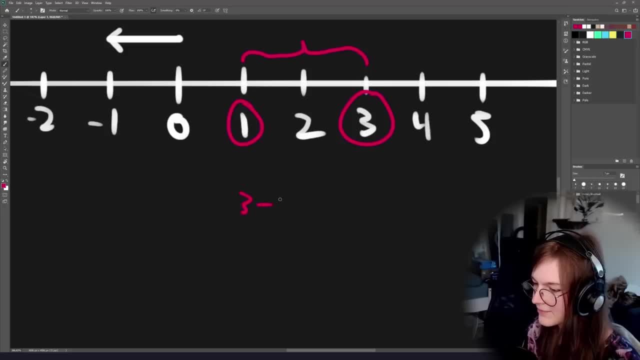 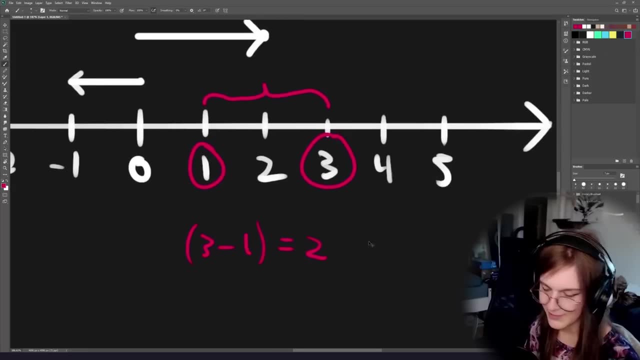 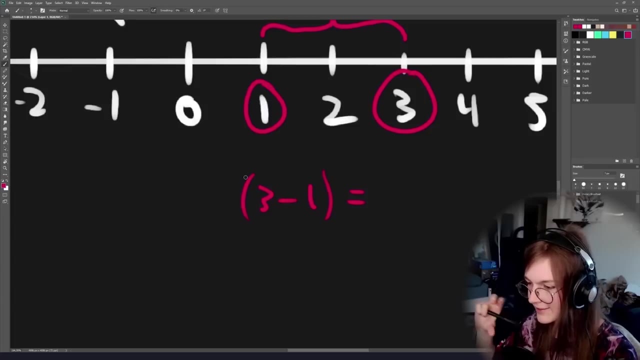 So in this case we want to do 3 minus 1.. And then that gives us 2, right? So then we get the distance between these two numbers. So usually doing like subtracting is usually it can be interpreted as getting the difference between two values, right. 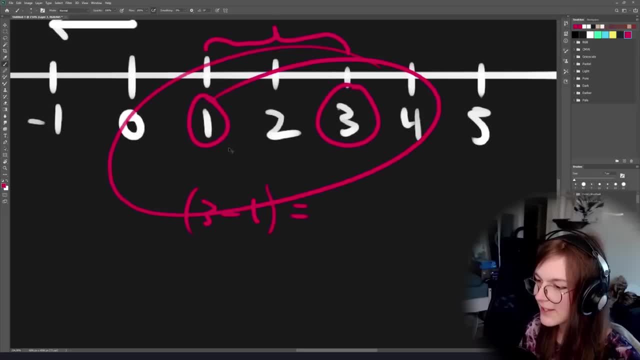 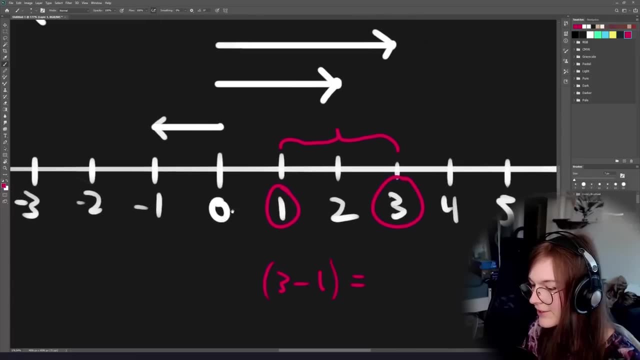 So if we want to get the distance between these two values, generally you do 1 minus the other. But if you like, flip the order of these. if you do 1 minus 3, you're going to get negative 2, right. 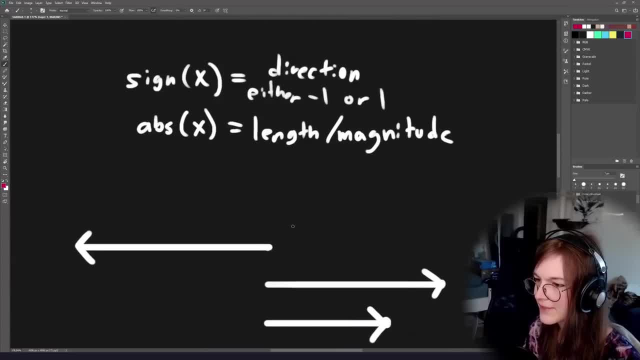 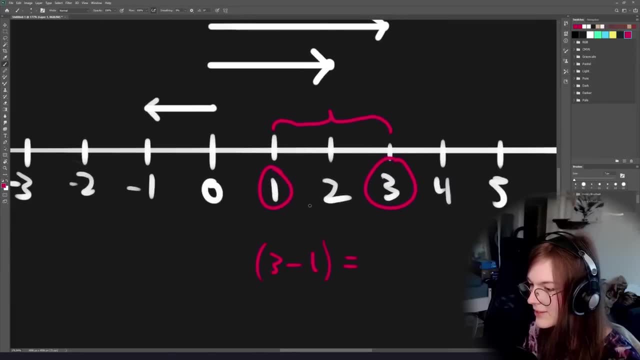 So in this case, we actually want to. we want to make sure that we get the length and the magnitude of this right, Because if we do 3 minus 1, what that gives us is that we basically take this vector. 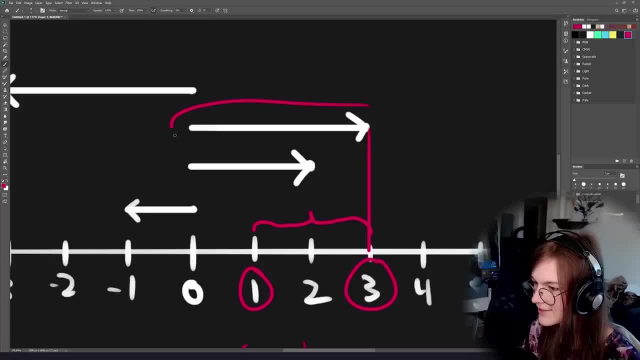 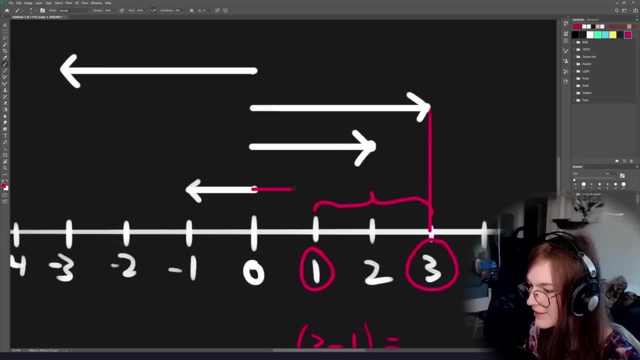 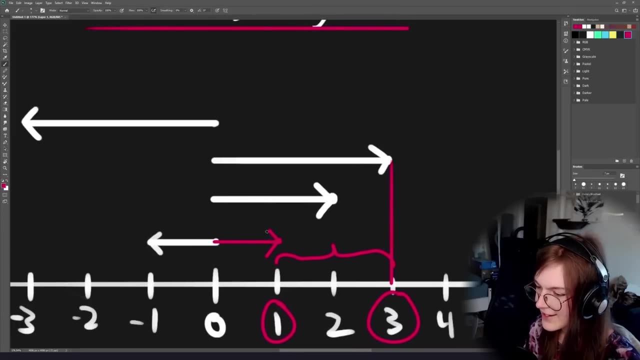 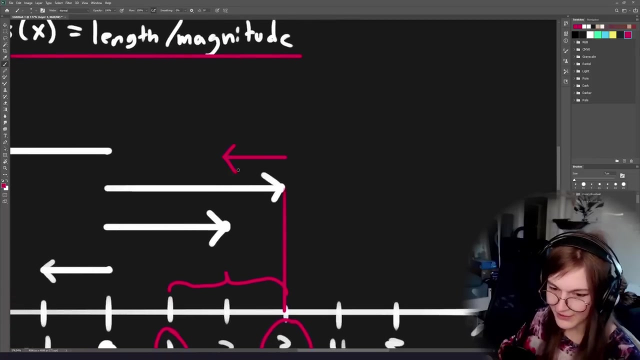 This is 3, right, Because it lines up here. This is the one-dimensional vector representing the value 3.. And then we want to subtract the vector 1.. And the vector 1 is this vector right? And the way to kind of interpret subtraction is that you can sort of take this arrow and you can subtract it, as in you flip the direction of the arrow. 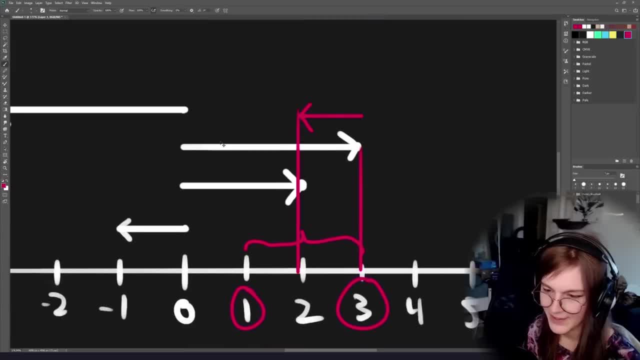 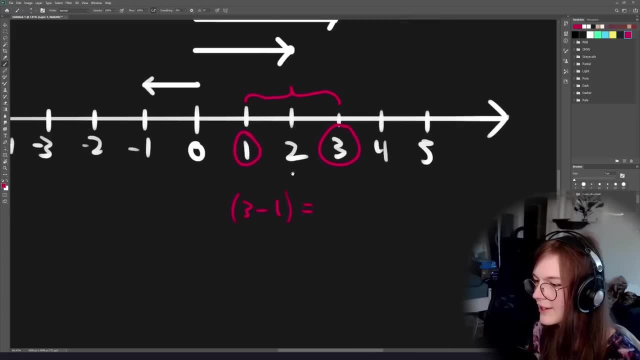 And then you get a new value that stops here, right, And that's going to be an arrow that goes here And this is the value 2, right, All right, So, but then again, this is order dependent. This presumes we have the 3 before the 1.. 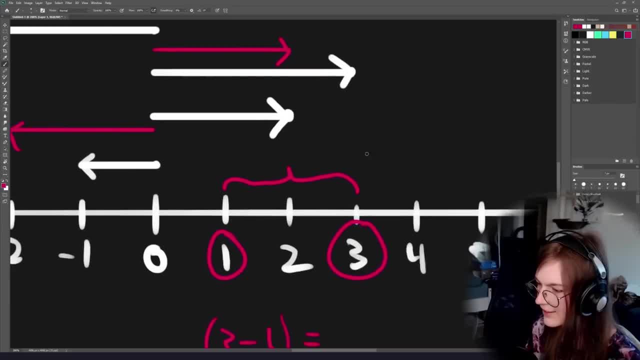 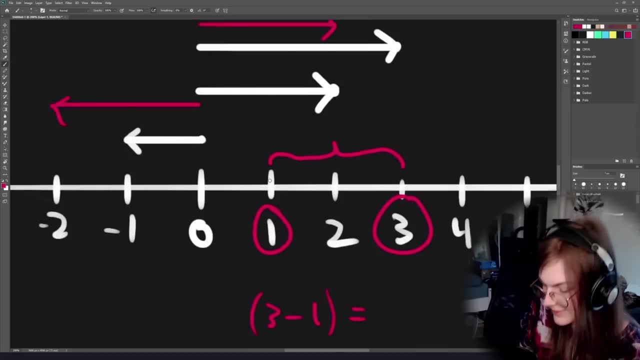 Otherwise we're going to get negative 2.. So if you ask the question, what is the distance between these two values? If you say negative 2, that's going to be a bit of a weird answer, Depending on the implementation. 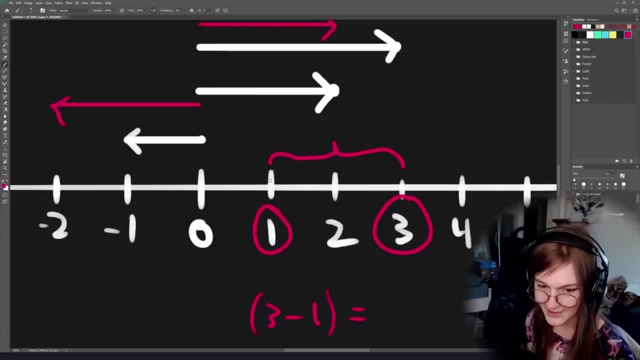 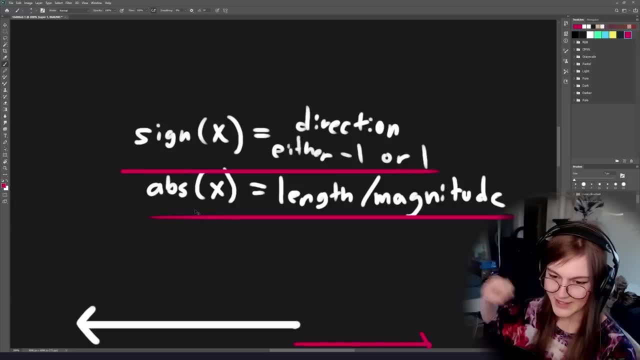 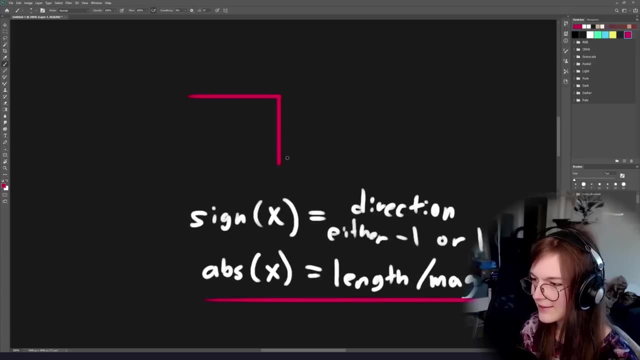 There are some cases where you want to get what's called a signed distance, And again, signed distance is referring to the fact that it can be either negative or positive, But generally distance values are always positive. Same thing with area, If you want to get like the area of some polygon. 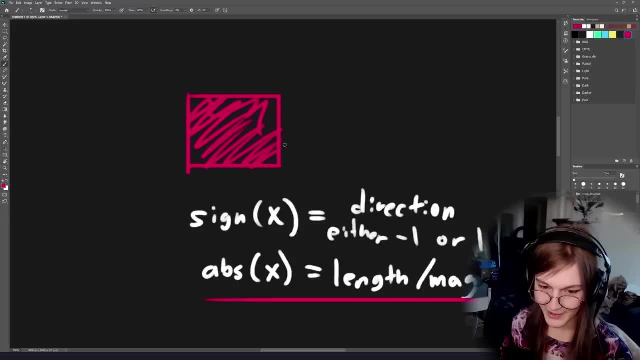 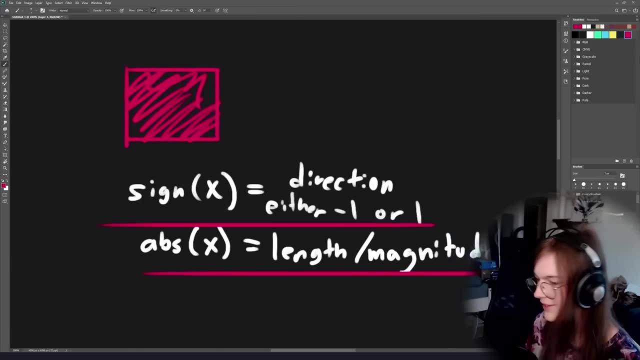 Then the area is considered to also always be positive, Except if you want a signed area. So a signed area just means that it can be either negative or positive. So you're probably going to hear a lot about like stuff like signed distance fields. 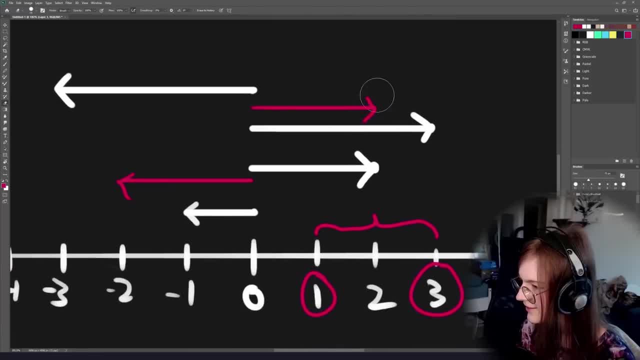 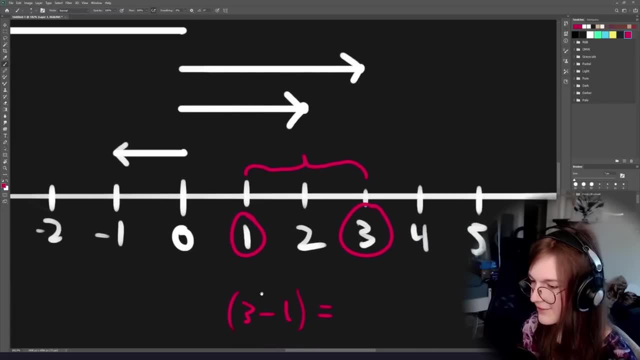 Which is a term that has kind of exploded for the past few months. It's just a fancy way of saying you have a field of distance values that can also be negative, All right. So if we want to get the actual, true distance between these two things, 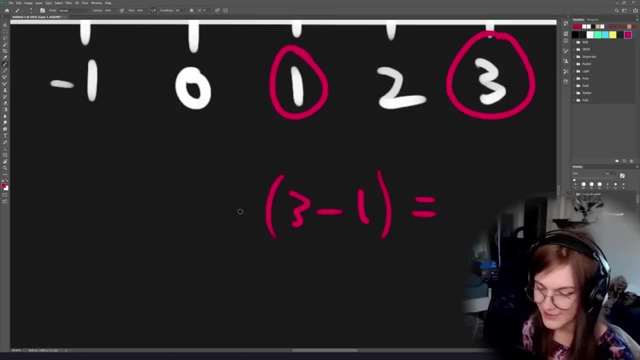 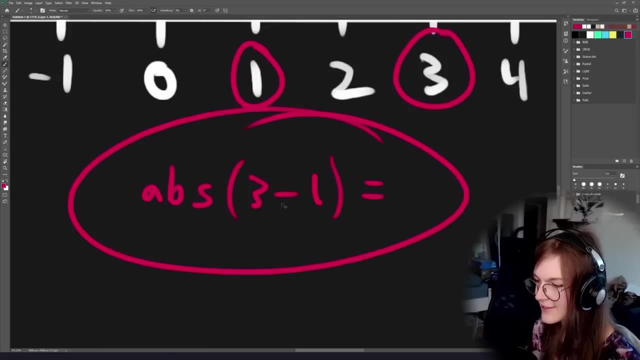 As in the positive distance, We would need to get the magnitude of this right, So that would be the absolute value right. So, generally, this is the way to get the distance between two values. Or, more generally, if we want to generalize this: 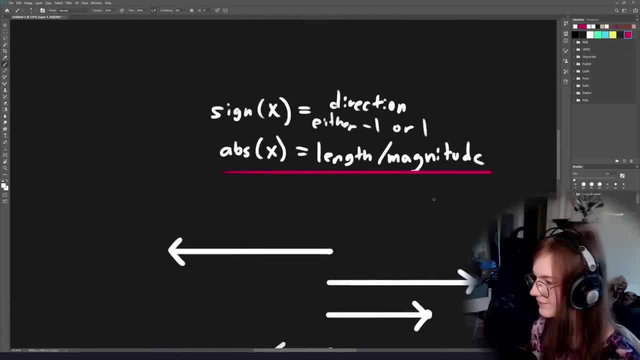 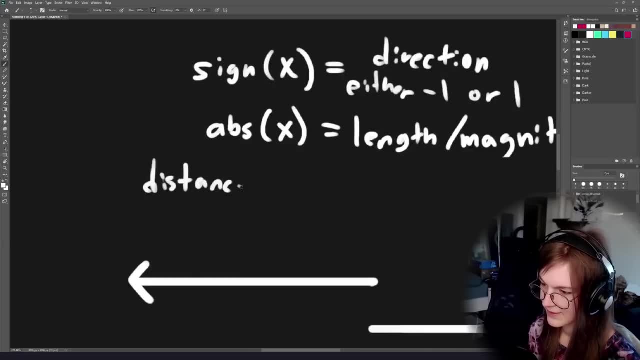 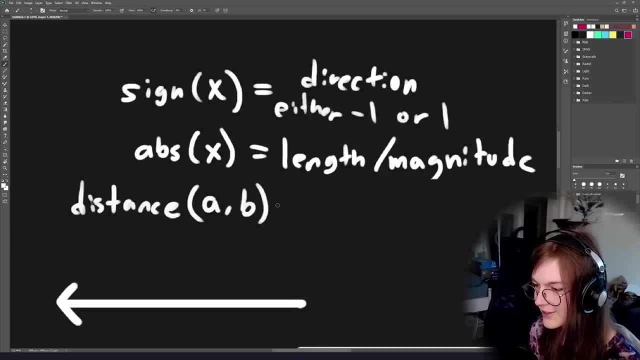 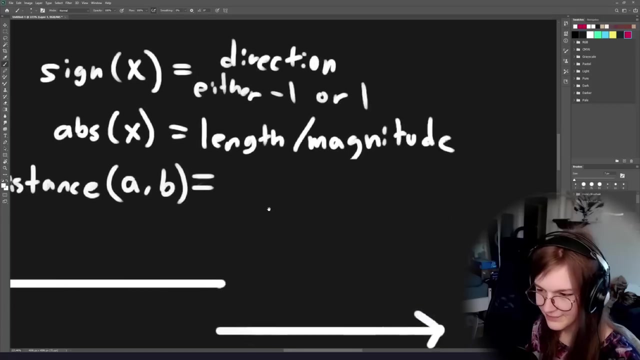 We can say that the Let's see The distance between. Let's say we have values A and B, We're still only talking about float values or scalars, One dimensional numbers. So if we want to get the distance between A and B, 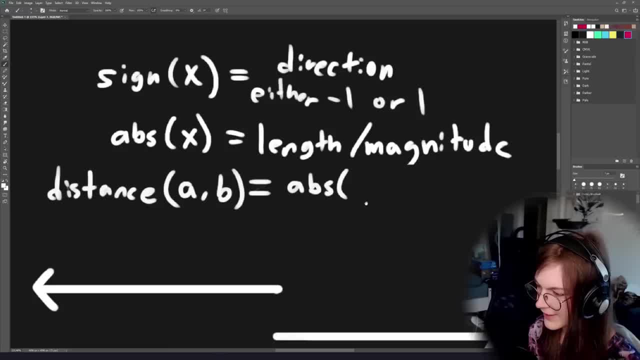 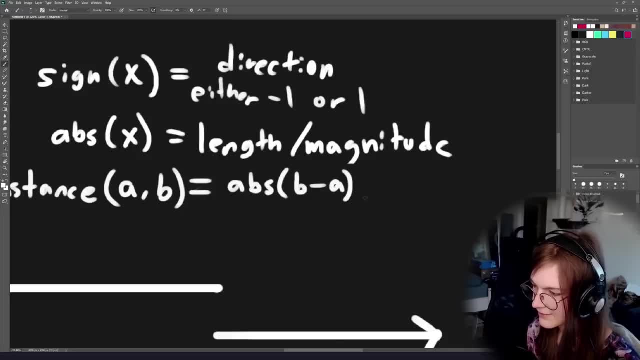 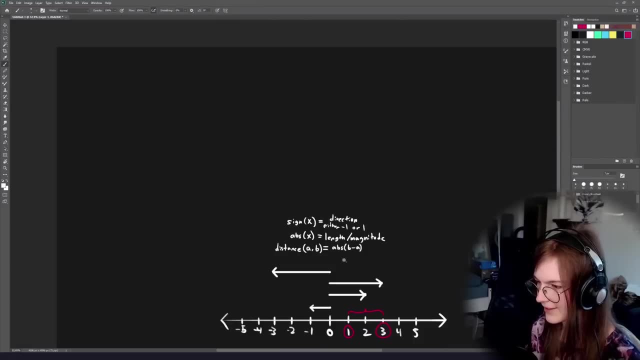 All we need to do is do the absolute value As in the length of the difference between A and B. So now we have the difference between A and B, And then we get the length of that, And then we get the distance value. 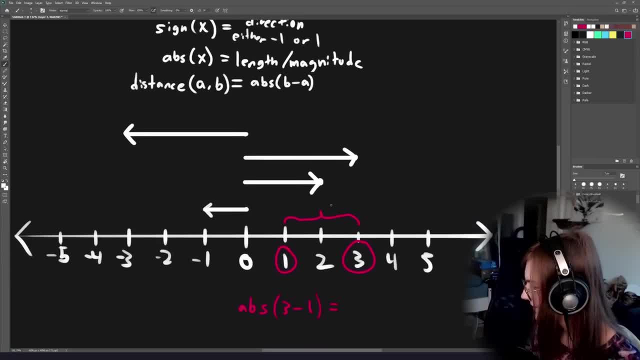 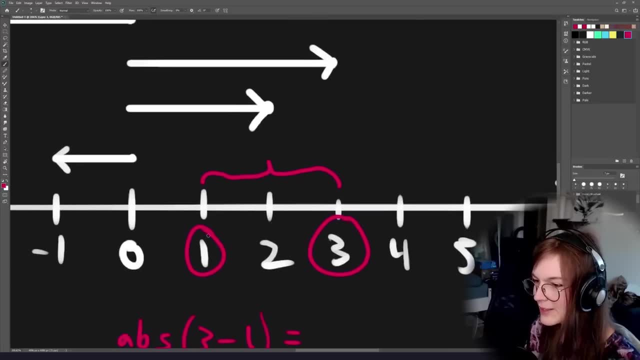 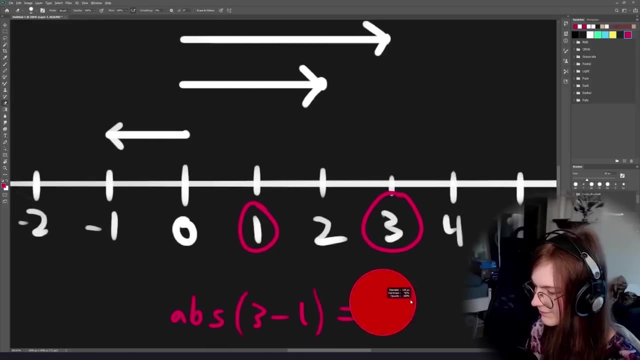 Okay, Everything clear so far. I also realized I haven't talked about addition. That might be a good thing. Addition is probably good to know, So if we want to do 3 plus 1.. Let me just erase things. It's a little messy. 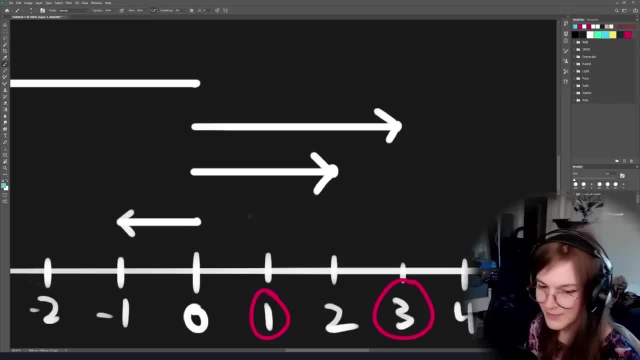 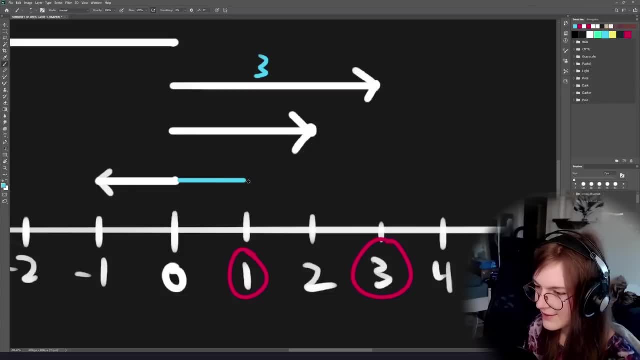 Let's say we want to do 3 plus 1.. Then in a one dimensional interpretation of vectors, Then this is 3. Right, And then we can have another vector. This is 1. So if you want to do 3 plus 1.. 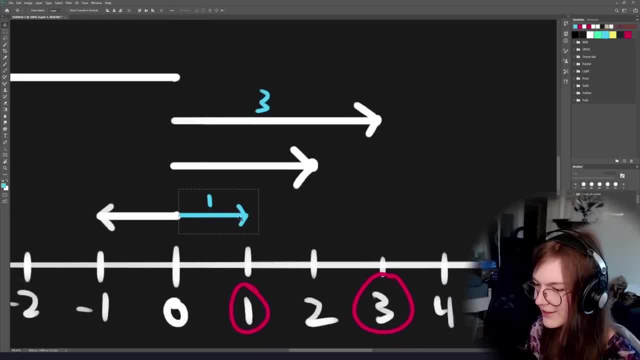 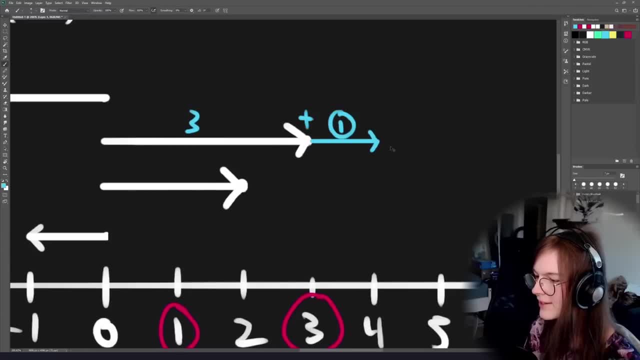 One way of interpreting that is that it's kind of like taking the vector And kind of just adding it on top of the other vector. So now we have 3. And then plus 1. And the final vector. we get out of this as sort of the result of this equation. 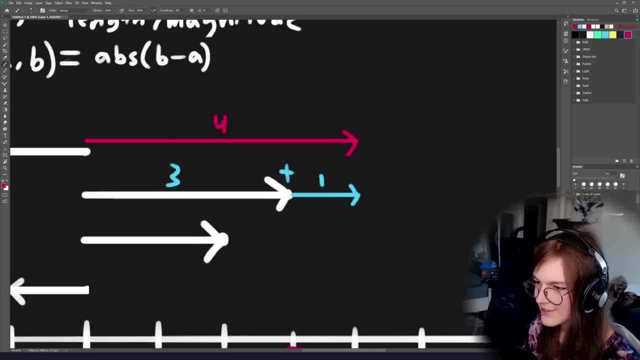 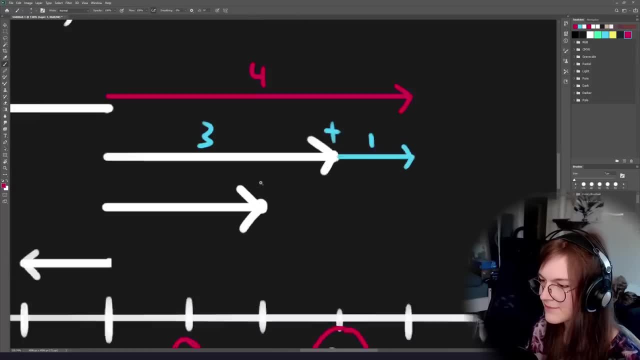 Is this vector Going all the way here, Which is the value of 4.. So that's kind of like how addition works. Previously, we did subtraction when we wanted to know the difference between these two, In which case, instead of adding this to the top, 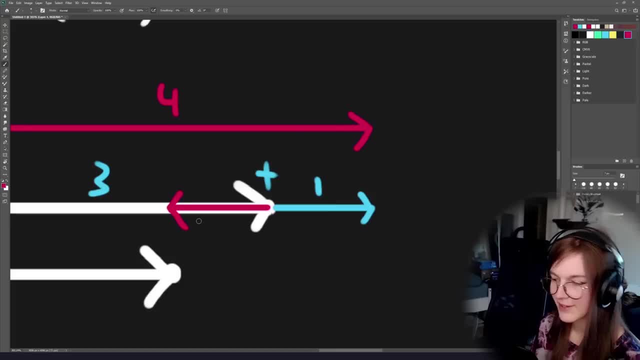 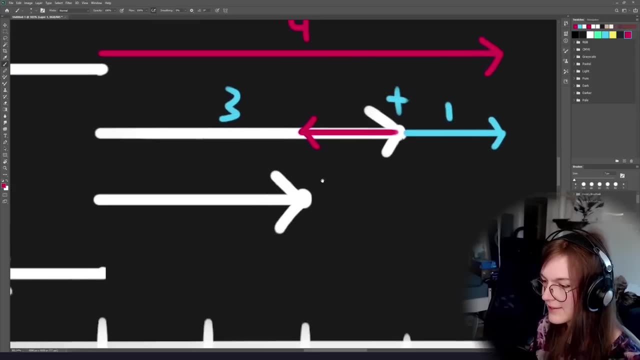 We negate it And then add it Right, Or just subtract it Right. Yeah, So then, doing that, we ended up with a vector at 2.. Right, Because 3 minus 1 is 2. As far as I know. 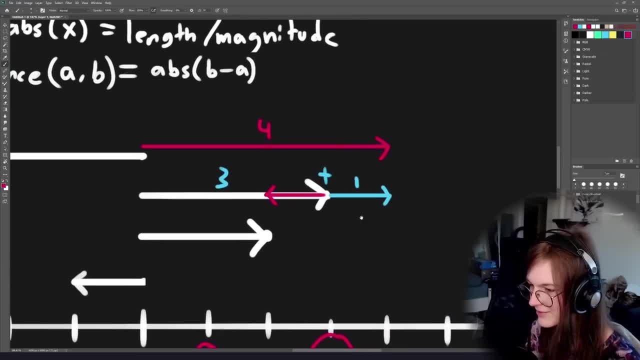 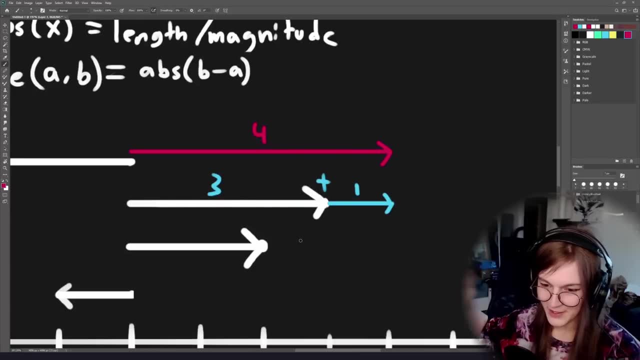 I'm bad at doing math. Like I mentioned before, I might be wrong. Okay, Cool, Any questions? so far, Sorry for the like weird one dimensional vectors, But right now we're only talking about scalars. We haven't gone two dimensional yet. 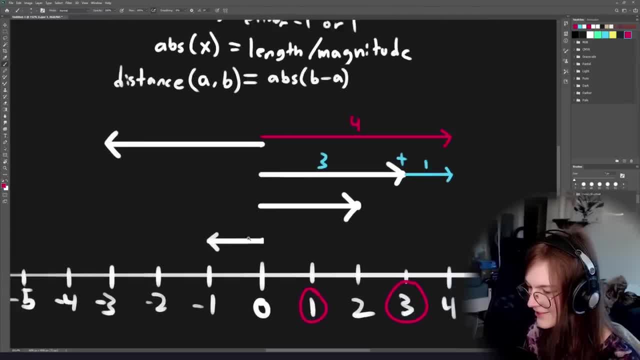 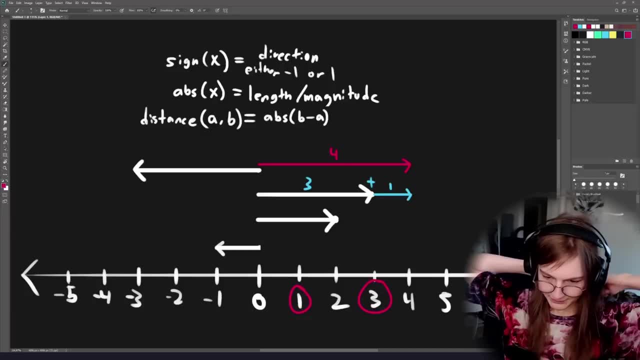 Yeah, So so far we've learned that 3 minus 1 is 2.. That's how well this math course is going. What's the difference between length and magnitude? Nothing, It's the same thing. 3 plus 1 equals 4.. 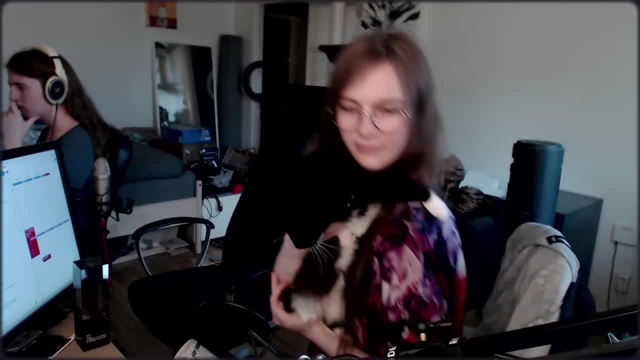 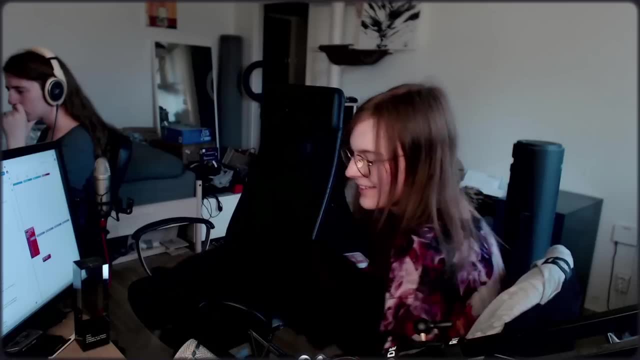 That's true, We did learn that too. This is Thor The void. Ow Ow, Thor, Buddy, You don't have to use your claws. Oh, I missed a question. Will we go deeper into quaternions later on in this course? 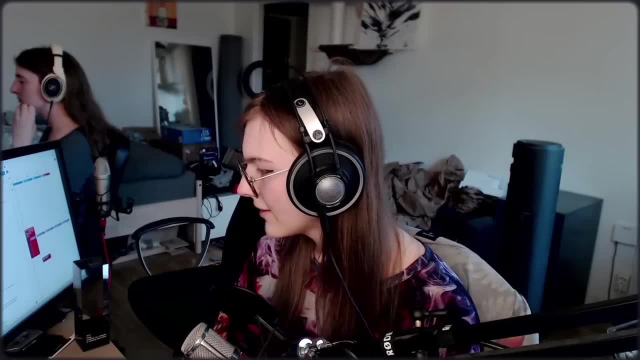 No, We're. I'm going to talk about how to use rotations, But I'm not going to talk about how quaternions work internally, Because that's not relevant. You don't need to know that In order to make that clear. 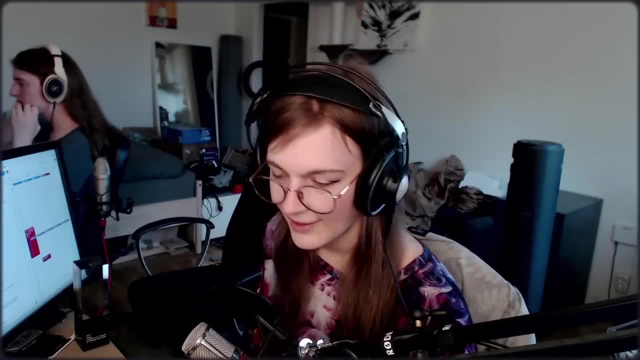 So we're going to talk about how to use rotations, But I'm not going to talk about how quaternions work internally, Because that's not relevant. You don't need to know that in order to make that clear. You don't need to know that in order to make that clear. 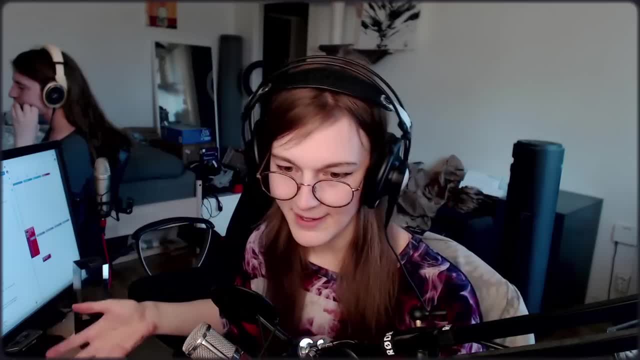 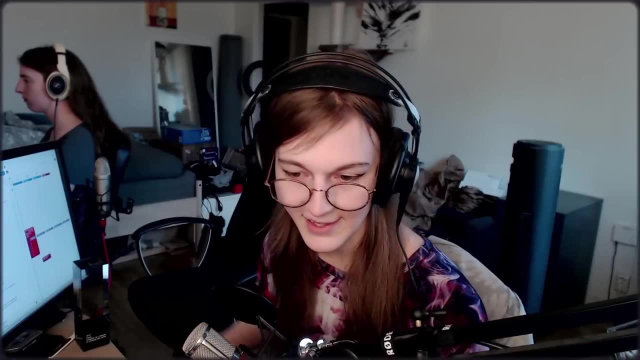 We're going to talk about how to make games, Because we're not going to be engine coders, We're going to make games, Right. So I'm not going to go into, like, how to write a quaternion class, But I'm going to talk about how to use Unity's quaternion class. 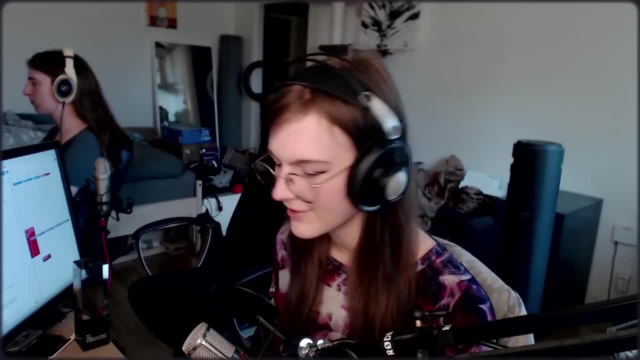 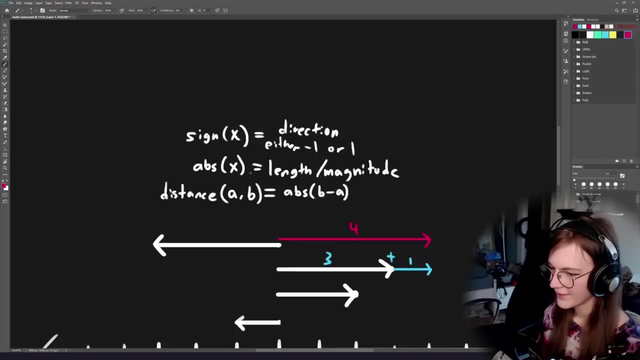 How to apply rotation, How to think about rotations, What they are, And so forth. What's the difference between quaternions and rotors? Mostly an interpretation difference, as far as I know. So let's see, There are a few things we haven't talked about yet. 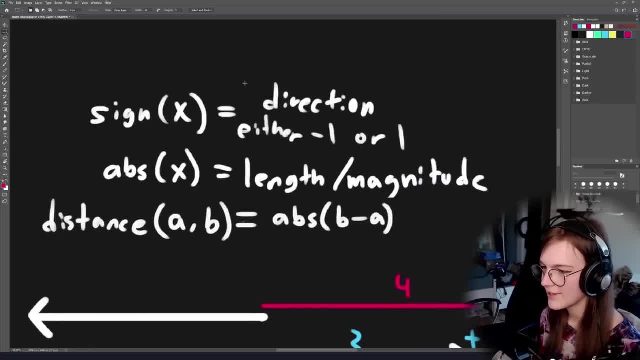 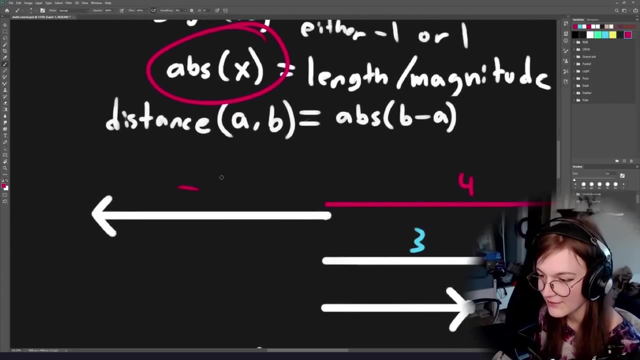 So we've talked about some of the operators you can do. You can do the sign will get you the quote, unquote direction of a one dimensional vector or a value which is either just negative one or one Abs. will get you the magnitude of a vector, which means that if you have a vector or a value of negative four abs of negative four is four, right. 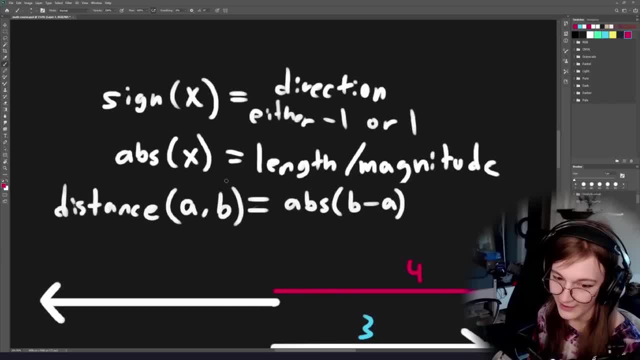 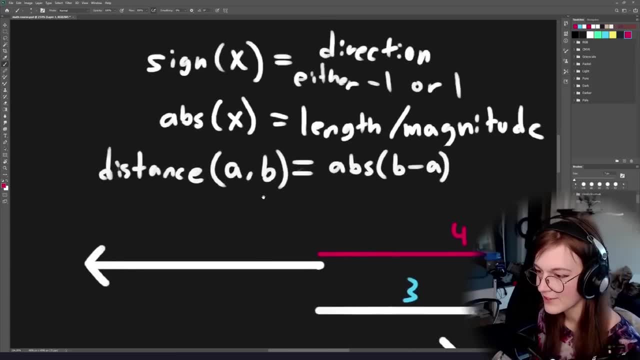 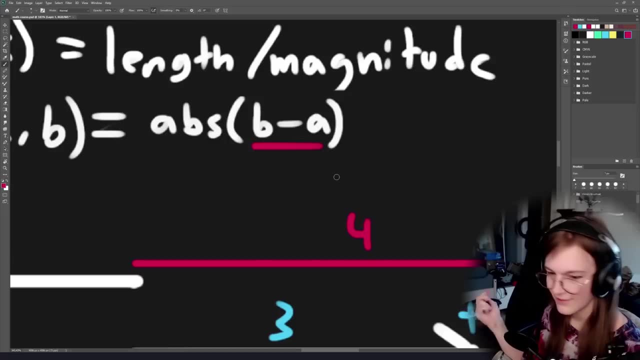 It just makes negative values positive In terms of one dimensional vectors or floating point values or scalars. right, It's a little different for two dimensional vectors And we're going to get to that. And then we have the distance. If you get the difference between two values, it could be like we had before three minus one, or, yeah, three minus one. 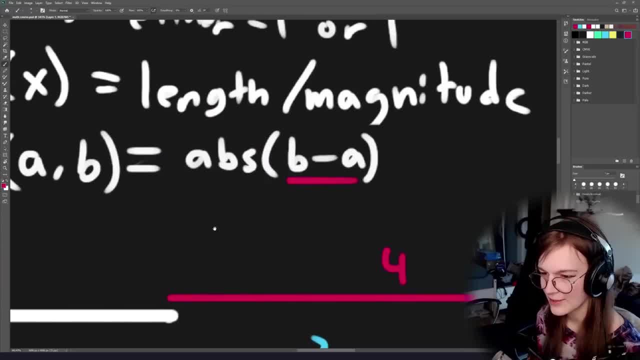 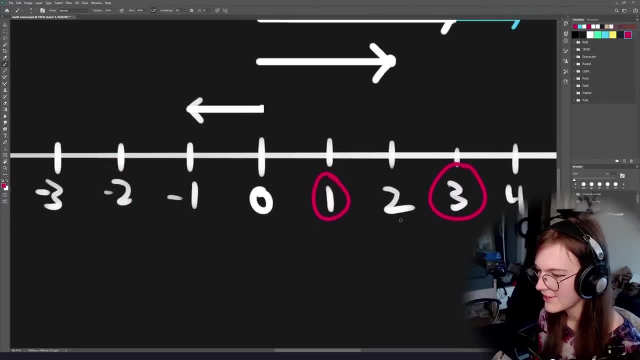 So that would be two. If it's negative two or whatever, then abs will make sure that it's positive And that's the way to get the distance between two values. So if we want to get the distance between negative two and two, like we want to get this distance, then we can just do that formula up there, right? 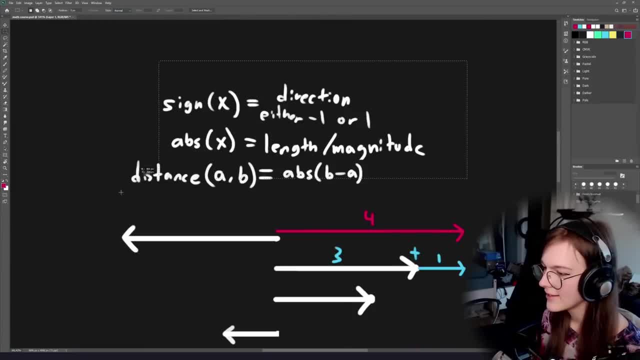 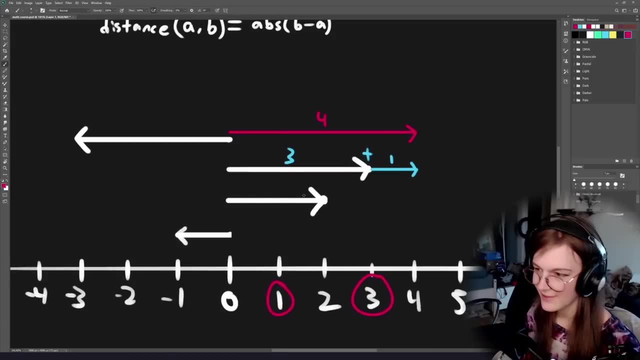 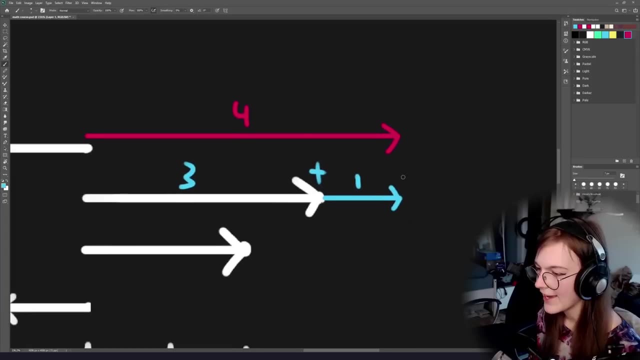 And then it will work out. We talked a little bit about adding And subtracting as well, But the next thing that we should talk about is: like: what does it mean to multiply a value, right? So usually the way that I like to think about it is that when you're adding something, addition is an offset. 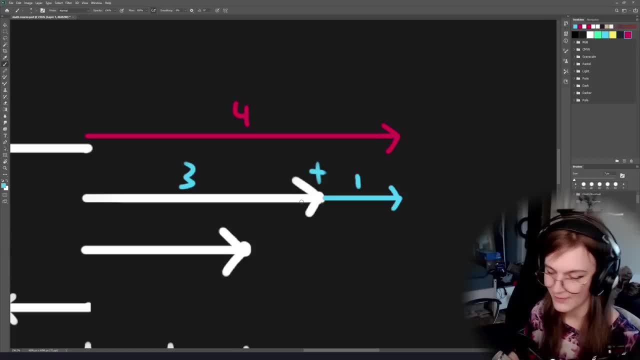 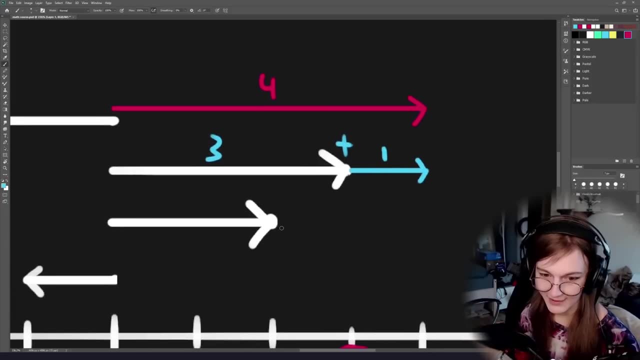 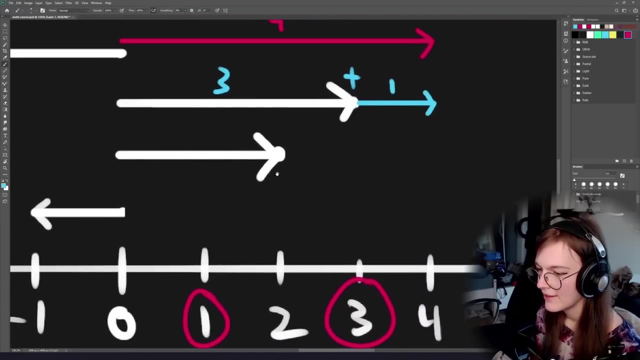 Addition is to move something or increase something by some amount, right? So I usually think of addition as an offset and multiplying as a scale. So we can scale something, We can multiply something by some other value, right? So let's say we have the number two, right? 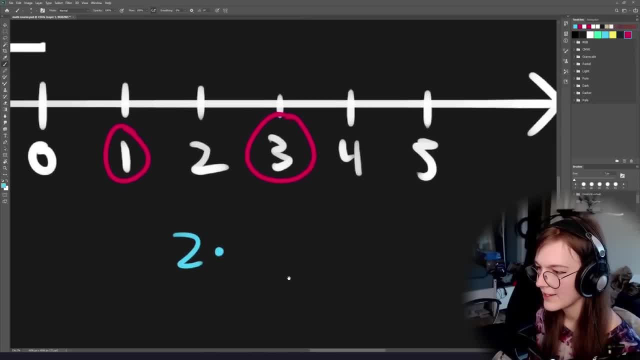 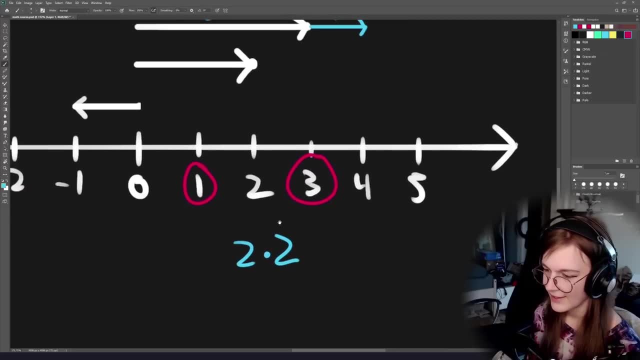 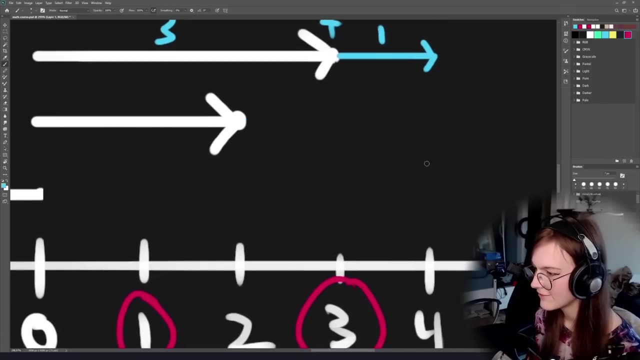 We have the number two And then we want to multiply it by some other value. Let's say we multiply it by two. So if we multiply that by two, what this means is that it's going to be twice as long. So that's going to go from being on two to being on four. 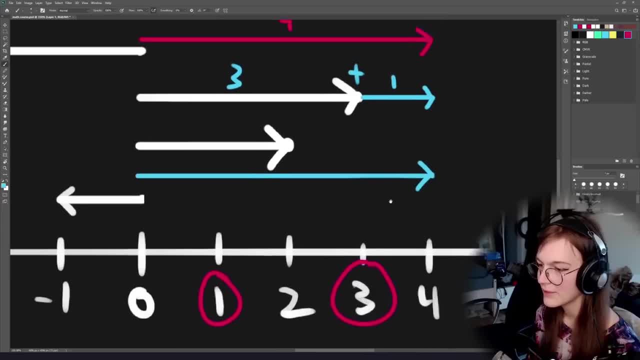 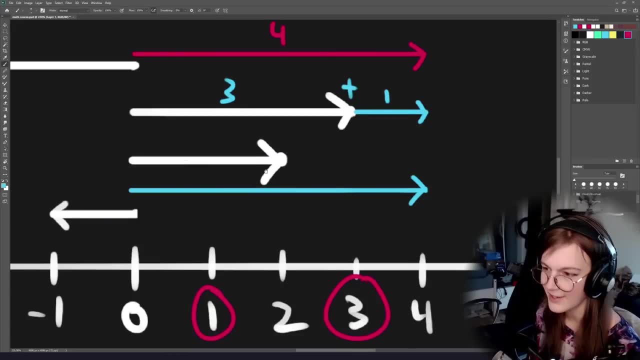 So the result of that is four, right? So what that means is that, Because we have multiplied by two, the length of this vector is going to be twice as long, right? Because again, if you do abs of this one and like check the length or the magnitude, 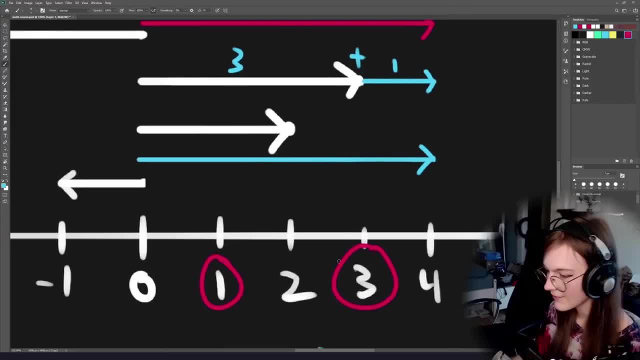 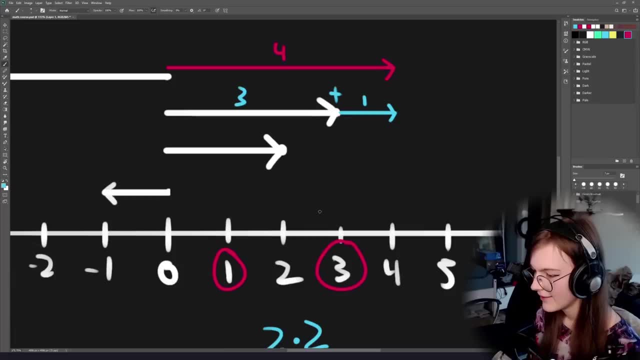 it's now going to be twice as long as it was before, And this relationship holds for any other vectors too. It's not just for scalar values or one-dimensional values. Okay, So, and then we can do other examples. So we can do two multiplied by. 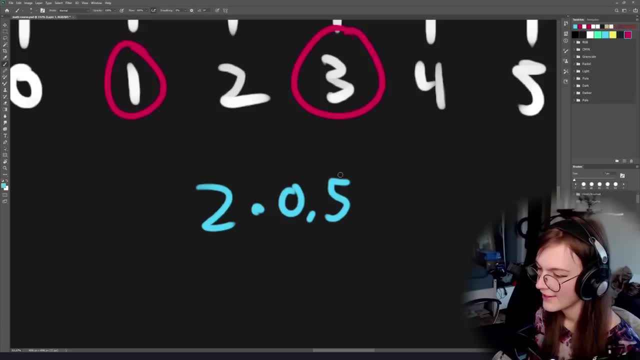 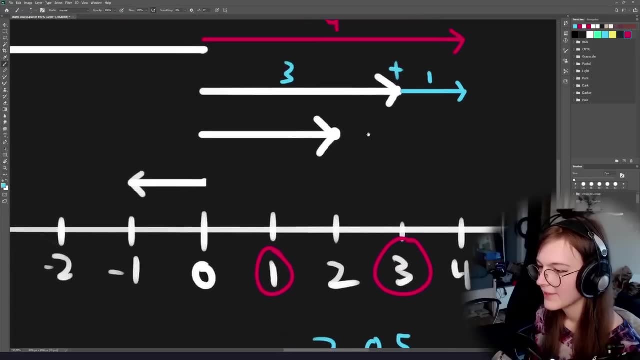 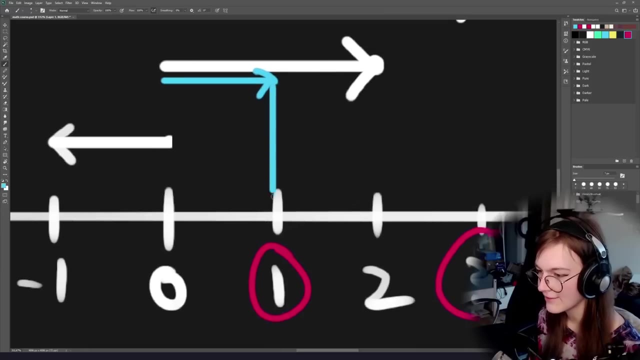 So this is basically half a length, right? So 0.5 is 50%. So what we're going to do if we multiply two by 0.5 is that it's going to be half as long, right? So that's going to have a value of one. 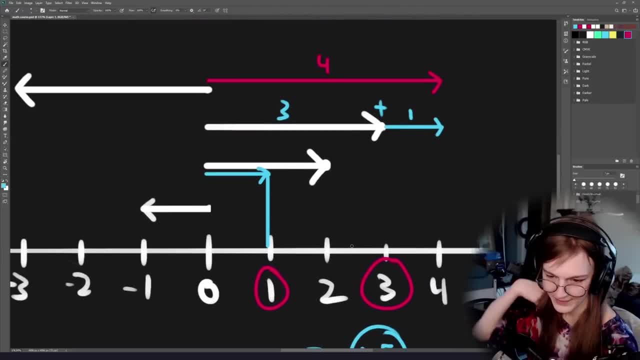 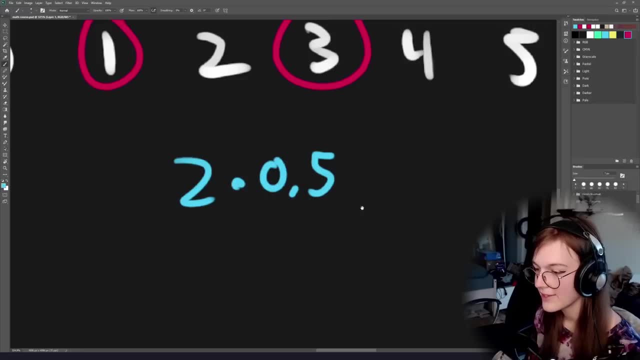 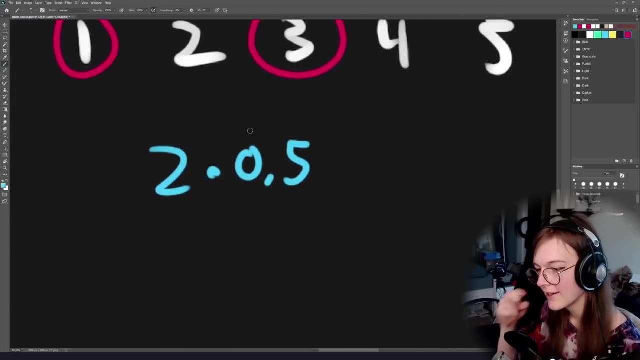 Because two multiplied by 0.5 gives us one And the same thing is. It's the same thing when it comes to dividing right. So this is the same thing. It's the same thing as doing two divided by two. So multiply and divide are kind of the two sides of the same coin. 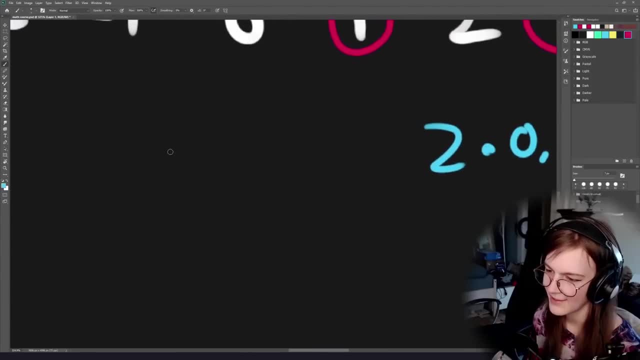 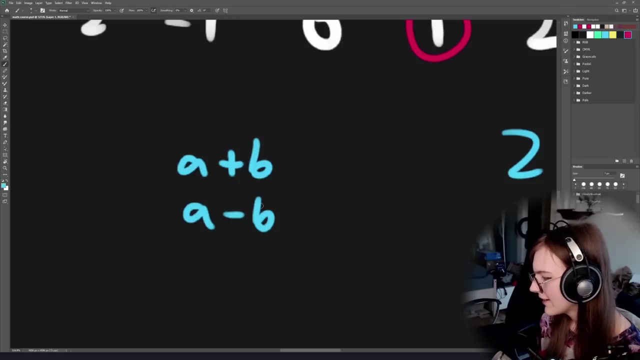 Just like. So, for instance, let's say, we have A plus B And then we have A minus B. Okay, So if If you think about these two situations, like having a, like subtraction, all that is is kind of like you're adding a negative number. 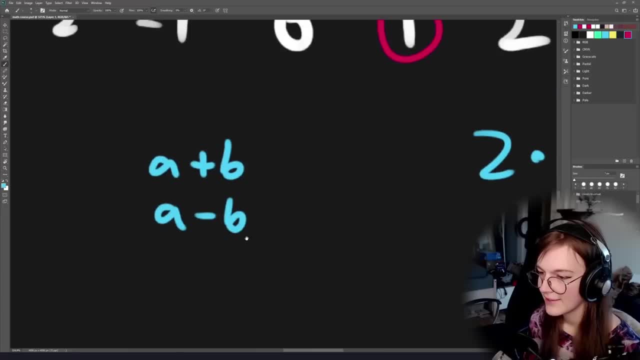 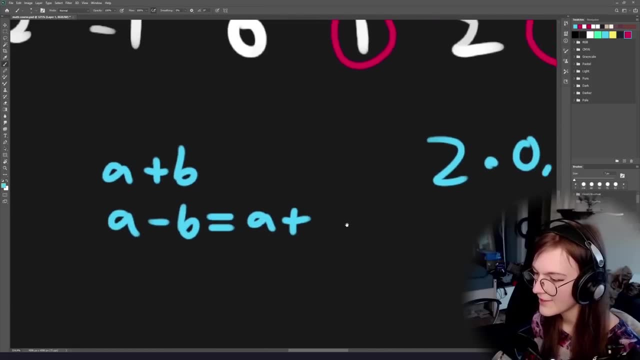 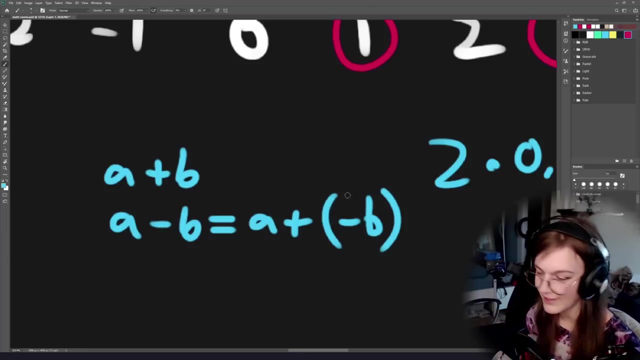 So another way of interpreting this is that, instead of looking at it like this, we could just say that this is the same thing as A plus a negated version of B. right And negation is not the same thing as subtraction Right. 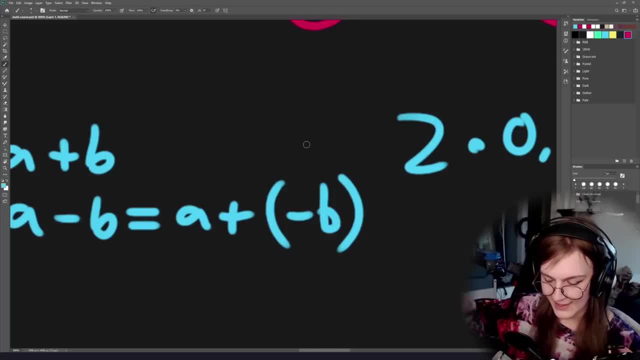 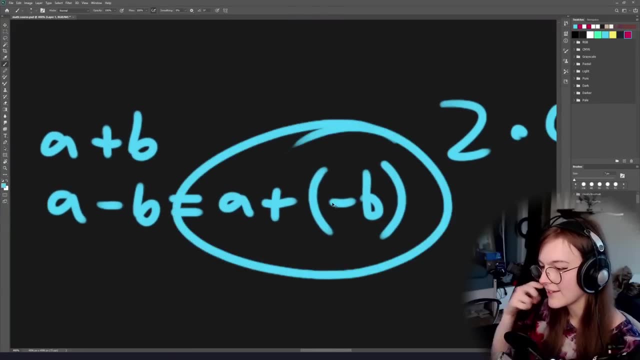 So this flips the sign of it And negation means that if it's positive it's going to be negative, If it's negative it's going to be positive. So, like, addition is generally kind of like, Or subtraction is sort of a special case of addition, right. 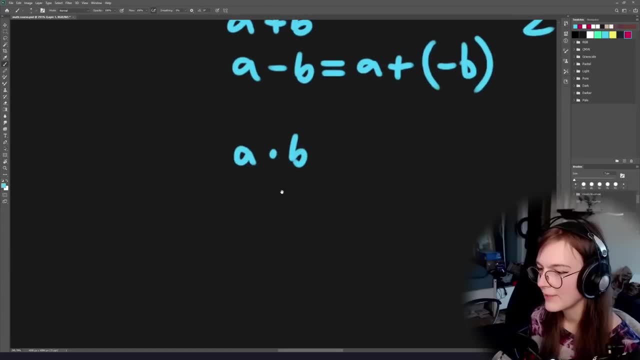 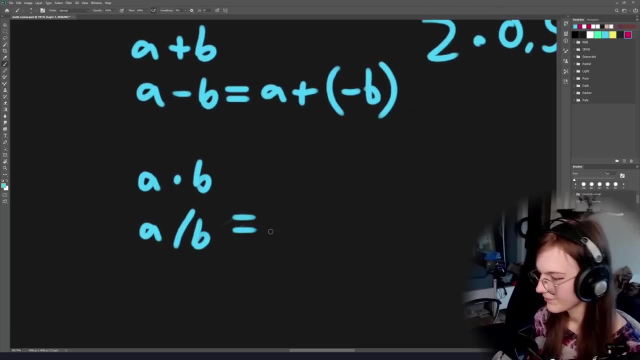 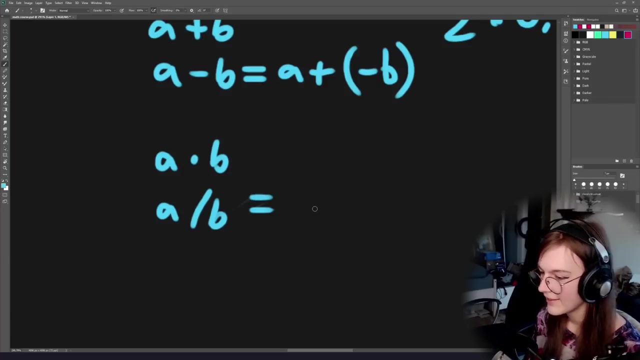 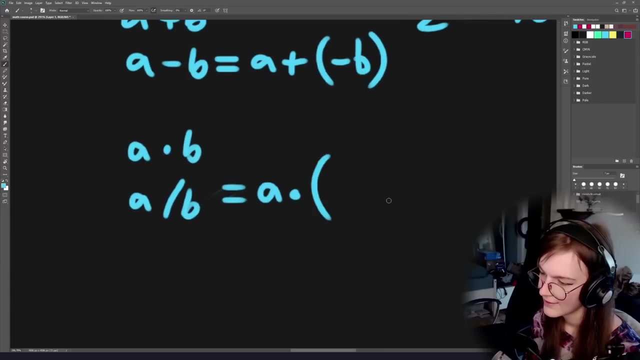 Actually, let's do No, let's do multiply. So A multiplied by B, And then we have A divided by B, right? So? So in this case, This is sort of also a special case of multiply, right? So in this case it's actually A multiplied by the reciprocal of B. 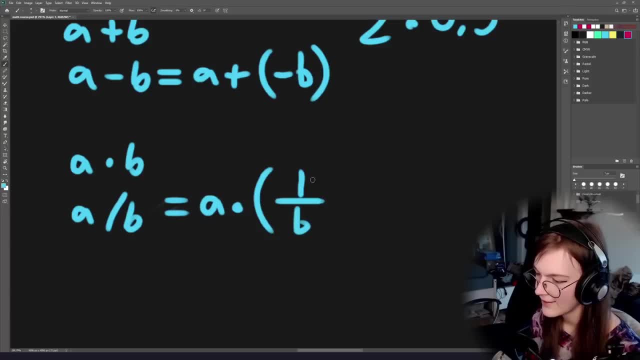 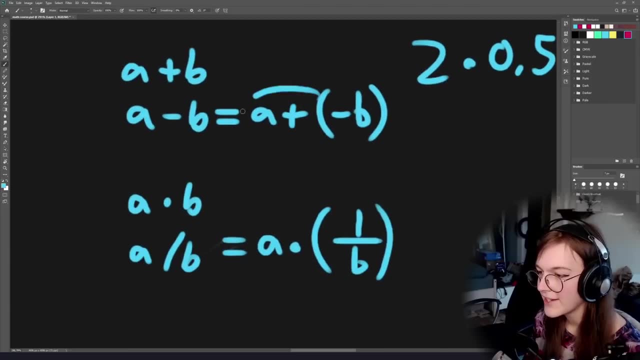 So reciprocal is basically 1 divided by the value. So these two are the same thing, right? So you can sort of think of addition and multiplication as the core Right Or things that you do where when you're doing subtraction or division. 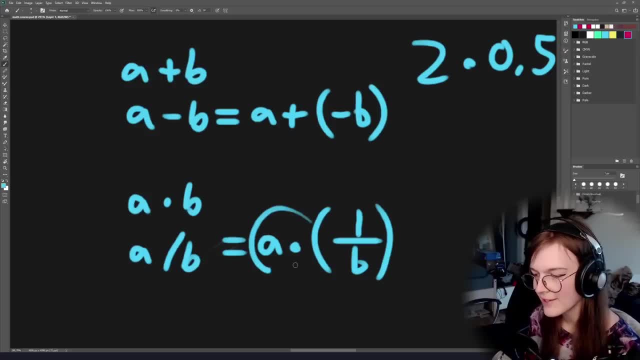 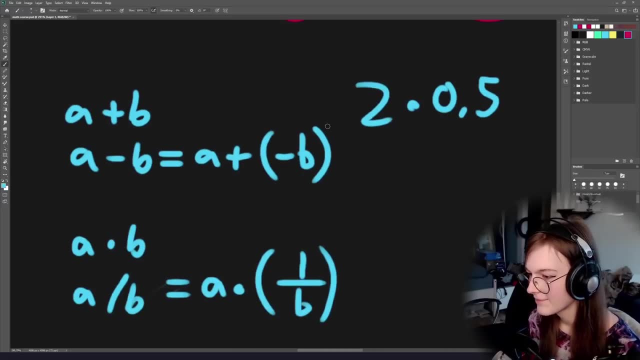 it's kind of like a special case where you're kind of multiplying by the reciprocal of something, Or in this case, you are adding the inverse of something, Right, Anyway, sorry, That was a bit of a tangent, Anyway, I just think that's kind of cool. 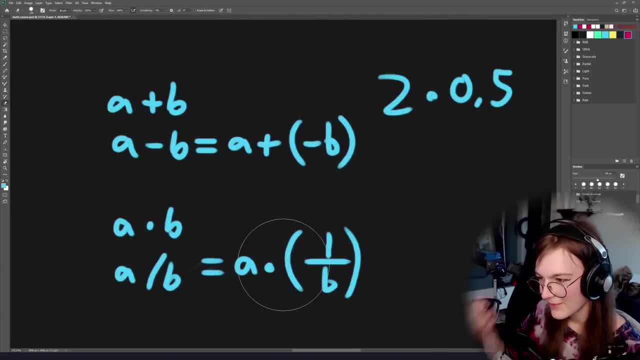 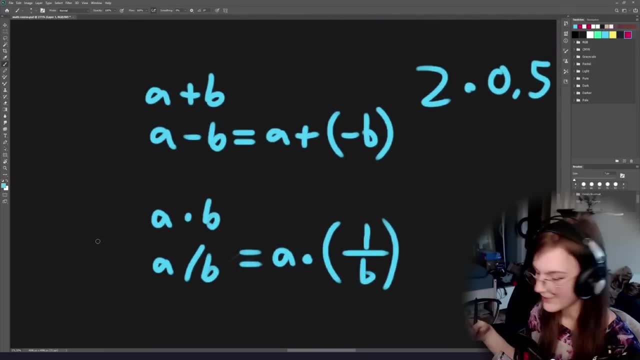 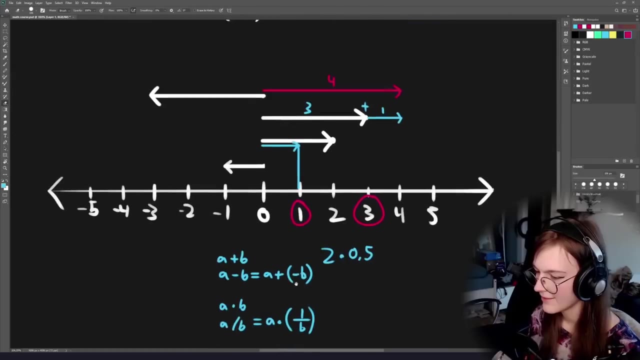 Probably not super relevant to know, But usually the point is you can kind of convert between these two. You can translate: You can multiply to a divide, if you want to, Or a divide into a multiply. Yeah, Okay, That's a big word. 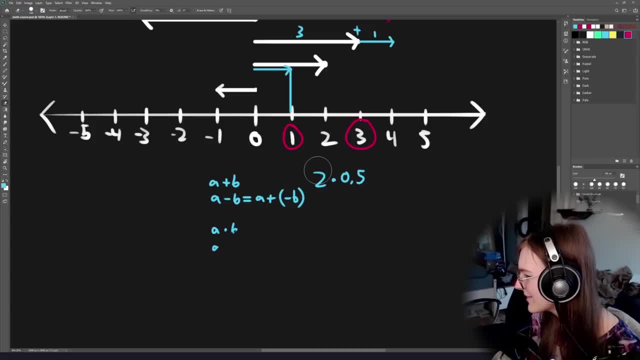 What's a big word. I love this meowing in the background. I had to bless our chat with our Thor emote. That's a great emote. Thank you so much, Marcus. Oh, reciprocal- Yeah, Oh, sometimes it's called one over as well. 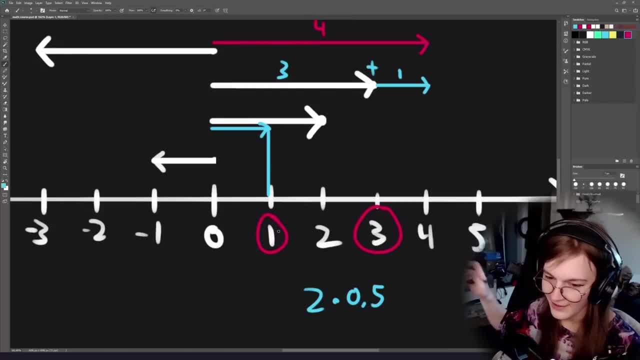 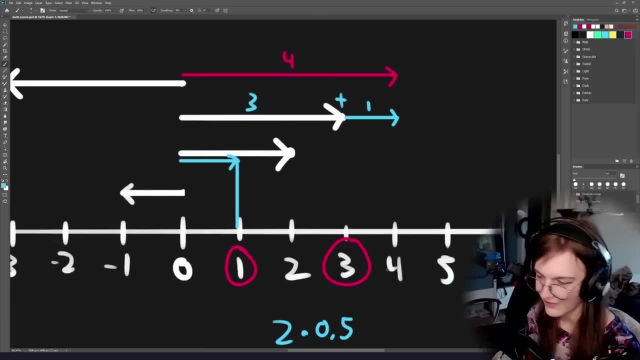 But yeah, It's like Sometimes there are actually cases where, instead of dividing, multiplying can be like slightly faster in terms of like computationally, But usually that goes into the category of like unnecessary micro-optimization. I guess it depends on what you're doing. 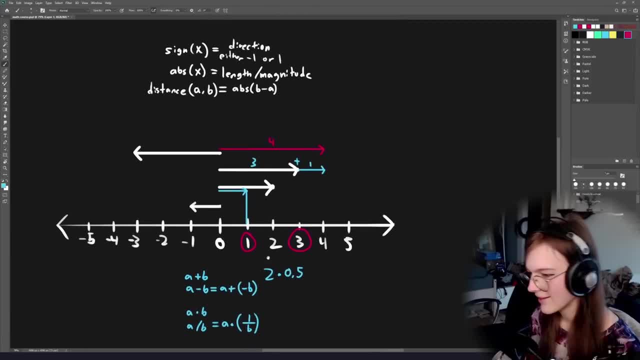 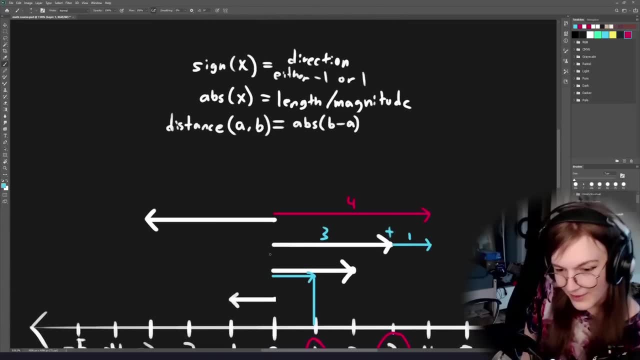 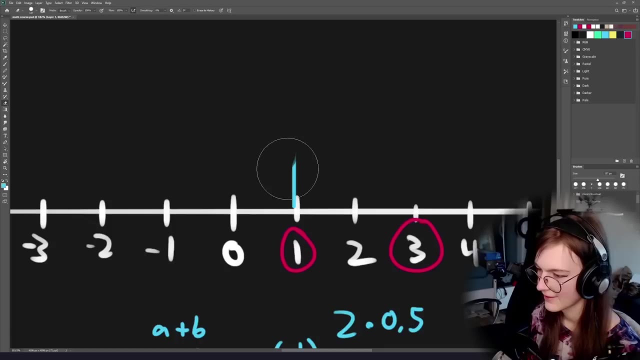 But yeah, Okay, Cool, Let's see, Are we? I think we might be ready to move into two dimensions. So let's erase a bunch of things. Don't need that. These are kind of weird. Why are these numbers marks? 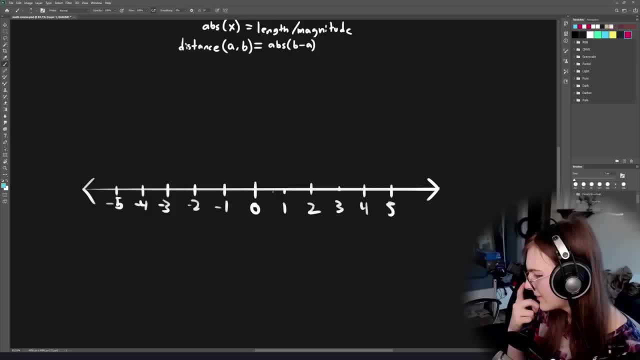 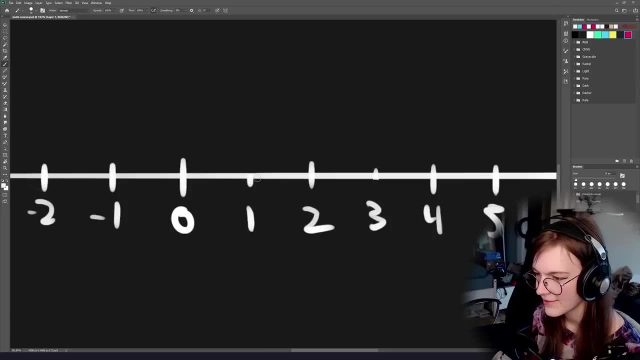 Why do those numbers matter? It's a little unfair actually. Can you explain Quake Engine's inverse square at some point? What part of it? I'm not super familiar with the actual maths of it, But as far as I know it was like: 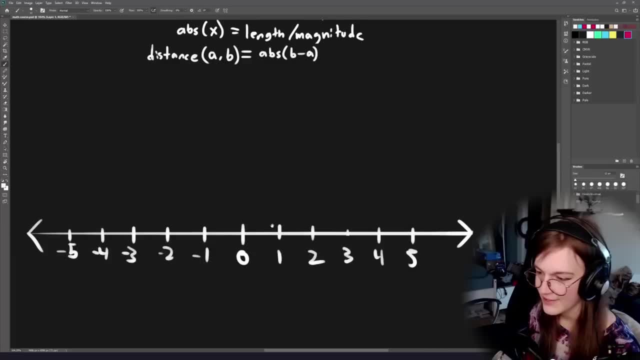 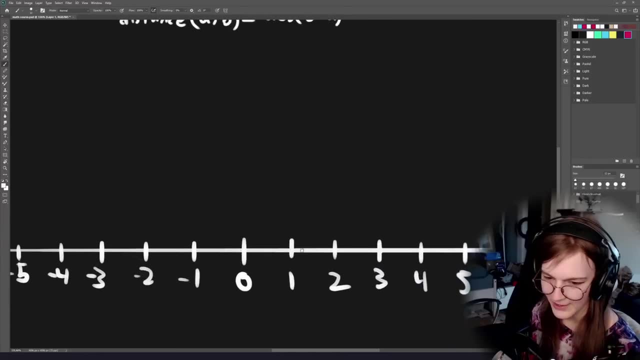 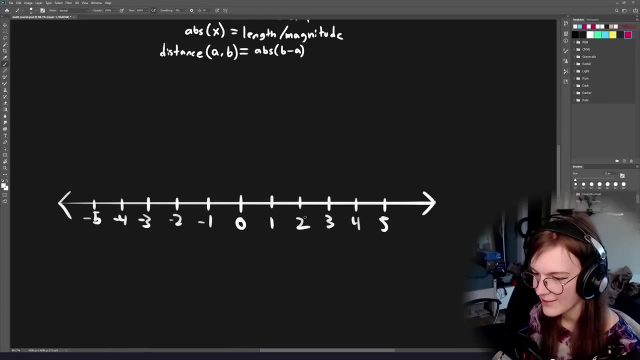 It was an approximation of doing the inverse square root of something And we used like kind of weird bits, bit shenanigans. that sort of only works with certain representations of numbers in binary. But yeah, I don't know too much of the history behind it except what I just said basically. 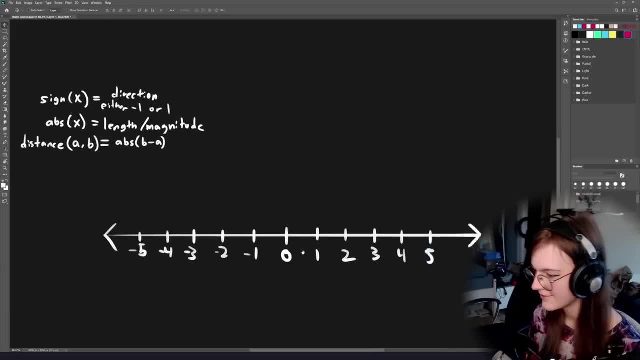 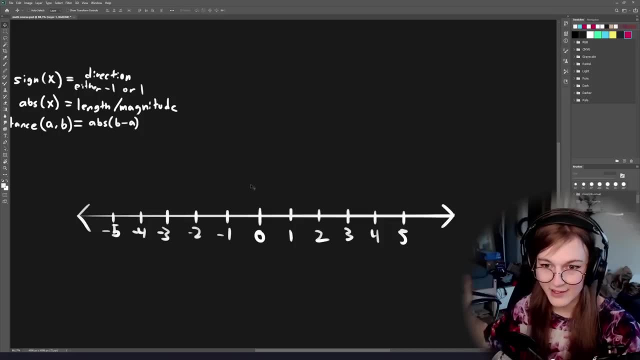 But I'm sure there's a Wikipedia article or something you can go to. Okay, We've talked about one-dimensional numbers. One-dimensional vectors are usually not called one-dimensional vectors. Usually people just call them scalars. People call them floating-point values in programming or decimal values. 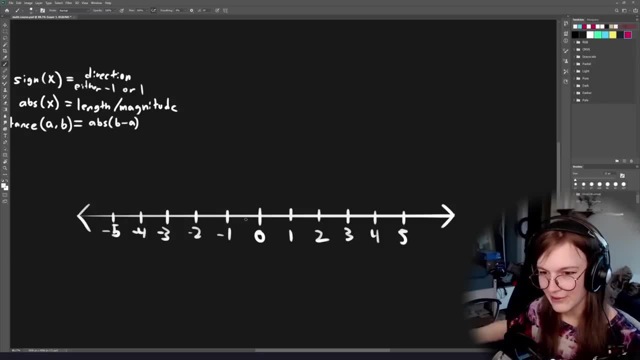 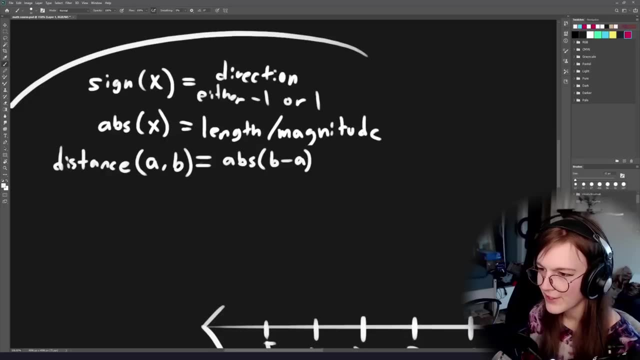 So I've sort of approached this in a non-conventional way. So don't call things one-dimensional vectors, because you're going to confuse people. But the only reason I approached it this way is because all of these functions have direct analogies to the higher dimension vectors. 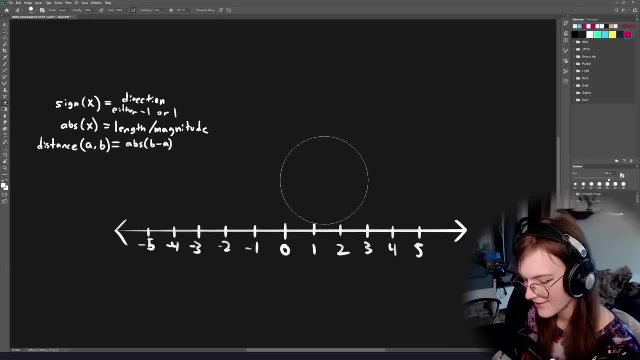 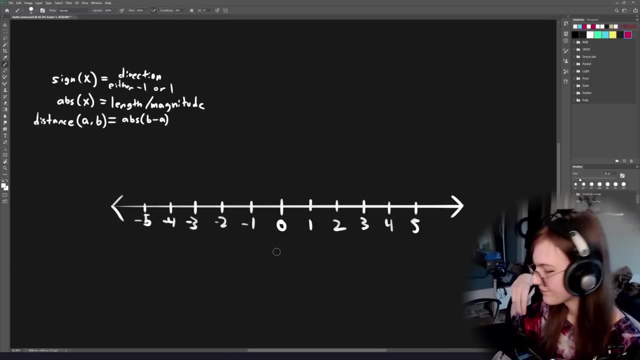 So let's go to two dimensions, Let's just enter another world or something like that. Okay, So usually when we talk about dimensions, usually we have axes right. Currently we've only had one axis, Like it's the x-axis usually. 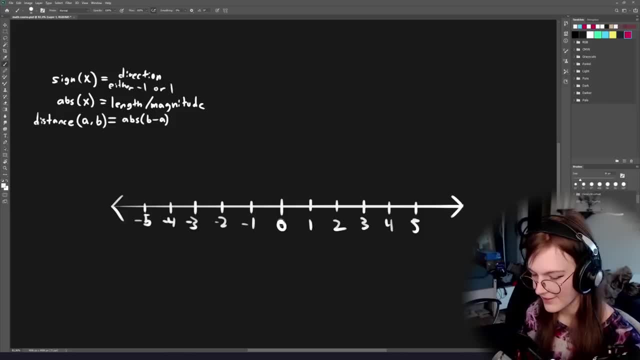 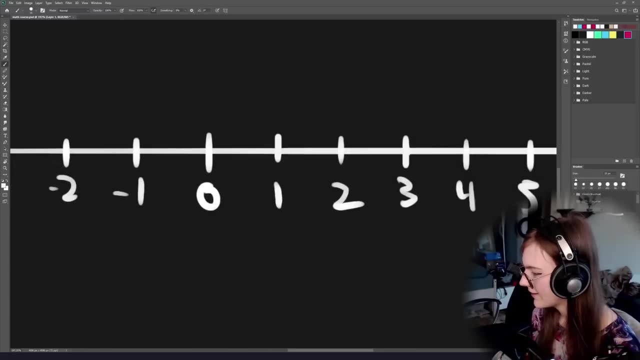 This is the number line. We only have the one axis where we have all the numbers right, And if we want to represent a position here, all we need is one number right And we also need to not lock alpha on the layers. 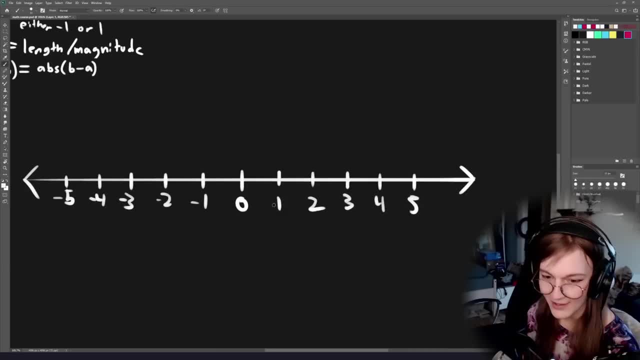 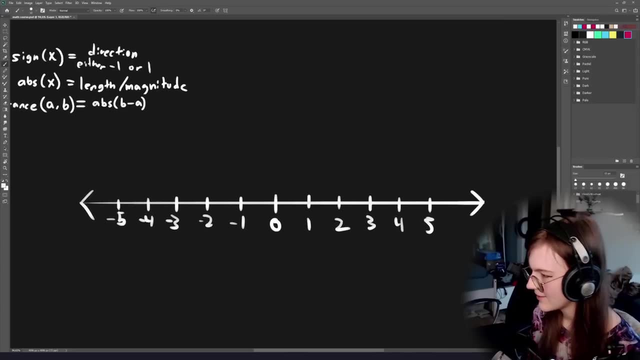 Anyway. So basically, if you want to represent a position on the number line, all you need is one number, because there's only one dimension. So what we're now going to do is that we are going to add a dimension to this. So, first off, when we work in multiple dimensions, it's really useful to use colors. 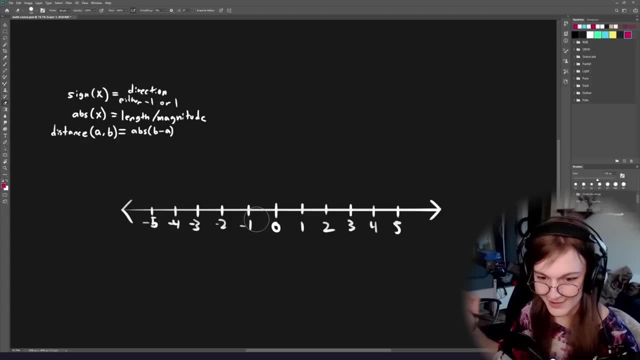 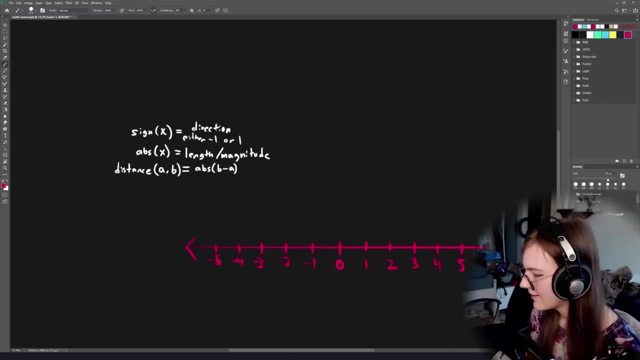 So usually when working in 2D or 3D space, usually we use the colors red, green and blue. So the x-axis is I'm using the eraser. There we go. X-axis is usually red And there's a neat little shorthand if you want to remember which one is which. 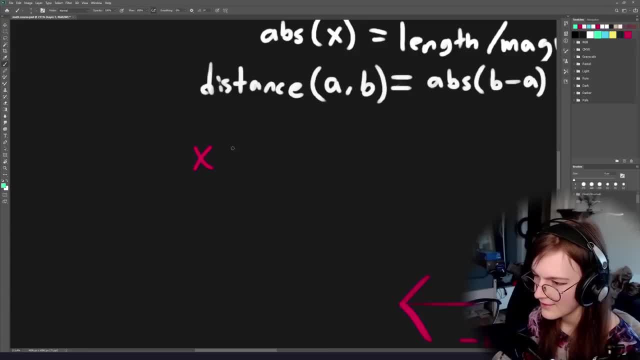 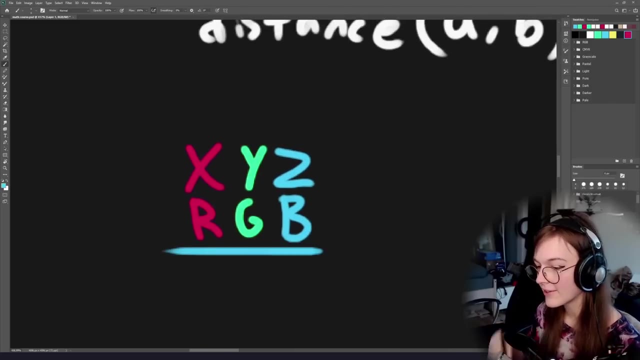 So usually you have x and y and z, So these directly correspond to RGB, right? So if you want to remember What axis is what color, then they follow RGB, Like RGB, is usually the color space we use and they directly correspond to the colors. 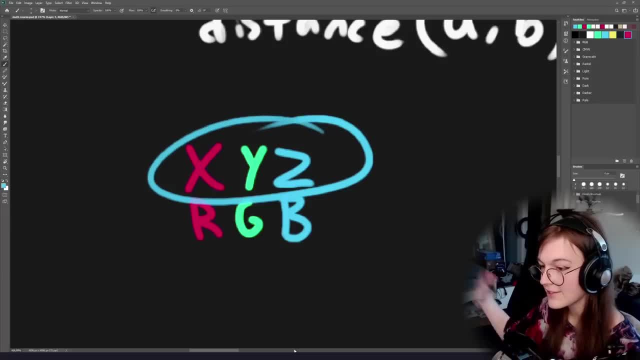 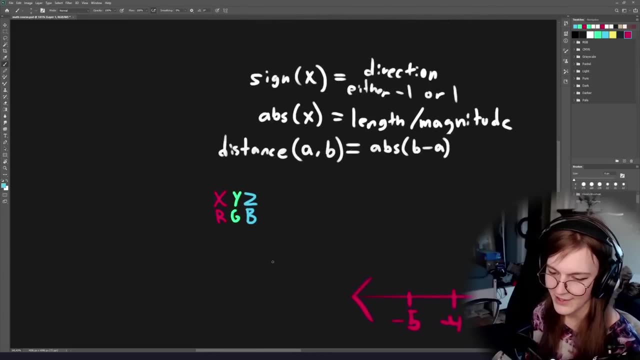 of the axes that we have in our- Or each dimension axes, basis vectors. whatever term you want to use, They correspond to those. So if you open up Unity, the colors of the gizmo is going to match this right. 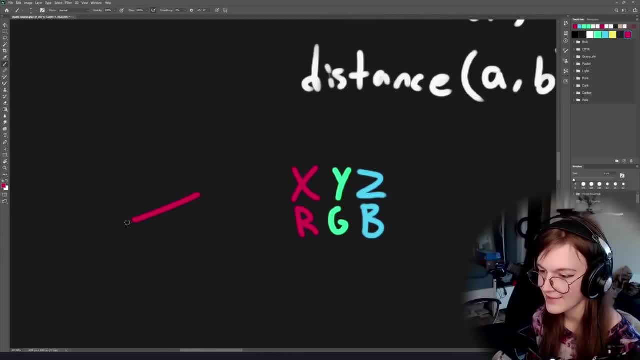 If you see a red axis, you know that that's going to be the x-axis, right? So it'll look something like this: Okay, There we go. It's something that like I don't know. It's weird. how many people have not realized that? 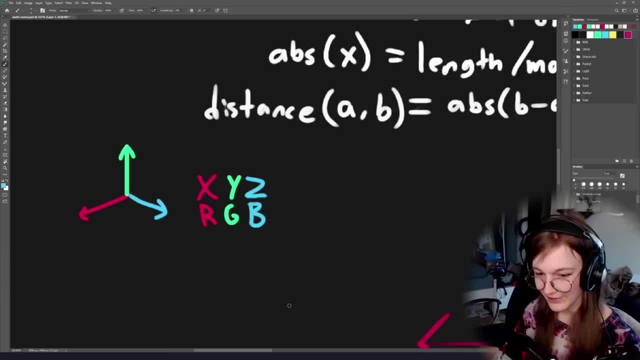 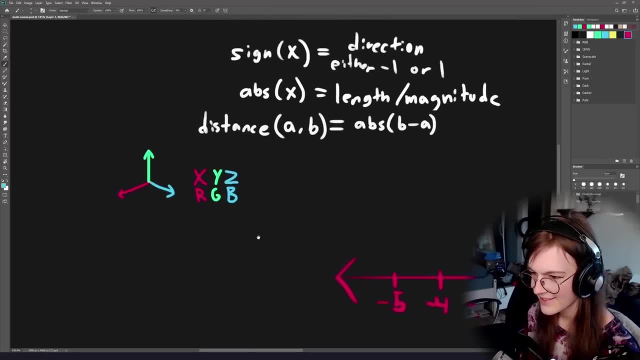 It's like It's one of those things that's obvious once you learn it, But before that it's like really not obvious for some reason. But yeah, Someone in Twitch chat said left-handed. The reason it's left-handed is because we are going to talk about Unity. 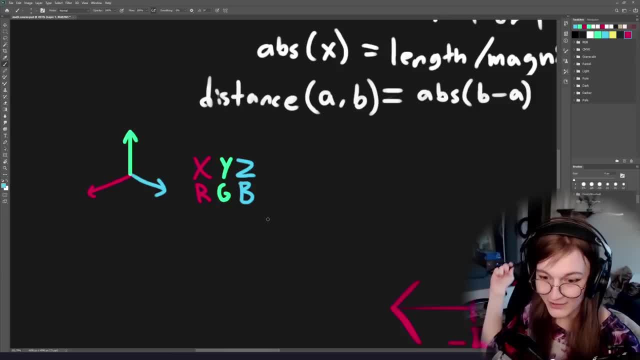 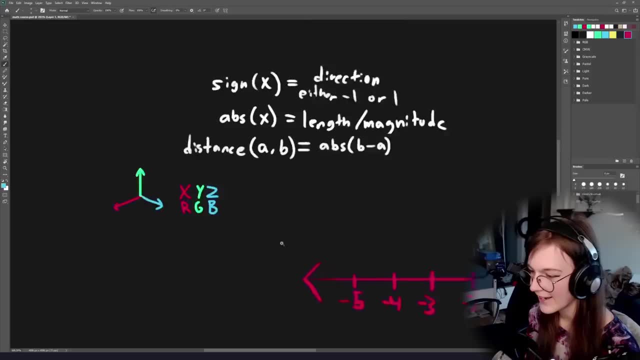 And Unity is left-handed And Unreal is also left-handed, Although Unreal is Z-up, But yeah Anyway, So that's why it's left-handed. So I'm sorry for any like actual professional mathematicians, Because math is usually right-handed. 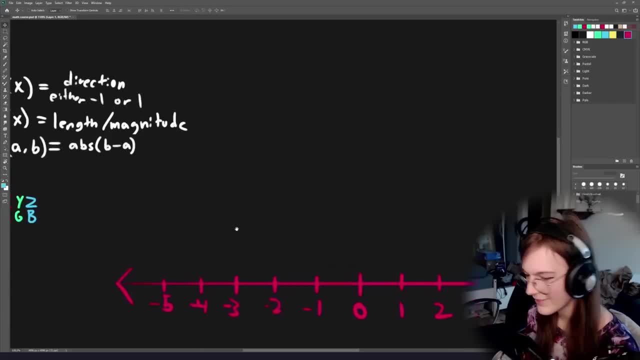 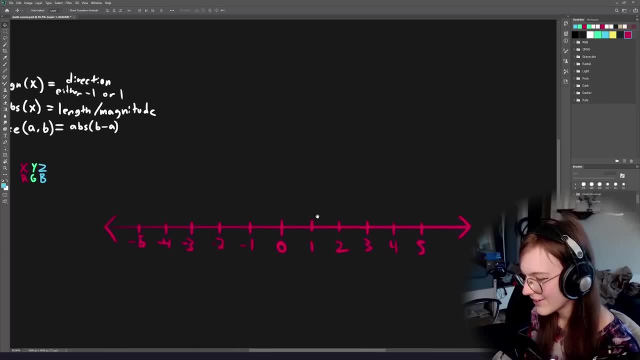 Which is kind of not great, But whatever, It's okay, I'm also left-handed. Neat. I'm glad you figured out your chirality right. All right, So we're going to add another dimension. So so far we've just had one dimension. 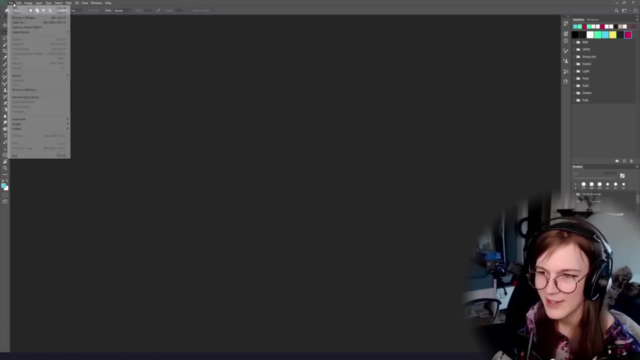 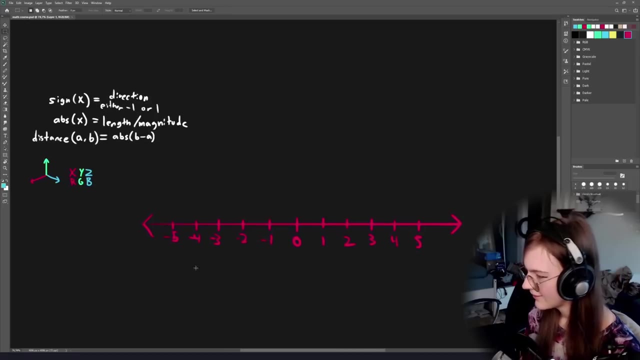 And we also need to close this document, Because Photoshop decided to lock the document, Which it sometimes does when I'm using the tablet. All right, So we're just going to take this axis and copy it and rotate it. There we go. 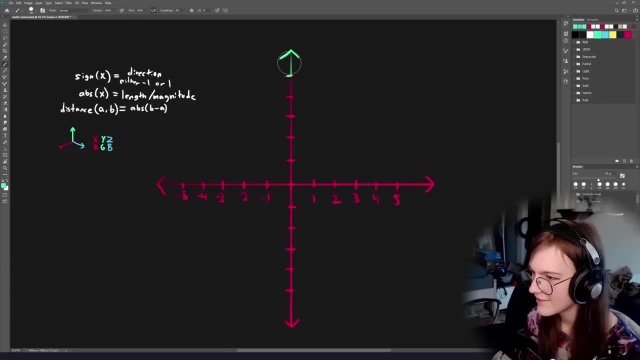 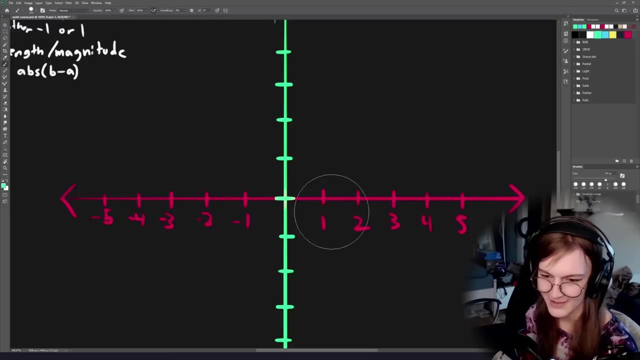 If you're, like, very familiar with math, this is probably painfully slow And I apologize, But I do want to make sure that everybody feels very covered and knows what we're talking about throughout this entire course. So sorry if it's a little, a little too basic. 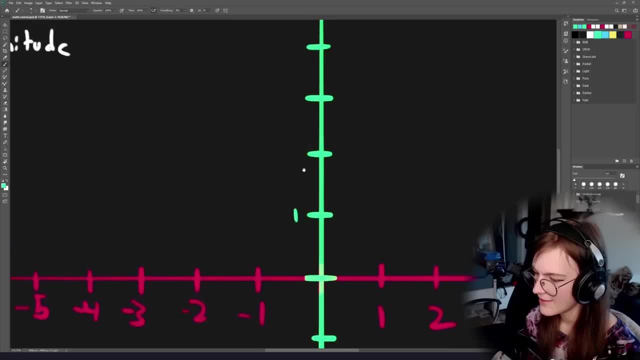 But that's okay. I hope that's okay, All right. So let's see, The number line still works the same way. We still have, like it's still a number line. We just have two of them, Right. 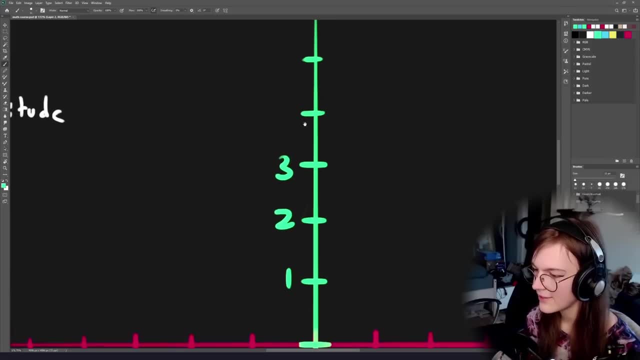 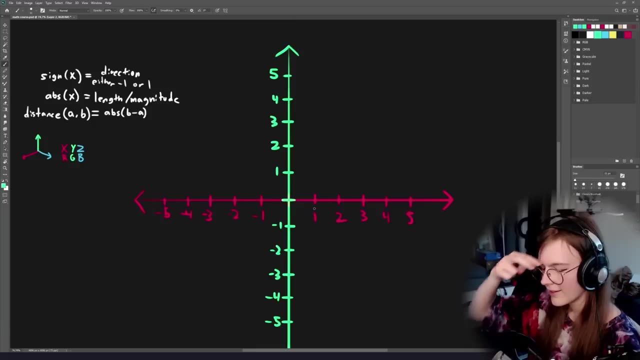 So now we have 1,, 2,, 3,, 4, 5, negative 1, negative 2.. Okay, So now, Instead of a one-dimensional space, which was the number line, we now have a two-dimensional. 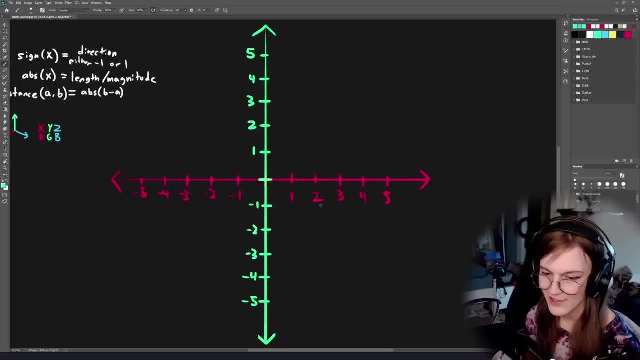 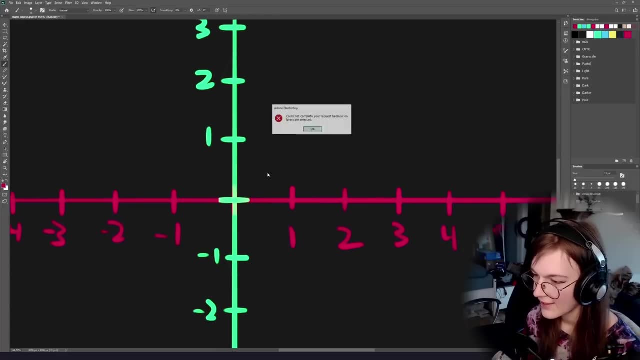 space. So generally when you add a dimension to something, the dimension is always perpendicular to the other dimensions, So, or the other axes. So whenever you're looking at something like this, then actually it's not always perpendicular. But if you want to have like an orthographic space which you usually work in, then all 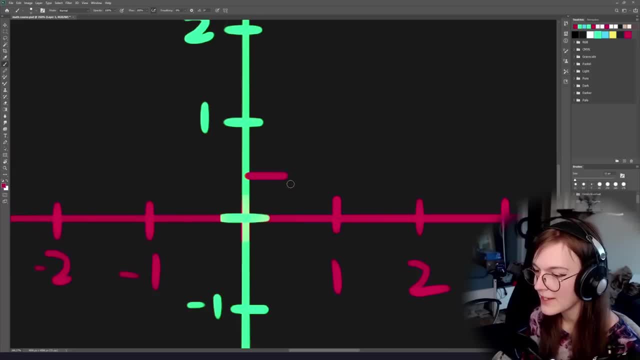 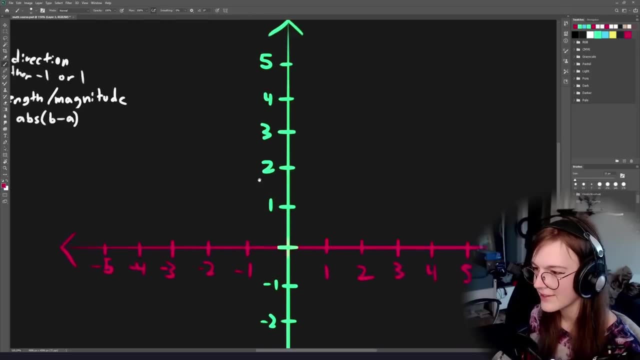 of the axes will be orthographic To each other, So they always meet at a right angle. Again, there are exceptions. If you're working with like projection matrices or whatever, then But whatever, That's irrelevant now, Sorry. 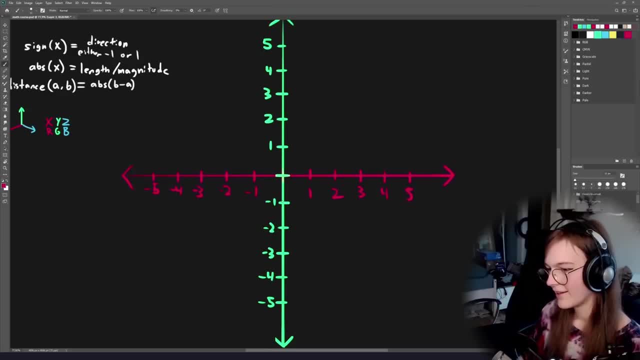 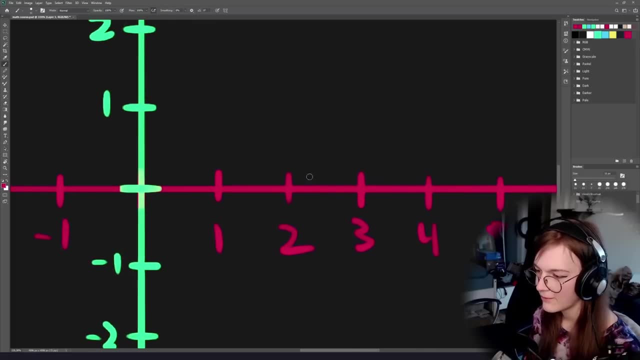 I'm going into unnecessarily weird details. All right, So now we have a two-dimensional space. So you know how we previously marked a point where you know we would say that some place is 3. Right In terms of position. 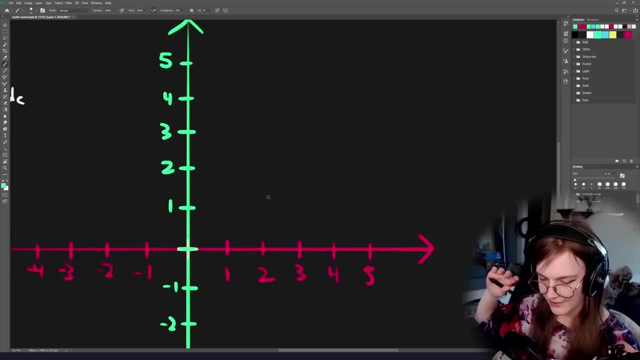 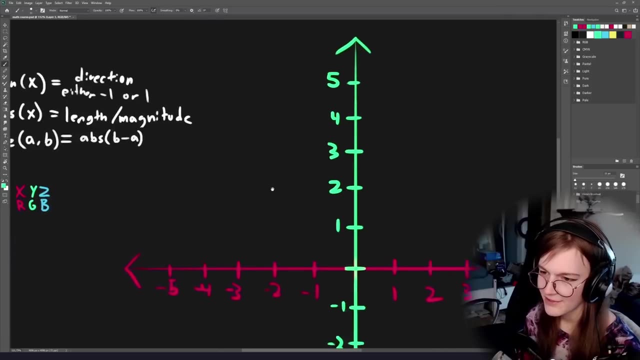 Right. So if you're working in two dimensions, instead of every point on the number line being a single number, a point in two-dimensional space is two numbers. So there are a lot of like different ways you can like write vector notation. 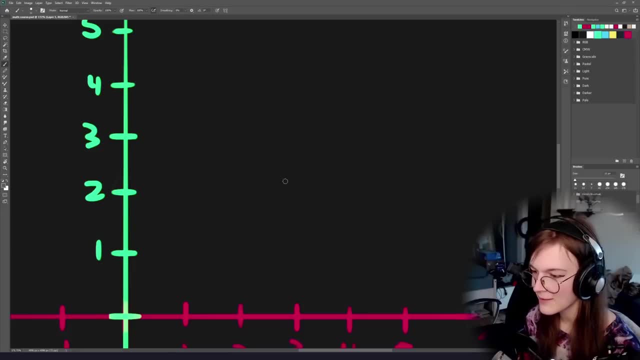 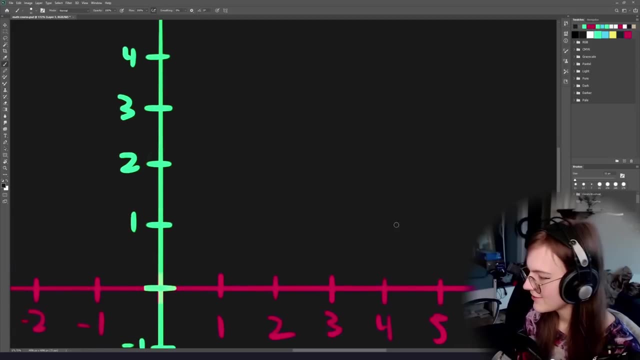 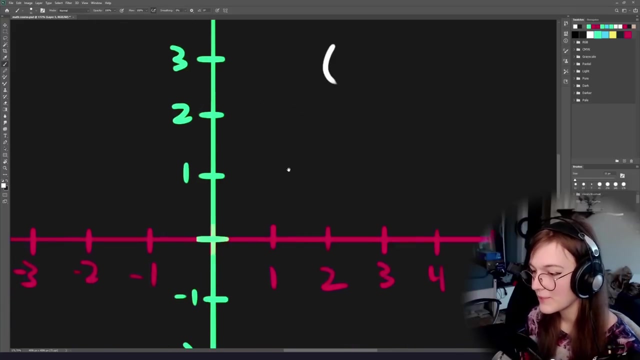 Usually in mathematics the notation is really garbage and terrible. So I'm just going to sort of do whatever because math hasn't worked this out yet. So usually I just do parentheses when I want to like mark a vector. So let's say we have, we want to get a position in this 2D space. let's say we mark this point. 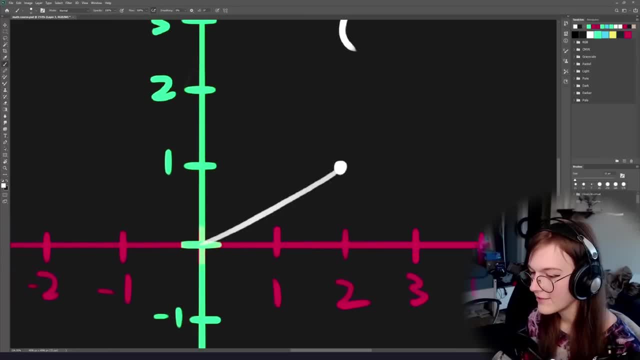 right here, Just like we did before, we could draw an arrow representing the position. And if you want to draw a position or a vector, vectors kind of always originate from zero, Because vectors don't have a root and a tip, They only have a tip. 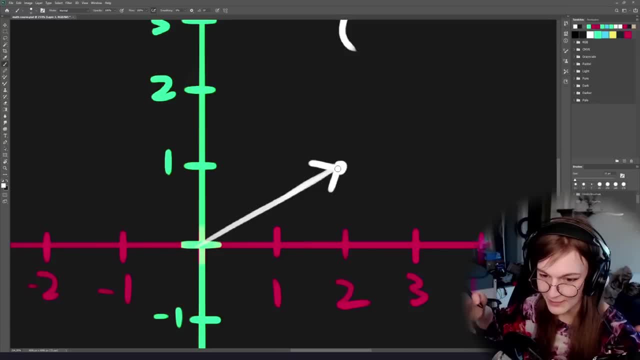 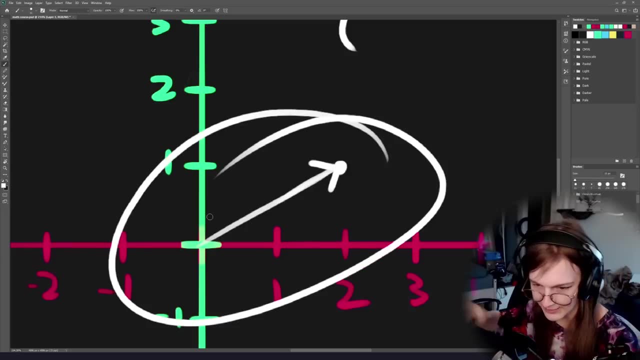 So like where you put the vector is only for like visualization purposes Or interpretation purposes. This is really important if you want to like know the distinction between like a vector and a point and a direction, which we're going to get into. 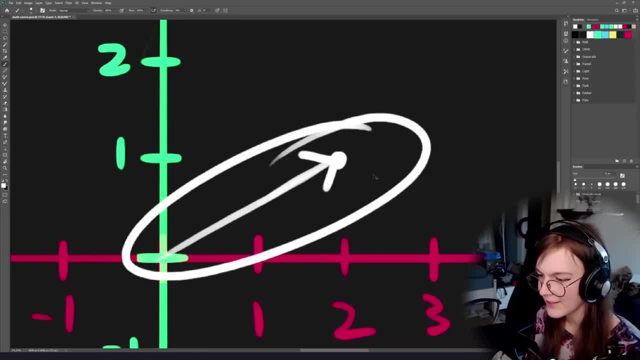 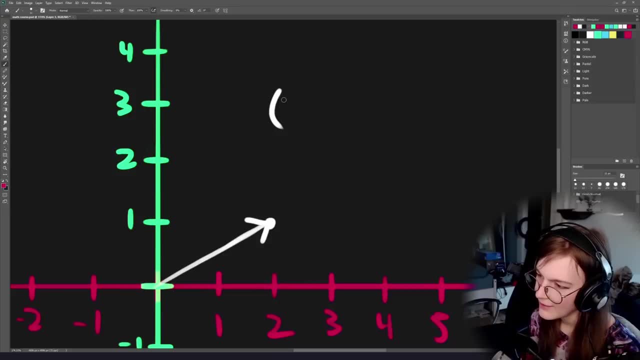 So now we have a point, So this is a point. We can represent it as a vector too. And now, if we want to like, type the coordinates of this one, it would be two on the x-axis And it would be one on the y-axis. 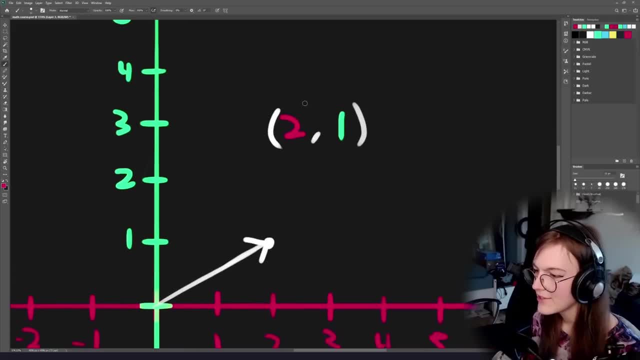 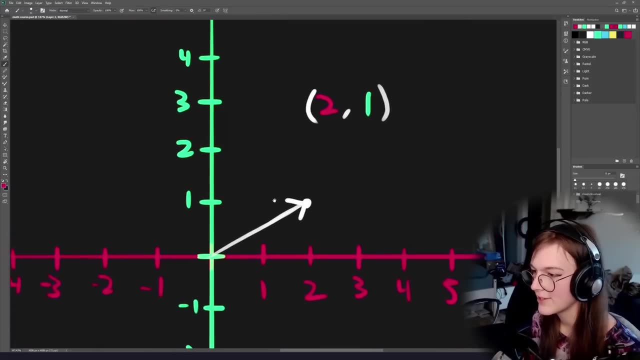 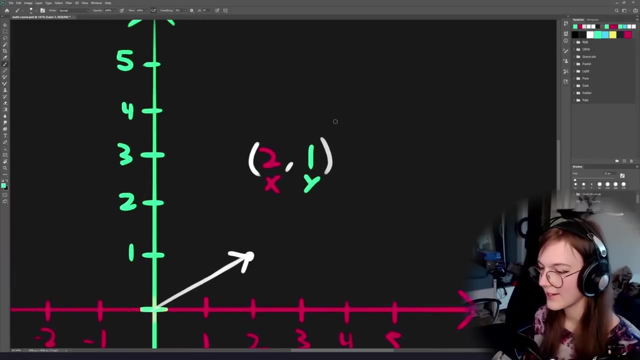 So basically, what this means is that each of these are called components, And these components of this vector correspond to each of these two number lines. So this is the x component And this is the y component of this vector. Right In Unity, this type would be called a vector 2.. 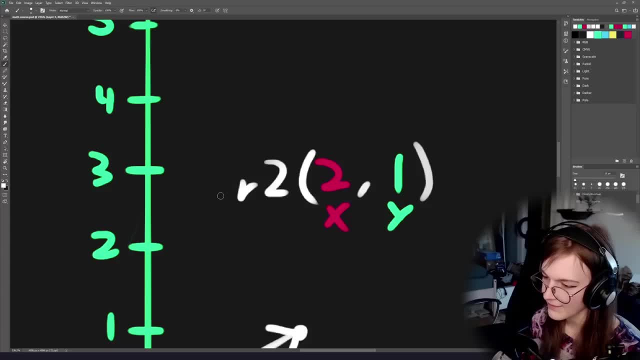 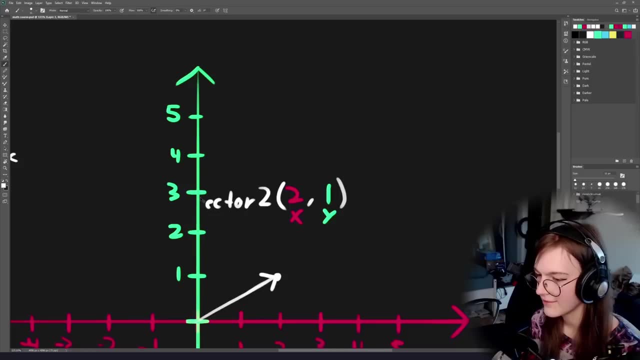 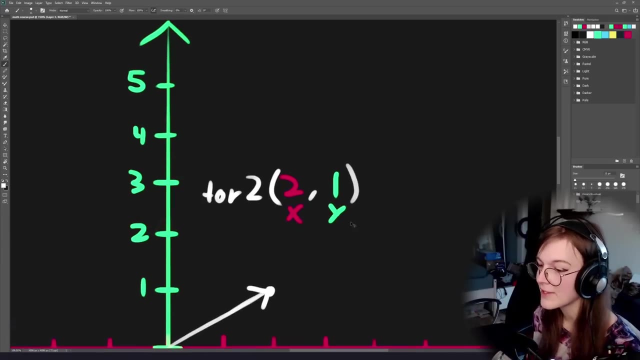 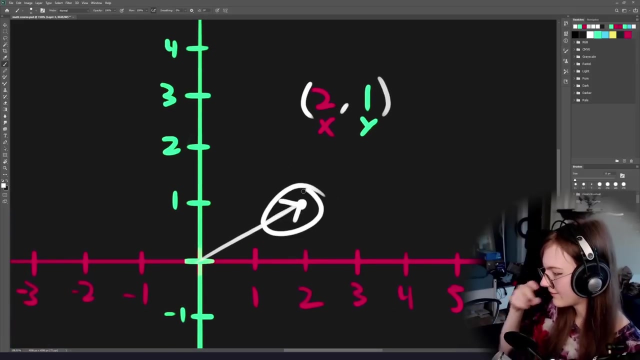 Because it's a two-dimensional vector. There we go, Vector 2.. So this is how you would sort of write it in code: You would do new vector 2, and then you have a two-dimensional vector, Right, Okay? So this, these are the coordinates for this point. 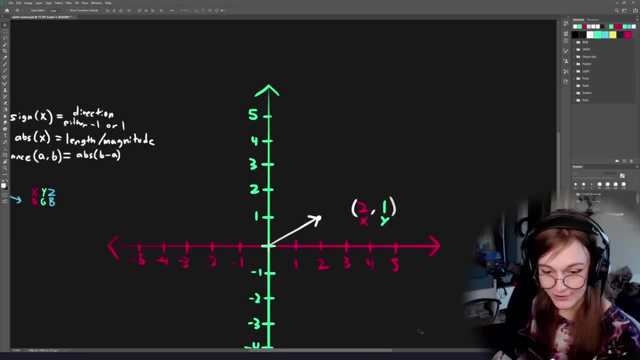 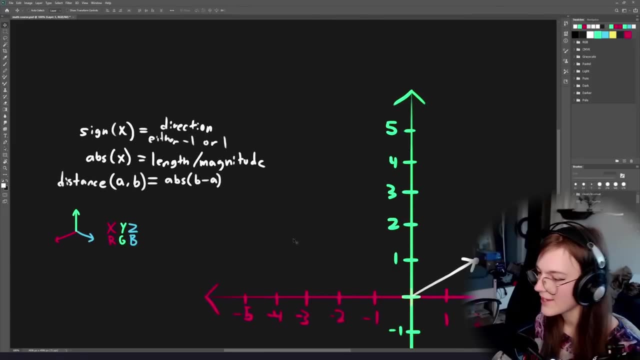 Right, All right. So now, if we look back at everything we talked about before, we can start doing a lot of operations with these. that works exactly the same way in two dimensions. So let's start with addition. Let's say: you want to add something. 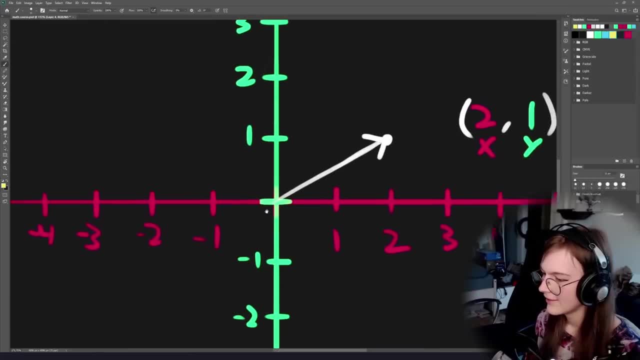 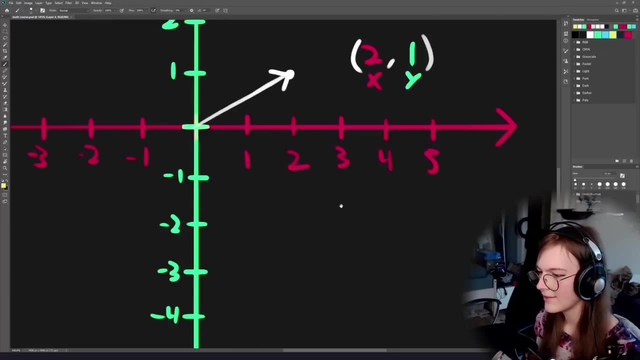 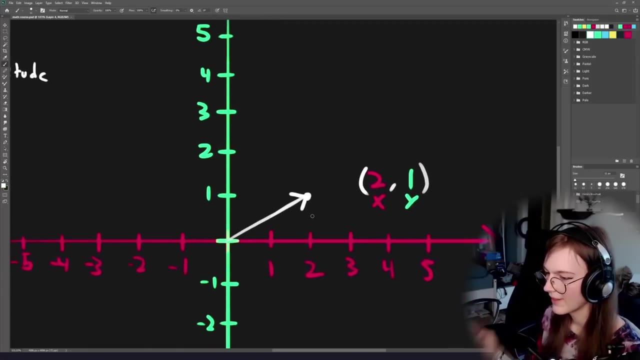 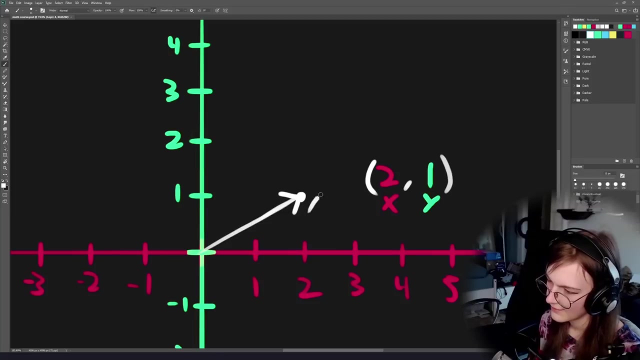 Right. So let's say we want to lock the Photoshop document again And then reopen it. All right. So let's say we want to add something to this. Let's call this something. Let's call it A Or maybe. I don't know if we should do lowercase. 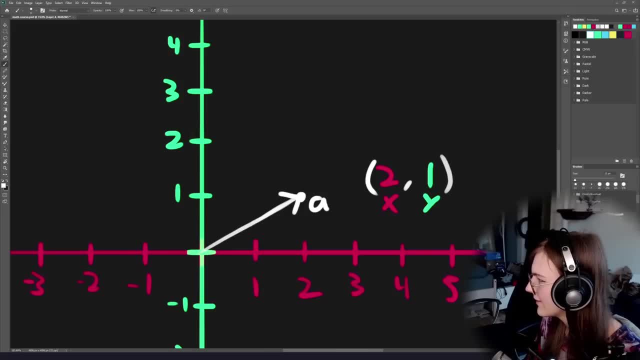 Let's do lowercase, Why not? Oh, I just said 170 new messages in the student chat. Hope not. No, We're fine. Okay, Thanks, Discord. All right, So we have the vector A. The vector A has these values. 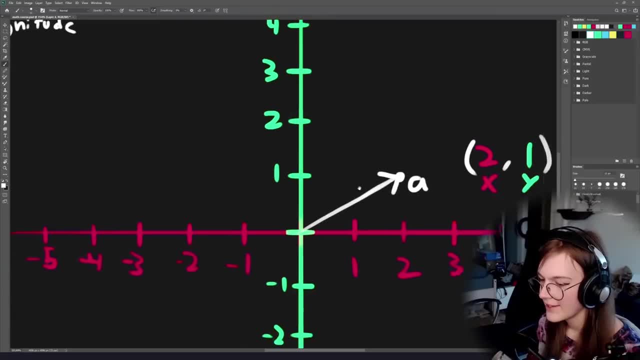 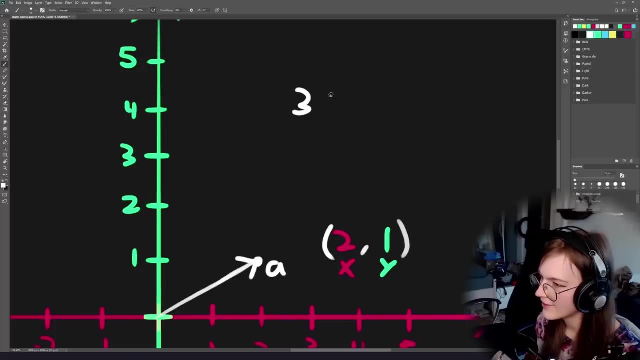 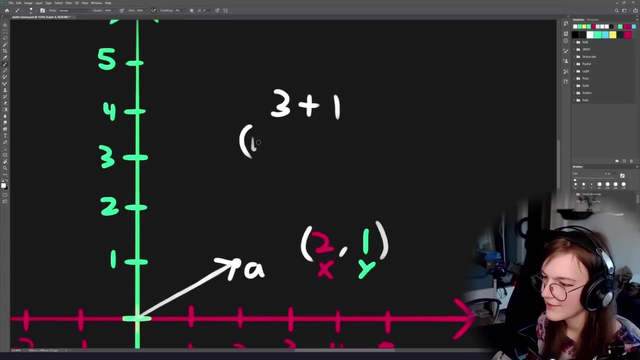 Right. And then we want to add to this. So again, when we were adding numbers, we sort of had one, a one-dimensional vector, plus another one-dimensional vector. Right, If we want to add two-dimensional vectors, you would kind of get some numbers. 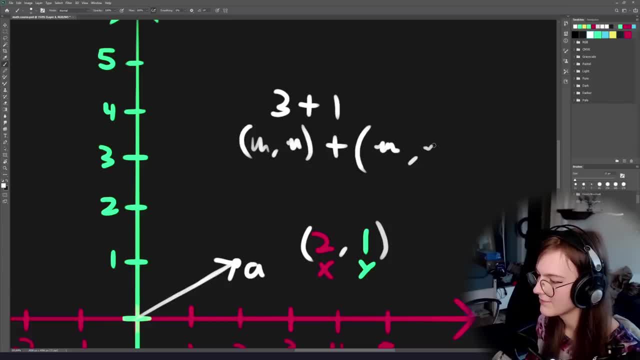 Some number here, some number here, plus some number here, some number here, Right, Because you have X and Y coordinates, Right. So you would have X Y, X, Y If you want to add two two-dimensional vectors together. 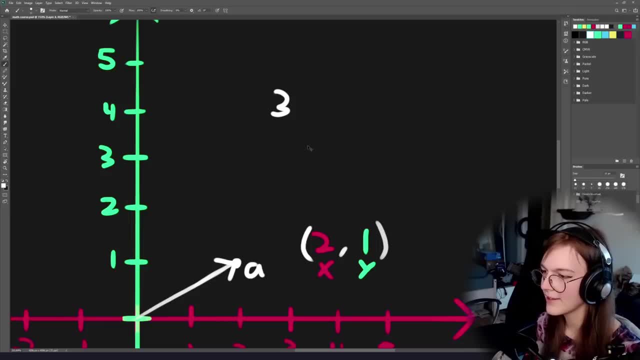 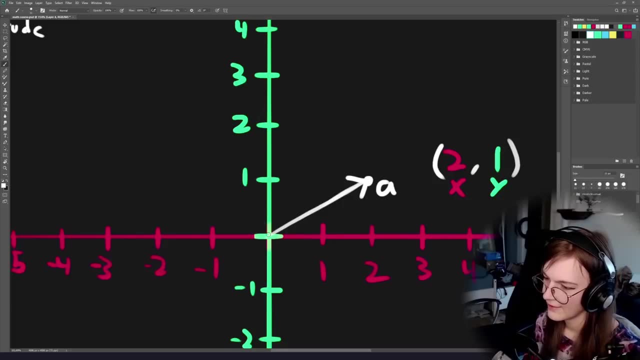 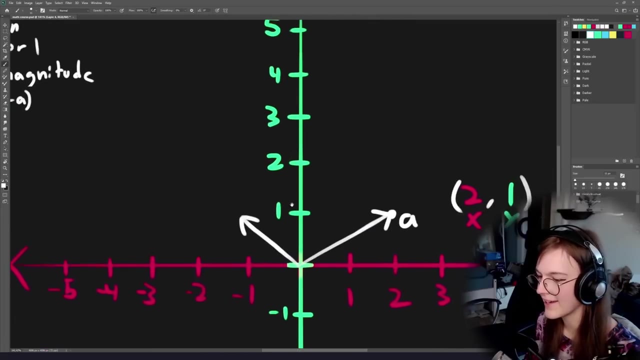 Right, Okay, So let's pick another vector. Let's say we want to do the vector here. So what are the coordinates? So this vector? There we go. A question for class: How would we write the coordinates of this vector? 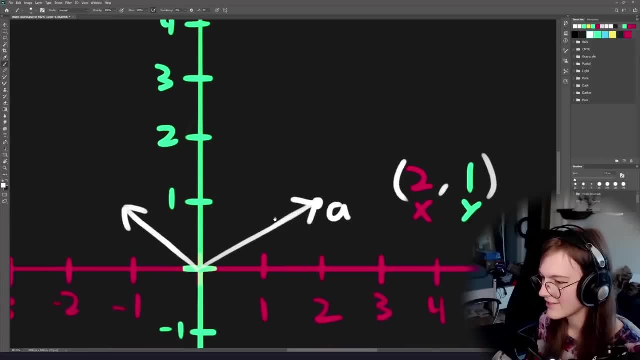 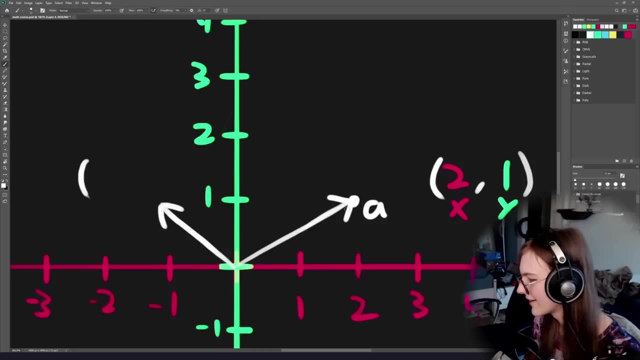 It's always really awkward when you ask the class for questions, because it's usually obvious And then some people don't really want to answer anyway And it's weird. I'm not going to do this again. This was a mistake, Okay. 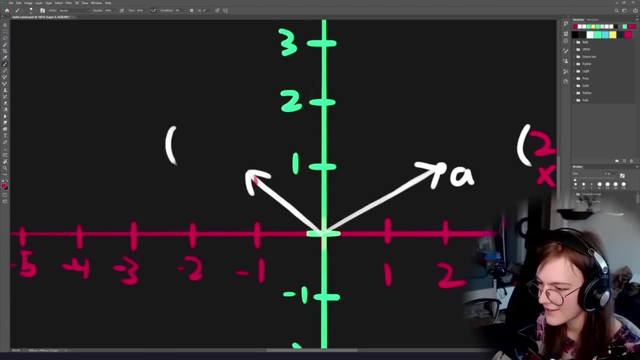 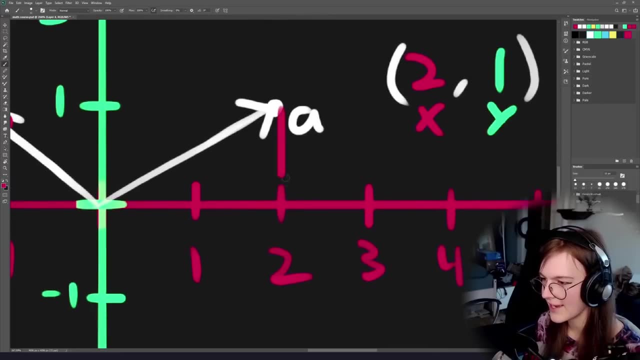 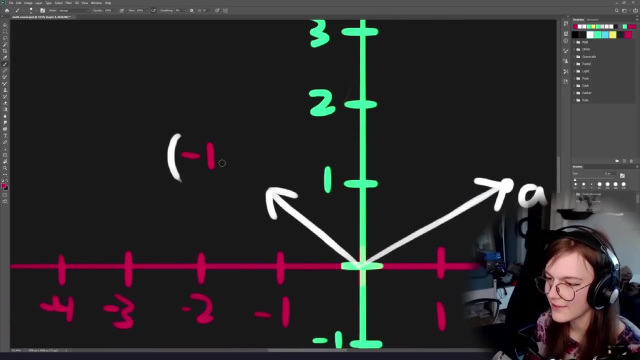 Negative one. one Exactly, Because if we look at the X axis here, this position on the X axis lands on negative one, Just like this position on the X axis landed at two Right. So now the coordinates of this one is going to be negative, one on the X axis. 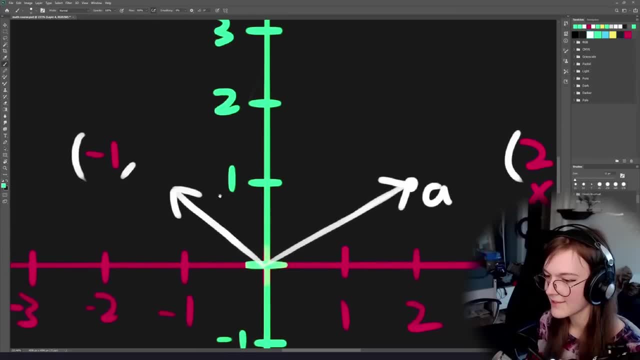 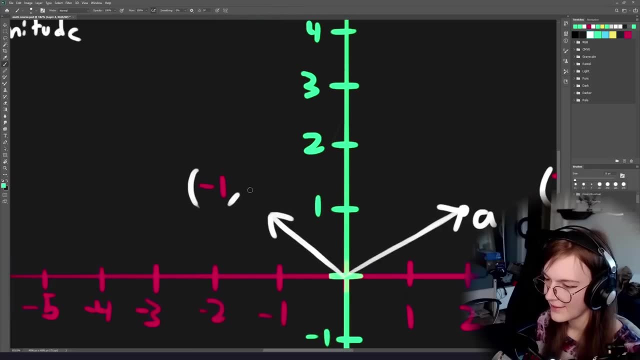 And then on the Y axis it's going to land at one, Just like the other one. This one was also at one on the Y axis, Right Cool. So this is the vector that we're working with. So let's say, we want to add these together. 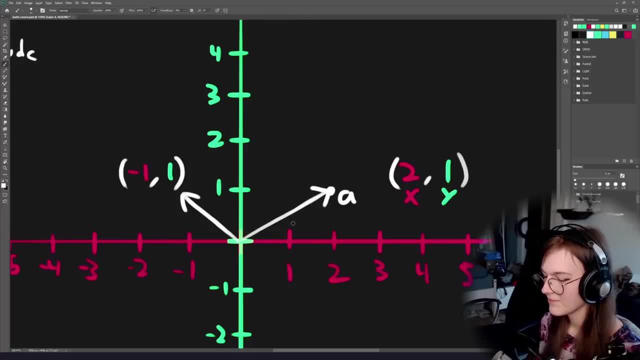 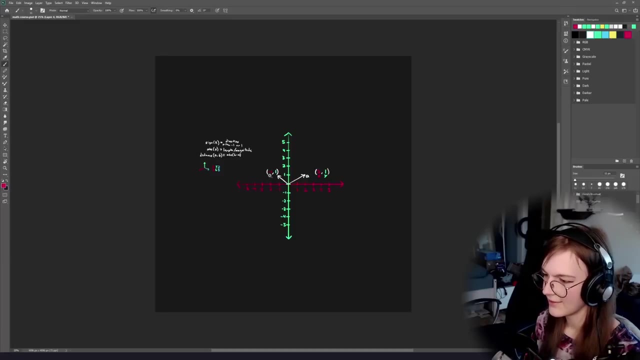 Adding vectors together, is you kind of do it exactly the same way? Right, You don't want to do it exactly the same way as you would do with scalars or one dimensional vectors, But you do it for each component separately. And Jesus Christ, Photoshop does not want to cooperate today. 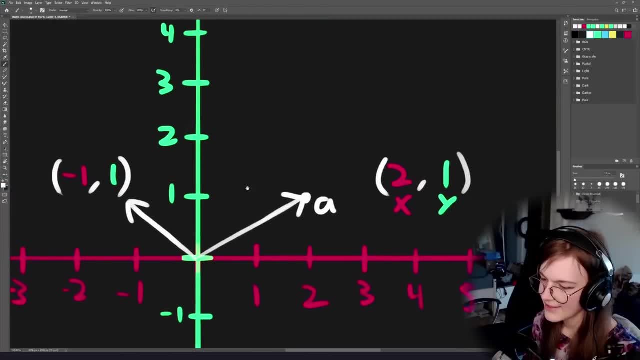 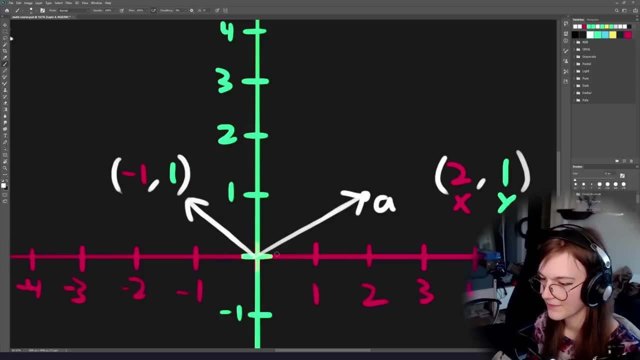 So one way to think about this visually is that you know how we sort of imagine taking an arrow and putting it on the tip of the other arrow when adding: Well, we can do the same thing with this one. We can kind of take this arrow and put it on the tip over here. 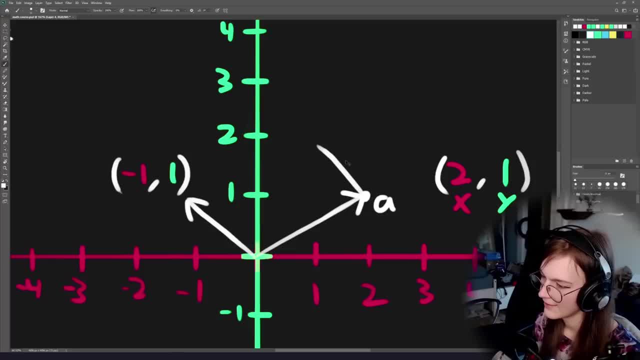 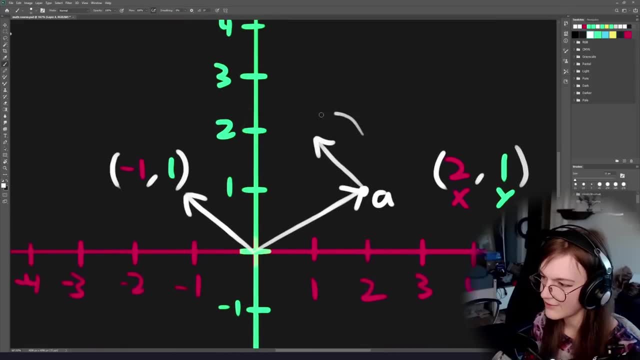 So that would give us this arrow, Right. I don't know how to draw straight lines. There we go. So now we've moved this one over here, Right, And what we end up with is that, oh, this is called B, by the way. 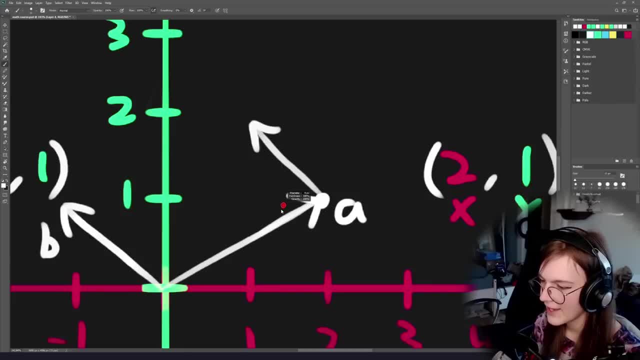 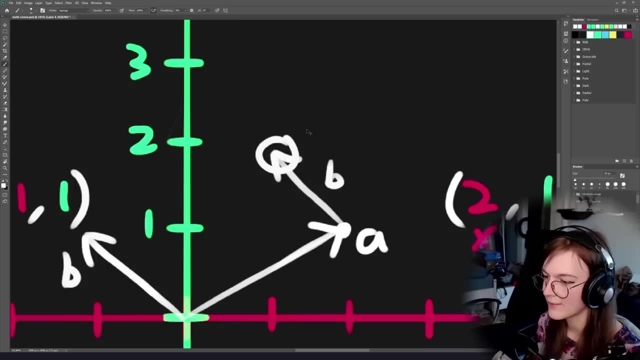 There we go, Vector B, So we have A here And then we're adding B here. So where do we end up? This is the point where we end up, right, Because we add this vector, add this vector. this is where we end up. 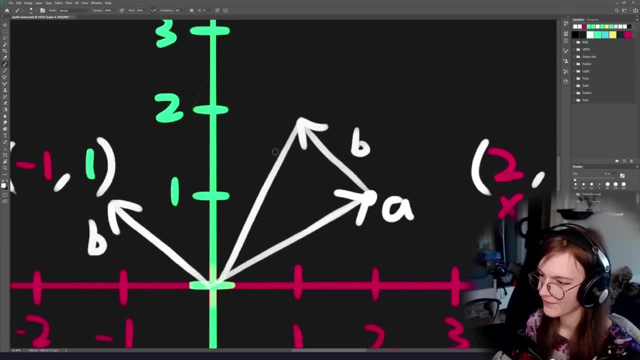 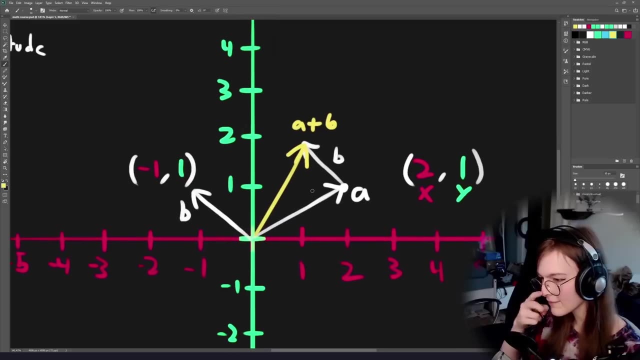 So what we get in the end is this vector right here. Let's do it in a different color, because that got a little confusing. We end up with this vector. So this vector, the yellow one, is A plus B, Right, And you can sort of. one thing that's nice about looking at it this way is that if you 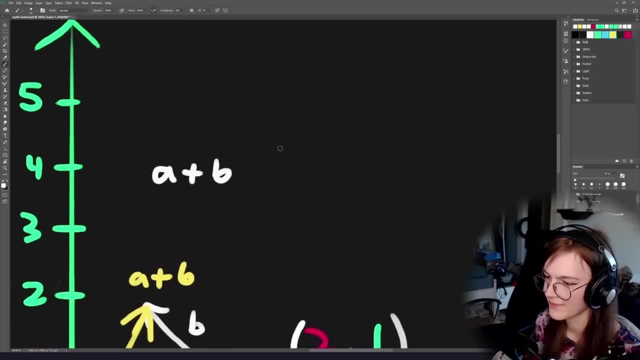 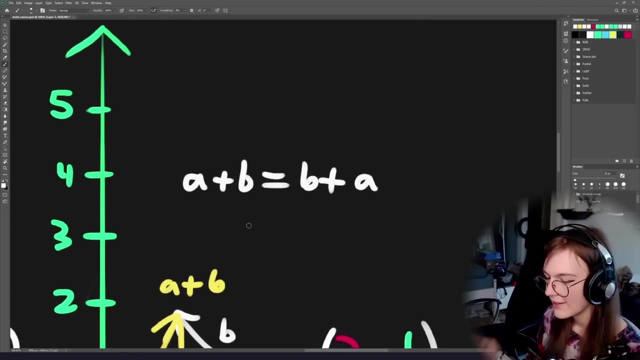 have some value like A plus B, this is actually equal to B plus A. This might seem like it's kind of trivial, that well, of course that's the case, Right, Well, why would it not be? But remember that that's not the case for, like, if you have A minus B, that's not equal. 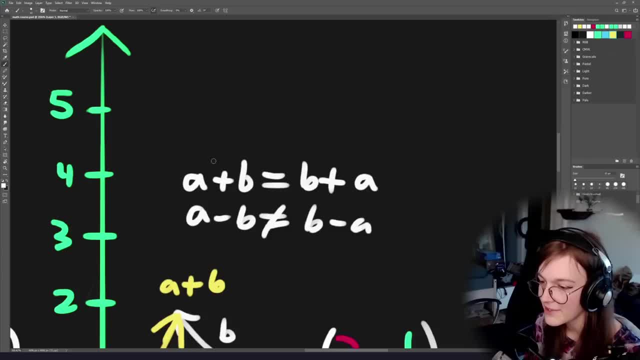 to B minus A- Right. So it's not always the case that if you flip the values you get the same result, Right. So it's really important to like keep in mind when things are. I always forget if it's. 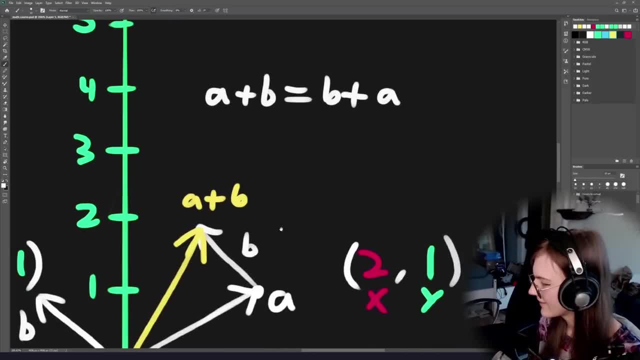 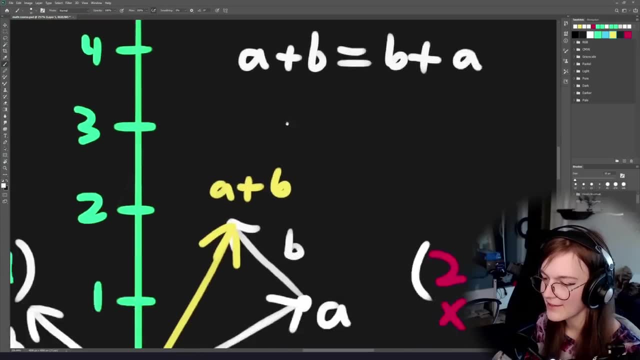 commutative or which one is which. There are terms for this, Anyway. so if we look at this, if we think about what we did here, we had the vector A at the bottom and then we added B to A Right. 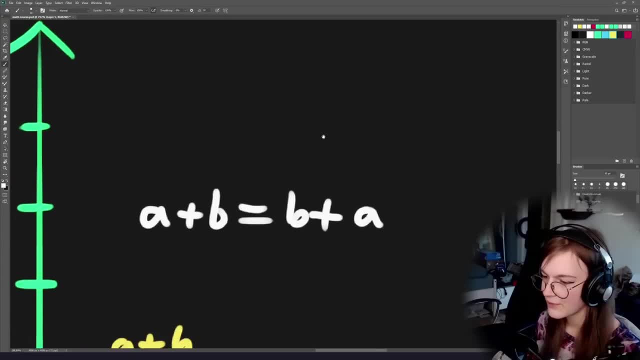 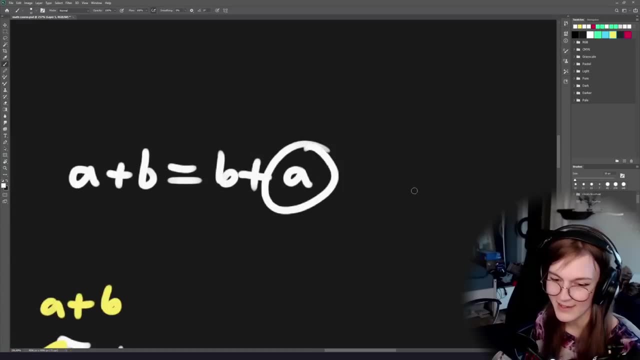 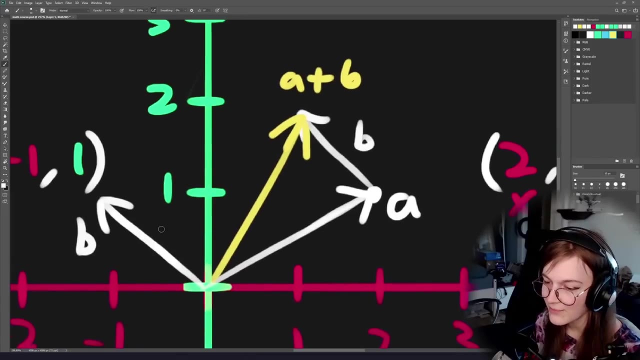 Because we added B here. So if we just look at the geometric interpretation of this, we should get the same point if we do B plus A, Right? So if we try that, then we have the vector B. So now, instead of moving B over here, we can move A over here. 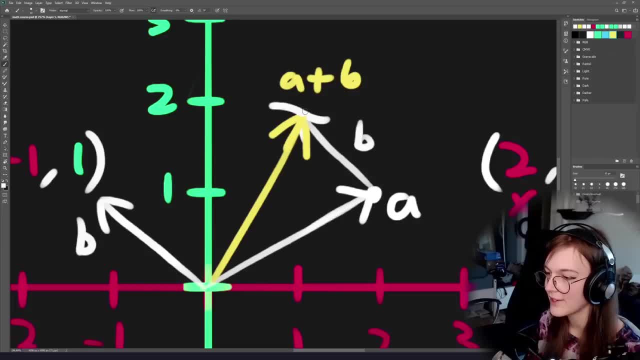 Right. So if we put A here, we end up at the same point. It's the same result, regardless of what order. we do this in Right Commutative. I think that is called commutative. Good, Okay. 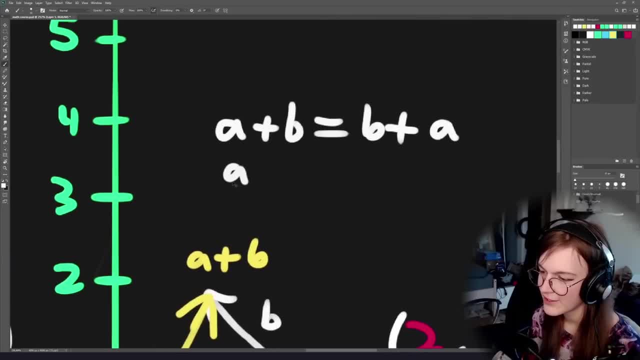 Anyway, sometimes that's a useful term to know- Like it's the same thing for scalars: A multiplied by B is the same thing as B multiplied by A, But that doesn't always apply. In some cases multiplication is not commutative. 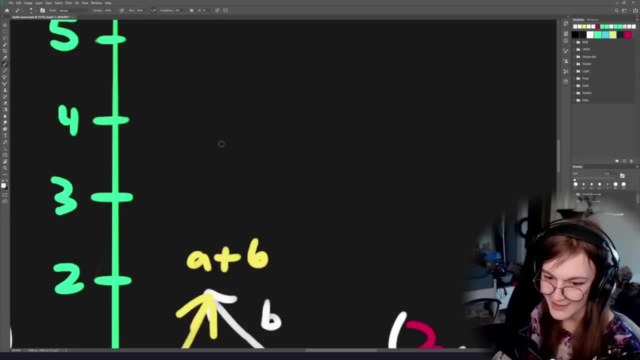 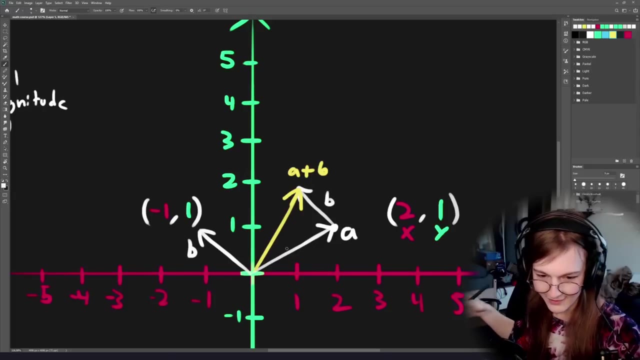 So, for instance, if you're working with matrices or quaternions, then multiplying those is different depending on the order that you do it in, But I think matrices are non-commutative. All right, Any questions? so far, Is this clear how things work, with something a little weird wonky? 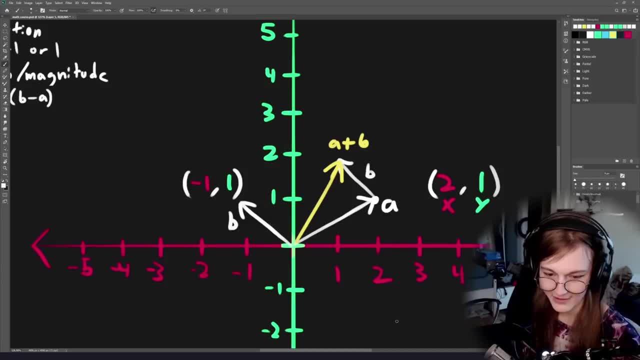 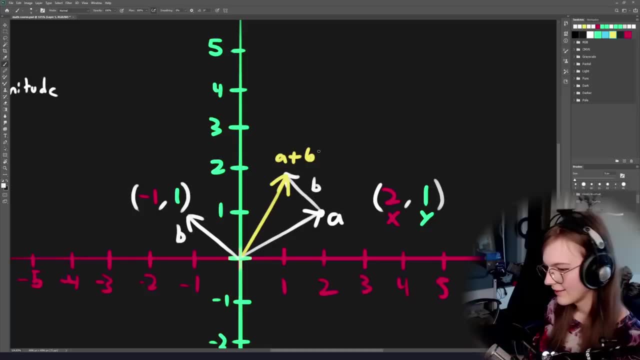 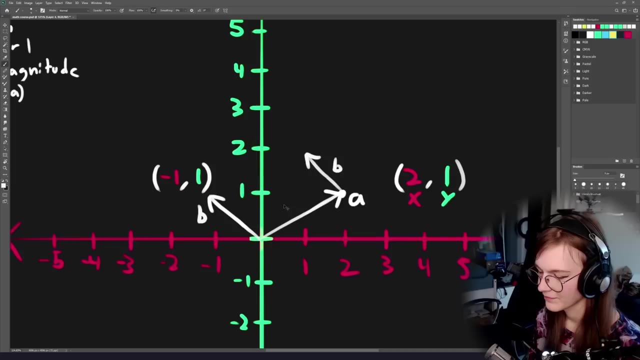 Then I guess, just ask questions at any time. I'm always up for answering questions, So that's sort of how addition works. Right, If we talk about, let's say, subtraction, Let's see I should probably undo a bunch of arrows. 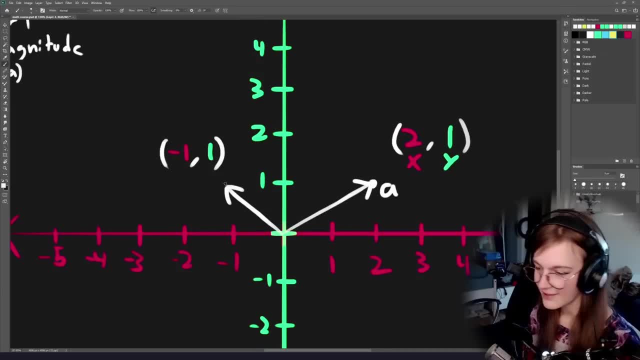 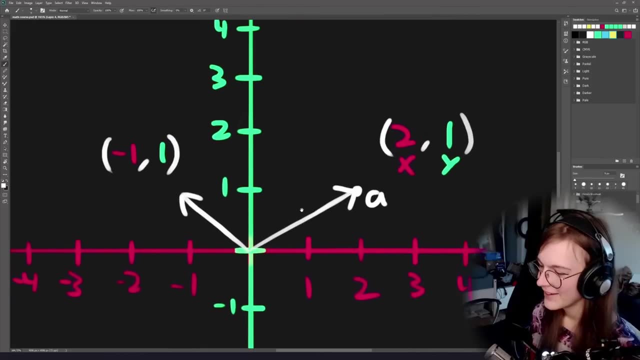 All right. So as Steve is saying in the chat that I'm not supposed to read, subtraction is addition in the wrong direction. So just like we took one arrow, put it at the tip of the other arrow. subtraction is again like we talked about before: subtraction is the same thing as addition, but we negate. 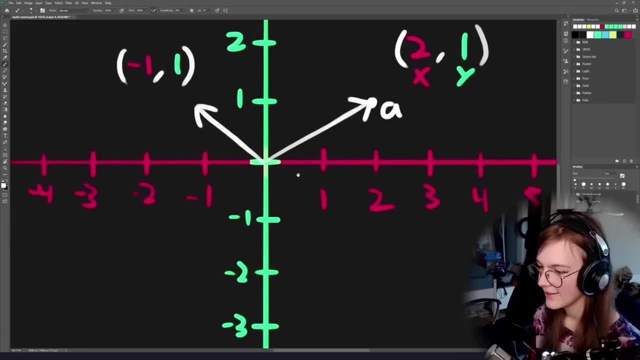 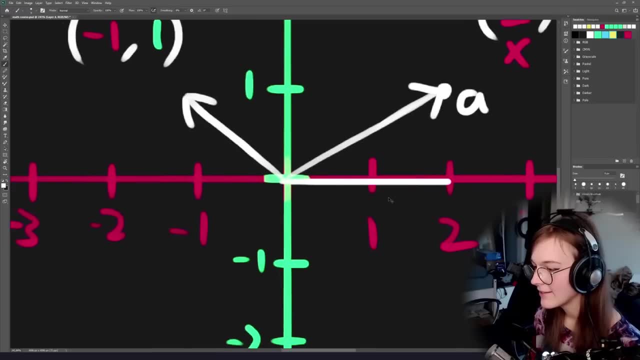 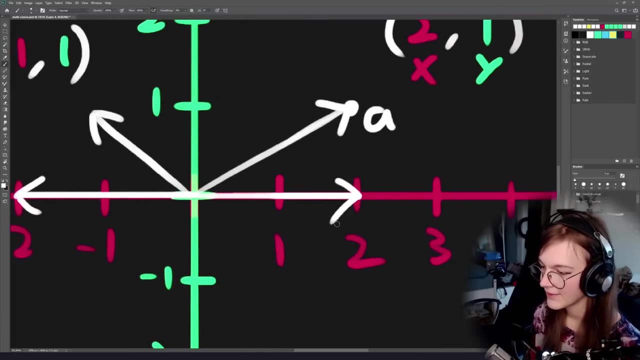 one of them Right And negate in this case. well, we were thinking about like one-dimensional numbers before right. So if we have a value of two and then we negate it, we're going to get negative two right. And if we have negative two and negate that, we're going to get two. 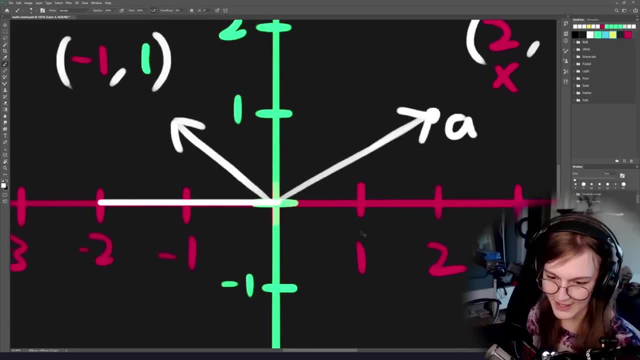 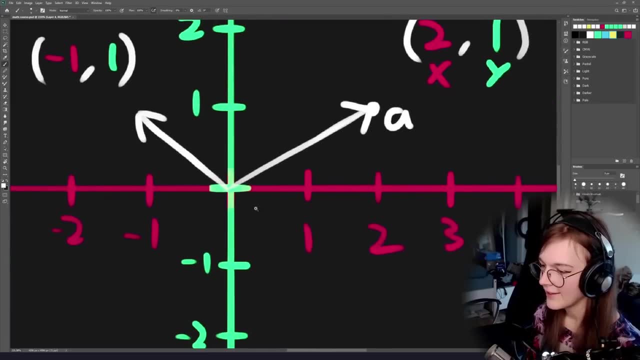 So negation is basically we flip the arrow to the other side around the origin. So in two dimensions it's exactly the same thing. We could do it like per component. We could think about like: what does it mean to negate the x-axis? 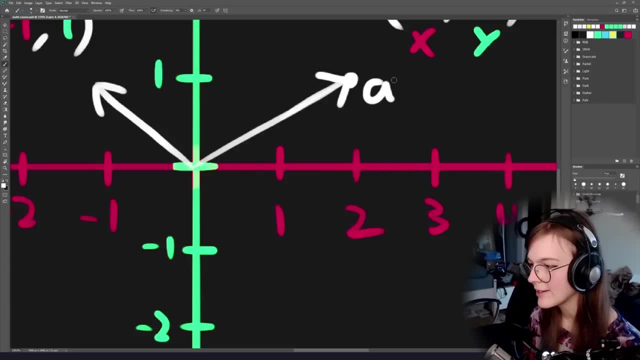 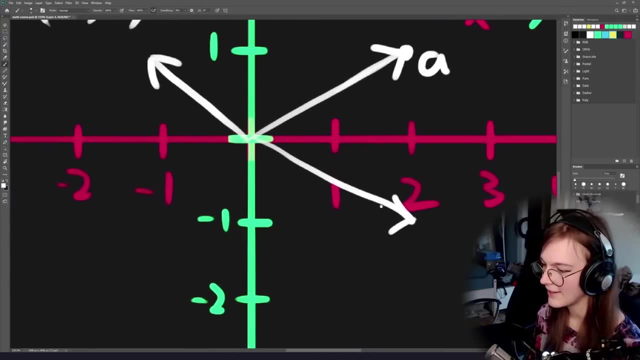 Well, if we negate the, Or if we negate the y component of this one, we're going to get this vector And then we negate the x component, which used to be two, and then it's going to flip to negative two, right? 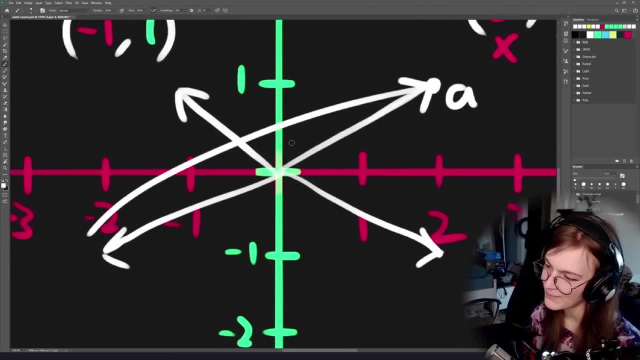 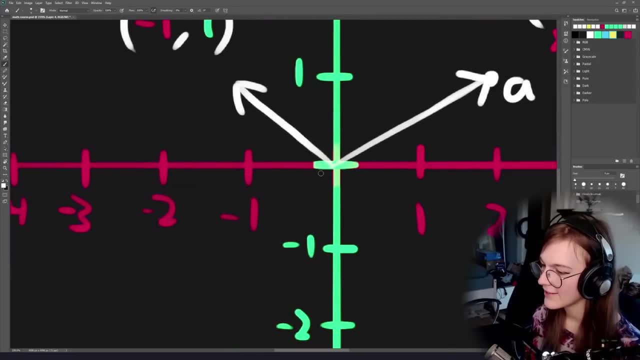 But an easier way of thinking about it is you just flip the arrow to point in the opposite direction, right? So if we negate this vector, then we're going to get this vector right, Which is the same thing as just negating these individually. 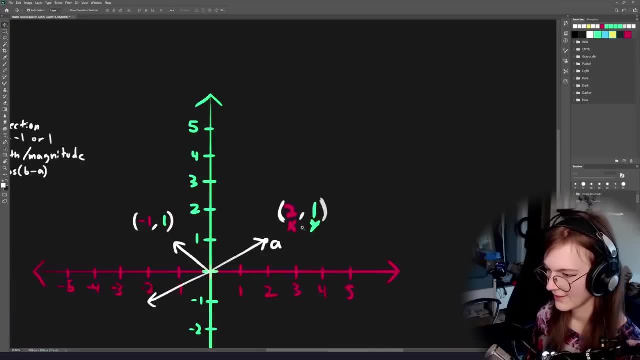 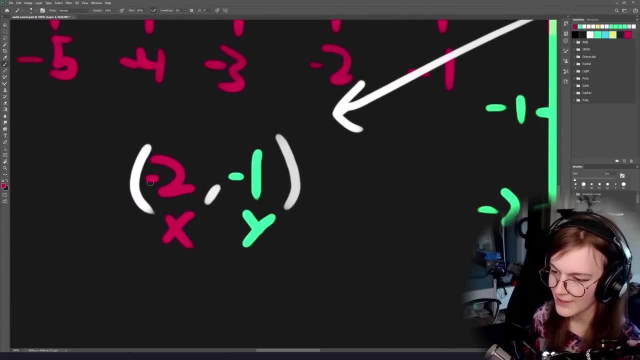 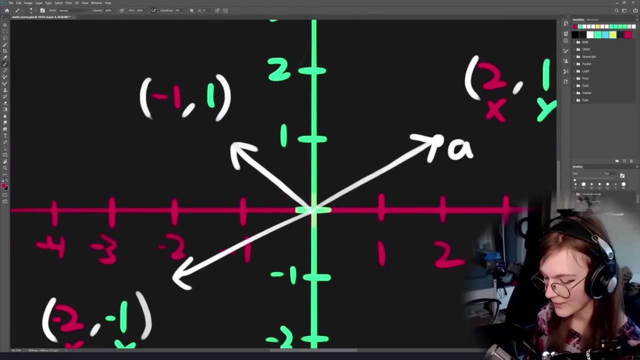 So we could just copy those, Copy those, Move them over, And then we have negative one and negative two, right. So now, if we want to subtract something, if we want to do b minus a, then we add these two vectors. 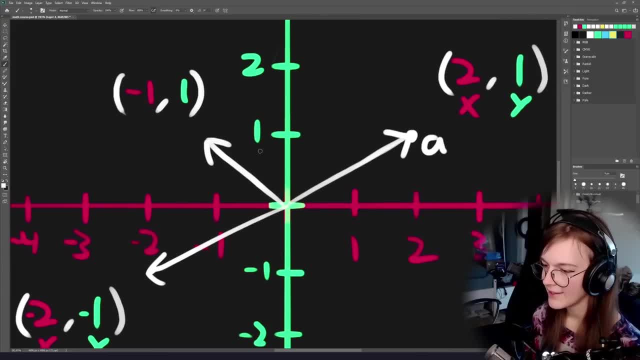 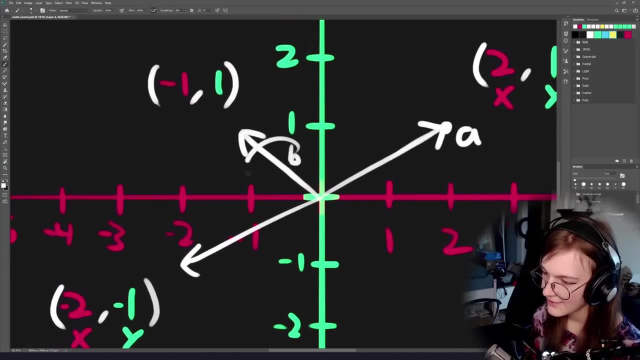 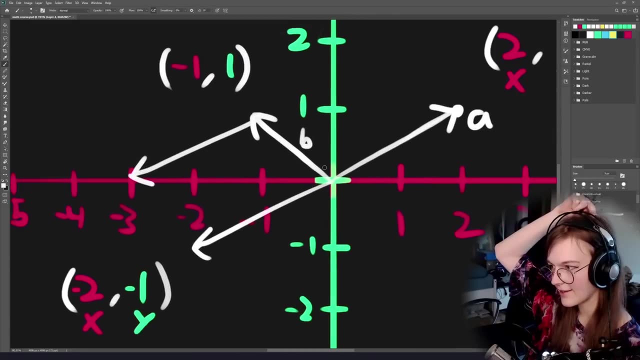 Or we do this one minus this one, right? So if we do b minus a, Then we basically take this vector and we add this vector, And then that's going to land us over here, right Yeah? And then if we did this in the opposite direction, if we flipped it, 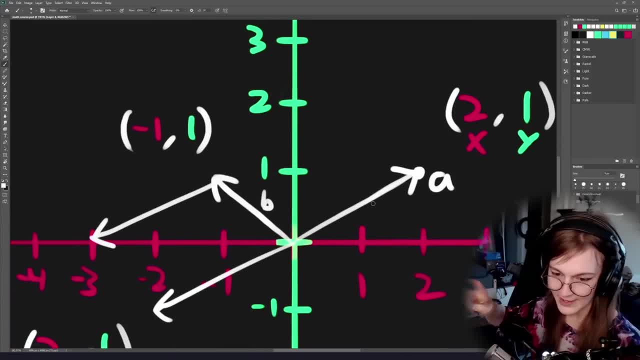 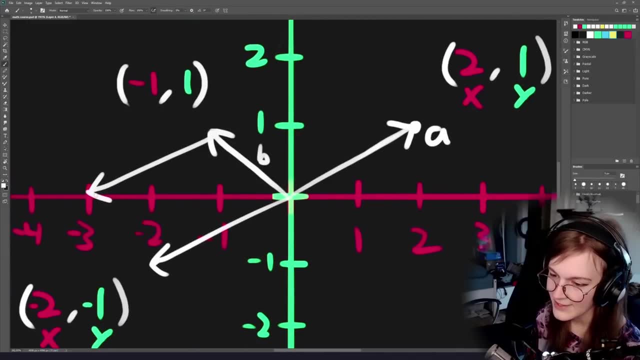 Because remember, when we did addition, flipping them gave the same result right, But in this case it won't right If we do So. this point right here: This is b minus a. This is b minus a right. 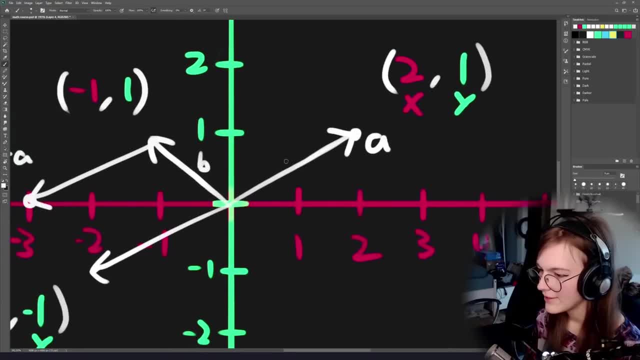 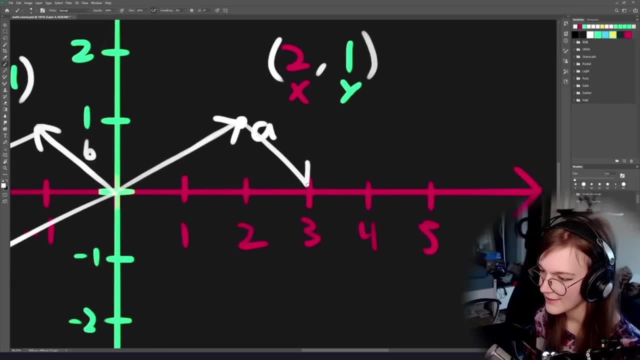 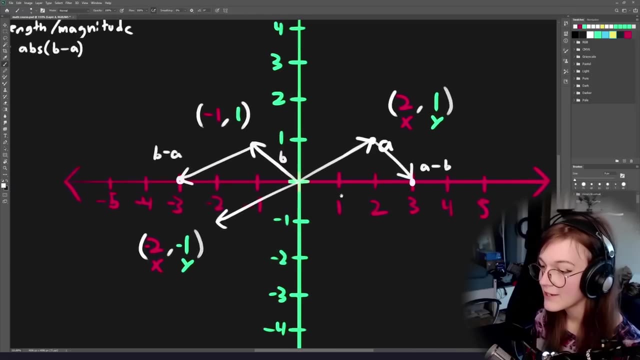 If we do a minus b, then we would, We can imagine a, And then we subtract this vector And that would get us over here, right. So over here we have a minus b. So here we can see that subtracting is not commutative. 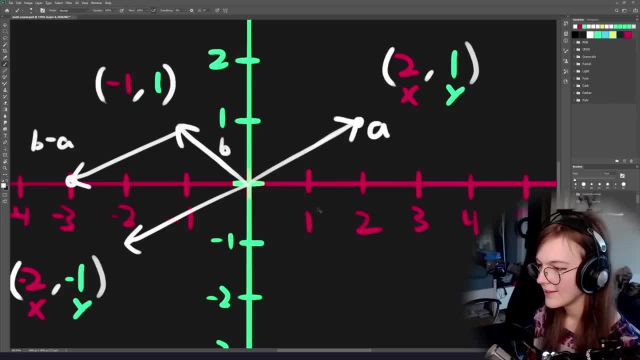 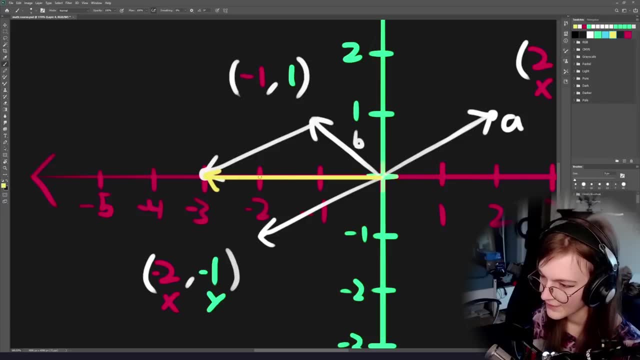 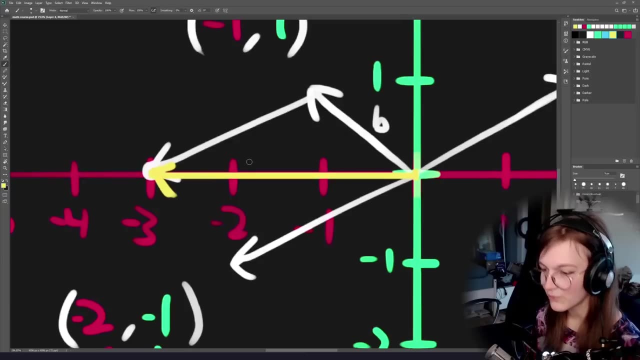 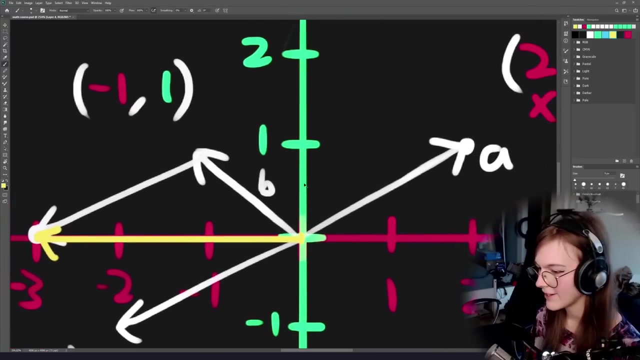 If we flip the order, we're going to get different results, right? Okay, So b minus a in this case, we're going to get this vector right here, So this yellow line going all the way here. So one thing that is really really important and crucial to know about doing subtraction between vectors is that this vector right here is the difference between the two points right. 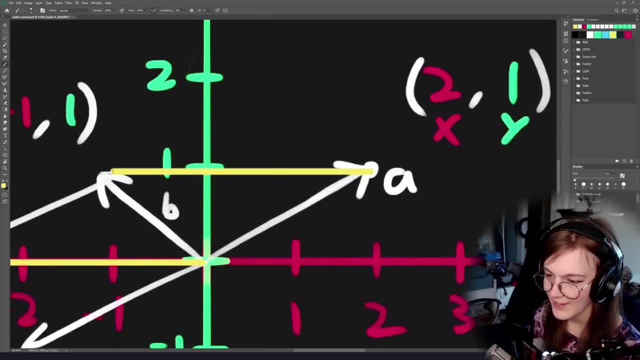 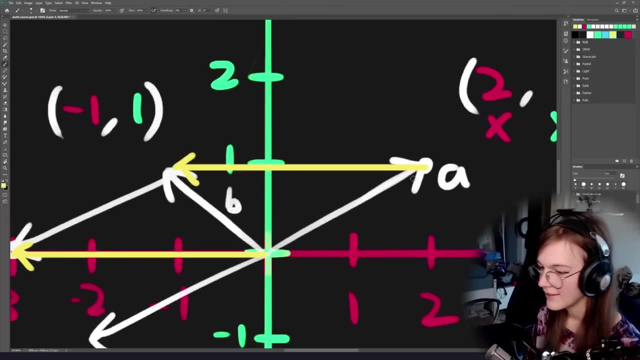 So this yellow vector is the same vector as this yellow vector, right? We've just moved it to a different place. So if we want to know, like, what is the again the difference between the points a and the point b, then that gives us this result. 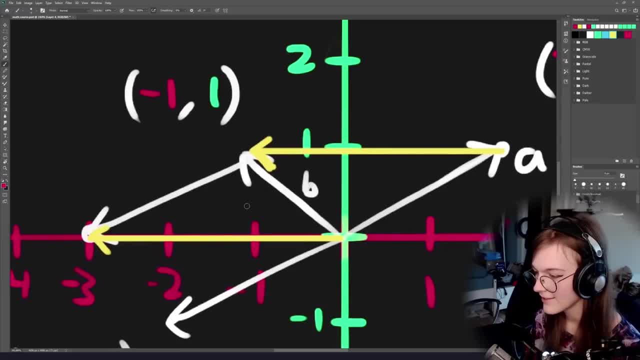 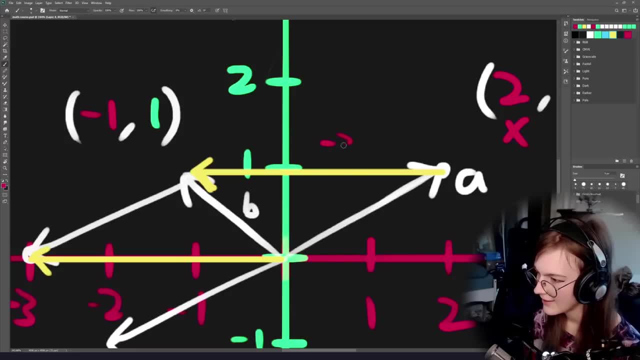 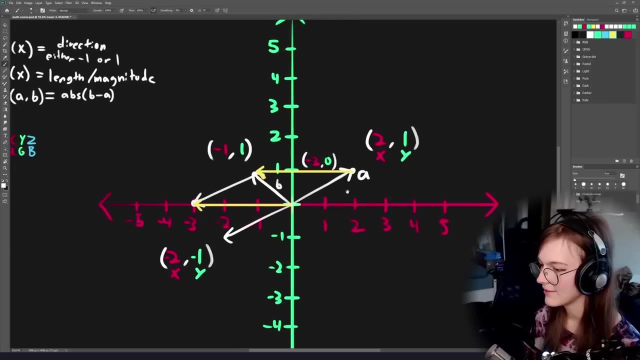 Which in this case this would be a 2D vector still. But the y component happens to be zero, right? So on the x-axis we have negative 3. And on the y-axis we have zero. So that's the difference between that's b minus a right. 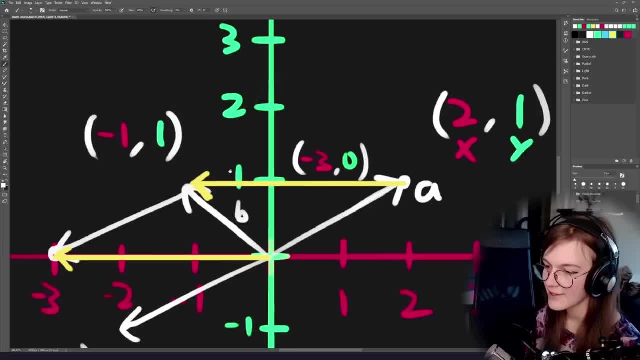 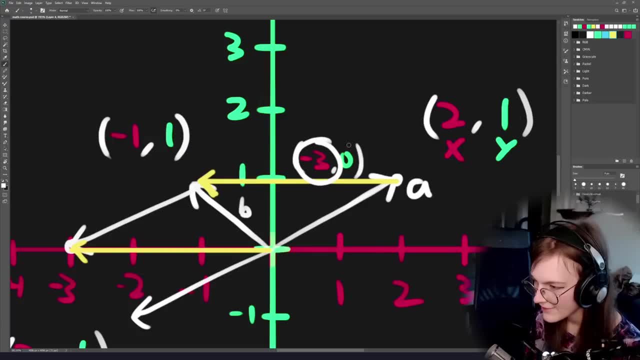 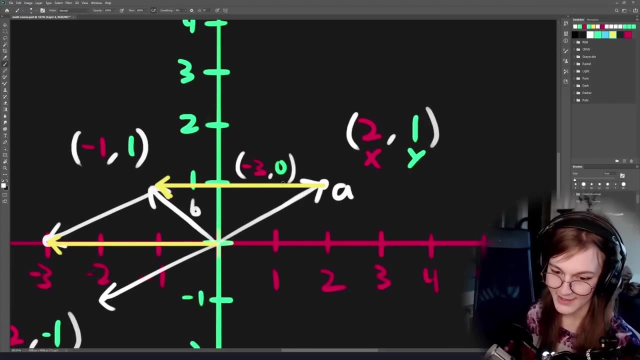 And, if you want, you can still do this component-wise. If you want to do b minus a, you could do negative. 1 minus 2 gives us 3, right, You can do: 1 minus 1 gives us zero. So you could do it component-wise as well. 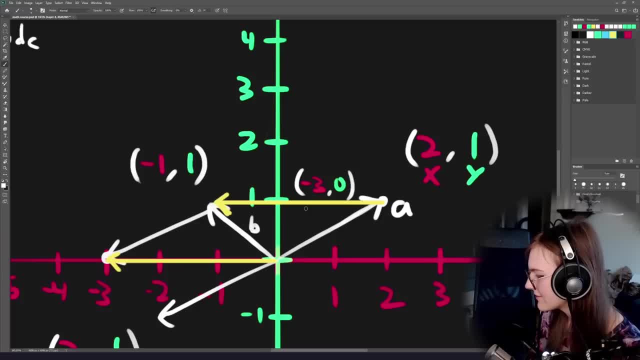 Okay, So with subtraction they become each other's inverse values- Not really, I guess it depends on what you mean by the inverse values- And they also don't become the distance from one to the other. The distance is a separate concept because the distance is a scalar. 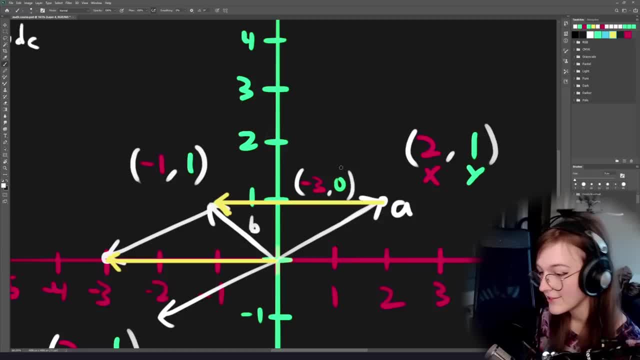 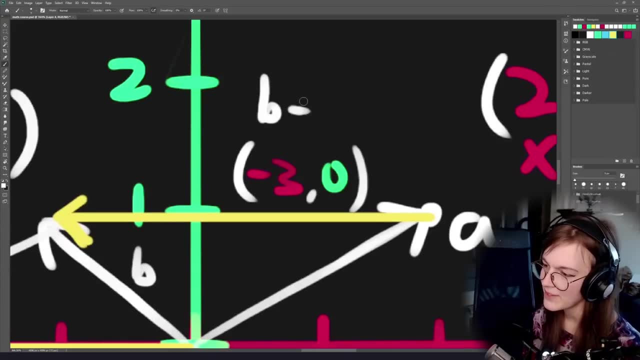 But if you subtract two vectors, you're going to get another vector, right. So the vector is a difference between a and b, right? So this is b minus a And this again is a vector, right? We're going to talk about distance soon. 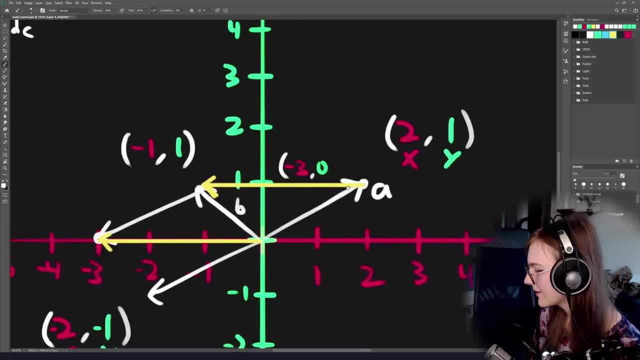 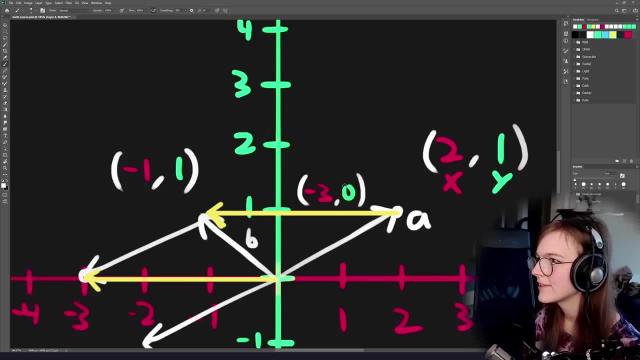 Right. So what we're doing here is we're doing b minus a right. Better described as an offset, Technically it's called a displacement, Or usually a displacement is used when it's like over time, I think. 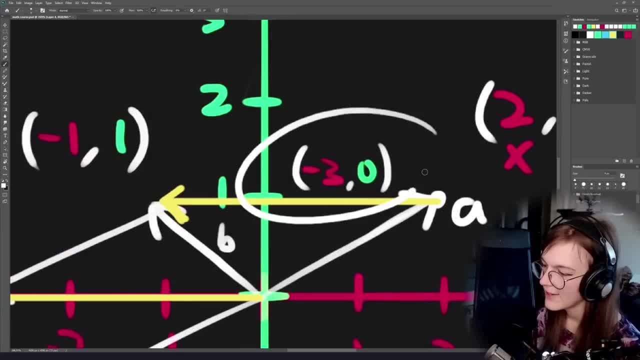 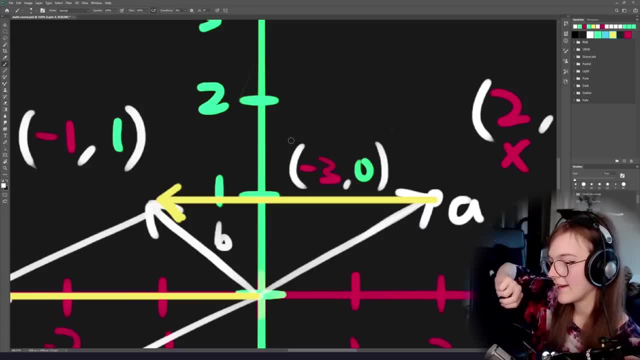 But yeah, Anyway. so it's important to remember that, like this vector, the way we want to interpret this, if this is the difference between b and a, is that this is not a position right Now. vectors don't inherently. 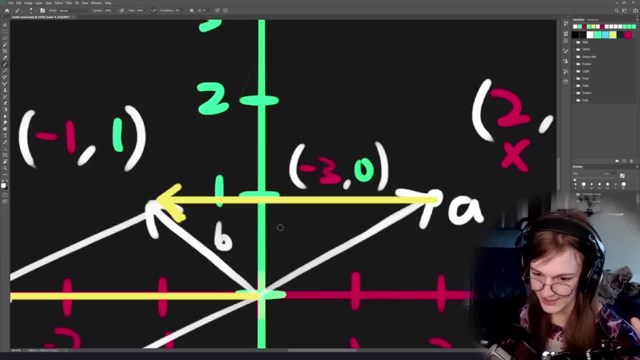 They don't inherently have a property that makes them a position or makes them a direction or makes them, you know, a quote-unquote vector. But we need to interpret things right And that is like super important to know what each vector represents, right. 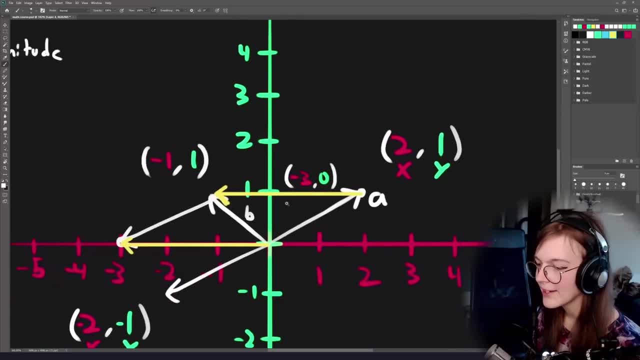 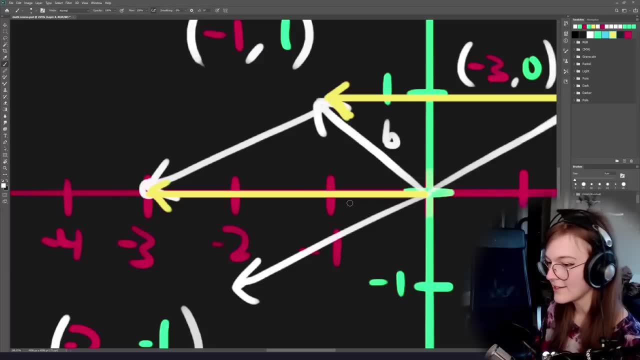 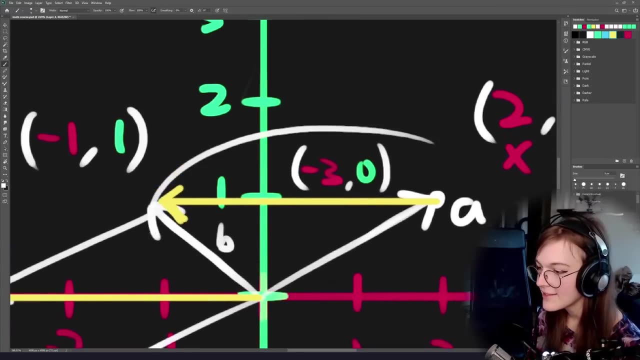 So if we have this vector negative 3 and 0, it's more helpful to visualize it as an arrow between a and b, But the actual values is negative 3 and 0 on the y-axis Right. So it's really important to like interpret this in the correct way. 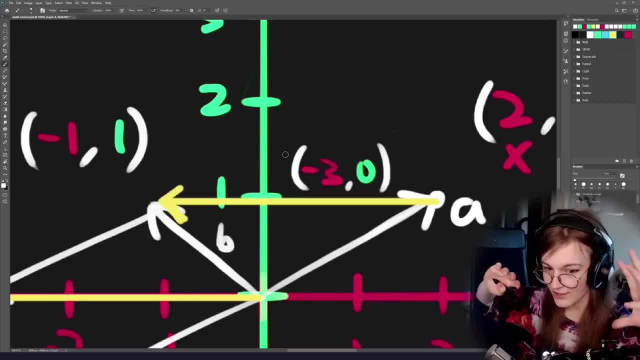 And also, when you're writing code, make sure that you're actually clear about what this is right, Like if you want to keep this vector for something, call it b to a, Or call it the difference between something Or the delta. 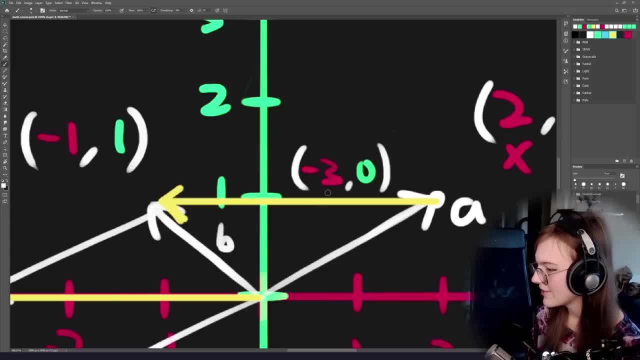 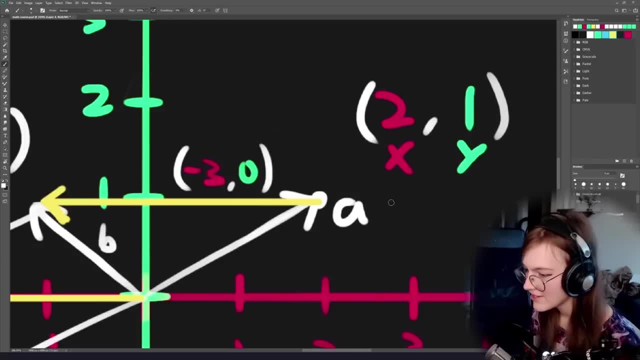 Or whatever. But if you just have a vector, then you're not entirely sure like: should we interpret this? Should we interpret this as a position? Should we interpret it as a position relative to a Which we are in this case? 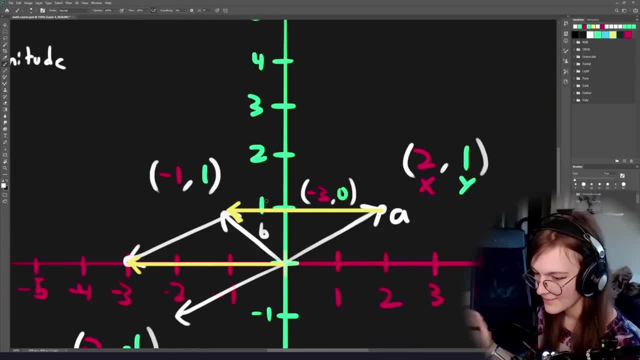 And so forth. Right, Yeah, So this is like a very crucial concept. It's very important Once we're getting into using different spaces. So when you're doing a lot of things in game dev, the difference between local space, world space and all of that stuff is really important. 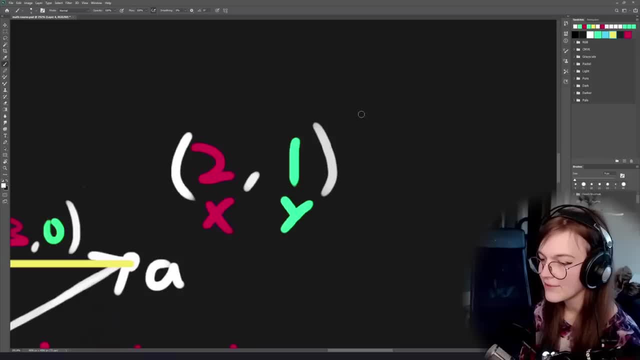 So you need to keep track of, like you know, if you have a vector like this, If it's in its own, this one doesn't say if this is in local space, if it's in world space, if it's relative to some other point, or like how this is used. 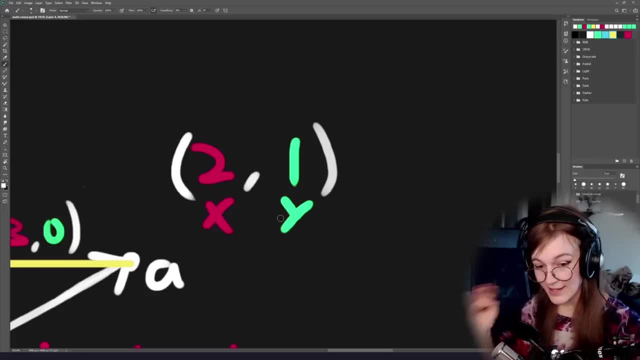 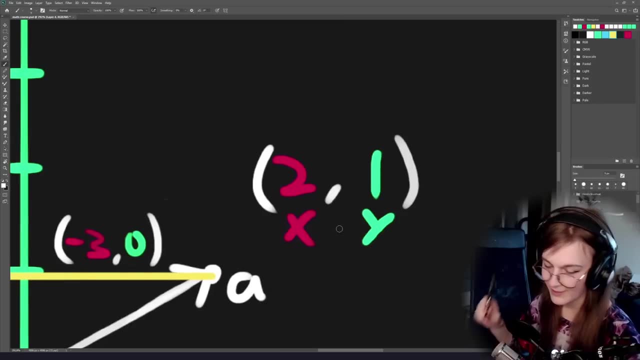 Right, So always be like very careful, like how you name your variables, when it comes to this. So like the. So this is something that I hate. math for Math is so bad at this. Math notation generally is really garbage. 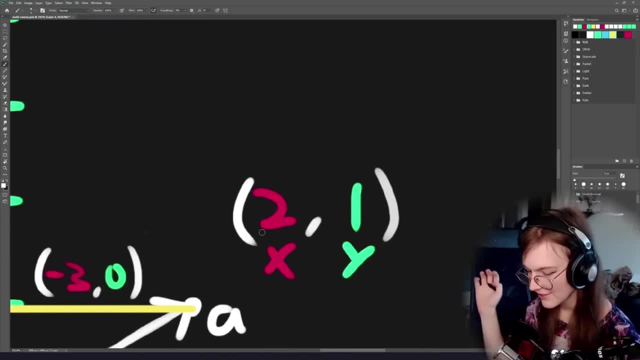 Because they Like there's so much stuff. that's very implicit. It's not notationally ambiguous, But in code we can actually name variables. We can make functions that are very clear what they're doing. So in code you can be very explicit. 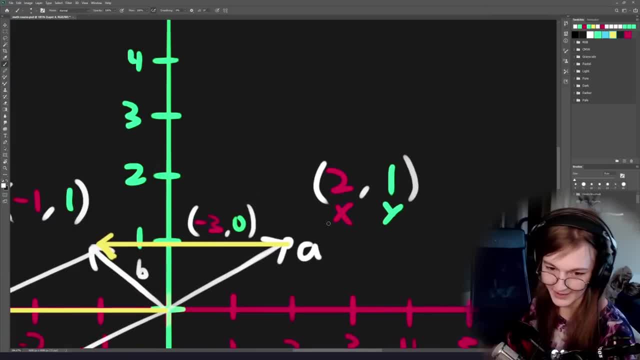 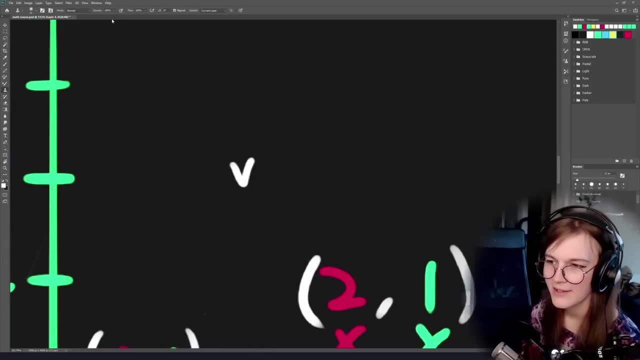 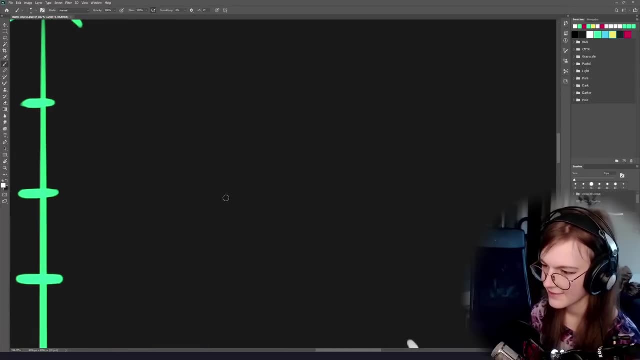 And I think that's really good, Because math is unreadable sometimes. Yeah, In math you would have things like: well, if you have V, then you need to restart document again in Photoshop. Thanks Photoshop. So sometimes you will have papers. 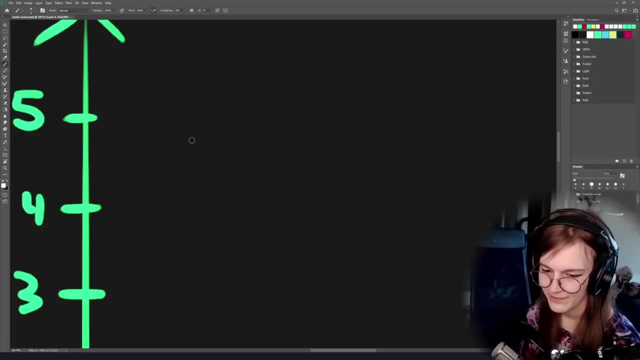 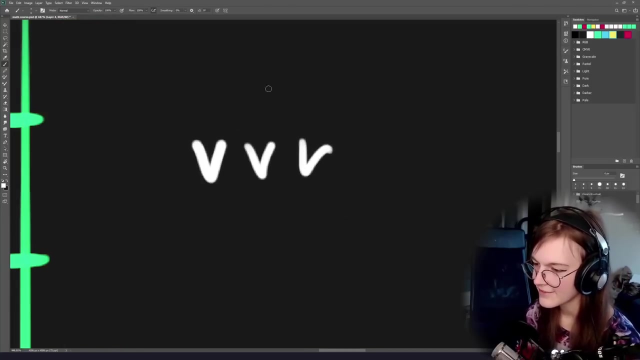 This is an actual case, by the way, Where like V means one thing- This is bold. But then you have a non-bold V that means a different thing, And then you have a cursive V that means something else. Like this is bad. 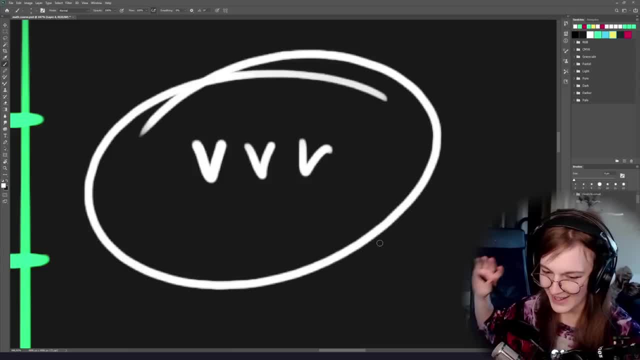 Like don't do this. I hate it that, like math papers actually do this kind of garbage. So like you will run into this, especially if you're like reading shader papers or whatever. That kind of stuff is really frustrating. 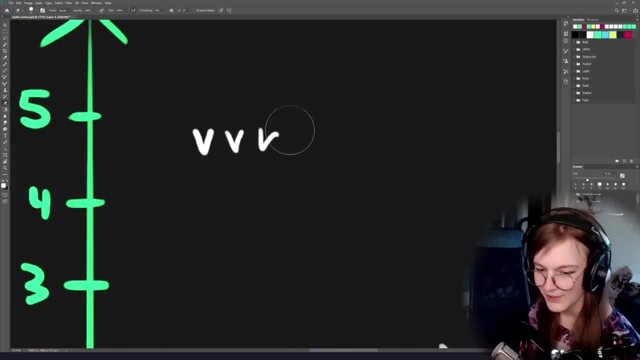 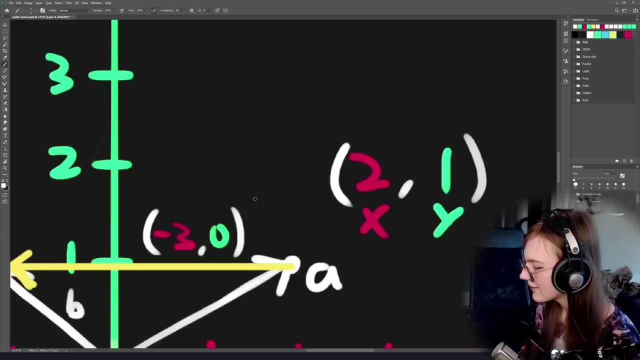 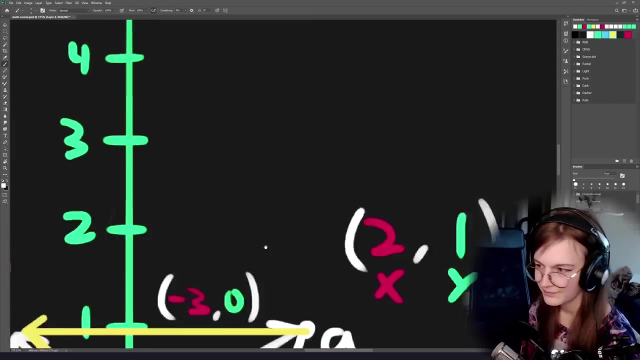 Yeah, So math notation usually relies on these types of things And it's really annoying. But in code, be explicit, Be very, like, clear with what everything is, Have variable names that make sense and so forth, Right, Yeah? 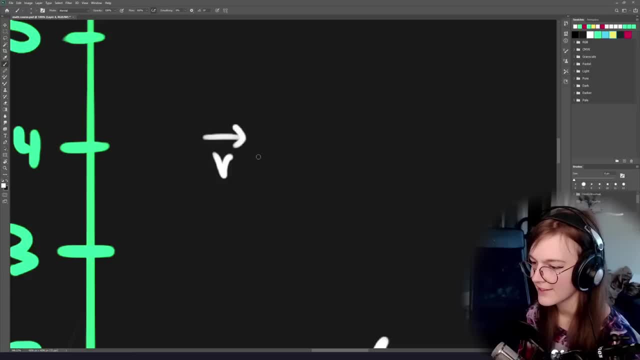 And then you would have things like: oh, if it's bold, this is a vector, But we don't draw the vector arrow because we're just going to presume that people know that this is a vector now, And if it's cursive, it's a scalar. 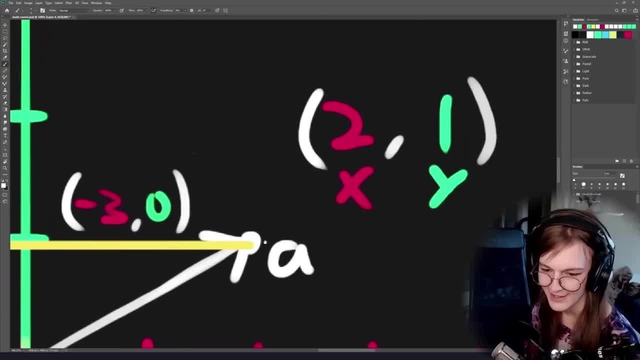 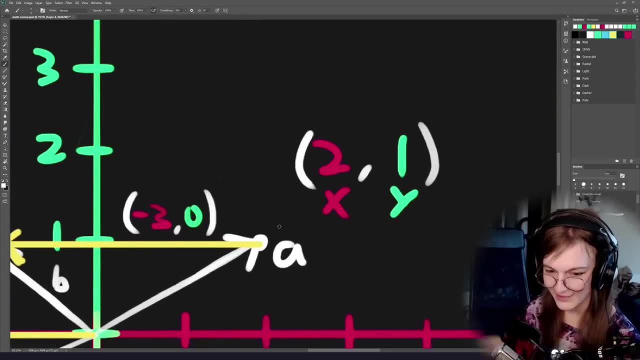 This is a component of the vector or whatever. It's frustrating, Anyway. stuff like this is why I don't call myself a mathematician, because I kind of hate math notation And I also don't know much math outside of game dev. Oh, speaking of which, if there's ever something where you are like, when is this going to be useful? 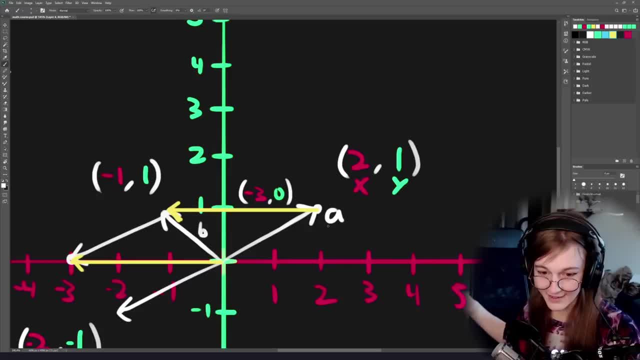 Or what is the point of this? Ask, Just ask. Everything I'm going to talk about is useful for game development. None of this is going to be like esoteric, unuseful, They're just bad things, Right. 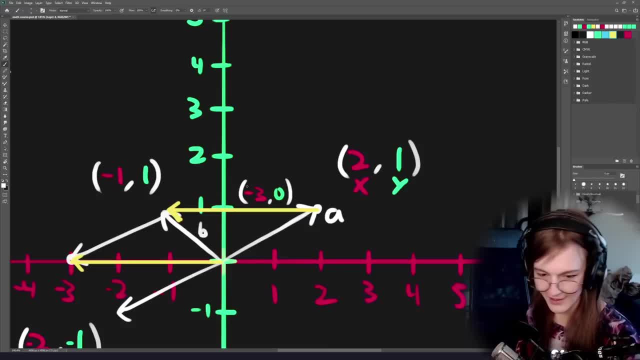 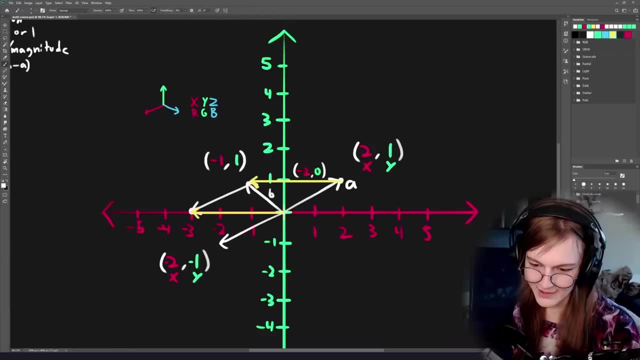 So don't be afraid to ask, like: when am I going to use this, Or can I order fries with trigonometry, That type of stuff, Right, Just feel free to ask questions. In my experience, vector math is probably 50% of gameplay programming. 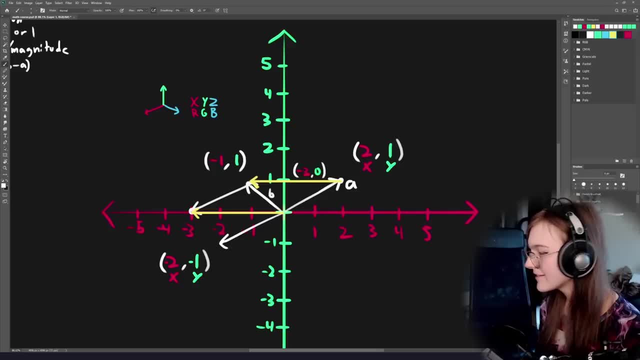 Yes, Pretty much Like. it's like again. people ask me many times like: do I need to know a lot of math to do game development? I'm just like: no, Not really. You need like vector math, trigonometry matrices, help. 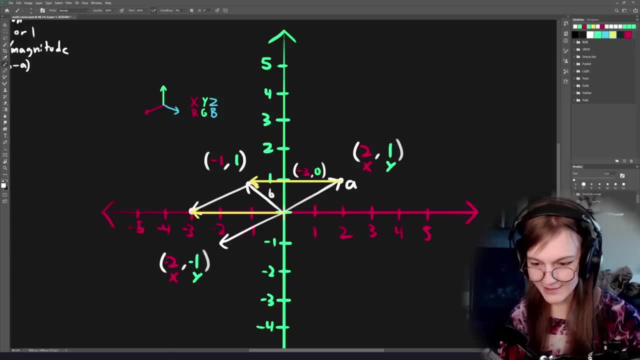 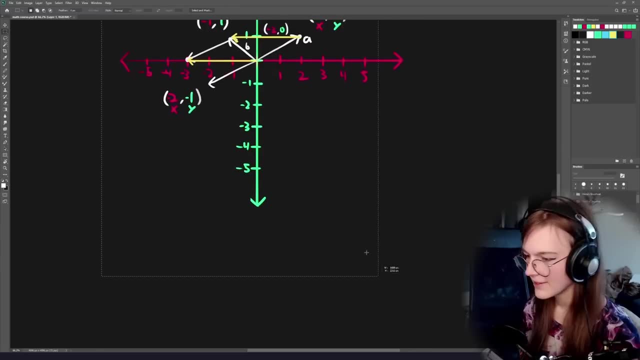 And then you need to know how to manipulate values like remapping ranges, doing oscillation, that kind of stuff. But usually you don't need that much. Anyway, I'm going to take a picture of this and send it to the students, in case people want to keep this beautiful piece of art. 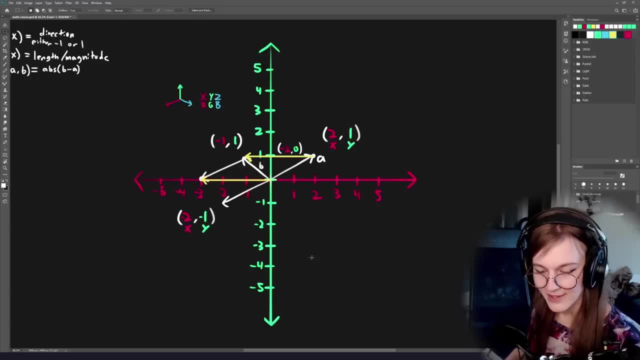 What does orthogonal mean? That they are 90 degrees off of each other. Have you ever worked in non-Euclidean geometry or altered space in any of the games that you've made? Not really. no, I guess there are, like there are, matters of like interpretation. 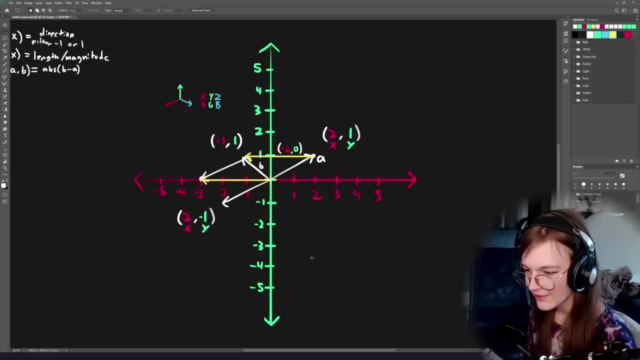 Right, I mean, if you want to call polar coordinates non-Euclidean, then yes, But usually outside of that. no, I haven't done a lot of that, Mostly because I like, I don't know, It's like seems like it might be fun, like experimentally. 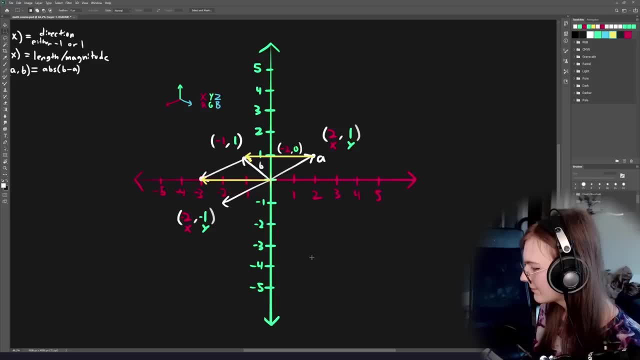 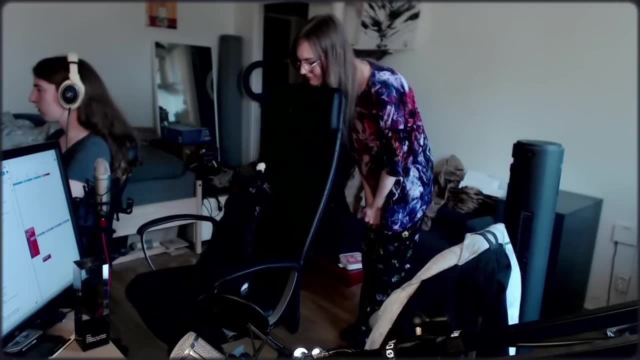 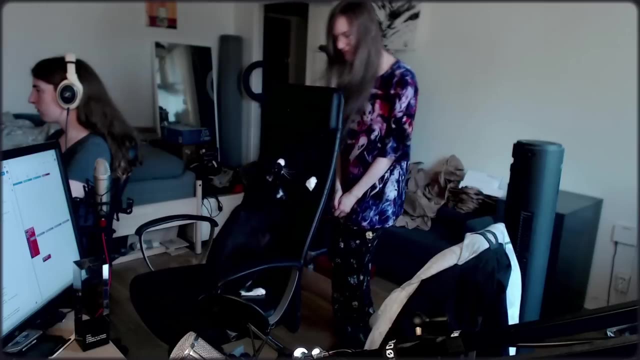 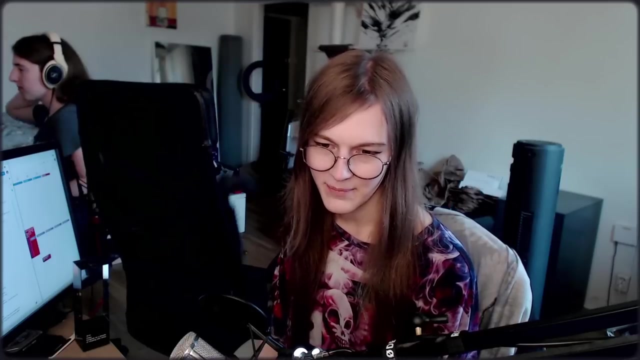 But I don't think I'm going to actually like make a game out of it, But it seems like it might be fun to like try those things. Keep playing Boop. Hey, Most interesting math problem I had in game. dev is trying to forecast the path of certain projectiles. 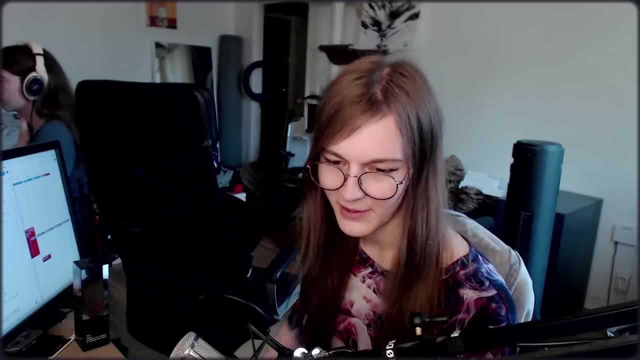 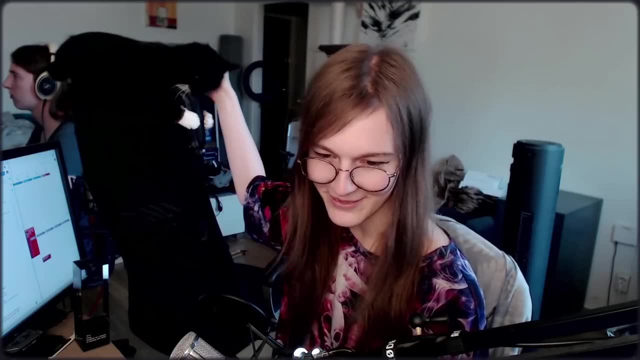 That is a thing we're going to talk about, Like ballistic trajectories, Freya's game dev math course. This is a vector. It's like two numbers stacked together. Twitch chat, Lauren's transform- Yeah Yeah. Last time I did a math course on Twitch there was someone who was like an actual mathematician. 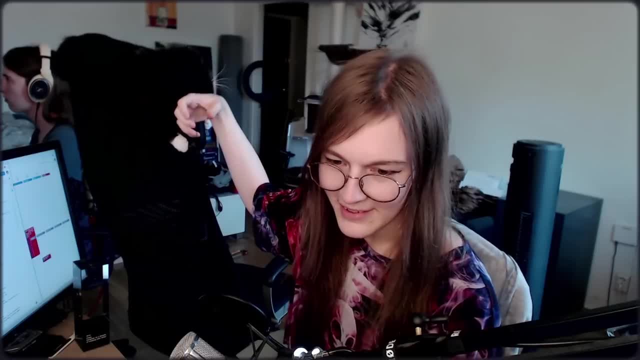 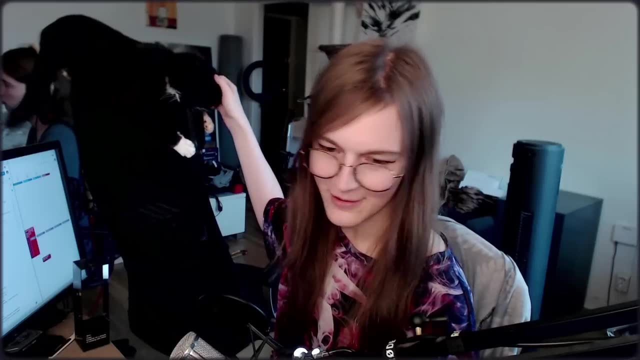 And every time I brought up a concept, they would like bring up the incredibly esoteric, like really complicated generalized concept in math with like really complicated words, And I'm like this is not the time, Like I don't even know what those things are. 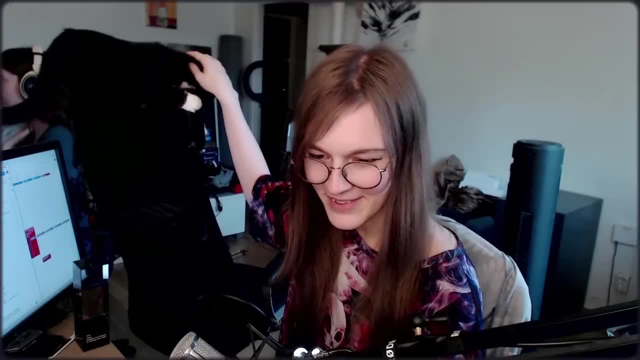 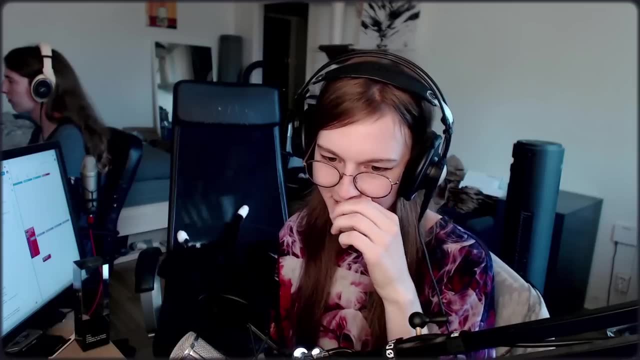 Chill, I'm not going to be able to explain, I don't know. lie groups and algebraic rings to students, Ah jeez, It's amazing how people can understand esoteric concepts in math but not regular social norms, Kind of yeah. 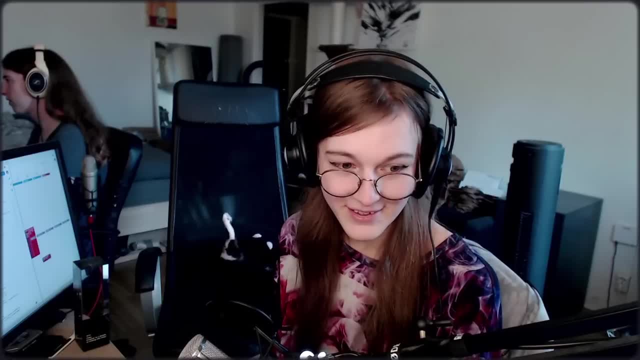 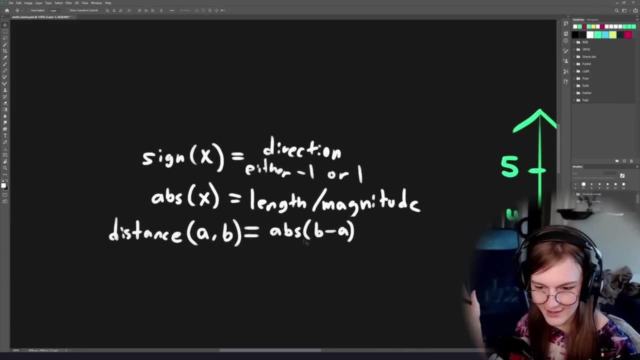 Well, but they are separate skills, So you know, that's how it goes, Okay, so we talked about these things, right? We talked about the sign of a value. We talked about the length or the magnitude of a value. 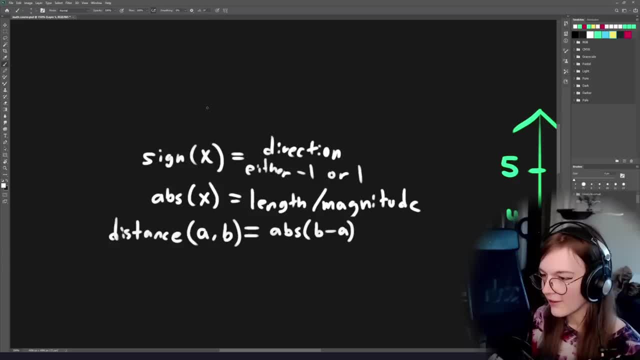 We talked about the distance between two values. All of these concepts also generalize to 2D and any other numbers of dimensions you want to use. So it works for 2D, 3D, 4D, 5D, however many dimensions, your game is in right. 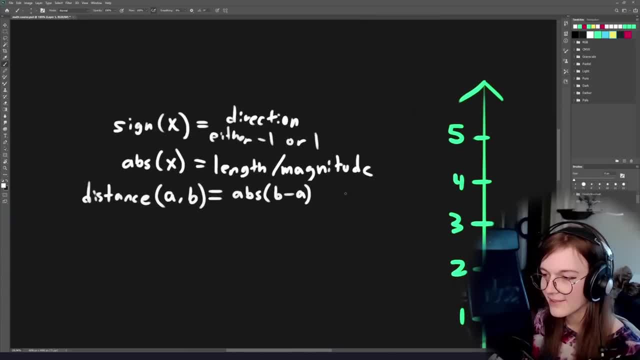 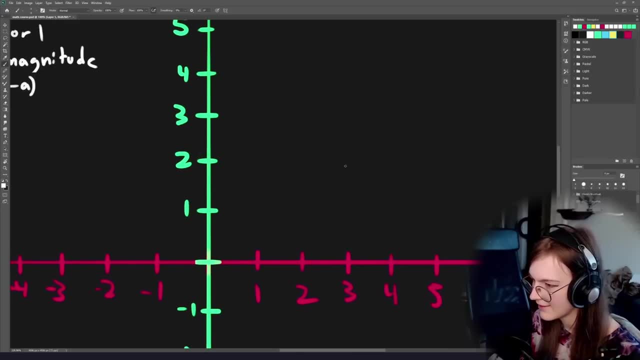 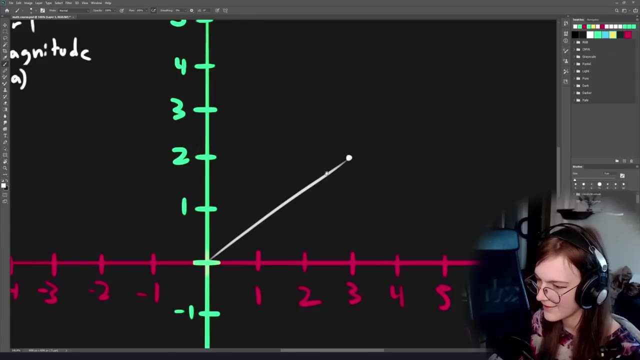 Okay, so let's see what these would mean in 2D, right? So let's bring back some vector. Let's say we do this one. You know, drawing straight lines is one of the hardest things in art. There we go. 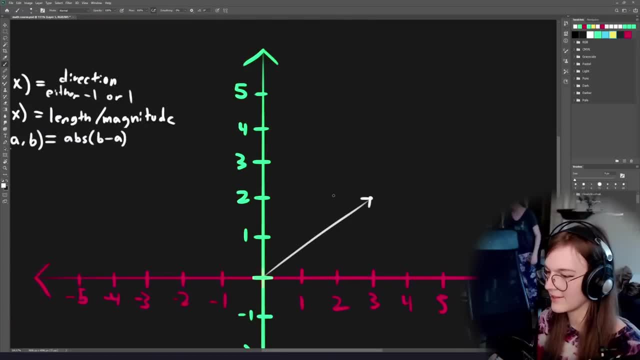 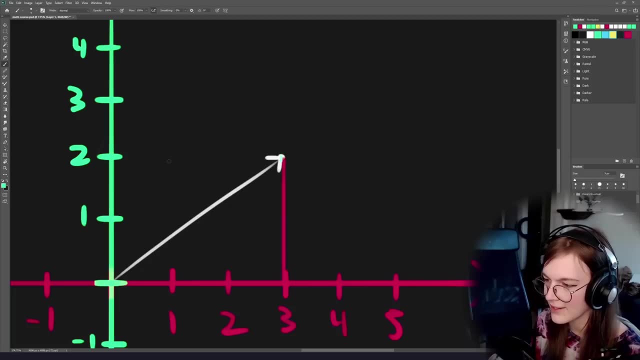 Nailed it All right. So now we have a vector. Cool. So the components of this vector: again, we can look at the axes here for the X and the Y components, And then we can see that the X component is 3.. 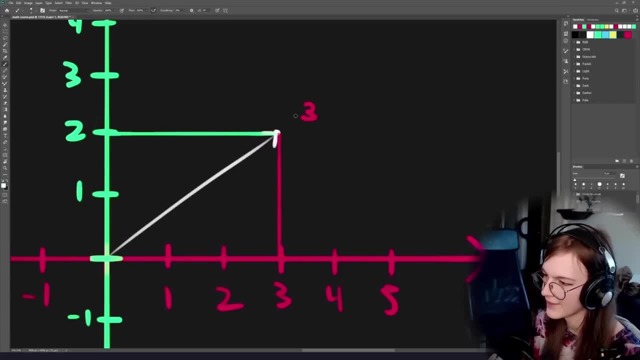 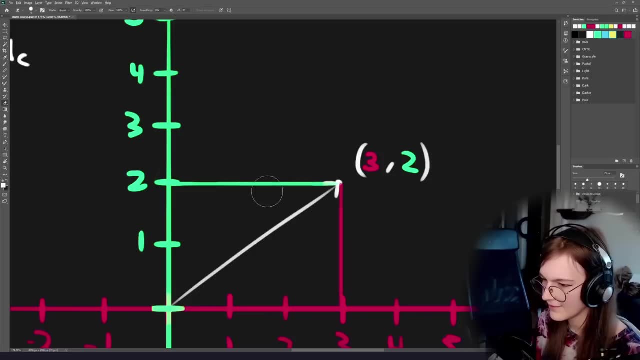 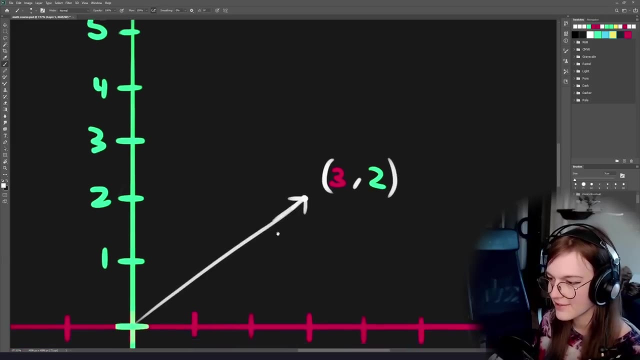 So this would be 3.. And the Y component is 2.. Cool, So now we have our vector. Also, didn't really want to draw all of this, All right. So now we have a two-dimensional vector, Again, two values: one for the X axis and one for the Y axis. 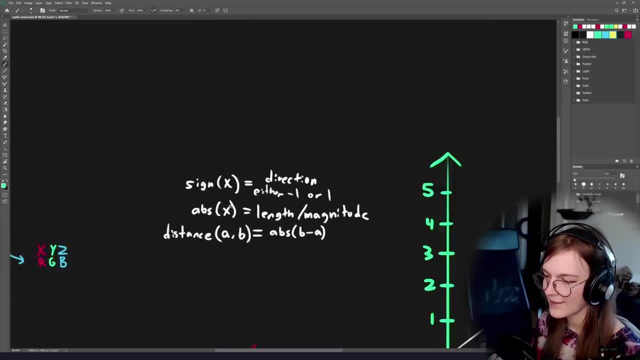 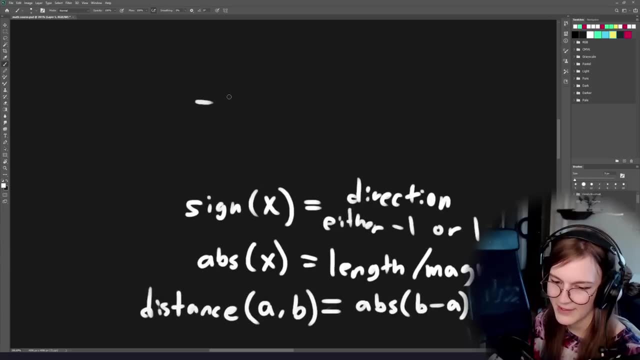 All right. So we talked about the sign of the value, right? So if we have a negative 5,, for instance, the sign of this is going to be a negative 1.. The sign of a value like 2 is going to be 1.. 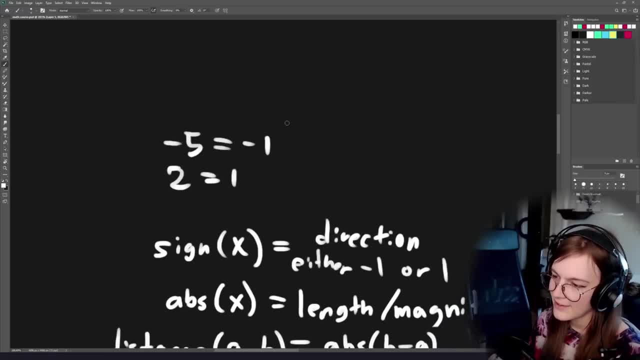 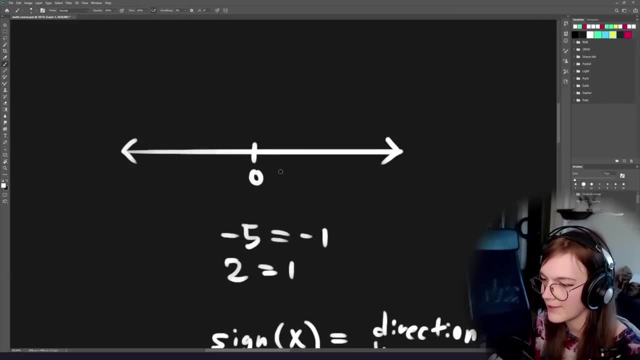 So basically, what this kind of represents is because again, we are on the number line right And we have zero somewhere. So what the sign kind of is is this: So what this means is that it can only be either 1 or negative 1.. 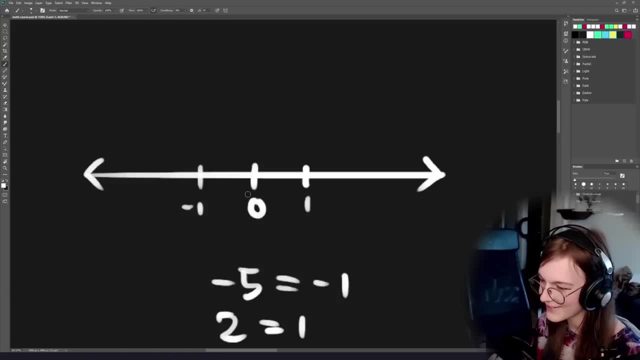 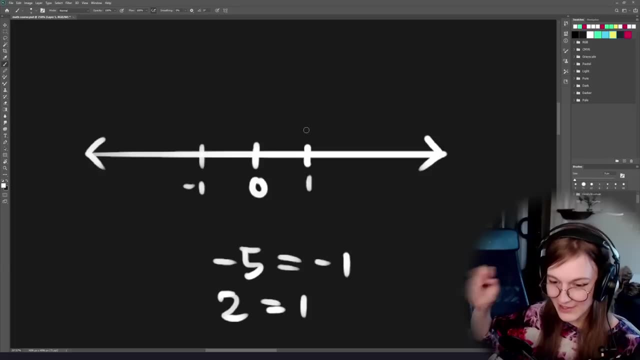 So I'm trying to think of if I should call these unit vectors one-dimensional unit vectors, which is a little bit of a cursed term. But if you talk about unit vectors, that means that you have a vector that has a length of 1.. 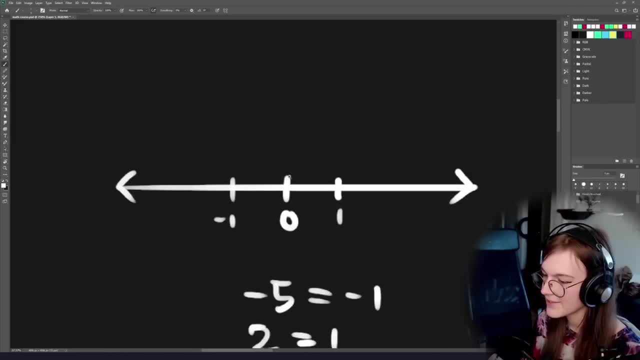 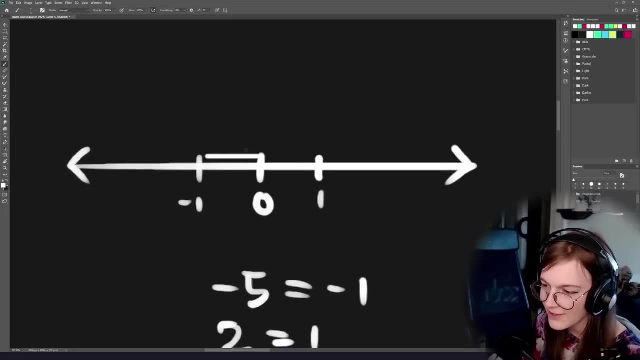 And both of these have a length of 1, right. So what this means is that the When we do the sign of something, we get the direction right. We get the direction for if it's going on the negative direction on the axis, or we get the direction pointing in the positive direction of this axis right. 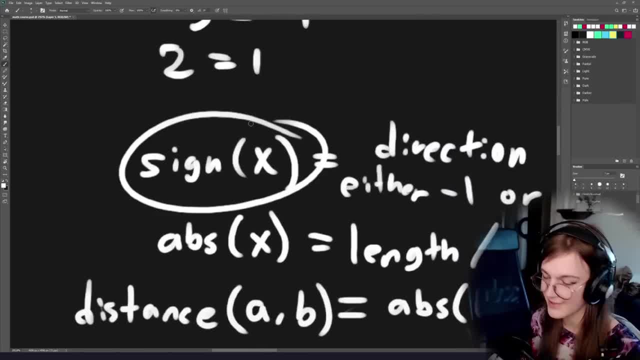 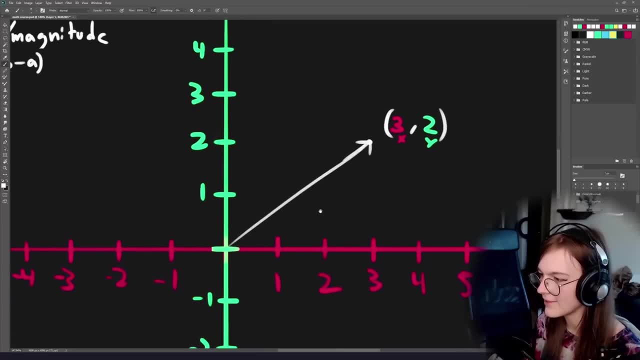 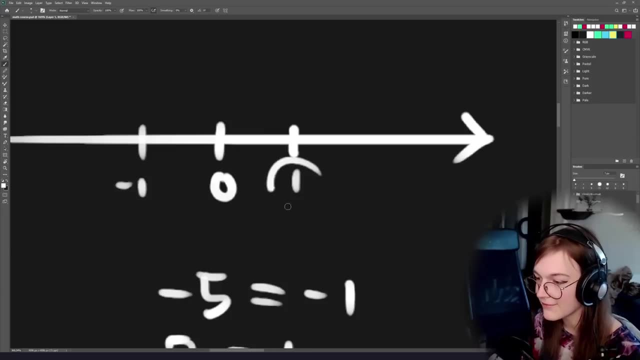 So what? the sign kind of What it really does is that it gives us a direction, usually direction vector. Okay, So what does that mean in this case? Well, we talked about- I mentioned- unit vectors. So a unit vector is a vector that has a length of 1, which both of these have right. 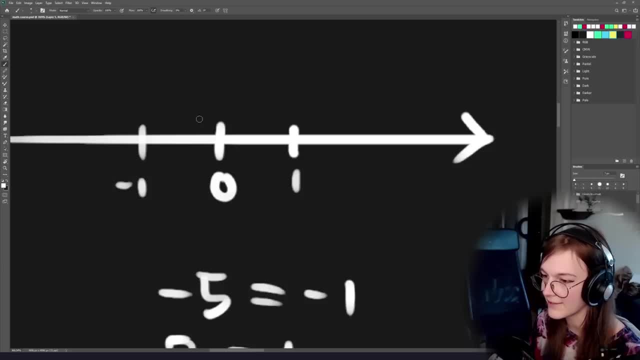 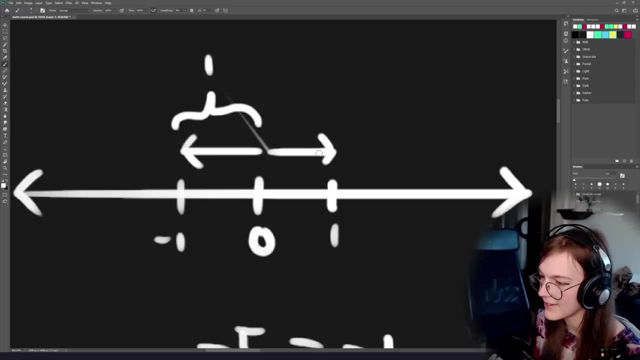 Even though they're one-dimensional vectors, they do both have a length of 1.. Because this distance right here is 1.. This distance right here is also 1, right. So one way of representing something that has the same distance is usually using circles. 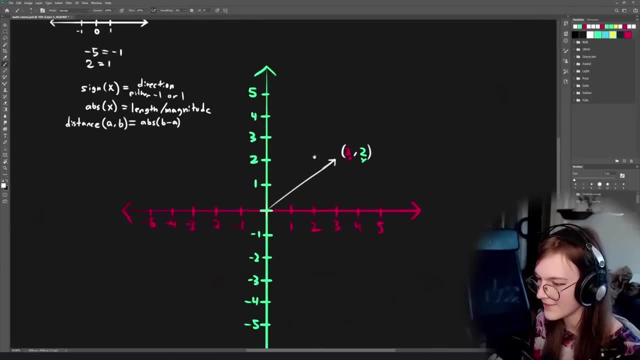 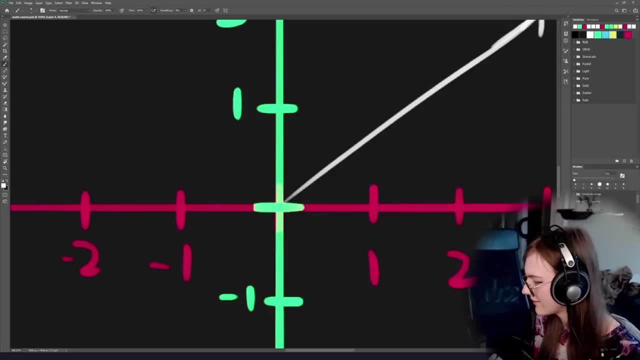 But in one dimension we can't really do circles, So let's go to two dimensions. So, now that we have two dimensions, basically, Oh God, I need to draw a circle. Drawing circles is hard. You know what? There are tools for this. 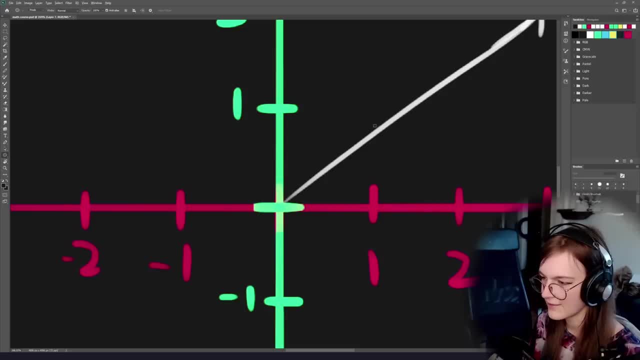 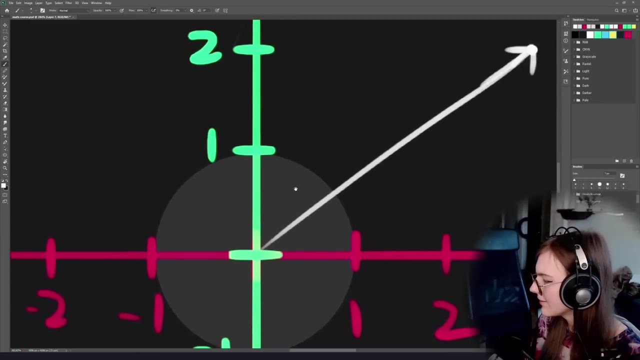 Let's do a, Let's cheat. There we go. What a beautiful circle, Okay. Is that visible on stream, or is it too faint? I think it's good, right, Okay, So all the, All the vectors that are pointing towards the boundary of the circle. 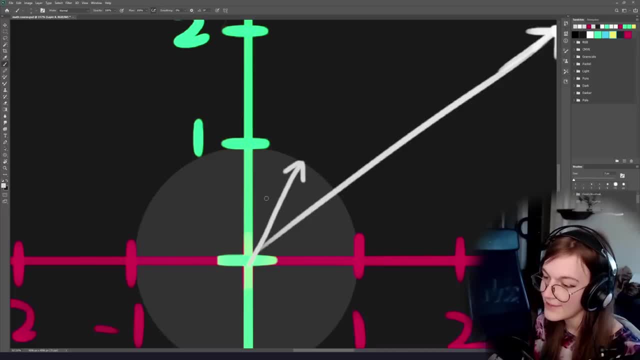 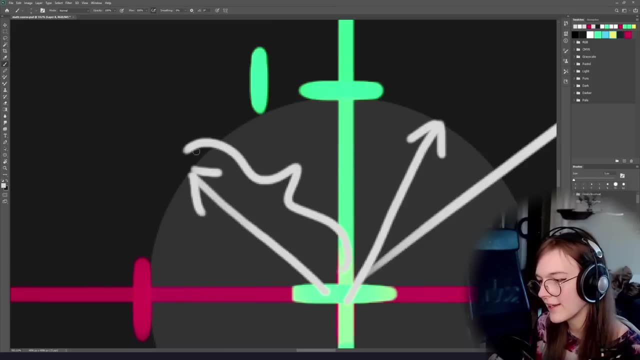 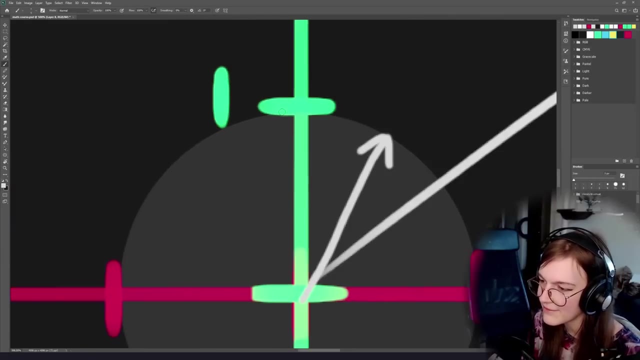 So if you have a vector pointing here, then this has a length of 1, right? This vector also has a length of 1.. If you just measure the length along this arrow, it's 1.. So what this means is that all the vectors that end up on the boundary of the circles are all unit vectors, right? 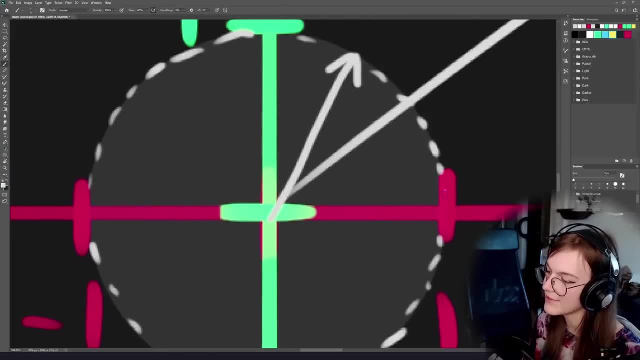 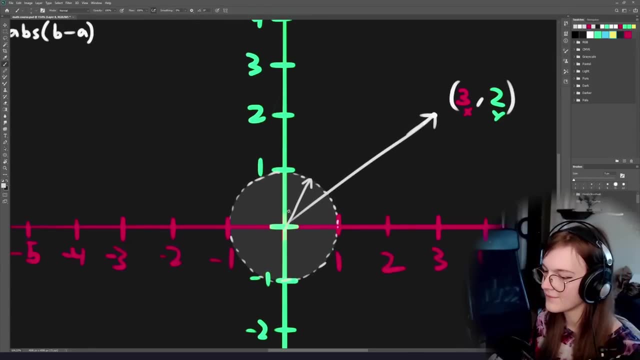 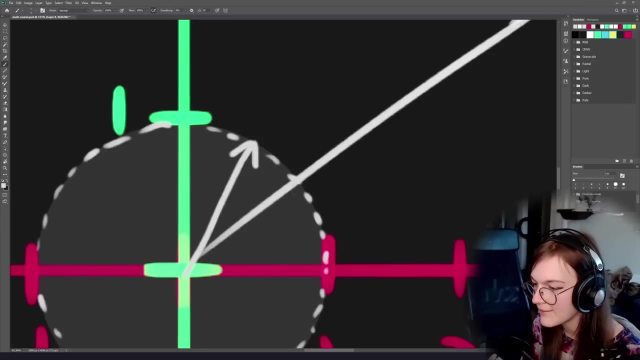 So when we talk about unit vectors, quite often they're referred to as directions. So directions are always unit vectors. So if we want to know the direction of this one, all we're doing is that we're kind of making it the length of 1.. 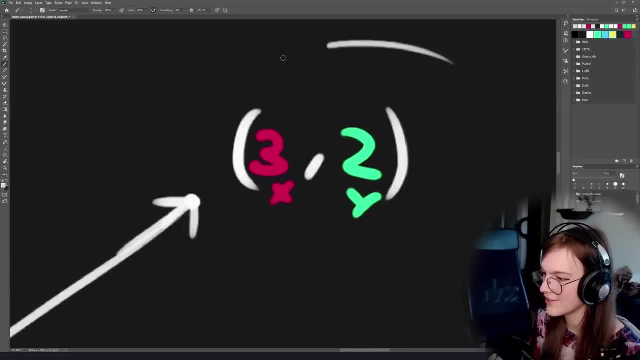 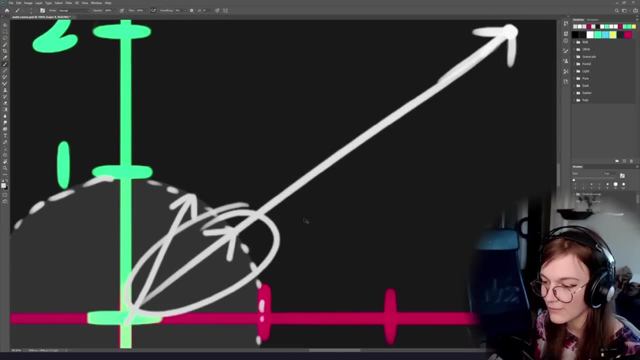 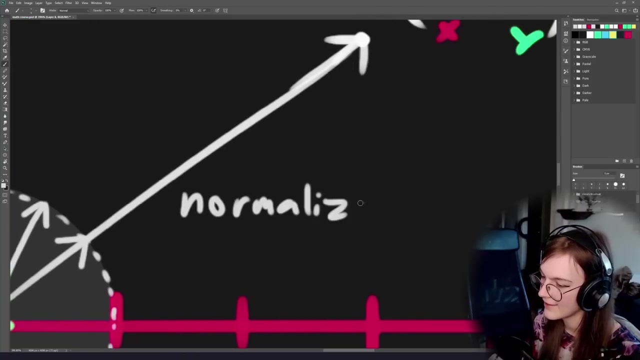 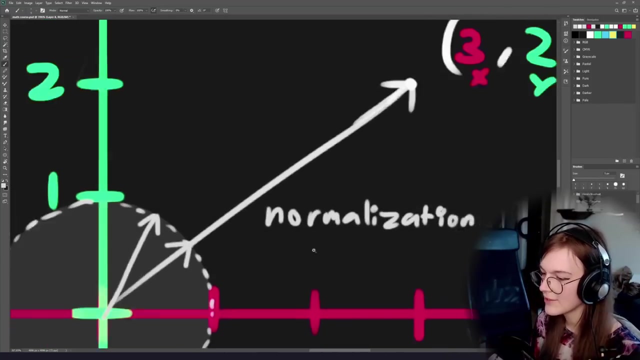 So this vector right, here is the direction of this vector right, And what this is called. The process of making a vector the length of 1 is called normalization. So Normalization. Eyes were inconsistent. There we go. So the process of making a vector normalized, or the length of 1 is normalization. 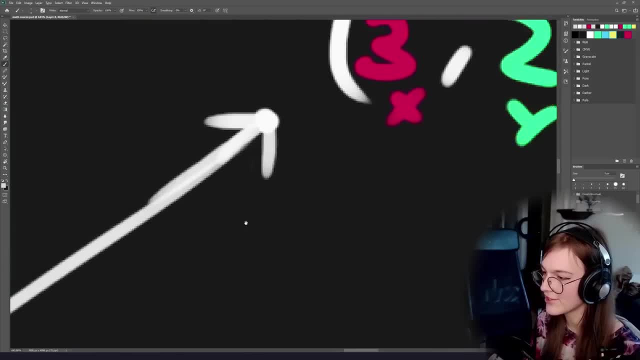 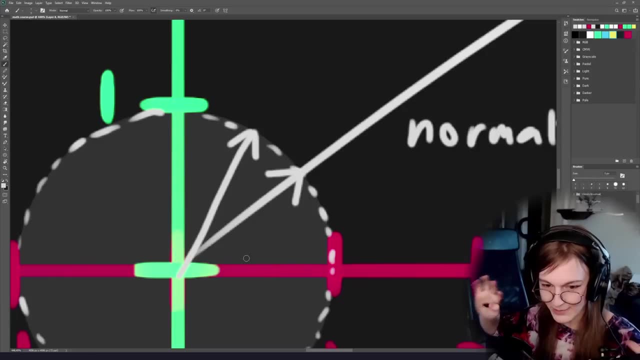 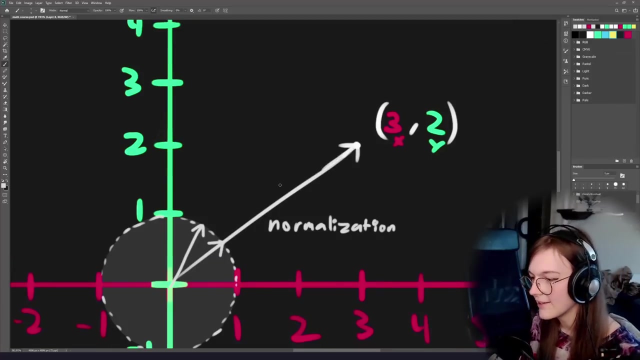 So this vector right here is the normalized version of this vector, And this concept is also very important, Like this is super, super useful in so many different ways. Yeah, This is like ubiquitous whenever you're dealing with vector math in terms of positions of objects, the relation to each other, the direction to some other object and so forth. right, 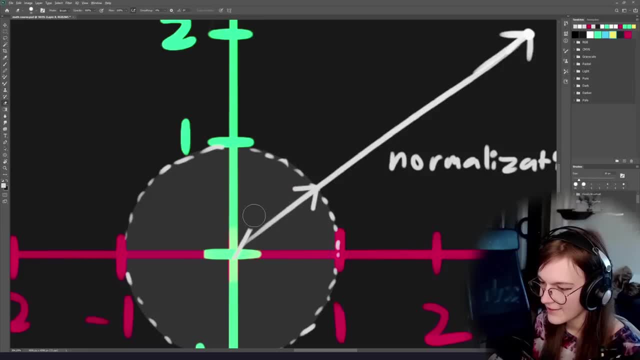 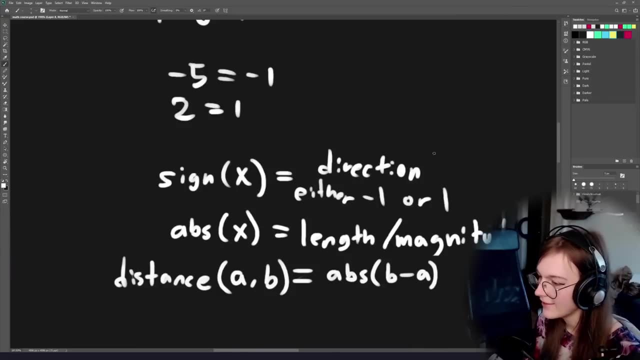 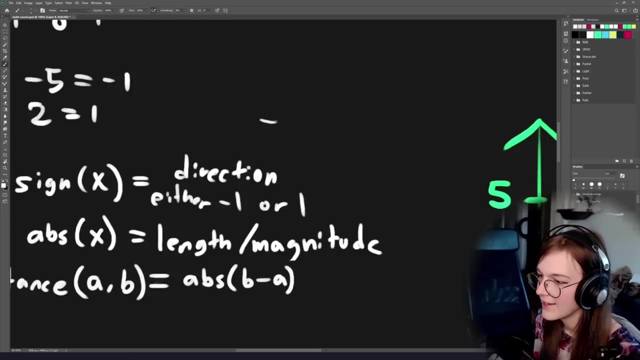 All right, So let's erase this confusing arrow. So this is a normalized vector, right? So that is the direction right. In one dimension, the vector could only have two states. right, It could either be negative 1 or it could be 1, right. 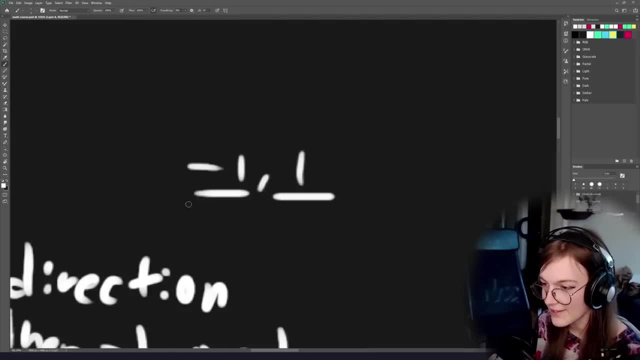 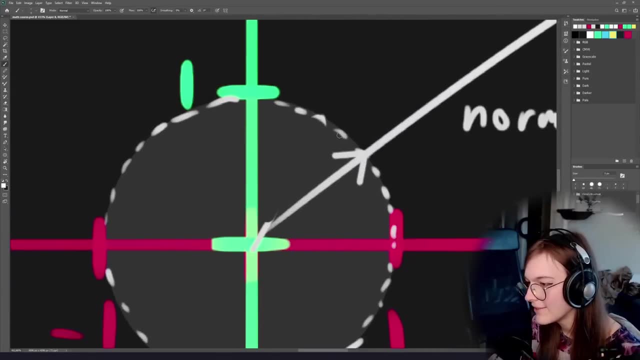 These are the only two states that are valid for a normalized one-dimensional vector right. But for a two-dimensional vector we have an infinite number of points right. This circle can fit so many points. It slaps the roof of the circle. 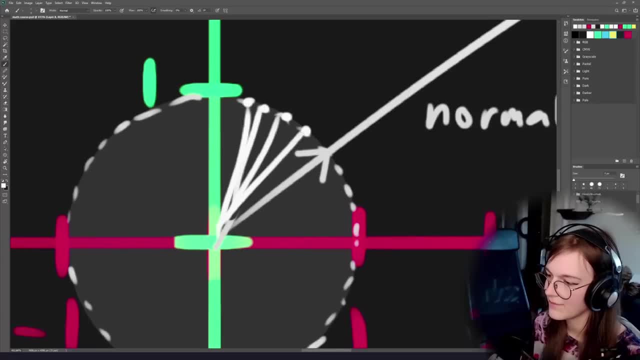 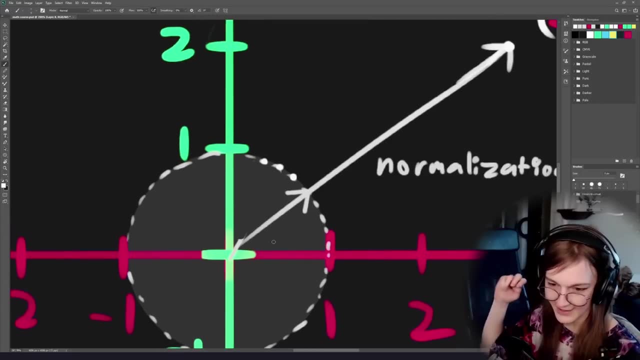 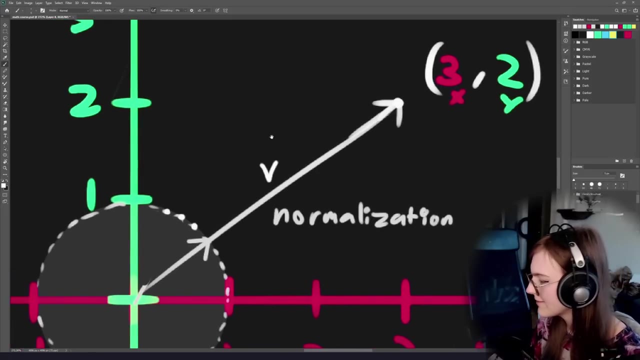 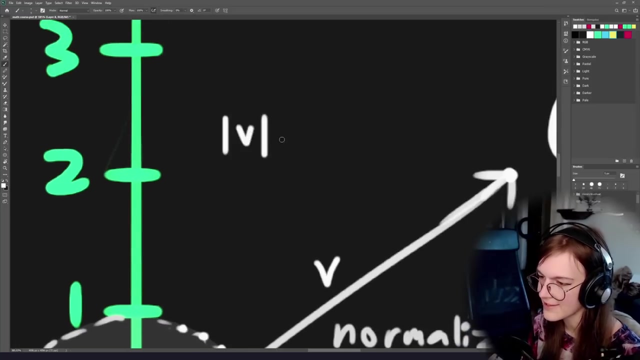 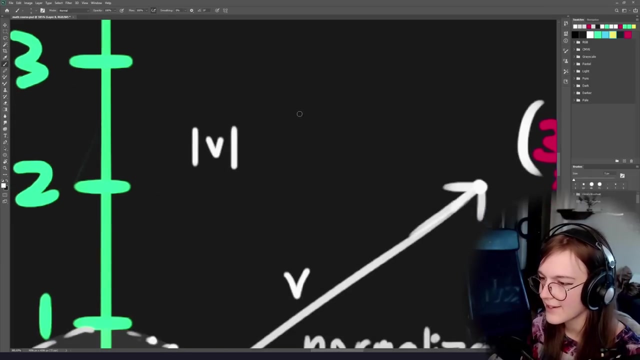 It's like a gamma, It's like an infinite number of points, It's like a cosine of a sine, It's like some sort of vector, I don't know. Well, actually this could be the length of it, sorry. 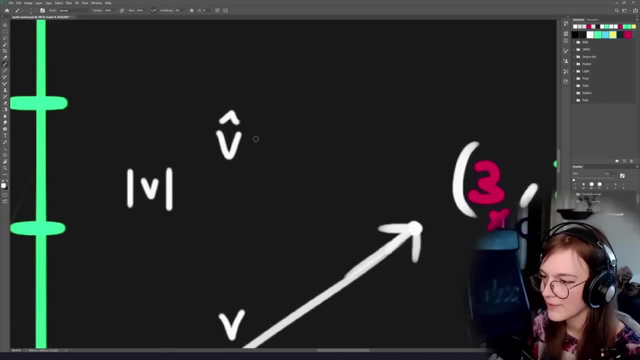 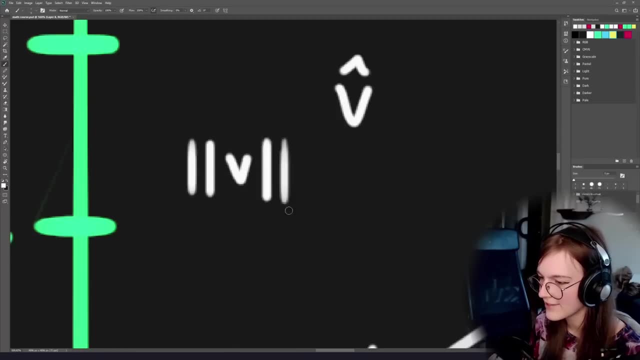 If you have v and then a little hat on top of it, this is a normalized vector. If you have bars on the side, that's usually the length of it. Sometimes you'll see two bars on the side, because nothing is consistent and everything. 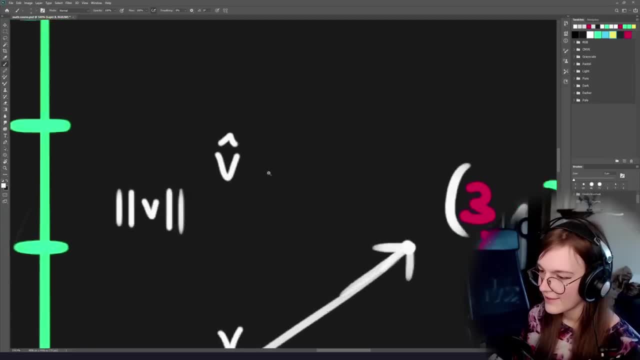 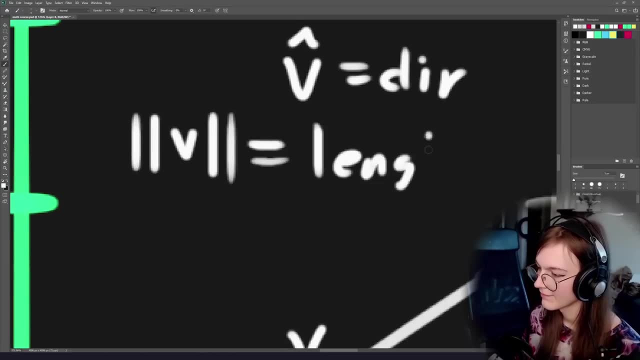 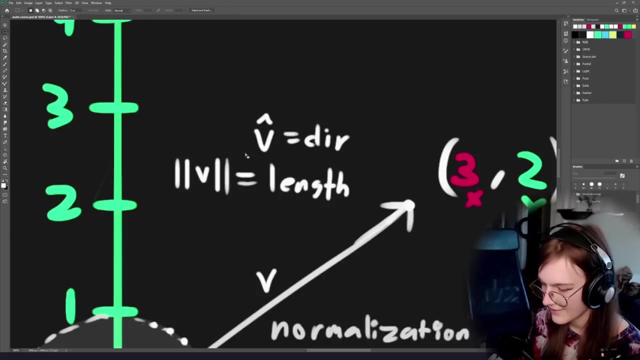 is garbage. But yeah, so usually this would be the direction And this would be the length Or magnitude- Same word. All right, so this is just the math notation garbage. I'm pretty sure this is correct. I feel like I have to relearn it every time I read a math paper. 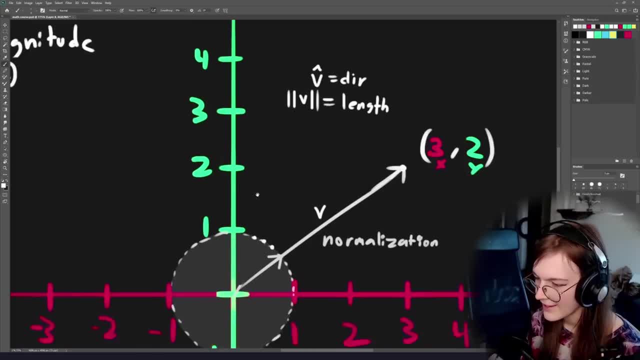 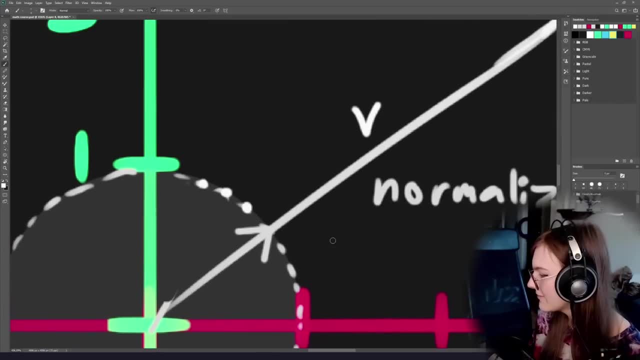 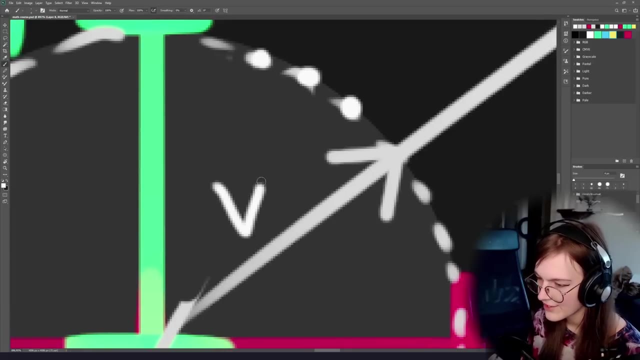 So we might wonder: how do you get a normalized vector right? How do you go from v to the normalized version of v or the direction of v? Kind of use those interchangeably right. So this little vector down here would be the normalized version of v, with a little hat. 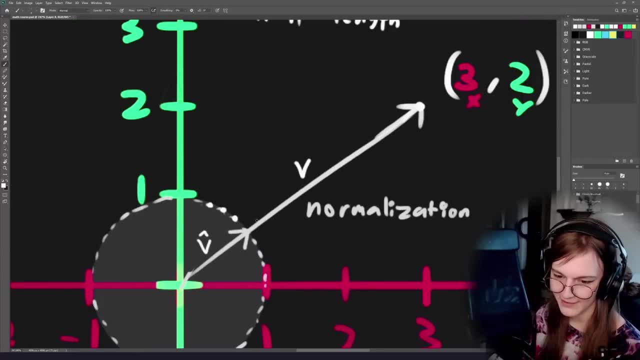 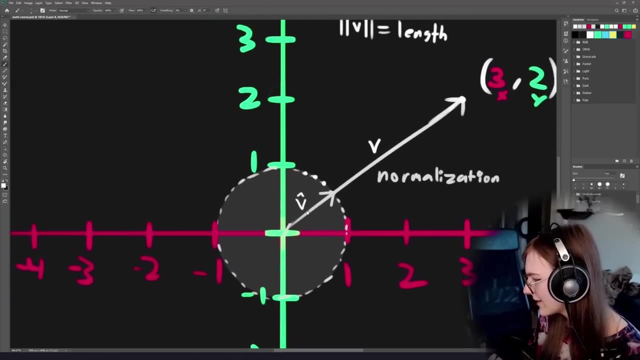 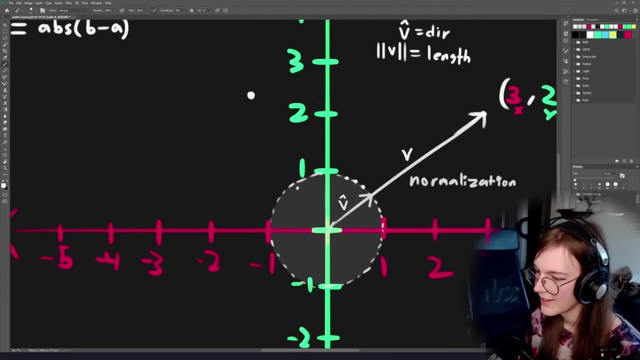 on top, But basically the direction of v. Okay, so we're going to talk about how to normalize a vector. So didn't quite get the normalization. So basically, if you have any vector pick up any point on over here, then that's going. 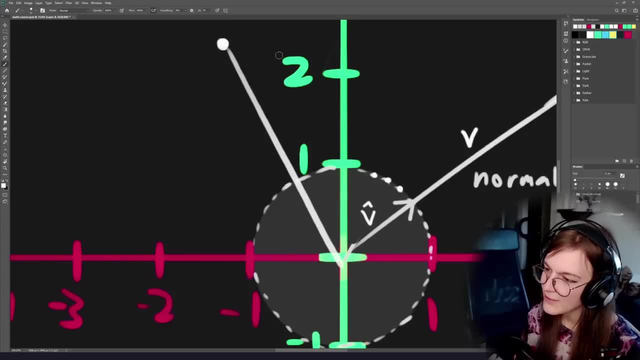 to be a line from 0, right. If you want to normalize this vector, what that means is that you make the length 1.. So what you get out of it is a vector pointing in the same direction. Okay, But it's got a length of 1, right. 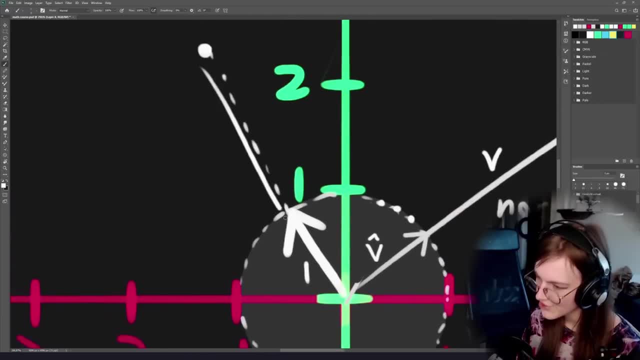 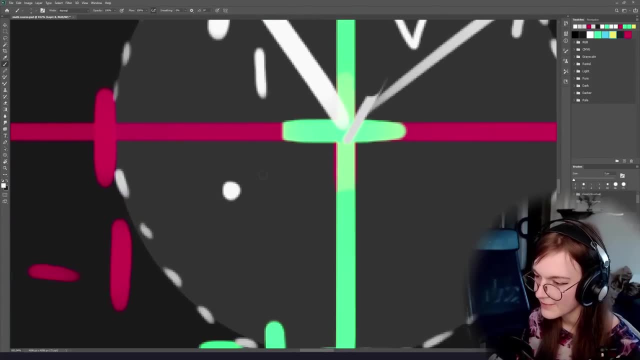 So it used to be this whole vector, But if you normalize it it's going to shrink down into a length of 1.. Or if you pick a vector that is a length that's smaller than 1, this vector is going to normalize. 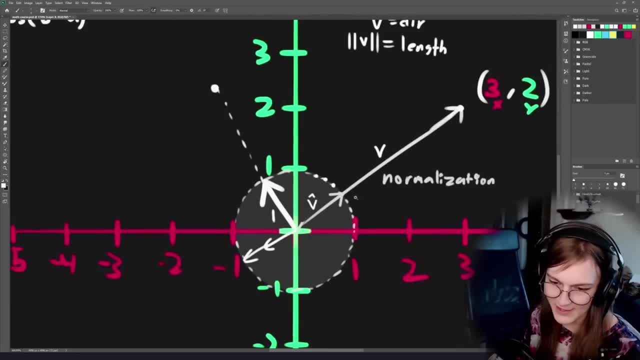 into being longer all the way out here. So basically you can sort of consider it to be a way from going from a point to an arrow that represents the direction to that point. Yeah, When do you usually need to normalize a vector? So the concept of a direction is really important. 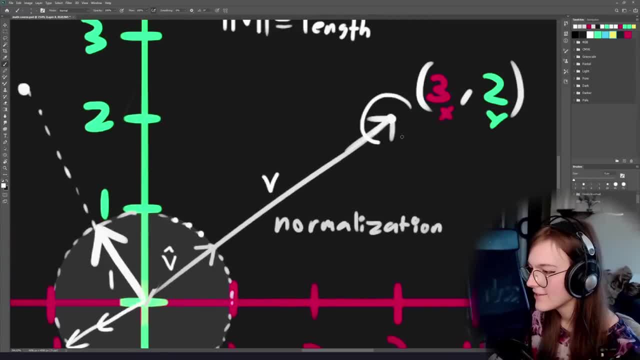 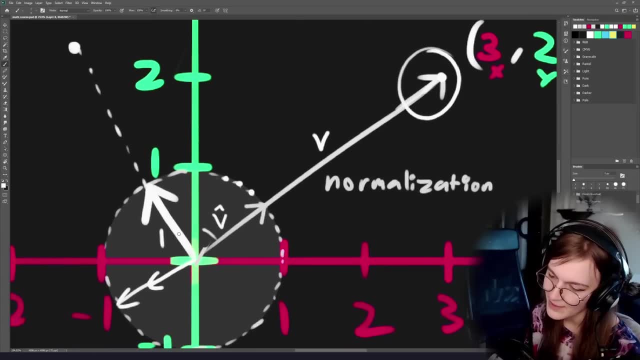 So say you have an object that is over here, Let's say maybe this is an enemy, like at this location. And then you want to know, let's say maybe the player is at 0. And you want to know what is the direction that you need to move in order to move towards. 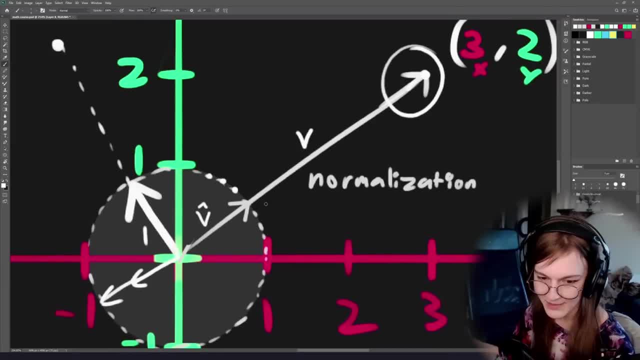 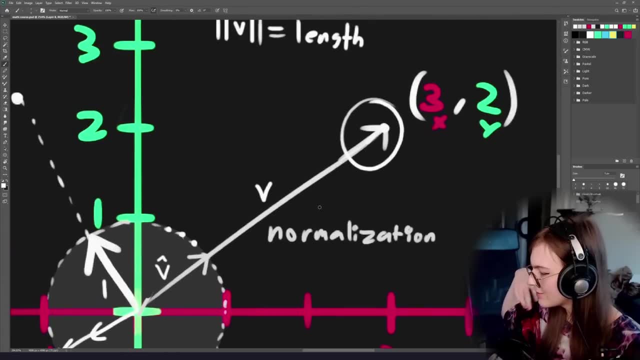 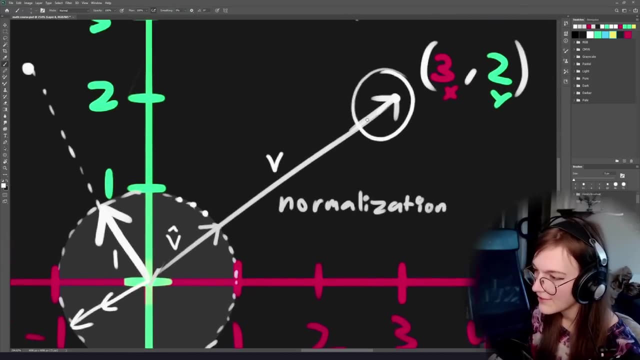 the enemy. So if you are dealing with like physics or something And you want to add the vector to move toward the enemy, Then usually you want to move at like a fixed rate in terms of speed, right. So what you usually do then is you normalize the vector between the player and the enemy. 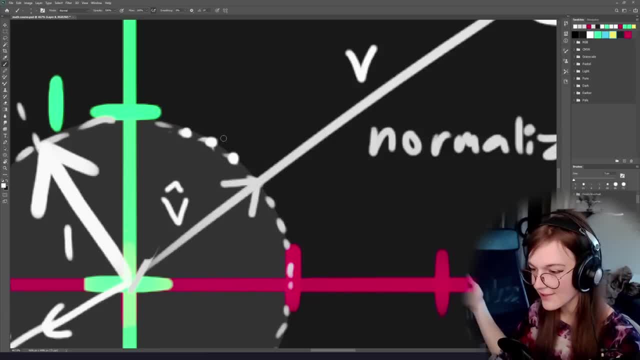 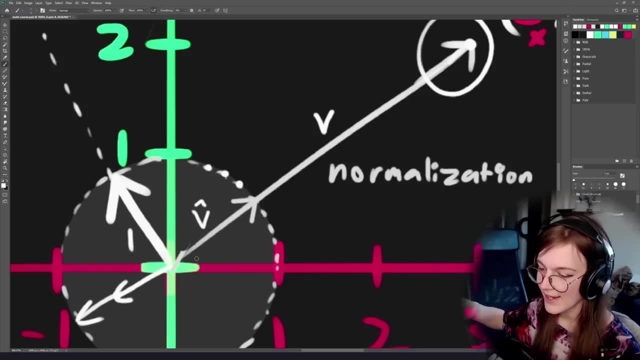 And then you have a normalized vector, which again that's a direction, usually in terms of terminology. And then, once you have a normalized vector, If you multiply that by your speed Or some value, that represents how much you want to move in that direction. 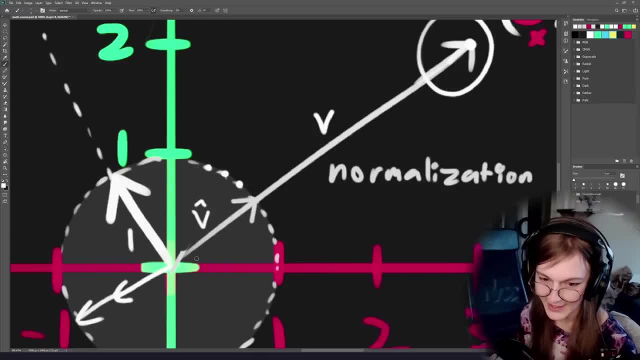 You can guarantee that that's going to be in, you know, meters per second, Or that that distance is going to be in meters, Because the length is 1, right. So that means that you get consistent movement in space. What's the difference between Yiddi's normalized method and normalized? 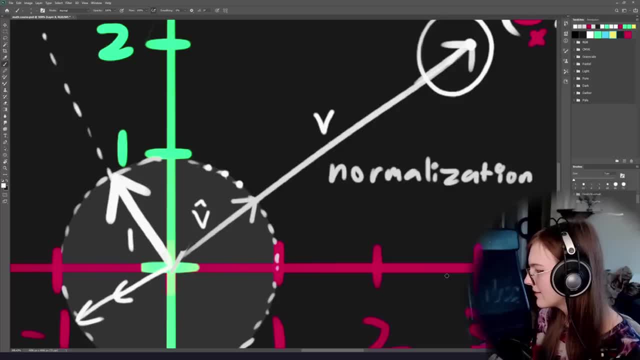 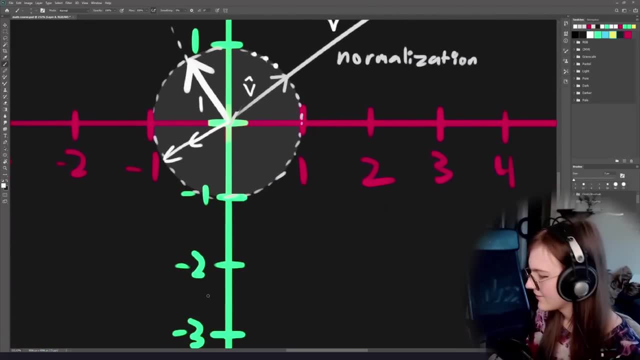 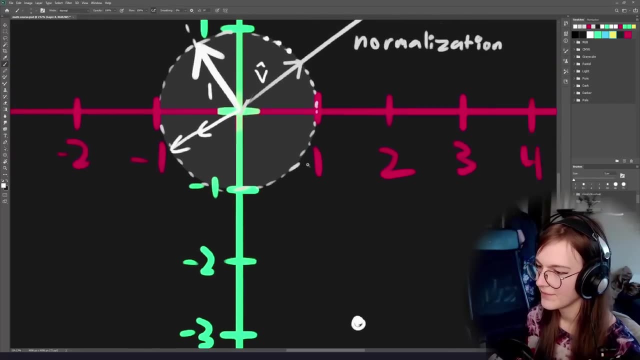 Yeah, the normalize will modify the original one, Whereas the other one returns a vector. Okay, Does that make sense? So, basically, pick any point. Normalizing it means you get the direction to that point, And a direction in this case I'm using the word direction to be interchangeable with. 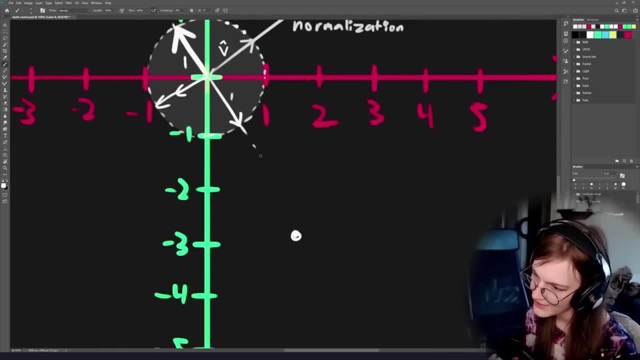 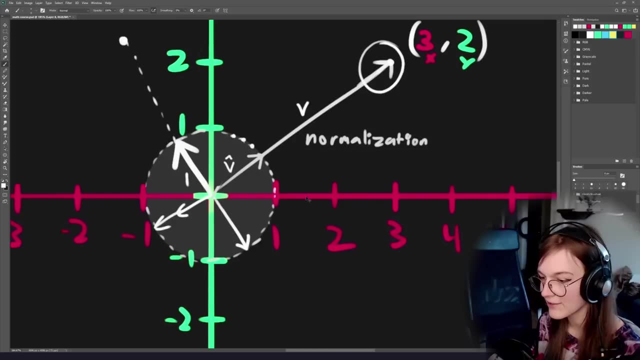 a vector with a length of 1, right, But it's still pointing towards that point, right? Like I mentioned before, one of the powers, the powerful things about having normalized vectors, is that. Let's see if I can undo a bunch of things. 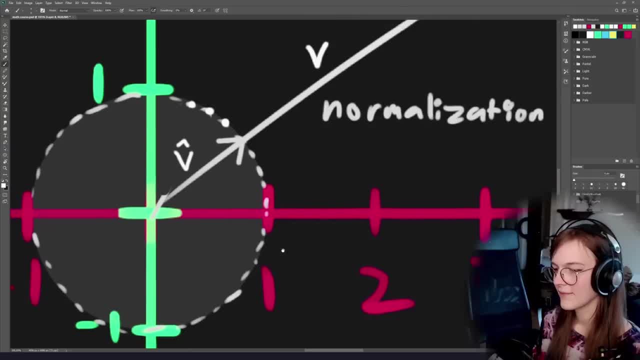 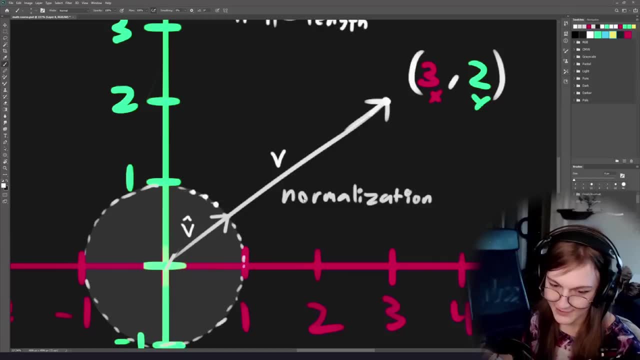 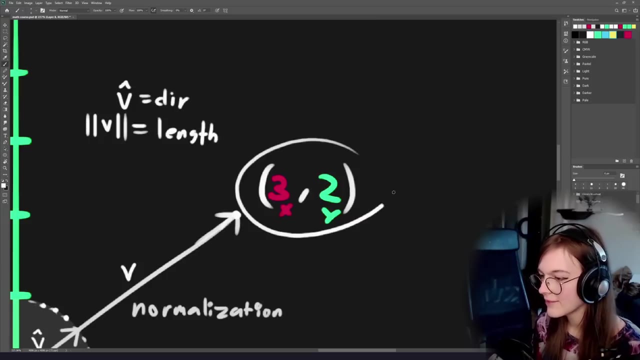 Okay, Okay. So if you have a direction like this, you can multiply a vector with a scalar, As in a single value, So if you have a vector again, usually when people say vector they mean multiple components rather than one. 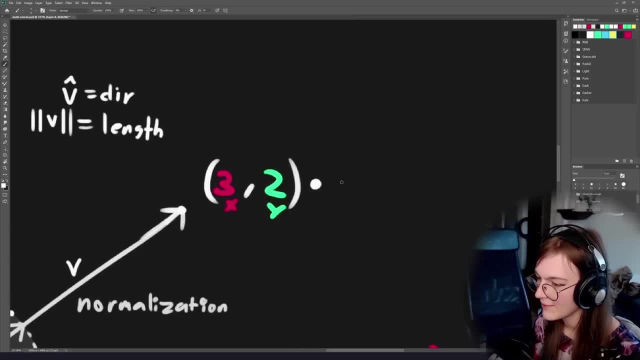 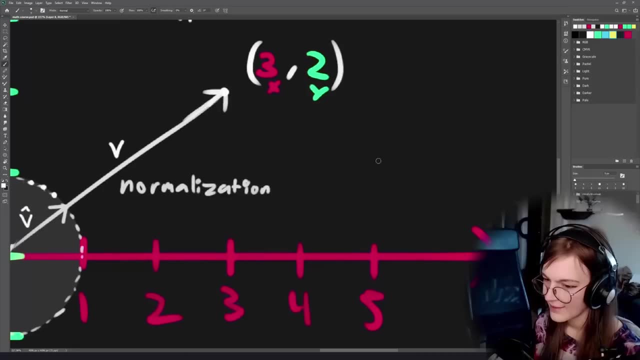 But if you have a two-dimensional vector, you can multiply that by 2,, for instance, Or like some number. But if you have the normalized vector, So let's say 1.. So let's say we have our vector, that's normalized. 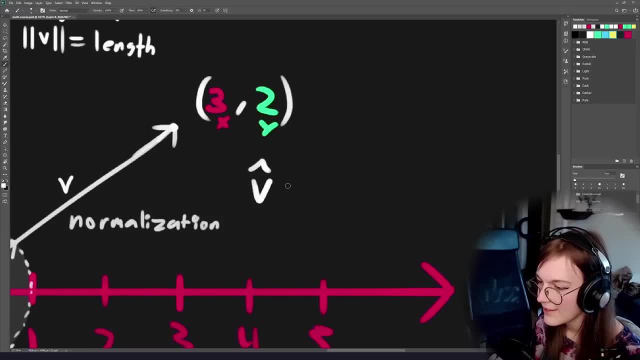 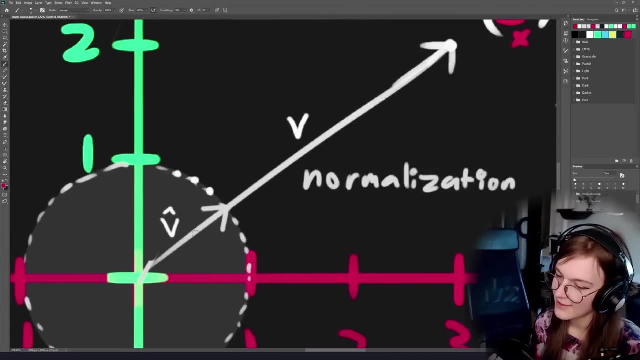 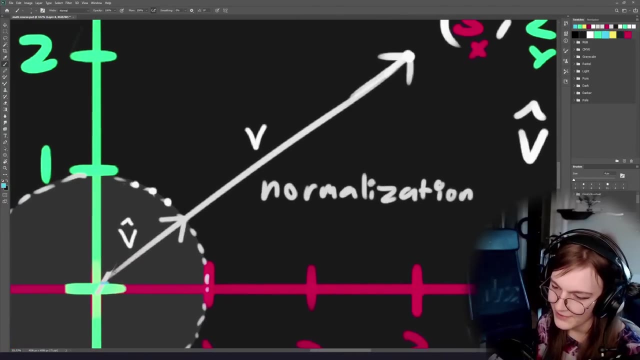 It's the same thing as this one, And then we multiply that by a value of 2.. Let's pick 2.. What that means is that the new vector we are getting out of this, that is going to be the direction along V, right here. 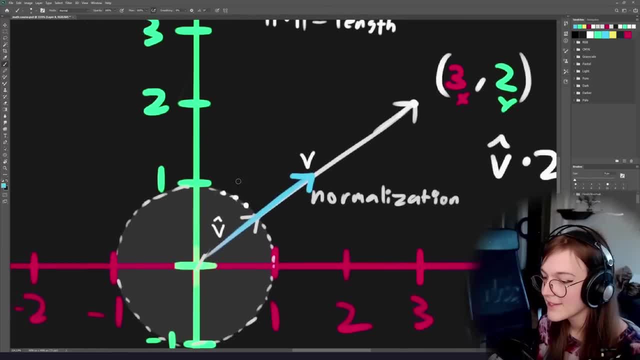 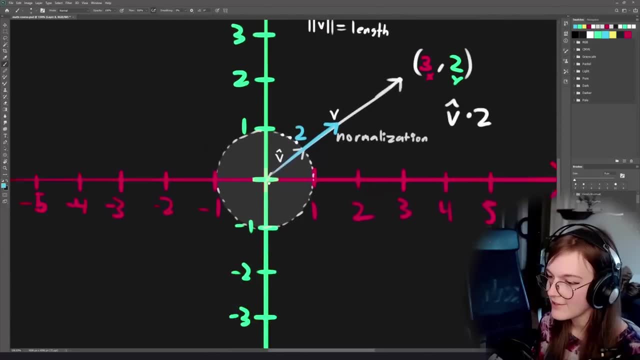 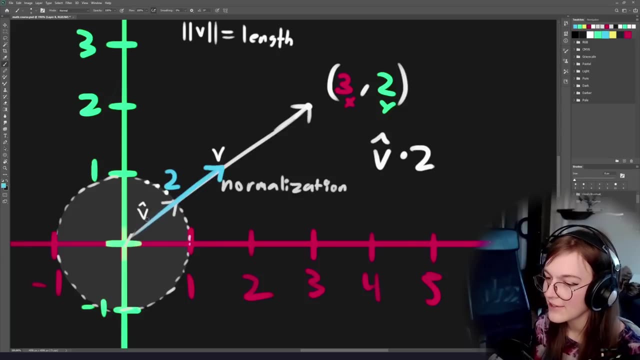 But the length of it is going to be 2.. So this is kind of what is Like extremely useful about normalized vectors, Because if you want to move like two units towards something, then having a normalized vector means that you can get a position that's exactly like some number away from some point. 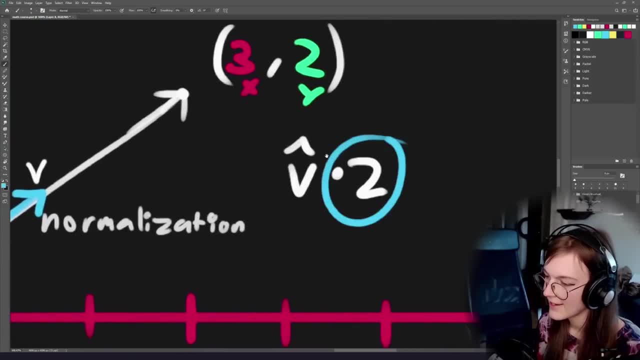 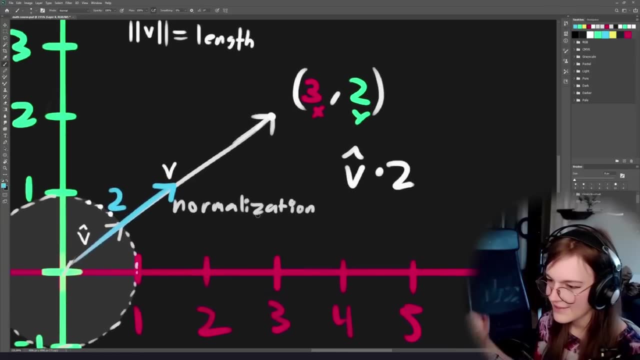 So if you normalize a vector, multiply it by a distance, then you're going to make the length of that vector the value you're multiplying it with, And it might seem like that's That's not. That's kind of trivial, But that's not the case with this vector. 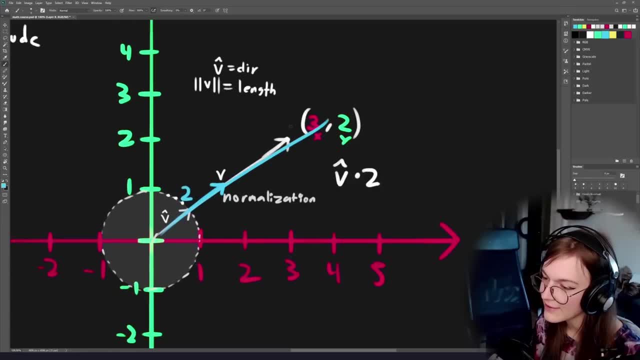 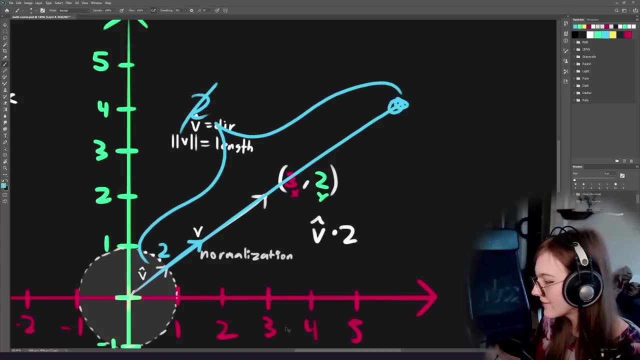 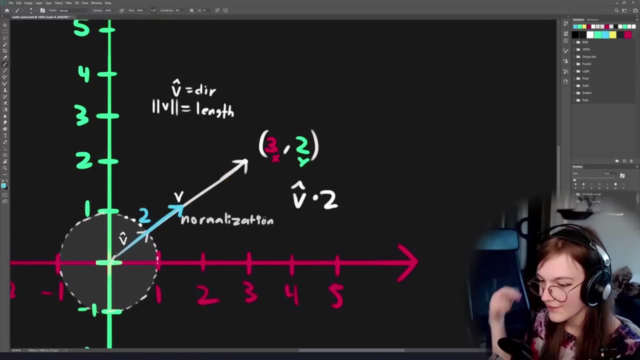 If you multiply this by 2, then the length of it is going to be all the way over here. So the length of this is definitely not 2.. It's way longer. So this is why normalized vectors are extremely useful. Because of the fact that the length is 1,. if we multiply it by some scalar, the length 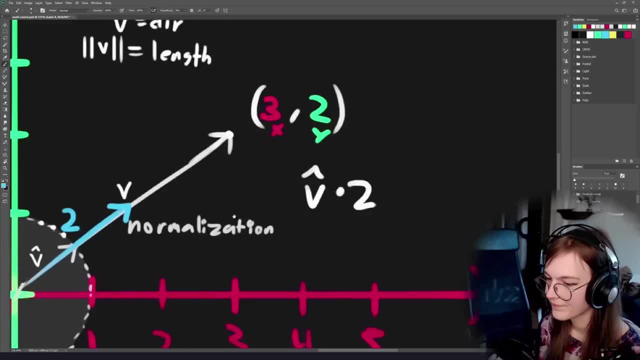 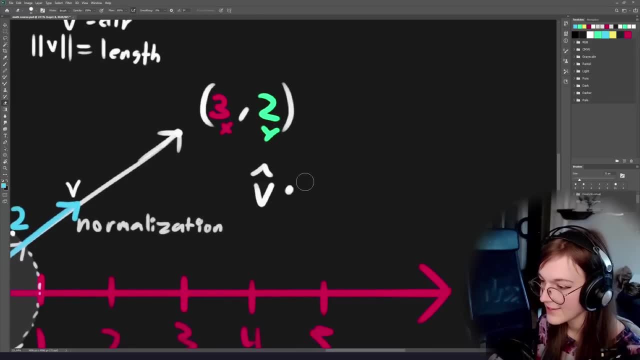 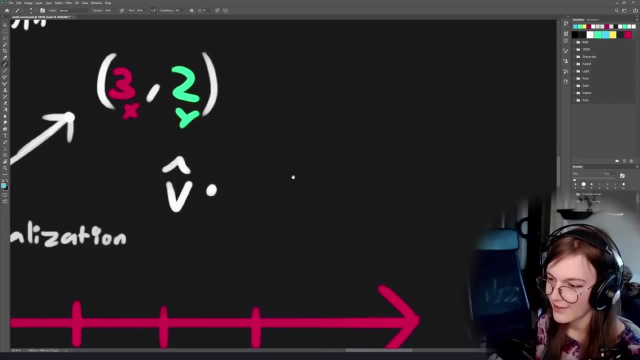 is going to be that scalar Right. So that's something that's useful when it comes to this. So, like I mentioned before, it's useful in physics, for instance. So if you have the normalized vector, then if you want to move something along this vector, 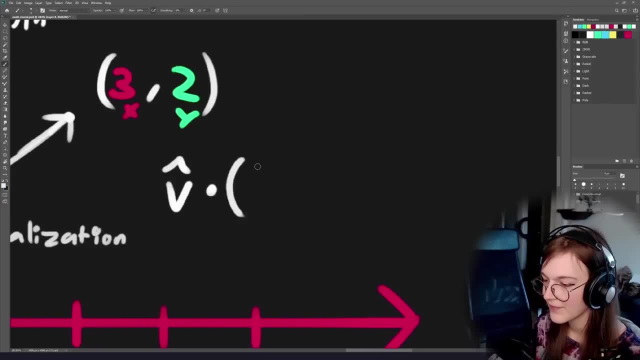 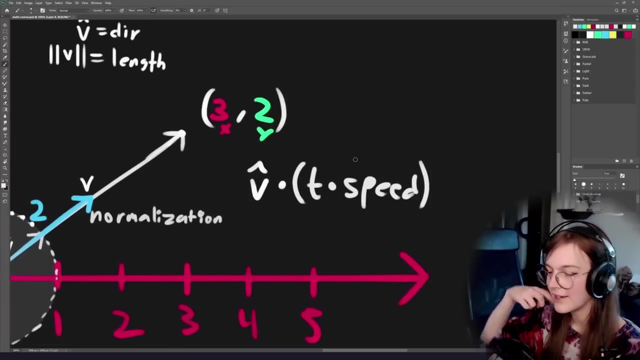 then well, what you can do then is that you could have time multiplied by your speed, for instance. So time multiplied by speed, So now we're just multiplying all of these together. So what that means is that, if time is a value that is ticking in seconds when you start, 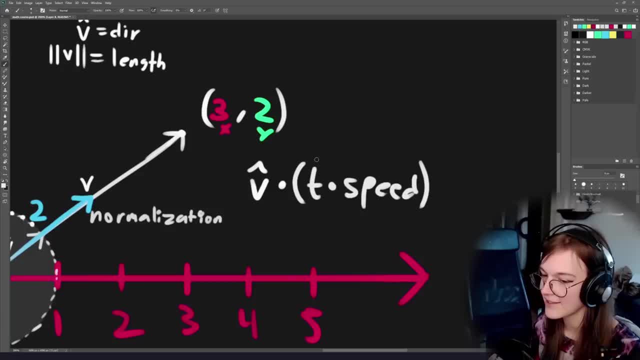 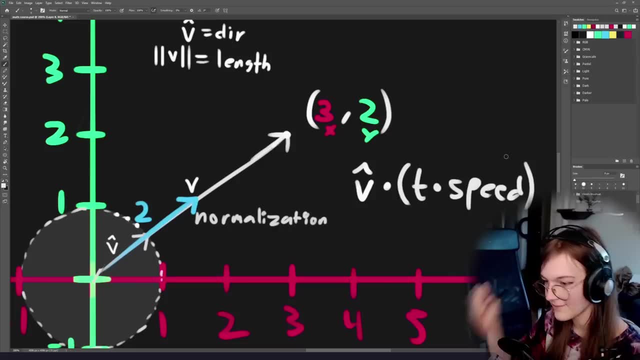 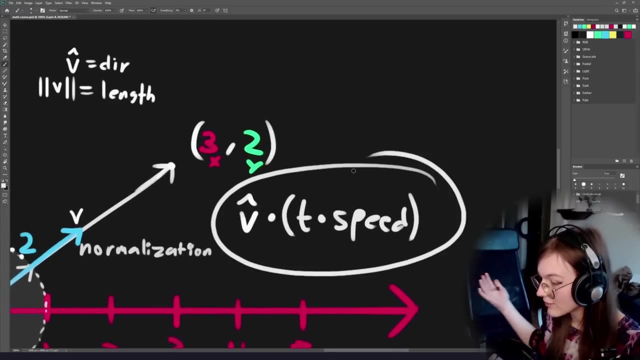 the game time goes from 0 to whatever the current. second is then you're going to have an object that moves along this vector at the speed you give. here We're going to go into more physics stuff later, So this is just one of the really really powerful things about having normalized vectors. 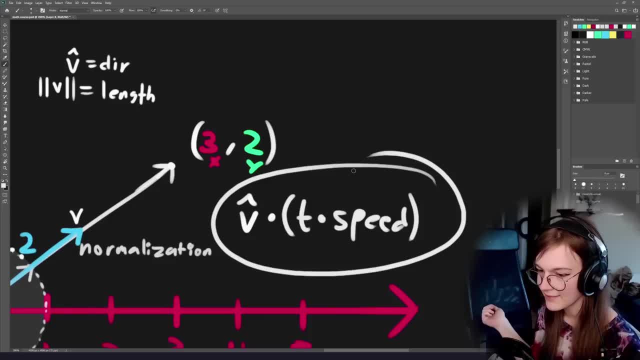 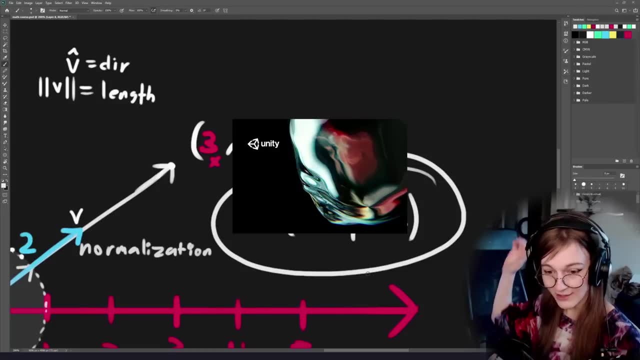 Right. Can you show an example in Unity? Yeah, sure. Do people want to see examples of this? Show examples of this, Yeah. Is this in Unreal? Nope, I think showing it in practice is really really good, because you're going to work in. 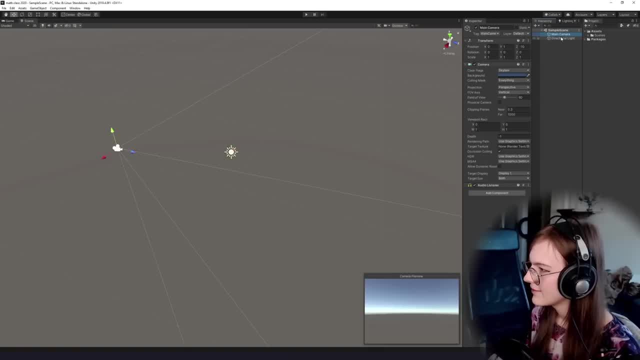 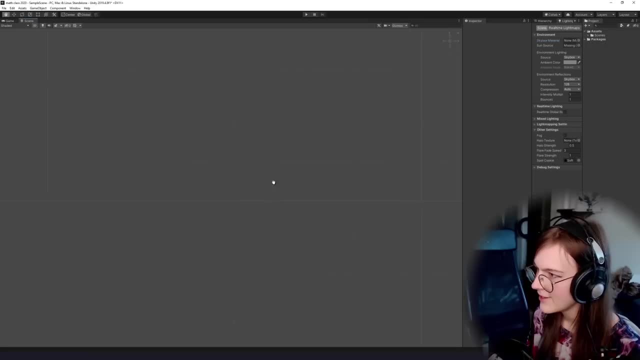 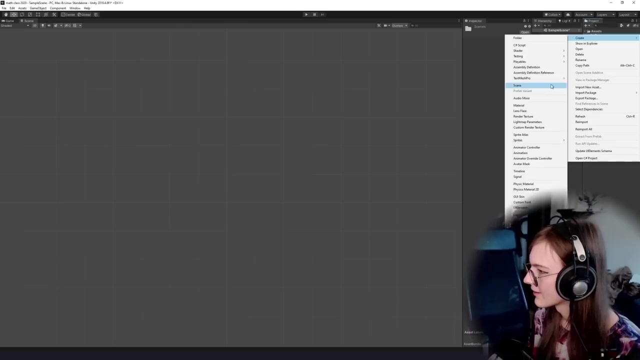 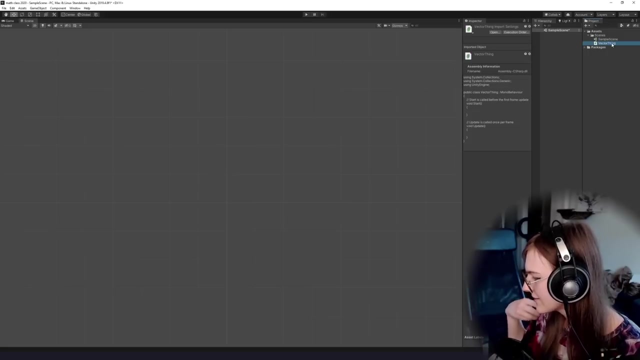 Unity. So why not? All right, Let's nuke some objects. There we go. Let's go 2D, because we're not into 3D yet. That's good. It's great. Will the game crash if it runs for more seconds than the float 32-bit line? You're going to have to run the game a very long time. It's not going to crash. It's just that your equations are going to get a hitch and a weird thing that's going to happen once it goes over the limit. I don't think it's going to crash. 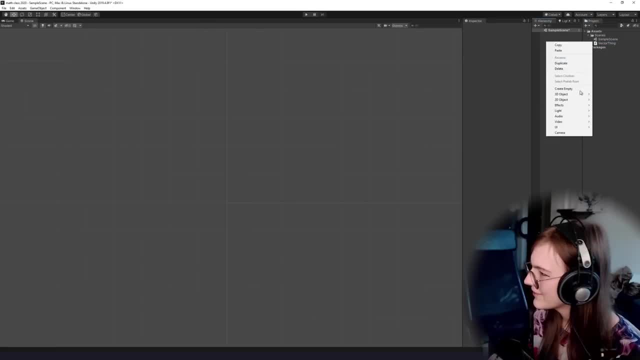 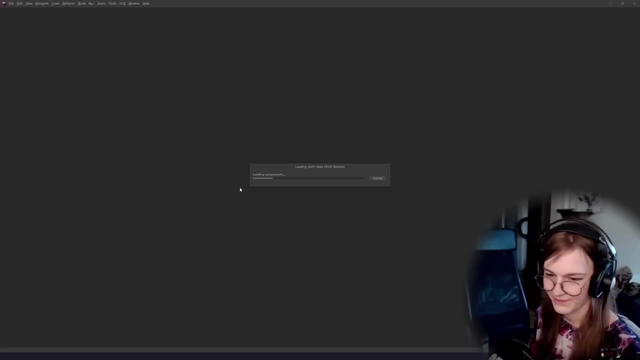 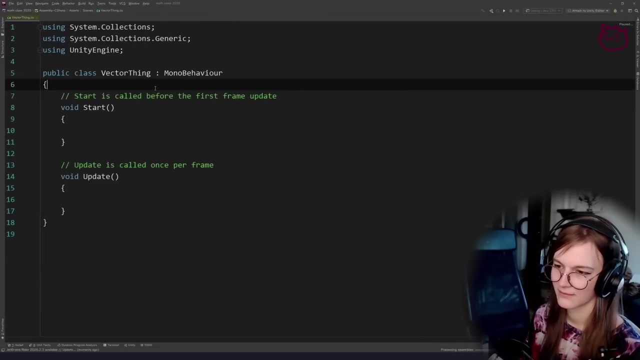 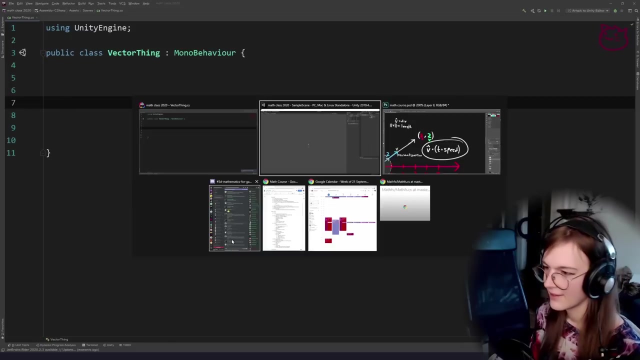 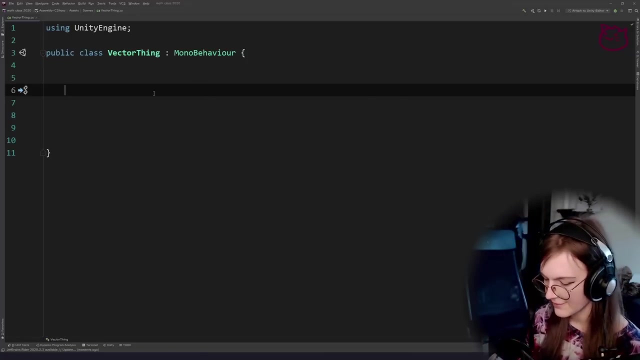 You're just going to have very weird behavior as soon as you hit that point. Okay, Let's see, I probably should have done code examples earlier, actually, because again, I like keeping things very pragmatic and practical. Okay, Let's just do some of the things we've done here just to show how it works, right? 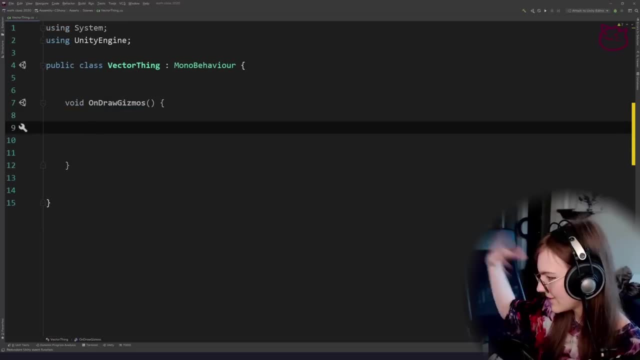 So I usually really like using onDrawGizmos because you can see it in the editor. You can very easily draw lines and whatnot. Okay, So onDrawGizmos is a special function in Unity that is called in the editor and you could 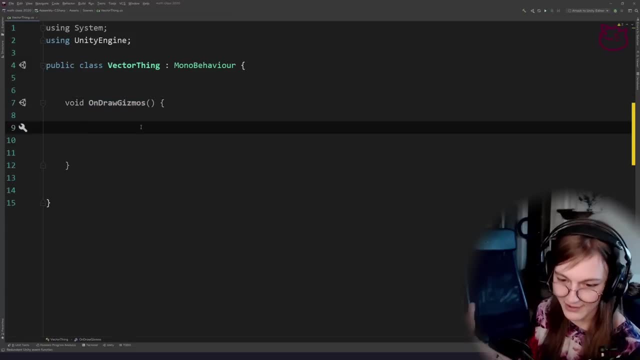 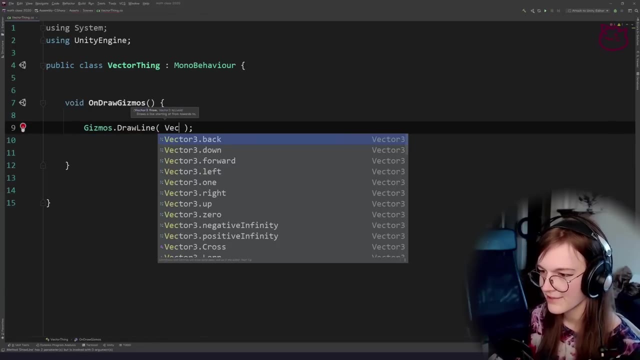 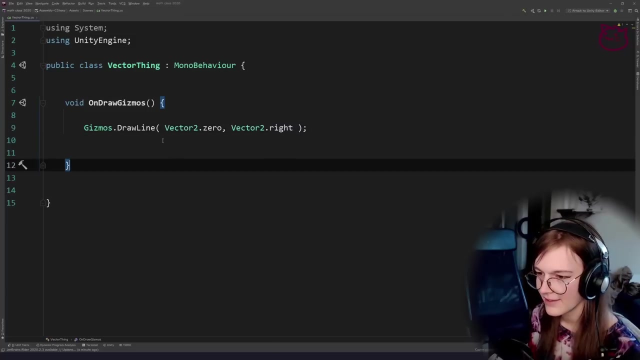 optionally enable it in the game view as well, where you can draw lines and whatever. So you can do stuff like gizmosdrawLine and then you can supply some positions, right. So we do something like that and we go back to Unity. 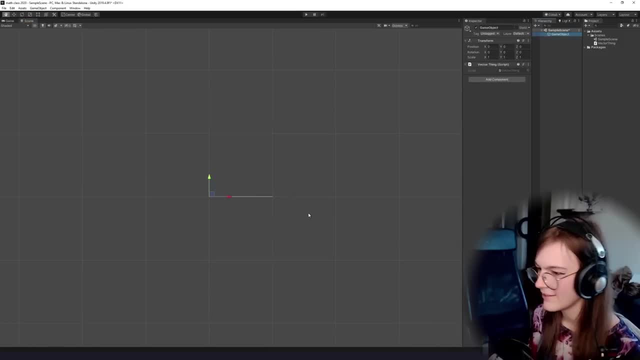 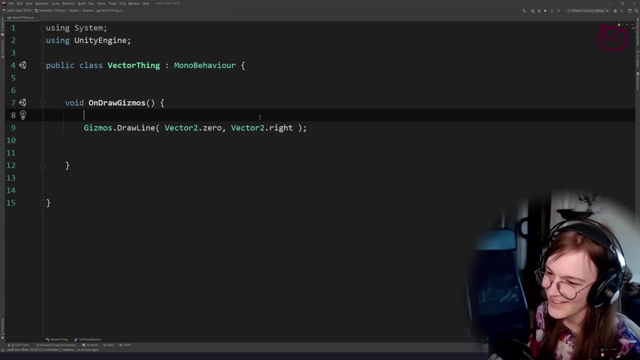 We now draw a beautiful, tiny little white line, Right, Cool, Oh wow, I wonder if there's a vector graphics package you can get. Okay, So All right. So drawLine, just a very simple one, But we probably want to be able to supply some other points. 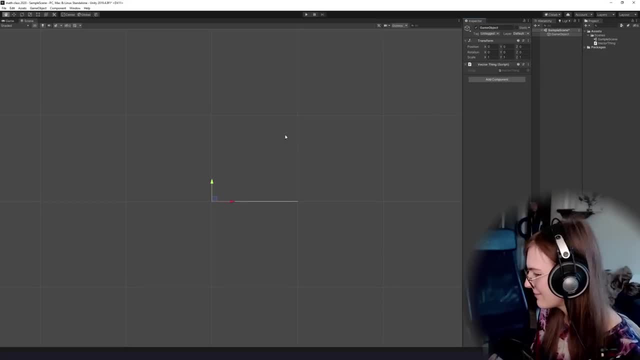 Do I have to wrap onDrawGizmos in? if Unity editor, I'm pretty sure that's going to get stripped for the rest of the game. I don't know that's going to get stripped for our builds, But I could be wrong. 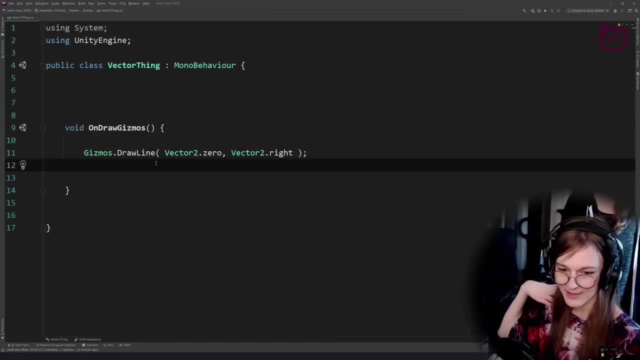 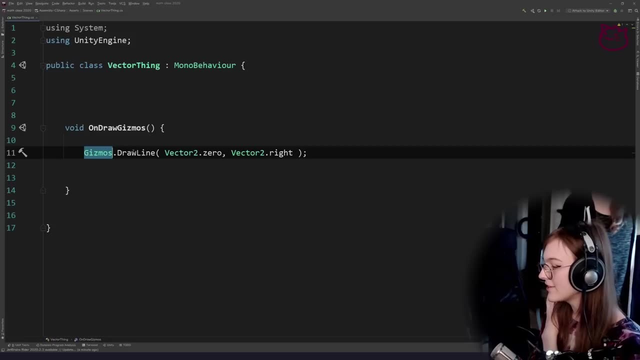 Sometimes you use methods in there that are only in the editor- namespaces and whatnot, but like if you use handles, for instance, But Gizmos, it kind of ignores that. I'm pretty sure, Yeah, I'm pretty sure, you don't need to strip it. 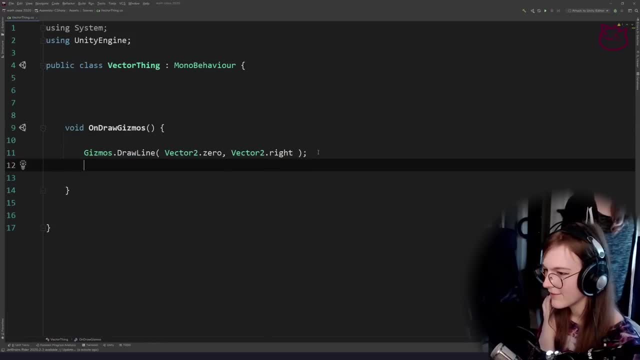 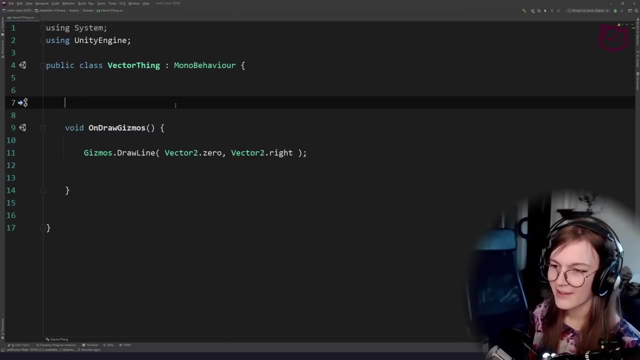 It's not going to like. maybe the code in here will be part of the assembly, I'm not sure, But at the very least it's not going to get called regardless. Yeah, Bye, love, Bye. Okay, all right. 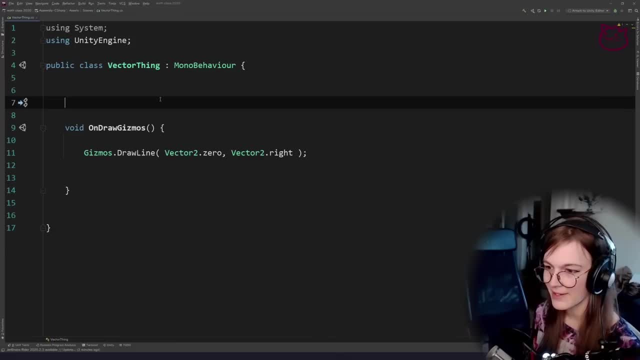 So we probably want to be able to pass a vector into this or a point or whatever, right? So instead of just hard coding it here, we can add a property, Or in my case, I'm just going to pass in a transform because it's easier to move it around. 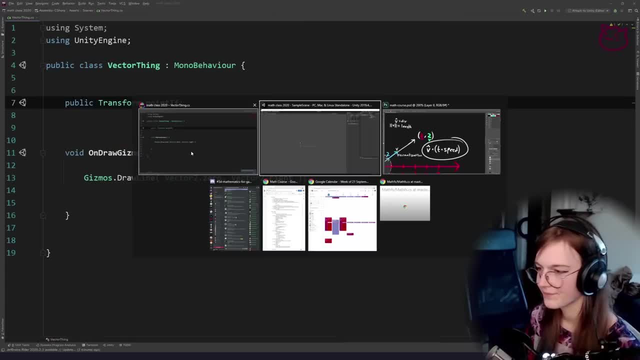 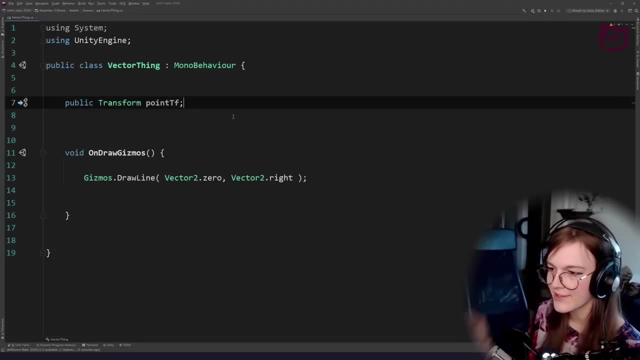 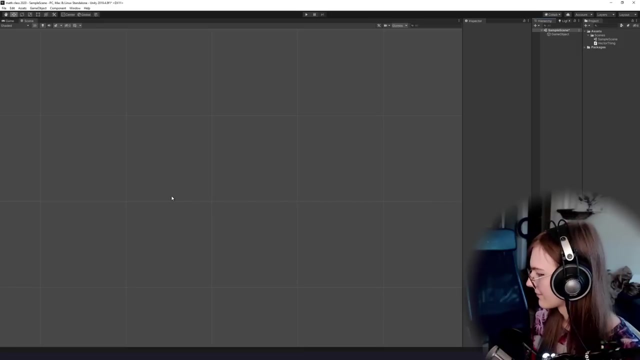 Let's call it points transform. Let's make a new game object. Actually, since we're drawing all of this in world space, we can just use this transform, All right. so now we're drawing a line between zero and this transform, right. 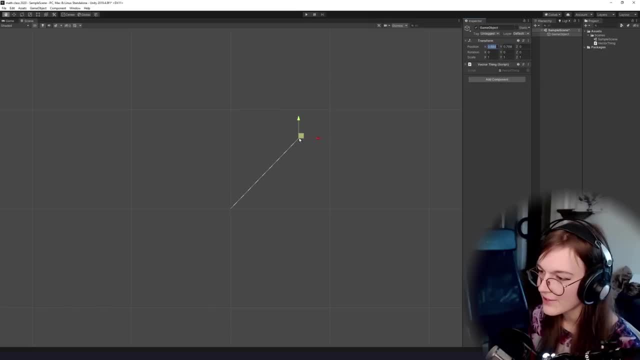 So now we're basically just taking the position of this transform and we're drawing a line to it, right? So again, we can think of this as the two number lines, right Yeah, The two number lines we had, where this is the origin. 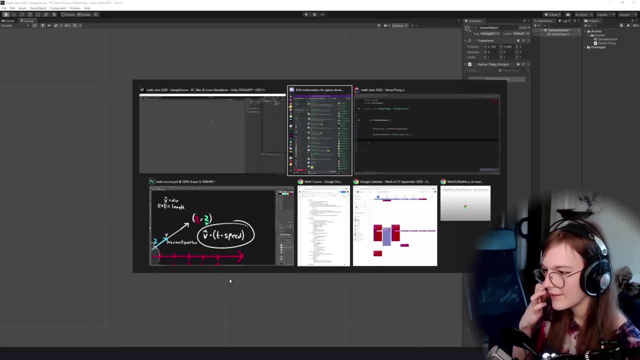 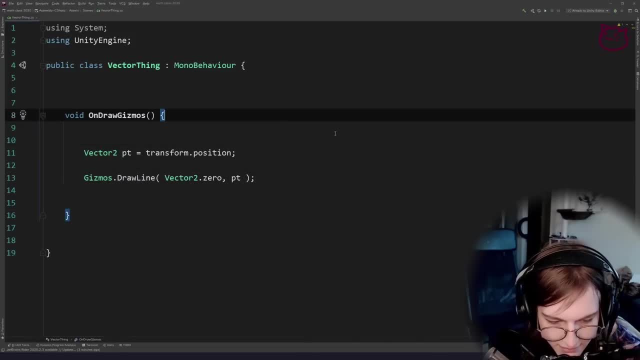 and then we have the x-axis and the y-axis right here. Oh, you couldn't hear the Discord. You should have been. It might have been a lower volume, So all right. So now we have the points right. So now let's say: you want to get the direction to this point. 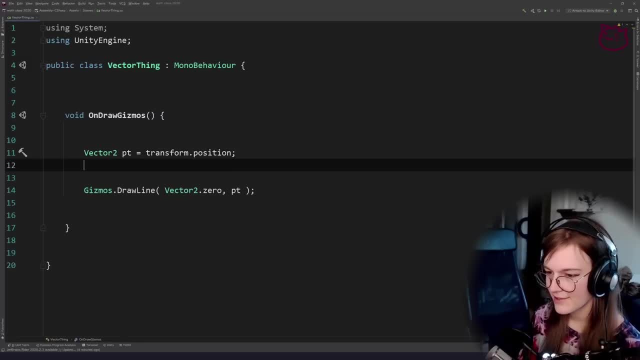 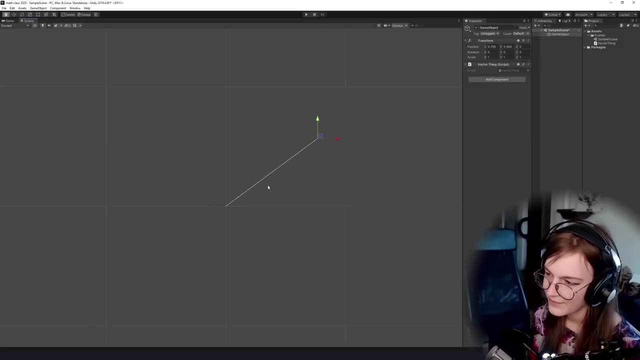 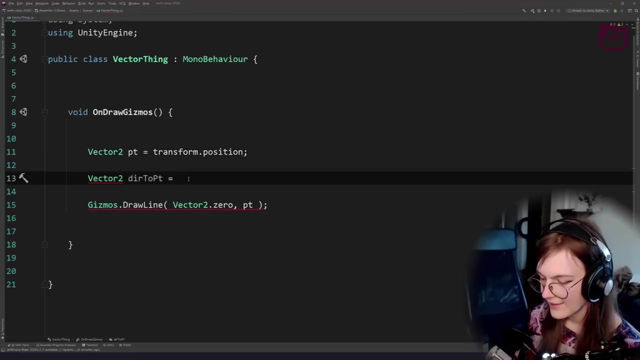 because we have been talking a lot about directions, right? So let's see, So, let's get that, So direction to points. So, in this case, because it's originating from zero and we just want the direction to this arrow, then all we need 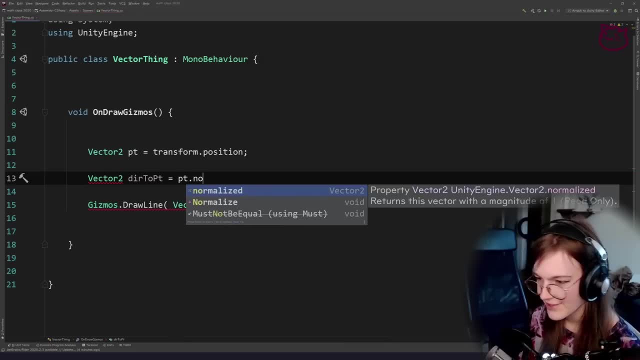 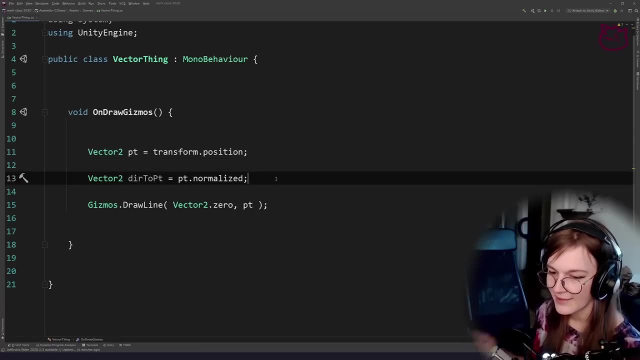 to do is normalize that point right, And Unity has a bunch of built-in functions You can do pointnormalized, and that's going to return a normalized version of this point, right, So yeah, So now we have the direction to the point. 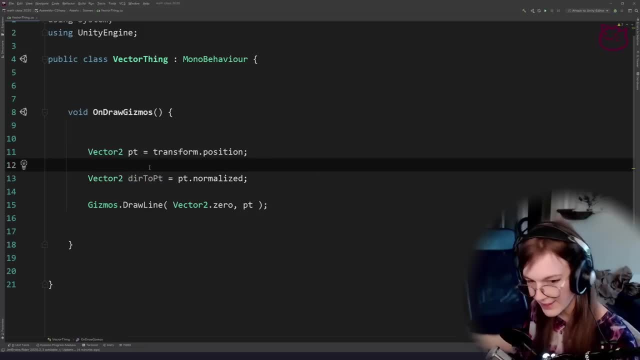 And again I'm using the word direction to mean a vector of length 1, which is sometimes also called unit vector, normalized vector, Like. it has a bunch of terms, but usually when I use the word direction I mean a normalized vector. 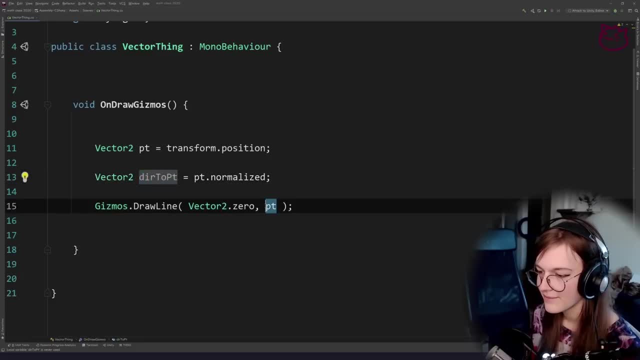 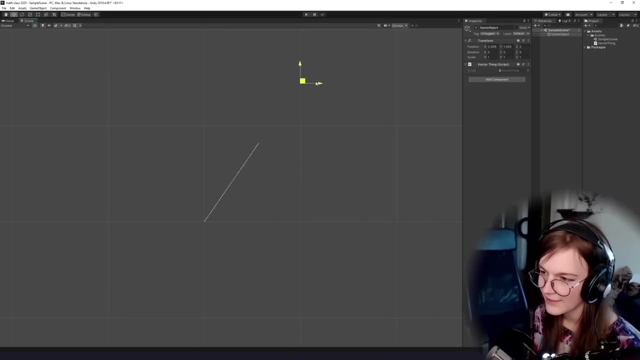 just to clarify. OK, So if we draw that instead and then go back to Unity, now this line always has a length of 1, right, Doesn't matter how far away the transform is, but this line, right, But the length of it is also 1.. 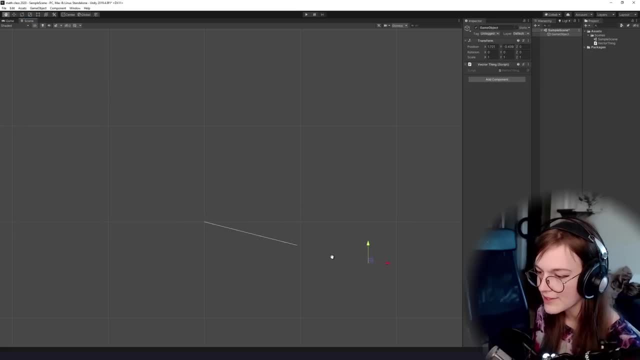 Even if it's shorter or longer, it's going to normalize it to always be unit length. So now it's sort of tracing the outline of what's called the unit circle. So the unit circle is just all the points of the vectors that have a length of 1.. 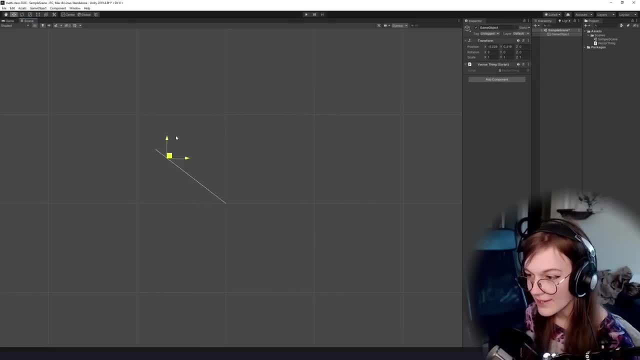 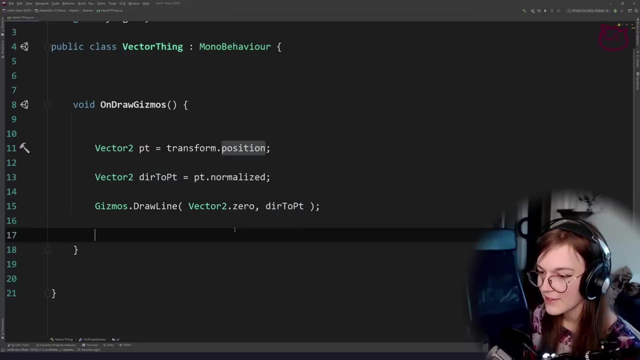 So it's this circle right here, right. So now we have a direction, right. What if you set the transform to 0?? So probably now it gets very sad because the- I'm pretty sure- normalized it looks like it's just returning a 0 vector. 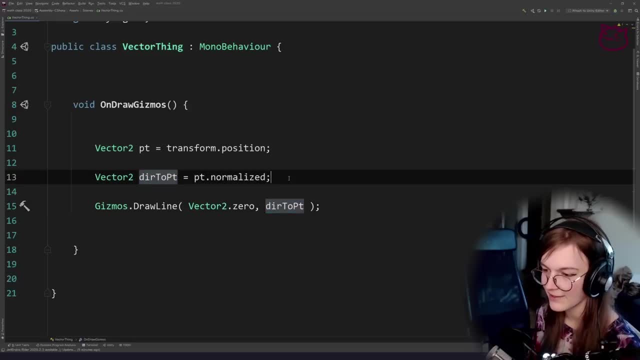 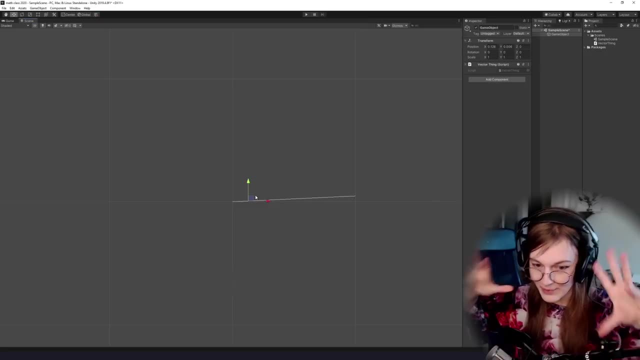 So now the quote unquote direction that this returns is going to be 0. So it's trying to draw a point from, or a line from, 0 to 0.. So, speaking about that, this is a very good case where, when you have something like this, 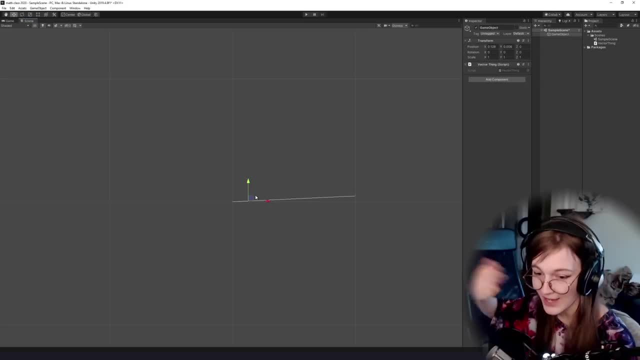 this is actually division by 0, like technically, We're going to get into how to calculate the length or how to calculate normalized vectors later, But this is actually division by 0, and something that is kind of beautiful in mathematics is that any time you are dividing by 0,. 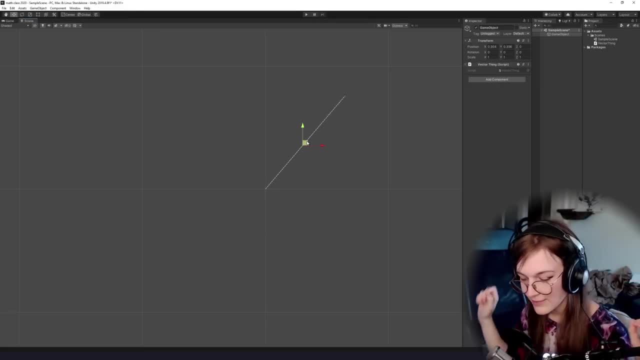 I think this is so mind-blowing. but every time you're dividing by 0 in some equation, that is kind of the math talking back to you saying that, hey, this is a weird case, You need to handle this case. 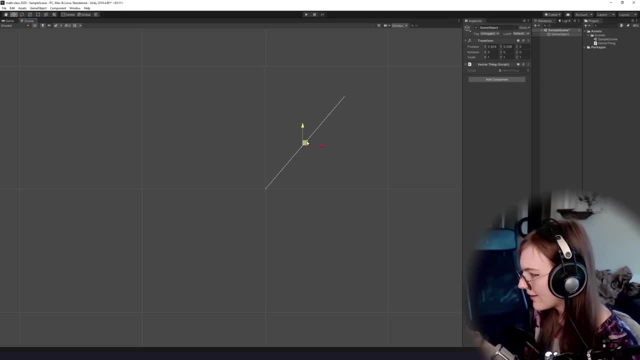 Something is happening here and you need to think about what do you actually want to happen in this case, Because it's kind of telling you that there is a degenerate case or a case that you cannot calculate because division by 0 is undefined. 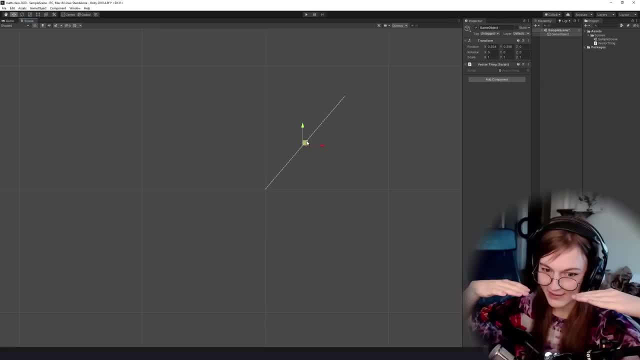 So, whenever you have an equation where there is a divide line, think about if the denominator can ever be 0. If it can be 0, figure out what that means. right, Like when would this be 0?? Anyway, OK, so now we're just drawing the normalized version. 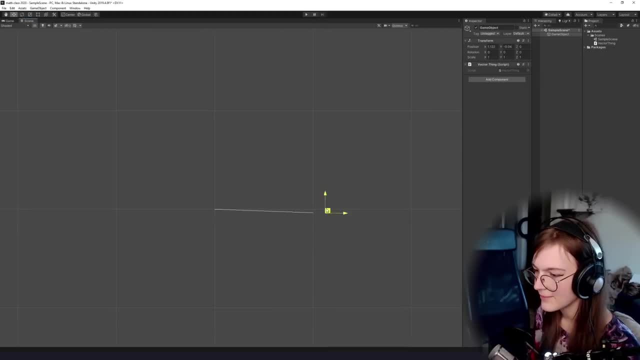 of this vector. Do you have a course at Udemy? No, but I have my YouTube channel, which is free, so you don't have to pay for it. All right, cool, OK, so let's talk about the length. 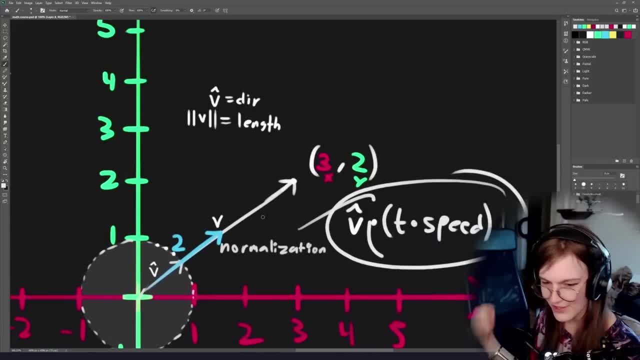 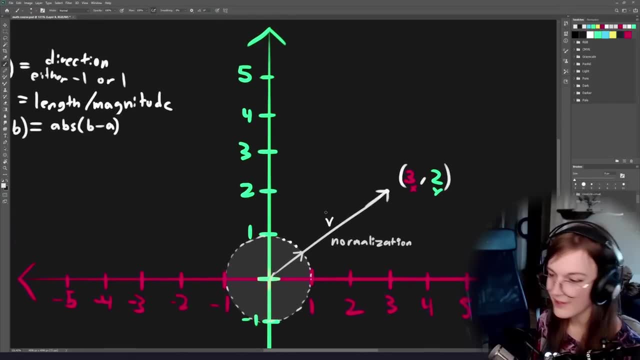 because we've sort of mentioned the length a lot when it comes to normalizing things. We probably should have talked about length before normalization. but you know what? That's OK, All right, so let's talk about length. How do you get the length of the vector? 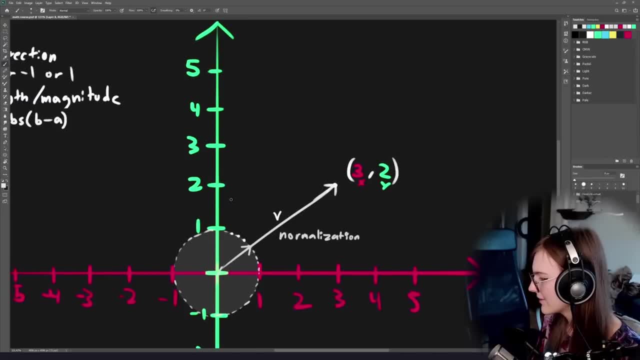 I might be skipping ahead. but when you say the vector2.normalize divides by 0, where does it do that? You are sort of skipping ahead. I'll get to that. But technically Unity's vector2.normalize handles that case and just returns a 0 vector instead. 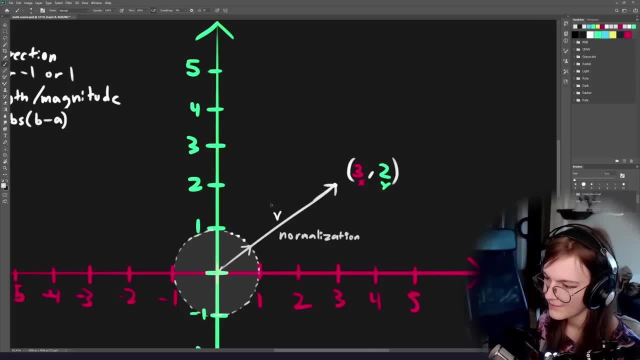 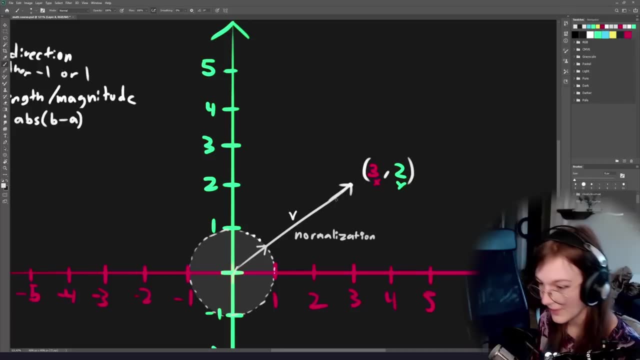 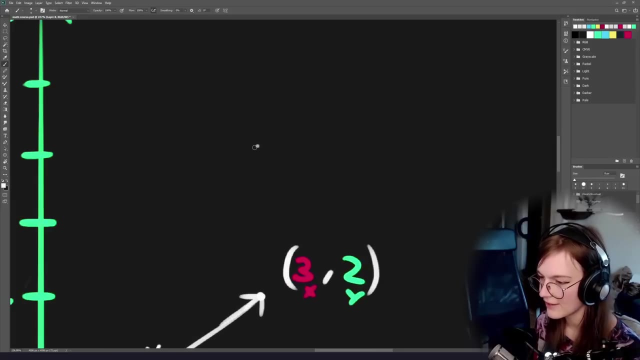 of crapping out and not knowing what to do. You could sort of make a normalized function that just throws an exception, which might be useful, But Unity's normalized just kind of just returns a 0 vector. Oh, a 0 vector is just a vector with components at 0.. 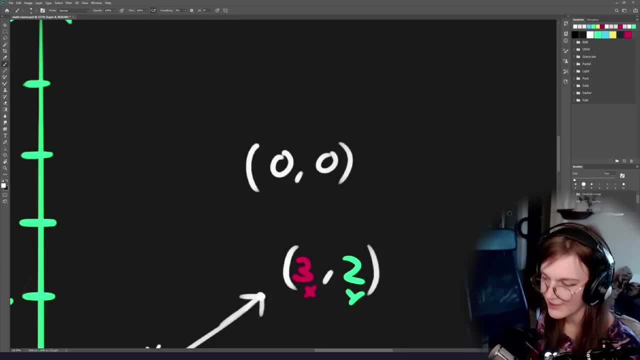 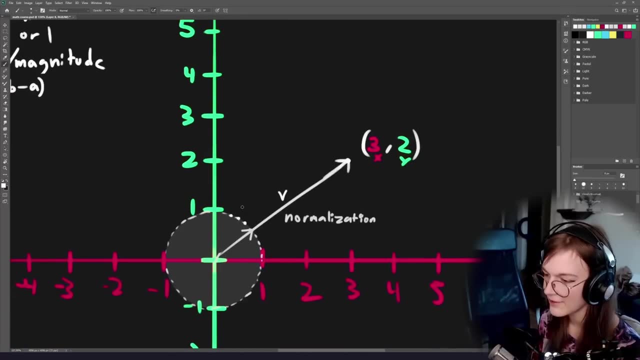 So all of the components are 0, sometimes called a 0 vector. Yeah, OK, so we talked about normalization, but not how to calculate it. Like, how do you normalize a vector? Like, how do you go from this to whatever the heck? 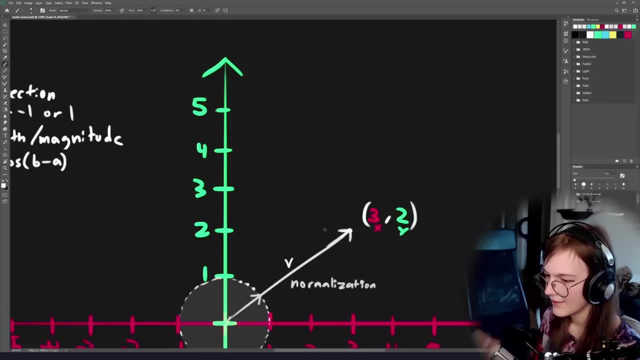 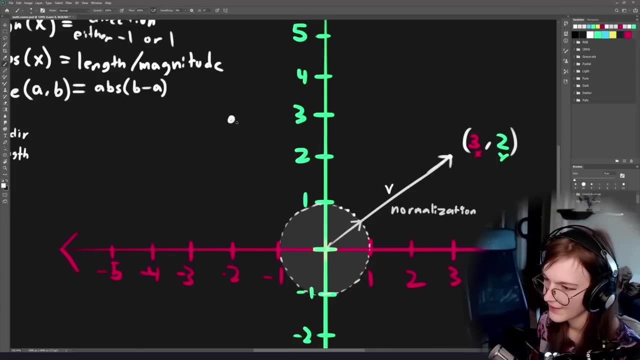 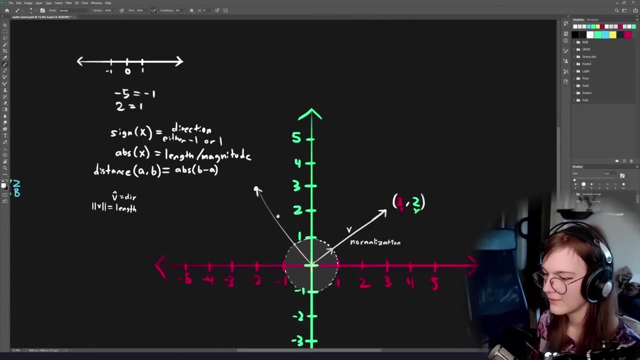 these coordinates are right, All right. so if there is, I don't know if we should use this vector- Let's do another vector. Let's do this one. What a vector. It's a little curved, but pretend it's not. 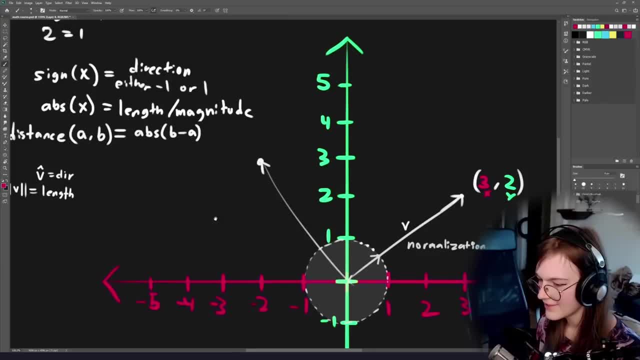 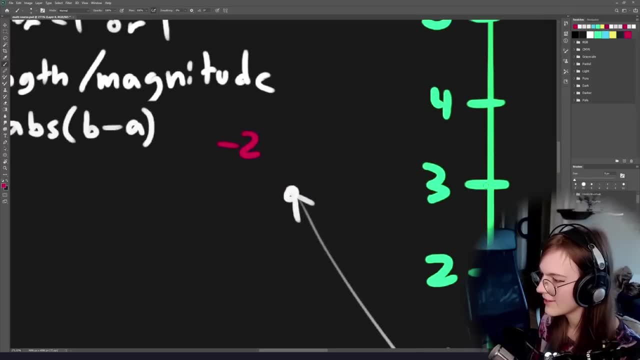 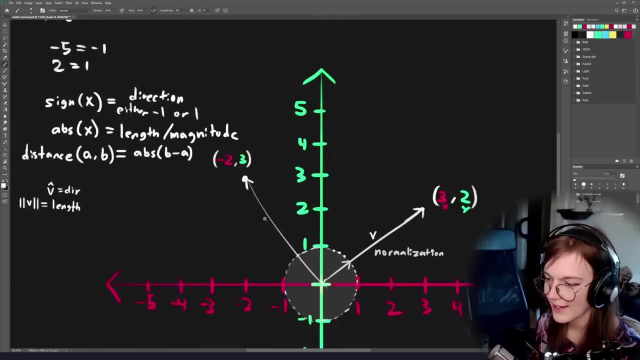 All right, so let's see What is this vector? So we have x-coordinate, we have negative 2.. y-coordinate: we have 3, right, So this is our vector. So now we want to know the length of this. 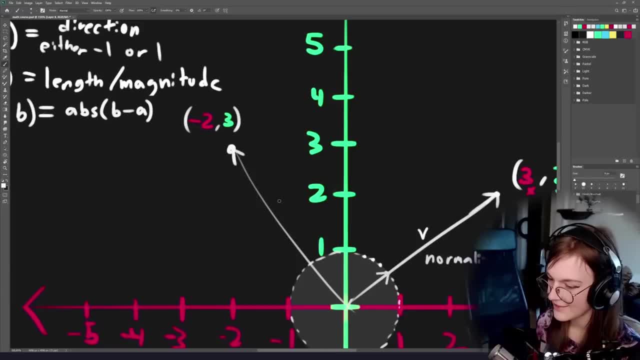 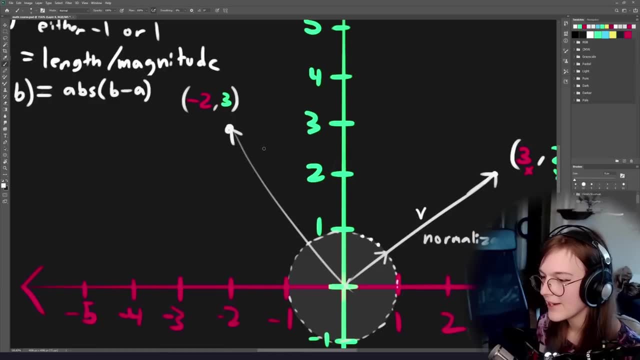 Like, how do we do that? So now this is going to get into the Hacking Pythagorean Theorem, right? Because if you think about it, if you want to get the length of this, you can sort of imagine a triangle here. 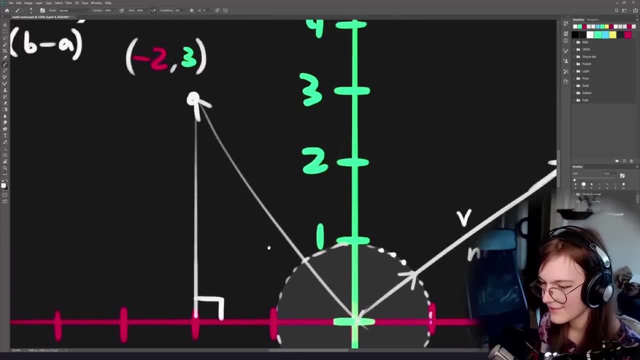 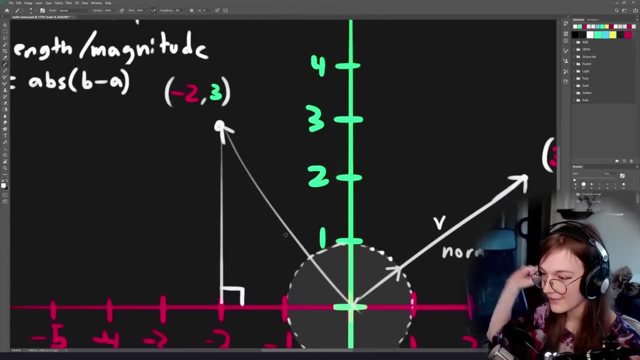 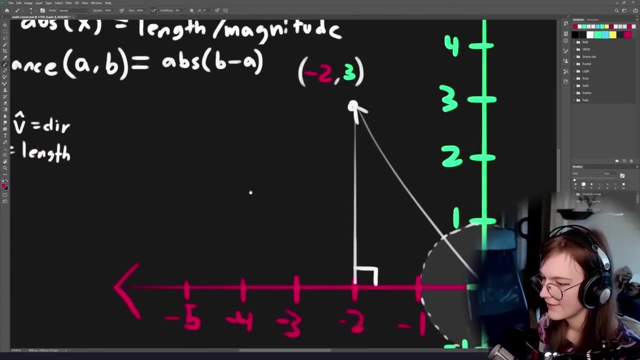 And this is a right angle triangle, And this is something that is taught in math class. So if you remember how to get the length of the hypotenuse, then you know how to get the length of a vector right. So, basically, what we need to do then is we take the x-component. 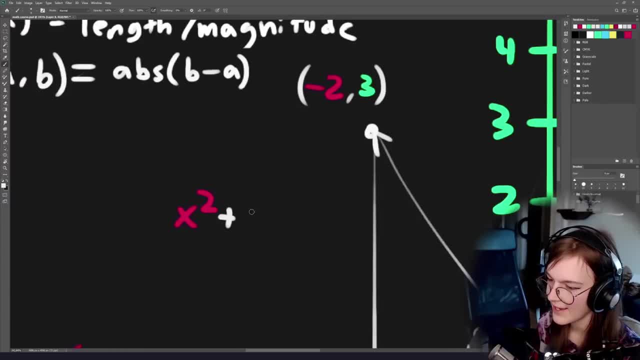 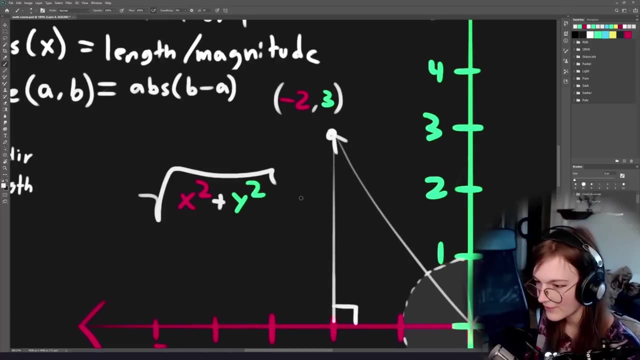 square that, and then we add the y-component and square that, And then we take the square root of all of this. There we go. That's the Pythagorean Theorem. That's how you get the hypotenuse of a right angle triangle right. 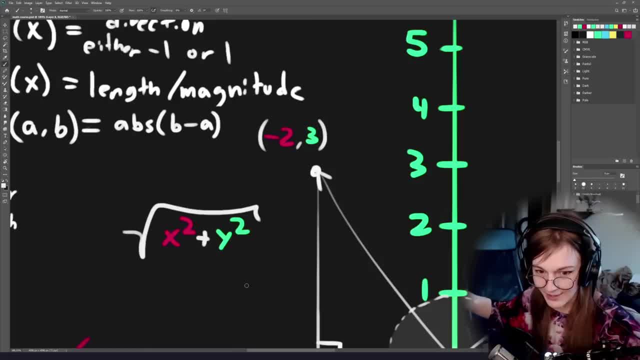 But this is how you get the length of a vector right. Is that clear? by the way, We haven't talked about like exponents or what it means for something to be squared, or talked about square roots, But I'm guessing we don't need to talk about that. 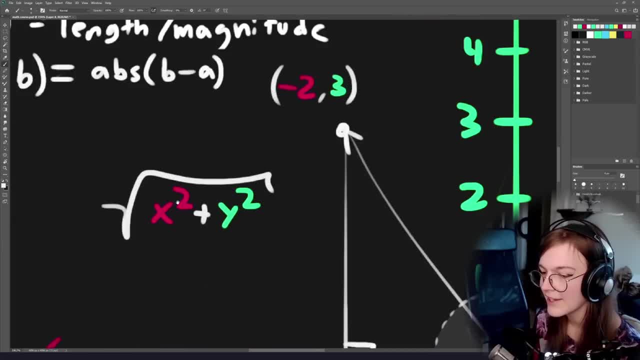 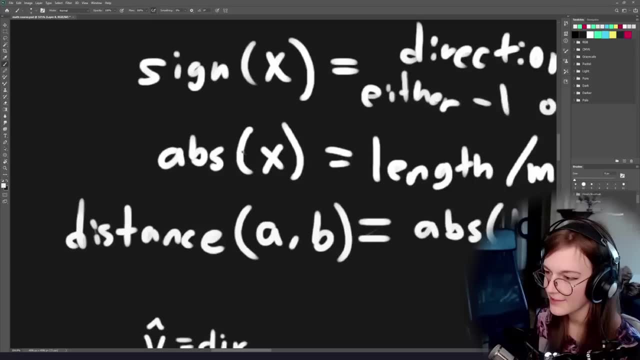 But if not, let me know We can talk about it. OK, So this is basically how you get the length of a vector. All right, that's it, I think. So now we've been talking about, we talked about for one-dimensional numbers. we have abs instead. 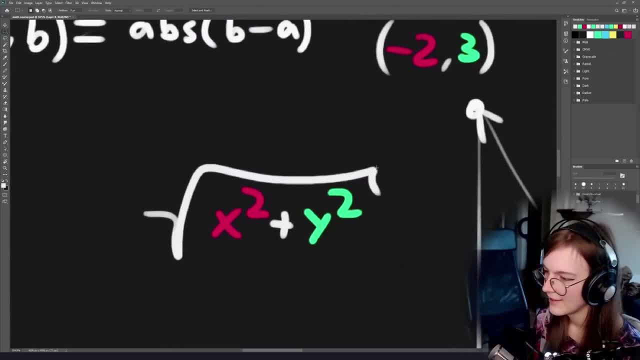 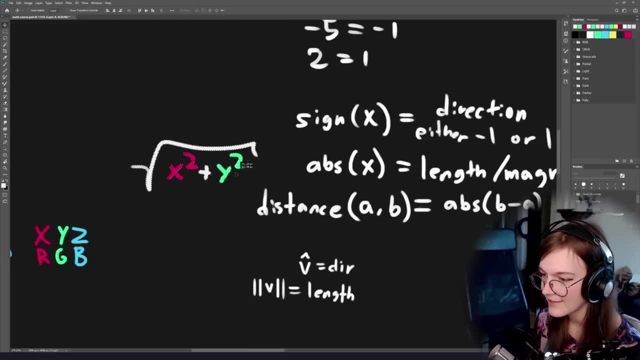 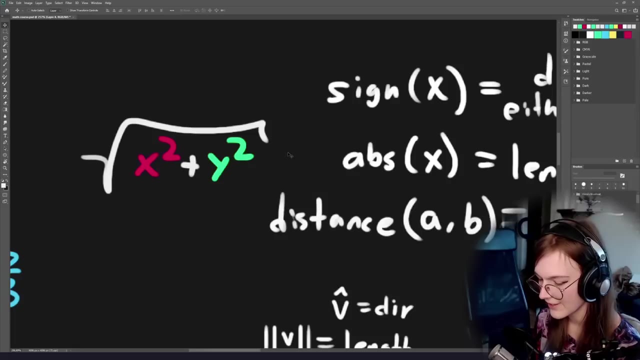 of something else But the generalized concepts. you usually write it like this for any other vectors: You can add more components inside of this square root. You can add z squared, and then you have the length of a three-dimensional vector. So it's the same thing like regardless. 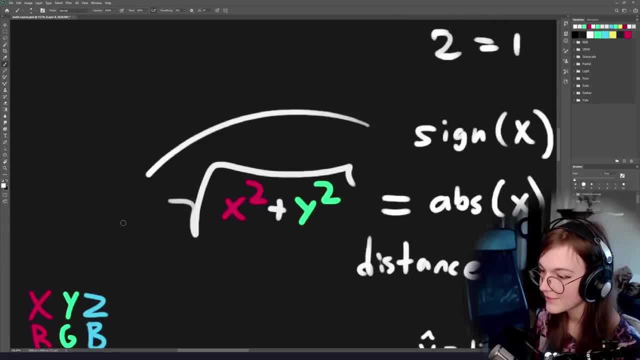 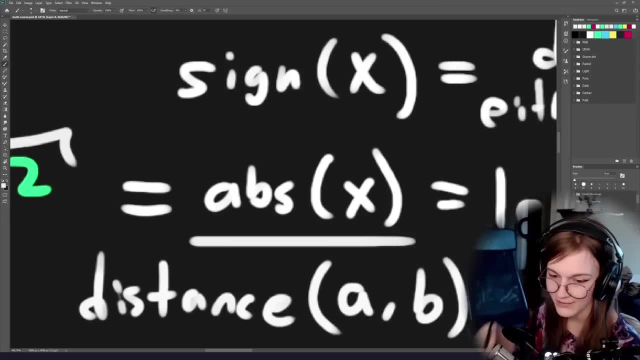 of how many dimensions we have right, And this actually holds even for one-dimensional vector. So we talked about one-dimensional vectors, where you can use the abs function, which is basically just: if it's negative, make it positive, But you can do this for one-dimensional vectors too. 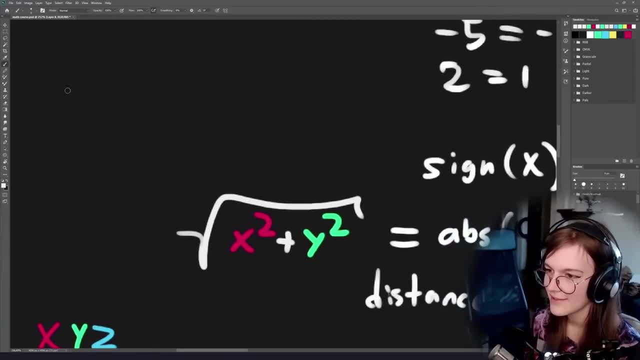 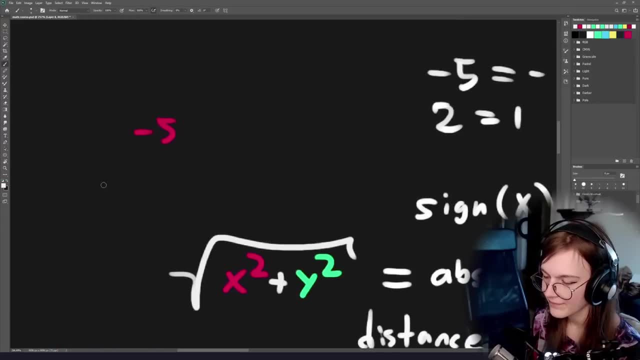 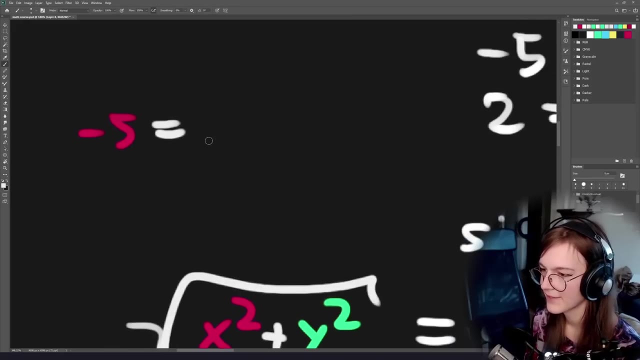 OK, So if you have the square root and let's say we have the one component of negative 5, for instance, All right, so let's just do the equation for that right, We do the square root of 5 squared. 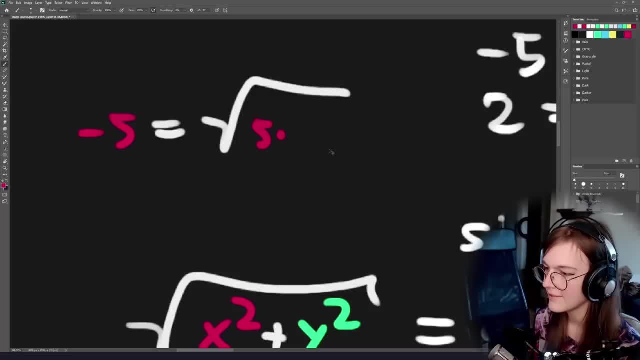 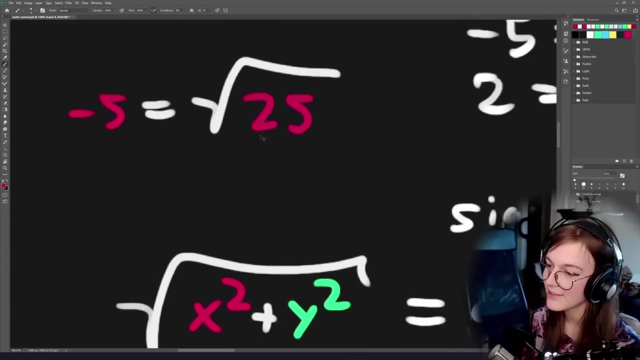 So that's 5 times 5, right, Which is 25, I think, I don't know Pretty sure. So that's 25, right? Oh, actually, sorry, Not 5 times 5.. Negative: 5 times negative 5.. 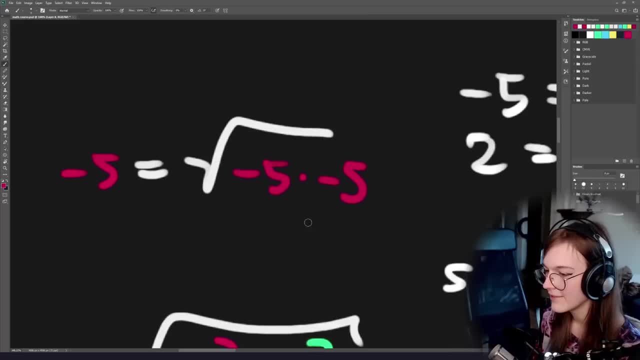 If you multiply two negative numbers then it's going to be positive in the end, because the signs sort of cancel out right. So we get positive 25.. And then when we do the square root of that, by convention, square roots technically have two results. 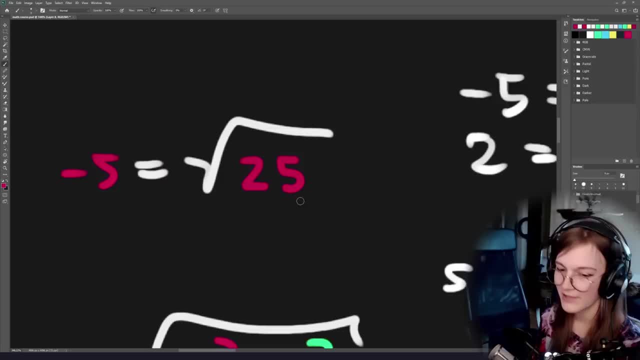 but we're not going to get into that. So technically, this then returns 25.. But we're going to get to the square root of 25, because the square root of 25 is 5.. The equal sign is incorrect. yes. 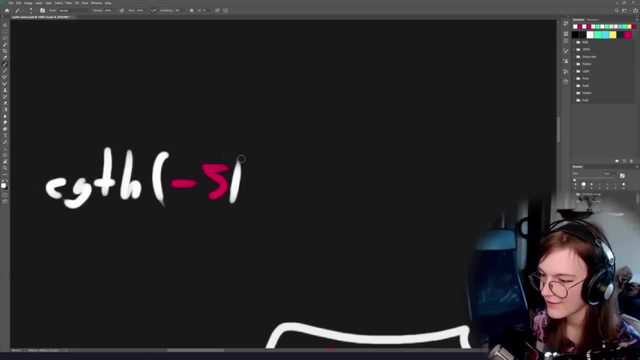 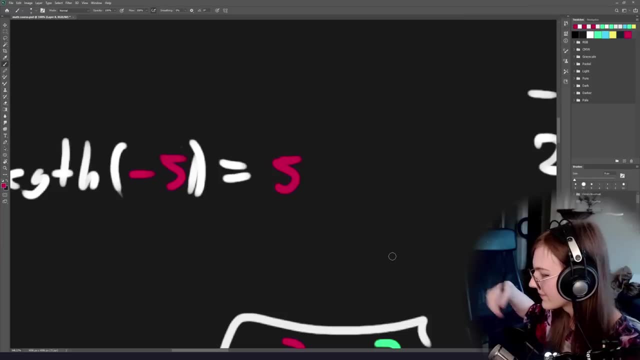 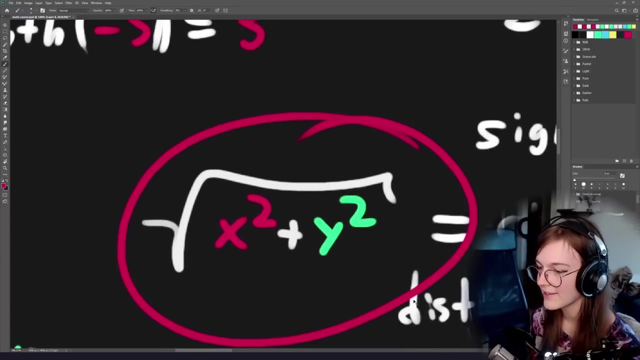 Because this is the length of that- Sorry Length of negative 5 then just ends up being 5, because that's what the square root then returns, right, So yeah, So it's just kind of like the same equation works for any vectors. 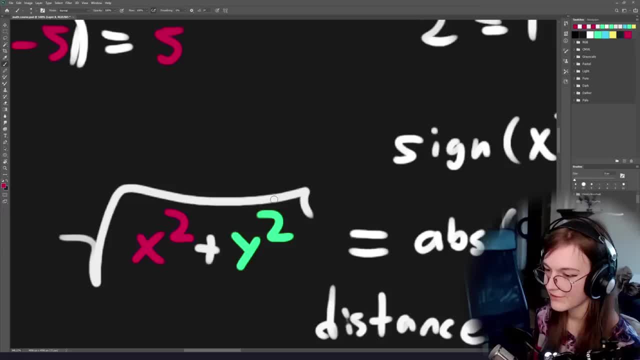 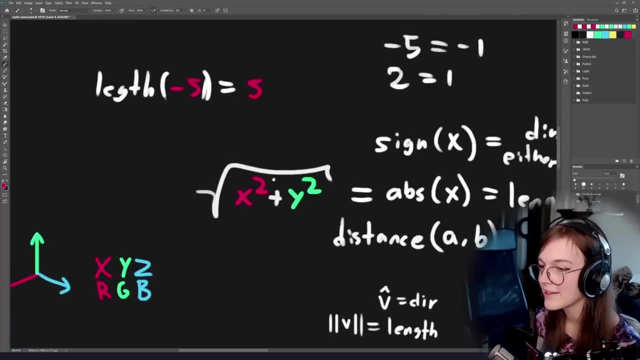 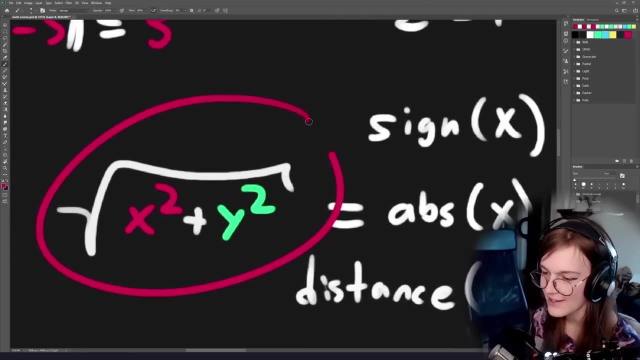 Now, in practice, when you want to get the length of, you know, want to get the length of a vector, For one-dimensional vectors or just scalar values, usually use abs. You don't actually do the full equation, But for anything like any dimensions. 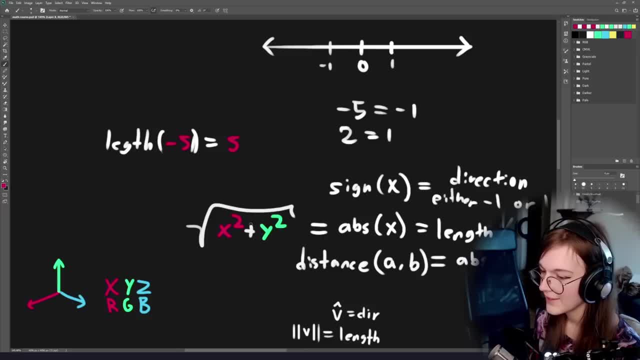 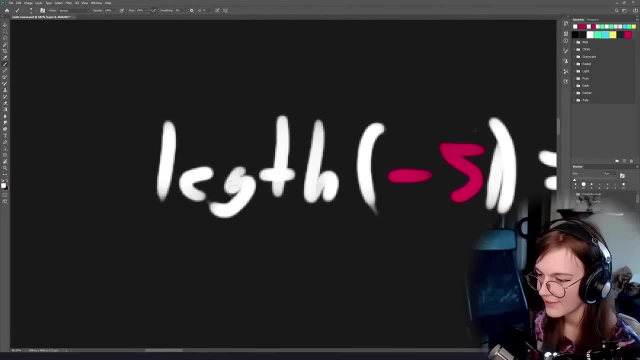 above that you generally use the Pythagorean theorem. Okay, So this works for two-dimensional vectors too? Oh, I actually didn't. Sorry, Legs, You know, I actually have a cold right now. So this is like canonically kind of more accurate. But sorry, Sometimes my backwards writing doesn't. 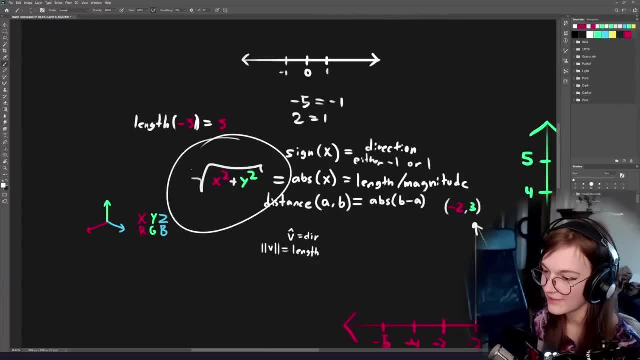 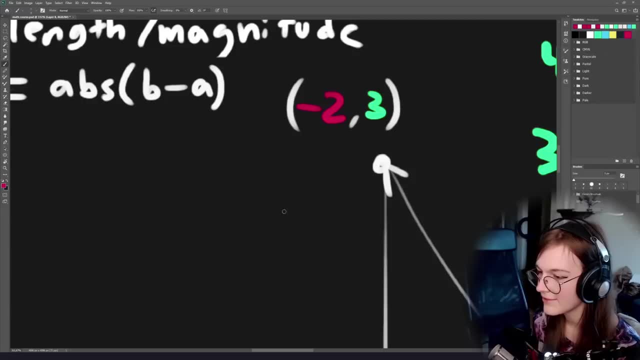 work out Okay, Cool. So now we have that. right Now we can actually do that math. So if we want to get the length of this one, we can just do that right. So that's negative two times negative, two plus three times three, And then we do the square root of that. 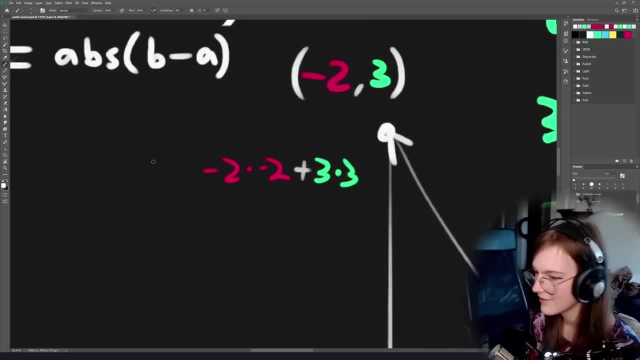 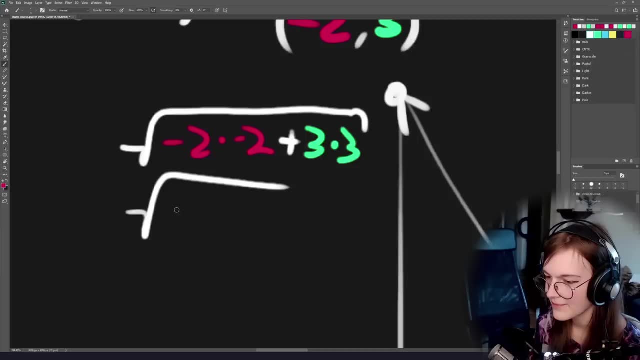 This is not a good looking square. Where's my good color? There we go. So then we can just run these numbers right. So, all right, we do: square root of negative two times negative two, Pretty sure that's four. So it's going to be four plus three times three, That would be nine. 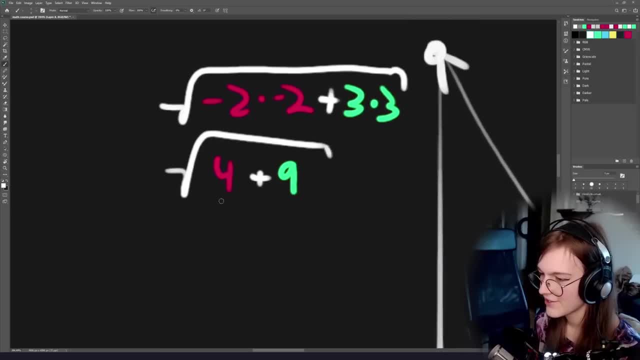 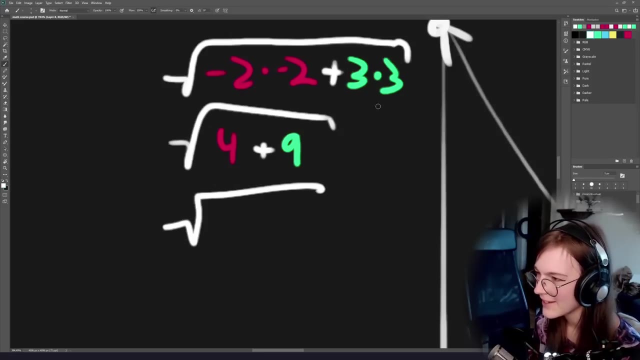 So four plus nine, which is, oh God, That's 13, I think. Look again, I'm really bad at doing math in my head- Pretty sure that's 13.. All right, So it's no longer really tied to the X or Y axis. 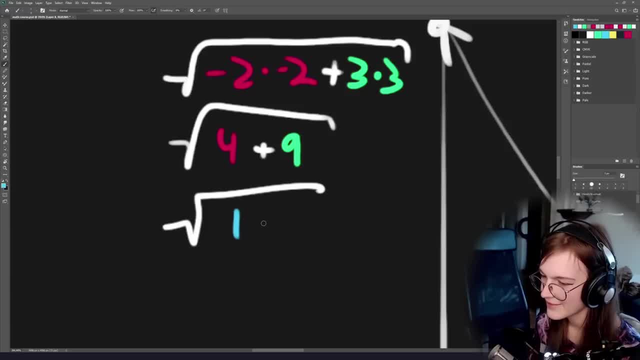 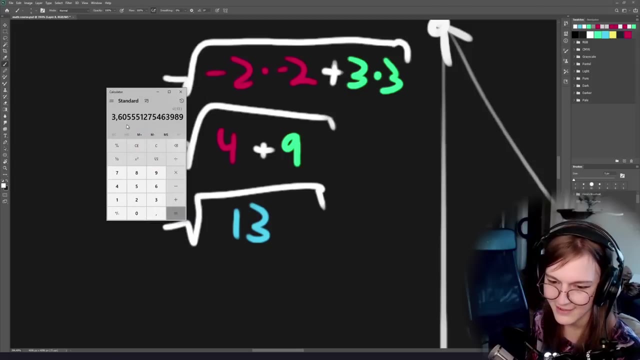 I guess we can make it blue or something, So that becomes 13.. And then we want to calculate that. So that's when you pull out the calculator And you type 13, and then you do the square root of that And it turns out it's 3.6, something. 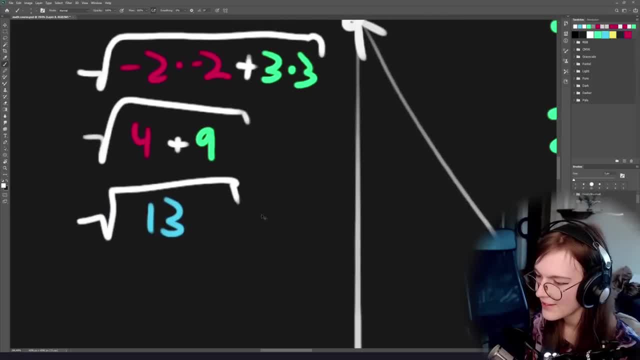 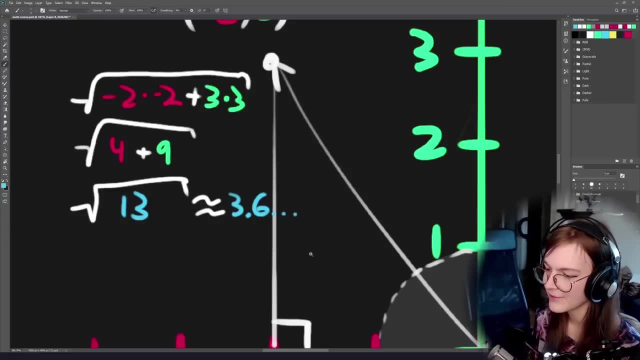 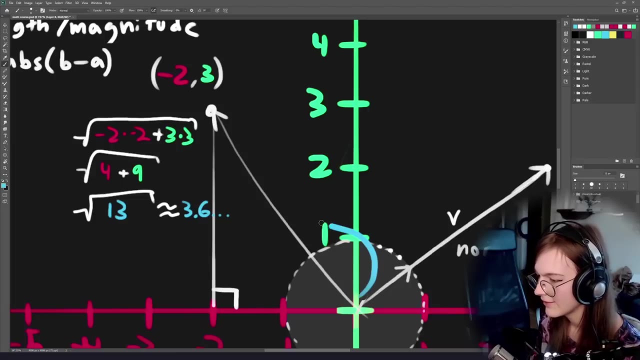 right, So this is approximately equal to 3.6.. Oh sorry, We will do it in blue, Why not? Cool. So that's how you get the length. So now, what this value represents is the length of this right here, right. 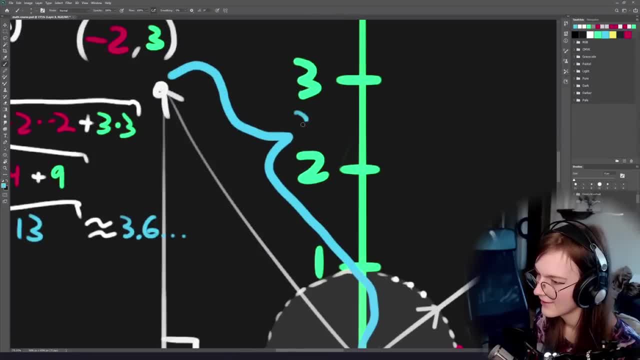 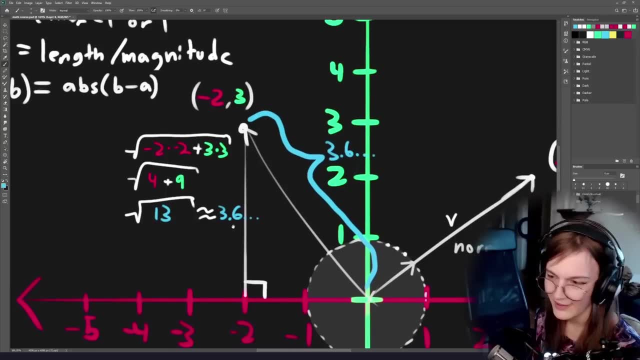 So the full length of this vector turns out to be 3.6. something, something, right? So now we know the length of it, right? Cool, That's how we do it, If you want to get the like, if you want to. 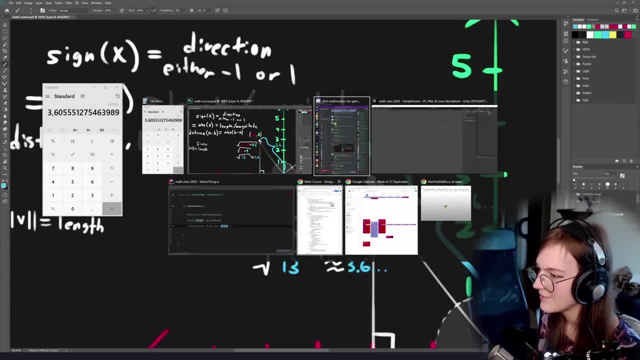 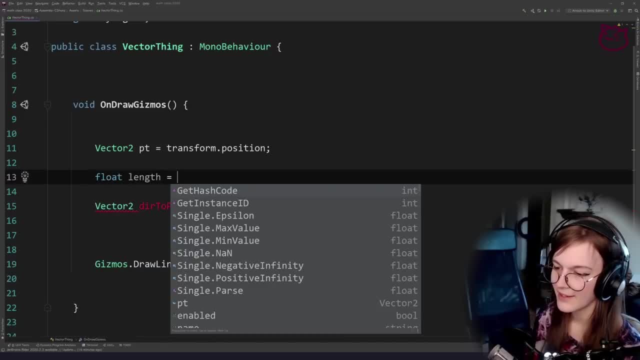 do this in practice. you almost never write this formula yourself. So if you go to Unity, if you want to get the length of the vector, again, length is a scalar, It's just a single value, So the length of this one would be. 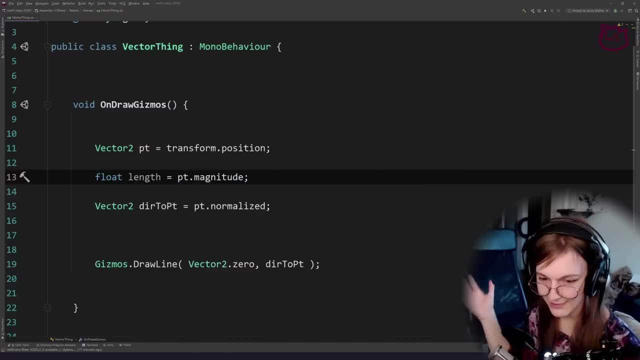 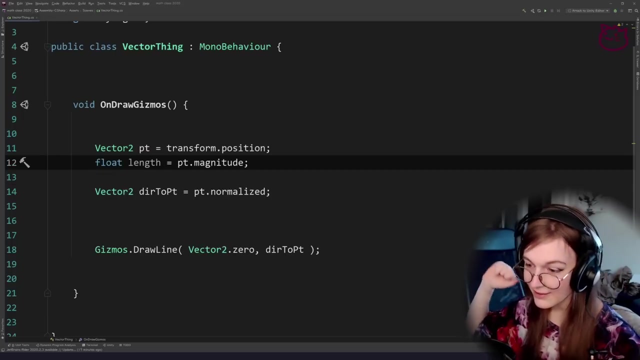 pointmagnitude, Because, again, magnitude and length same thing. Yeah, So this is how you get the length. Sometimes it can be useful to calculate the length manually, Because sometimes you want both the length and the normalized vector, And in that case calculating things manually can be. 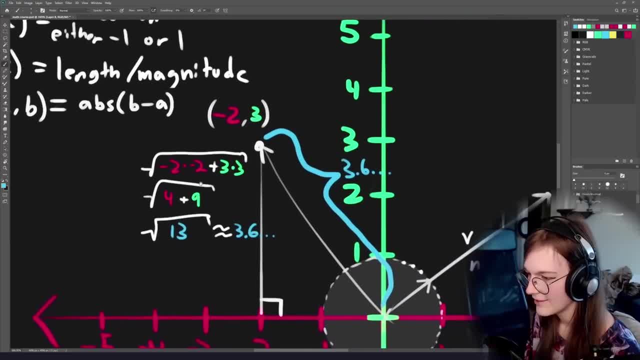 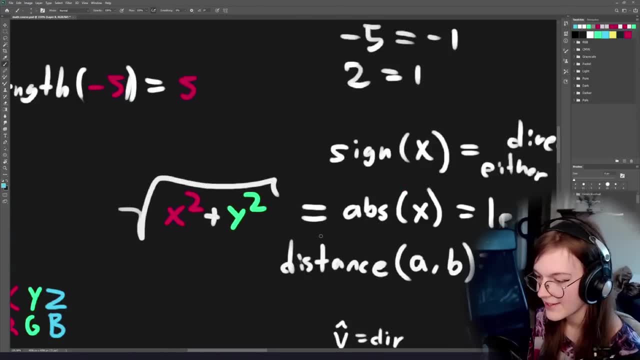 really useful, Cool, Everything clear so far: How to get the length of a vector. So now we've just talked about how to get the length, And now we're going to talk about how to get the length of a vector, But not how to get the direction or sign, And not how to get the distance. Okay, Let's do. 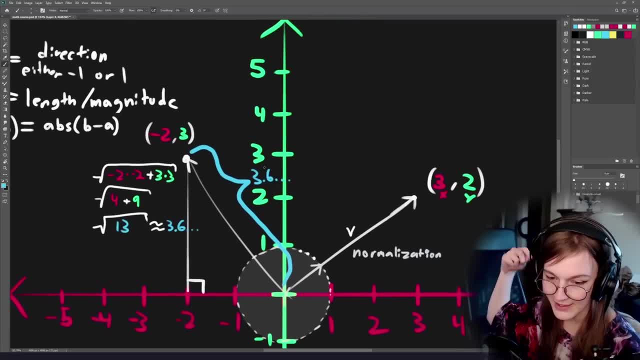 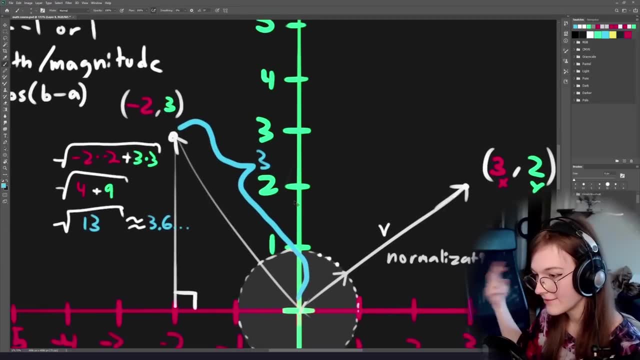 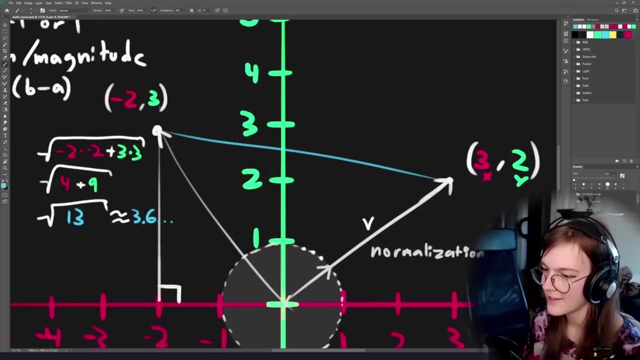 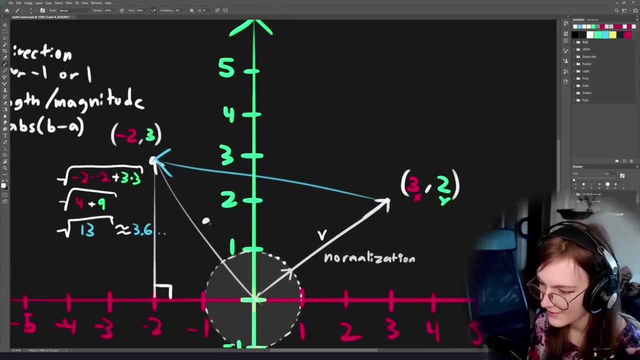 the distance. So the distance, now that we know how to get the length of something. now, if we get the difference vector or the displacement between two vectors, let's say we want to get this vector between these two right here, Then this vector this would be- we don't have names for these, We'll 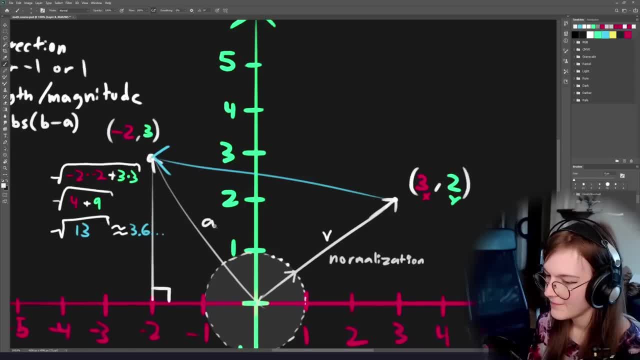 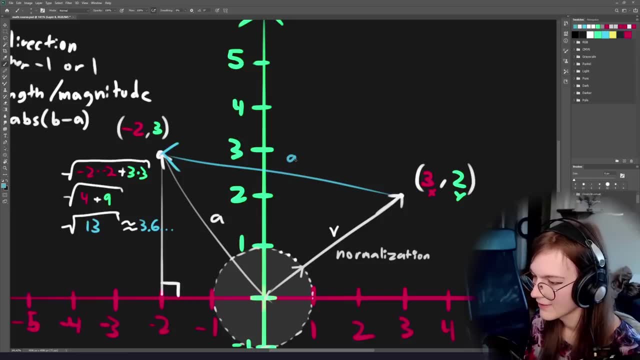 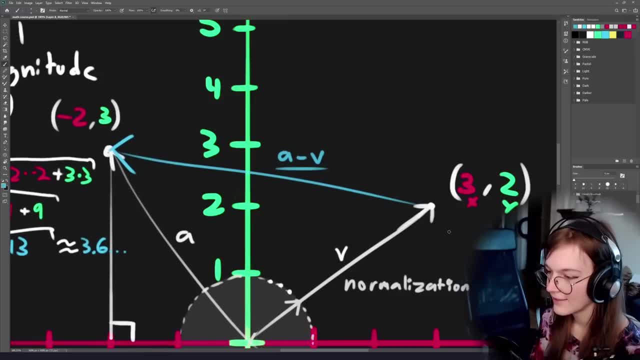 v. So now we have the difference between these two points, right? So if we want to get the length or the distance between these two vectors, all we need to do is get the length of this vector, Because that, like, if we know how to get the length of this, 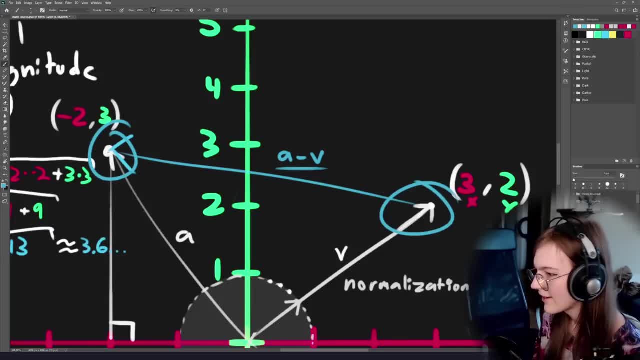 then we now know the distance between these two points. And in this case it also doesn't actually matter if we do v minus a or a minus v, because if we're just interested in the distance, the distance is always positive. so it doesn't matter which order we do this in. 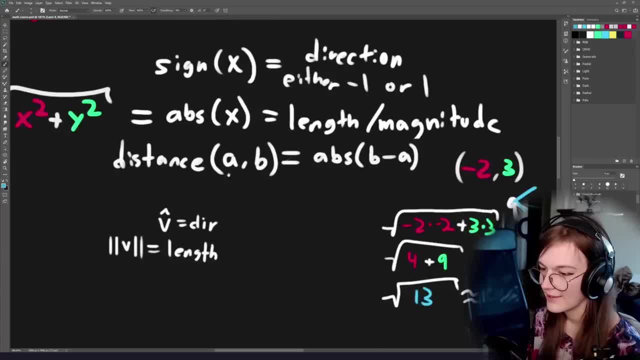 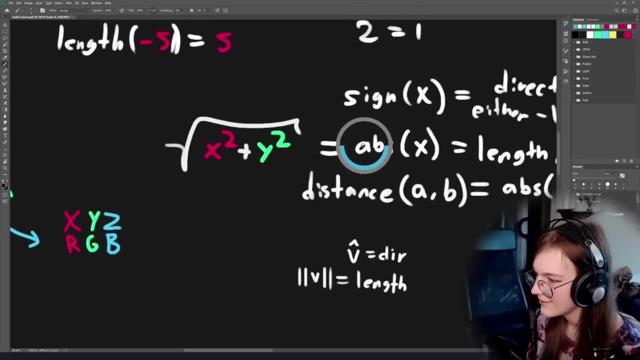 So if you want to get the distance between two points, previously we did the absolute value, because that's how we did the distance in one dimension- Actually, we never call it length Anyway. so this is how you do the length, So we can basically just replace this. 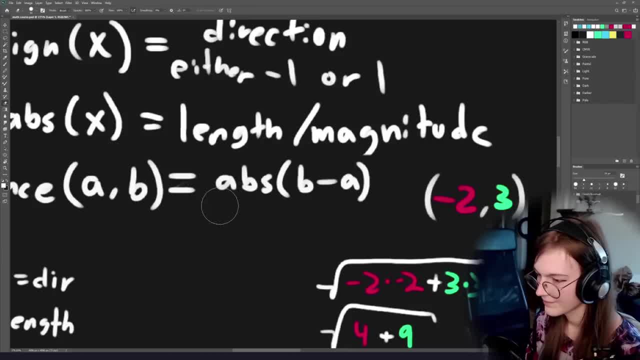 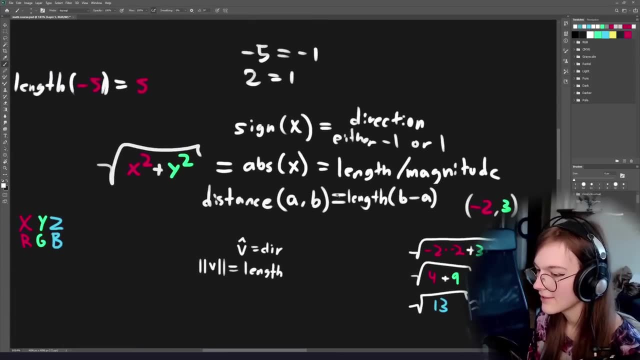 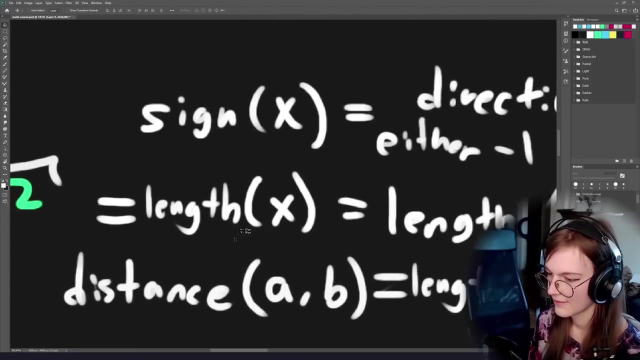 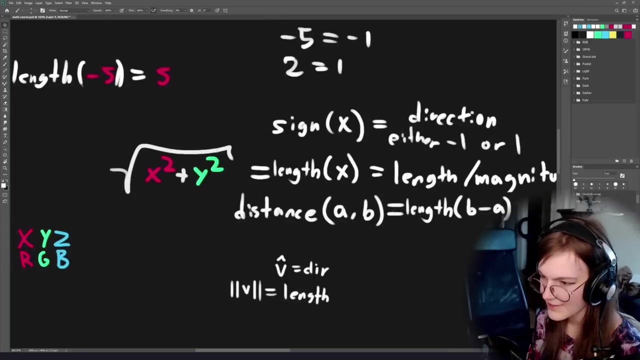 by calling it length instead. right, So now we can get the length of this one, and the way to get the length is this one: right here, right, There we go, All right. so basically, this is how we get the length. 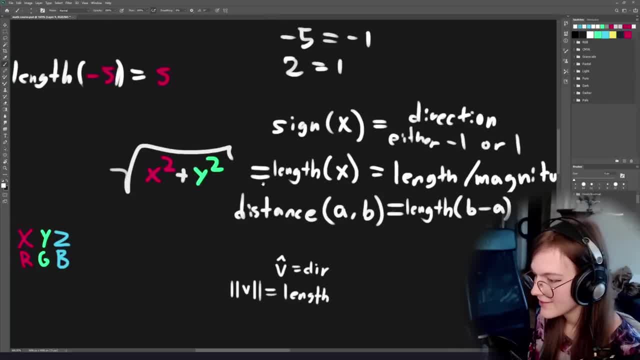 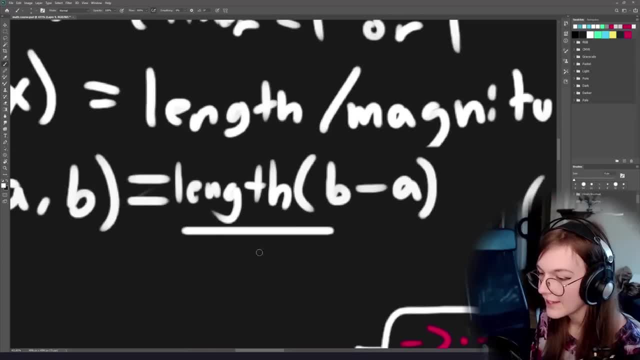 If you want to get the distance between two points, then you subtract the points, one subtracted by the other, and then you get the length of that vector and then you get a distance. So there is a slight difference in terms of interpretation. 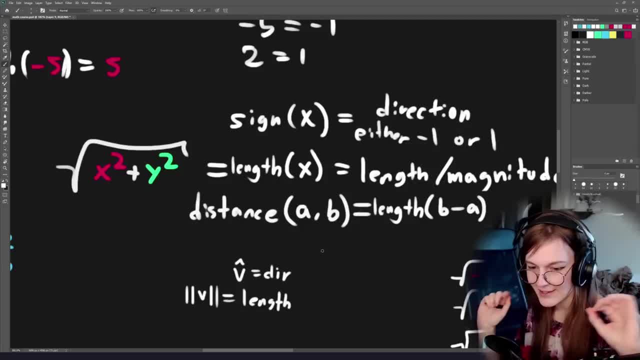 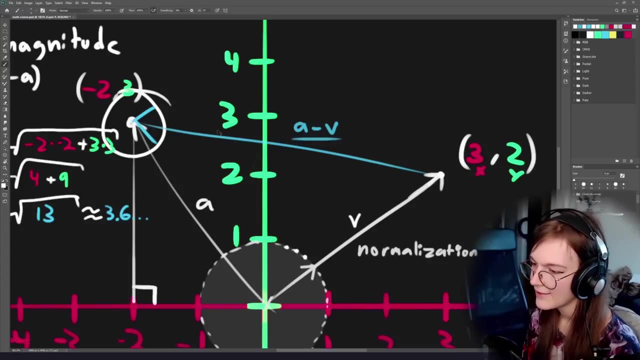 between distance and length. So distance usually is between two points And length is usually the length of one point or the length of the vector that represents that one point. So when we want to get the distance between this point and this point we first subtract them from each other to get the difference vector. 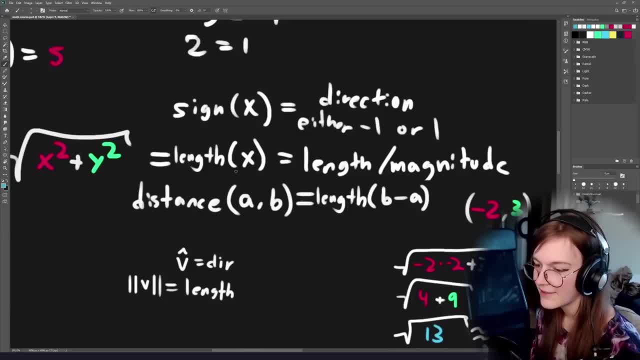 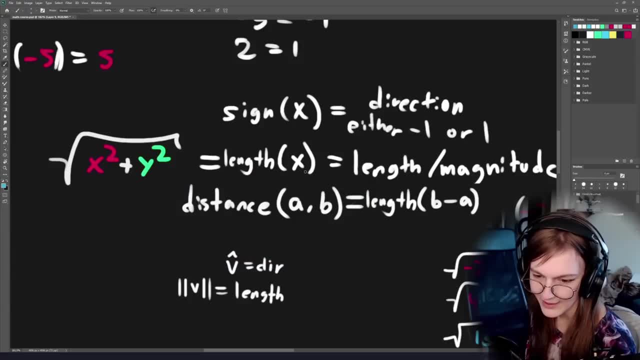 and then we check the length of that difference vector. All right, so now we have a way of getting the length, We have a way of getting the distance. Have we clarified that the resulting blue vector is still centered on the origin? We talked about that. 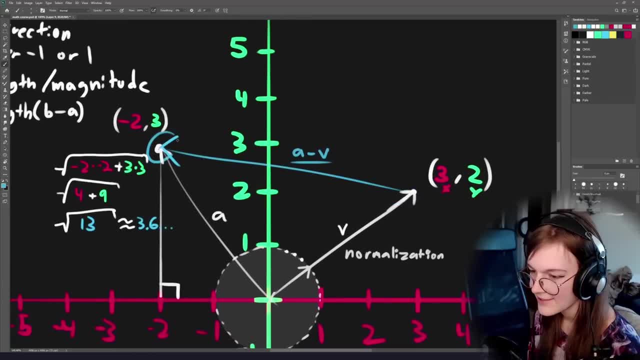 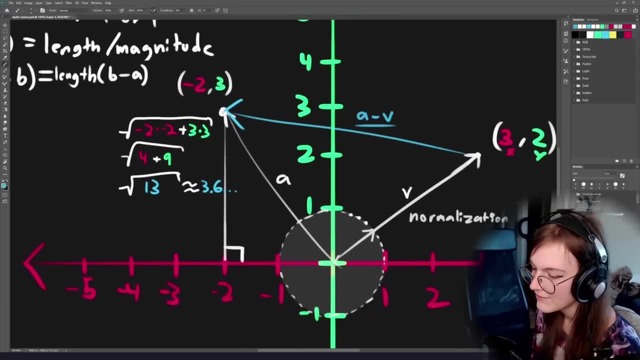 Yeah, like vectors don't have a root and a tip, It's only the vector data itself, right? So we talked about that when we talked about subtraction, that if you want to draw it at its origin, it would be this vector, right? 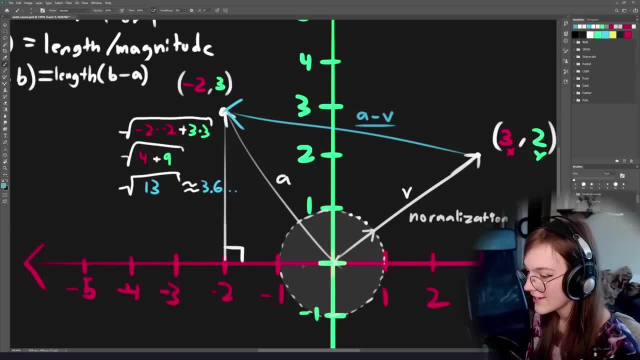 Length magnitude is of the vector. Distance is between two vectors Generally, yeah. So when you talk about distance, that's a special case where you want to know how long is the vector, that is the displacement between these two points, basically. 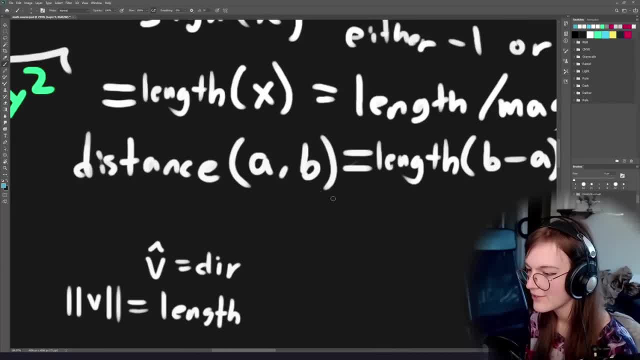 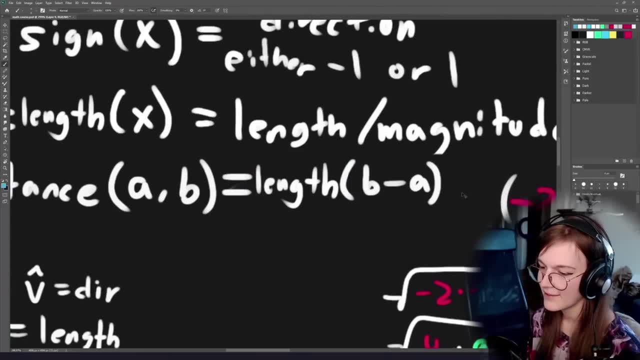 So when you talk about distance, again, distance has an input of two points usually, And then you get the difference of those two points and get the length of that, If you want to know the length of something. it's just one input, right. 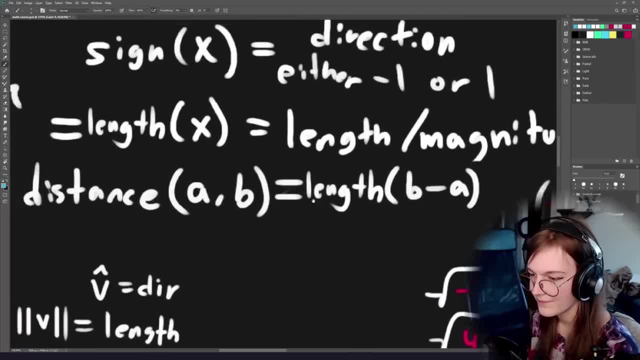 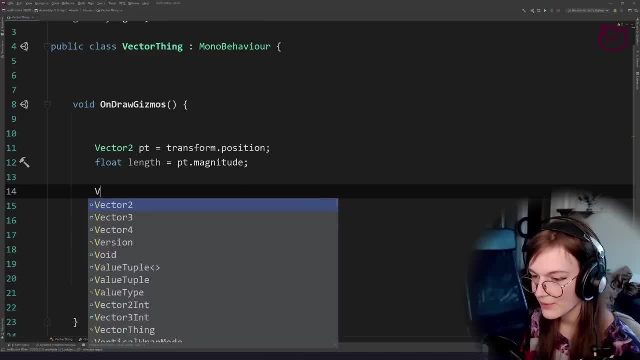 So that's just the length of one vector. Yeah, of course there are built-in helpers for this. You don't have to do it manually. So if you want to know the distance between two points, you can use vector2.distance from A to B, or DB null, I guess. 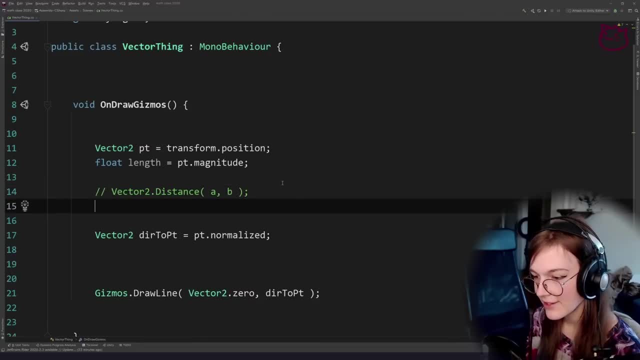 So this would give you the distance. But you can do it the other way around too. You could do A minus B dot magnitude, for instance. This would also give you the distance. It's the same thing, right, All right. 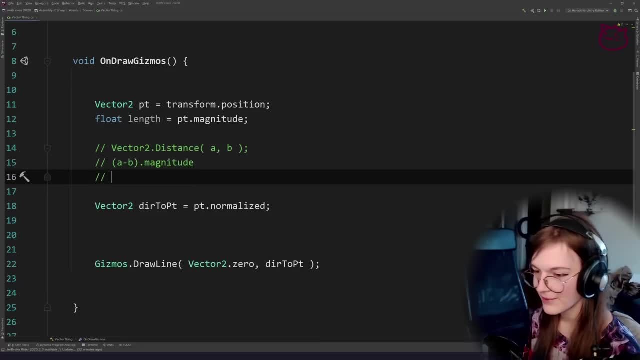 Or you could do the manual way, if you want to, of doing A minus B, like A dot X minus B dot X, And then you square that And then you add the same thing but for the Y component, And then you do the square root of all of that. 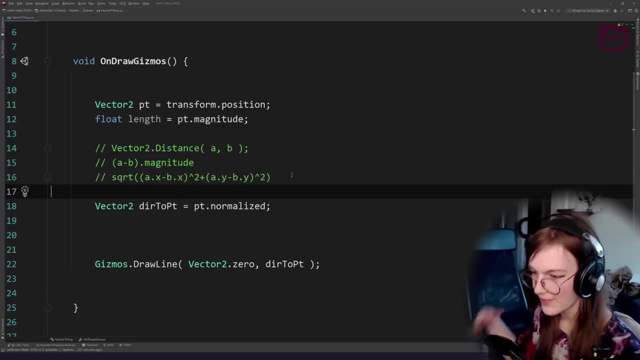 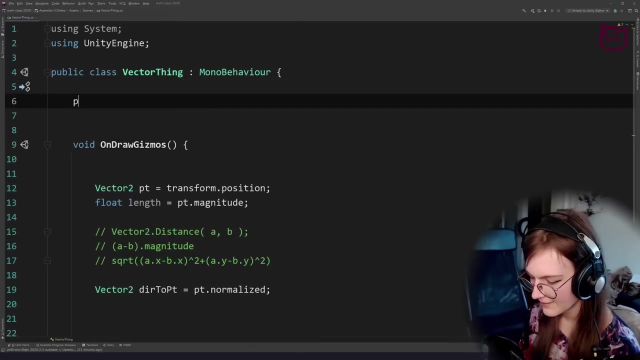 So this is the same thing. This is also a way you can get the magnitude or the distance between two points right. Yeah, just different levels of abstraction. I guess How to apply it in practice? Well, we could make Two points. 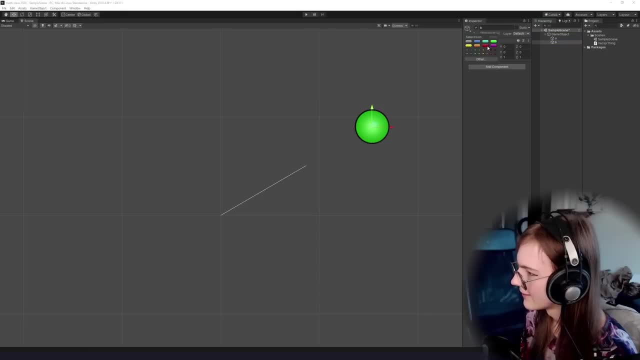 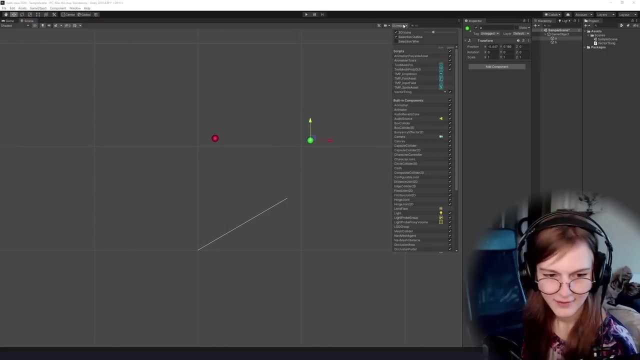 All right, Let's make A green, B red. Now we have two points, right? What a good pair of points. Okay, Let's say we want to know the distance between these two, right? First we need the actual points. 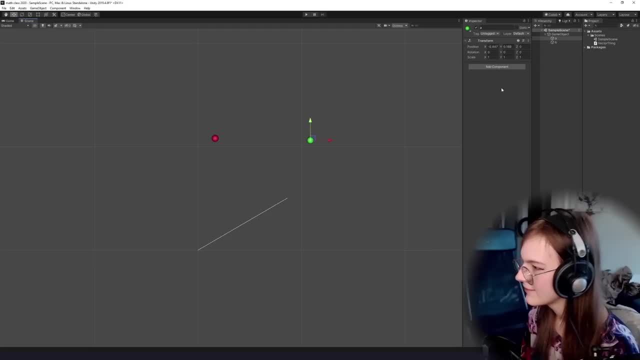 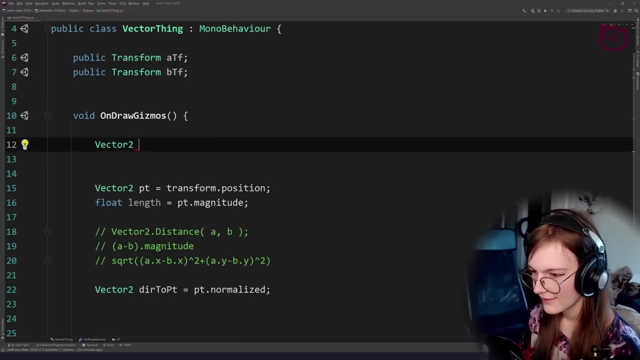 because we only have transforms here. So it would be. Oh, I need to probably assign them in the inspector. There we go. So now we have, Let's see, We just call them A. So that's going to be A transform dot position. 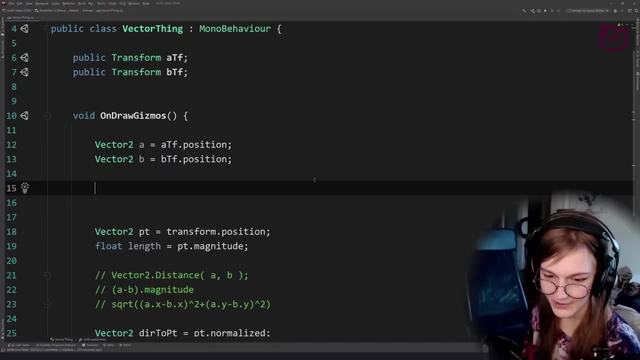 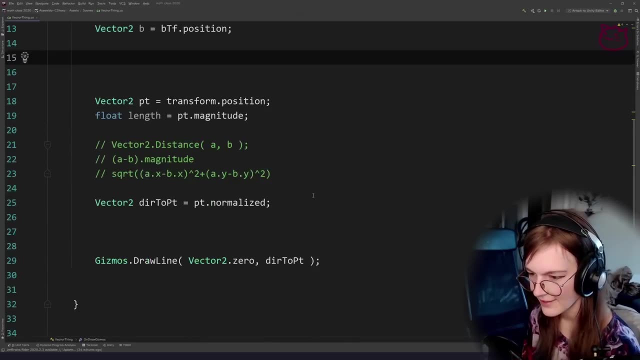 Then we do the same thing for B. So now we have the two points, A and B, And again we can draw lines. to make sure that this is working Right, I'm not using my library. Gizmos, Draw a line from A to B. 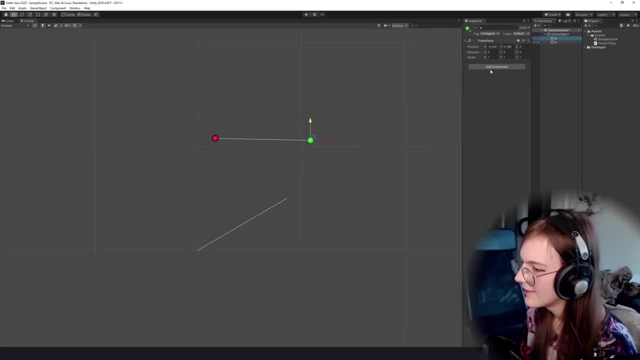 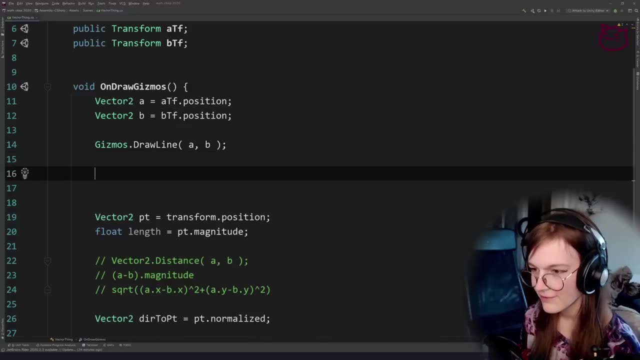 There we go, Cool. So now there should be a line between these two points So we can move them around And we now have: Yeah, What a good line, right, But we want to know the distance of that. So if we want to know the distance, 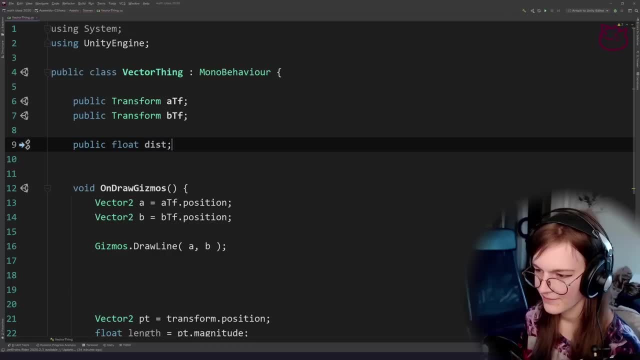 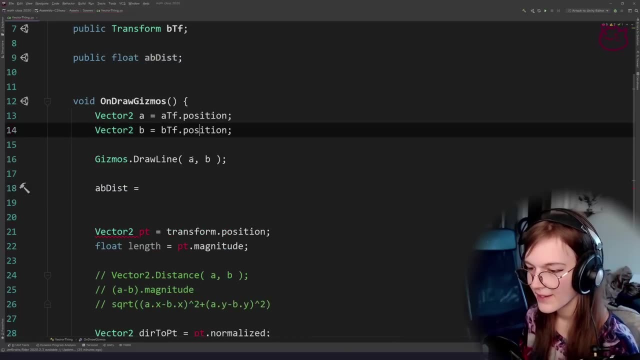 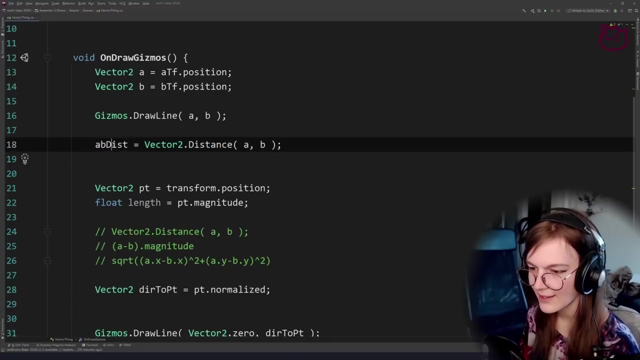 I guess we can print it in the inspector or something. So if we want to know the distance, then again we can use everything we typed here right. So we can do vector2.distance, And now we should set this value right here. 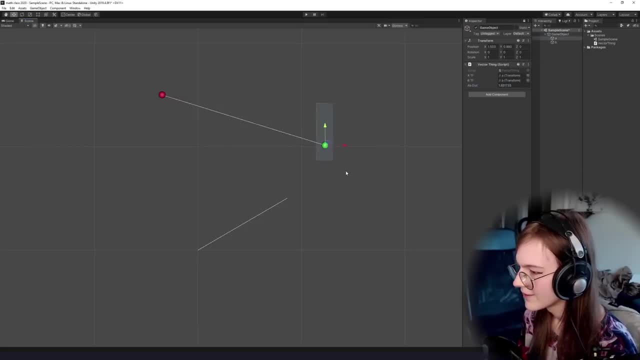 It might be hard to see it in the inspector, but there's a little value there. There's updating. Now it's 0.45.. Now it's 1.9 and so forth. So now we actually have the distance right there. 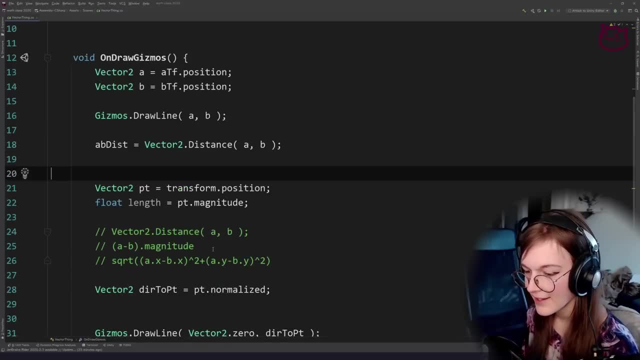 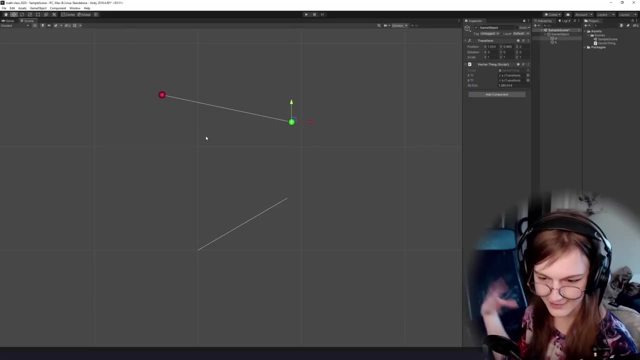 Yeah, So that's how you use it in practice. And again, the distance value is going to be exactly the same thing if we do A minus B dot magnitude, So we can compile this. It's going to work. And, yeah, still have the same distance. 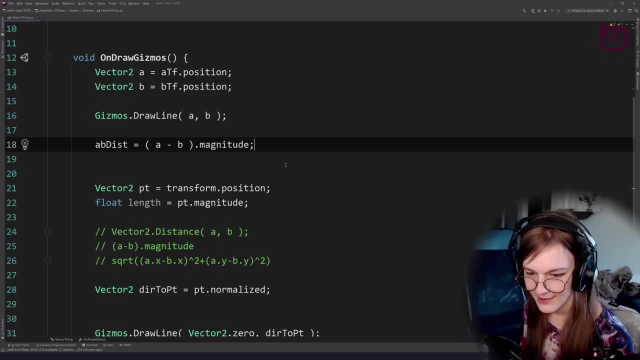 Any other questions before lunch? Any thoughts How to make a game like Angry Birds? I can't answer that. That's a very long question and a whole production pipeline. Start doing things. That's how you make games Generally speaking. no one's going to get mad at you. 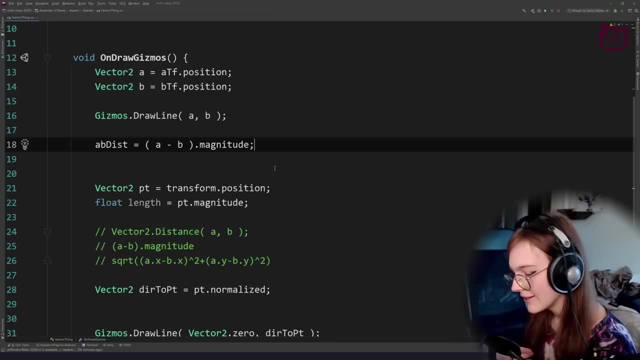 for doing A minus B dot magnitude instead of vector2.distance? I don't think so. I mean the first one might be slightly more esoteric because you sort of need to know the underlying math for that to be readable. But I think the- I mean most people should know about that. 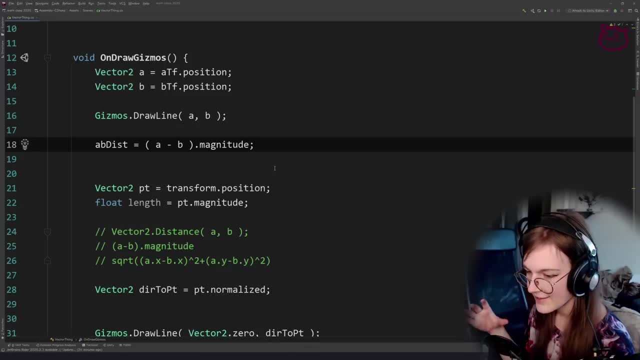 It's a very important concept, like vector2.distance. The nice thing about using that one is that you're being very explicit, that you literally want the distance between two points. If you use the A minus B dot magnitude, it's a little unclear like you get the length of the difference. 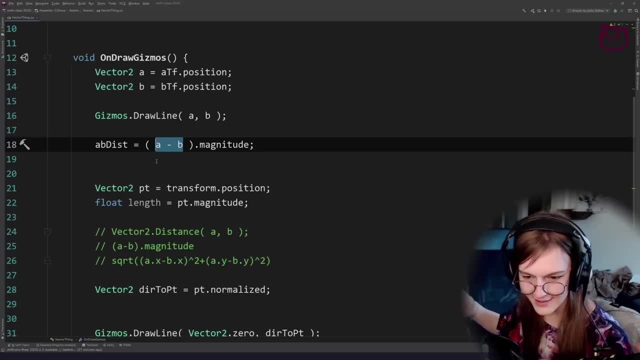 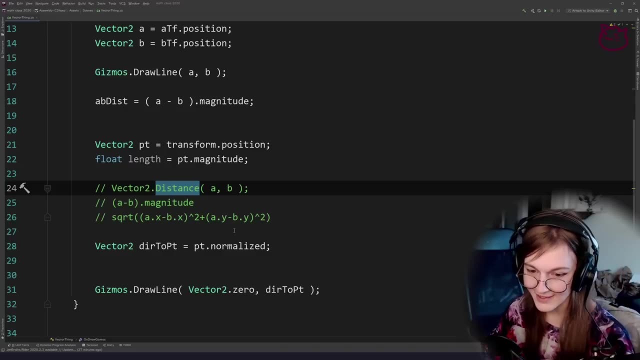 between these two, but, like, are we going to interpret it as a distance? Maybe these aren't points, maybe this is something else. So, you know, sometimes it's useful to use the one that literally says distance, because it's very clear that you kind of want a distance, right. 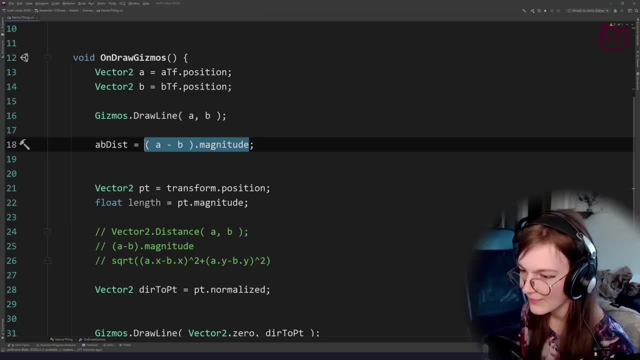 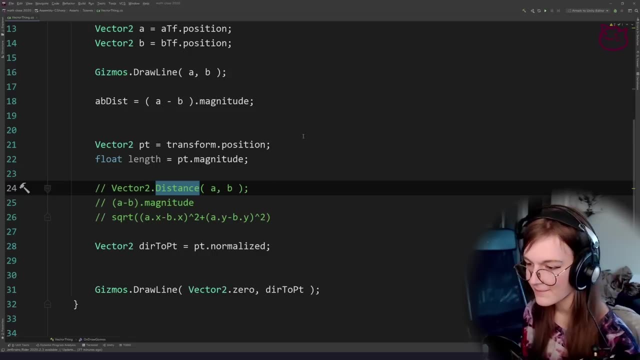 And, conversely, if you don't want, if you want to do the same math as this, but it's not a distance value, then using vector2.distance is likely going to be more confusing than useful Right. So it kind of depends on the context. 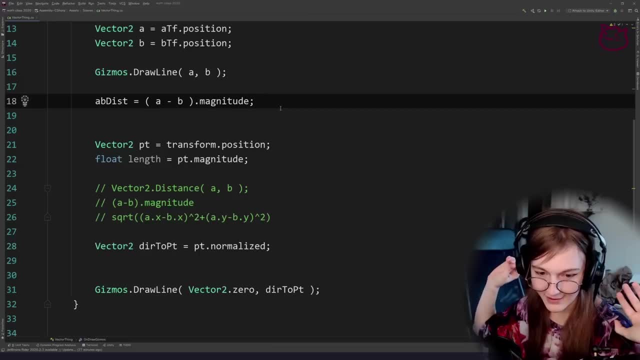 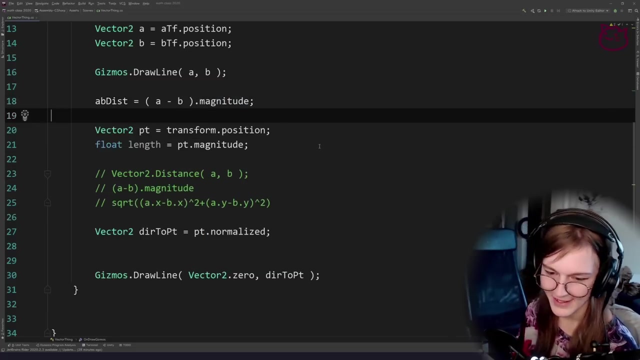 I personally really like doing like being explicit and clear with my code. Hugo, you're spoiling it. I haven't gotten to that yet. But yeah, actually, let's just. let's just, we can just talk about that, But that's the last thing before before lunch. 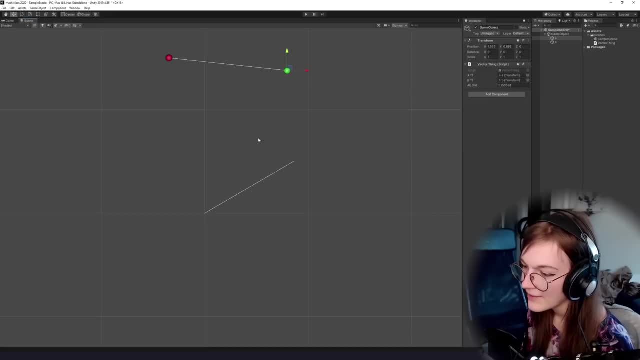 OK, so we talked about the. we have this line right here, right, The, the one that's pointing to the right, The one that's pointing in the direction of the. this transform, right. So what this one is. that is the normalized version of that point. 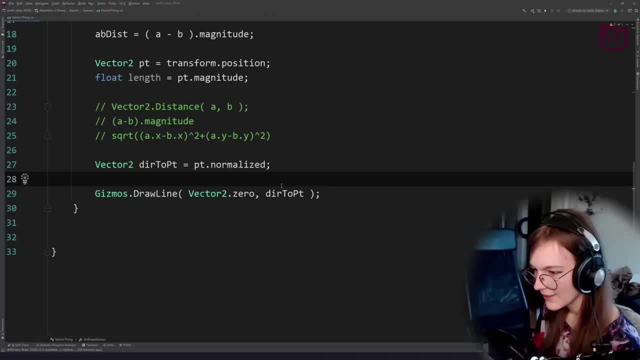 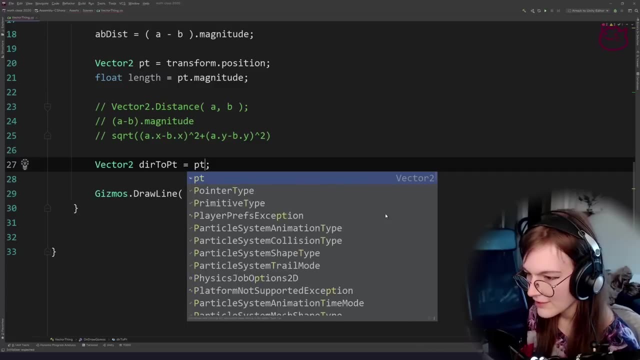 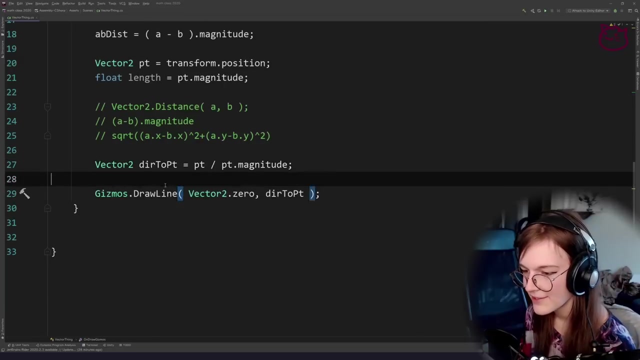 Like this is: this is the only thing we've done there. So so the way to calculate a normalized point. So instead of just doing dot normalized, we can do the point and then we divide it by the length of that point, right? So point dot magnitude. 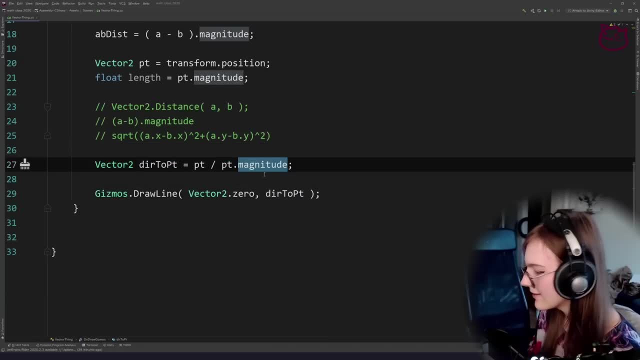 So this is how you normalize a vector. So by dividing it by the length, the, the length becomes one, right, Yeah, So so that's how you normalize a vector. I previously talked about the fact that there is a degenerate case where you're dividing by zero. 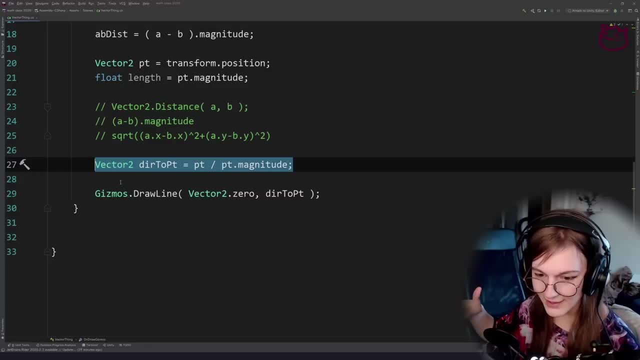 And if you look at this equation, you can probably tell what the what is what. the degenerate case is right, Because points dot magnitude can be zero. So what that means is that point Is at zero. So if you have a point that's at zero and your goal is that you want to get the direction that this point has from the origin, 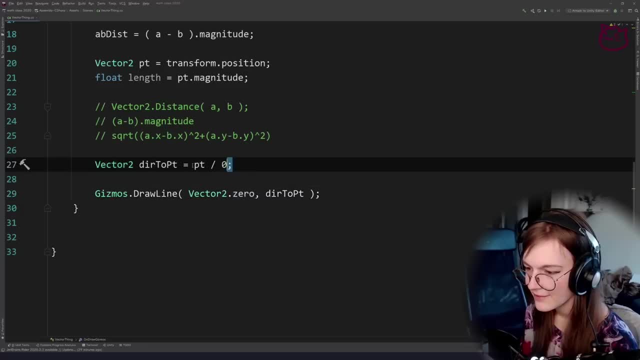 But if the magnitude is zero, then you're dividing by zero. So now again, math is telling you that something is messed up and you need to think about what you actually want to do here. So what this means is that you're trying to figure out a direction of a vector. 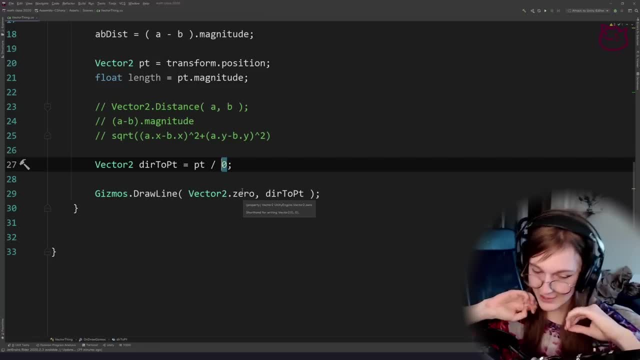 A vector that doesn't have a direction. It's zero. It doesn't point anywhere, right So? so usually in these cases you need to figure out: OK, what? what do I do to handle this special case If it's at zero? do we want to fall back to just using zero? 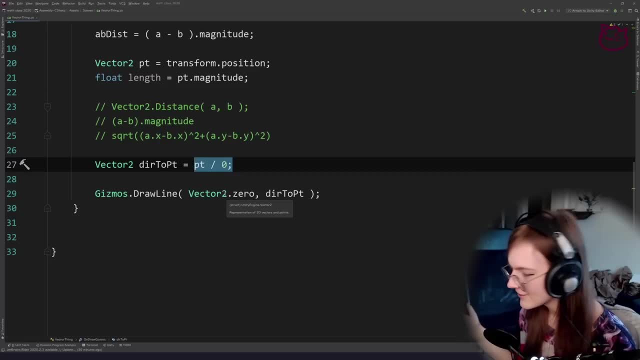 Do you want to check if the length is zero and then not draw it or not execute some piece of code? Usually it's. it's really like every time you see a division operator, It's really useful to think about if the denominator can ever be zero. 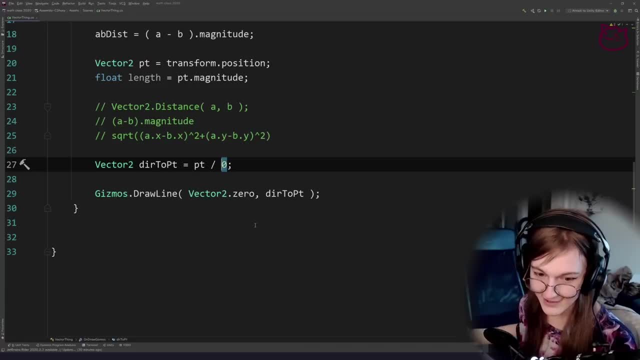 If it can, then that means that you have an interesting case to solve. Yeah, All right, I think that's it for lunch. Yeah, we're going to talk about the square magnitude stuff that you're talking about in the like after the break. 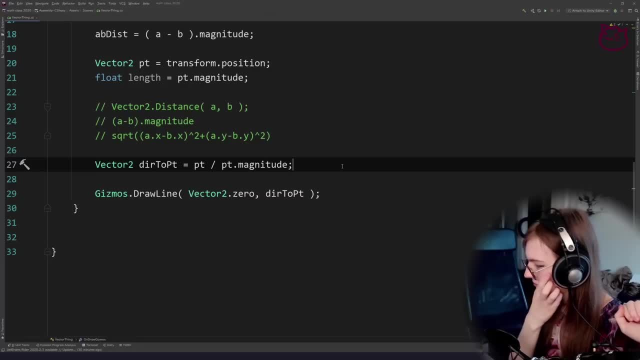 And yes, doing square magnitude is faster. Yes, I think there are some intricacies of like the property call itself Has some weird overhead, But if you manually do the square magnitude it's like way faster than actually doing magnitude. So I've heard 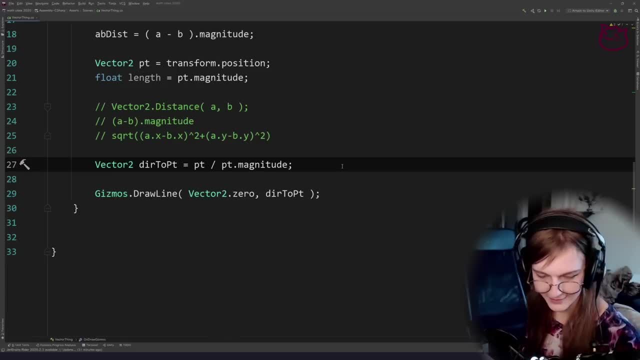 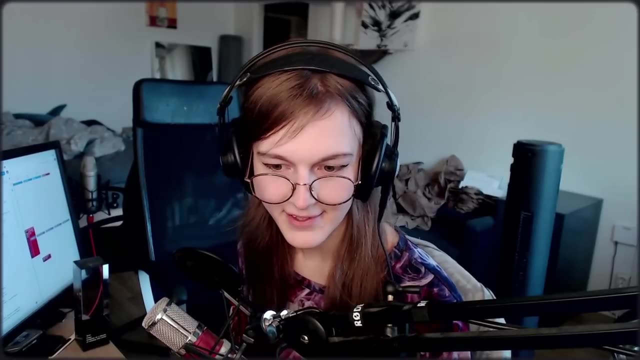 But that's not for mathematical reasons, That's for silly overhead reasons. Actually, we should do a, we should do a lunch break. I'm just there's no audio in the lunch break room, So so, yeah, I'm just going to place an image here. 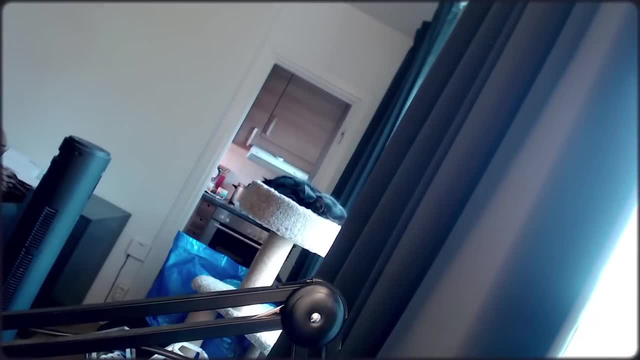 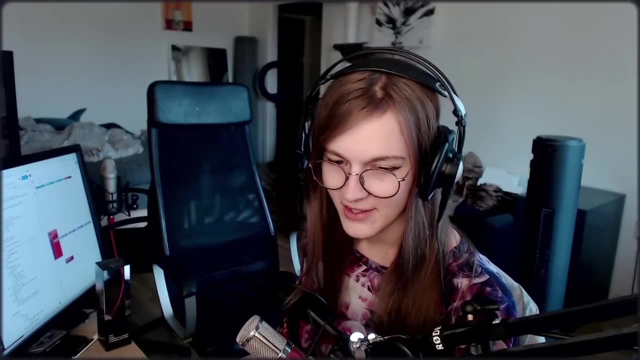 See you soon, See you after lunch. Look at that little boy sleeping in the goblet. He's a peaceful little cat. Now where were we? Oh, we just covered how to actually normalize vectors, how to do that right. 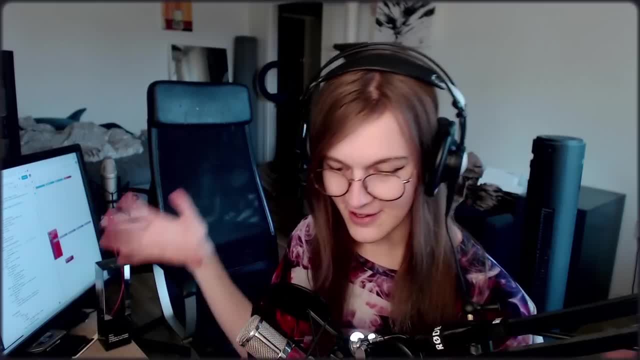 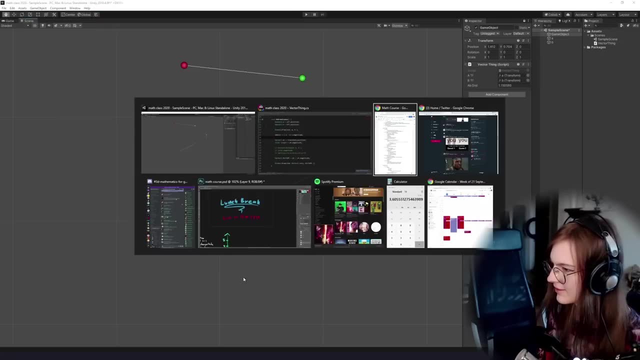 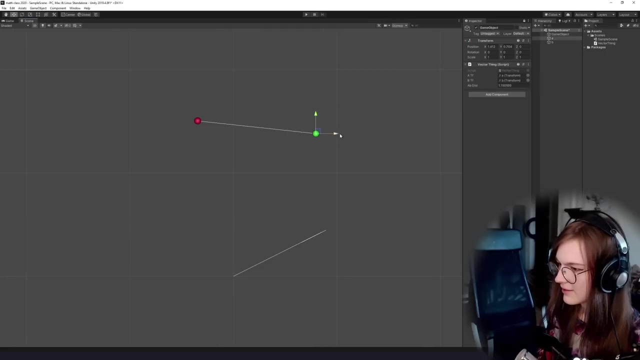 Not not just in terms of what it is, how to do it using Unity's helper, but how to actually do it yourself, right? Okay, what's the state of things? So we have our code and we were just showing Directions, right? 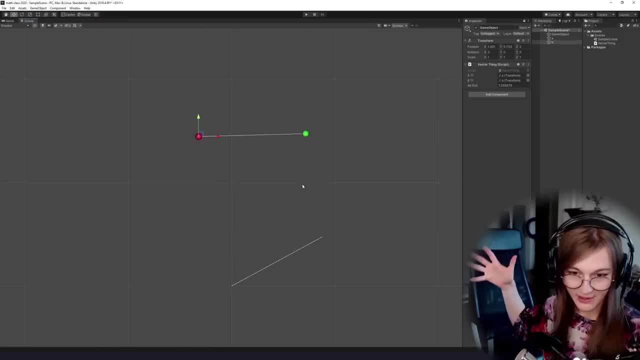 Okay, All right. So so here's: here's a short little exercise that we can think about together. So so, for instance, now we have these two points right Previously, when we looked at direction here, this is the direction of the point itself in world space, right. 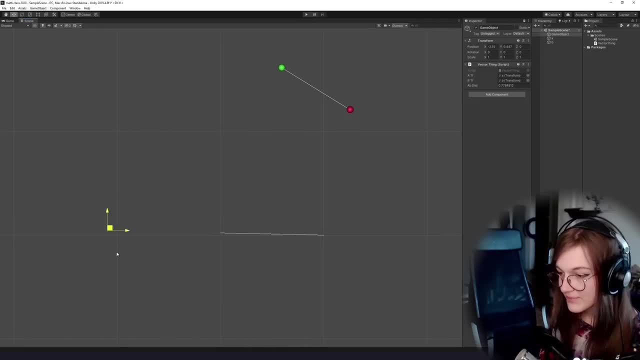 Like this one is. it's just a line drawn from zero in the world and then out to one distance away from the center, in the direction of This point that we move around, right, So, But yeah, so so let's say we wanted to draw the direction between these two points. 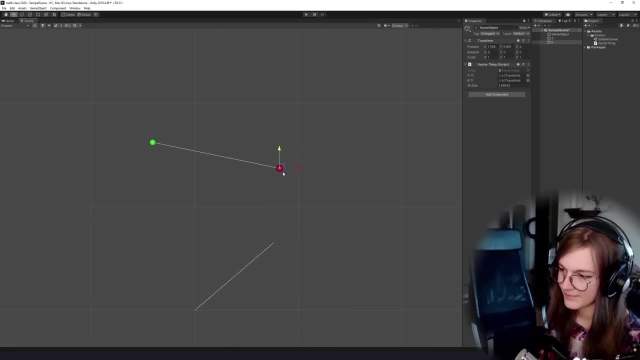 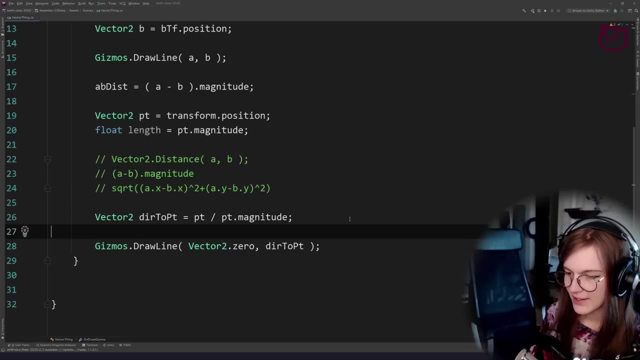 Let's say you want to do direction from from A to B. So so let's do that. Let's just figure out how to do that, right. So We're going to ignore the center point, so let's just hide this. 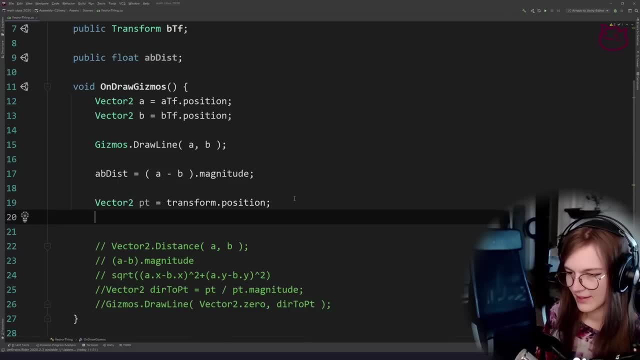 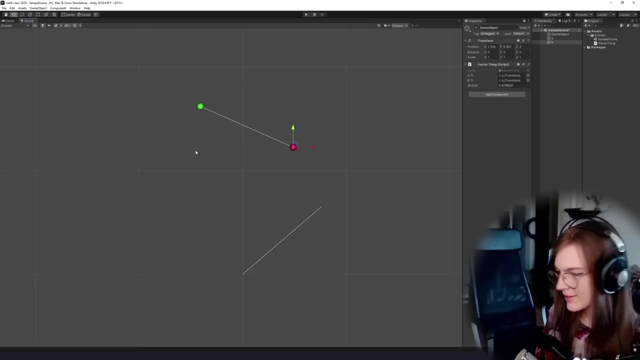 Let's forget all about this. Let's let's forget about this too. Forget about everything. You have learned, nothing so far. Okay, so now we are drawing a line between A and B, right? So I should just keep this line. 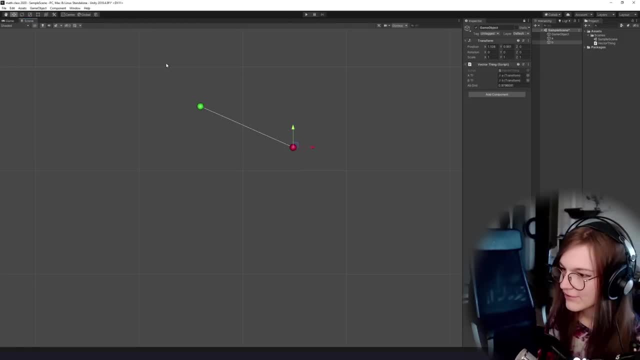 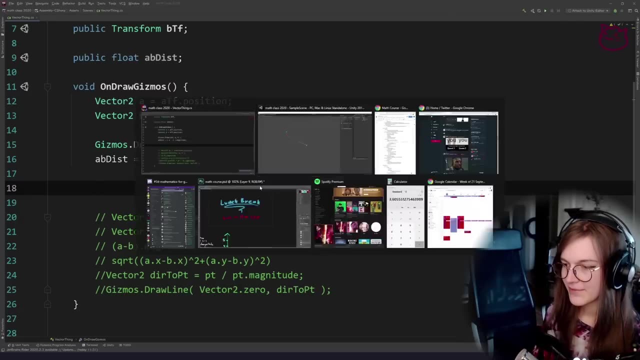 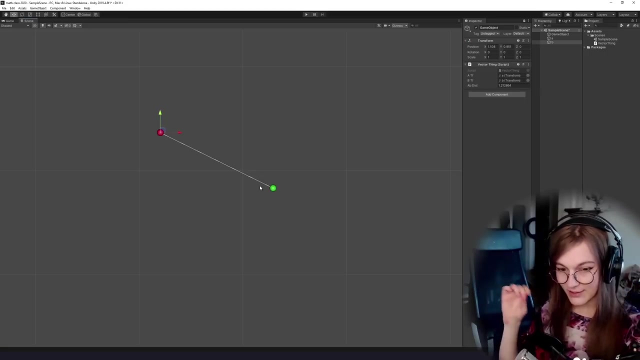 And so now the goal is that we want the direction from a, the green points to be the red points. So so we want that arrow right. So so how do we get a direction between Two points? Well, the first thing we need to do is to get the difference between these two points right. 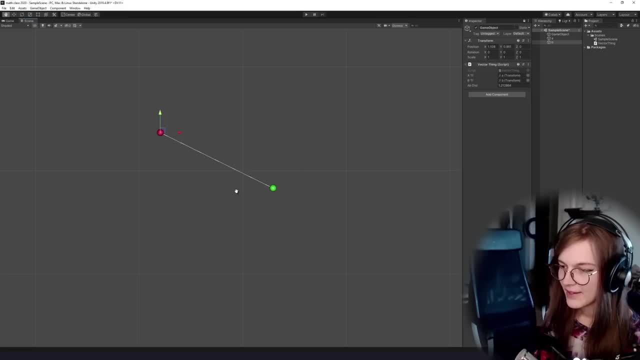 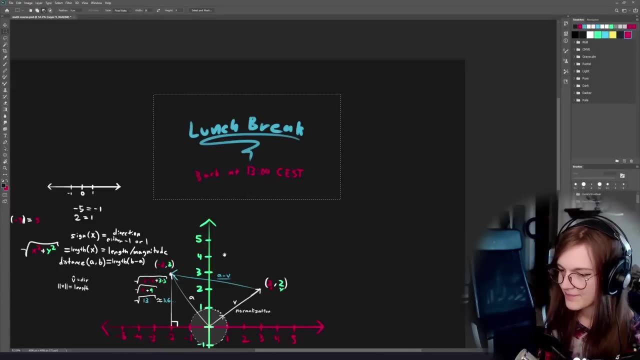 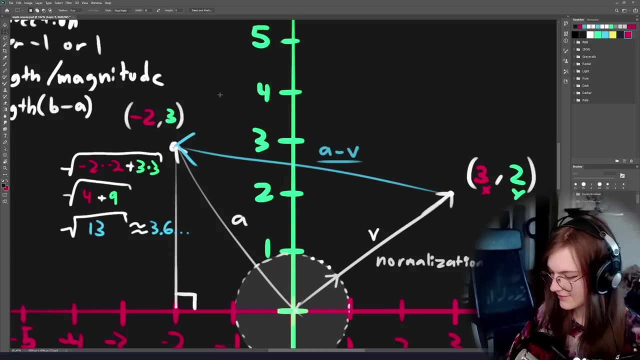 So if we take one point and subtract it by the other, we get the vector going from one to the other, right. So that's something we talked about earlier. Like the, we have the two points here, both of these. Sorry, my desk layout is not in tablet mode, so we have this points and we have this points, and then we want to. 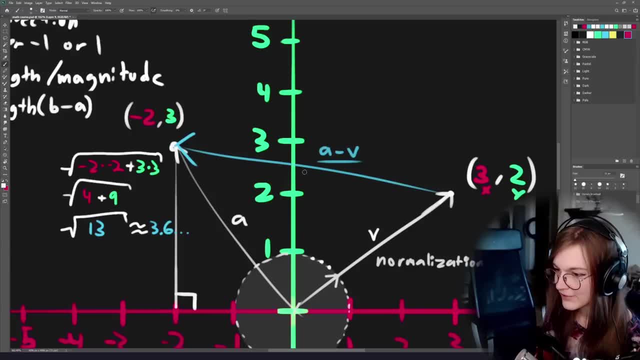 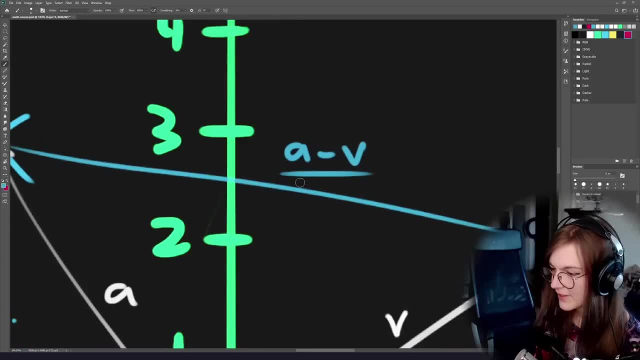 Get the direction between these two points. but first, in order to get the direction, we need this blue vector right here, right, So all we need to do is subtract one from the other. The order in which we do the subtraction will change the direction that the arrow is pointing right. 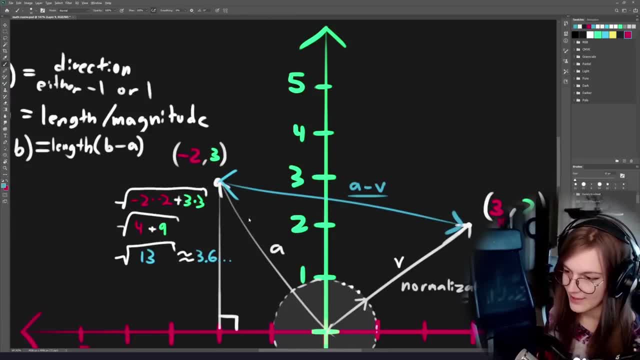 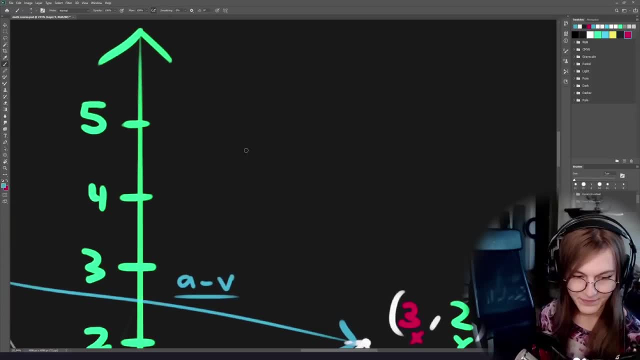 So usually you can go either way, depending on how you do the subtraction. So so generally it's kind of annoying that if you have, if you have two points, like You have A and you have B, and you want to get the direction from A to B, 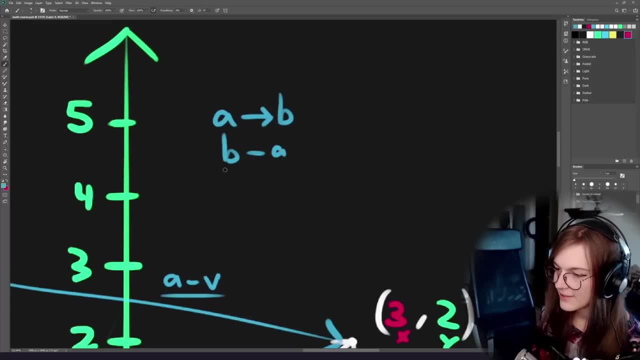 The way you do that is B minus A, and it's kind of annoying that this is the order that you do it, because it feels like you kind of want to have the A first. But I kind of just have this mental model of you always have to like flip them if you want to get from A to B. 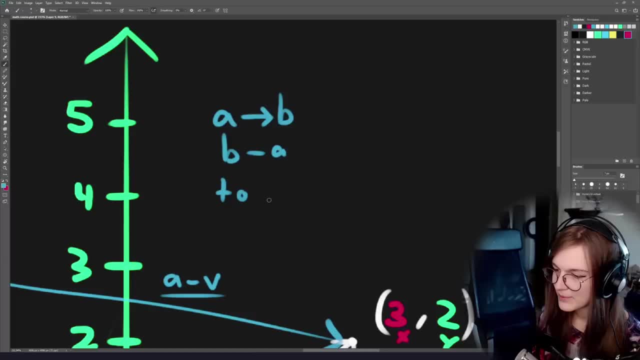 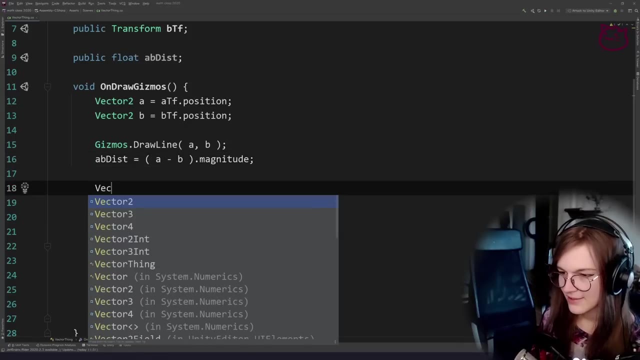 So yeah, so it's always like the: the two points minus the front point. So then, from this to this, in terms of like direction, Okay, so that's all we need to do to get that vector right. So let's, let's do that vector. So that's going to be called A to B. 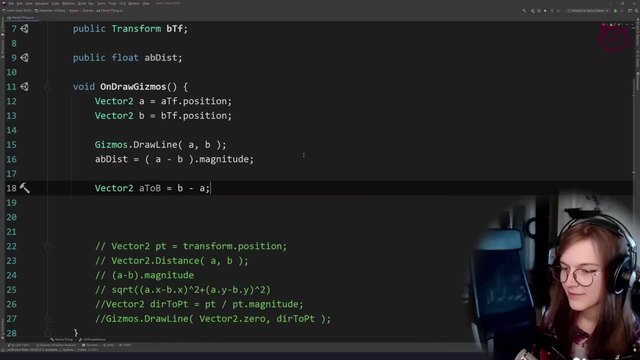 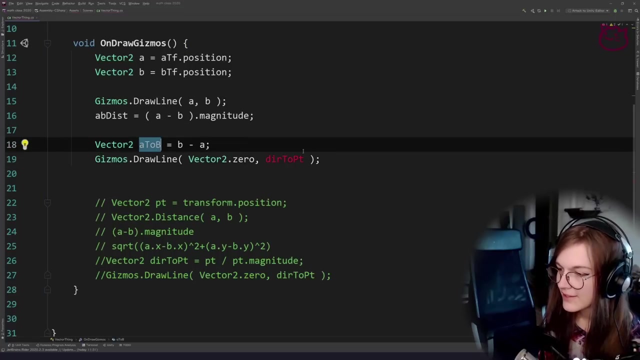 And That's going to be B minus A. So now we have the vector going from A to B, right, All right. so now that we have that vector, what happens if we draw that one? Well, we can try it out, right, Draw it from zero to that vector. So now we're just going to visualize the raw vector, right? 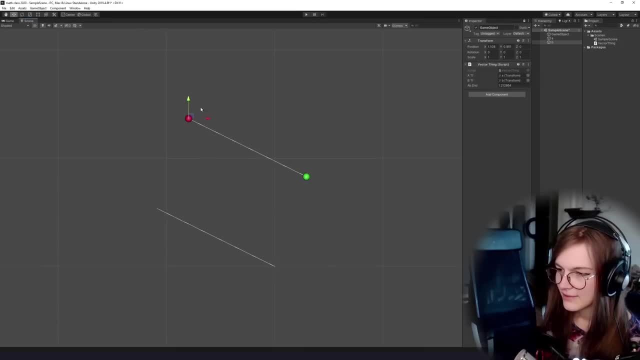 So if we do that, It's now going to draw at the origin right, Because the vector itself doesn't have a root of the arrow right, So it doesn't really care about the location where we did this calculation, but it is getting the correct vector. 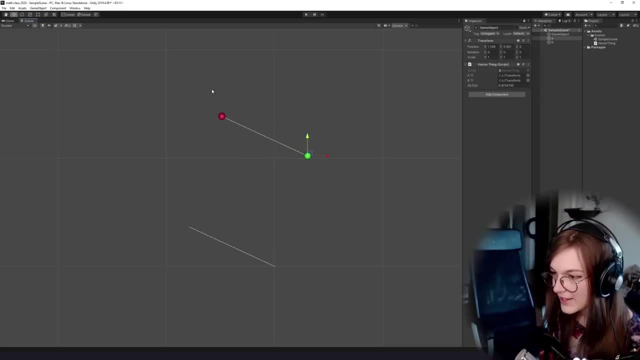 Like. this is the vector going from- From A to B- right. So what we need to do now is that we just need the direction right. So we don't want the actual full vector, We want this have a length of 1. So if we want a direction vector, we need to normalize this right. 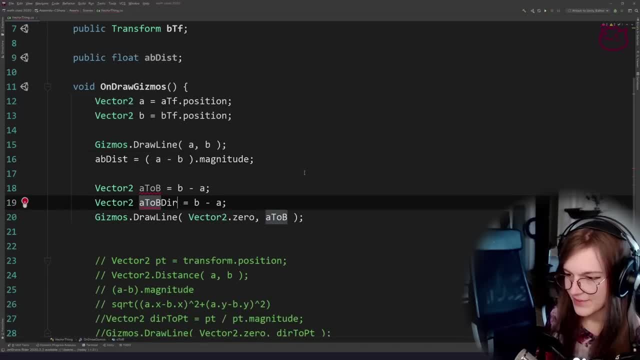 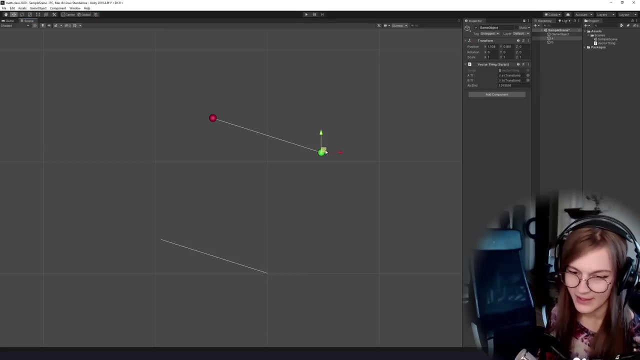 So well, let's make the direction so A to B direction, So then we can do A to B Dot normalized, And then we can draw the direction So num disp X, And now this one is always going to have a length of one, So it doesn't matter how far apart they are, but we do have the direction right. 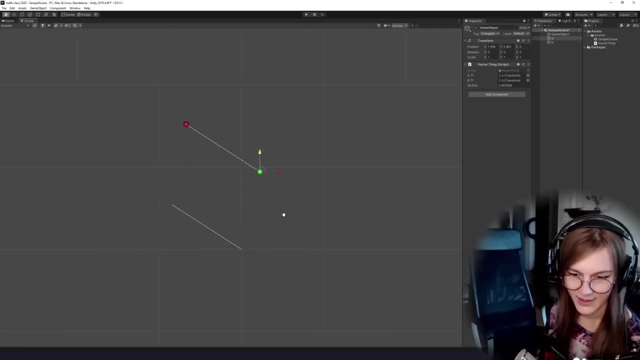 We can move either of these points and the direction is still going to be correct. Okay, so far, so good. But now we probably want to draw this one at the correct location, because it's kind of confusing that it's down here Like the direction is correct, but the visualization of this vector is kind of offset. 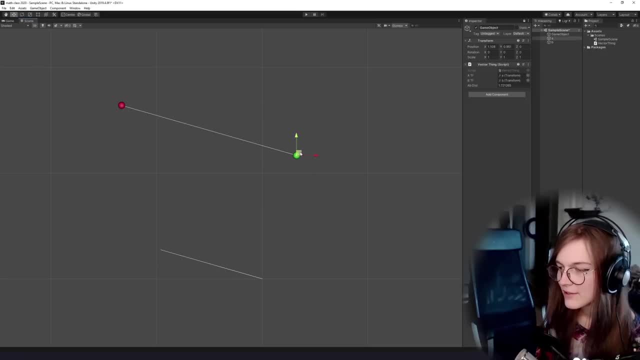 We kind of want to see it here, right, Like we want to see it go from the green point to the red point. Okay, so we need to move this vector. We also need to hide this line, because that line is going to be covering up a bunch of 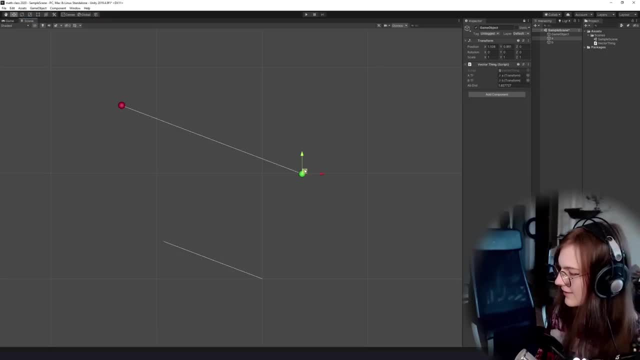 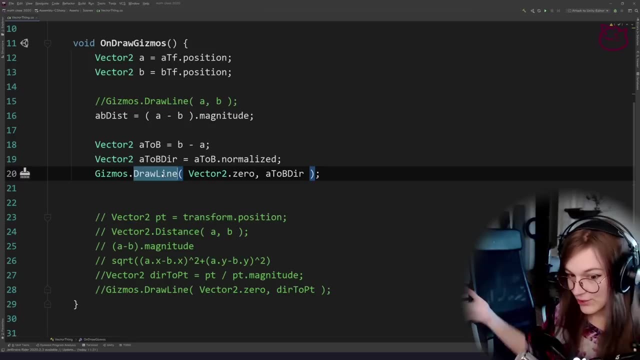 stuff that we want to see. So let's first hide that line And then we want to move this vector. So drawLine is: you supply two points in it, right, And the first point is A, because we want to originate this line from A. 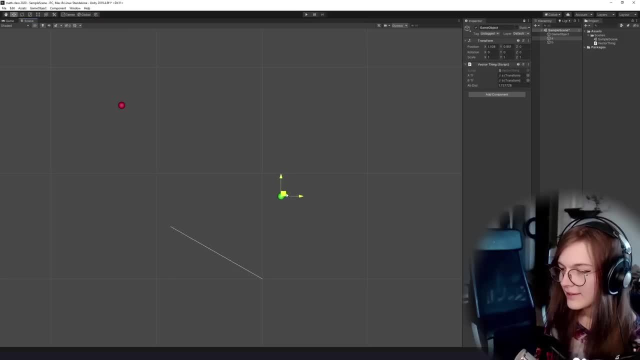 So we can just pass the point A into that one, And then, in order to make this be relative to A, all we have to do is add A, because then we're going to move it up by this vector, going from zero to A right. 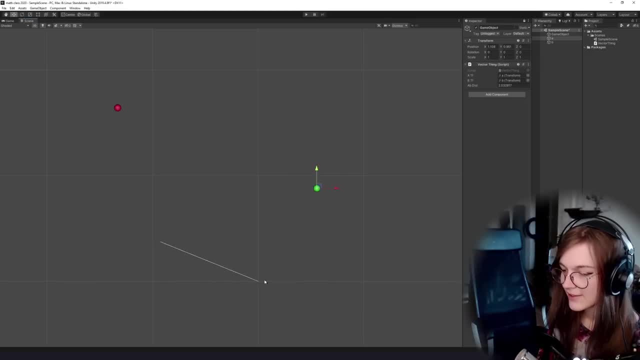 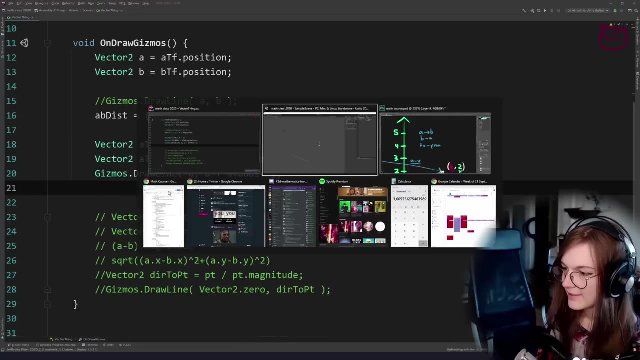 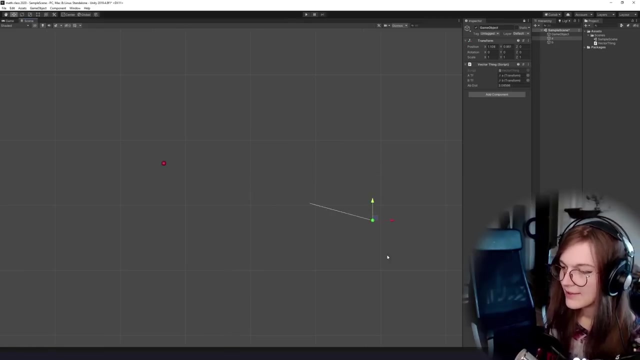 Because that's what A is. The coordinate of A is a vector going from zero to A, So then we can do A plus that direction And then we recompile. It's now going to point toward the red point right, And so now you can start to draw. 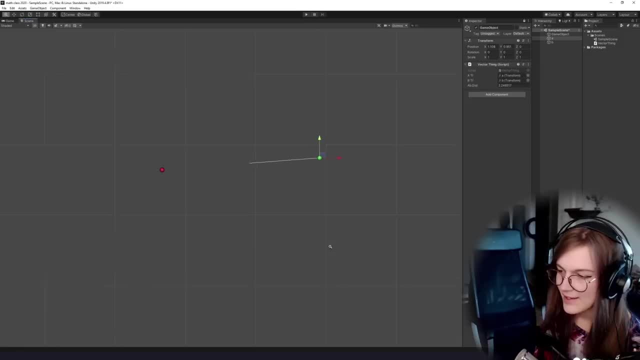 Okay, So now you can start to see like you can imagine these being units in a game, right? And you need to point toward some target or whatever And you need that direction somehow. Then this is a way you can do that, right. 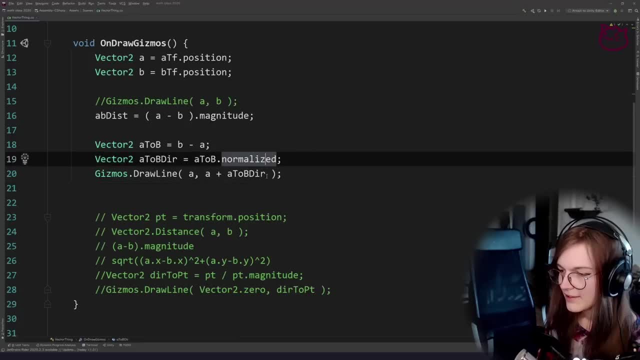 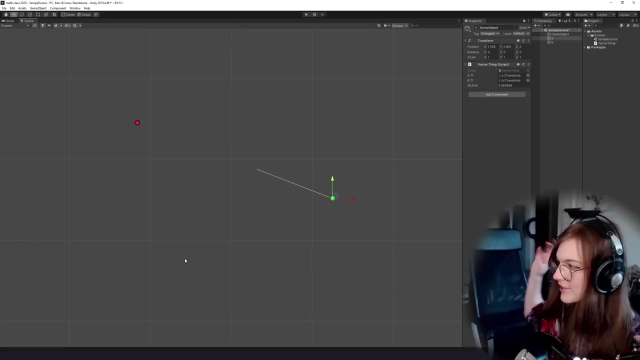 Yeah, Although this part is only for drawing purposes, You already have the direction here. The only reason we had to do the A and A plus the direction is to draw it at that location. right, But the direction itself is already done. So, in terms of directions, in terms of interpretation, directions should not be like they don't. 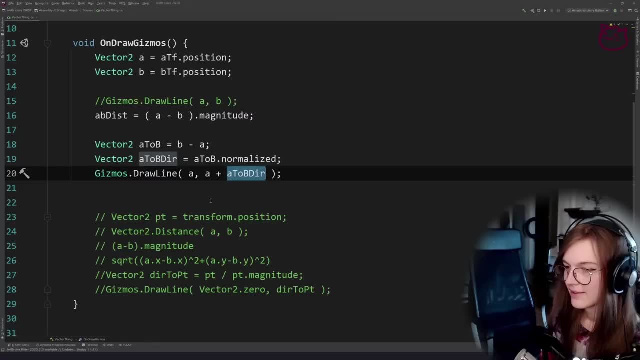 really have a position. It's just a direction, right, Yeah, Okay, Did that make sense so far? If it didn't have A plus, it would point to the location based on zero. Yeah, If this is just zero or the sorry, a zero vector. oh, it didn't. it was sad about that. 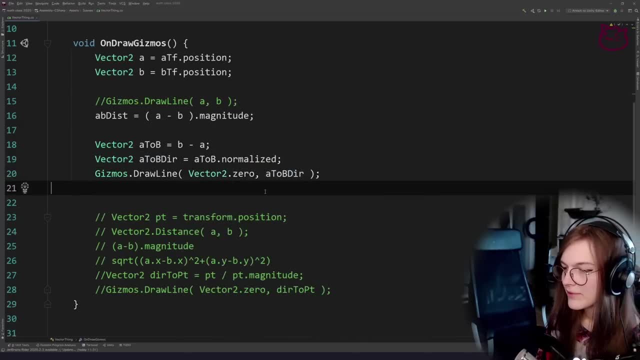 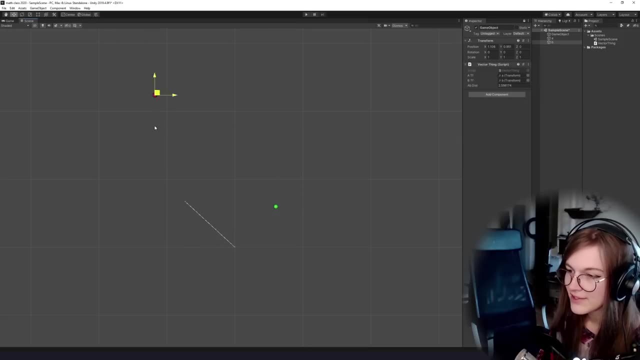 If we just set this to vector two dot zero, We remove that one, Then it's going to be positioned at the origin, But it's going to have the correct direction, right. So the direction is correct here. Yeah, So kind of usually the you only need this direction. 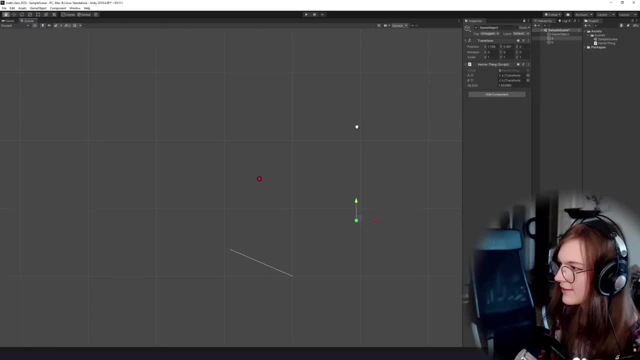 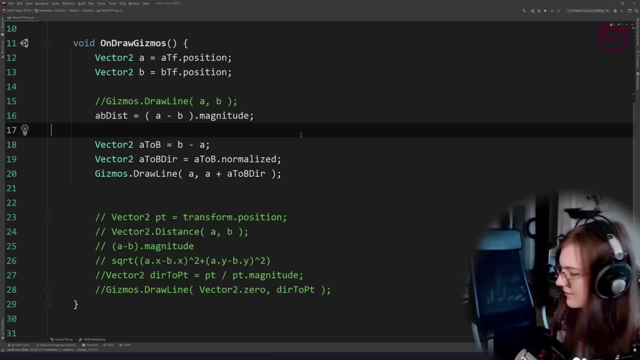 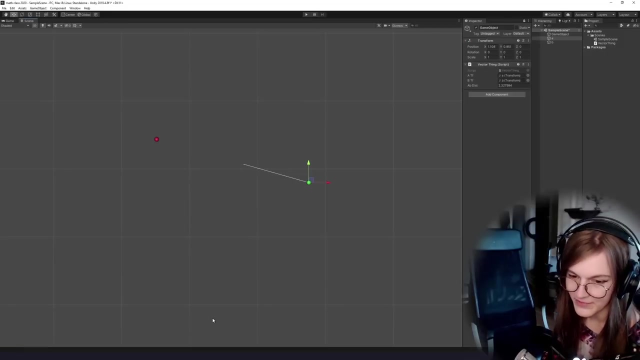 Usually you don't have to move it there. We're only doing that for visualizing what's going on. Okay, Cool, Cool, Okay. Why are you doing A plus? Because we want to draw at that location, right? So if we don't do A plus, it's going to draw the vector going from zero in the origin of. 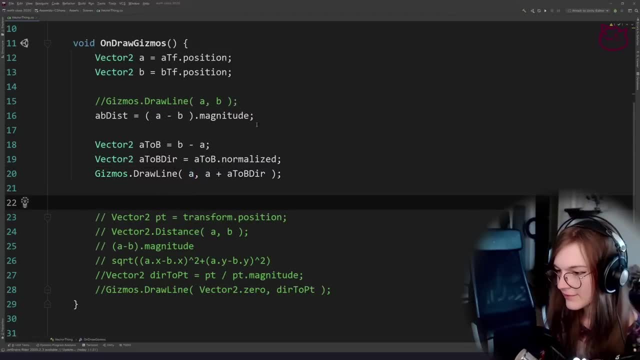 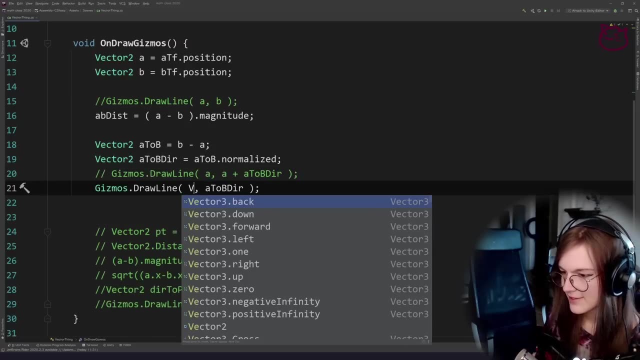 the world to the direction that the vector is pointing, right. But in our case we want to draw it at the location where it's relevant, right. So again, if we just do this, vector three dot zero Recompile. 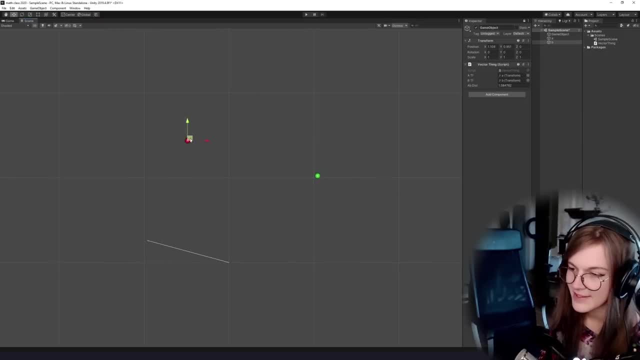 So now it's going to be at the origin of the world, just at zero. So now we're kind of showing the raw data of this vector But in terms of like visualizing it, it's kind of like annoying that it's at the origin. 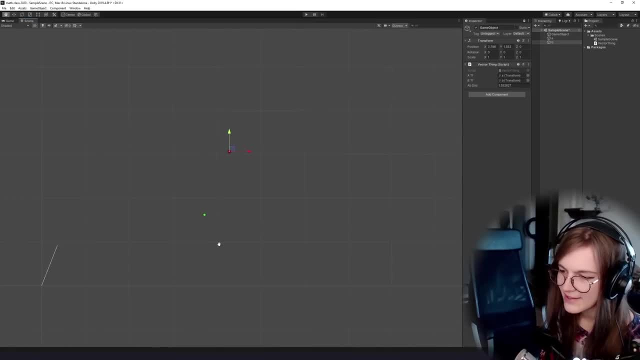 because if these things are very far away, then we don't even see the origin, even though the direction here is correct. This is the direction going from A to B, right. So the direction is correct, but just visualizing it. we need to supply two points to draw it. 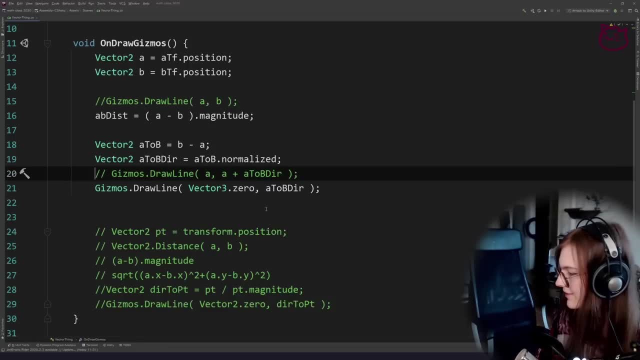 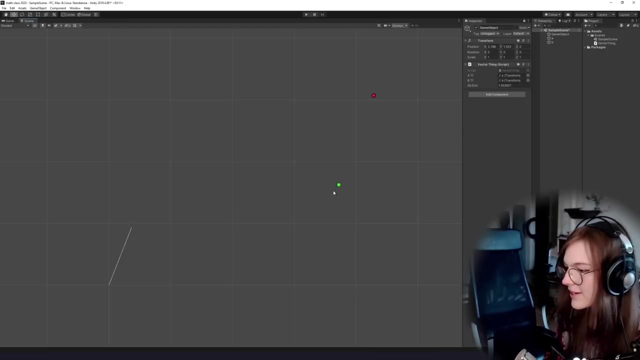 right When we're using draw line. So yeah, Oh yeah, there is also a draw ray one if you want to use it, although I tend to not use that one. So the A here is just to offset everything, so that it's positioned here instead, right? 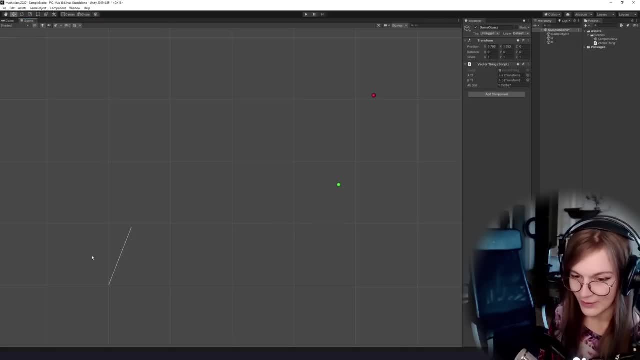 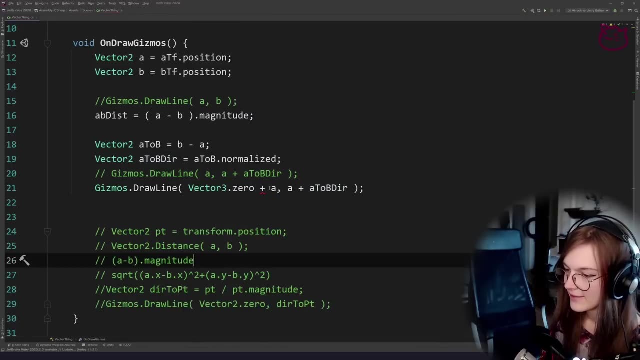 So yeah, So all we need to do to make this one positioned at A is that we add A, So zero plus A and A plus A to B direction, And this is unnecessary. So we can just remove that, And then we have A to A plus A to B direction. 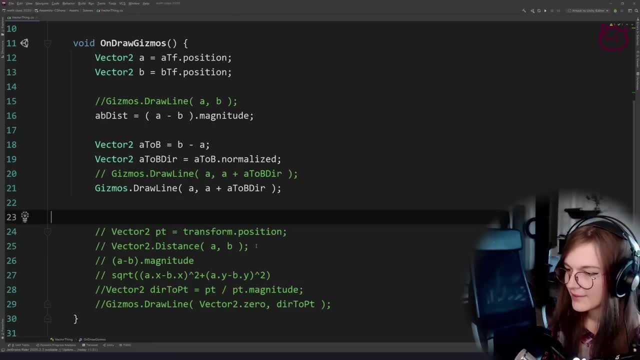 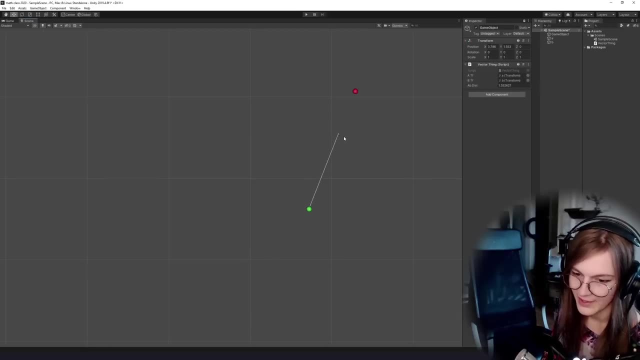 And then we get the two points right. So what A plus A to B direction is is the point here. It's the end of this line right here. So that's what the second point is, And this is where the first point is. 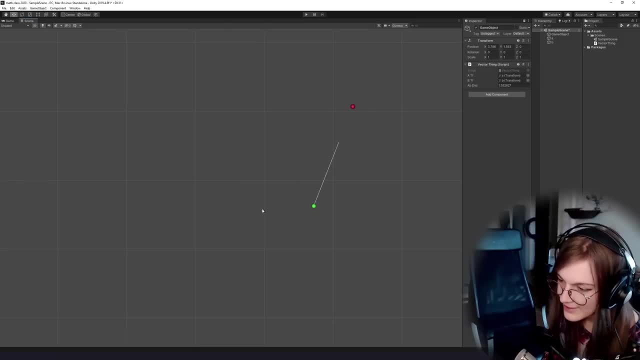 So what this gives us is this point, which again goes from the origin all the way out to this tip, Depending on if we want to interpret it as a vector or as a point. we can visualize it in different ways, right, But that's what that returns. 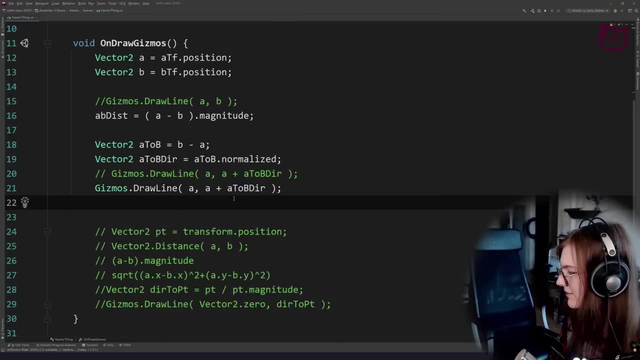 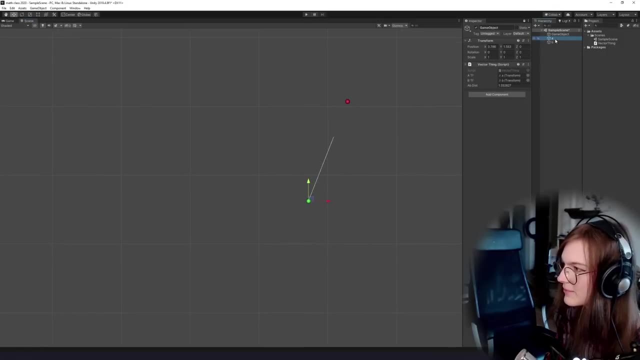 It gives us that point right there. What happens if we do draw line A A to B direction? I mean, it's just going to be confusing. There's no interpretation that makes it useful sort of Yeah, So there's not really much point of doing that. 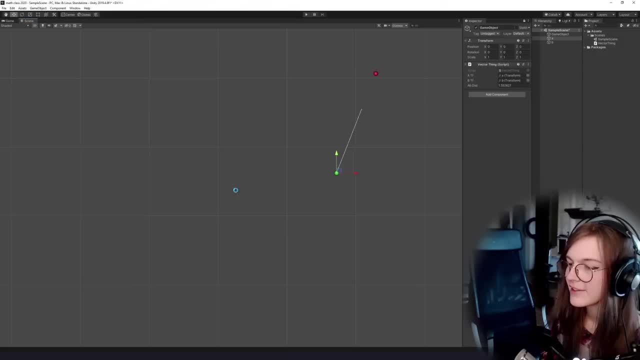 Although it is very common to sometimes forget to do things correctly. So sometimes you will see issues like this. Yeah, You're kind of just confused about what's happening, right? Because this doesn't look like a direction at all. This does not have a length of one, right? 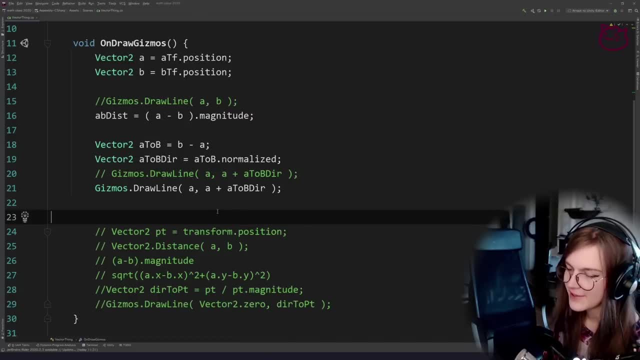 Yeah, Because then what we're doing is essentially: this point is originating at the correct location, but this one would still be if we didn't have A plus. it would still draw the end point at the origin. So we need to move both the origin of the line and the end point of the line. 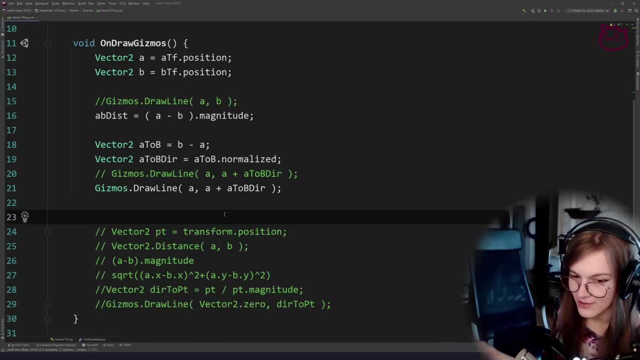 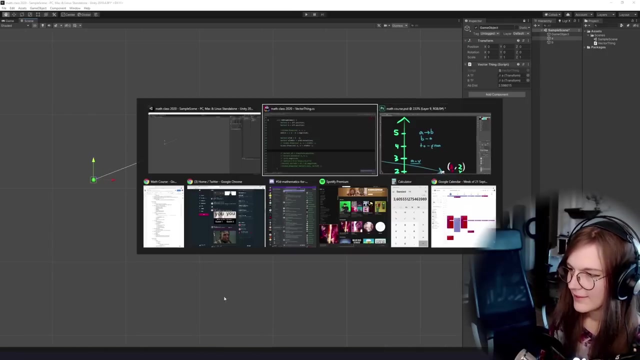 Yeah By A right, So that it's relative to A Yeah. you're offsetting both end points, or the starting point and the end point, with A All right. So now we have a way of getting the direction between these two right. 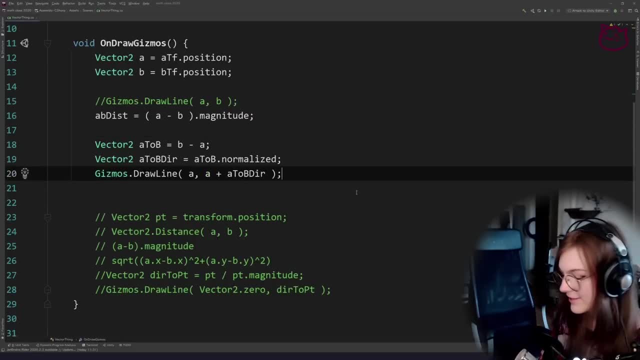 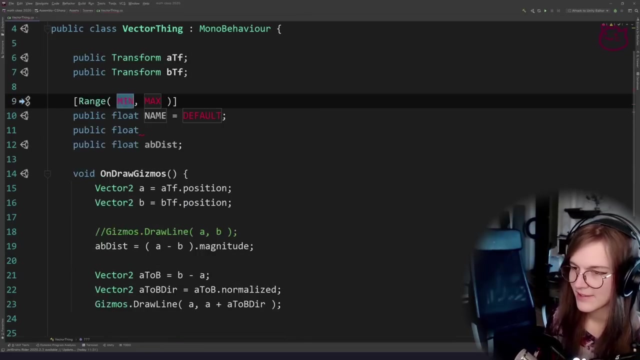 Let's see There have been a few more things we talked about. So one of the more useful things about directions is that we can very explicitly position things a fixed distance along that line. That is very easy. Let's do the right. So let's say: you have some float value. let's make it a range actually from zero to four. 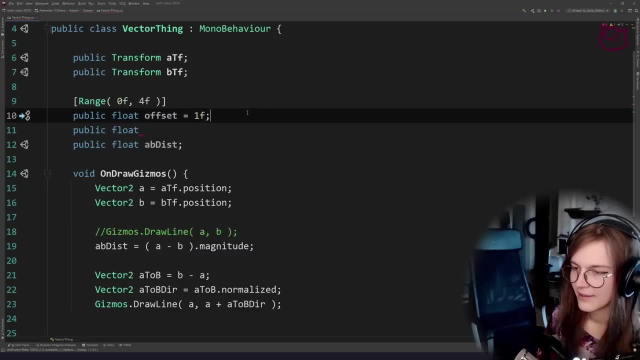 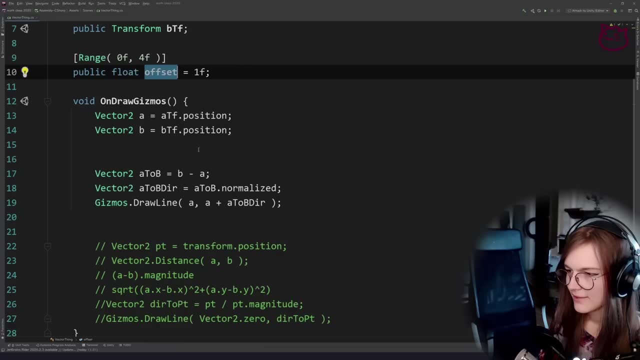 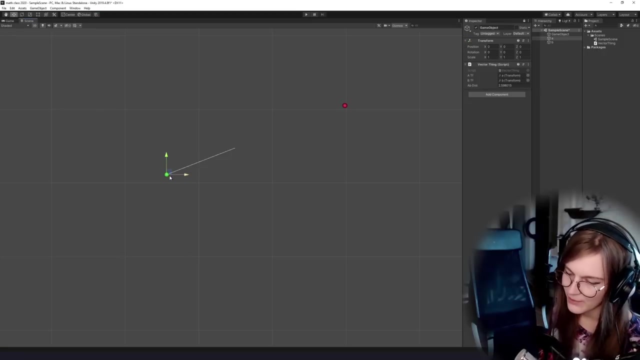 Let's call it offset, It's fine, All right. So now we have a value called offset, Don't need AB distance anymore. All right, Okay. So let's say we want to draw a point between these two points. We want to draw it along the line that goes here, right? 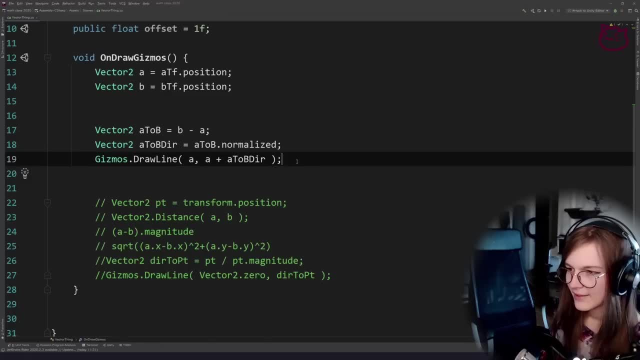 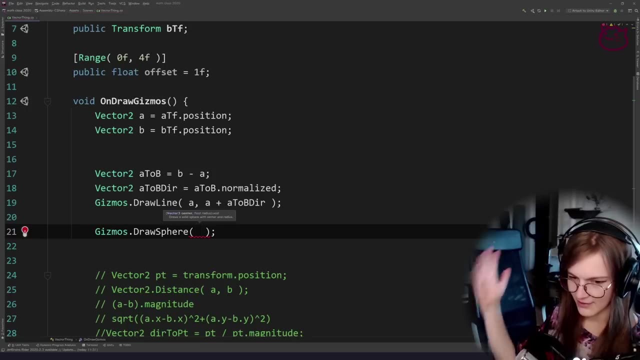 And we want to set the distance away from the player. So now we're going to call that offset And we can do gizmosdrawSphere, So just drawing a little point. So we want to draw that one at the location. So just to make sure that this works, we can try. 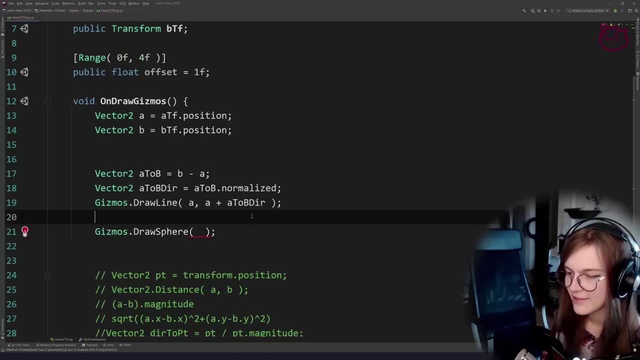 Let's draw at the middle. Okay, So we want to draw a midpoint between these two. So if you want to get the midpoint or the average of two points, as you would do with any other numbers, you do the same thing with vectors. 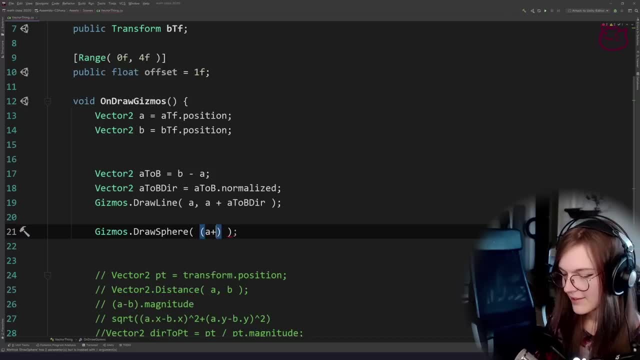 You add them together and then you divide by the number of entries you have. So A plus B divided by two gives you the average point of these two coordinates. right, All right. So then we also need a radius. You can just make something pretty small. 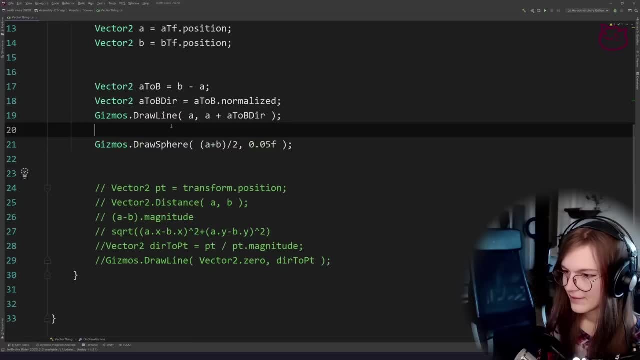 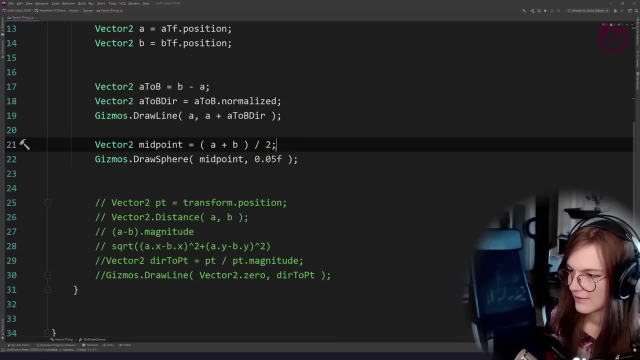 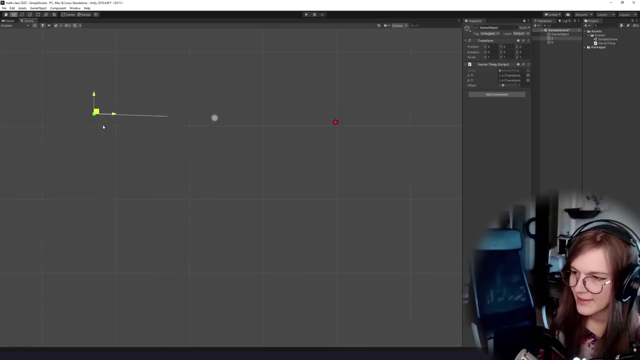 Actually, that's being a bit more explicit. So midpoint equals that, There we go. So now we want to draw a sphere at the midpoint between these two points. All right, So we got this gray little sphere- And it is right- between these two points. 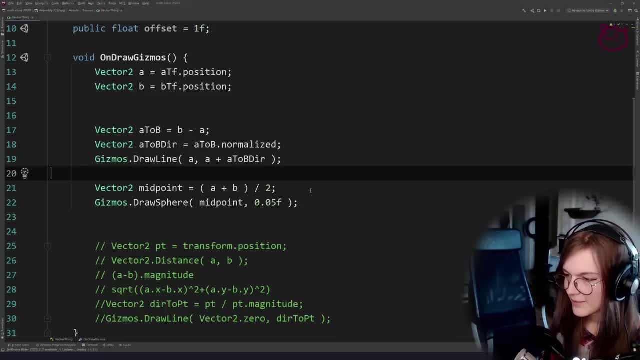 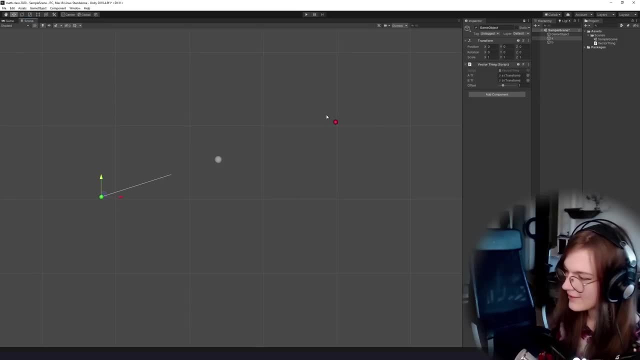 Okay. So now we got this thing that we can draw, But we don't want to draw it at the midpoint, So we want to draw it a fixed distance from the starting point towards the center of the sphere, And then we want to draw it at the end point. 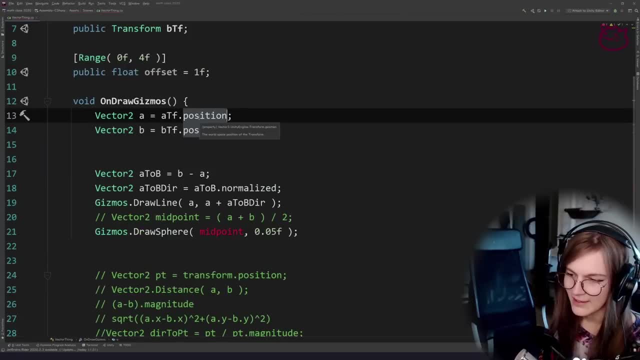 So if we want to do that, like I mentioned before, the fact that this direction is normalized means that if we multiply it by some value, we know that the length of the resulting vector is going to be that value. That's not true if it's not normalized. 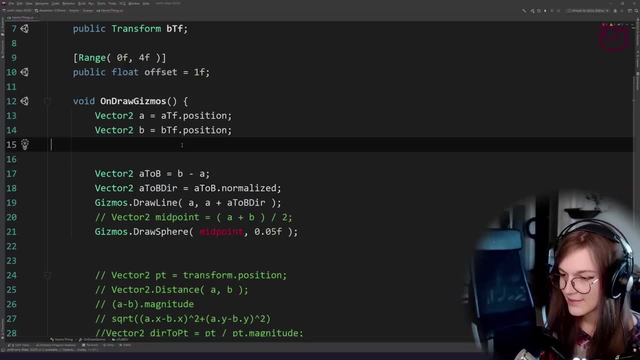 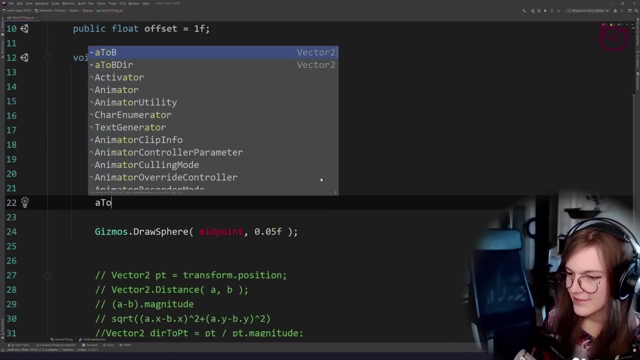 So this is kind of the really really powerful things about direction vectors or unit vectors, normalized vectors: Same thing, It's the same word. Wait, Different words, same concept. So we have the direction here And then we want to get a point along that right. 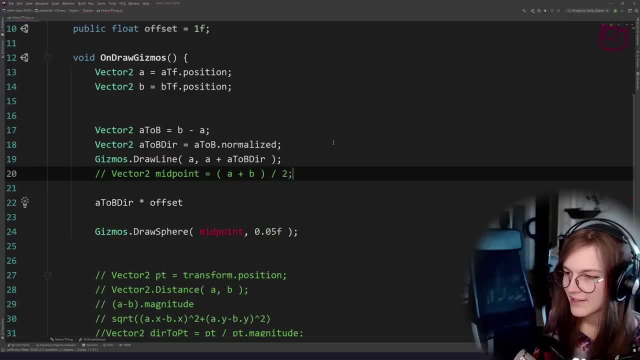 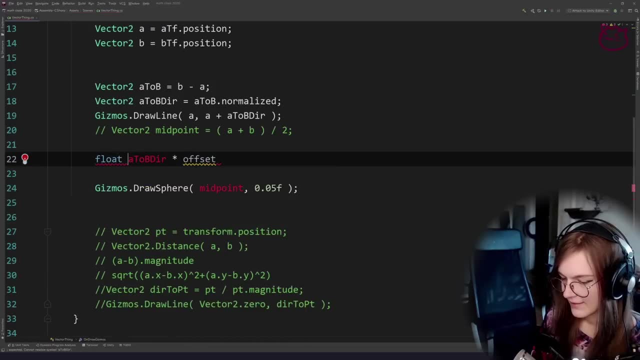 So we can do A to B direction. multiply that by our offset. So offset is the parameter that we can tweak for the distance along this line. So let's call it offset vector. So now There we go. Sorry. So now we have the vector that is the offset that is going to move from this one toward. 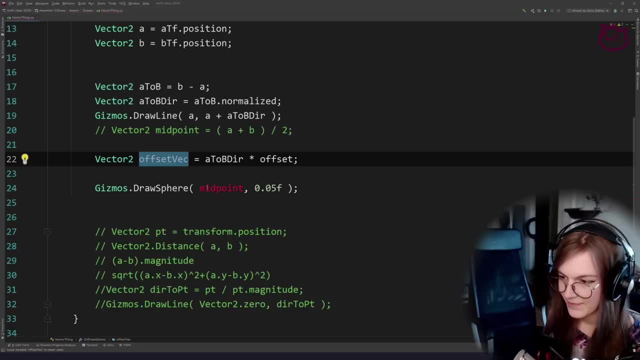 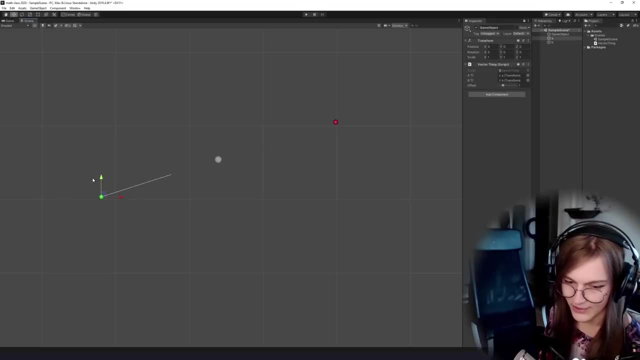 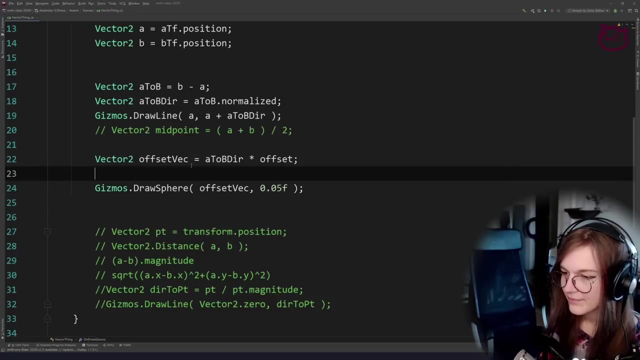 the red one. Now, same thing as before. If we just draw this one, it's again. this offset vector is relative to the starting point. So if we just draw this vector, it's going to be drawn at zero in world space, right? 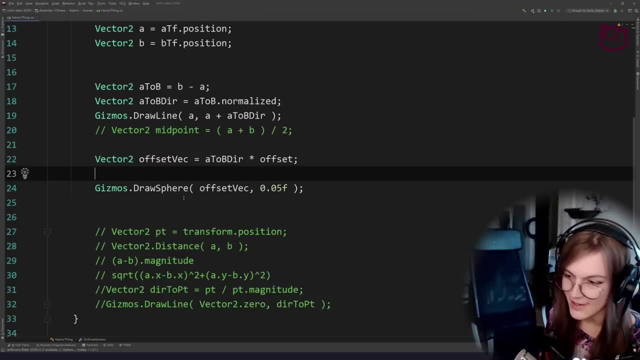 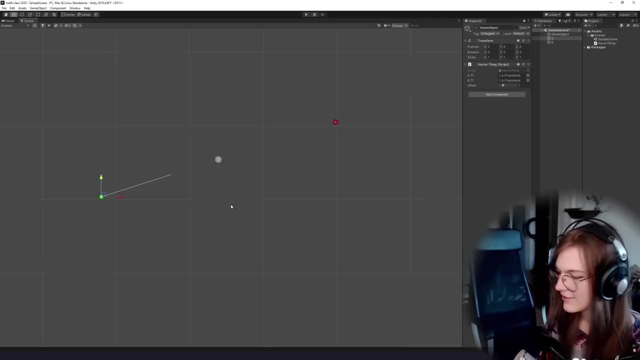 So we probably want to move that one. So we want to make sure that it's relative to A, Just for drawing purposes, right? So we add A to offset vector And then we can go back to Unity. Now we can see that we have this sphere and it's exactly one unit away from the starting. 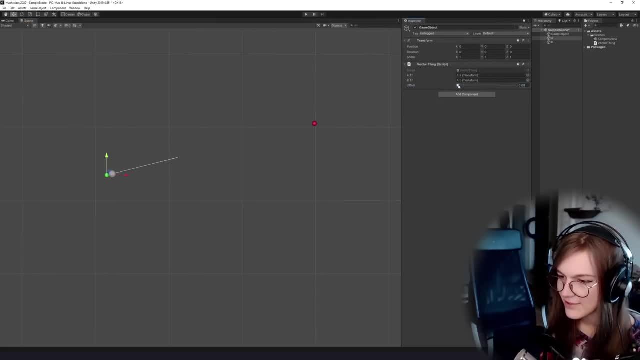 point And we can change this offset. So if we set it to zero, it's zero units And if we set it to two, it's exactly two units away. And, unlike the midpoint that we got before, this one doesn't squash and stretch. 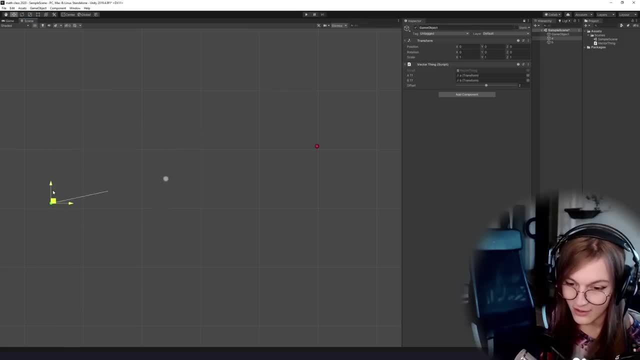 So we can change this offset. So if we set it to zero, it's zero units, And if we set it to two, it's exactly two units away. And if we set it to two, it's exactly two units away. And if we set it to zero, it's exactly two units away. 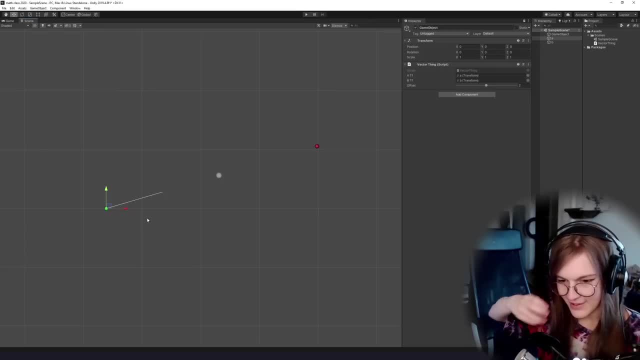 And if we set it to two, it's exactly two units away. And if we set it to zero, it's exactly two units away. So this is the same distance away from the player, right? So what is the point of this? 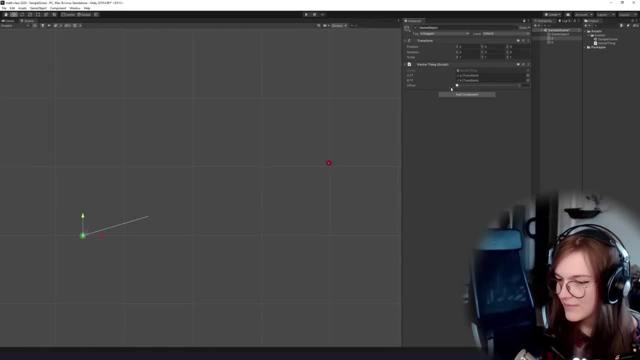 What's the use of this? Well, if you imagine this offset being a time value, then we just created a projectile, right? This thing is just moving at a fixed velocity, right? So now, all of a sudden, we just have a very simple formula where, if we increase offset, 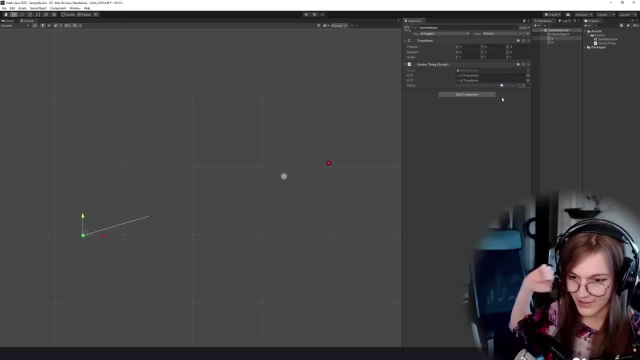 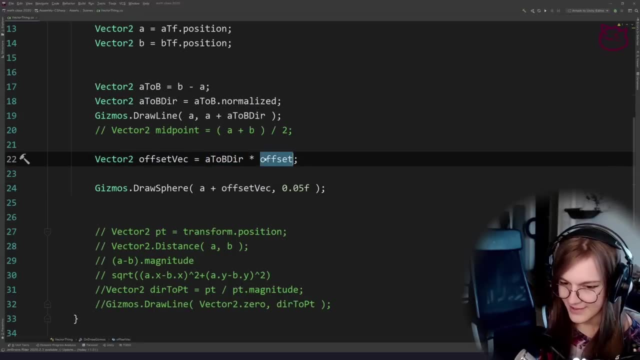 over time we have the flight path of an object in motion, And all we've done is basically take the direction, multiply it by the distance and that's it. If you increase the distance over time, then you have a moving object that's moving along. 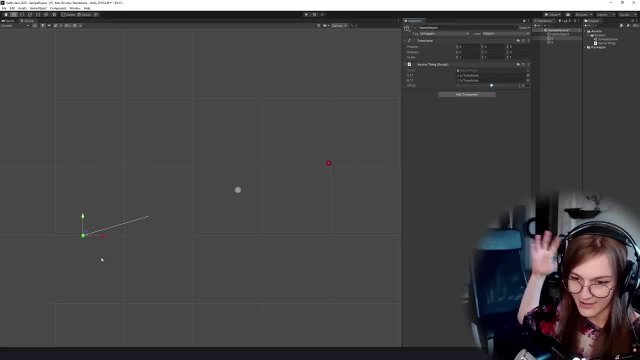 that direction vector right. Okay, did that make sense? Any questions or things that were not very clear? Such a good way of explaining it. I wish I had this lecture three years ago. You should be a teacher, or something. I should be a teacher, you know. 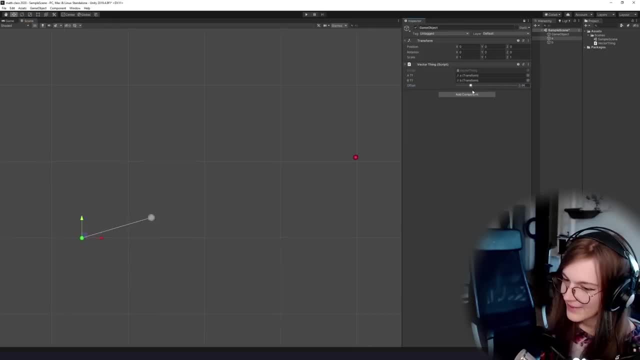 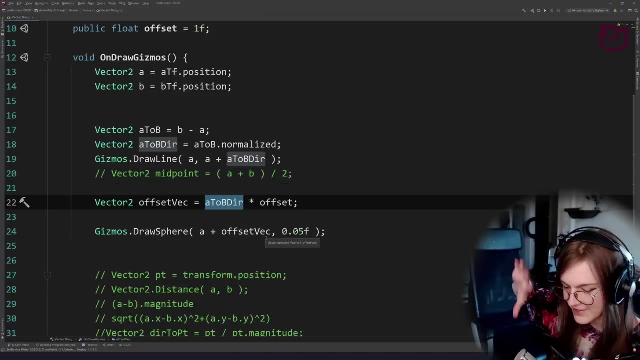 If only I was a teacher. Yeah, Okay, So, yeah. So now this is like very much a like. this is very, very central and very core to working with vectors in games, And the concept of a normalized vector or a direction is super crucial to have a good 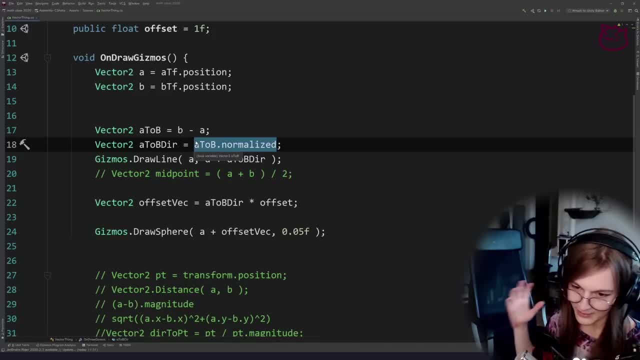 understanding of. I'm probably going to make that a very central part of all of the like, all of the assignments that you're getting, Because this is extremely core. Okay, Let's see Where are we in the schedule. Oh right, 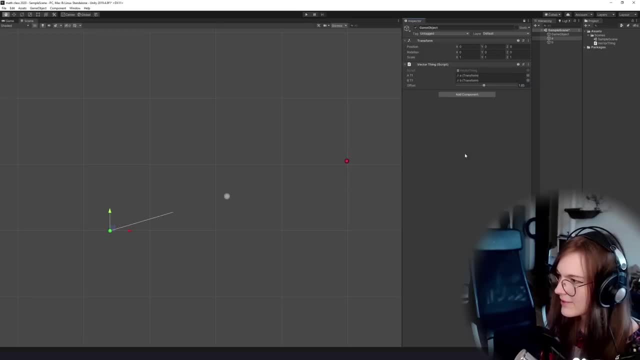 Okay, Maybe we should make more than one script, just to make sure that we're not like cluttering this whole thing. I forgot my hotkey for disabling objects. There we go. All right, Let's make another script Just to like. show more examples of like. why is this useful? 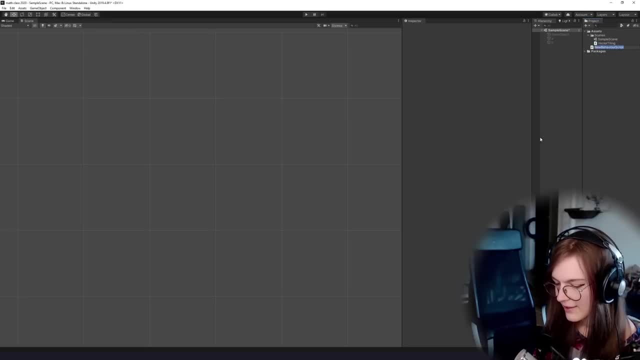 So let's say we want to make a A radial trigger, Like we have a trigger and we want something to happen by the distance to that thing, Right, So let's create it there. Okay, Okay, Okay. 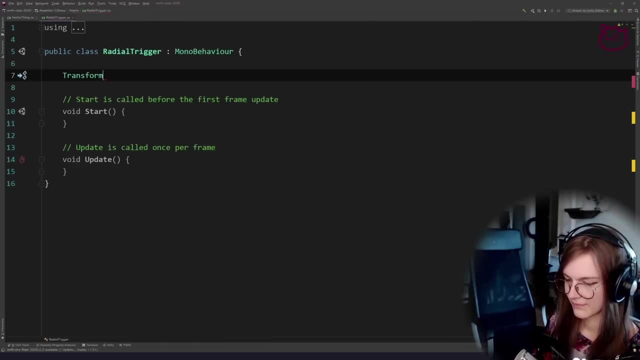 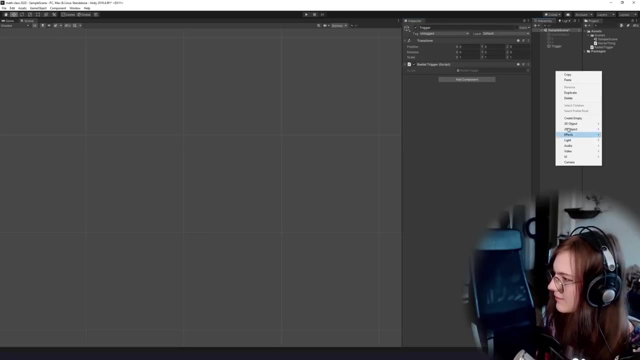 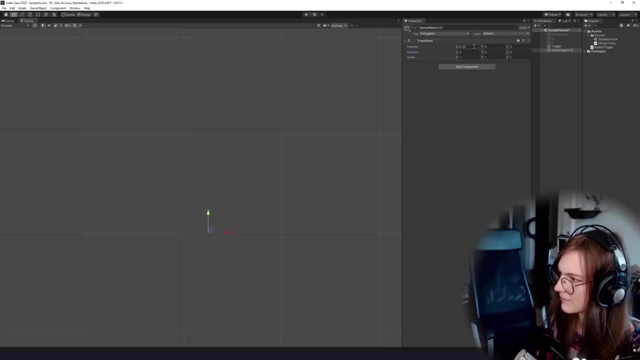 So I'm just going to go ahead and open example R and put it in here, And then some objects. we can test the code. Maybe this is a player, Maybe it's an enemy, Who knows? All right, So We have an object now. 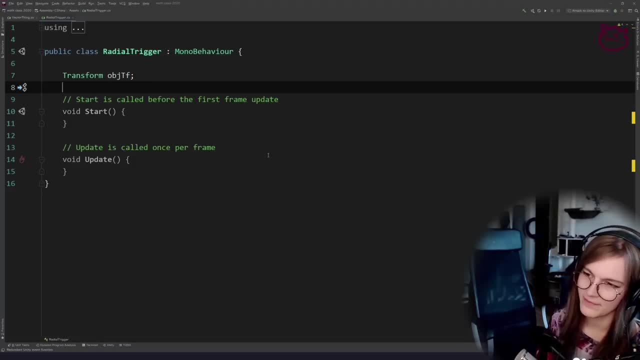 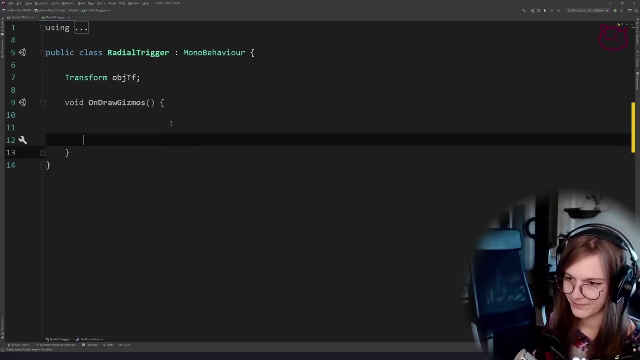 And we have our trigger here. trigger, that is just nothing right now. um, so let's go back to andragismus again. uh, because it's useful for just testing things very quickly. uh, there we go, okay, so let's see. well, what do we want to do in this trigger? uh, for instance, we might want to set a 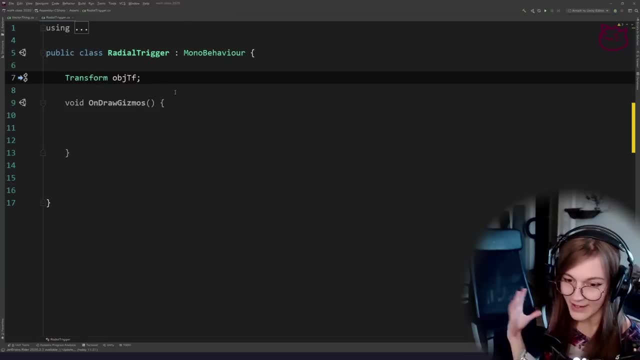 radius on this one, right, like what is the threshold at which we want to want this trigger to activate, right? so let's make another range, um, from zero uh to four uh, and then this is going to be the radius and we default to one, all right, and then we probably want to draw this so that we can. 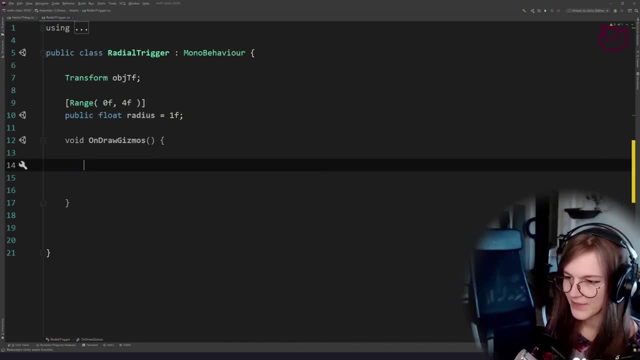 actually like see what the radius is. um, this is, by the way, something i talk about a lot when i have my tool dev courses, uh, andragismus- to just visualize things like radius and whatnot- super important and really good for level designers so that they can actually see. 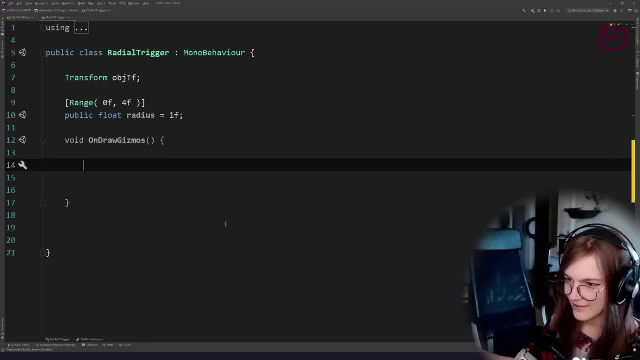 what the range is of everything. right, otherwise everything is kind of like difficult to parse. um, all right, so let's draw this. uh, we can do that with. uh, gizmos dot uh, draw. uh, let's see there are many functions here we can do. draw a wired sphere or instance, so wire is um wireframe, uh. 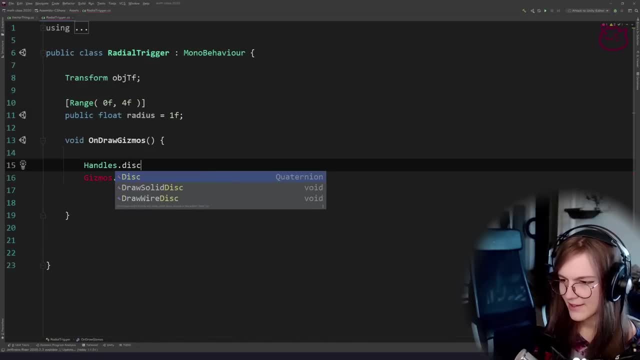 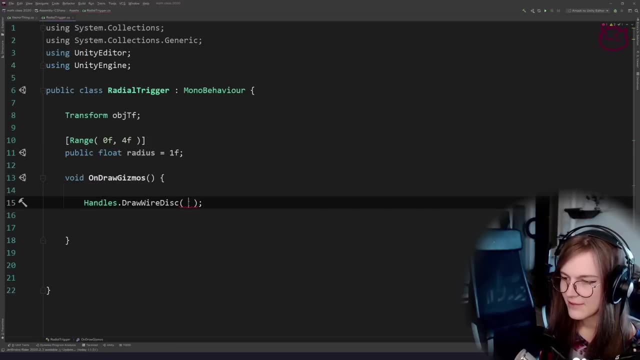 okay, i don't know. i think the- i think handles- has a wire disk. uh, maybe we should use that one instead. okay, one thing to note though: whenever you're using handles, uh, handles is in the uh editor namespace. so if you want to ship a game and you're using handles and andragismus, uh, you have. 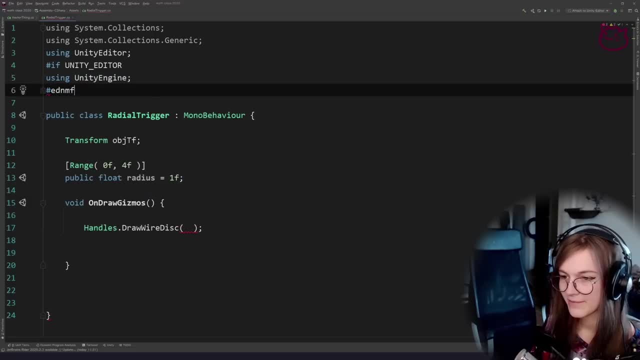 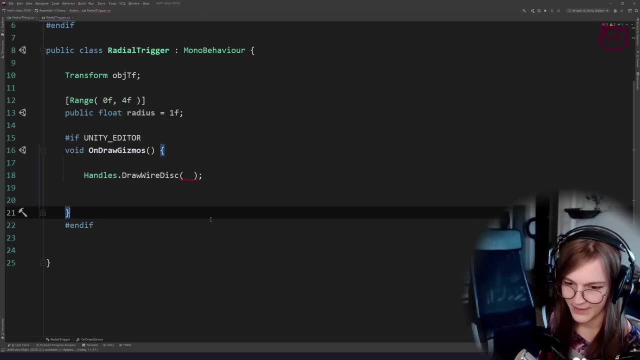 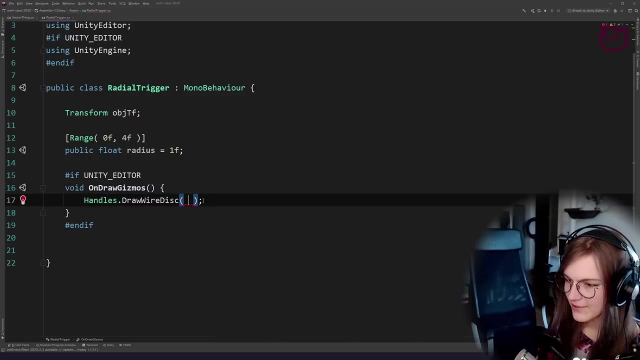 to make sure that you um, compile that out, right. uh, so in this case, if, as soon as you're using handles, always make sure that you, you, um, compile out the um, um, the code, right, otherwise you're going to get builders and that makes people sad. okay, so we're doing handles. uh, let's draw a disk. uh, we want to draw this. uh, at the location of 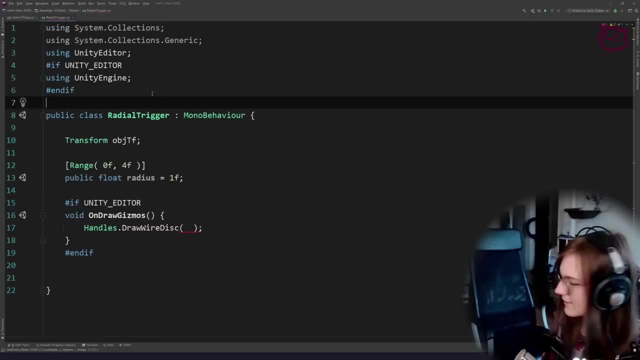 this trigger, right? um, that's the wrong using. that is true. uh, there we go. unity editor is the one that should be wrapped. uh, all right, so we want to draw this wire disk. uh, and let's see, uh, we need a center point. so the center point is going to be the location of this trigger, right? 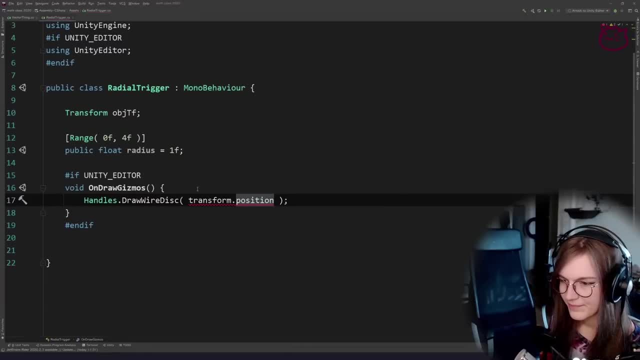 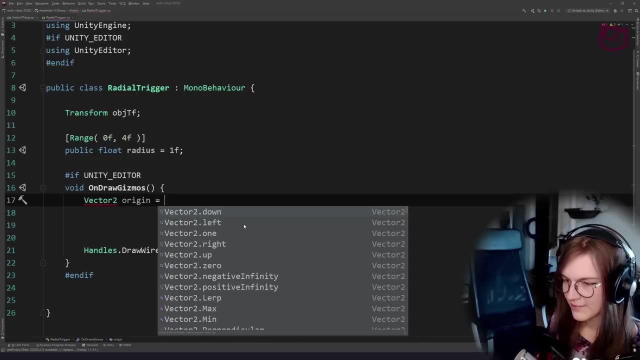 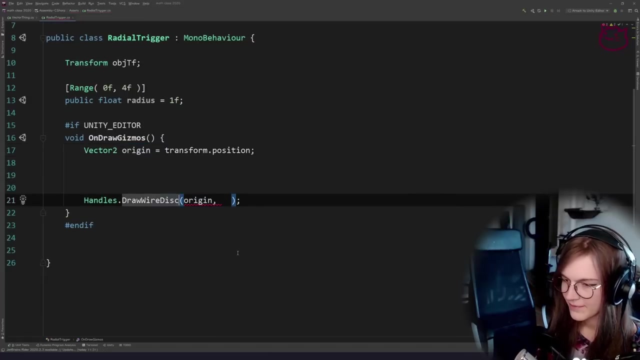 so it's going to be transformed opposition. um, actually, let's abstract this a little bit more. uh, so we have the origin right of the trigger, so that is just transformed opposition. uh, so we're going to draw that there. um normal: okay, we need to supply a normal for the disk. uh, we haven't really talked about 3d. 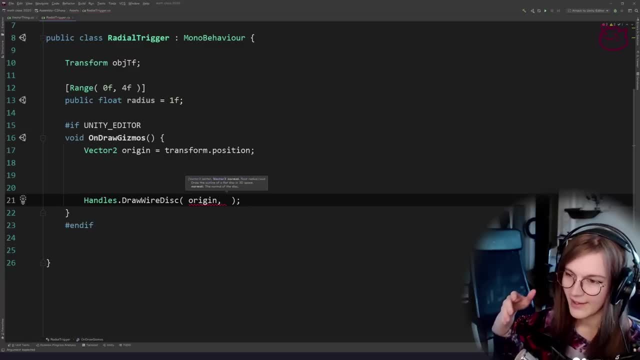 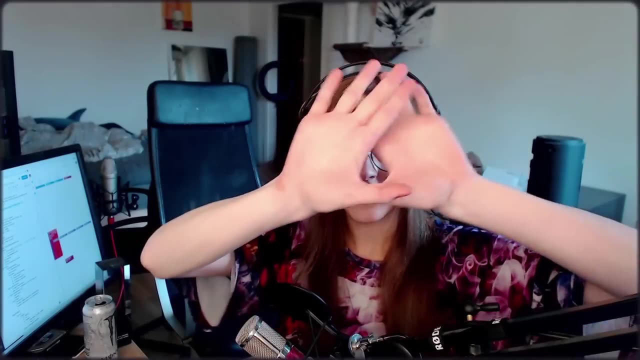 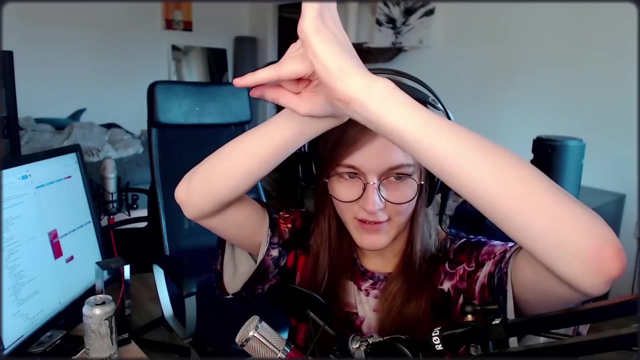 vectors- yet we're going to get to that later- and what normals are in general. quickly, if you imagine you have a plane, um like not a, not an airplane, just the physical plane, um, then the normal is the direction that is pointing out from that plane. so my finger right. 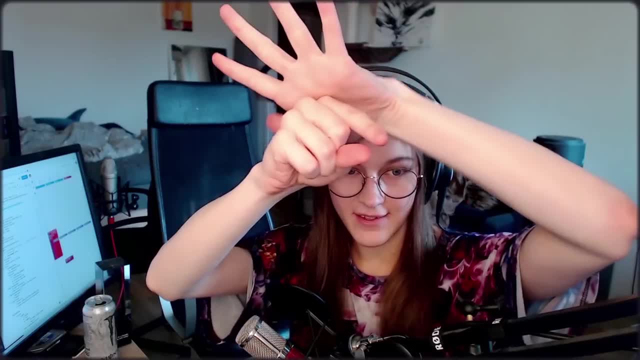 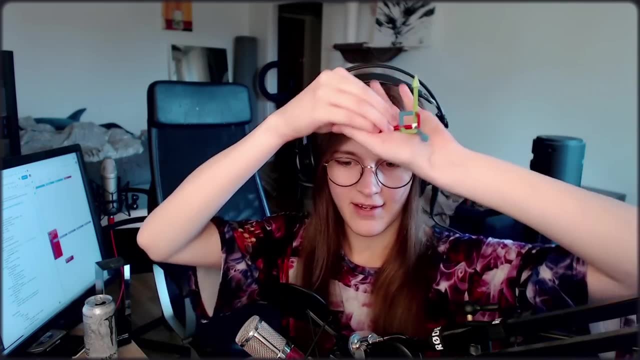 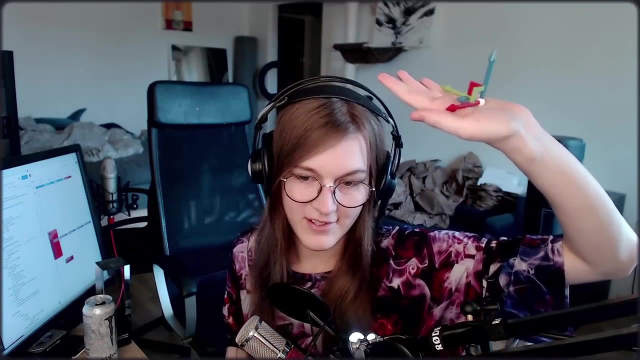 now is the normal of um, of the, the plane of my hand right, uh, so that's the normal direction, um, or it's there we go now. now we have a better, better normal direction, although usually z is the normal, uh, for surfaces. so, so the blue vector there is the normal of my hand, um, so, in order to draw a disk, 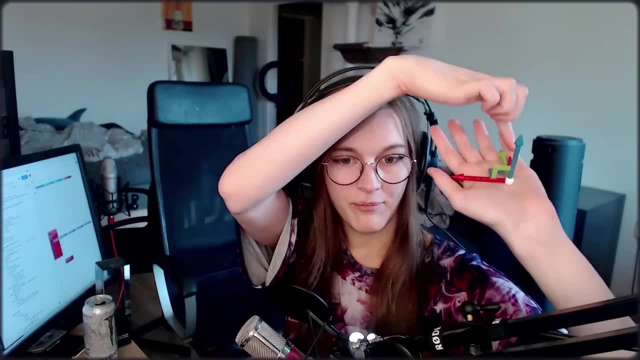 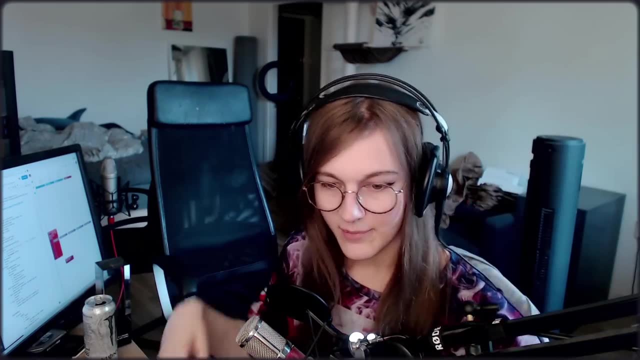 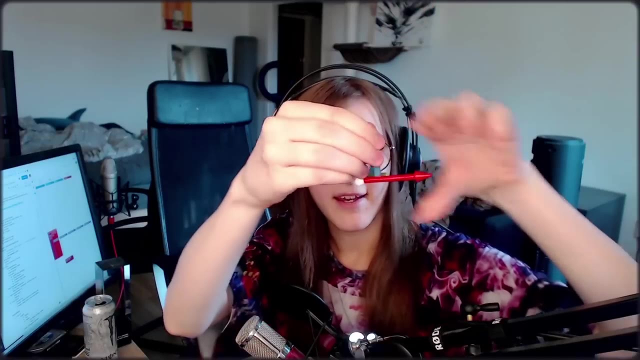 what that means is that, uh, the normal of a disk uh makes the disk lie in the plane of my hand if we supply the blue vector as the normal to this right uh, but we're in 2d right so so in our case, we, our coordinate system- uh, it's heck, kind of looks like this right uh, so we just need to supply. 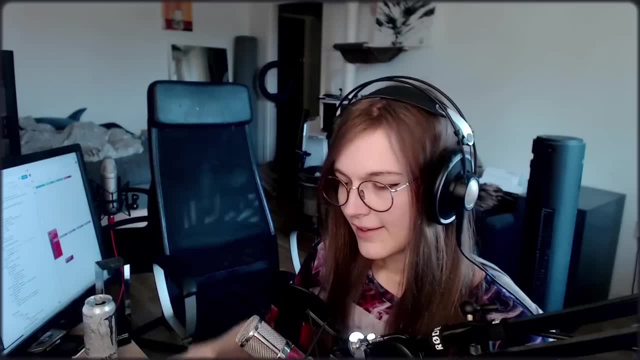 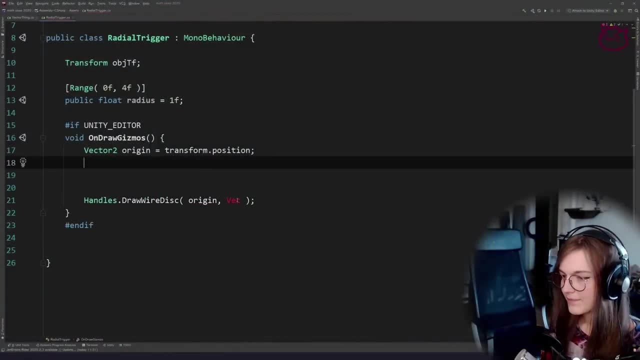 z-axis in world space. so in this case the um we're in 2d, we can just um tip over our water, water bottles, um. so, uh, we can just do vector3.forward. uh, this is equivalent to uh doing new vector3001. so this is just a direction vector that is pointing in the z-axis, right? um, all right. 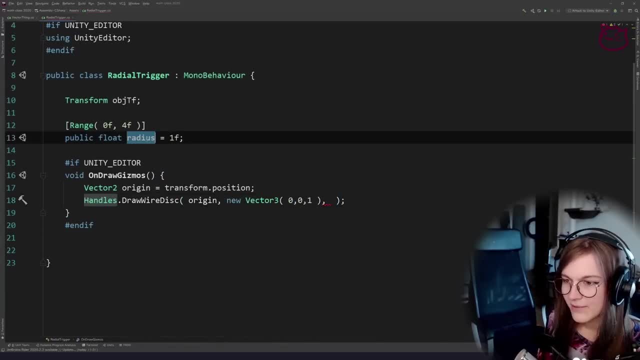 and then then we have the radius, so we want this radius to be the same as the radius of this trigger, right? um, jesus christ, all of you want to have that my gizmo. i only have two and i hand made them, so i don't know how to like sell them, um, yeah, anyway. so now, now we've supplied a normal through this. 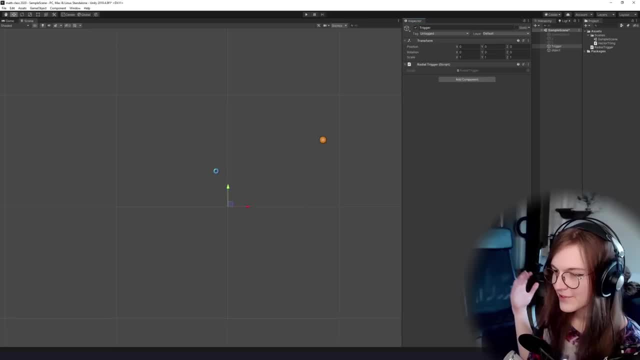 disk. we have a radius and an origin, and so now we should be able to see a wireframe ring around the this trigger. uh, cool, um. so now we- um, we cannot tweak the radius right. we can change the radius and the ring will change size. we can move this around and um, everything is working as expected. 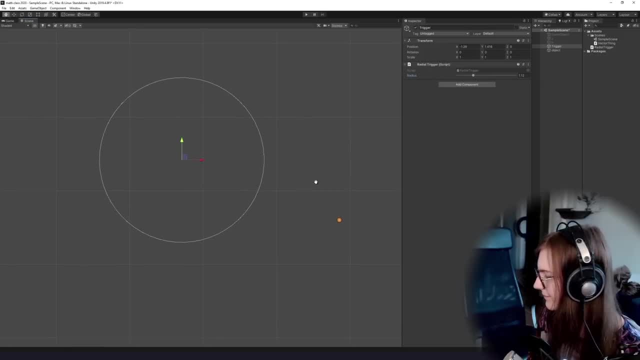 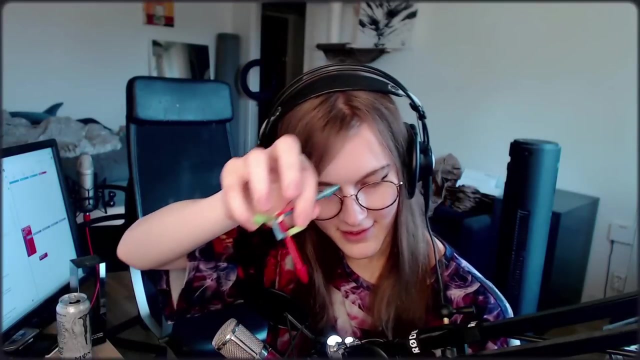 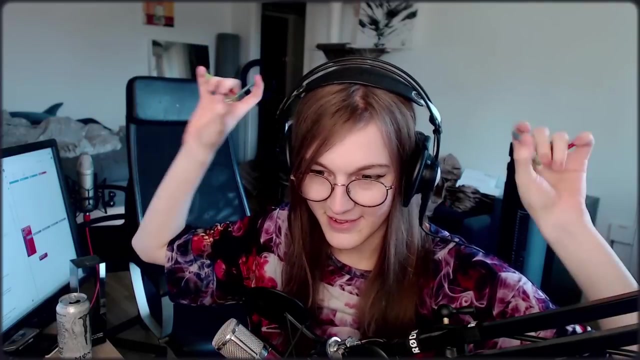 right, um, okay, i 3d printed my gizmos, um, and then i painted them. that was my process. that's about it. yeah, these i have two. they're very useful, especially when you get to talking about cross products. it's, it's super good. do you have the schematics? um, i just made the 3d model at. 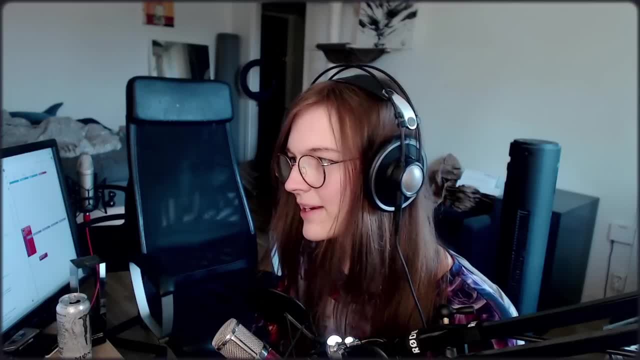 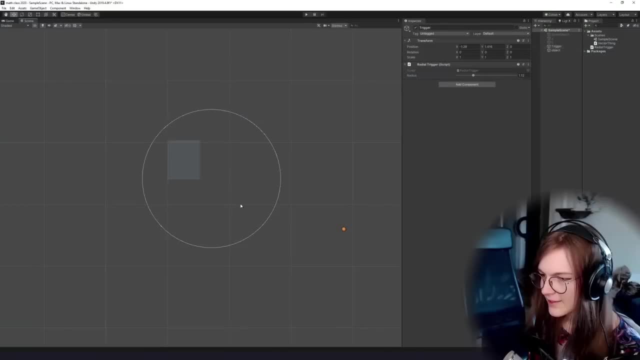 some point. i don't know, it might actually be at my work computer at necorp, but i could just remake the model or whatever. it's not a very complicated model to make, all right. so now the question is: how do we actually get the like? how do we know if we are inside of this trigger? 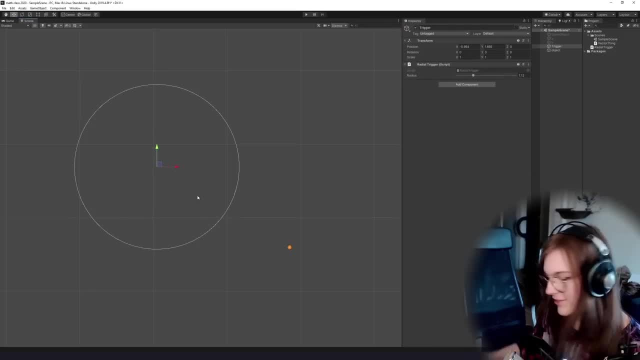 or outside of this trigger, right? so? so now, all of a sudden, we have a math problem that goes through all the concepts we've been talking about, right? so we have, uh, we have a point: this is going to be a player or an enemy or anything else, right? and then we have the point that is the center of the 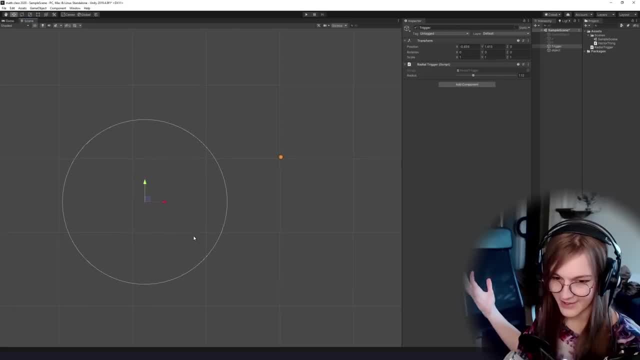 um, circular trigger. all right. so how do we solve this? um? does anyone have any ideas in chat about how to how to do this? what are we going to do? move it. all we need to. all we want to know is whether or not this point is inside or outside the trigger. how do we know that it's a boolean state, something we can put? 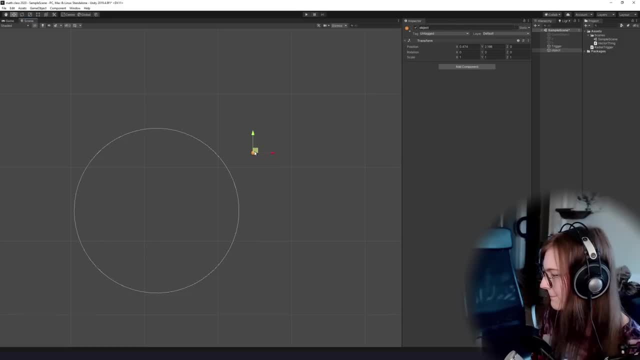 in an, in an if statement: right, check the distance between the two objects. yes, okay, we have the distance. what do we then do? uh, if it's greater than the radius, it's outside. yeah, exactly, physics dot overlap. that works for physics objects, but right now we're not using any physics objects. 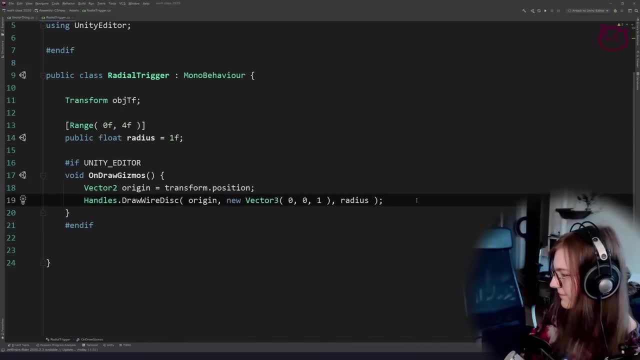 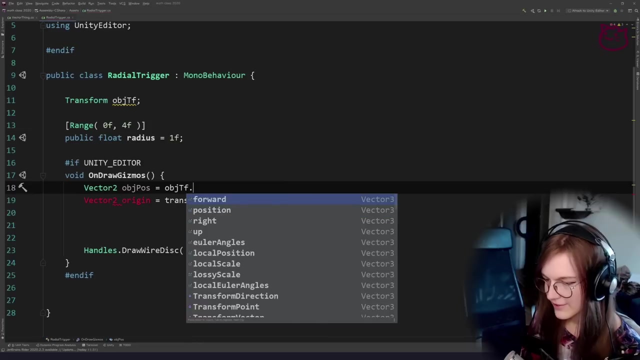 or colliders, um, all right, cool. so let's do this again. how do we check the distance between these, these two points? uh, well, we have the origin, uh, and then then we have the object position, uh, let's call it object position, uh, that's object transform, dot position, uh, okay, so now we need to know the distance. 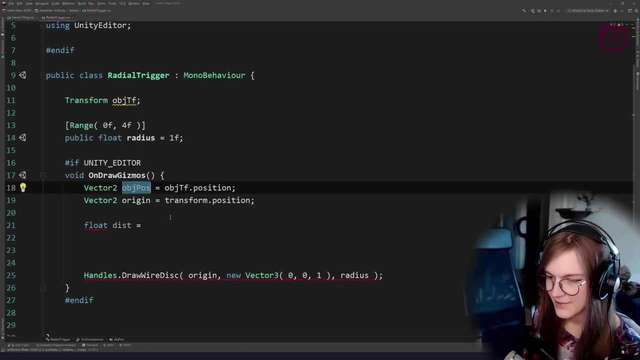 between these two. so distance equals- uh, we can do vector two, dot distance between object position and the origin. so now we have a value for, uh, how far away is this object from the trigger right? uh, but now we also need to know the state of whether or not it's inside or outside. 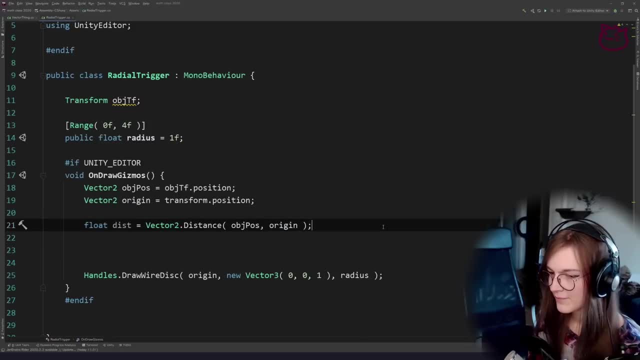 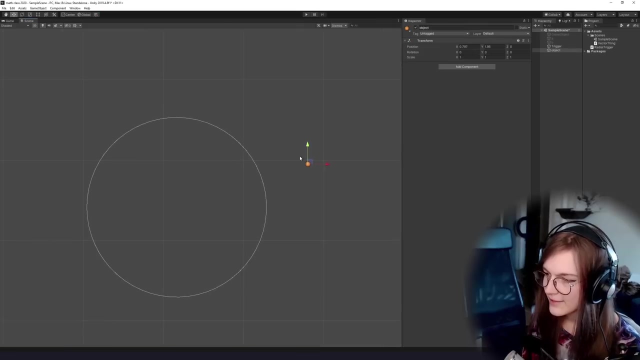 the radius of the trigger. right, that's kind of what we're interested in. um, okay, so we have the distance and the radius, so all we need to do then, uh, is to: uh, we can make a boolean state. so, uh, let's call it is inside, uh, and the only case where this is inside is if the distance is less than the radius of the trigger. 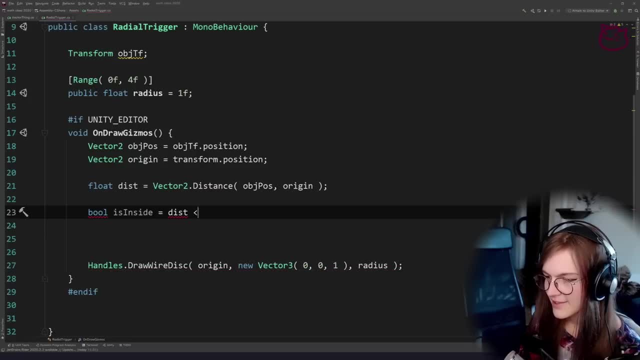 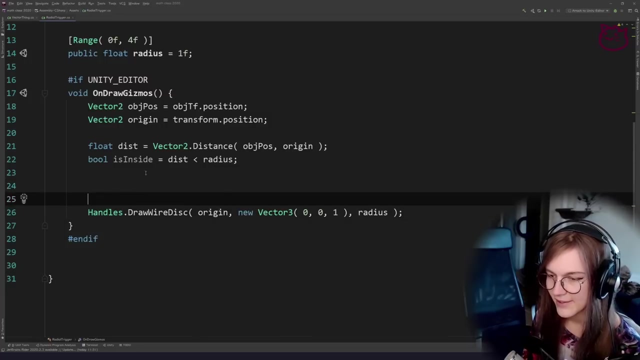 right, so if the distance is less than the radius, uh, then it's inside. uh, you could do less than or equal to implementation dependent depends on how you're going to do this. um, yeah, so now we have a state for whether or not it's inside and let's- uh, let's, set the color of the ring to be red if it's. 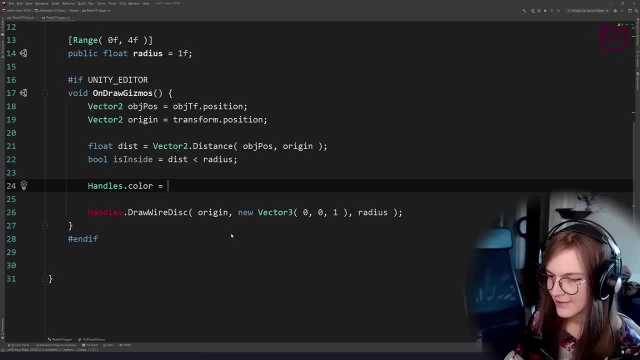 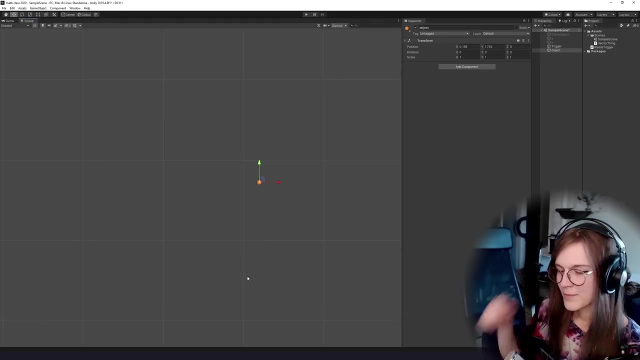 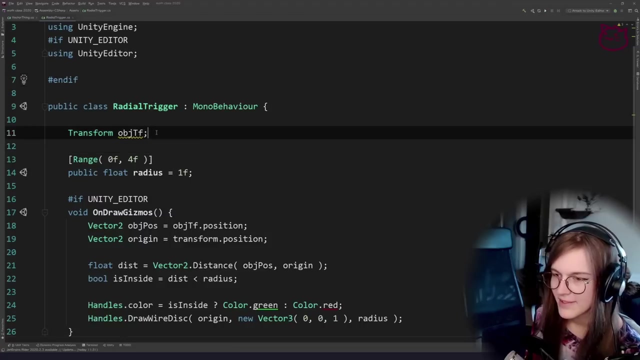 outside and green if it's inside, So handlescolor is inside and if it's inside we want to do colorgreen, not green otherwise colorred. So red outside, green inside, And transform has not been assigned. so now we have a bunch of null refs because this: 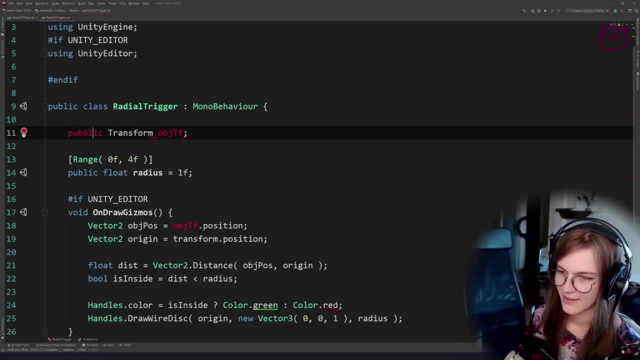 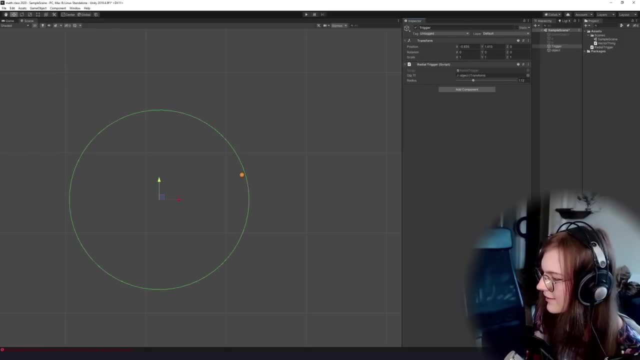 is not serialized, So let's serialize it. All right, still null. There we go, Cool, All right. so it's green, Move it outside. it's red And it seems to be able to check this distance right. 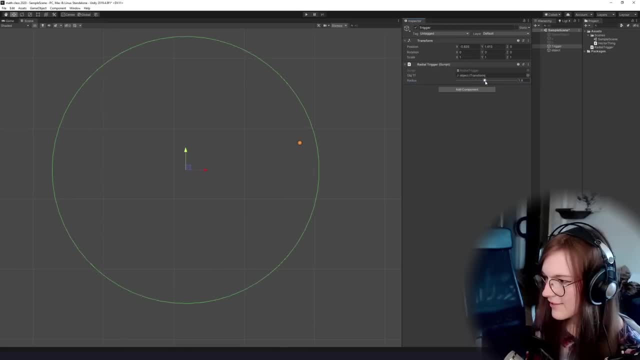 So, as usual, you need to test things, make sure you can change the radius and it still works. Seems like this is working. Was everything clear- how this was set up, why it works and everything? Oh, what's the vector 001 needed for? 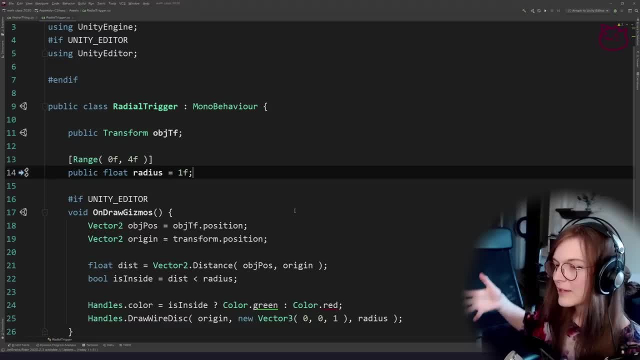 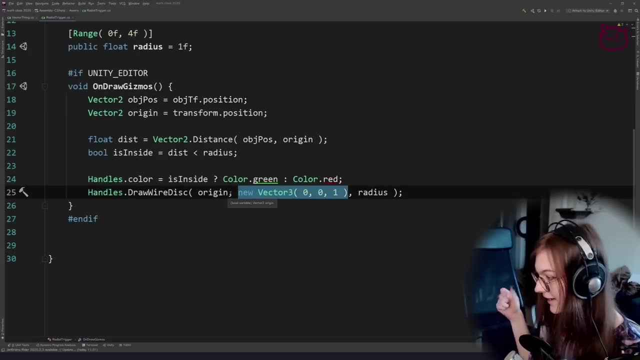 Yeah, that's just because the disk function is meant to be able to draw in 3D space. So this is just our way of telling it to. we just want to draw on the xy plane, right? Because we set the normal of the disk to be on the z-axis, which means that the disk is 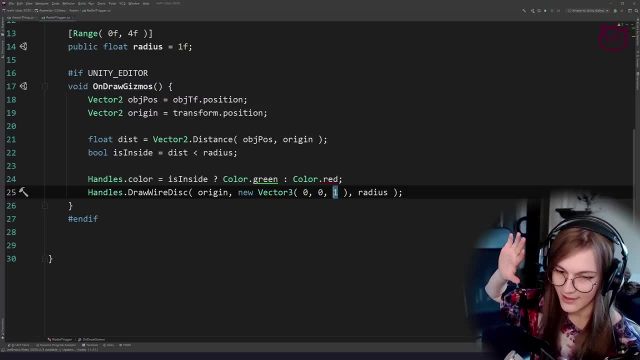 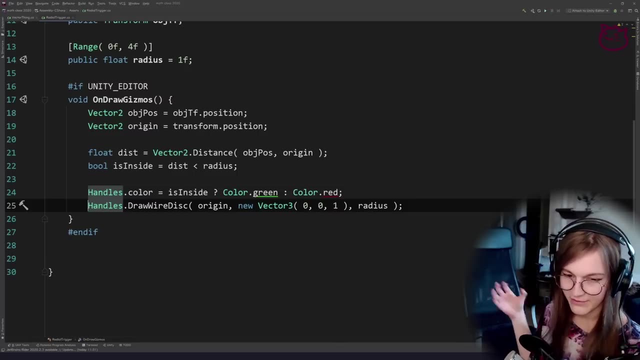 going to traverse on the xy plane, Right? Why not use vector3.forward? I mean, if I were to write this code when I'm working on something, I would write vector3.forward Just for, like educational purposes, talking about what this is, what it means, vector3.forward. 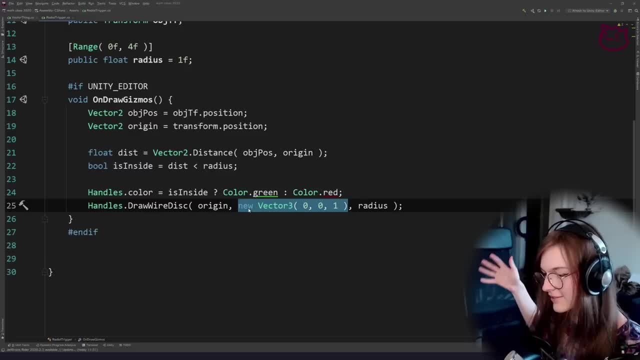 is a little bit unclear when I'm teaching what vector3s are. So in this case I just typed vector3, because it made things a bit more clear in terms of what the underlying data is right. But yeah, that was the only reason. 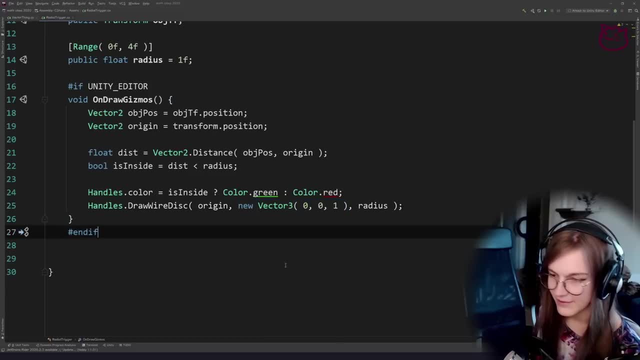 But otherwise this is equivalent to vector3.forward. It's the same value, right? The only reason that I sometimes don't do it is because transformforward is very much not the same thing as vector3.forward, so you need to keep in mind what you mean when. 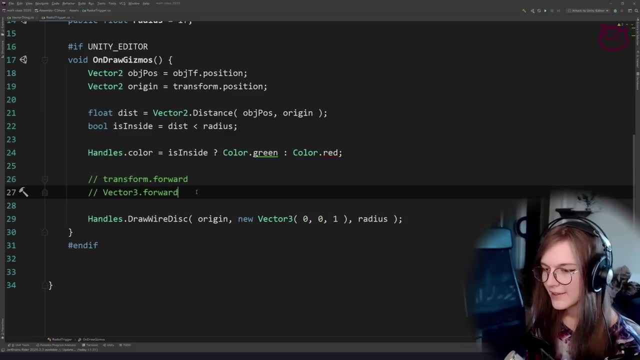 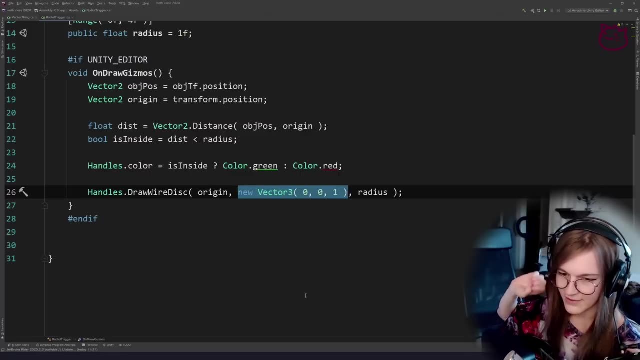 you type the forward and sometimes you can confuse the two. So, yeah, so sometimes I think it's good to just write the whole vector out to clarify that this is just a vectorforward. Yeah, It's a vector on its own. 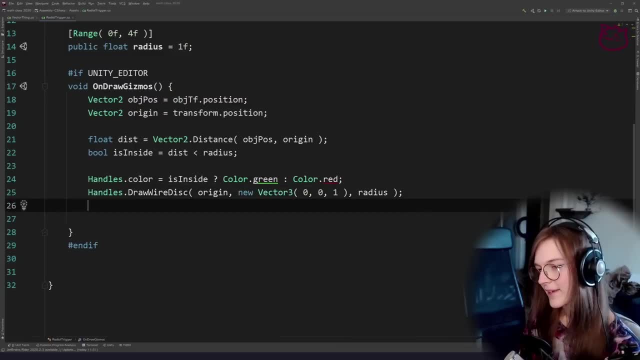 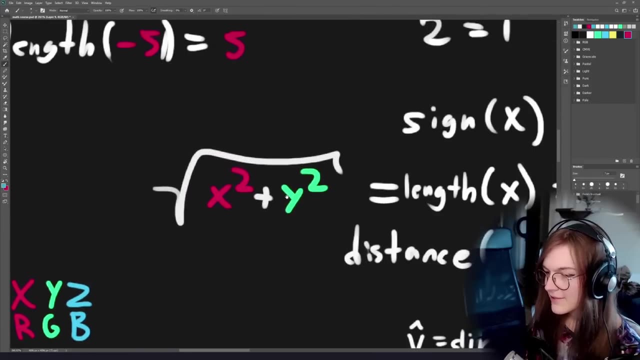 One more thing. So we talked about how to get the length of a vector right And, if you recall, this is how you get the length of a vector right. So you have an x component of a vector, You square that and then you add the y component, squared, and you take the square root out. 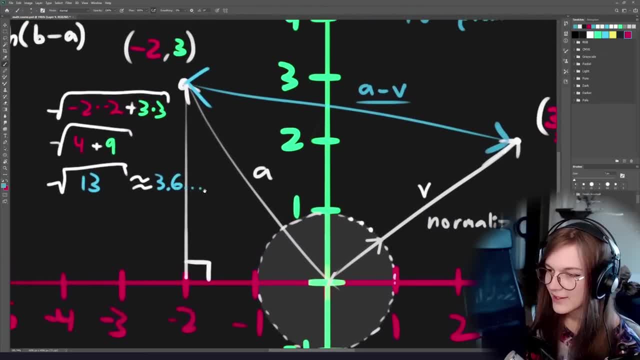 of that. It was the Pythagorean theorem that we talked about earlier, that whenever you have a right angle triangle, you can get the. You can get the length of the hypotenuse using that formula right, Which is equivalent to asking what the length of a vector is right. 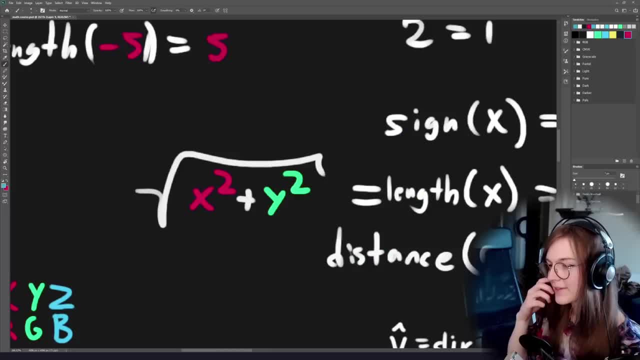 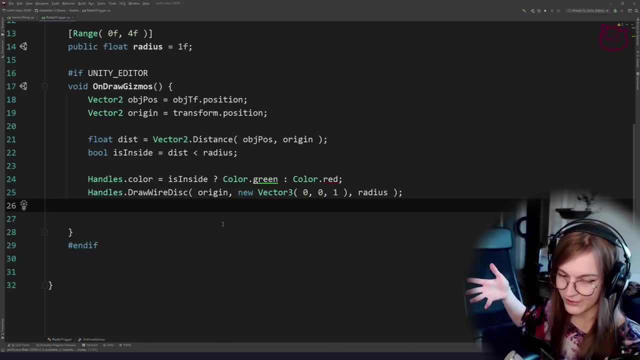 Okay, So we got this formula and we can use this to calculate the exact length of a vector. If you're doing, If this is in some sort of for loop, and also this person in Twitch chat is really annoying, Can we just time out this person? 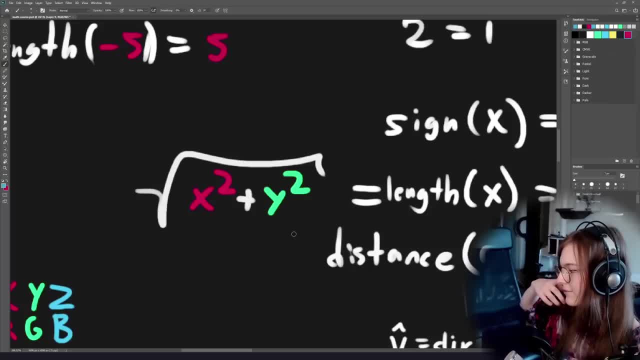 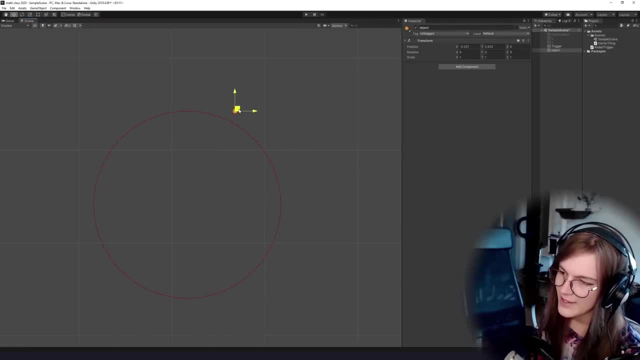 There we go, Great So okay. So if we can, We can use this distance value to check a threshold, just like we did here, right? So if we, We can check if it's less than some value or greater than some value, right. 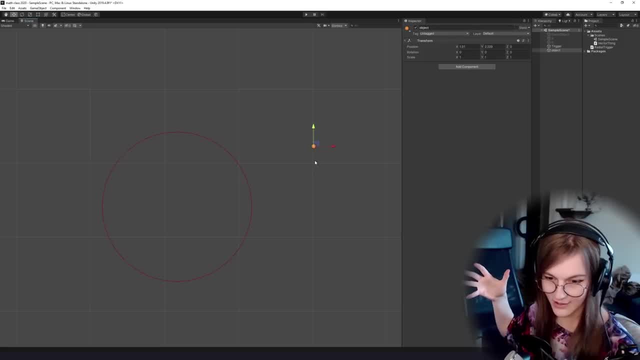 So if you are doing some code that is like iterating over 600 objects or whatever, so in that case then you might want to optimize this, because if you're doing a distance check, like, Let's say, you're doing a game across 600 objects or maybe even more, so in that case you might 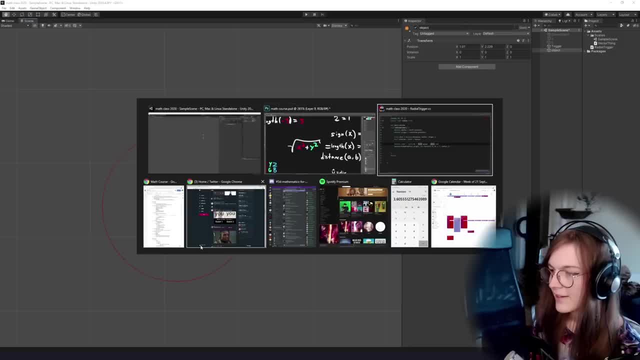 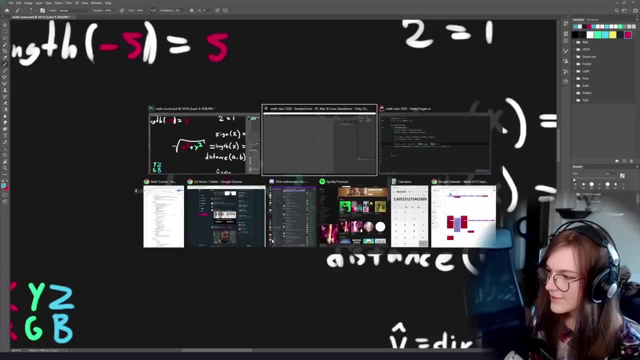 want to. You might want to optimize it right, And there is a very nice way you can optimize distance checks when you're doing stuff like this. So one thing that is probably good to know is that square roots are not like super. 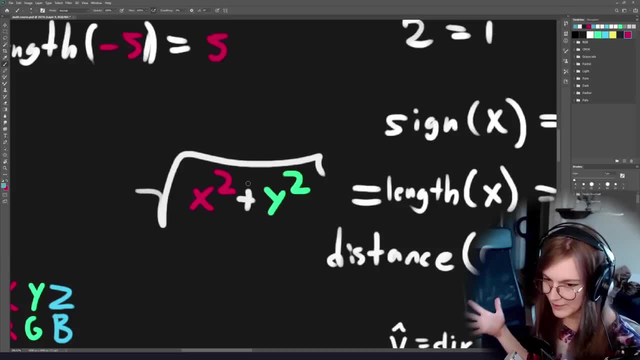 expensive, but they're a little bit more expensive than, like, multiplying. They're a little bit more expensive than adding or subtracting. So it's It's really good to keep in mind that the square root itself has a cost to it. 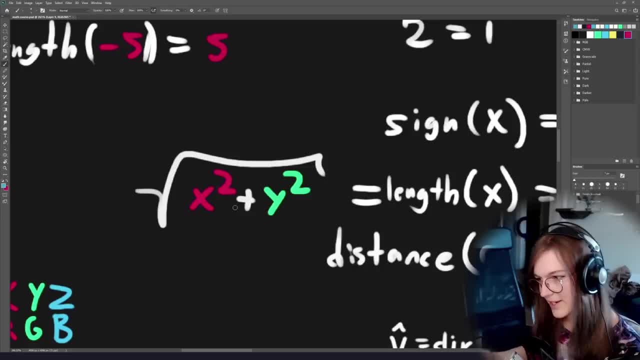 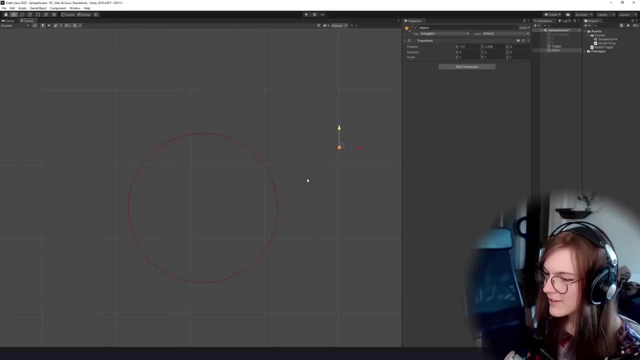 So, again, when you're doing four loops over many objects in an update loop or something, that's when it really matters, right? Otherwise, don't micro-optimize this all the time, because it's going to make your code unreadable. 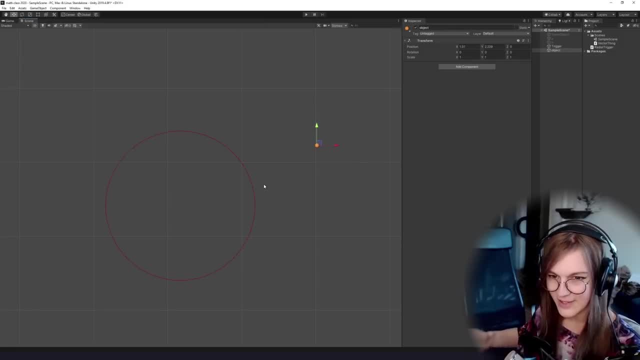 So don't do this all the time. I'm just like bringing this up as an optimization tip when you have like very heavy, many distance checks and whatnot. All right, So if we want to make this cheaper, we could actually get rid of this square root. 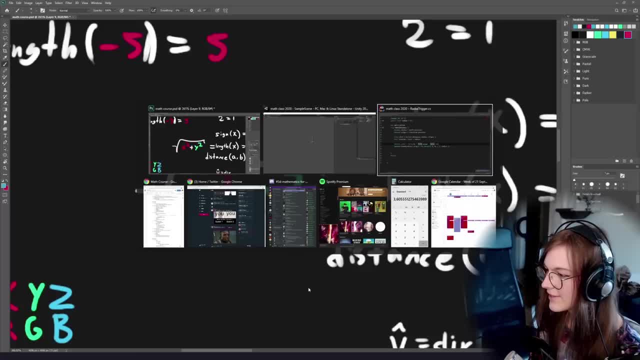 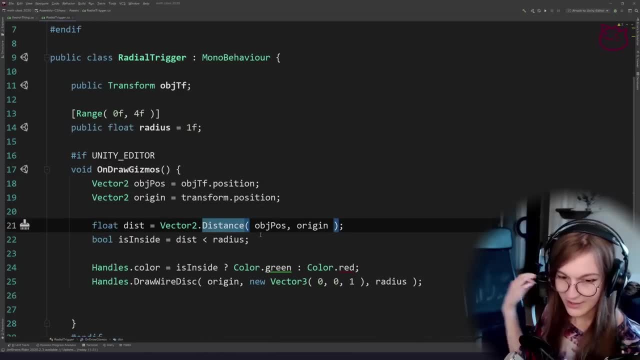 We could just nuke it, Just remove it, and then we can see what happens, right? Okay, So previously we were checking the distance, right? This distance in and of itself contains the square root, So this one is doing the whole square root check, right? 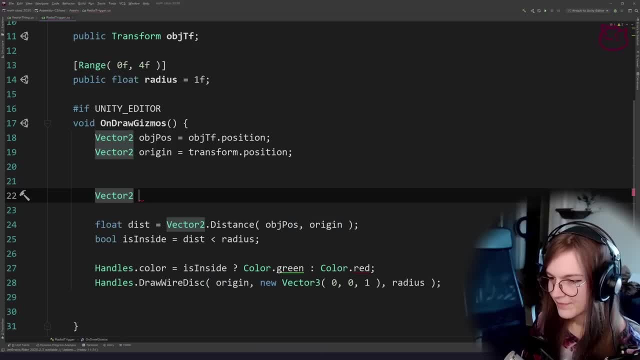 But we can do this manually. So let's first get the displacement difference vector. We can call it Z Trigger, Actually, let's call it displacement. There we go. Now we're going to use esoteric terms. So the displacement here is that we subtract one from the other, right. 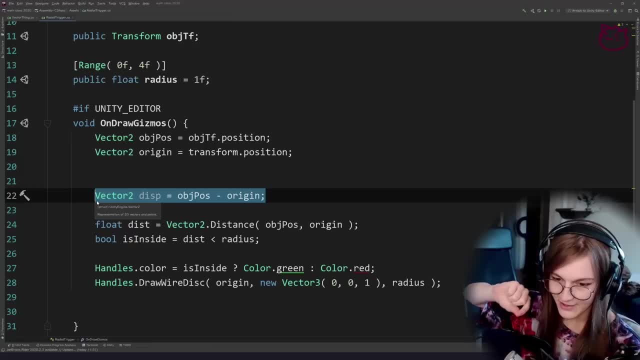 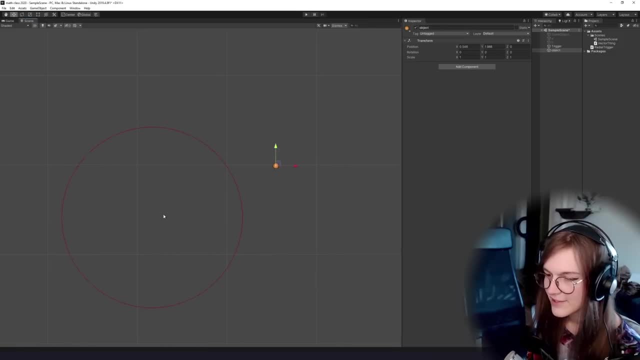 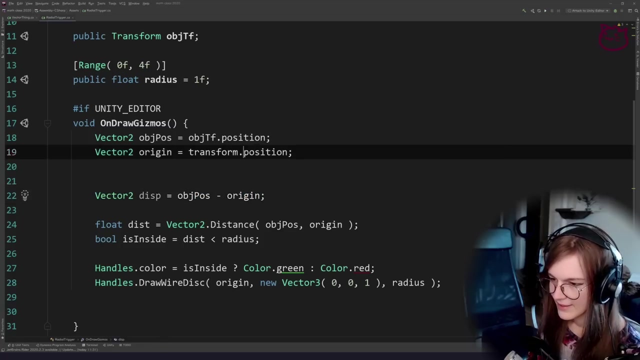 So this is the vector going from the origin of the trigger to the object that we're checking the distance to right. So that's the vector going from the center to this one, right, Okay, All right, So that gives us the displacement vector. 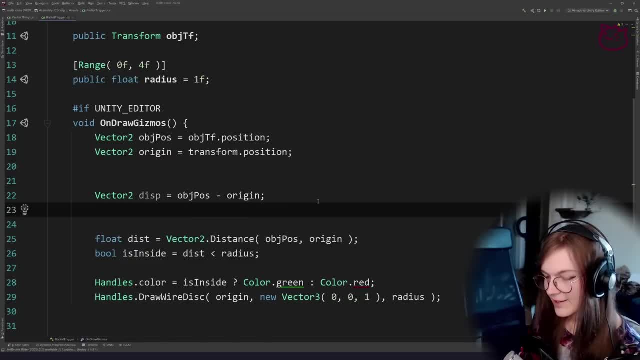 Now we want to calculate the length of this, right, So we want to get the length of this. We could do displacementmagnitude, but if we want to do this manually, just to clarify the math involved in this. So the length, Or this, is technically the distance. 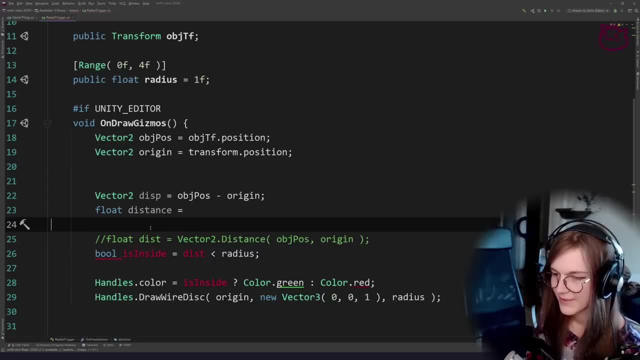 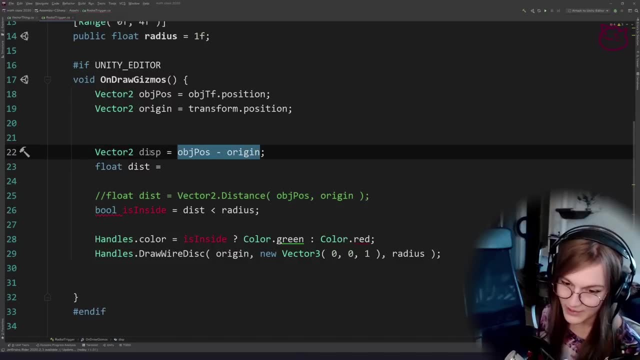 Maybe we can call it distance: There we go, Comment that out, Or just dist, There we go, All right. So we want to get the distance, So we want to get the distance between these two points right, And the way we do that is get the length of the displacement vector right. 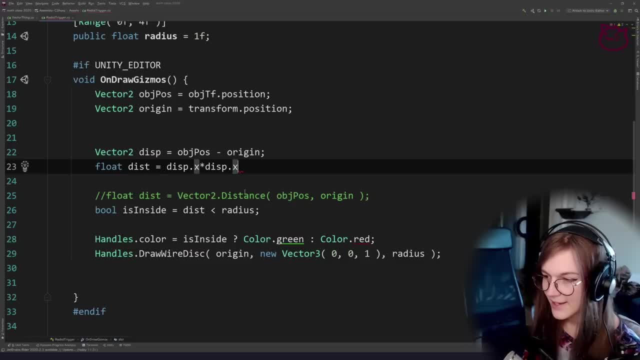 So we do the x component and we square that as in multiply it by itself. Usually, if you want to square something, multiplying it by itself like this is usually faster than using, like a floating point, power function. So if you do like displacementx to the power of 2, in some cases this is going to be way. 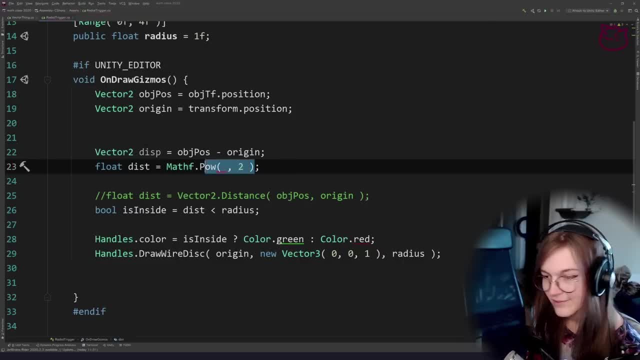 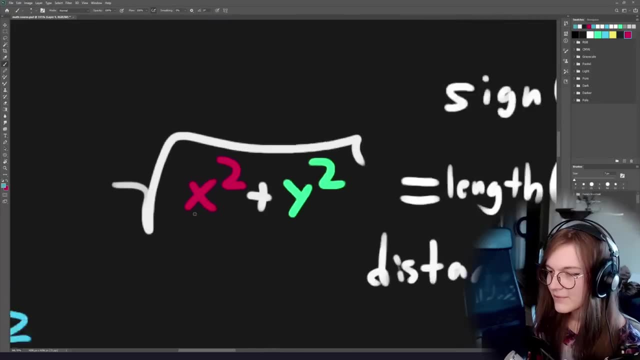 slower than just multiplying it by itself, right, So that's a useful thing to know. So, displacementx times displacementx. What did we just type? Well, we just did this part right. The x squared, All right. So now we do the same thing for y squared. 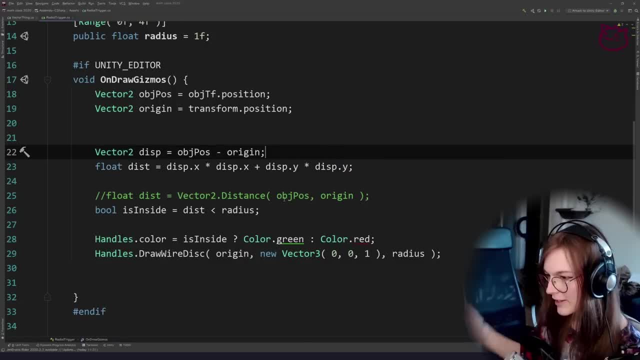 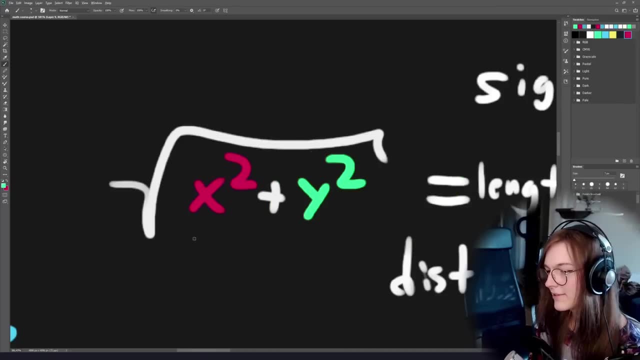 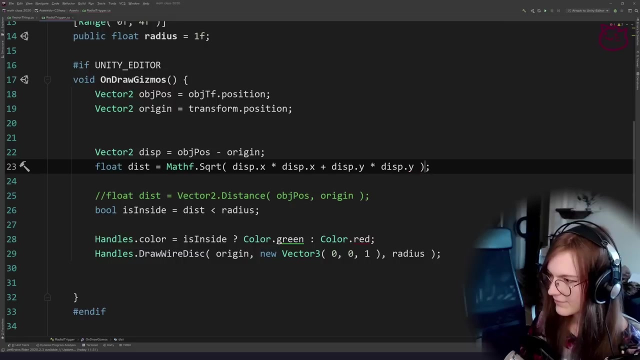 So we add displacementy multiplied by displacementy. So now we did this part right here with the y components, And then finally we do the square root of the whole thing. All right, So math dot, square root of all of this. So we got the distance. 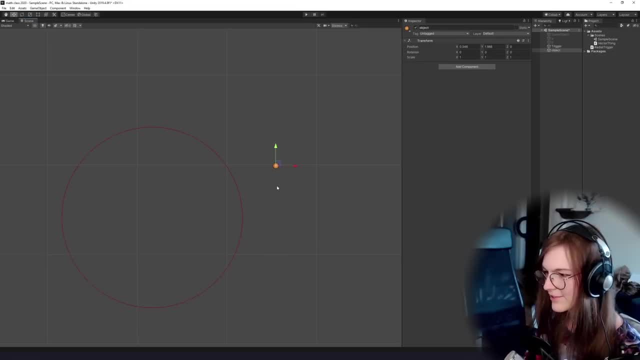 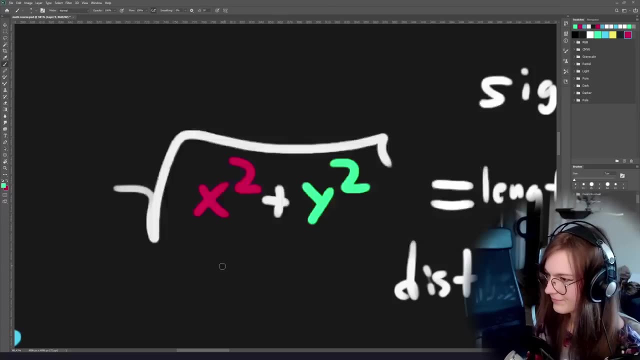 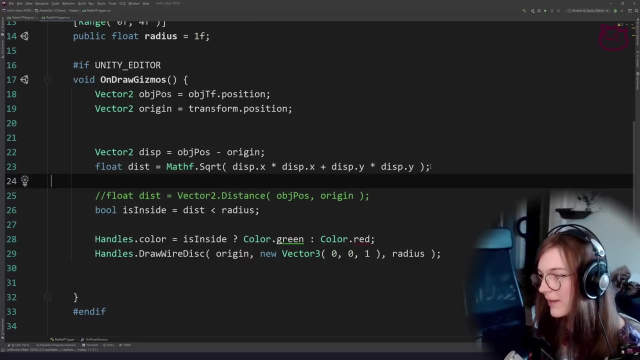 And now I'm pretty sure everything should work the same way it did before, unless all of my math is wrong. All right Seems to work, So nothing's changed so far. So now all we've done is basically replace Unity's distance function with the math underlying. 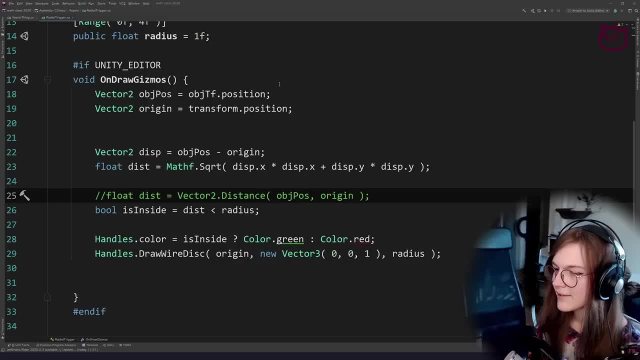 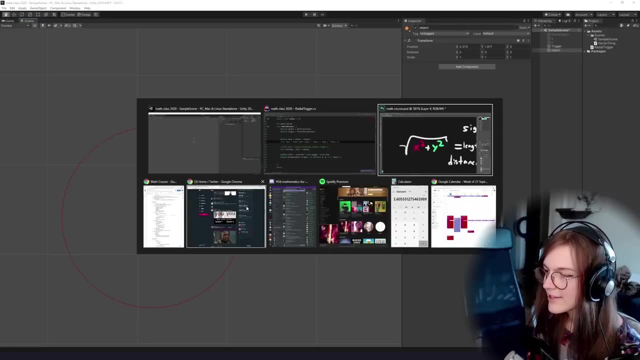 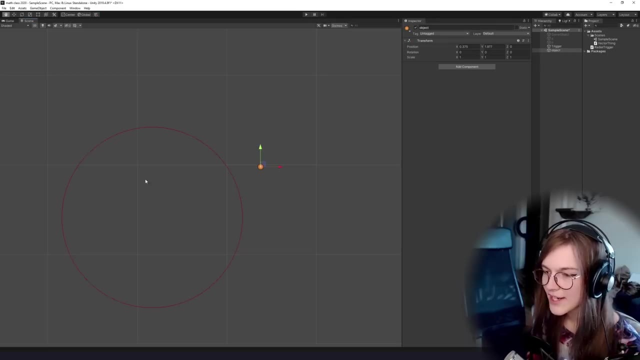 all of that stuff, right, Okay, So what we're now going to do is the optimization part. So we talked about how you can actually remove the square root and still make the math work out so that we can do a threshold check, Because, again, we're only checking a threshold. 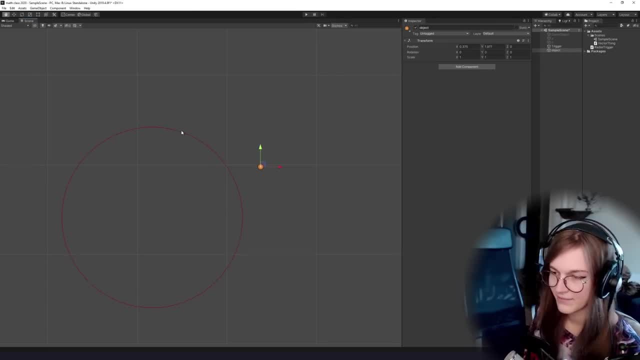 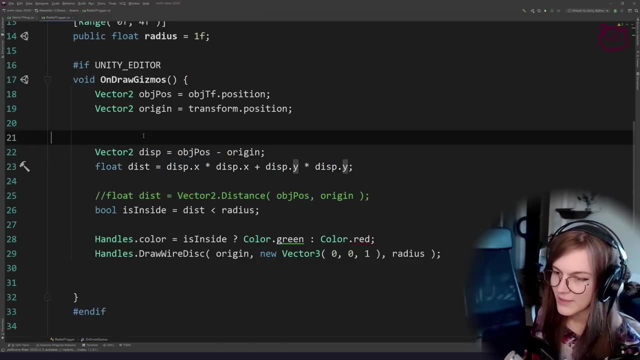 All we're interested in is: is it less than or greater than some value, right? So in that case we can remove the square root. So what does this mean then? Well, now, this is not the actual distance, But this is the distance squared, as in the distance multiplied by itself. 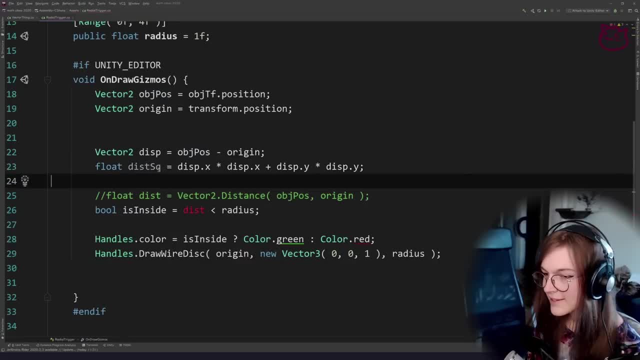 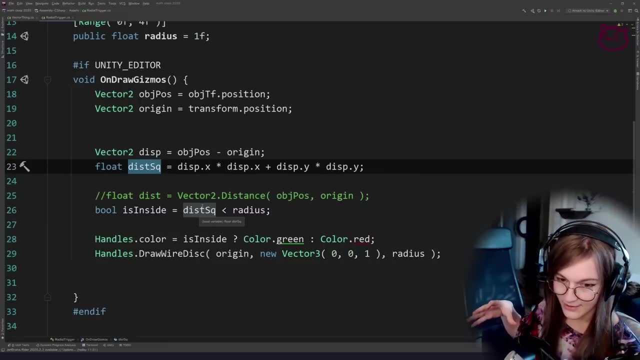 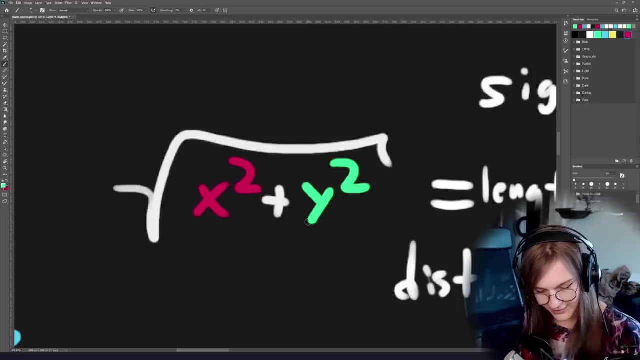 So usually it's good to like. note that with like SQ is usually what I use whenever something is squared right. But now the distance squared is not the actual distance, right? Oh, if you want the like actual algebra involved in this, sorry, should, probably, should, probably. 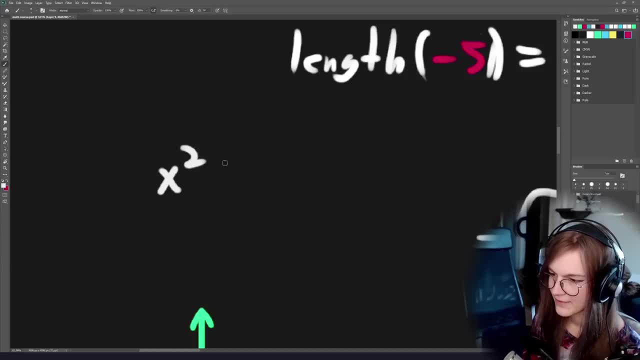 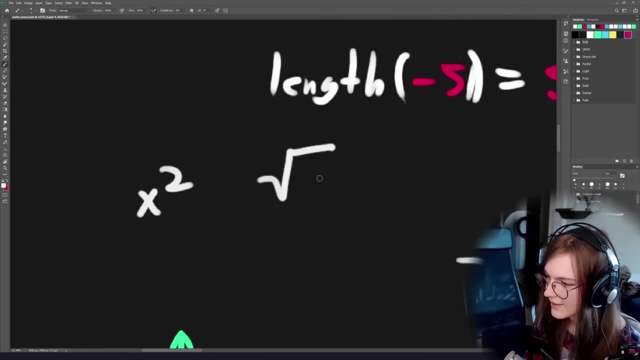 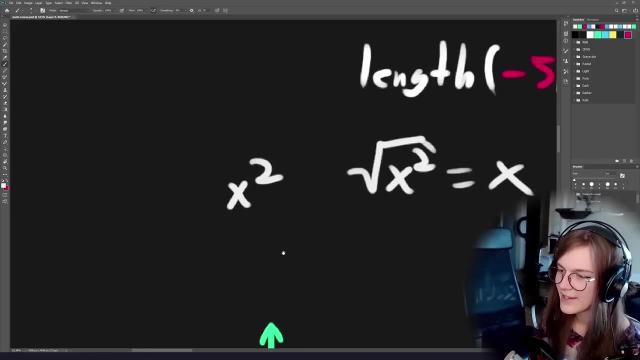 write that down. So X squared. if you want to get X out of this, then if you take the square root, if you take square root of X squared, these are going to cancel out and you just get X in the end. So like the square root and reason something to the power of two. they're kind of like. 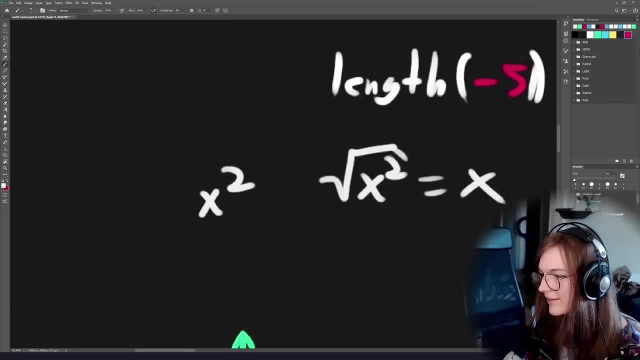 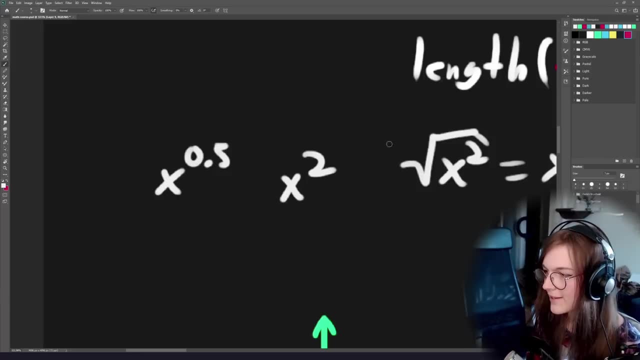 opposites of each other, right? So technically, square roots are: it's just X to the power of 0.2.. 0.5.. We just usually write it out as the square root symbol, Anyway. so basically they can cancel out and whatnot. 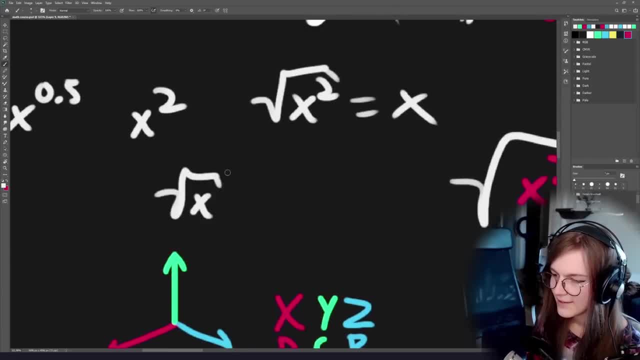 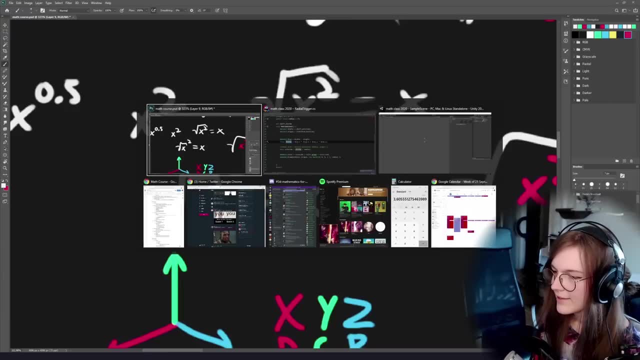 So if we take the square root of X and raise that to the power of two, then we get X. So same thing between these two, Okay, So so basically, when we get the distance here where we remove this square root, we 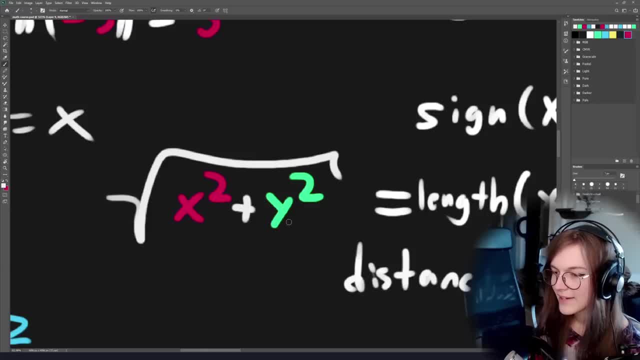 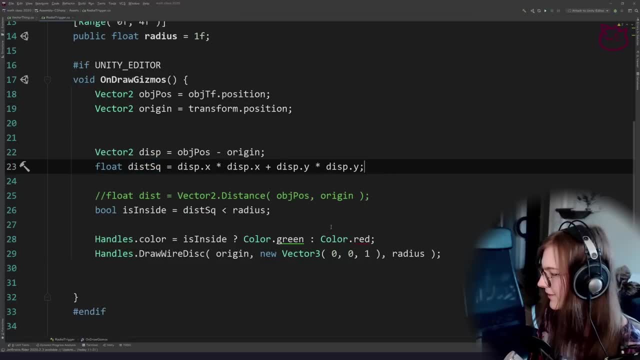 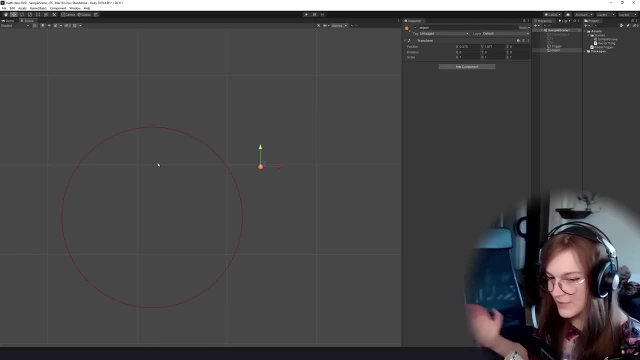 actually have the, the squared distance, not the actual distance, Because if we want to get the actual distance, we need to do the square root on it first. All right, So now we have this weird, weird squared distance value. So now this one is going to be incorrect, right? 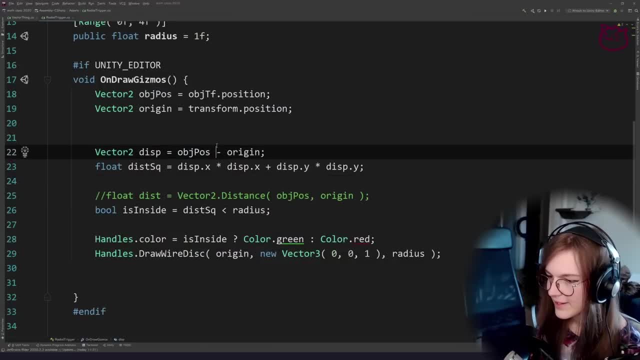 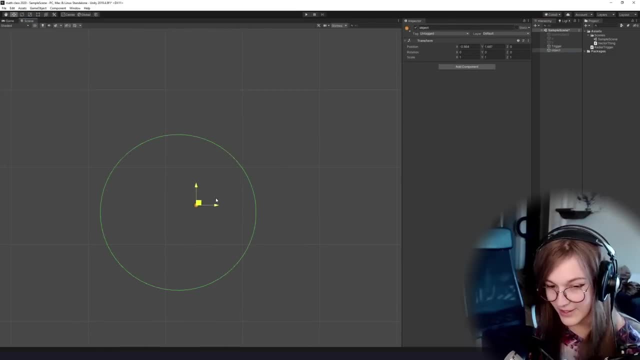 Because we just removed a piece of the math. where we just removed a piece of the math that happens to work. in this case- And this is again important to check for or to test your code Right- The reason it works here is because our radius is one. 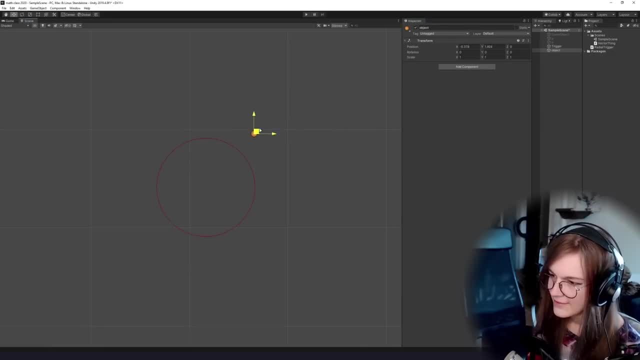 We set radius to 0.5, then now you can see that the threshold is incorrect. It marks it as inside here. And the same thing. if we make the, if we make this larger than one, then it's, it's counts. 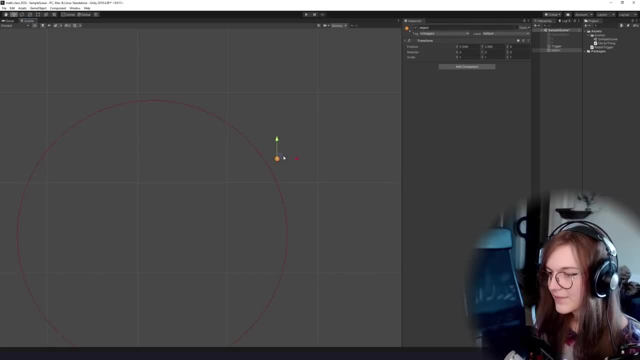 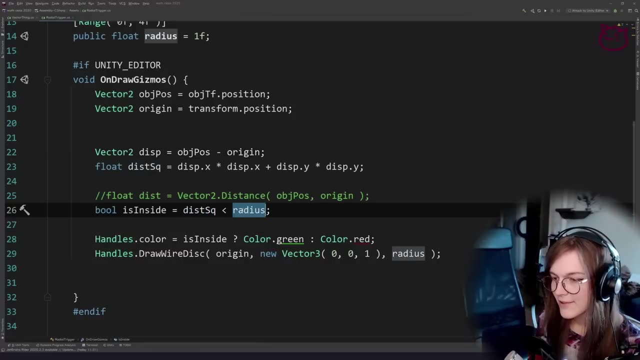 as outside already here, when it really shouldn't do that, Right? So the way to do this is that we're using the squared value here, But the radius we're comparing to is the actual distance. but what we can do is that we can take the radius and square that. 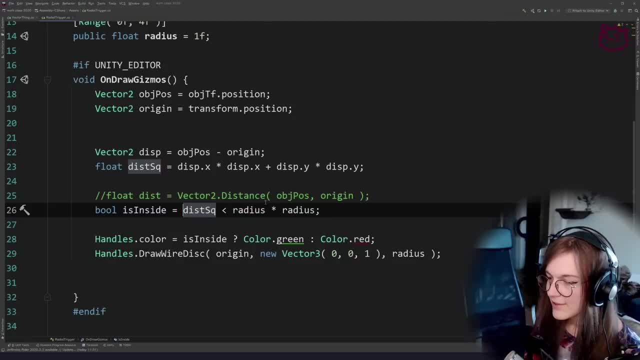 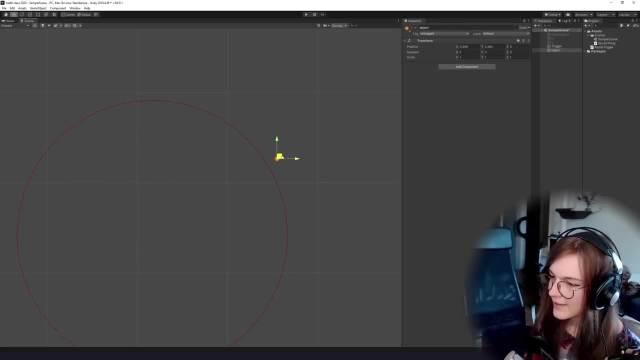 So now both of these are squared. So if we square the radius, we're comparing the squared distance with a squared radius. And now, if we go back to Unity and recompile, this is now correct And everything is like working exactly the way we want to, but we managed to optimize. 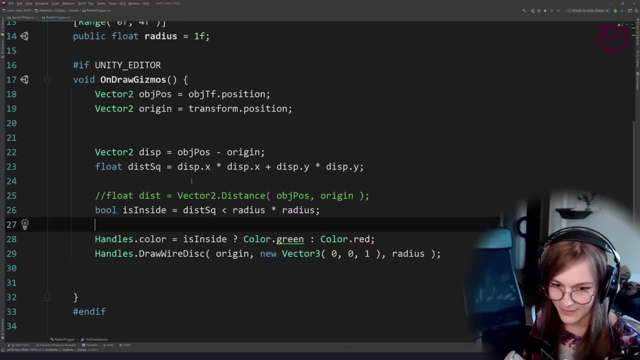 away the square root, Like we're not actually using a square root anymore. All we're doing is one more multiply instead of the square root, which is much faster in many, many cases. So if you're again, if you're doing very performance sensitive code, you can get rid. 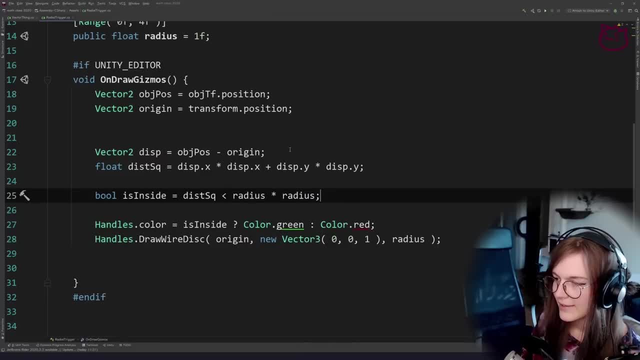 of that square root. Now it's a little annoying to have to type all of this, So there are built in functions for this. So instead of like typing all of this manually, you can get the displacement vector and do squared magnitude. So this is built in. 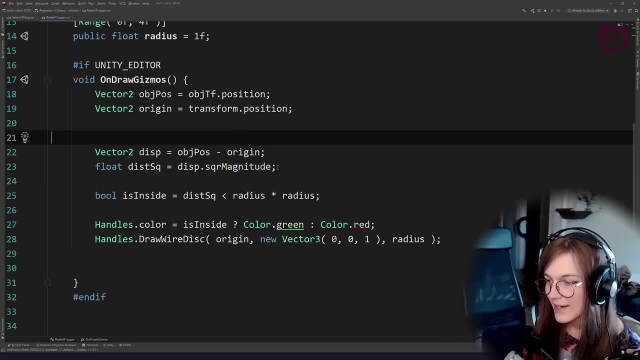 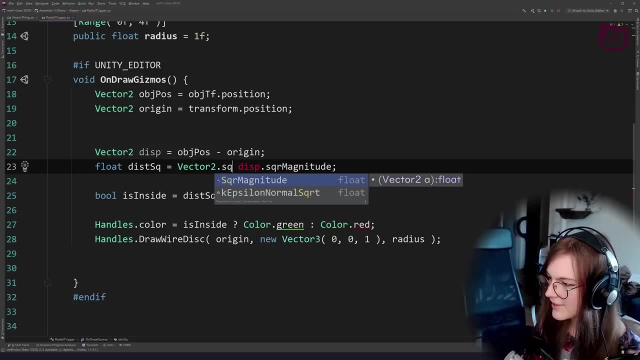 So you can just do squared magnitude, And now you have the- well, the squared magnitude of the distance between these two, And there is also, actually, is there a there's no squared distance, Okay, Well, anyway, this is sort of the squared distance then. 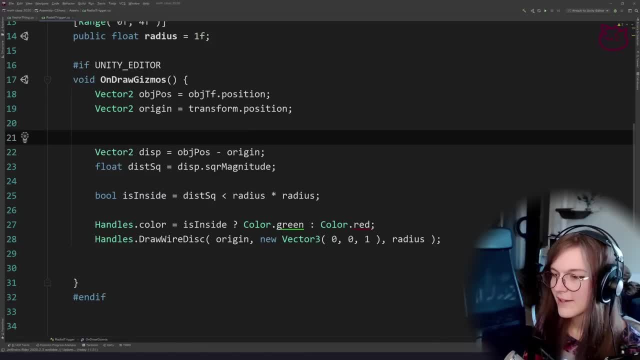 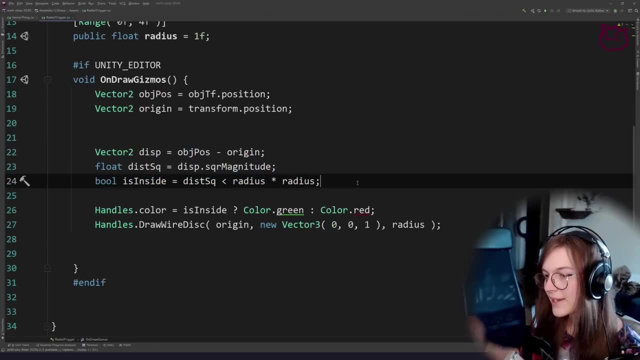 We're just doing the displacement vector manually And then we'll get the square magnitude of that displacement vector right Anyway. so this is a neat little optimization you can do. But one thing that's very important: this only works if you're only checking a threshold. 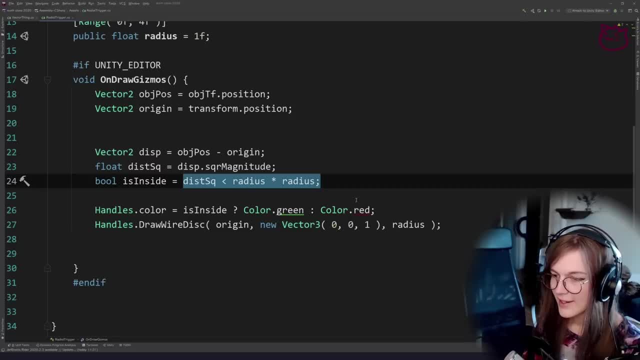 If you need the exact distance, you have to do the square root, because we are no longer calculating the distance. All we're working with is this wonky space that is not linear, right, Actually, let's, I can show you the quick little example. 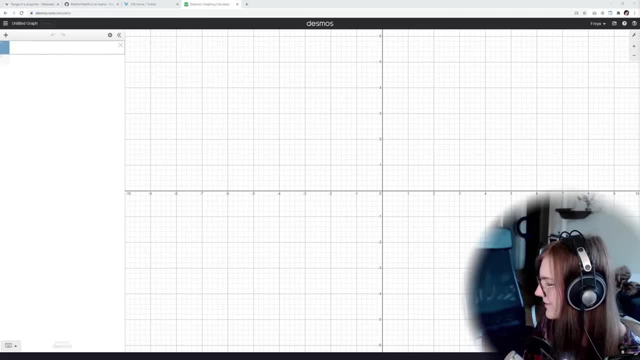 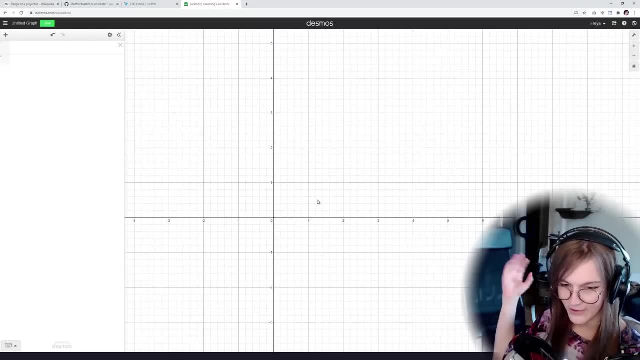 Oh, desmoscom slash calculator. Okay, It's an incredibly useful tool. We're going to use this a few times throughout the course. It's good. You should use it Anytime you want to graph something, All right. So let's say we have our distance. 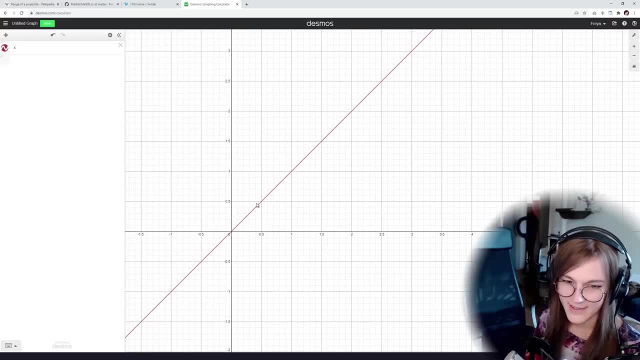 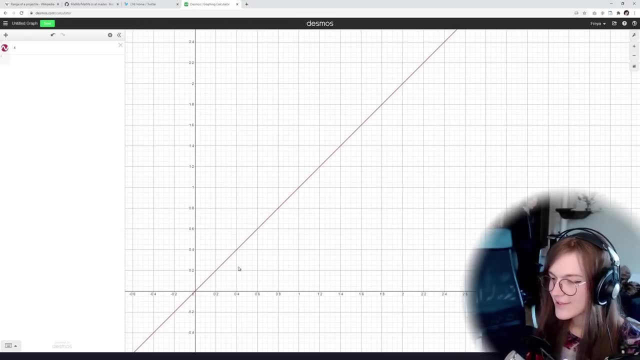 Let's say that's X. So if we interpret this along the X axis, so now we have a value representing the distance as we go further away, right, And obviously it's just going to be. it's just going to be one. 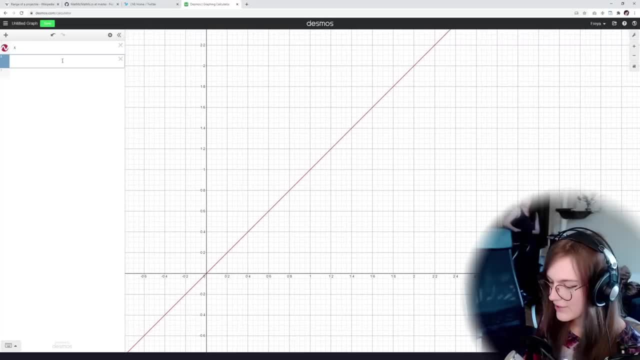 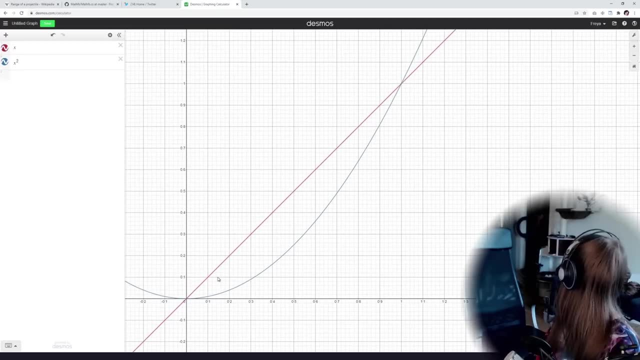 It's a diagonal that just goes up there. But if you do X squared, then you can see that. But wait, are you what? Oh, no, Oh, I'm sorry. Okay, All right. So, like I mentioned, this only works for thresholds. 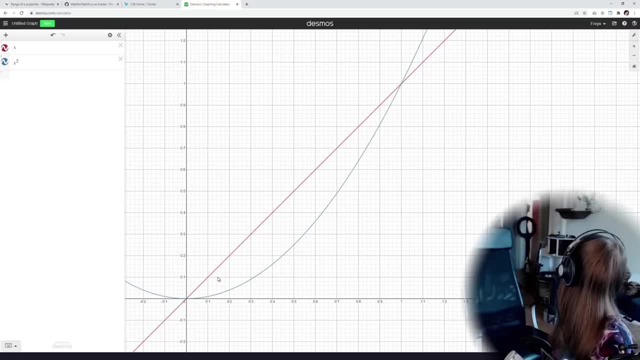 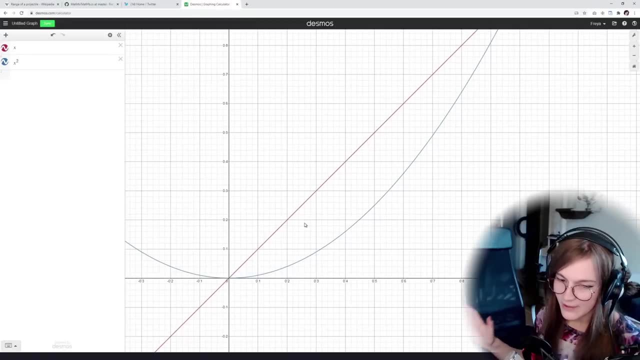 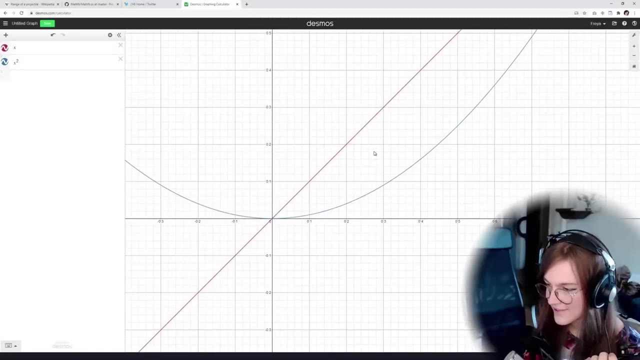 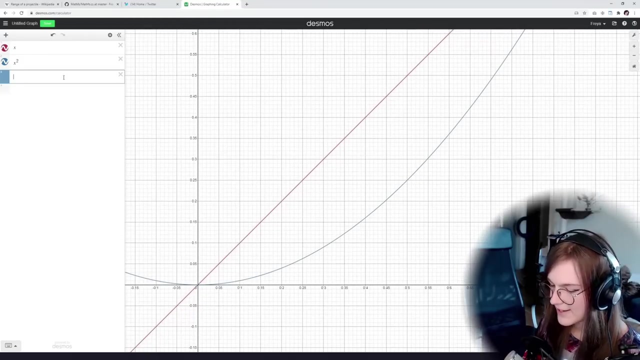 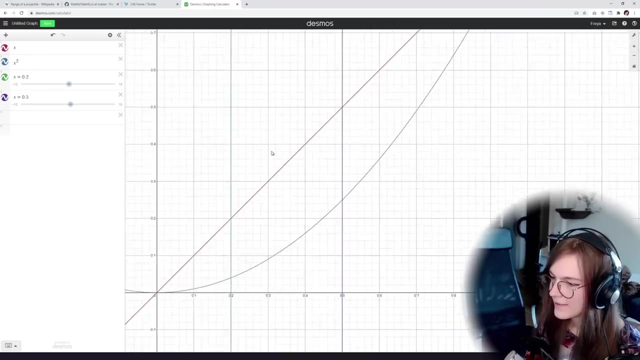 If you want to know the exact distance, then you want the red value here, not the blue value, because this is not a distance value. But if you take any points, Like if you, If you say, here we have one coordinate and then we have another one here, 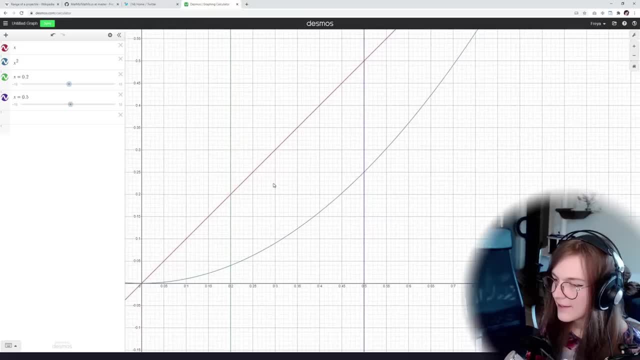 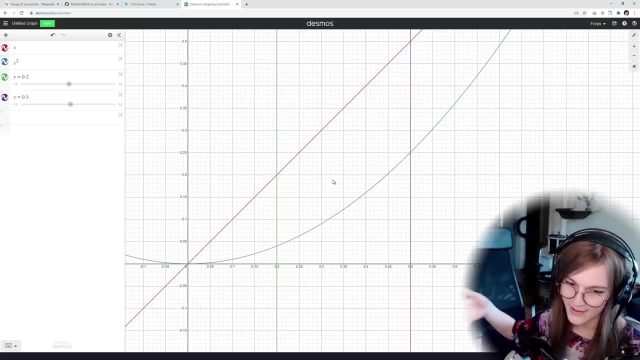 We want to know if you're to the left or to the right of this value. That's going to be true regardless of which of these two curves you're using. This is a little esoteric if you're not, like, accustomed to reading curves, but basically. 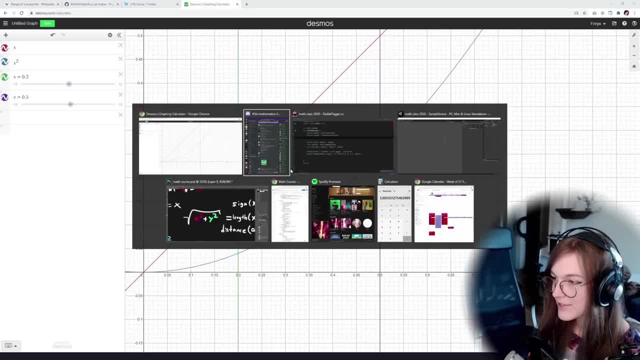 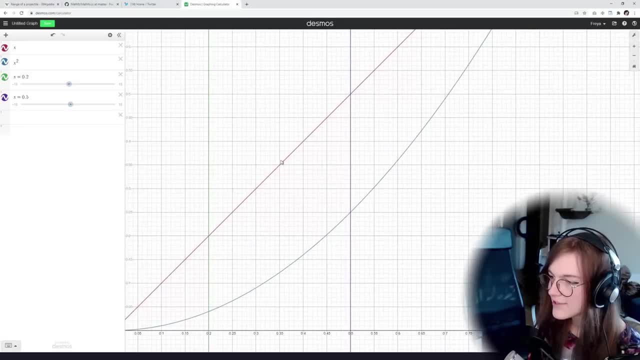 if you want to check if something is less than or greater than something else, which is exactly what we're doing here- we're only checking if it's less than or greater than something. In that case, you can just use the squared versions, because the comparison is true regardless. 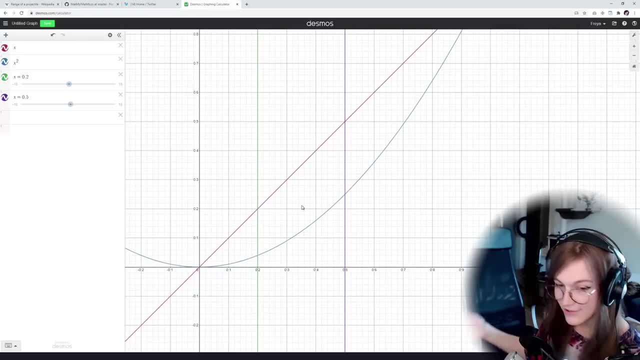 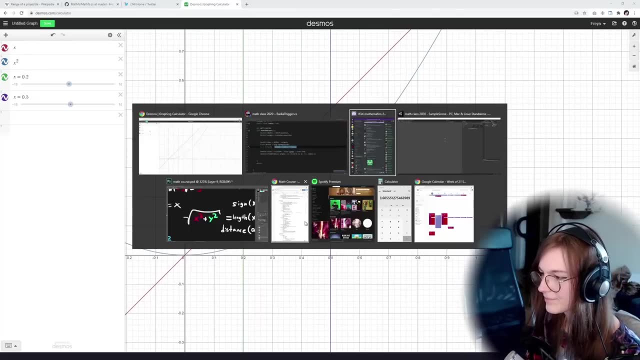 of if you have the square root or not. That's why we can do this optimization, but only when checking thresholds, because the blue line is not an actual distance, It's a squared distance. That was a long thing. Any questions so far? 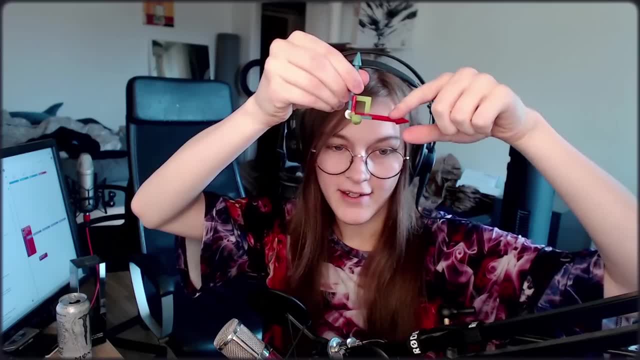 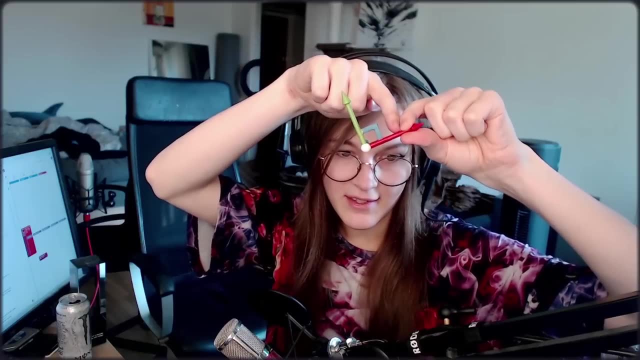 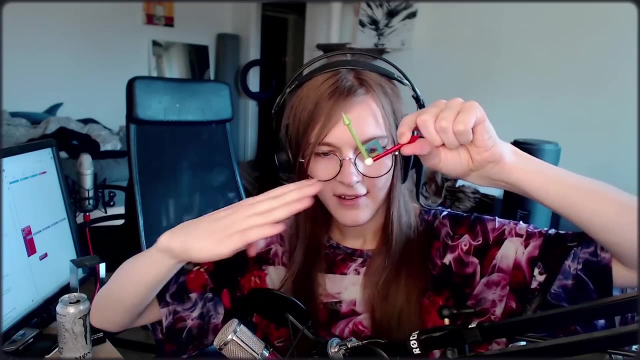 say, your plane is defined by the red arrow here and this is 2D, then the normal is just going to be the red arrow rotated 90 degrees and that's it. If you imagine the plane extending along the red axis, Then you can just rotate the direction of that plane to get that normal. 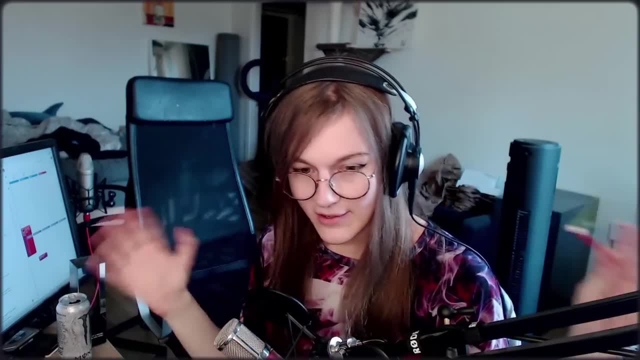 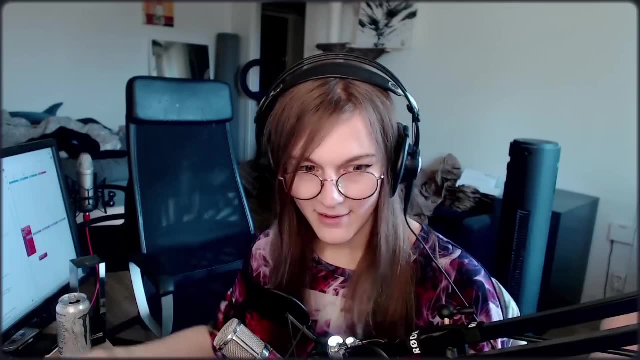 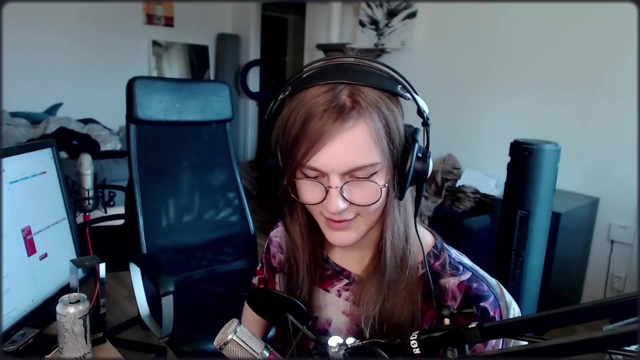 But then again, the thing is that whenever you have mathematical plane, the norm is usually built into the plane so that you can usually get the normal of the plane out. But it really depends on what your plane is defined by. A mathematical plane works in one way. 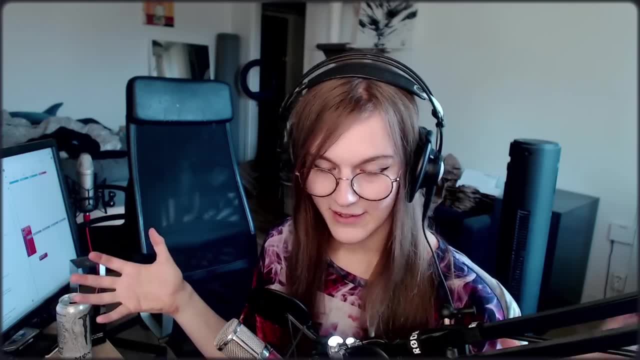 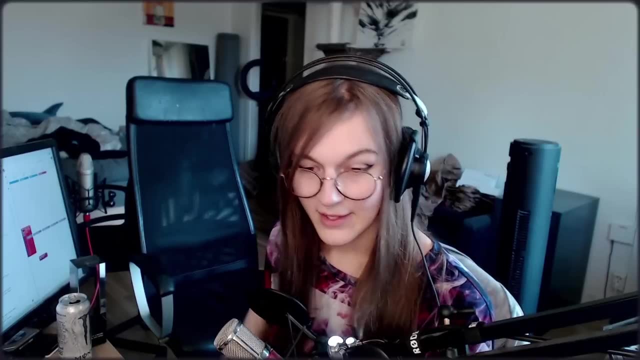 Bertrand Neuha Mans weiter über paradise aus Mittel beliebt. hat man eine 3D-Mathän, 3d mesh, then things work in different ways, right, because now you have triangles and maybe colliders that you need to like- i don't know- raycast against or whatever now. so that works differently than 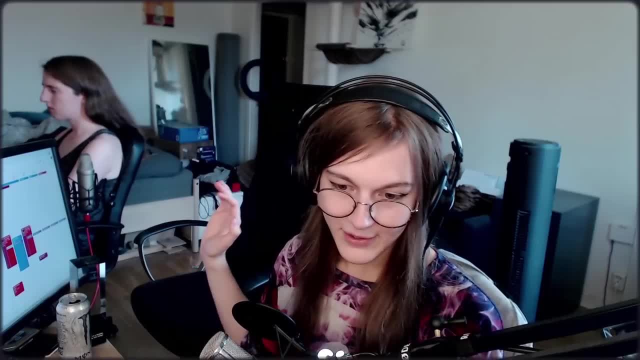 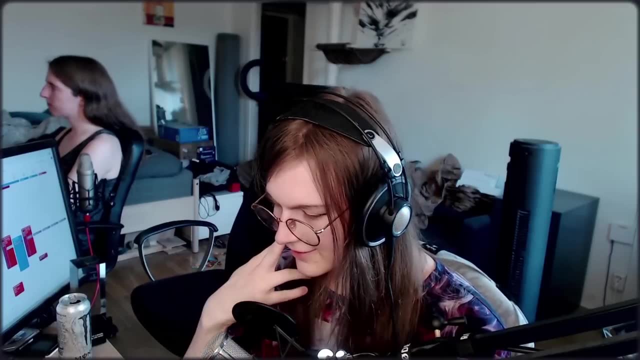 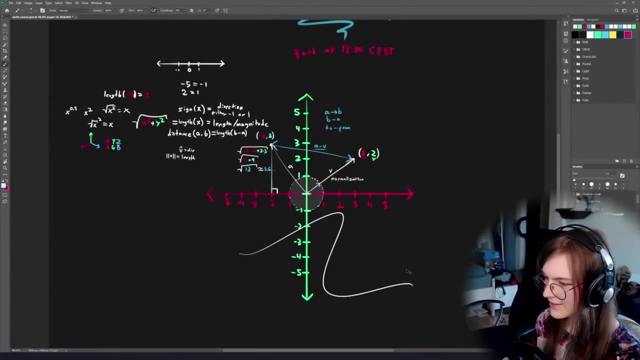 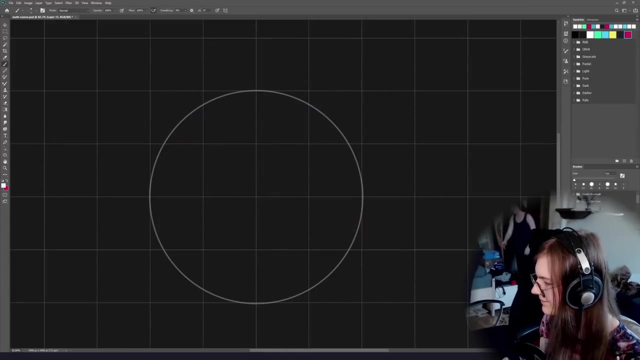 like purely mathematical planes. okay, so the last thing we're going to talk about now, um, before we end today's thing, uh, we are going to talk about the dot product. uh, so, uh, swoosh, i think we might need to clean up this whole thing. okay, there we go. what a good, good circle. um, let's make a new layer. 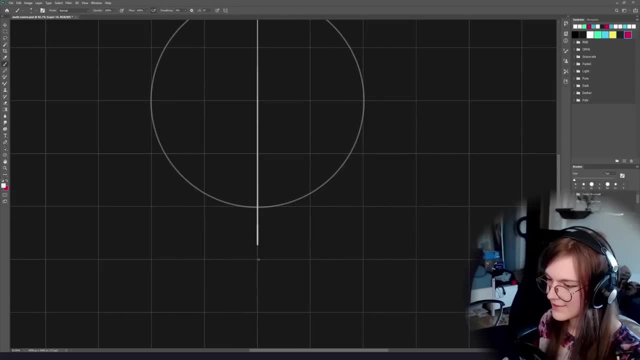 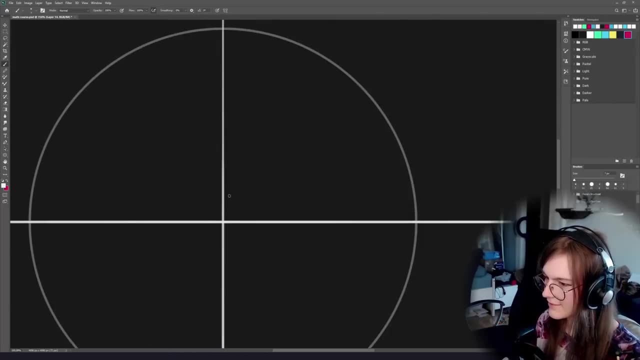 let's draw some lines now. okay, so this is: um, this is going to get very close to trigonometry, but we're not going to have time to talk about trigonometry today, um, so instead, we're just going to talk about trigonometry today. um, so instead, we're just going to talk about trigonometry. 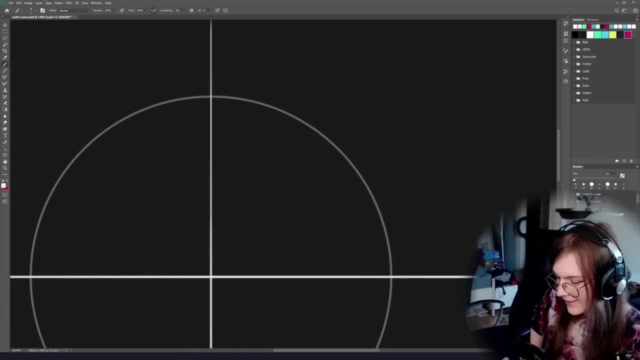 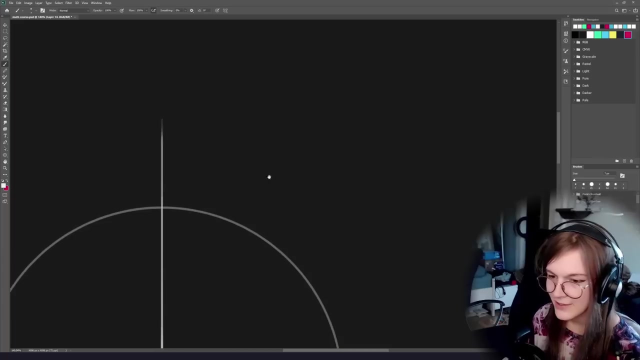 about the dot product, so the dot product. um, when you're talking about multiplying vectors together, um, generally, uh, that is an ambiguous statement. um, so, when you talk about multiplying two vectors, there are many, many different ways that we can like approach that. like, what do you mean by? 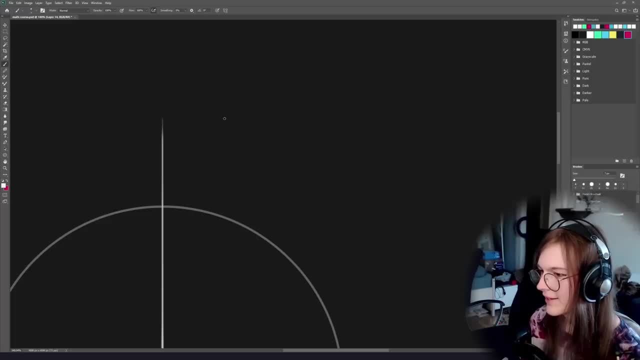 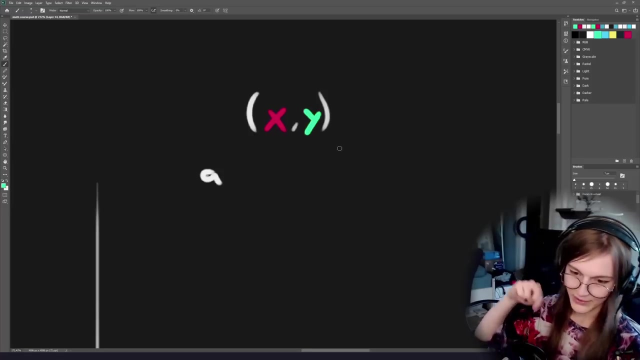 multiplying kind of. the most straightforward one is that, uh, let's say you have two vectors, you have vector a and again the the vectors are, uh, their components. you have the x components and then you have the y component of a vector right, or, if it's a 3d vector, you also have a z component right. so what does it mean to multiply two vectors? 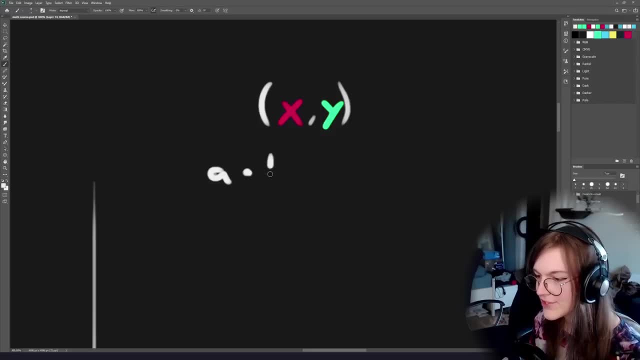 so if we do a multiplied by b, uh, if you just write this sign here, just this little dot um, usually that means that you're doing the dot product between uh vector a and vector b, and the dot product is actually very specific type of multiplication. um, when you talk about multiplying vectors, there are like 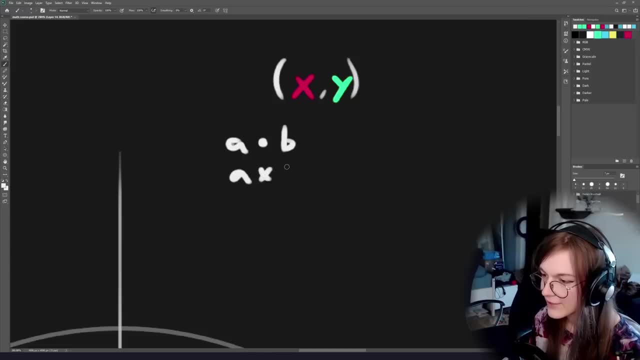 um, there's the dot products, uh, there's the cross products, um, and i do believe the wedge product, but the wedge product is very close to what the cross product does, um, but anyway. so so there are different ways of multiplying them and knowing which one you want. 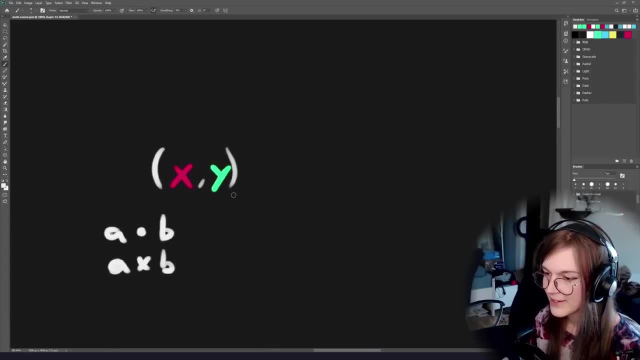 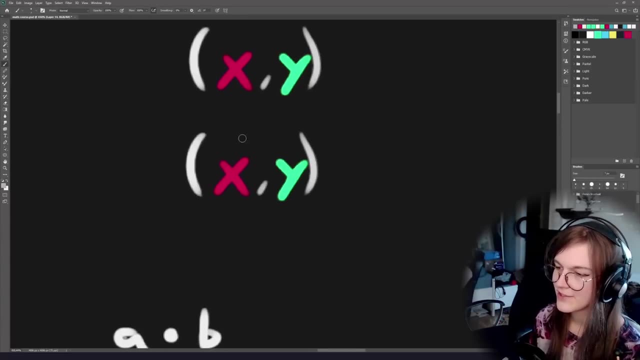 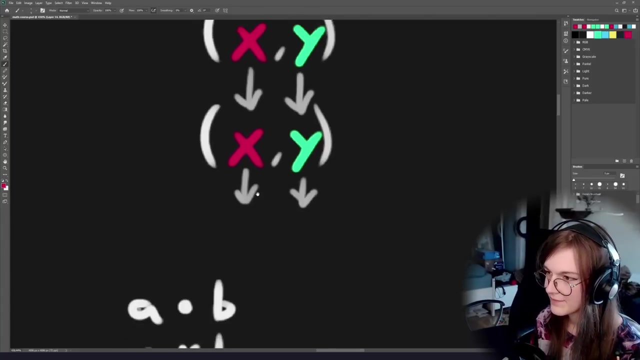 to do is really important. there's also component-wise multiplication, where you kind of take uh, so, so there is there's the component-wise multiplication, where you kind of multiply these numbers together and then you get a third vector out of that. that is the. you know, this x multiplied by this x gives you some value here. and the same thing with 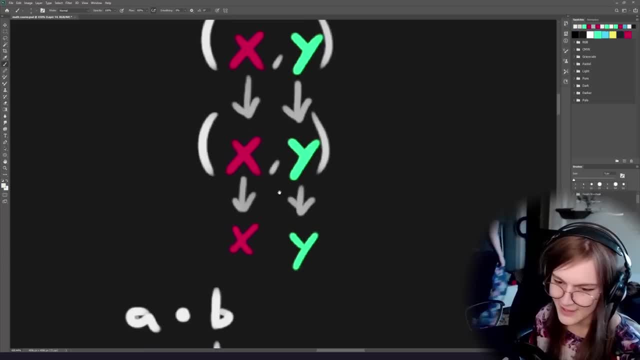 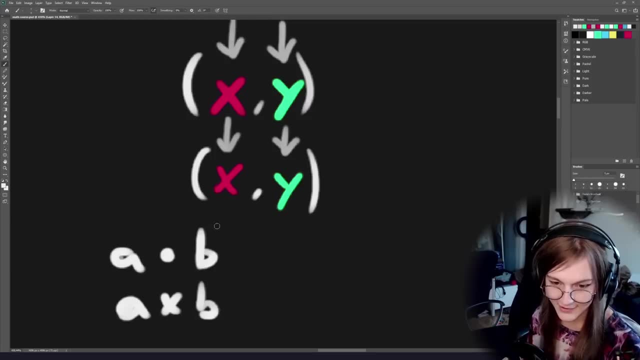 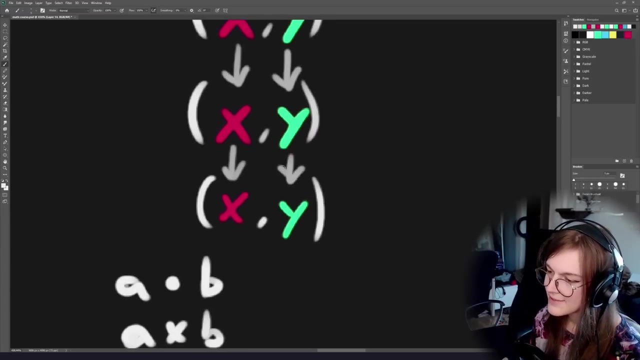 the y component, then it gets some value here. um, this is actually one of the least common multiplication methods. this is almost only used when you want to scale things on like a non-uniform scale or whatever, so so this is usually called component-wise multiplication. um, unity has it in. 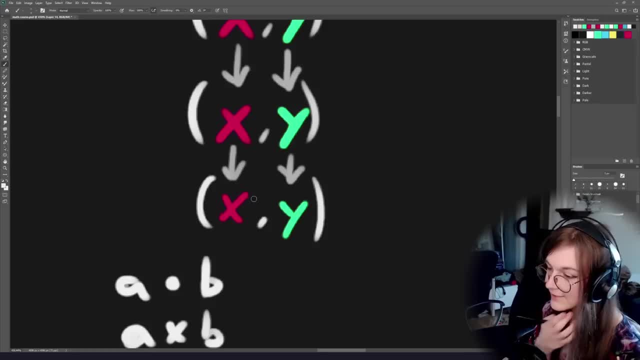 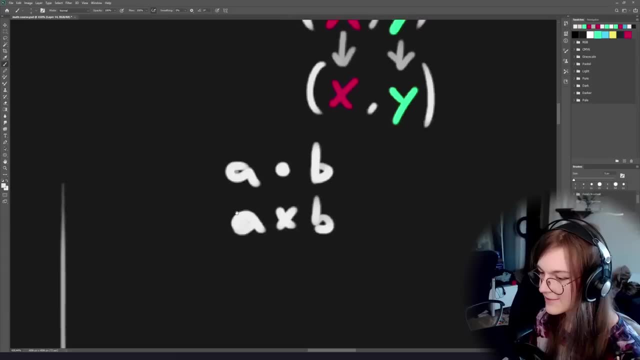 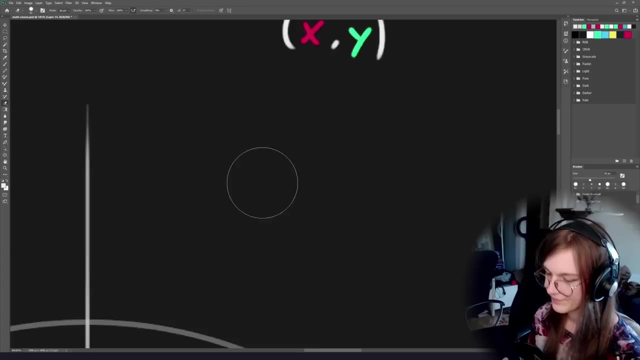 the form of vector2.scale or vector3.scale. yeah, so this is usually a very specialized form of multiplication, that's that's not always very. this is not used very much actually, um, except for scaling. okay, anyway, so let's talk about the dot products. um, now, the way that i usually like, 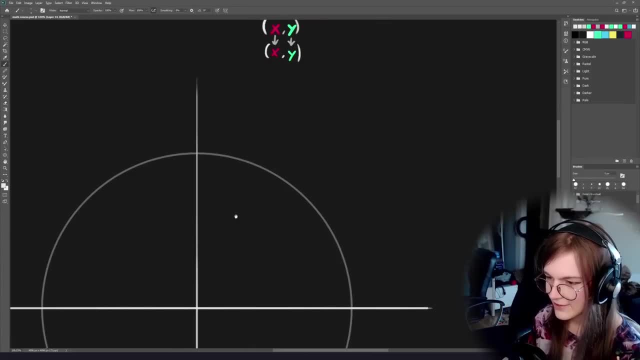 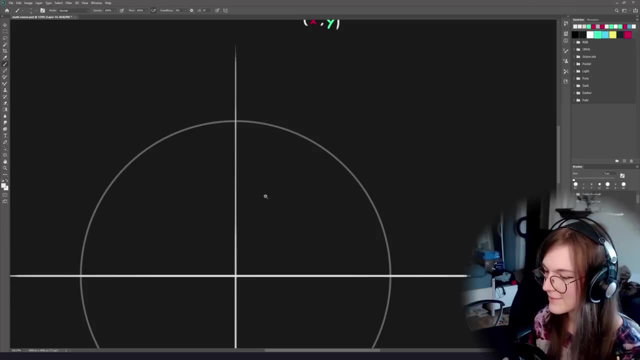 to approach the dot product like. there are many approaches, there's a lot of different approaches. Some people like to go through trigonometry to talk about it, But I like to think about things geometrically because that makes sense to me in many, many ways. 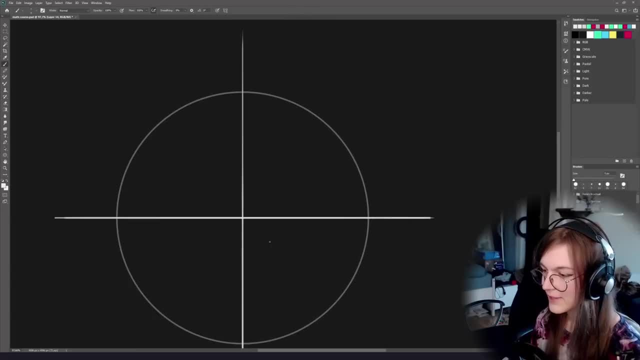 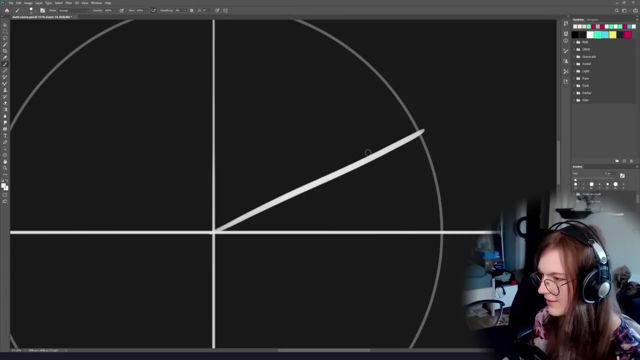 All right. so we have our unit circle. So by unit circle I mean that the radius of the circle is 1.. So any vectors that is pointing to the edge here has a length of 1, right, All right. so if you have, let's see. 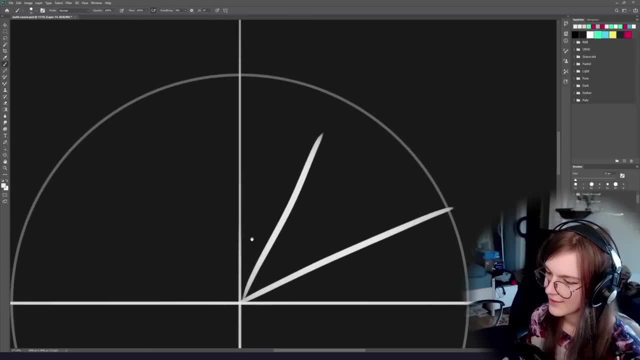 Let's put two vectors here. We have one vector there and another vector here. Actually, let's use separate colors, because that's going to be useful. So we have a vector here, Let's call it A, And another vector- Actually, let's do this one. 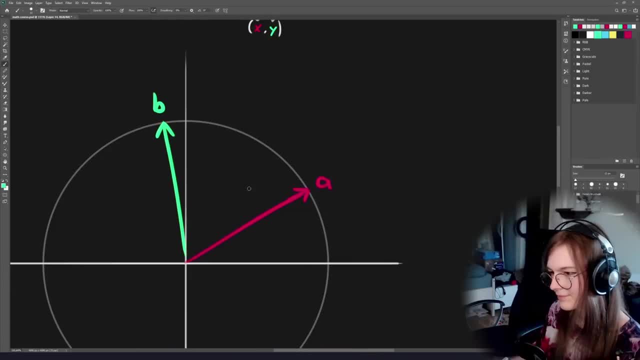 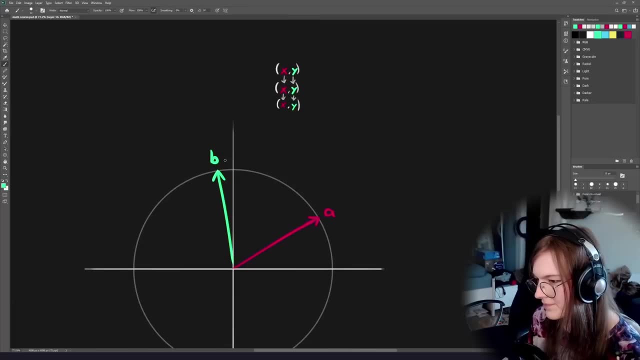 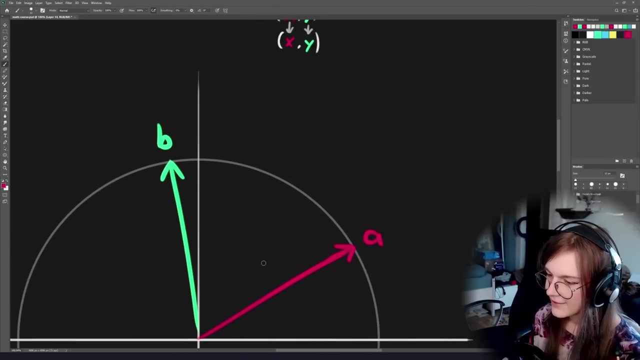 There we go, Perfect And B. So now, if you have, now we have two vectors, right, We have vector A and we have vector B, And then we can ask what happens if we take the dot product of these two vectors. 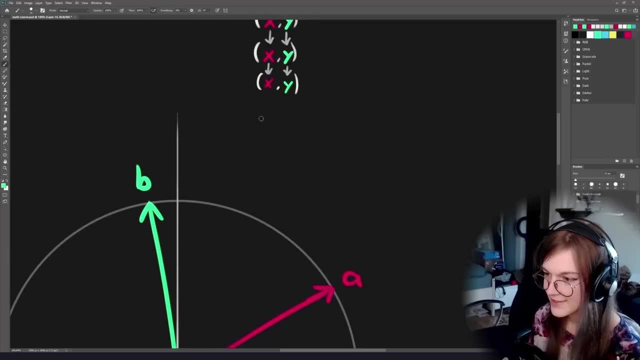 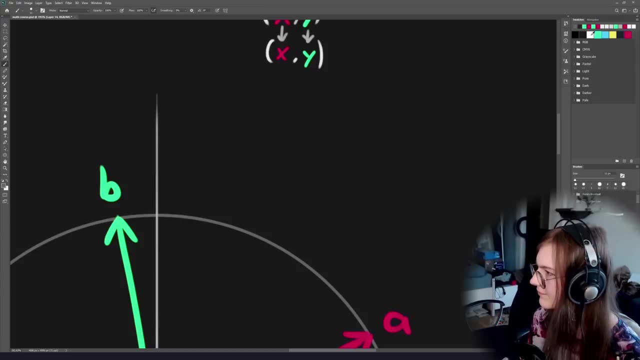 Because the dot product has two inputs. It has two vectors as input, Usually in math libraries and whatnot. it's just called dot, So let's write that down: The dot product between A and B. There we go. Okay, so the dot product. 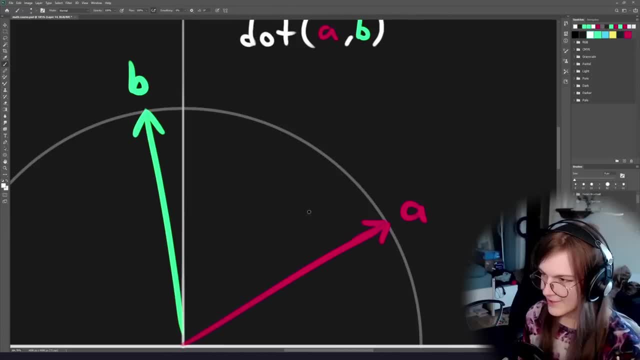 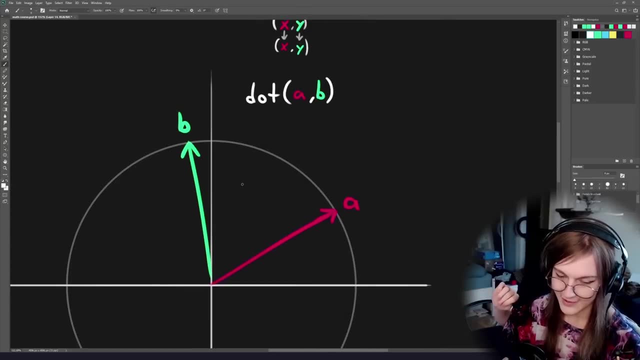 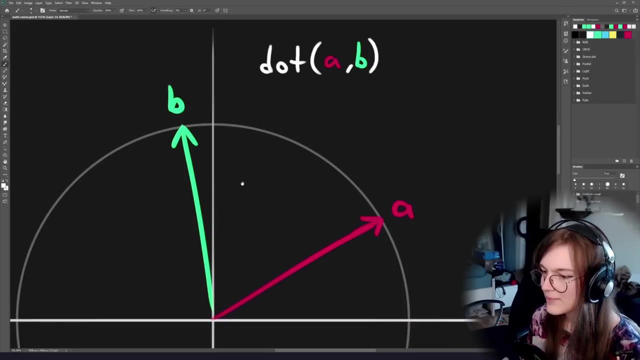 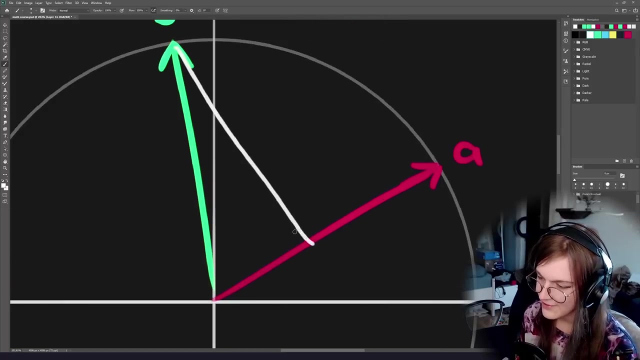 What is the dot product? Geometrically, you can think of the dot product as projecting one vector onto another vector. Okay, So if you look at B here, for instance, if we do the dot product between A and B, what we're going to get is actually, if you can think of B flattening onto A perpendicularly- 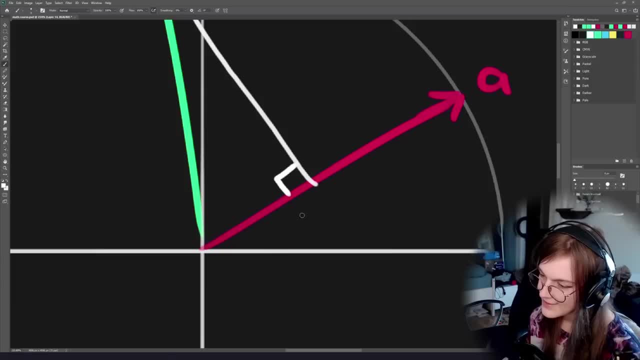 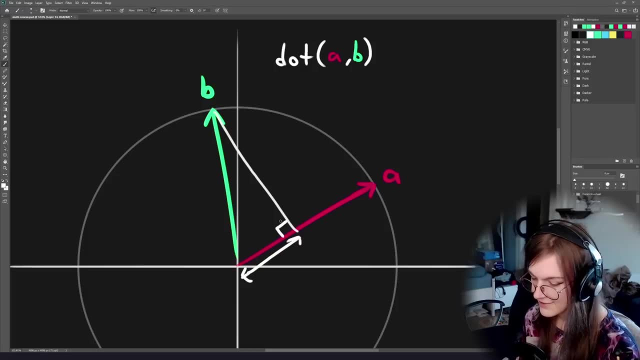 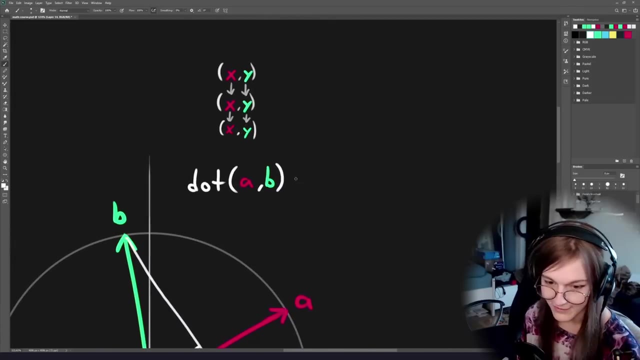 what the dot product gives you is this length right here. So sometimes the dot product is referred to as a scalar projection. Because of this reason It's called scalar, because the result of the dot product is not a vector. The result is just a numerical value. 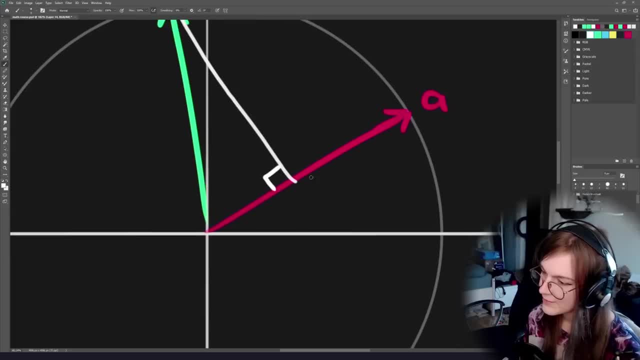 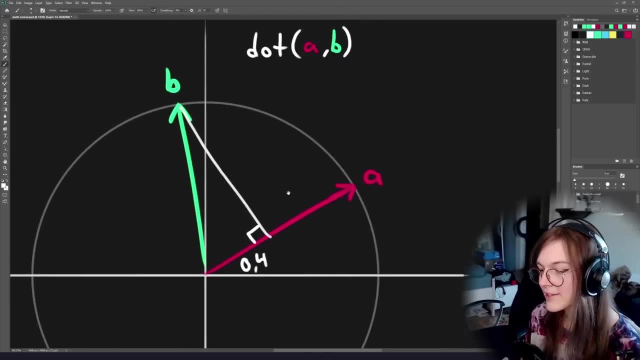 So the dot product between B and A here would be: well, the whole thing is one, So this is less than half. So I guess this is like 0.4 or something, So it's approximately 0.4 in this case. 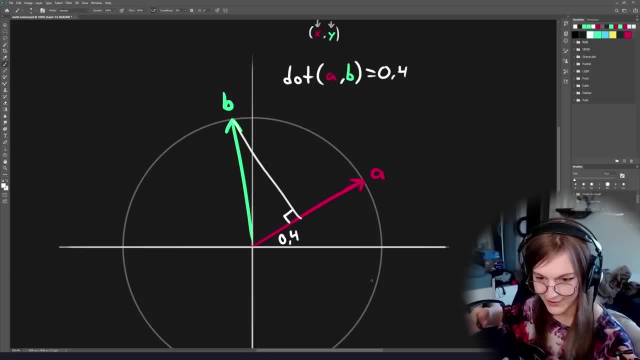 Okay, So you can sort of think of it as projecting one vector onto another. Now there are some caveats. For this to work, A has to be normalized. This one has to be a length of one. You can change the length of B. 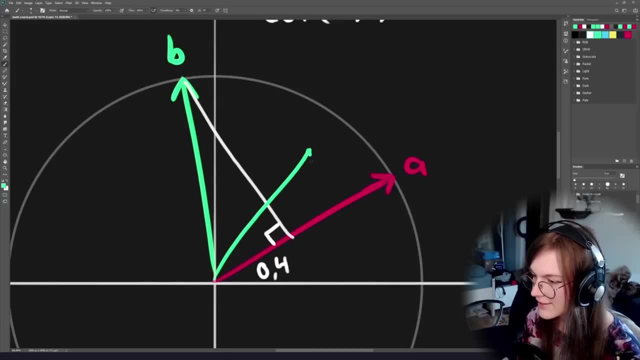 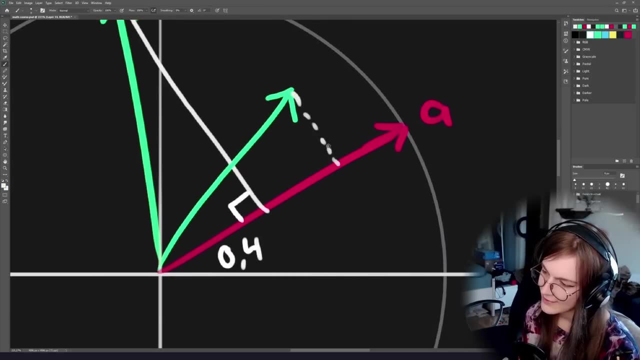 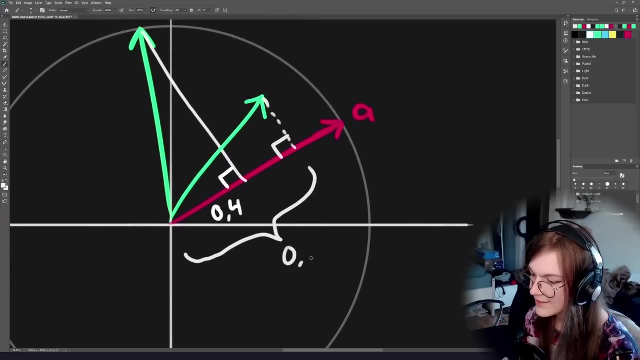 So if you say, make B this vector, now the length of B is not one, But the scalar projection is still going to be the projected distance along here, Right? So in this case it's going to be like 0.8 or whatever. 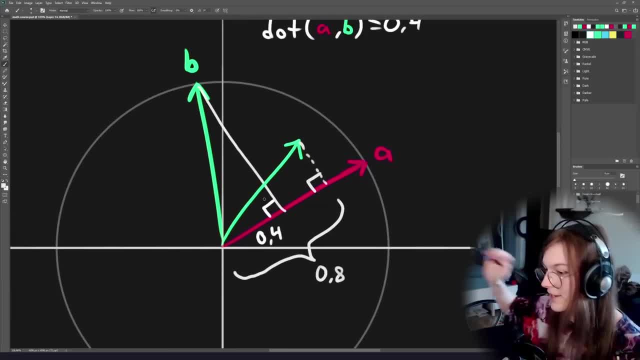 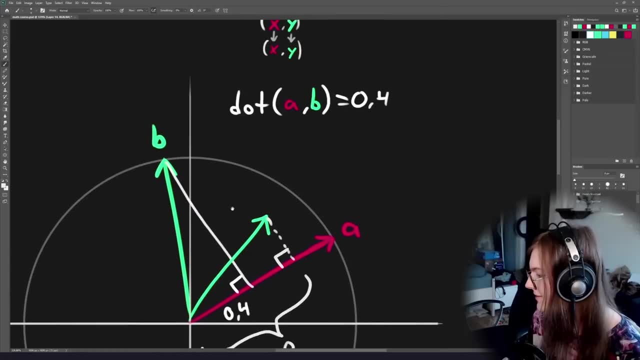 Okay, So that's what the That's a very, That's a very like, simple way of like visualizing what the dot product does. It projects vectors onto each other And in this case, if you reverse the order of A and B, you actually get the same results. 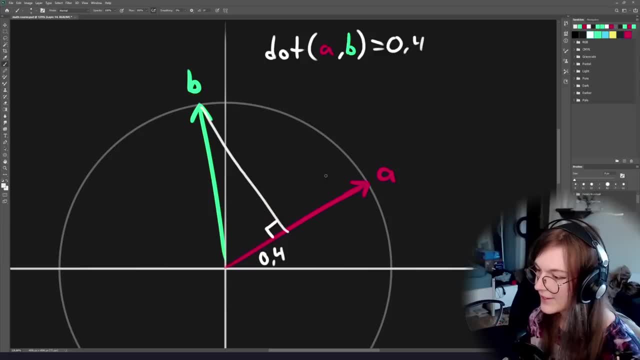 So this one. it doesn't matter what direction you do this in, Because, again, if you do this the other way around, then we're going to do a 90-degree projection onto B, And that gives us this distance right here. 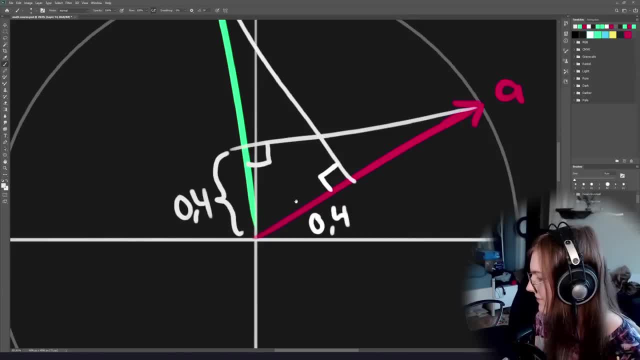 Okay, And that is also 0.4.. Right, So it doesn't matter what direction we do this in. All right, So you can swap those. It doesn't matter, But you still get like a valid value out of that. 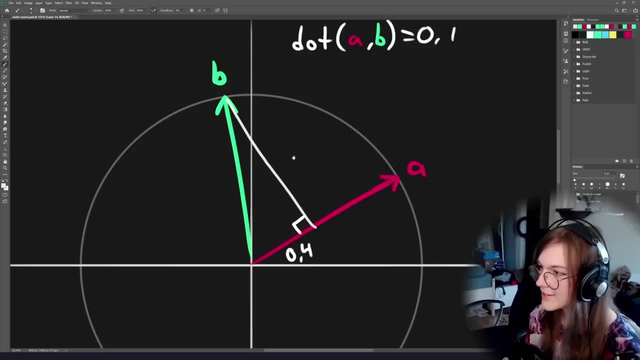 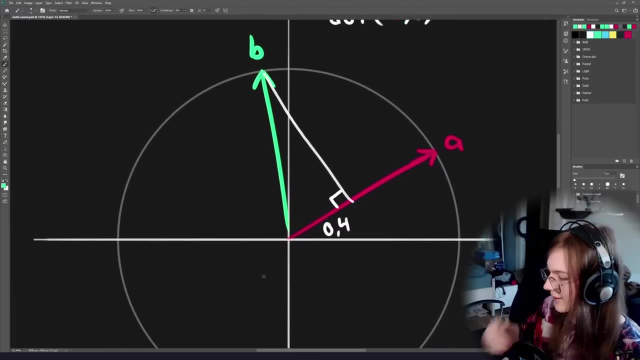 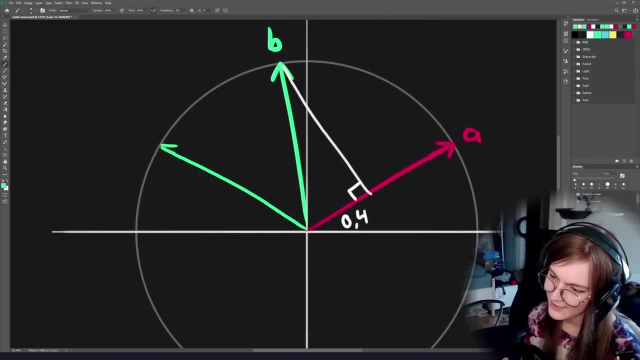 Right, All right. So that's what the dot product does. One thing to note, though, is that the dot product can be negative, So it's a little bit misleading to call it a distance. So, for instance, if we have this vector as our B. 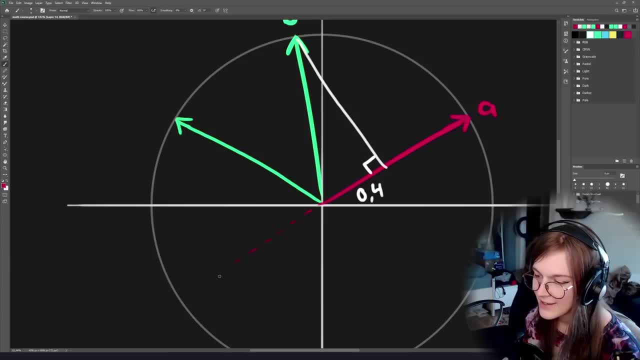 then what's going to happen is that the dot product is going to be negative. So what's going to happen is that it's going to project against the kind of the infinite line here, Right? So in this case it will be the same thing. 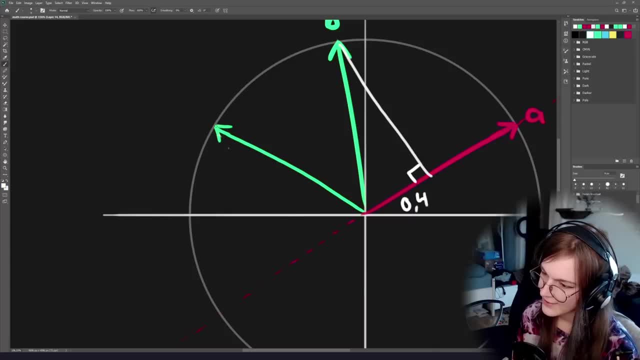 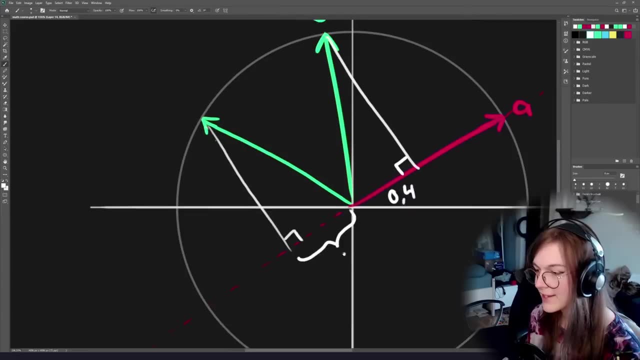 It would project against the other vector like this 90-degree angle, And then you would get again. you would get this distance, But in this case it's going to be negative. So you can sort of think of this as a signed distance in this case. 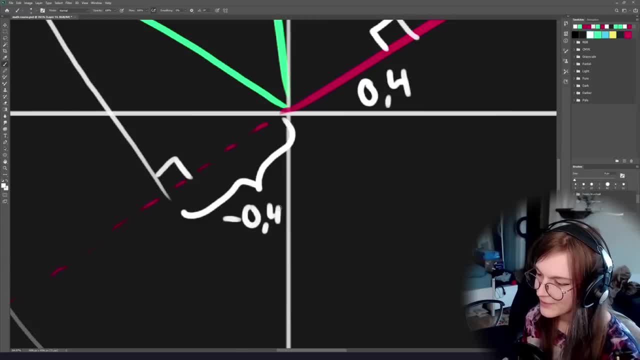 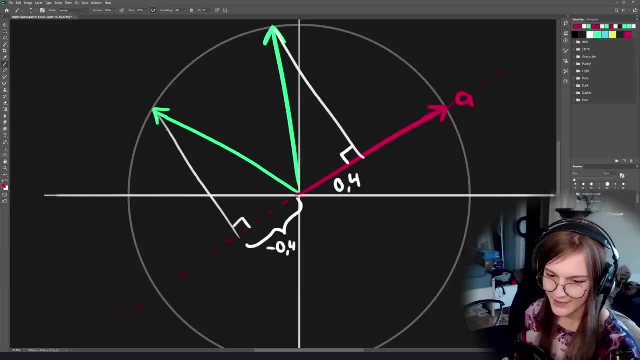 Right, So this is a negative 0.4.. So here's a very useful way of thinking about this. Now, if you look at A here and you look at the values we have, we have 0.4, we have negative 0.4.. 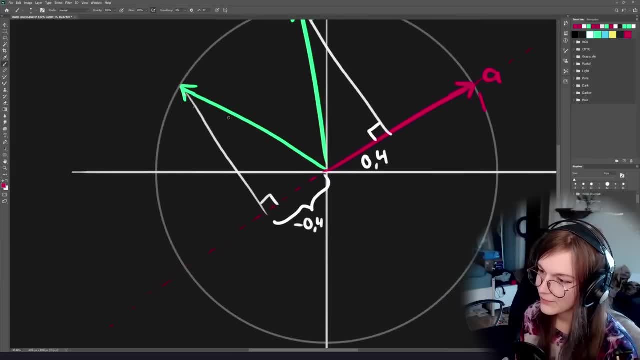 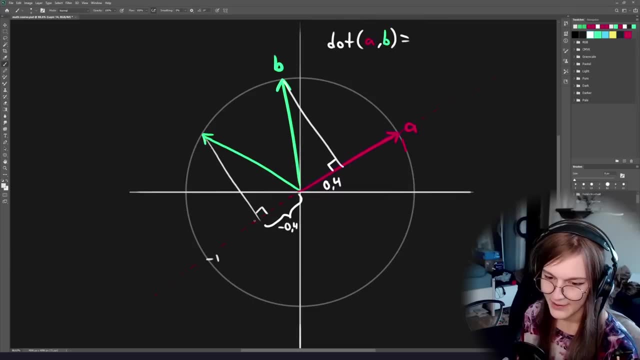 It's 1 over here And if we were to do the dot product where they're completely opposite of each other, we would get a value of negative 1.. Right, And you know how. we've talked about a number line before, right. 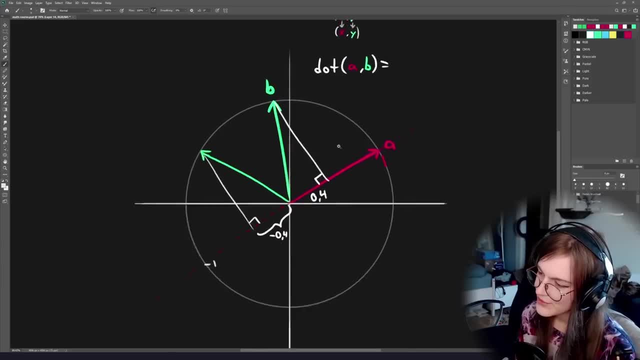 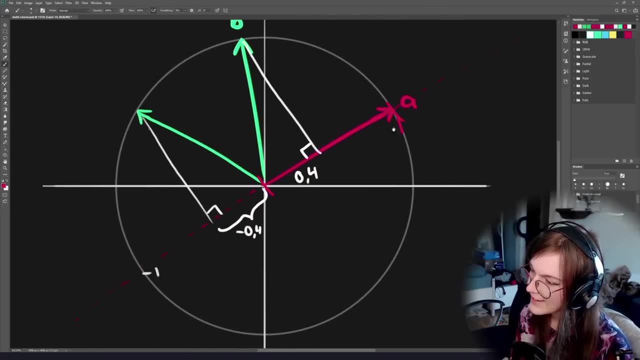 If you think about it, B projected onto A is kind of a way of getting a number on the number line of A Right. So you can sort of extend A and consider that to be a number line Right, Sort of like this. 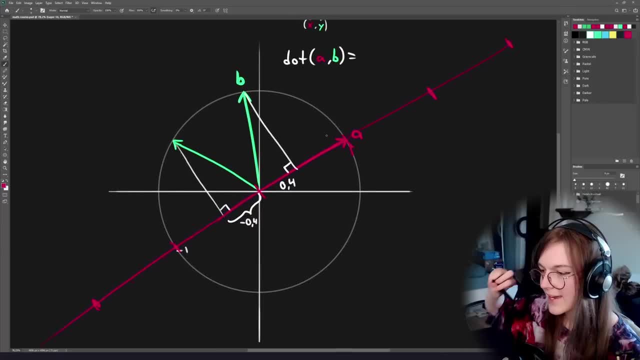 So when you project it onto that, you kind of get the coordinate along the direction of the axis of A. So this is kind of a very nice way of just converting something to some other coordinate, And this is actually used if you want to do space transformation. 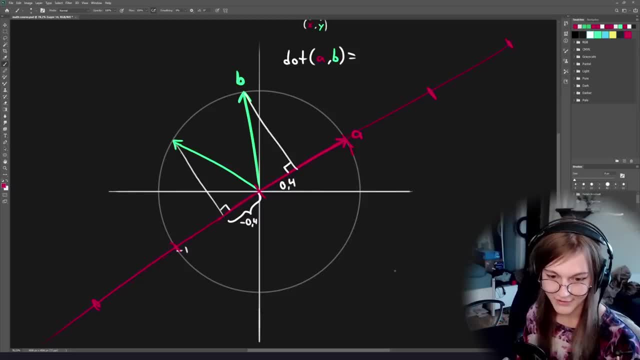 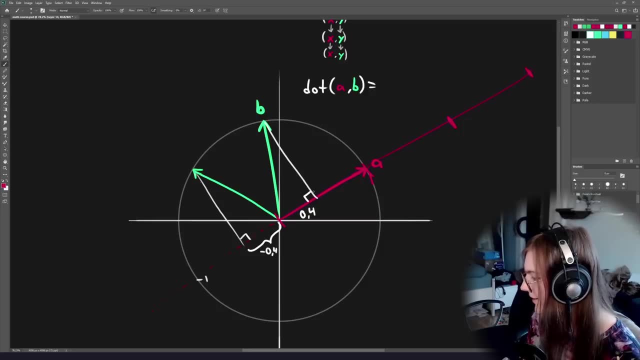 which we're going to talk about next time. This is used for that, for instance: Okay, Where do you use dot? I'll get into that very soon. First, I'm just going to talk about how you do the dot product. 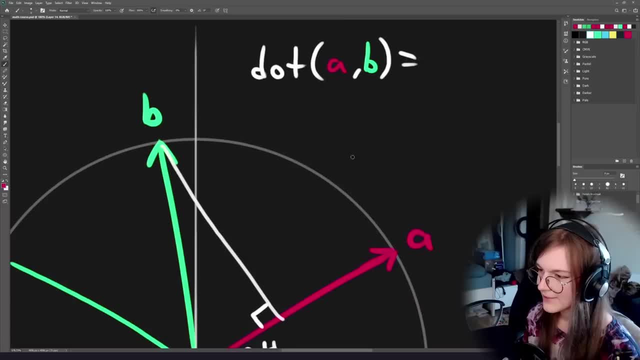 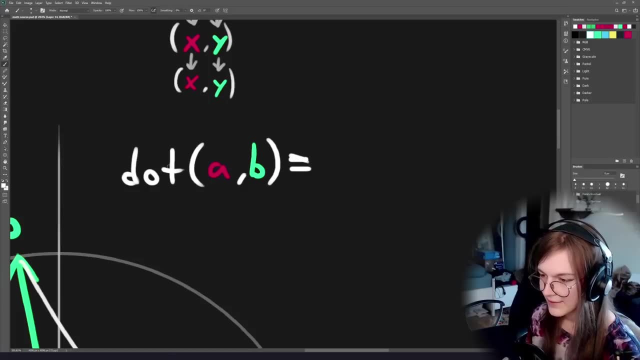 Like: how do you calculate the dot product between two vectors? It is very, very simple. It's like surprisingly simple for something that is incredibly useful. So the dot product between Vector A and Vector B- This looks like it's not equals. 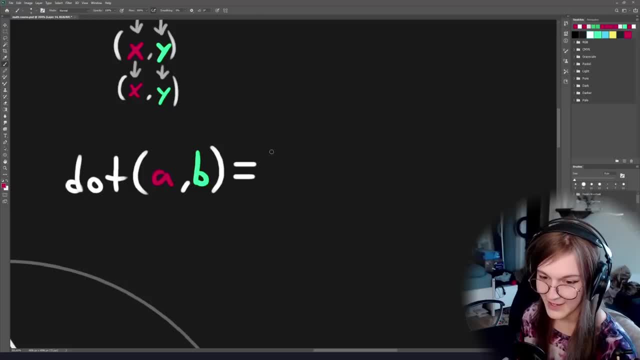 So the way to get the dot product- Well, the actual practical way is that you use the dot product function in your vector library. But if you want to do it manually, you would do A dot X as in the X component of the A vector. 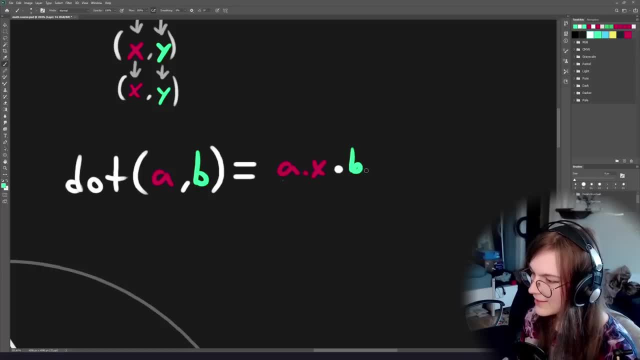 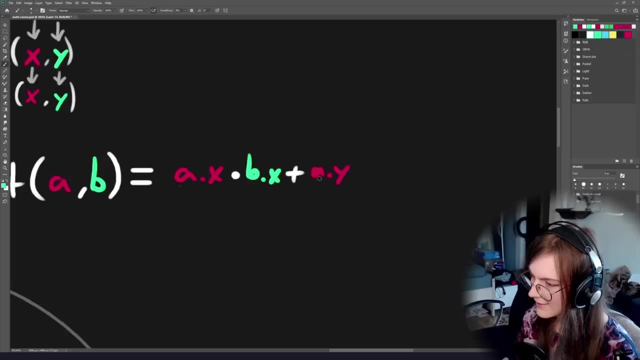 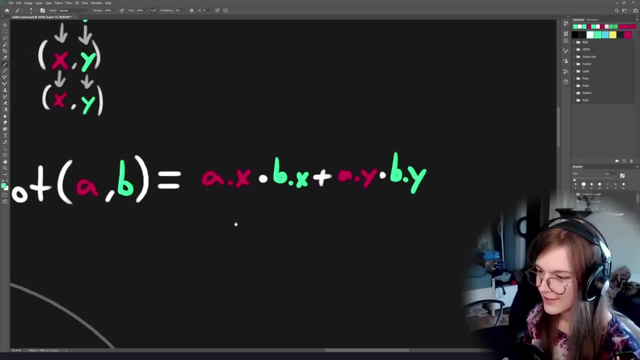 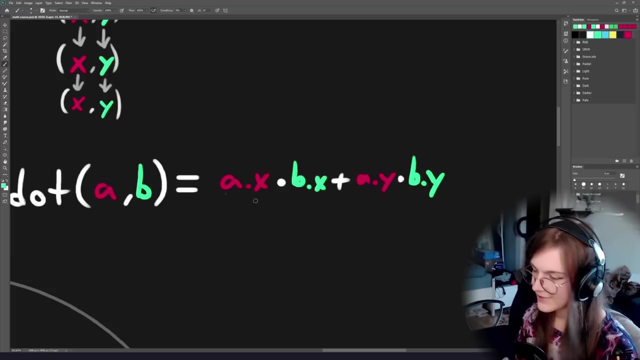 And then you multiply that by B dot X, And then you add A dot Y And then multiply that by B dot Y. That's it. It's very straightforward: Multiply the X components and then add the multiplied Y components. There's not much more to it. 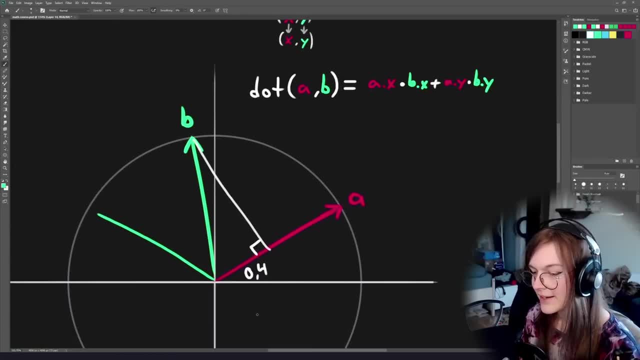 So that's how you get the dot product between two vectors. Now again, this projection example is only valid if one or both of your vectors are equal. If one of them is normalised, it doesn't quite work out if none of them are normalised. 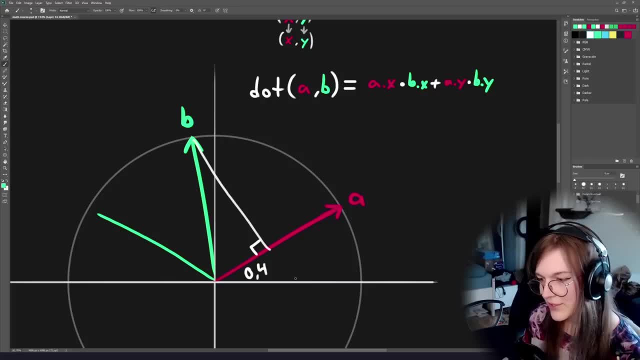 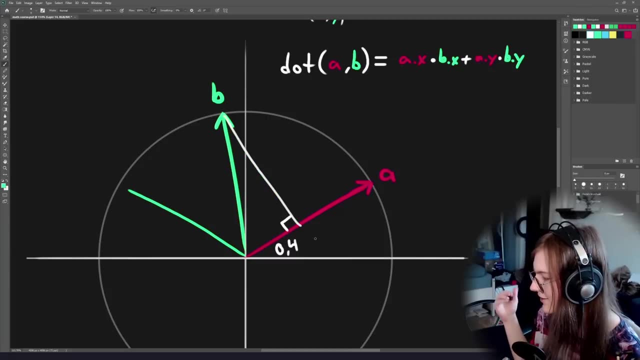 Because then it doesn't really project, Because then it projects and scales that distance. So it's good to keep in mind that the projection interpretation mostly holds, if you're doing, If one of them is normalised. So again, the number line example kind of presumes that A is normalised. 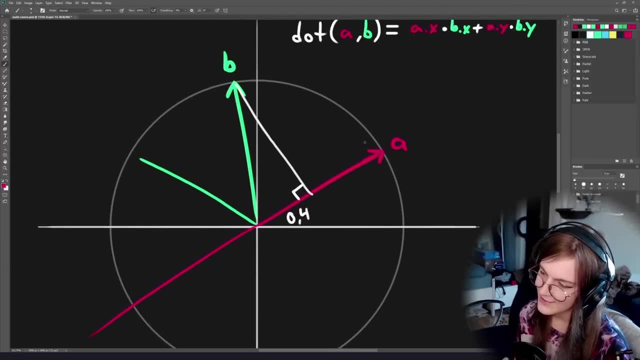 Because then you're kind of getting the B coordinate along the vector, The vector of A. Okay, Another useful way of looking at it is that Let's see, Let me erase some things I'm erasing too much. Why did I draw these on the same layer? 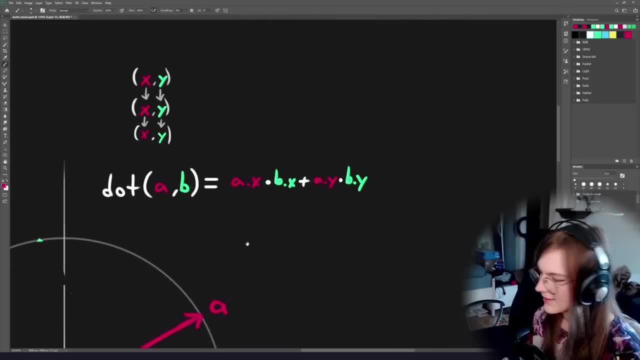 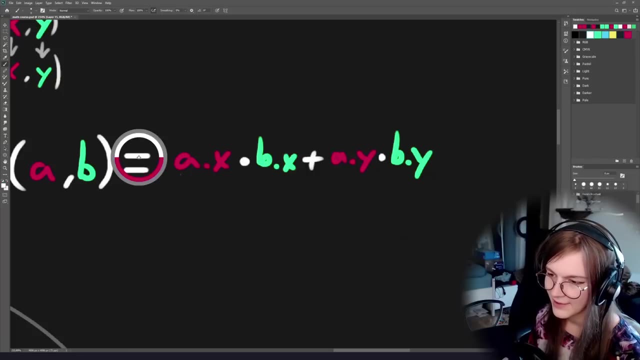 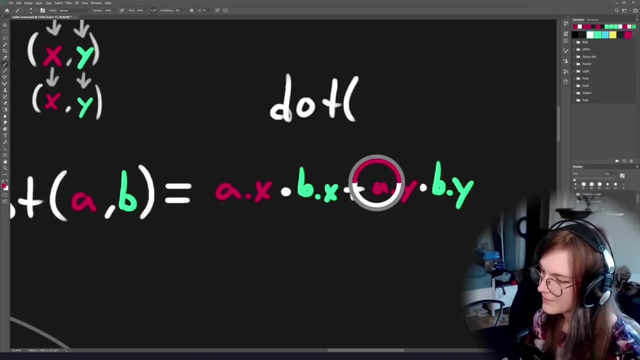 It's fine, Everything's fine. Oh yeah, Like, someone is mentioning the square magnitude, This also happens to be the way that you get the square magnitude of something. So if you, So, if you do the The Dot product between A and A, 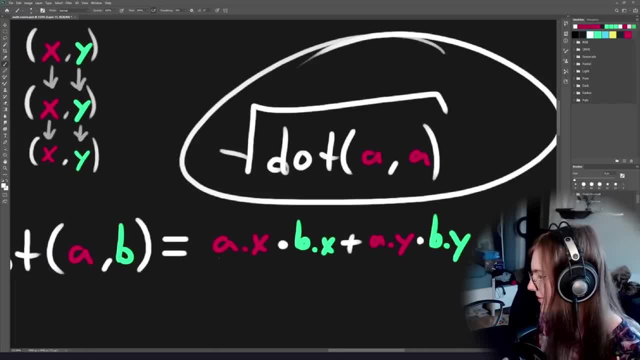 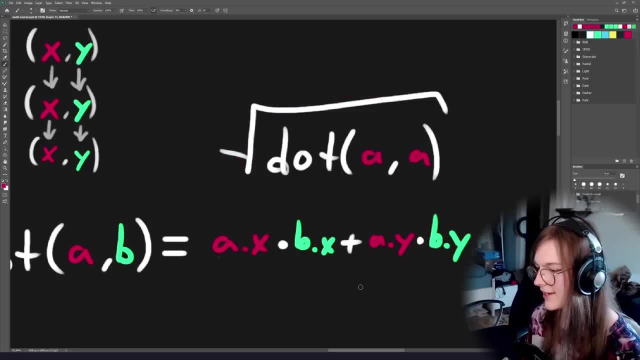 And then you do the square root of this. You have a distance function. This is mathematically equivalent to getting the distance or the length of vector A. So it's kind of a shorthand to do that. And if you use the same vectors for both inputs for the dot product, 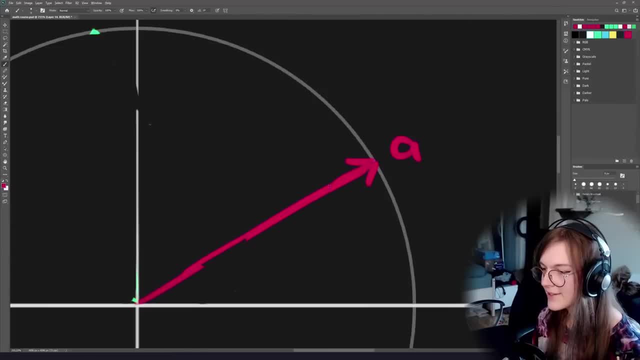 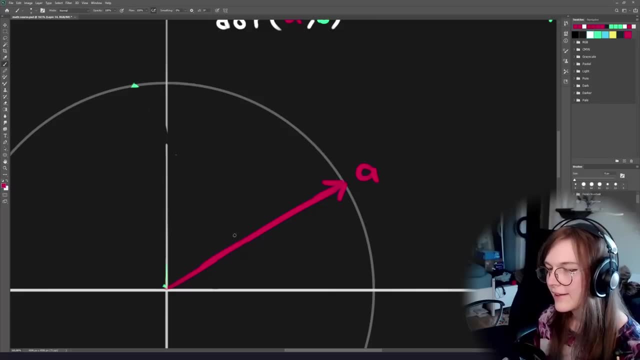 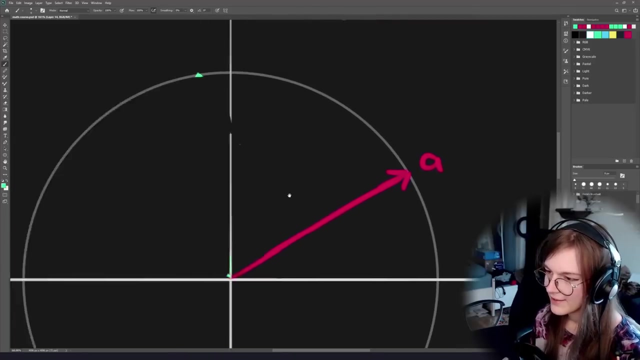 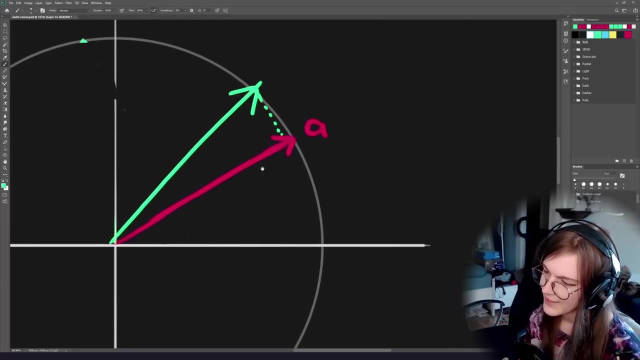 Okay, So here's another way to interpret the dot products. So the dot product can also be used to kind of figure out how close are these vectors to each other. So if you think about A here And you have your vector B, When you project this one you're going to get a value that is very close to one. 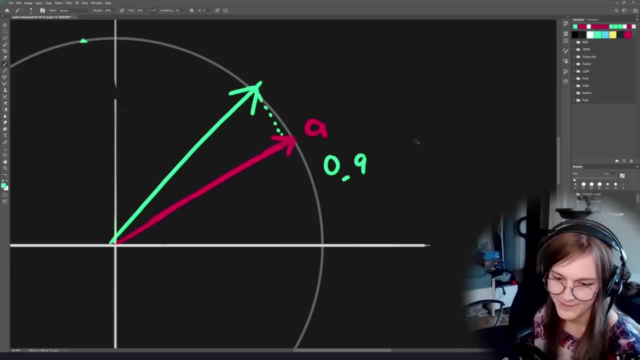 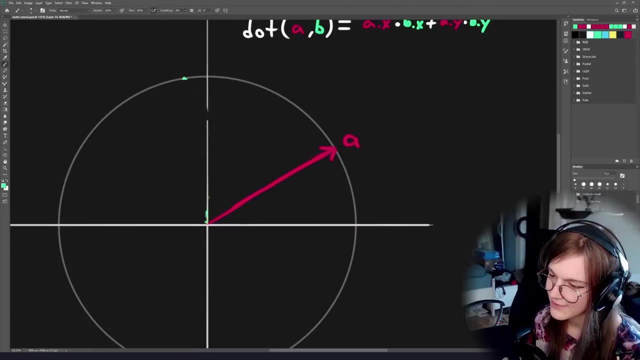 This is going to be like 0.999 or whatever. If they are exactly equal, As in, the vectors are the same and they're both normalized, The dot product is going to give you one. So if we can kind of think about what happens when you rotate this vector around, 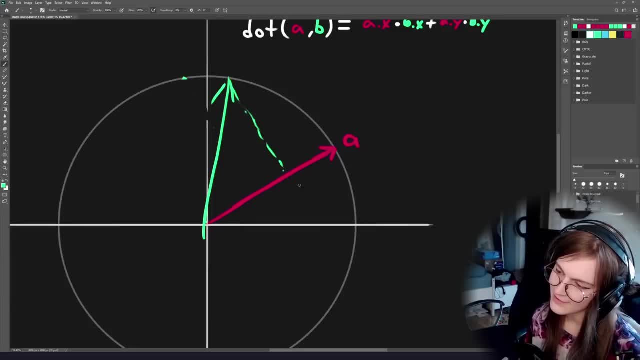 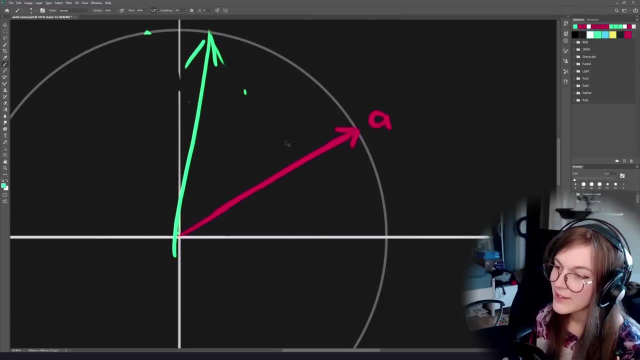 If B is pointing here, We're going to get a lower value in the projection Right Because it's moving toward the center now. So this is going to be 0.6 or something And then, when you kind of imagine, keep rotating this one. 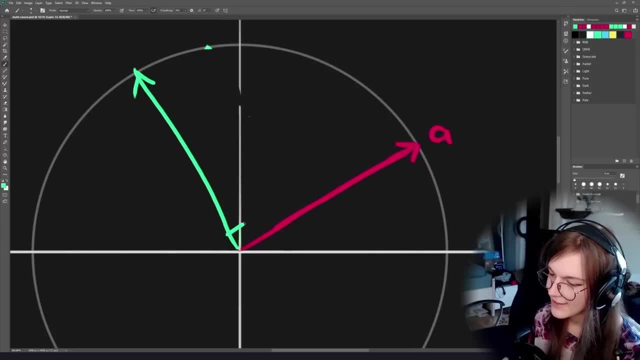 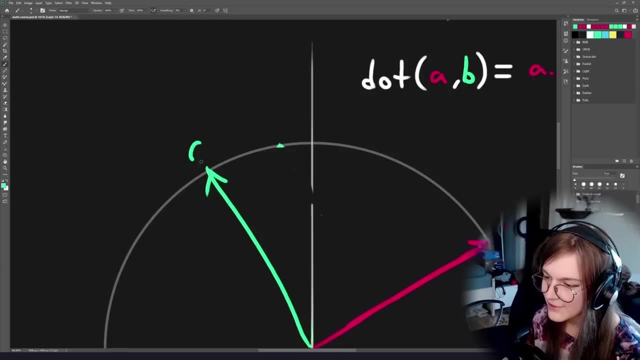 If it's perfectly perpendicular Like this, As in it's 90 degrees off of A, Then the dot product is going to be 0. And this is really really crucial. So this is important to know. So if we track what the values are, 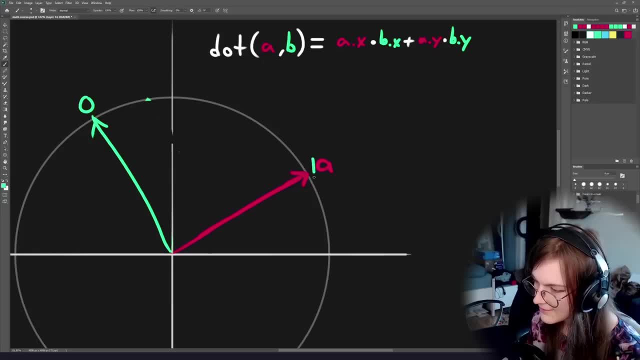 Then it's going to be 1. over here, Let's do 1.. Somewhere here it's going to be 0.5.. Right, Somewhere here It's going to be like 0.8 or whatever, and so forth. 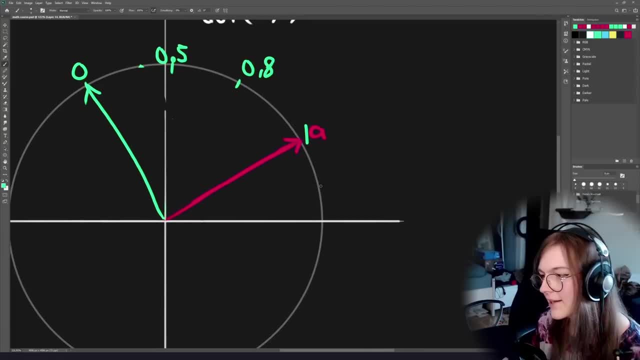 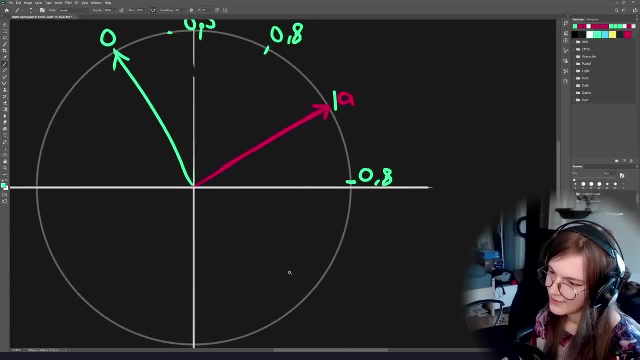 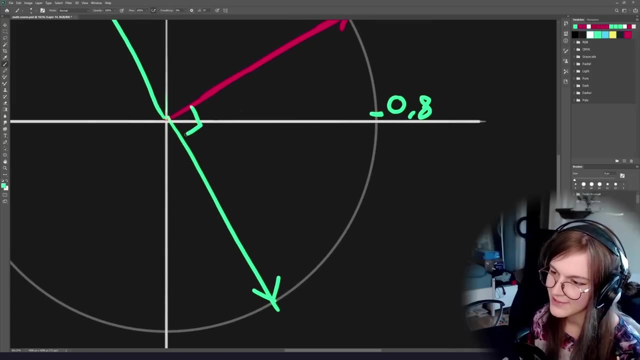 And because it's because we're projecting this onto A. There's also symmetry in this, where we would have 0.8 over here as well, And if we go perpendicular in the other direction, This would also be 0.. This also projects to 0.. 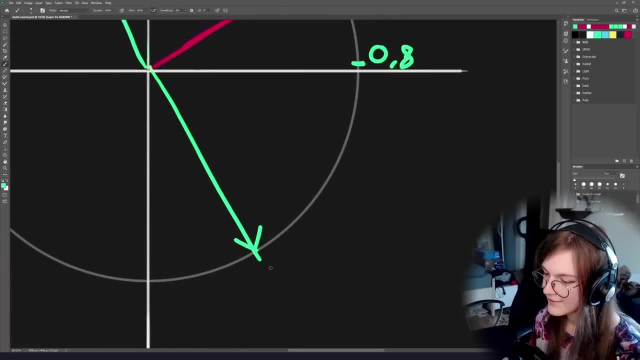 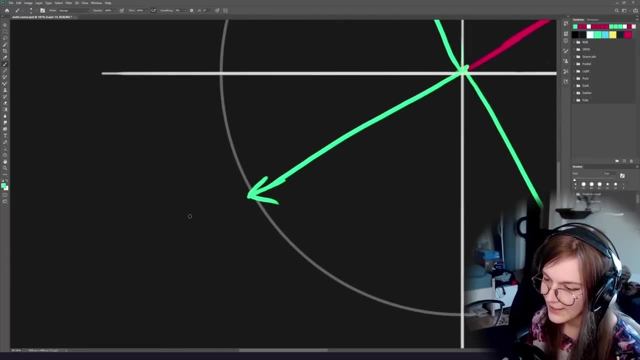 It's 90 degrees off, It's going to project towards this and it's 0 again, So we get back to 0 and then we can continue to the other side. if they're completely opposite, Then you get a value of negative 1.. 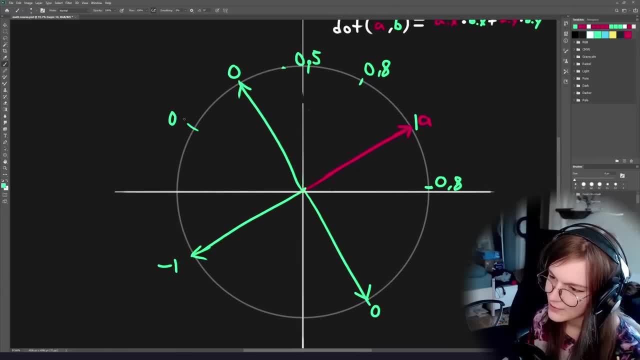 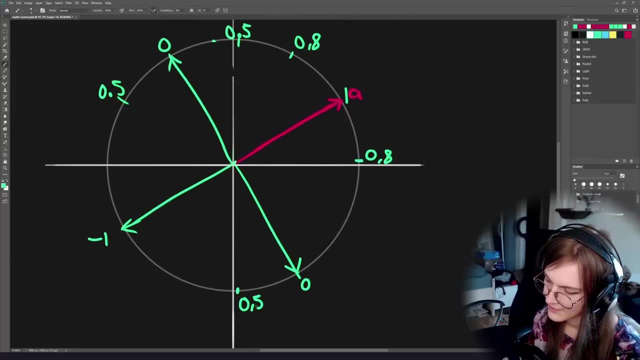 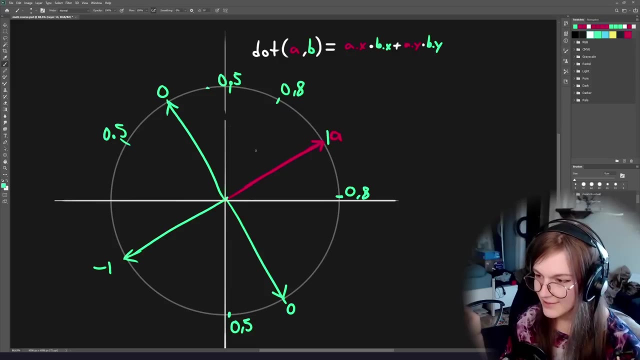 And then you have values in between here, So you know you would have 0.5 here And 0.5 somewhere here, Right? So what does this mean? This means that if you have two normalized vectors, And these are: 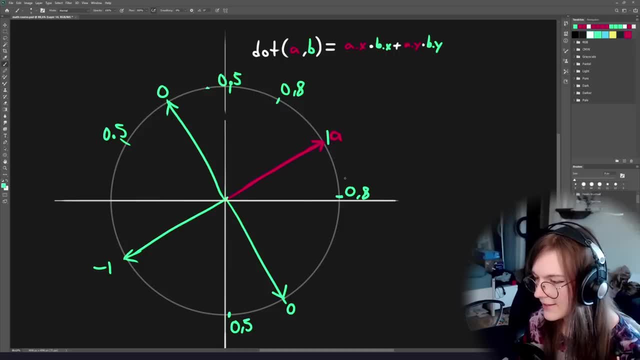 And you're comparing two vectors. What you are getting is kind of an apropos, An approximation for how close they are to pointing in the same direction, Right? So in this case I'm just talking about normalized vectors. Both of these are normalized. 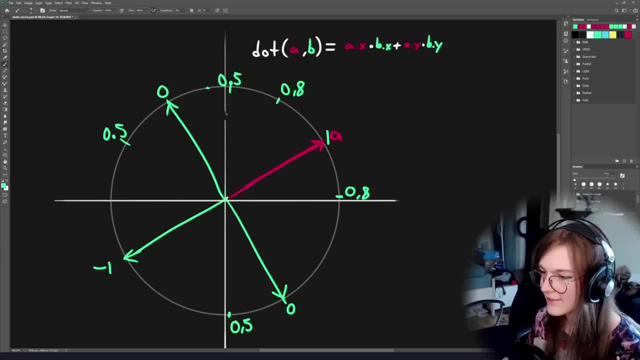 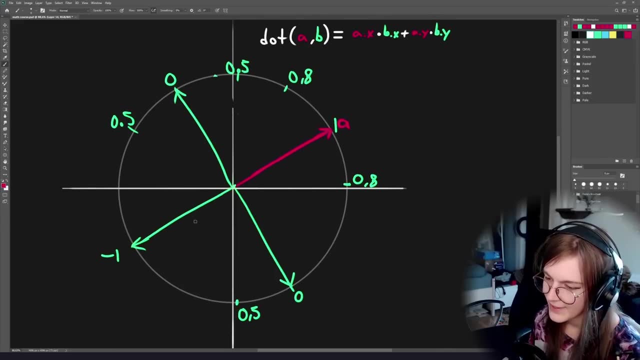 So if one of them is not normalized, then these values are not going to be interpreted exactly the same way, But the sign of this still holds. So what you can notice now is that all of the values on this side are negative. All of the values on this side are positive. 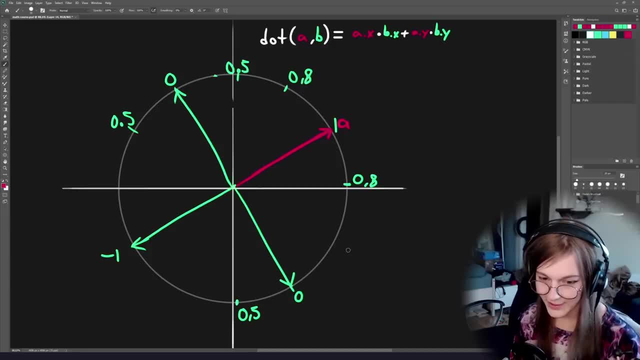 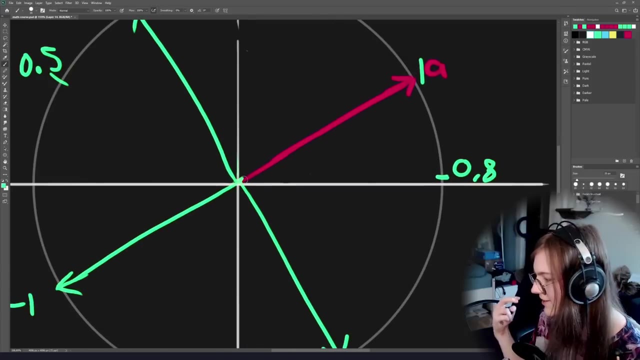 Right. So One thing that the dot product is very useful for Is: Is this vector pointing towards something Or is it pointing away from something? Right, Because now, if we consider the green arrow to be the direction a player is looking, 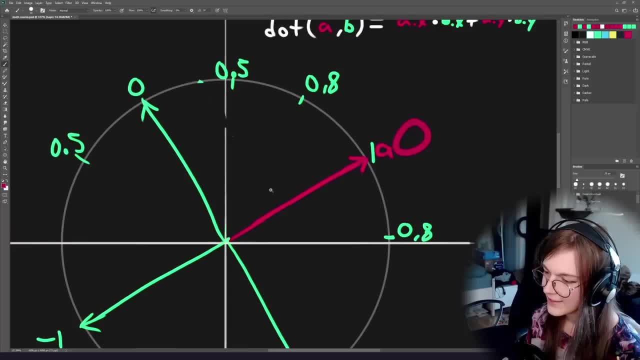 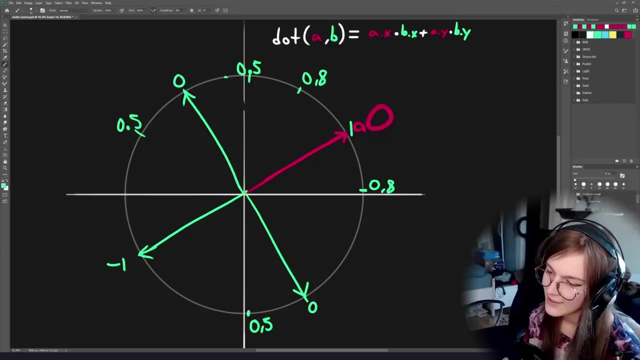 And the red arrow is the direction to an enemy or something. Then we can tell if the player is looking away from the enemy by doing the dot product Right. If the player is looking in this direction, Well, Oh, This should be negative. 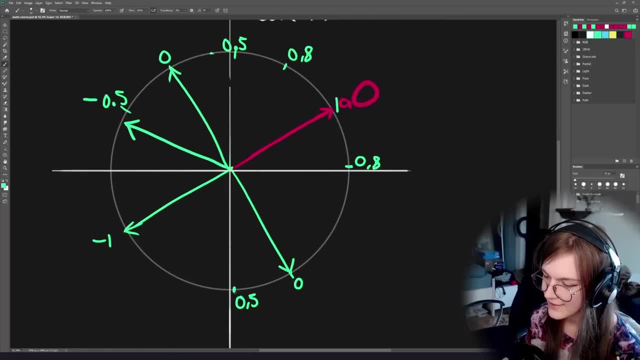 Sorry, Then this is a negative value, Right, Because all of these are negative. Sorry, I forgot to do negative for these. Yeah, So all of these are negative values, All of these are positive values. So now, if we do the dot product between the player direction and the enemy direction, 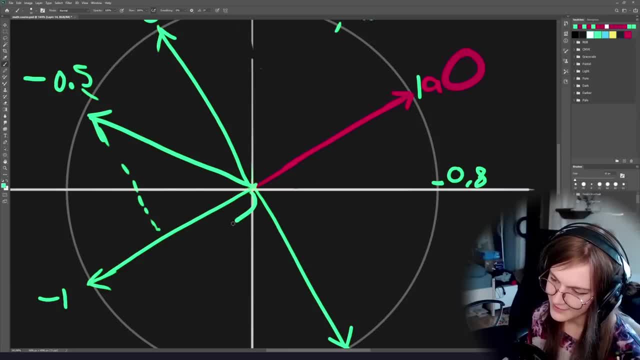 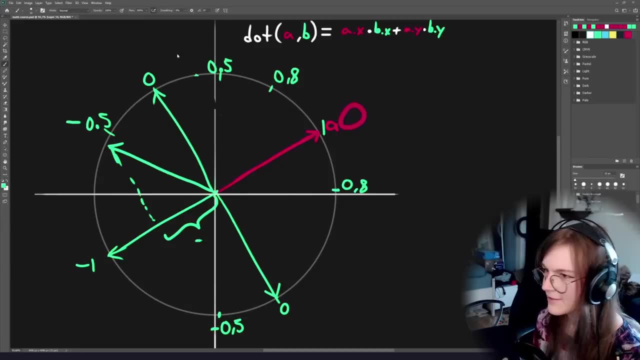 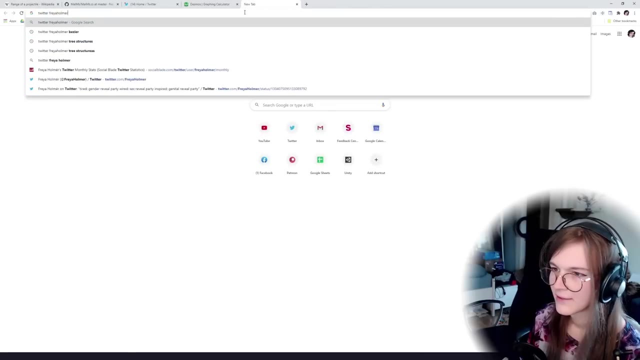 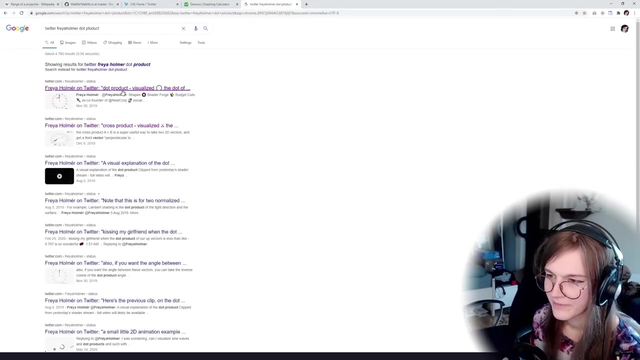 It's going to be negative here, Because it's projecting here, Got the distance here, And that's negative. So this is super, super useful. I do have an animation for this too. Not that animation, It's the wrong one. So here's an example. 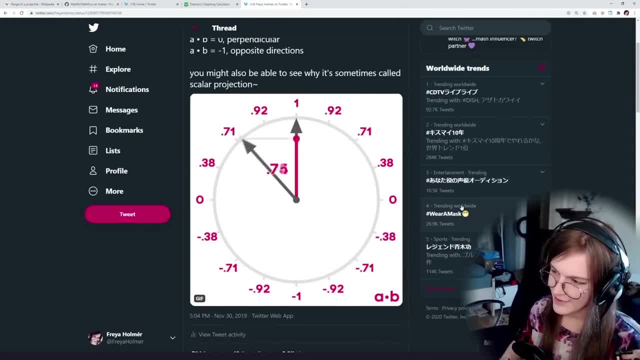 This is basically what I've just been talking about. now You have two vectors. If they point in the same direction, You have a value of 1.. If they point directly perpendicular to each other, It's a value of 0.. If they point completely in opposite direction, it's a value of negative 1.. 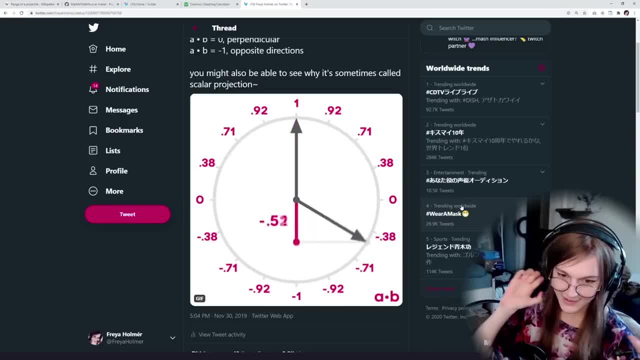 And that's kind of it. So again, this is only when you have two normalized vectors. If one of them is not normalized, the positive and negative thing- those rules still apply. In that case they don't have to be normalized. 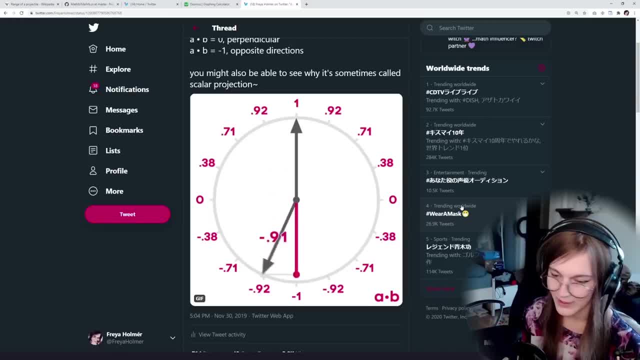 But for these values to be exactly 1 and negative 1 when pointing in opposite directions? um, they have to be, um, one of them has to be. they have to be normalized, right? Can I calculate the second vector if I only have the first vector and a dot product? 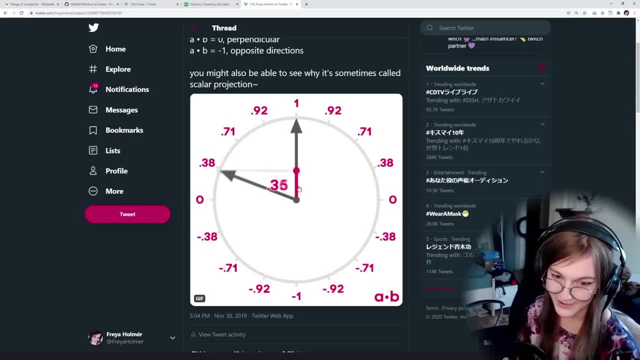 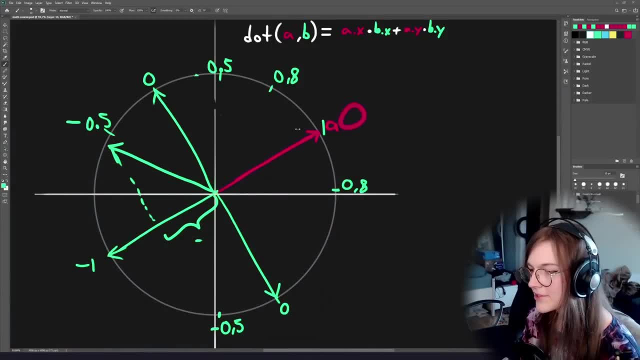 Um well, it would be ambiguous, right, Because you would have two results, not one, But I believe it's possible. Yeah, Is there any point having one vector larger? Yes, If you don't want to check the, if you're not interested in checking, like. 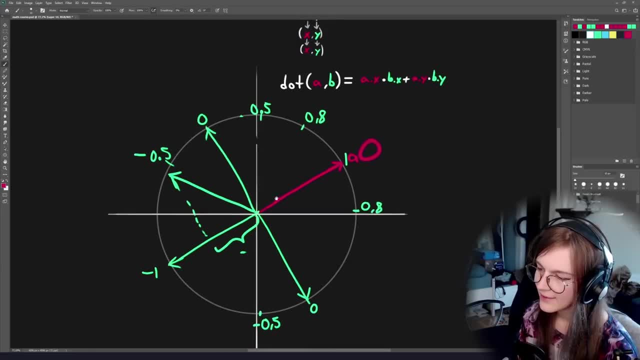 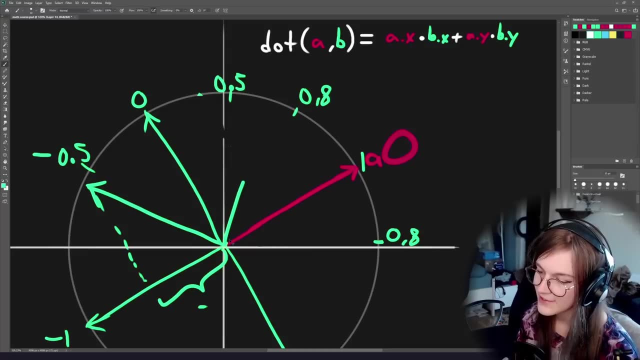 are they facing the same direction or some other direction? Um, sometimes you want, or very often actually, uh, the vector is shorter or longer, uh, than a normalized vector. Uh, so this vector projected onto this one? um, sometimes this distance is still interesting. 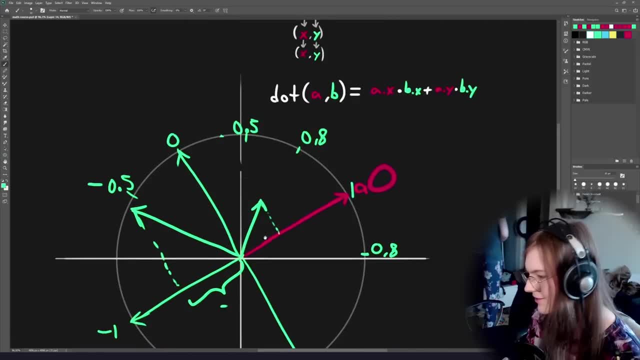 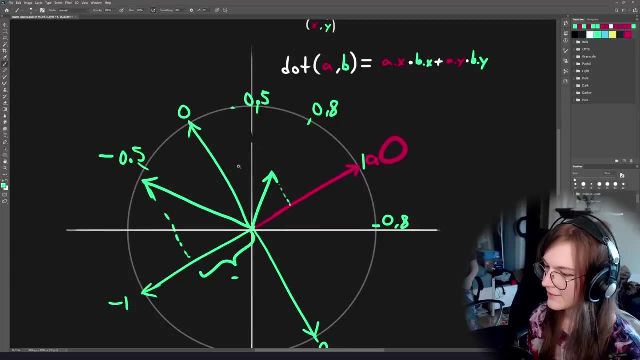 And it's very often interesting as well, Um. so let me be a bit more practical, Because we've been talking about, like, esoteric things, And let's let's think about, um, what this can be useful for right. 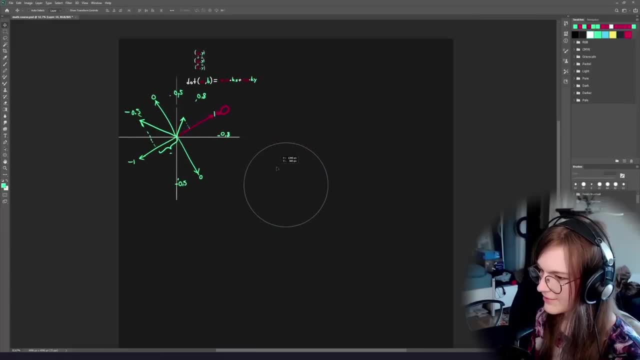 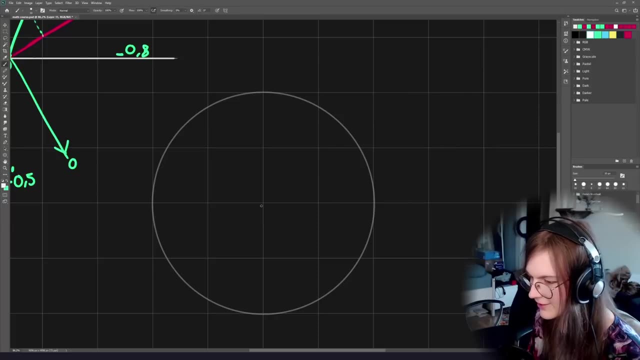 Let's see. Maybe I should move. Do I move that Or do I keep it? Angle is implied by the dot product. No, Angle is. we're not talking about angles. Angles is spoilers. We're not going to get into angles as soon as we talk about trigonometry. 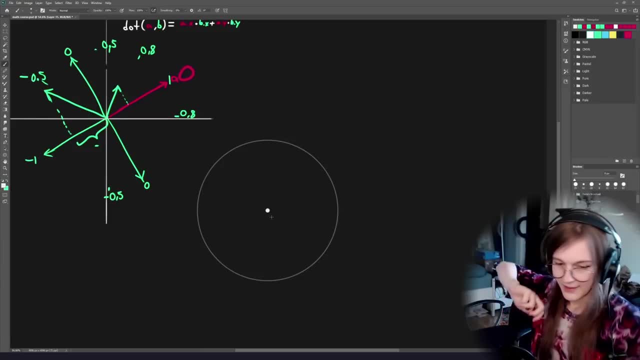 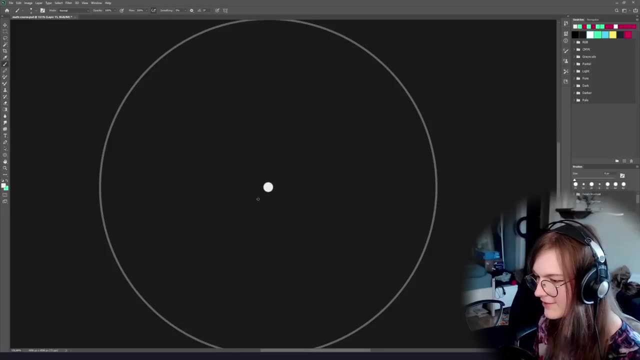 But right now we're just doing vectors. Okay, Here's an actual example from the game that I I'm working on. So let's say you, you happen to have a game that has a surface of all things, Um, so let's see. 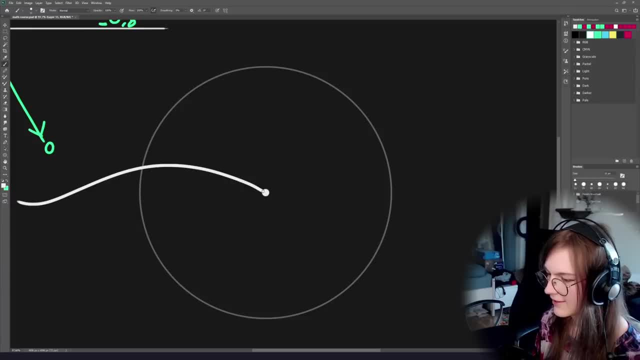 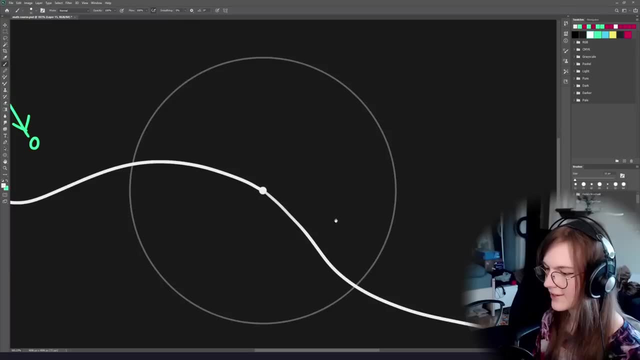 I guess we can give it some, some direction. There we go. So this is soft and good. Um, I don't know how to make this continuous. There we go, Cool, Okay, So we have a surface. Uh, we have a point on the surface. 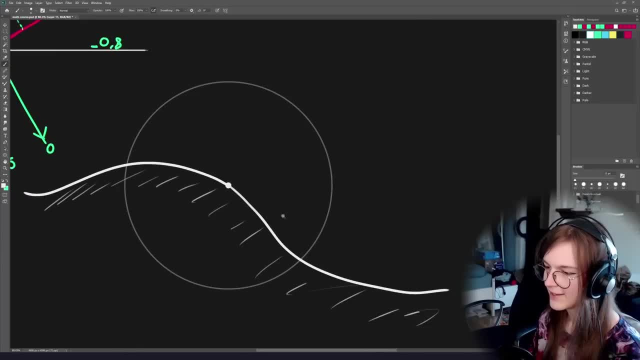 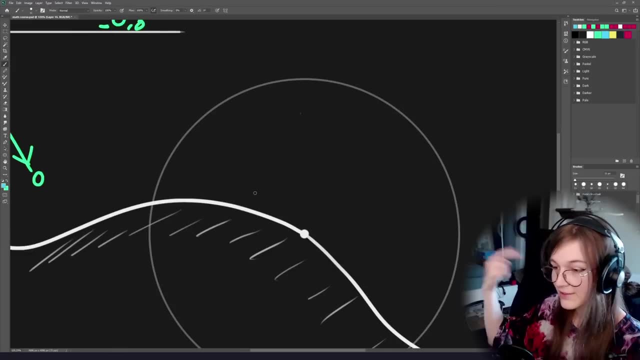 Uh, it's solid underneath here, So you can just pretend that this is a solid uh and you have air here. Uh, now we, we quickly mentioned, uh, or we briefly mentioned the, the normals, or what a normal is, of a surface. 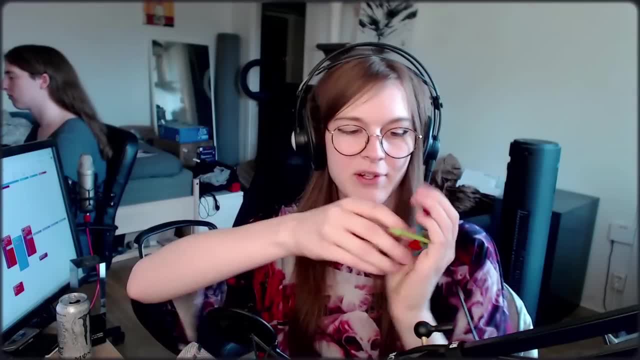 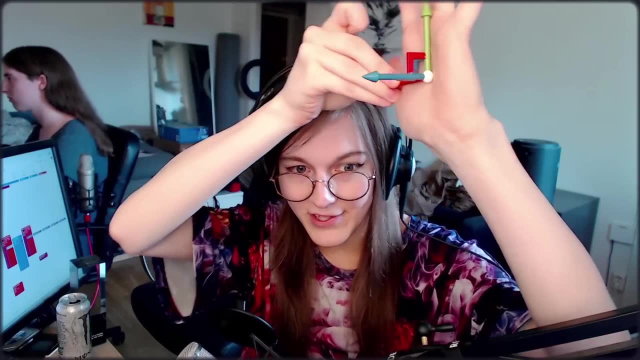 Uh, and again, a normal is a, um, something that is pointing directly out from some surface. Um, so, like the, the blue vector here is normal to the palm of my hand right. Uh, the other two vectors are tangent to my hand. 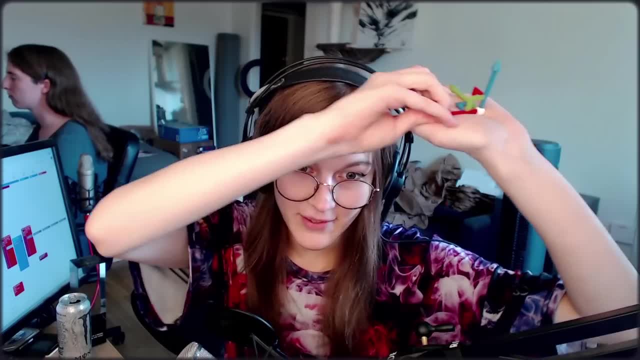 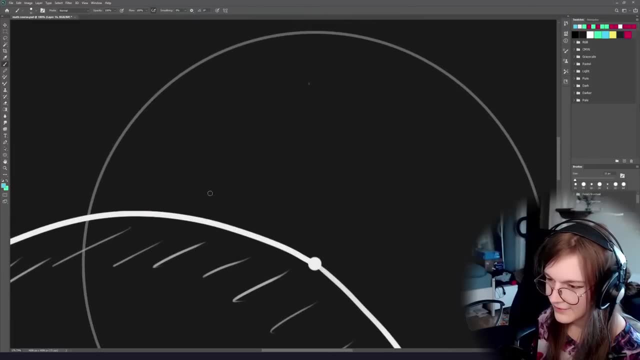 They're not normal, Right? Uh, so pointing directly out from some surface, that's the normal. So let's, let's, um, let's, visualize some normal. So, if you have this surface, uh, again, the normals point directly out from the surface. 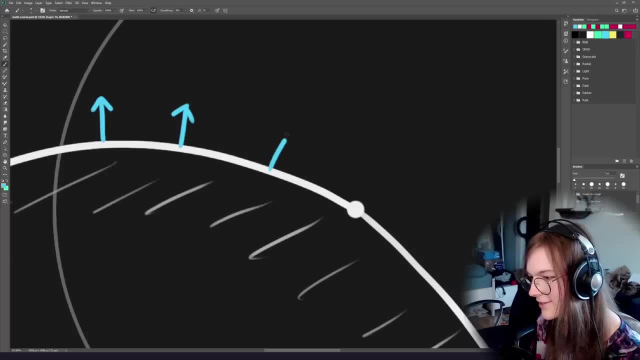 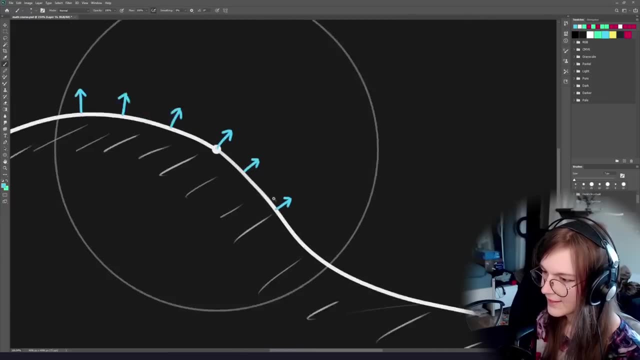 Um, so the normals along this surface would like kind of Continue like this right, And then you would get a vector like that and so forth. You imagine these have a length of one. Uh, so these are the normals of the surface. 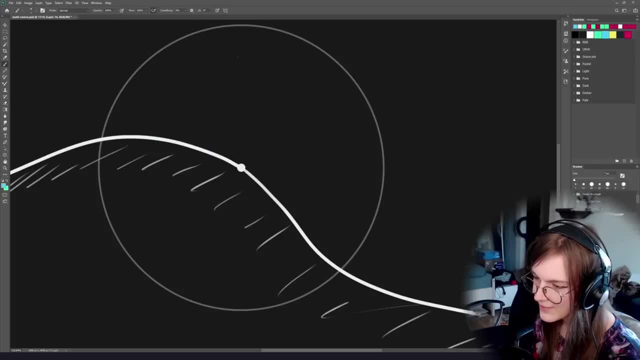 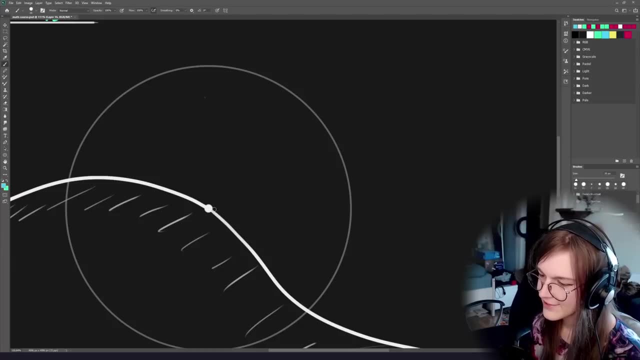 So let's think about this point in particular: Um, and let's draw the normal. The normal is going to be very large because our circle is very large. Um, so this is the normal, So let's call that um, and now we have the normal of the surface. 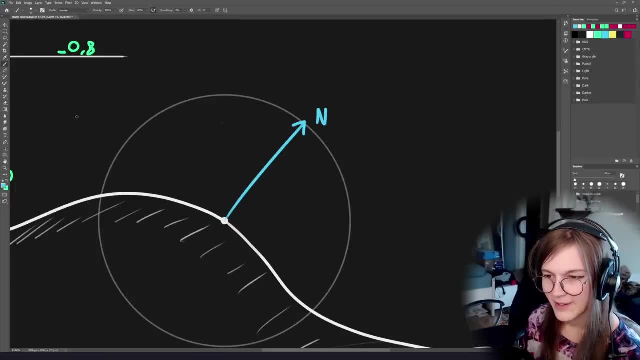 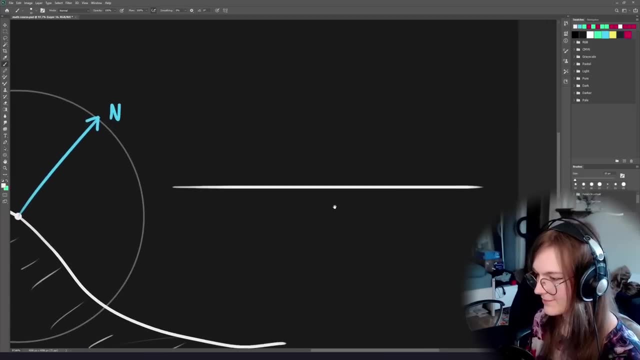 So here was a problem that I had, um, when I was working on a game back in the days. Um, if you have a surface and then you have an object, for simplicity sake, let's say we have a, have a sphere or a ball or whatever- 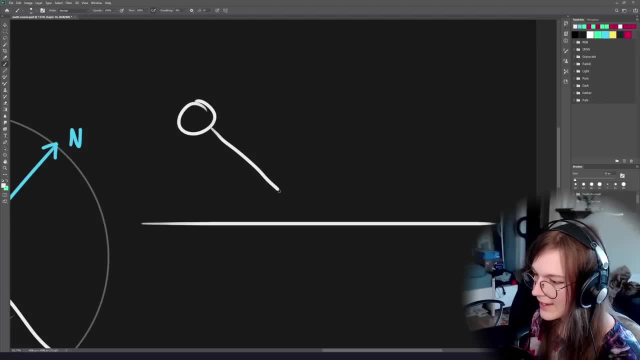 And this object is moving at some speed And It's Going to hit the uh, this ground and then bounce off of it, right, Uh, okay, cool, Uh, it can bounce off of this surface. Now you want to play an audio clip? 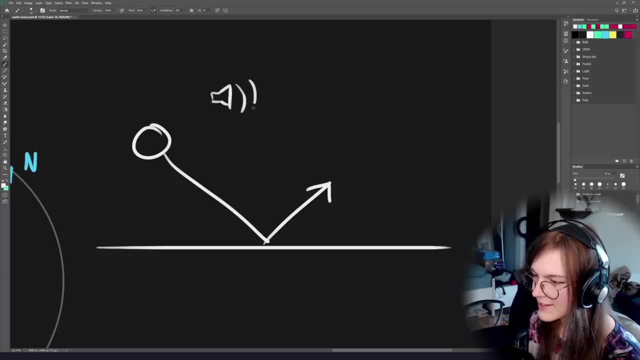 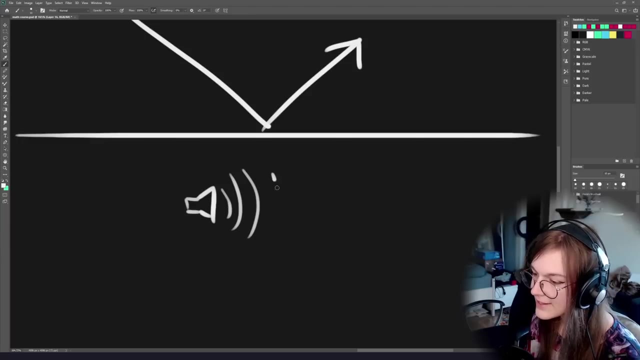 Um. so let's say, you, you want to play some audio clip. There we go. That's my audio clip symbol, because you have an impact sound. You want to make a clunk sound when the ball hits the ground or something. Um, and now the question is: um, what is the? 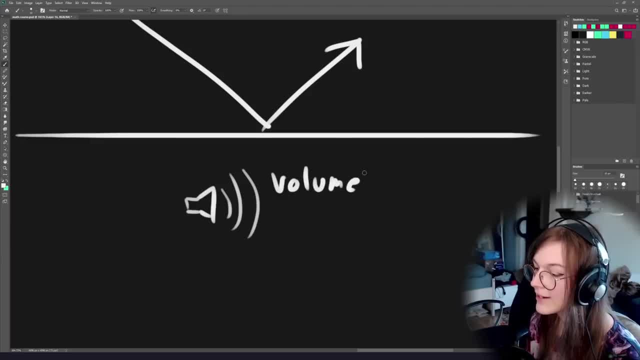 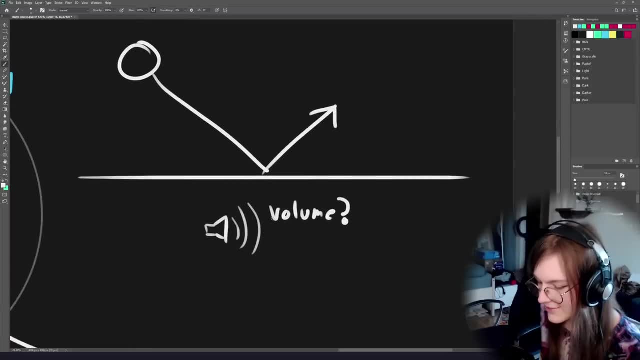 Volume of this sound Like. how loud should this be? Um, how would you solve this problem? Um, so, so now we're getting into like trying to figure out: okay, if we are moving very quickly, uh, then obviously we want it to be louder than if it's not moving quickly. 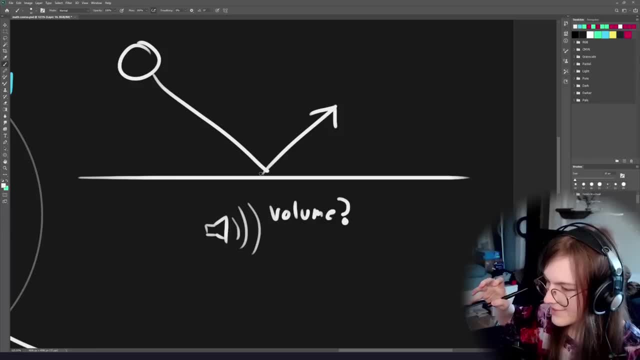 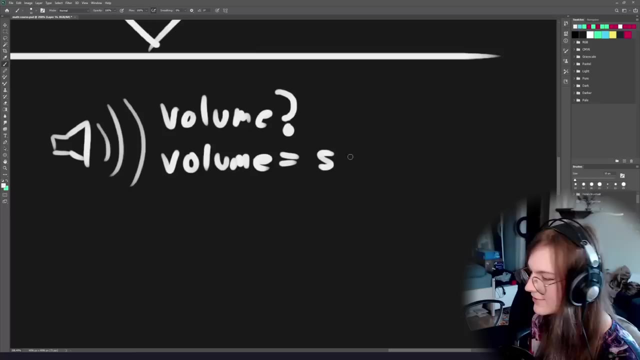 Right, If it's moving very slowly, hits the surface, uh, then we might not even want to play a sound, Right, Okay, So let's just think about this some more. So, so, maybe volume, uh, it's just the speed of the object, right? 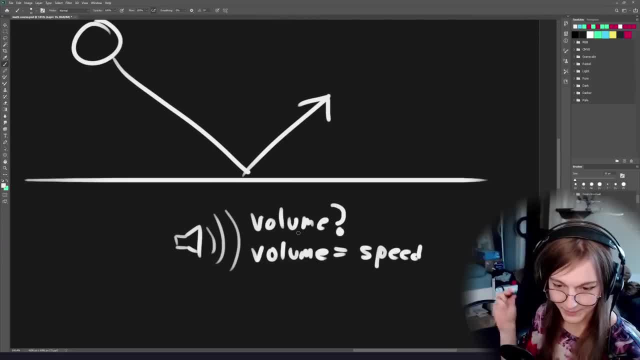 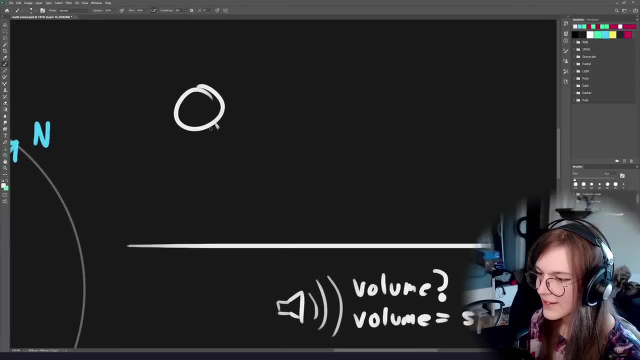 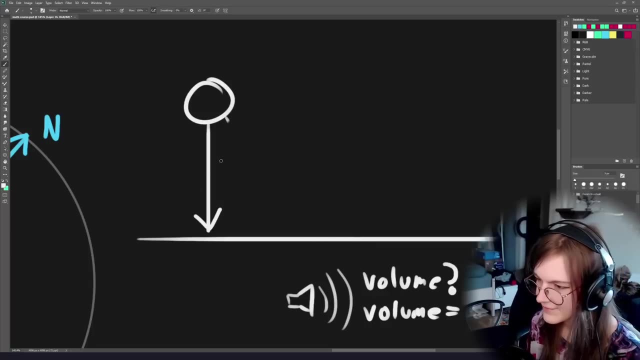 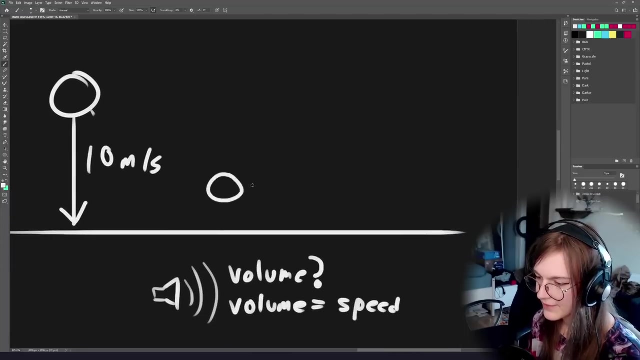 Cool, All right, We got the volume equals speed. but consider this case if you erase these, all right. So we have this ball. let's say we throw this one down straight down at uh, some speed. Let's say it's uh, the 10 meters per second. and then we have another ball that's at a very low angle and it's going to hit the ground at the same speed. 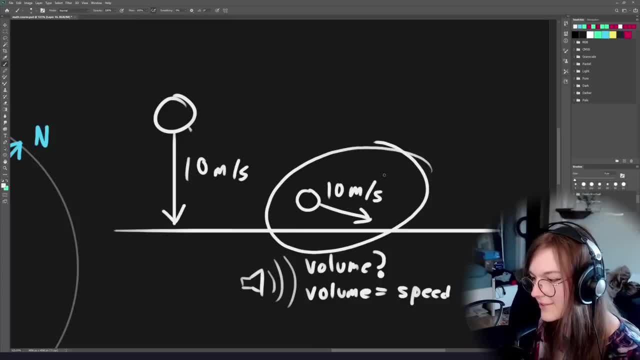 So we want this one to be louder than this one, right? Uh, because obviously this one is going to make a very hard impact on the surface, Um, whereas this one, it's not going to make a very hard impact, Like it's going to mostly going to grace the ground and then do a little bounce, right? 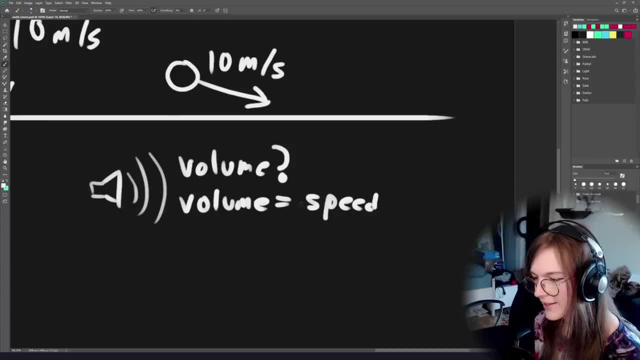 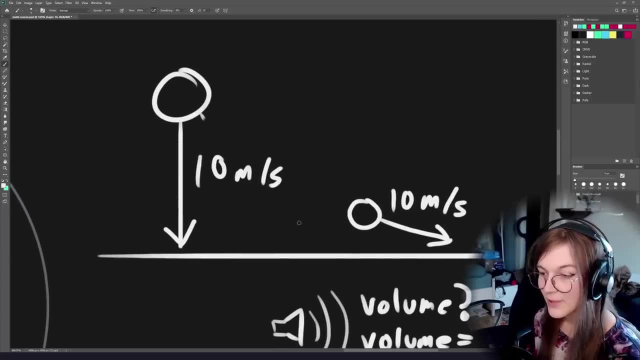 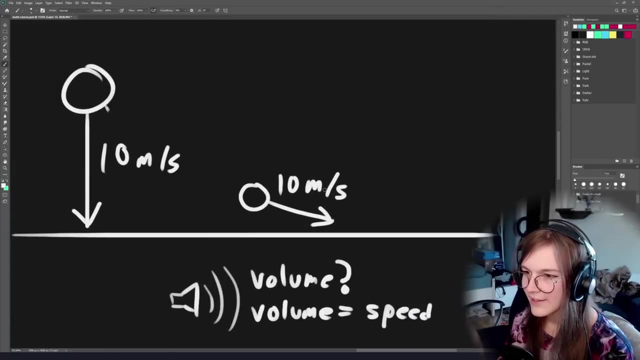 Um, so now we have this issue of like: well, it's not just based on speed, We have to do something else, right, Okay? So what can we do? So what we can do is that we can use the normal of the surface to figure out: how quickly is it moving toward the surface? 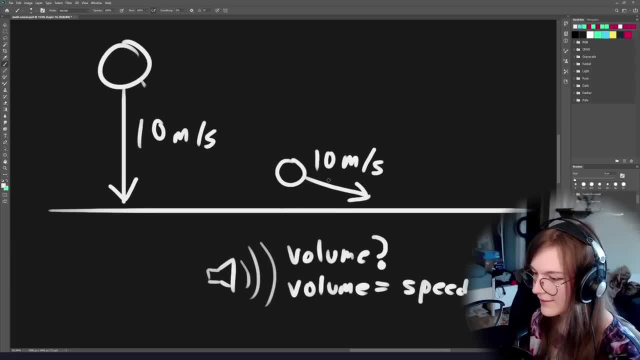 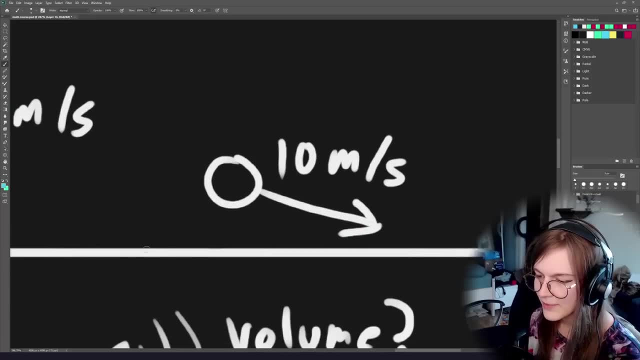 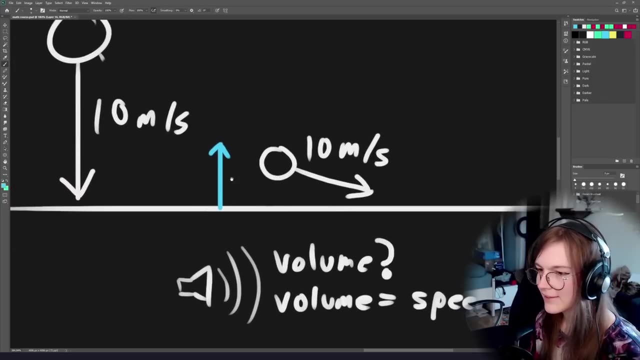 Cause that's the key thing that we need to know, Right? Um so, so let's, let's bring out the normal again. So the normal represents the direction of the surface, right? And what can we then do? Well, we can think of these arrows here as our velocity vectors. 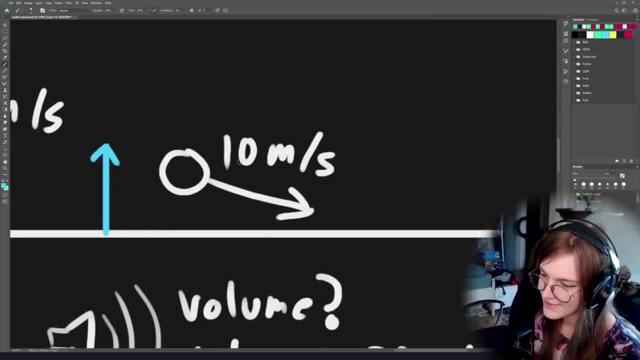 We're going to get into more physics later, but you can sort of represent velocity as a vector, Um. so basically each component, like X, says how quickly you're moving along the X axis and Y is how quickly you're moving along the Y axis. 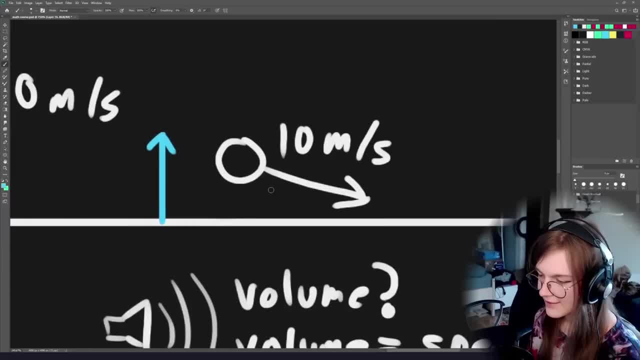 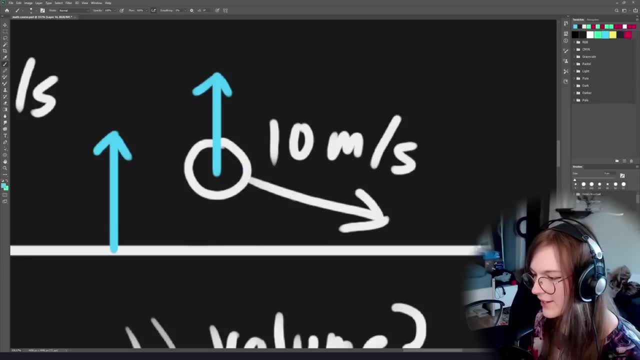 So okay. So how do so? how does the dot process work? How to come into this? Well, what we can do then is that, um, if you imagine this normal here, we have the velocity vector here, and then we can project this onto this line. 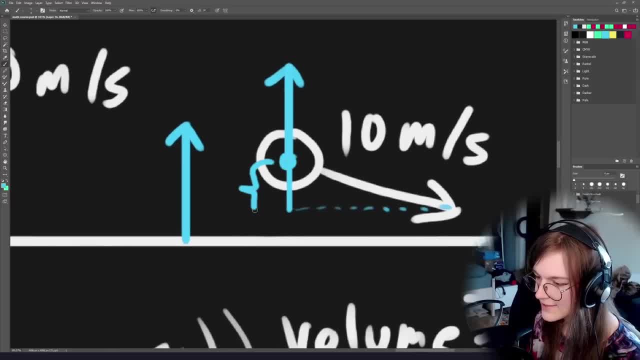 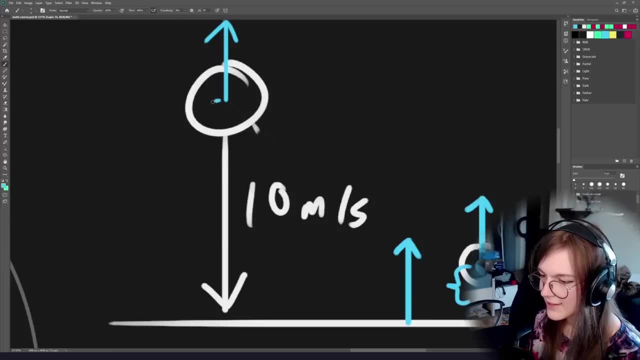 Right, And again the dot product gives us the projected distance here, Um, and then we can do the same thing here, right? Uh, we take this one, do the dot products, and now we get this distance right here, Um, so, even though I guess we pretend, 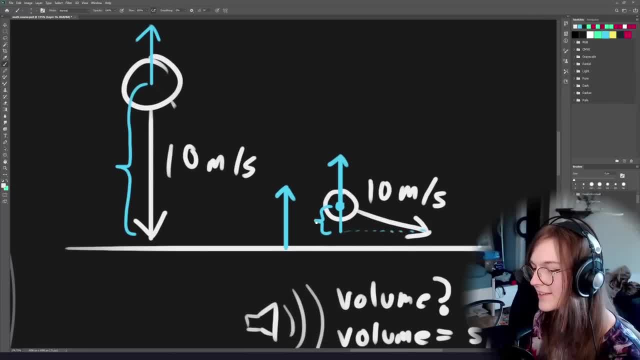 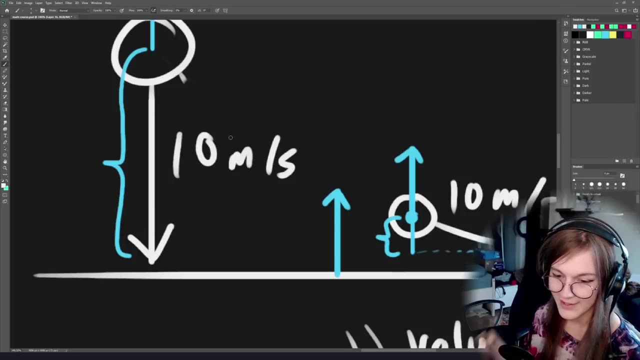 This arrow is as long as this one, uh, but the. the point is that now, using this normal, we can get speed in this direction rather than speed um overall. right, Like getting the uh, getting the length of the velocity vector is your overall speed. 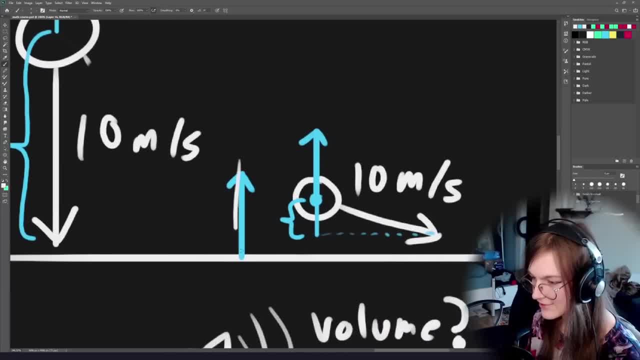 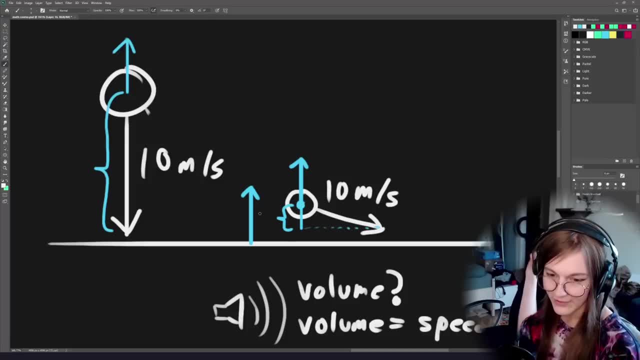 Uh, but it doesn't say what the speed is in the direction of the surface, right, But that's what we're interested in. If you're moving directly toward the surface, it should be really loud. If you're moving Really fast but you're not really hitting the surface fast, you're kind of moving fast just tangentially, um, then we don't want it to be loud. 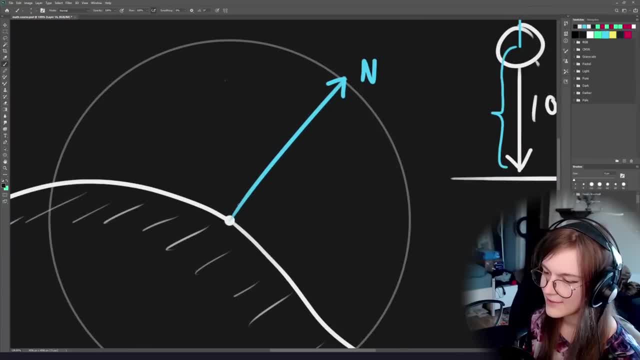 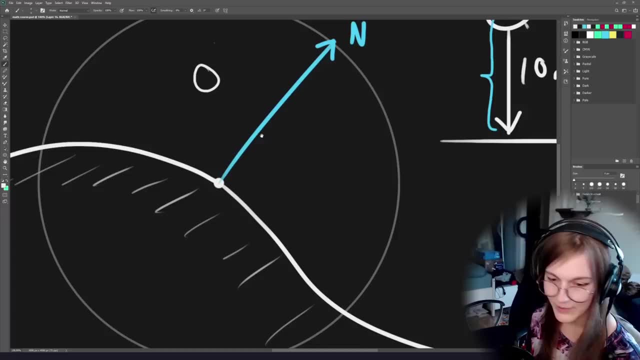 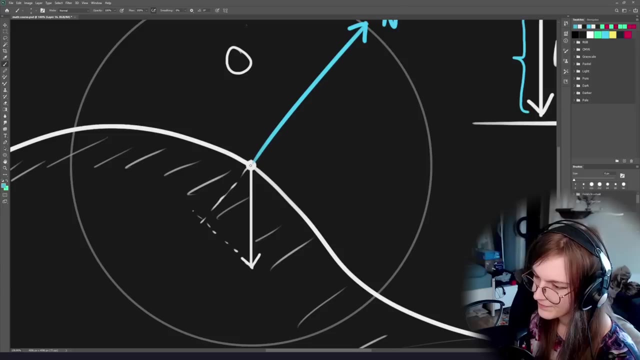 So in this case, every time you have some object, um, that is hitting some surface, um, you know this object is flying onto the surface, uh, then we can just do the math: Uh, if the, if this is the velocity, we project this onto um, onto the normal vector, uh, and then we get. 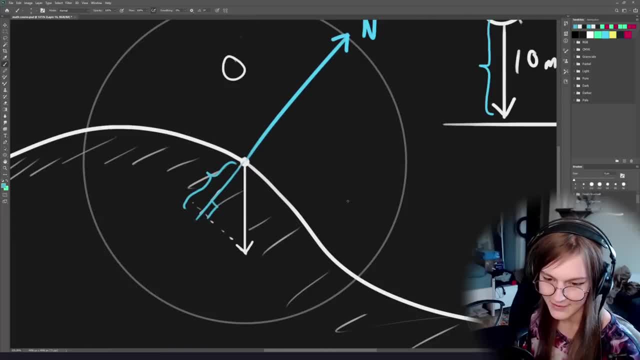 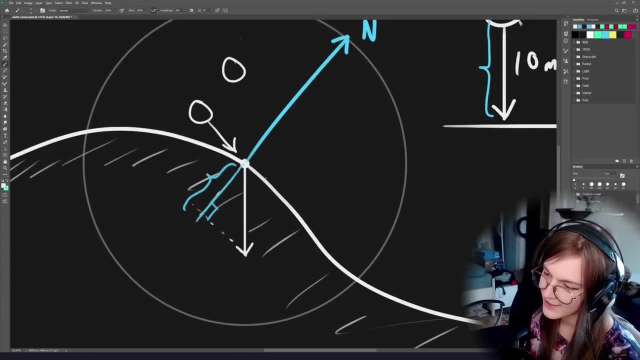 A magnitude here for how loud this should be right. Okay, So let's try a different direction. Um, another ball that's flying in this direction. Um, well, if we do that, then we're going to get a vector like this: 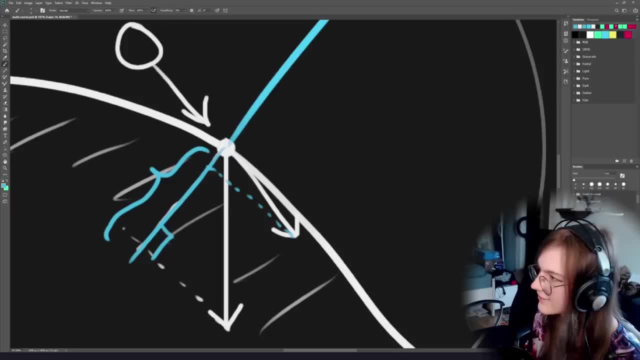 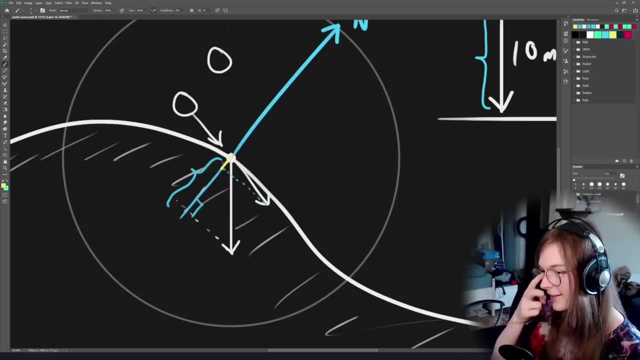 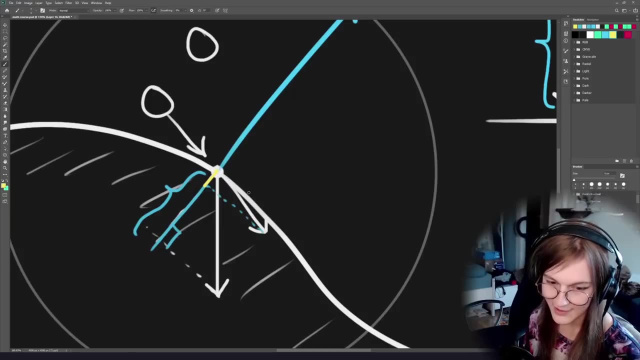 And when we project this one, it's not as loud, right Cause now we're only using this span right here, and this is much shorter and a much smaller value. Um, so so what we're getting is the Direct or the, the, the speed along a specific axis. 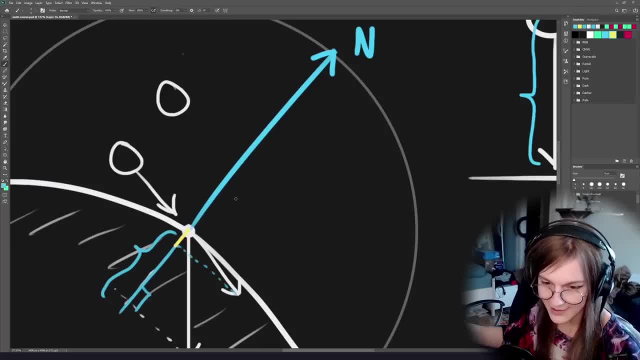 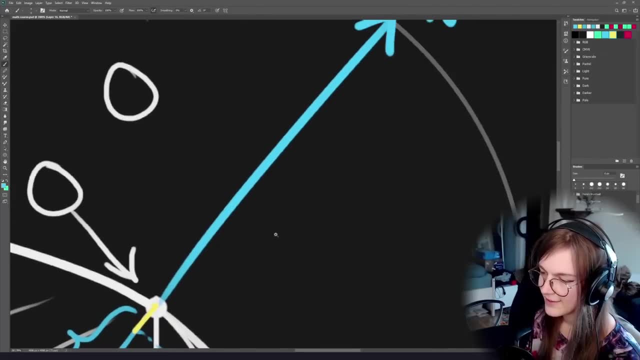 So we get the speed along the normal. That's what we're getting when we do the dot product between, you know, the velocity vector of the object and the normal of the surface. Um, yeah, so long story short, you need the dot product. uh, basically. 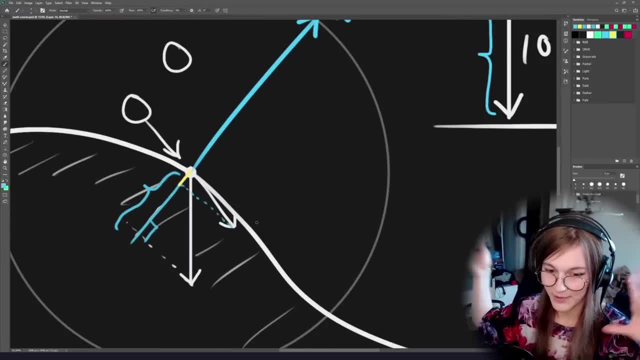 Yeah, So so that's. that's one use case. So that's what I've used dot product for, For instance. there are millions of use cases for the dot product, but this is just one of them. Um, yeah, 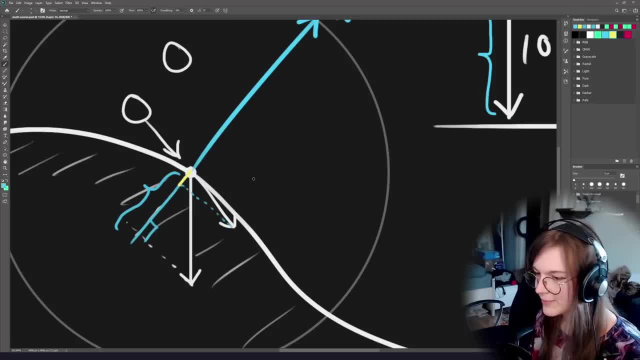 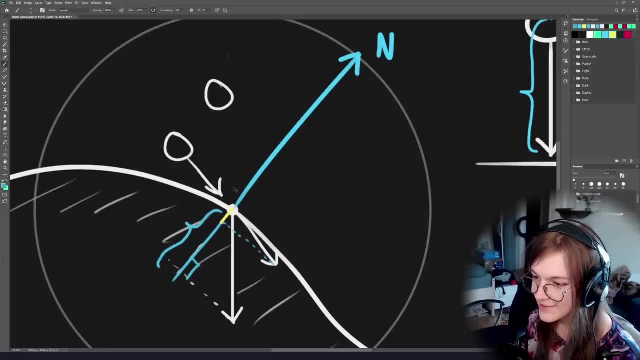 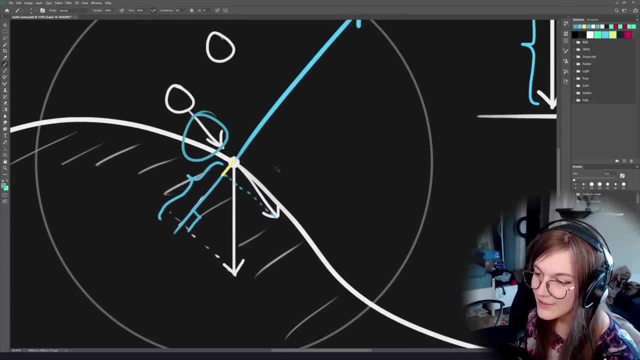 Um, do both of these vector need to be normalized before using the dot product? No, So specifically here it's very important that the normal is normalized and that the velocity vector is not normalized. Uh, because we do want to. uh, the longer the velocity vector is, the faster this object is moving right. 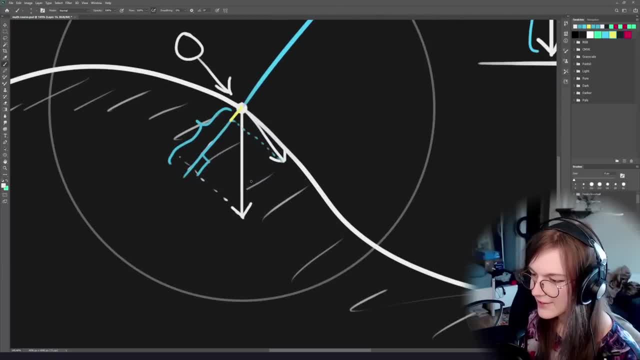 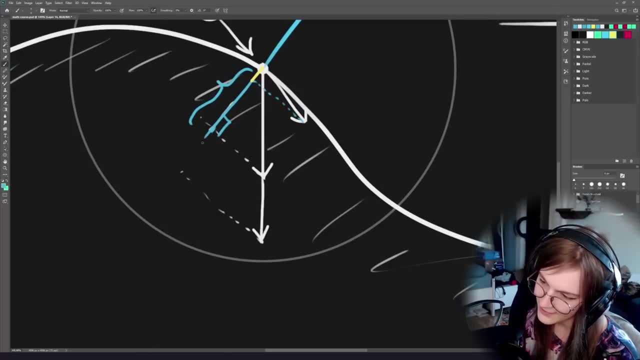 So if you imagine the one that's moving downwards, that's this velocity vector. if it's moving faster, we want it to To be louder, right? So that would still project onto this line here, and then we get this value here. 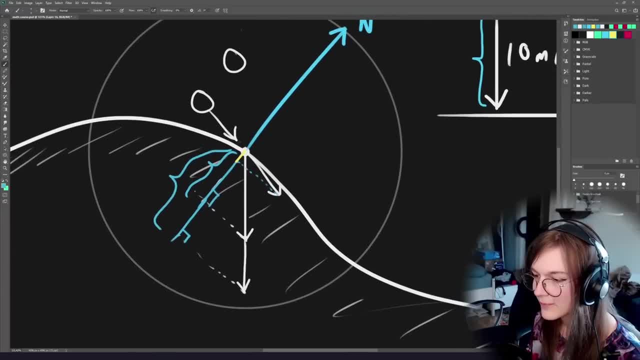 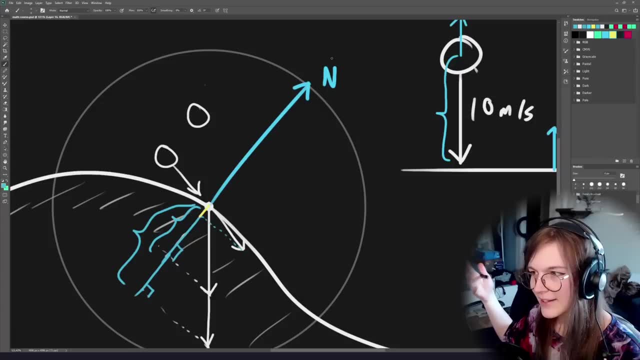 Uh, so we still want it to be louder. Um, so we don't want to normalize the velocity vector. We do want to normalize the normal vector, though. Um, otherwise we're not going to get things that are in meters per second anymore, and it's not going to be a correctly projected um speed along an axis right. 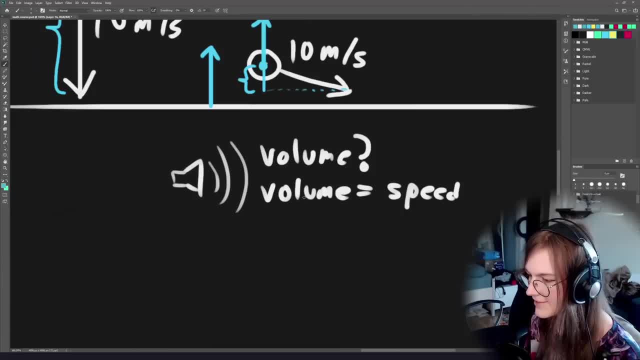 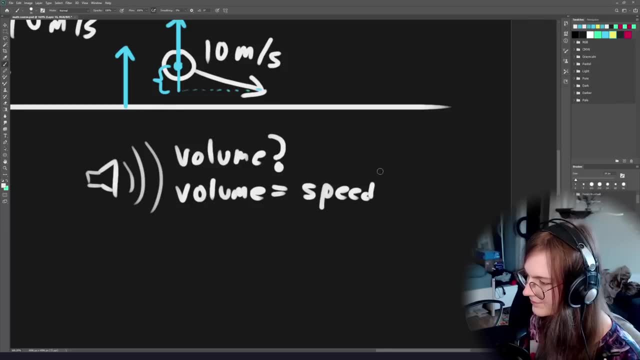 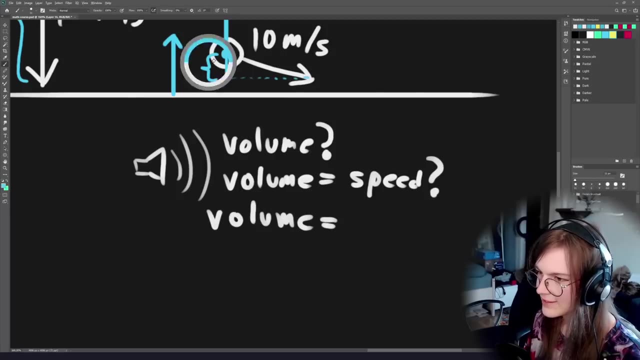 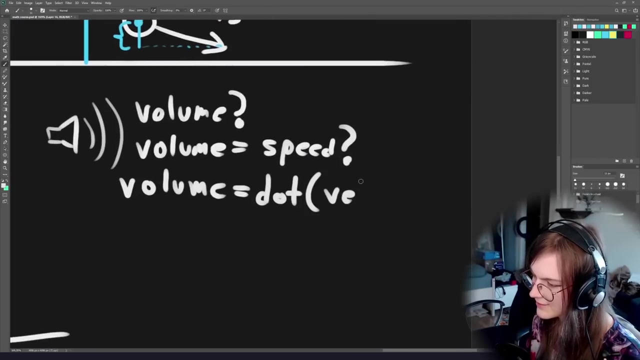 Um, can you, Can you post that image here? Yes, Uh, right, Let me just um complete this, cause I kind of left this incomplete. Um, okay, So so better way is something along the lines: of volume equals, uh, the dot product between the velocity and the normal. 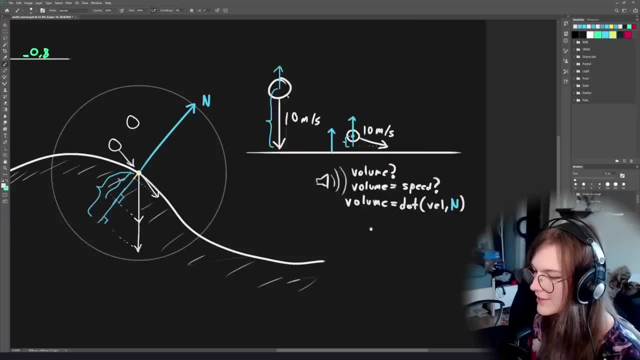 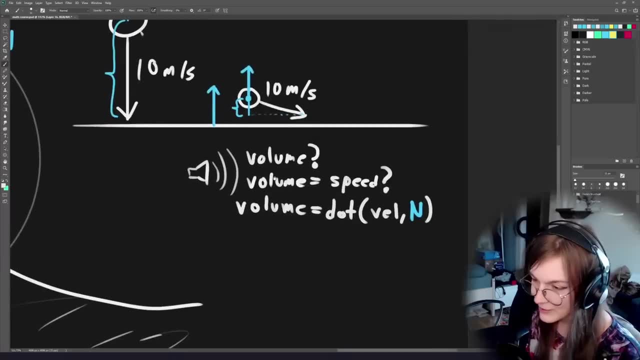 There's some caveats here. Uh, so If you remember how the dot product works, uh, these values are going to be negative. uh, so you have to like make sure that they're positive. uh, you might want to multiply them to change the overall loudness or whatever. 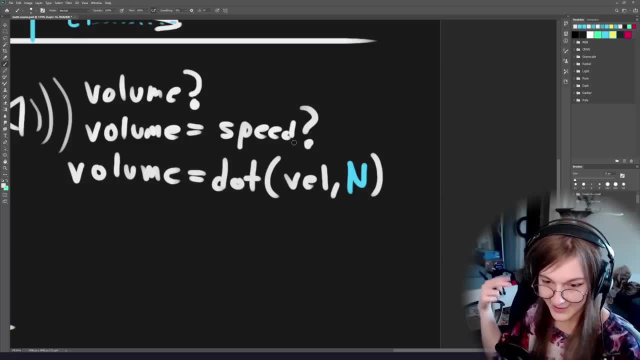 Um, yeah, but if, but, but again, the dot product product is a scalar. Um, if it's negative and you don't want it to be negative, then you can just do the do the absolute value of that Right. 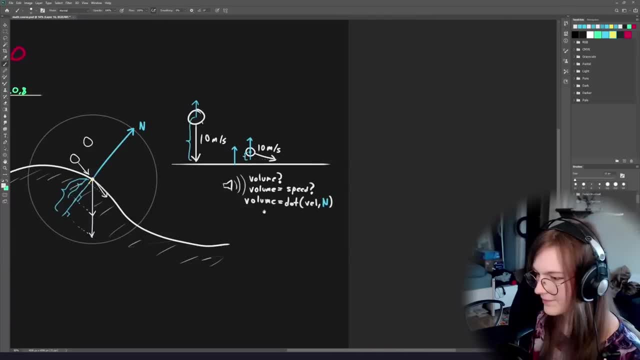 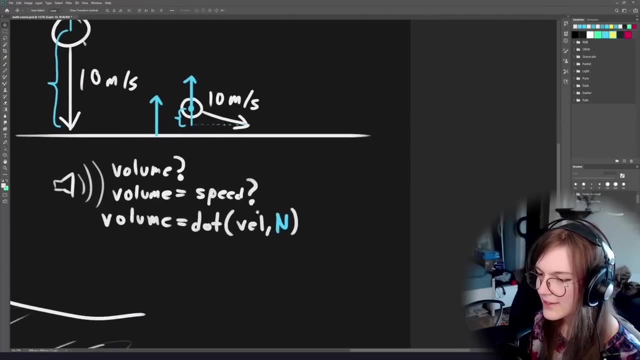 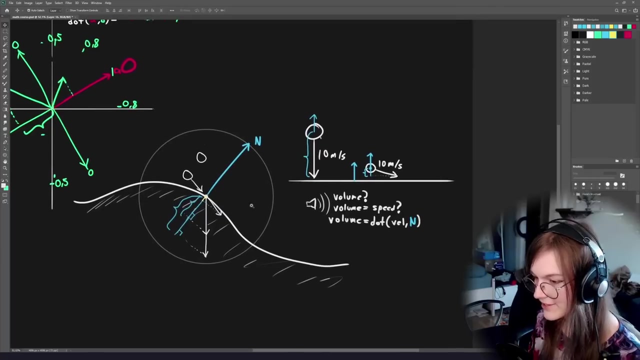 Um. so getting the absolute value of this would get you um, get you some volume Um. but the core concept is that with the um, with the dot product, you get a projected um, projected velocity along some axis. in this case the axis was the normal of the surface. 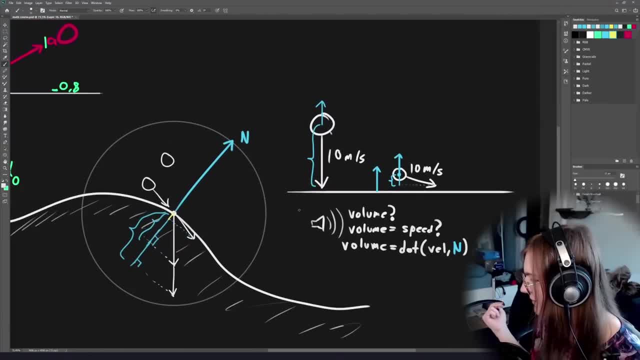 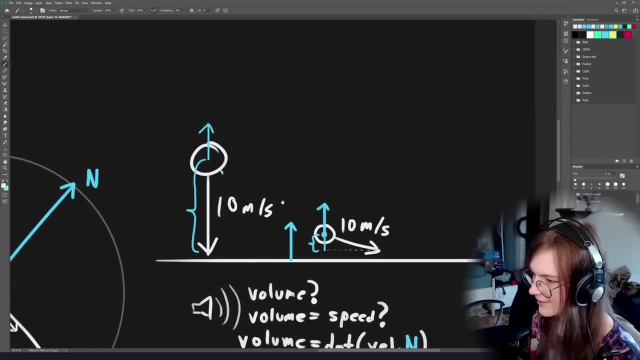 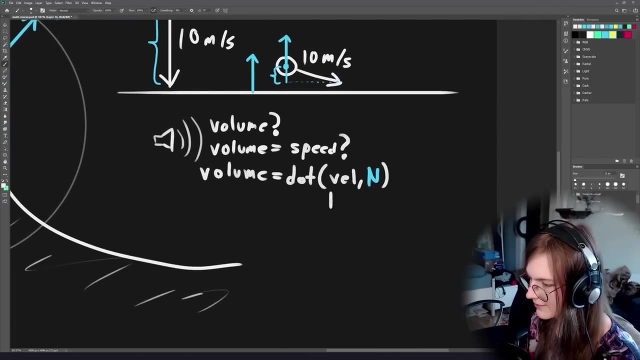 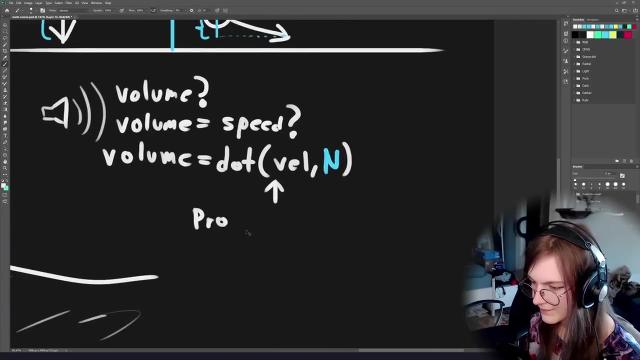 Right, Um, was that clear, by the way? Uh, yes, I can post that image in the discord. Actually, let me write some notes to make sure. Um, it's a little misleading to say speed, because speed is generally not signed. 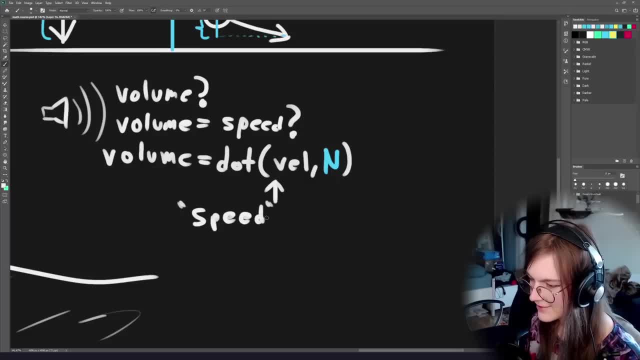 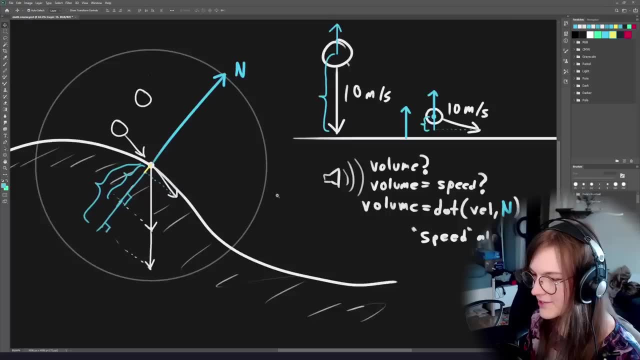 It's pretty much always positive, So I'm going to put that in quotation marks. Oh, people are talking about the cosine. Uh, yes, the dot product has a a very intimate relationship with the cosine. but we haven't done trigonometry yet. 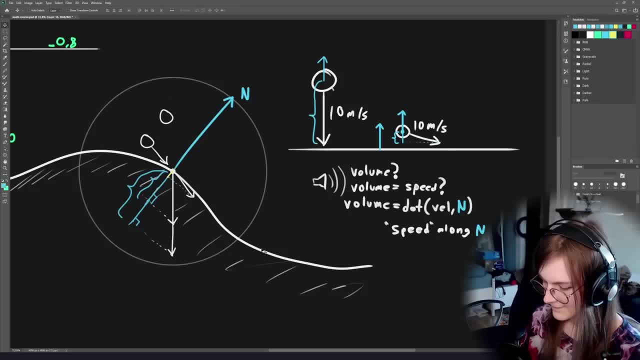 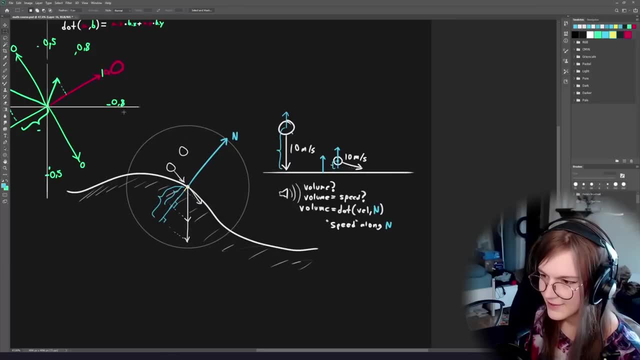 So we're going to do trigonometry later. Um, okay, Yeah, Let's. let's post this in your discord. Jeez, When people are skipping ahead of your math class and spoiling the. what's going to happen in the next chapter. 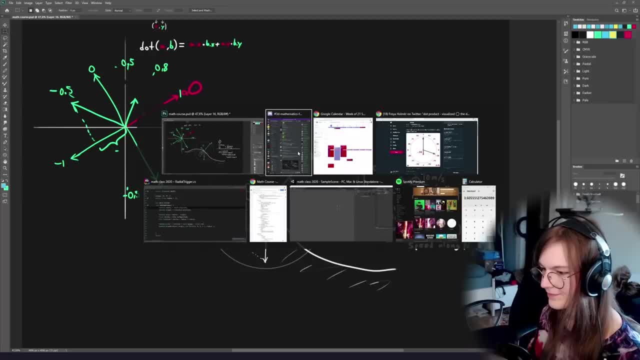 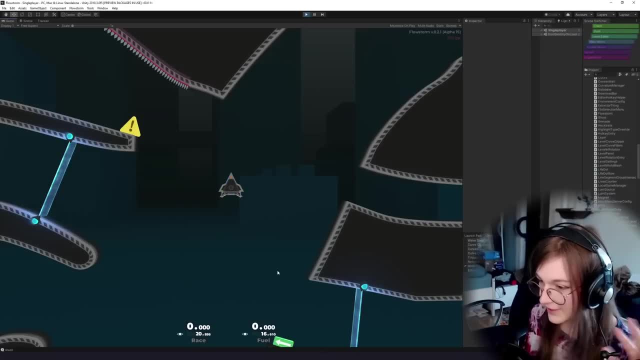 Yeah, I can just show you another example of the dot product. Um, if you want to see in game this time. Um. so here's another use case for the dot product. So I'm working on this game. This is called flow storm. 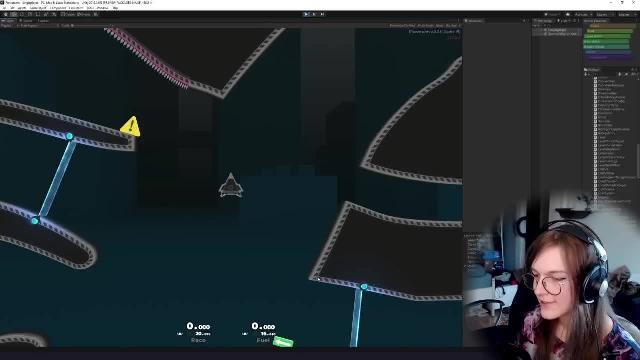 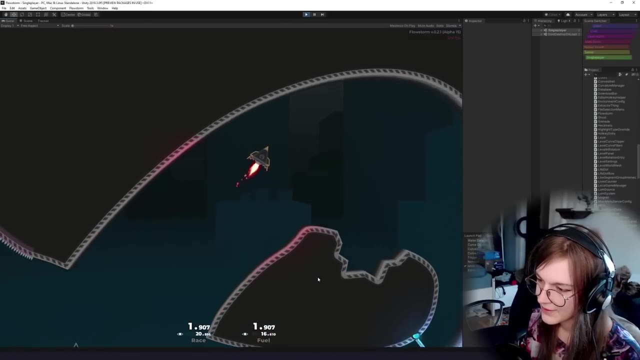 Um, so, so, right now, the another thing that I used the dot product for, uh, was the uh pitch of the thruster of this rocket, right, Uh, so if you listen to the rocket here, um, you can hear that the pitch is changing depending on what's happening, right? 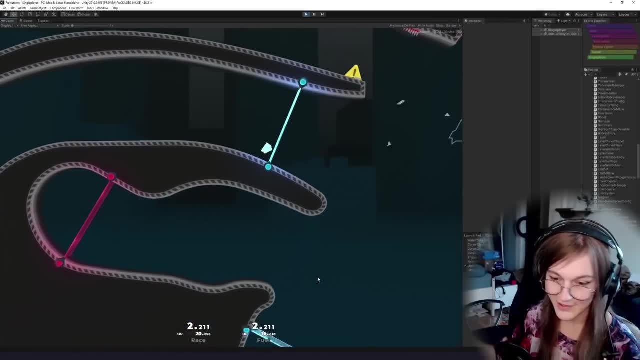 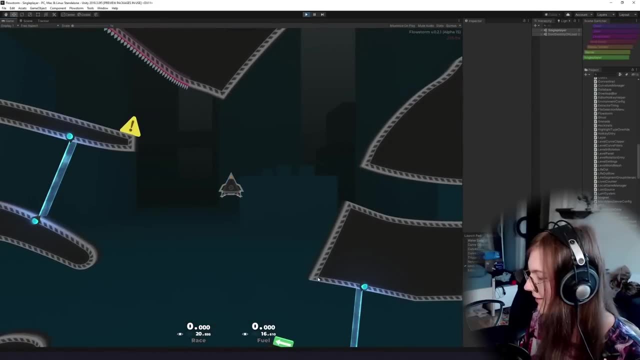 You can hear that it increases in pitch. Um, okay, So so far no dot products, right? Uh, if you move fast, we increase the pitch. If you move slowly the pitch is lower. Um, sort of the same thing with uh sliding. 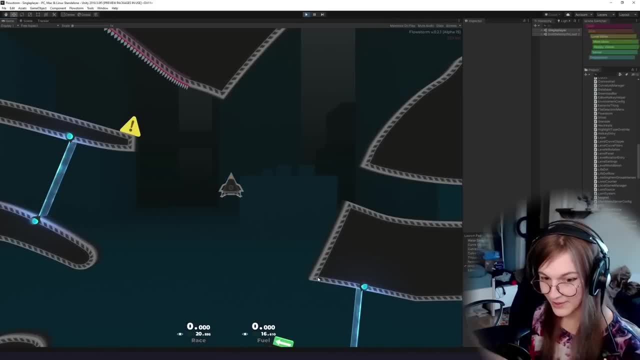 Like you can hear the pitch change depending on, um, if you're moving quickly or slowly, Right, Um, so the thing that I'm using the dot product for is that if you are accelerating and you're turning the rocket left and right, actually, let me do. 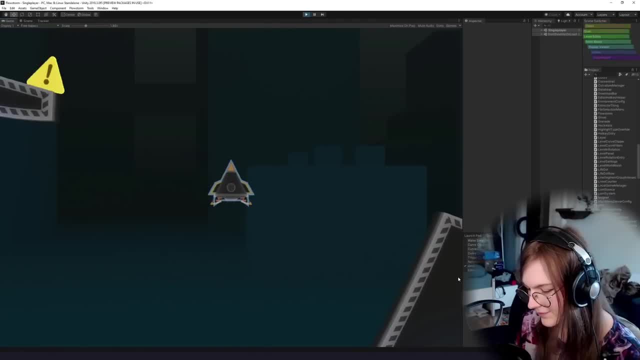 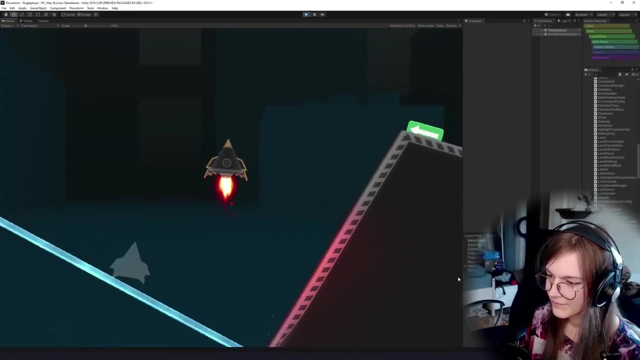 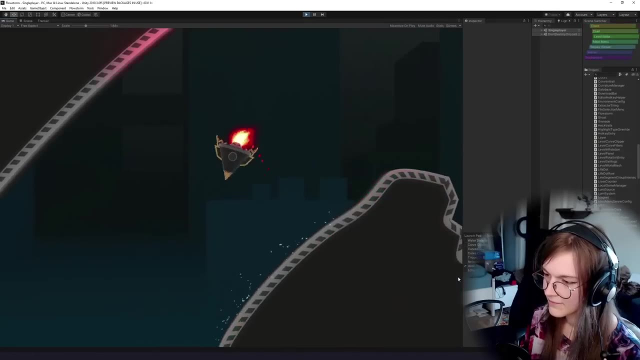 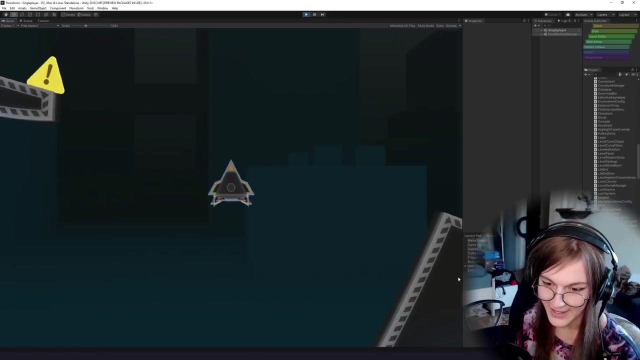 Uh, zoom in, uh, then the the pitch is going to be different. It's not just based on speed. So if you listen to this while watching the rocket, like if, even if I'm moving, sometimes when I turn the rocket, the acceleration or the the pitch goes down again, even though I'm moving fast, right, 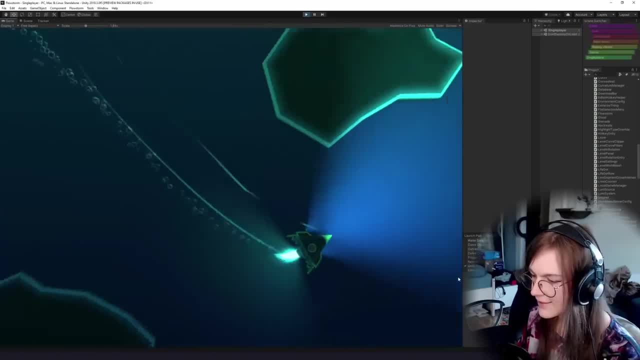 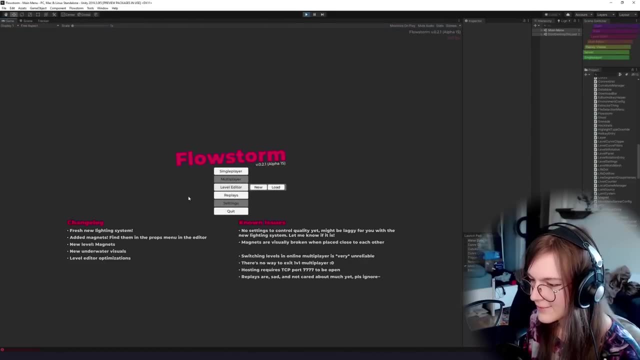 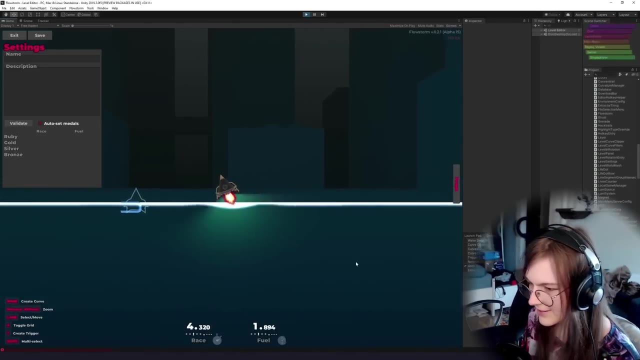 Um, Yeah, so basically what I have done is that actually let's go to the level editor instead, because there's more space. Oh, no, level editor is currently broken. That's okay. We can have NullRefs in the console. 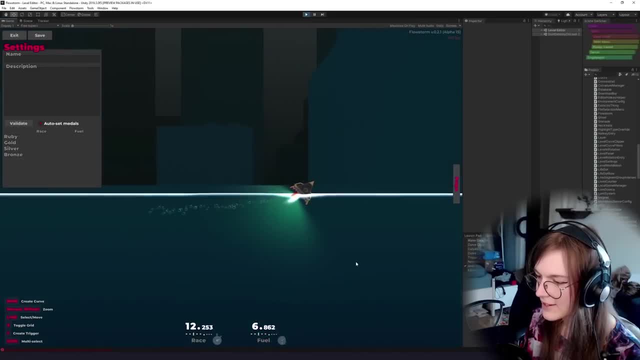 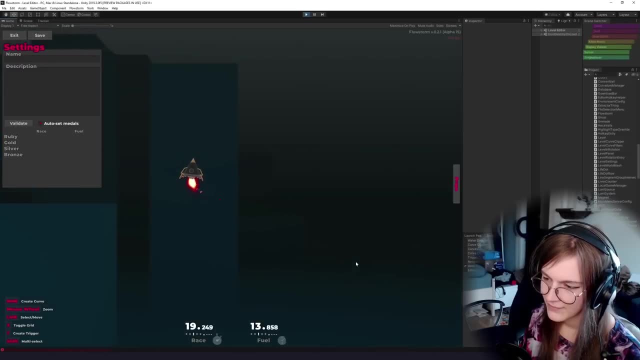 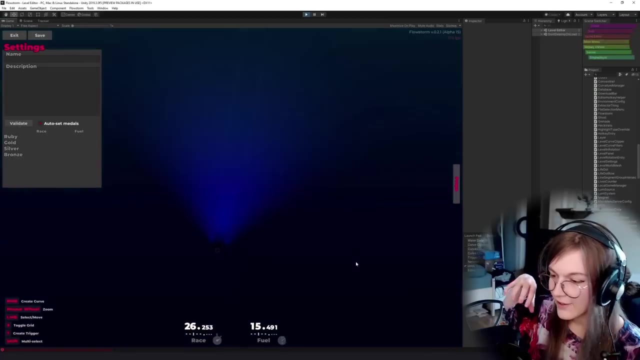 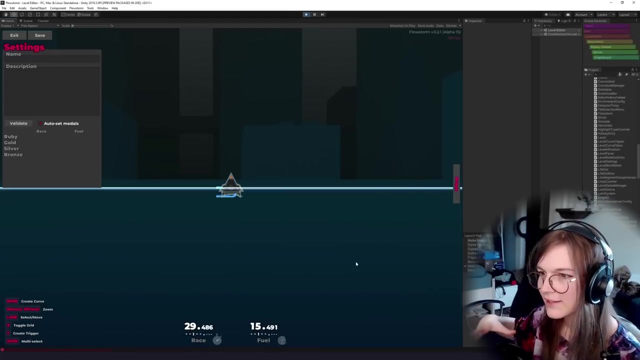 So if you listen to the rocket now we're moving faster and faster sideways. but then I look up, You can hear that every time I turn where the rocket is now perpendicular to the velocity vector, the audio will now change pitch, because what I'm really interested in is how quickly. 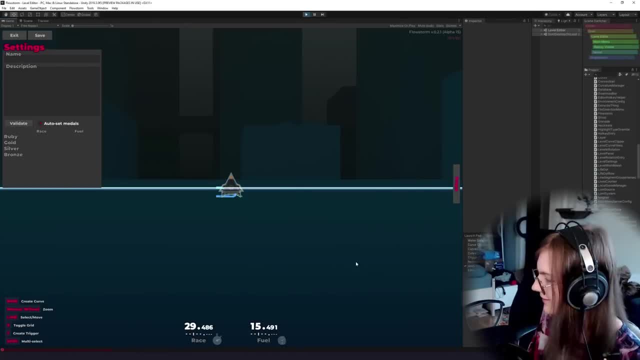 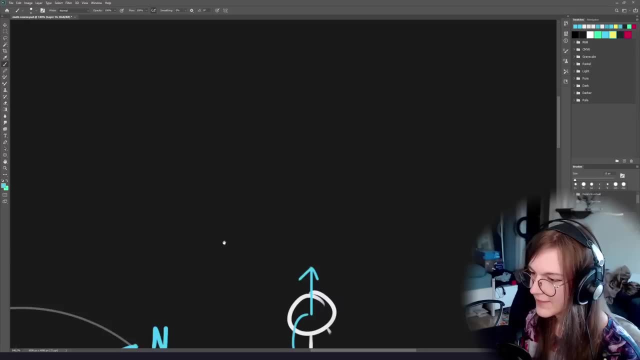 is the rocket moving in the direction you're pointing. That's the crucial thing here. So in this case, what I'm doing is that, instead of a normal direction, I have the direction of my rocket right, So I have this vector right here. 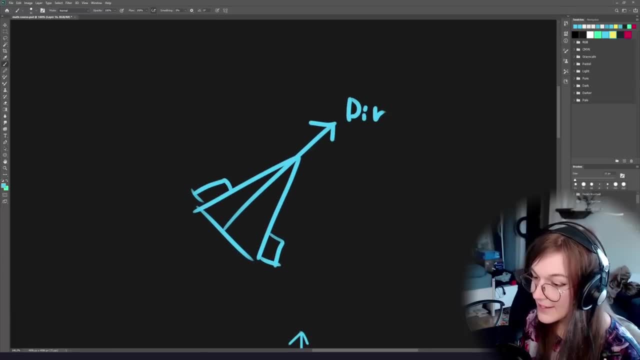 This is the direction. And then I have the velocity right, The actual velocity vector for how quickly you're moving in that direction. right, So the actual velocity could go in either direction. right, It could be in this direction, It could be along this. 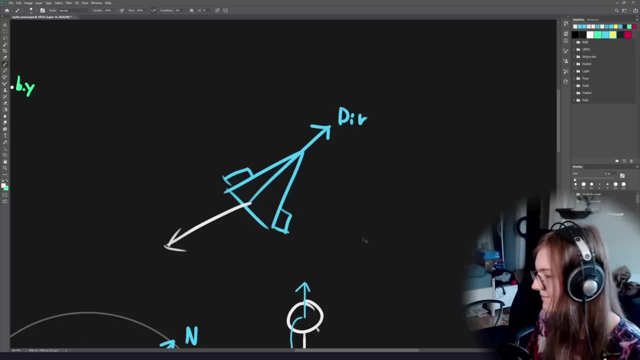 It could be opposite towards it. right Yeah, So that way I can get the speed in the direction, I can get the speed in the direction, I can get the speed in the direction of the rocket, And then I can use that to change the pitch of the rocket. 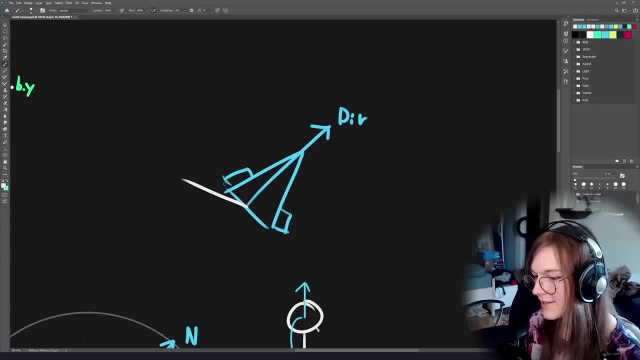 So that's kind of it. That's basically like: just depends on how you're moving, and then project that along the direction of the rocket, And then what I get is: what is the? how much are you moving along this direction? And that's it. 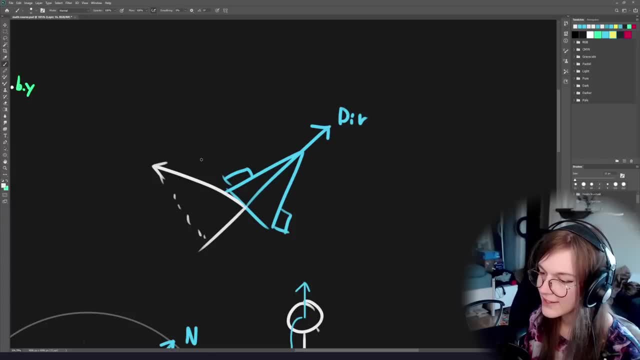 That's how I got the pitch. there Sounds like it's the absolute value of the dot product. Yes, So so that's that's kind of it. Do I use the dark product for something else? I do use it for the impact sound. 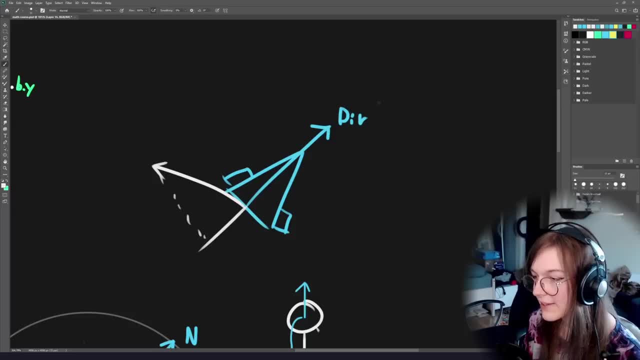 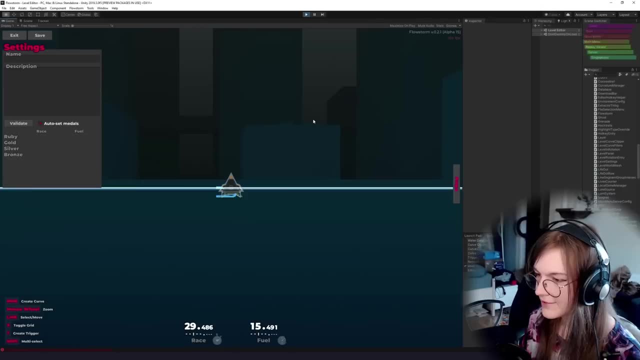 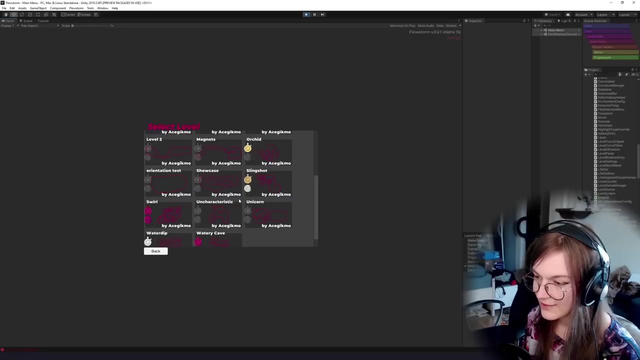 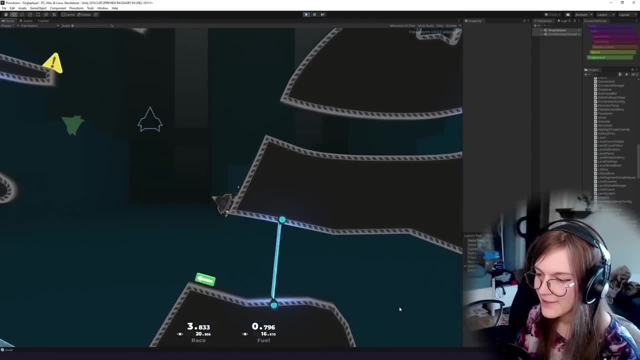 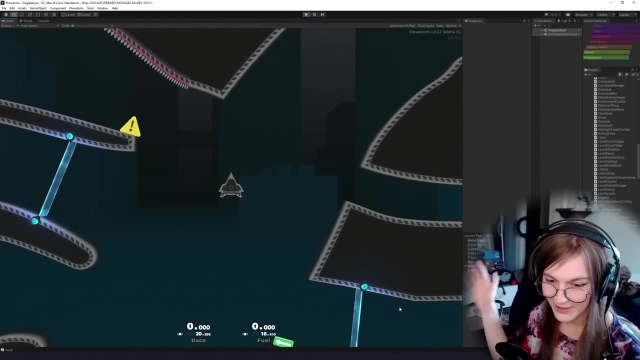 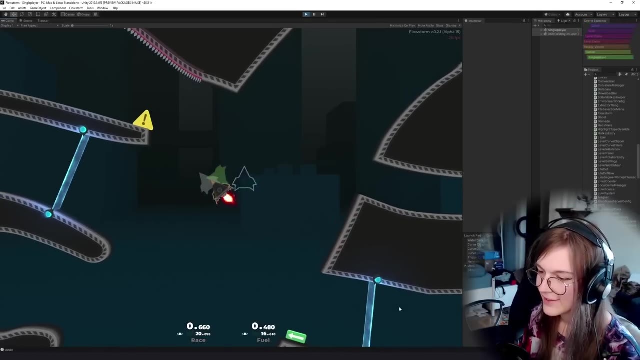 So when you hit the surface, there are little sounds that play. that one is based on the Dark product, just like we talked about. Yeah, Otherwise, there are many like placeholder sounds, like when you crash that's a placeholder sound. So there's lots of stuff that I haven't done in this game, but, yeah, 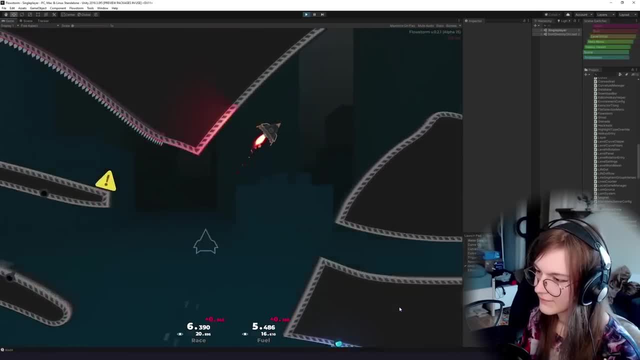 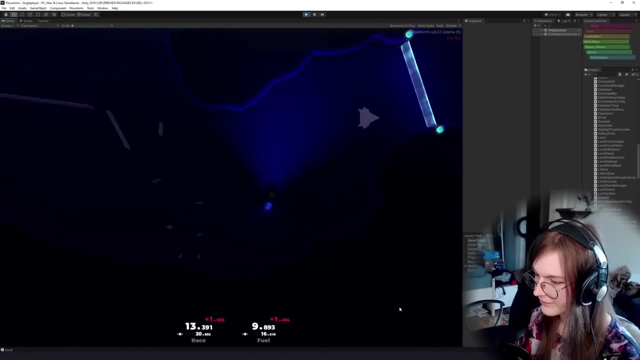 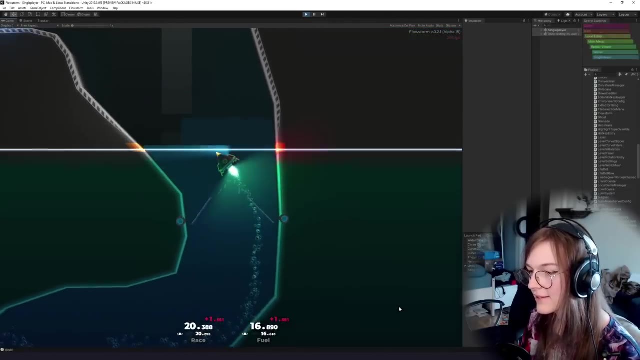 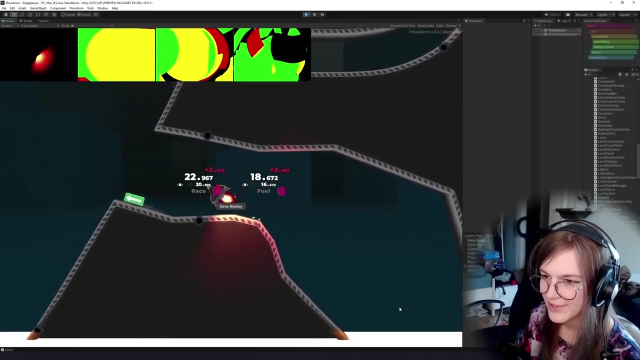 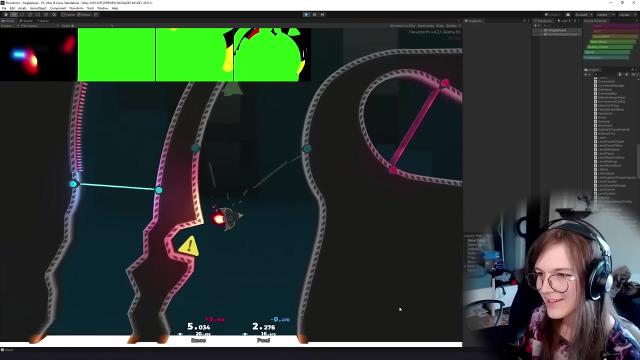 That's r. Oh, someone asked about the lighting in this. No, the lighting is not Unity's built-in one. I wrote my own custom lighting system. Here's some lighting buffers, if you're curious about how my lighting system works. The first lighting buffer is kind of self-explanatory. 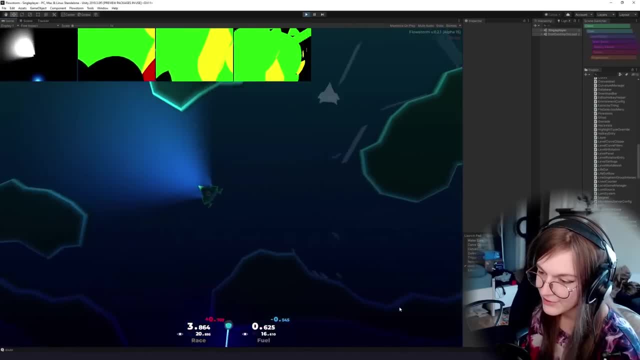 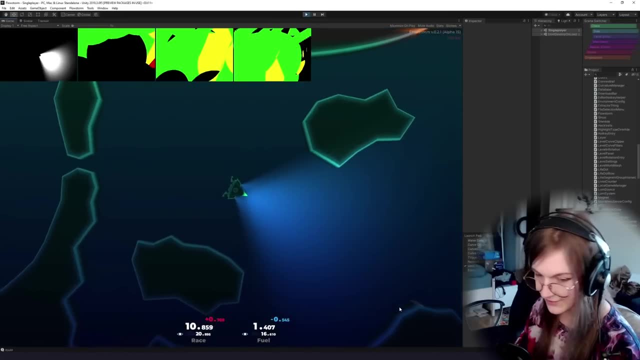 The other three are a little esoteric. Oh, I also use a dot product for the water physics. So underwater, I kind of want you to be able to turn the rocket and that would also change the direction of the rocket. Again, you do stuff with the dot product and the direction you're moving versus the direction. 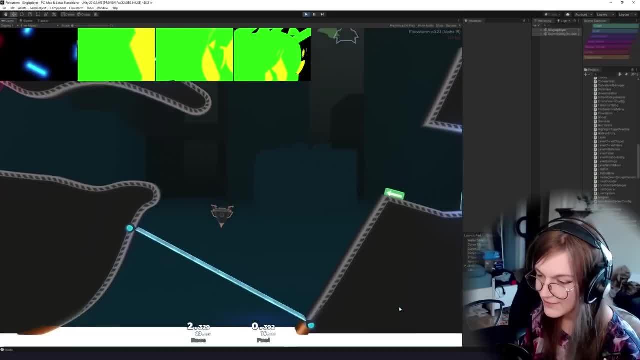 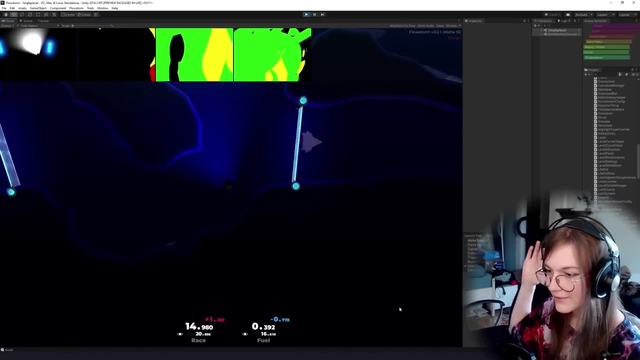 you're pointing, and that way you can make the rocket sort of behave as if you have drag underwater, Right, Yeah, Otherwise, I think that's it, unless you have more questions. Now I'm going to try to figure out what assignments to give you. 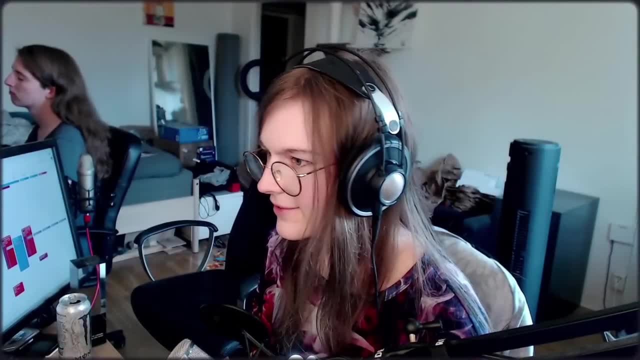 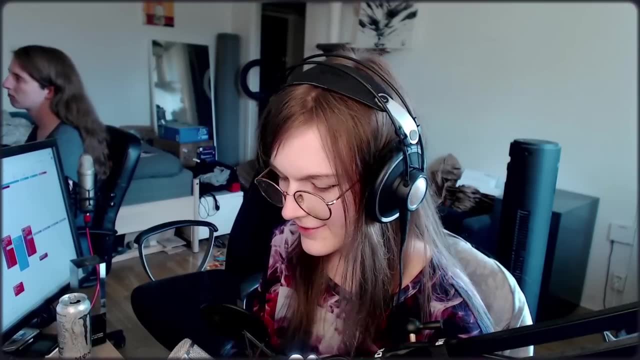 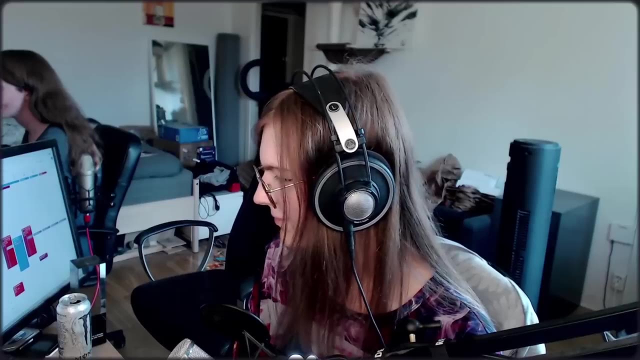 Yeah, I'm just going to have a slow Q&A thing while I figure out the assignments. All right, I got two out of maybe three, four assignments- I haven't decided how many yet. Be gentle. I mean, we've mostly gone through a lot of fundamentals right now, so I'm not going to 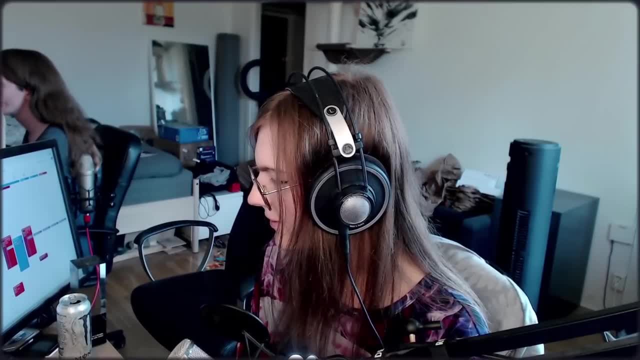 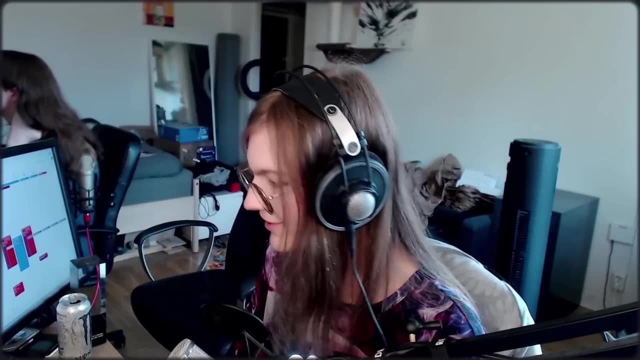 do something super advanced. What do these assignments do? I have no idea. I think Krista is going to do one. Okay, I'm just going to do all of the assignment stuff. He's also going to be correcting them, so I'm just going to make assignments and then. 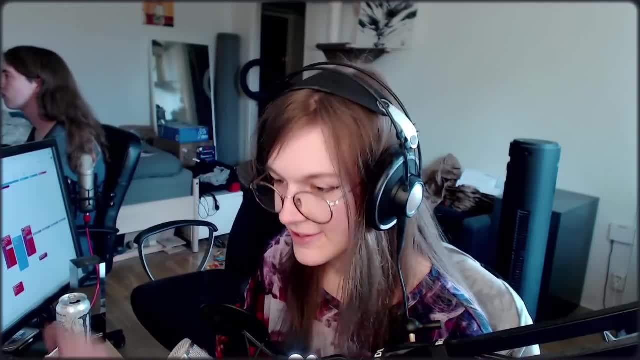 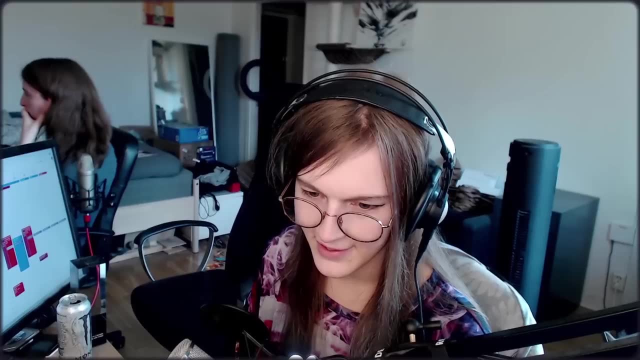 Krista can decide everything else, And also Krista is going to be doing the grading and whatnot. Okay, There we go. Assignment one is now ready and I'm going to reveal all the assignments as soon as I'm done writing them. 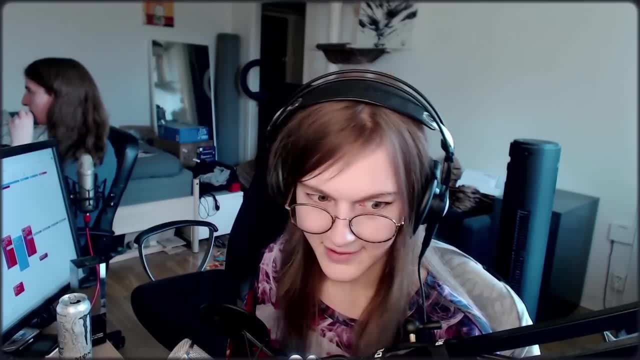 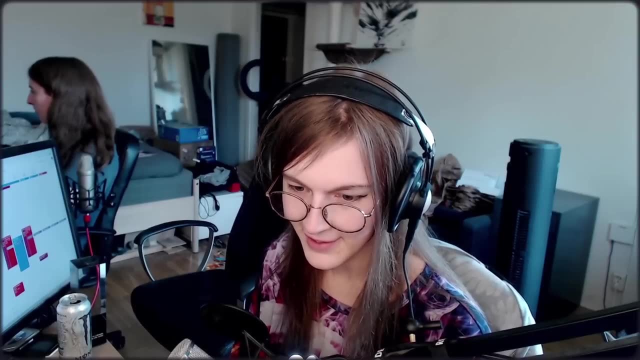 Assignment two has a thing we didn't talk about today. Isn't that spicy? Okay, All right. So I'm going to show you all of these. All of you know what transformforward means, or transformwrite, because those are going to be irrelevant. 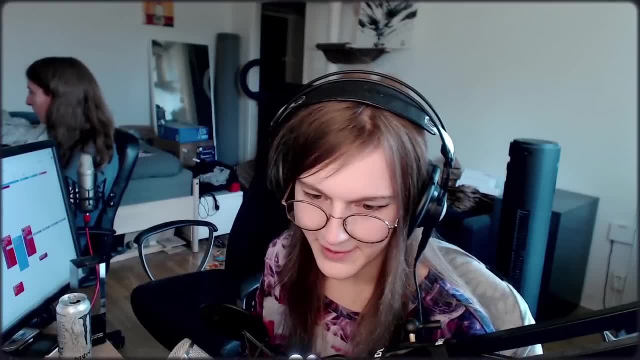 But I presume you've done that already because you've been using Unity for a while. You don't have to be a student to see them. I will show them as soon as I'm done writing them. I'm just jotting down notes now for the assignments. 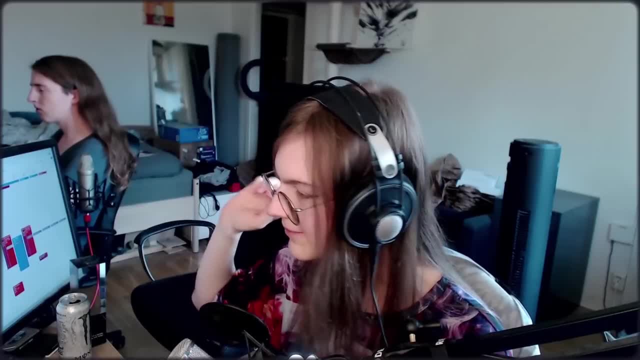 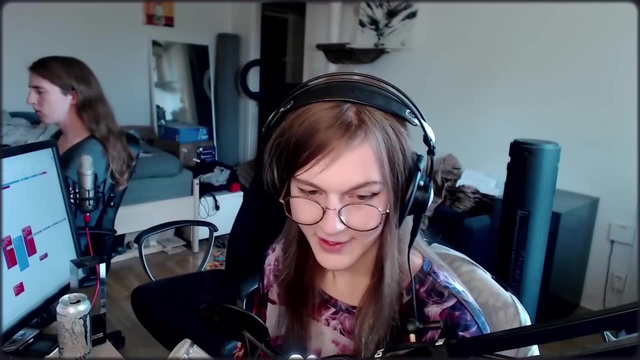 I'm going to draw more specifically. I know you can't see right now. I'm going to draw what the assignments are going to be. A lot of these concepts are probably going to be very easy if you rewatch the stream and whatnot. 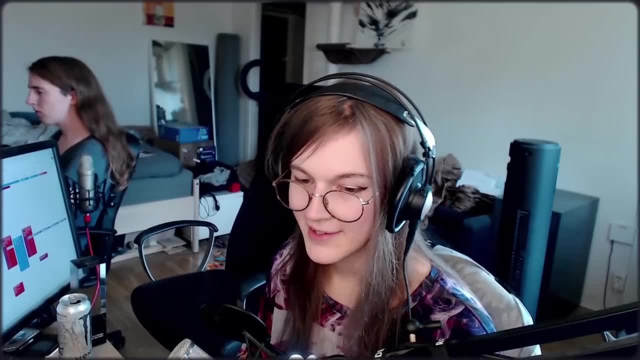 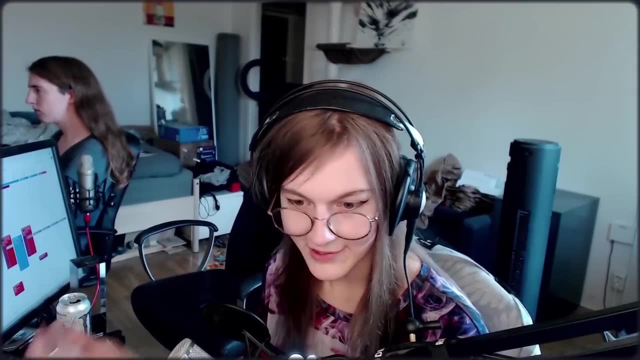 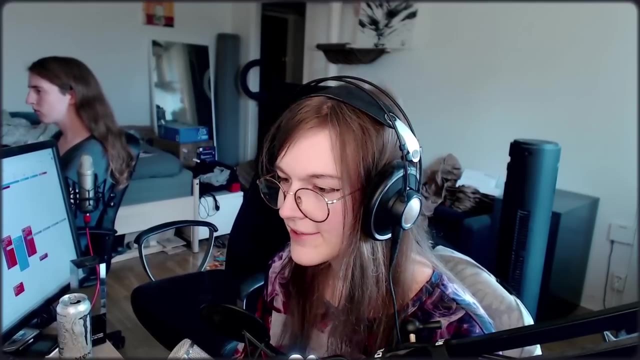 So it's mostly about I want you to get some practice in actually doing the assignments and practically writing code that does the things we've been talking about, because that usually helps you solidify what we've been talking about. So try not to copy code from each other unless you really really have to. 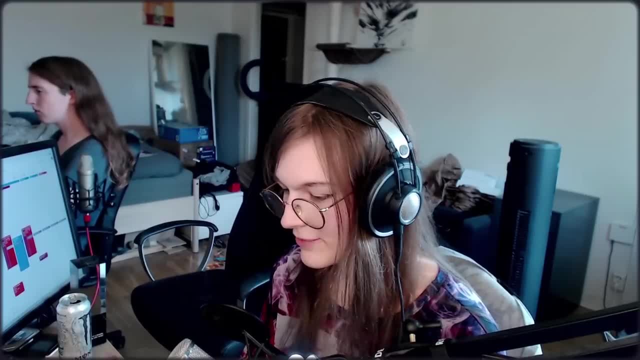 So try to see if you can do it on your own at first, because that's kind of a better way to make sure that you've learned the things you need to learn. Otherwise, of course, look things up if you need to, But it's always good to make sure. 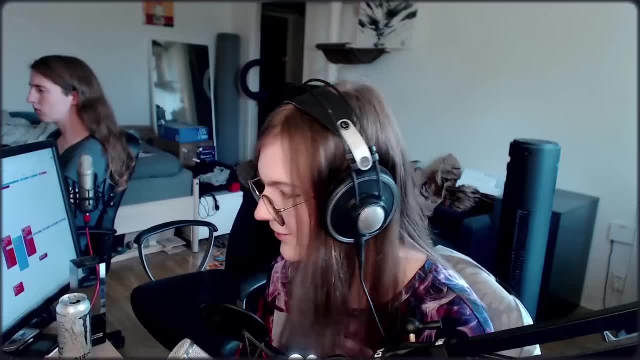 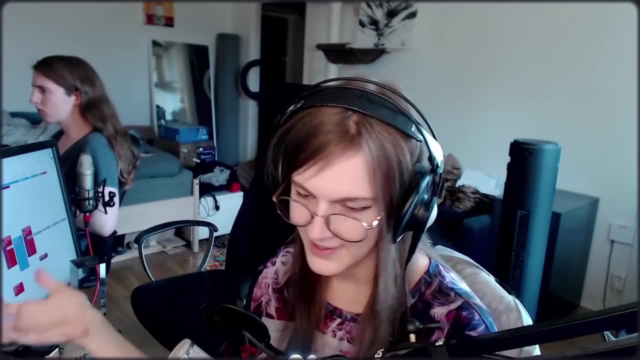 It's always good to make sure that you actually know what you're typing. If you're not sure what you are doing when you type vector2.dot, you should know what is happening when you do that, which you might not if you just copy someone else's code. 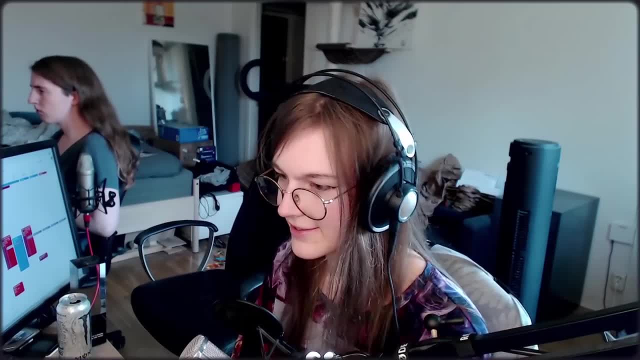 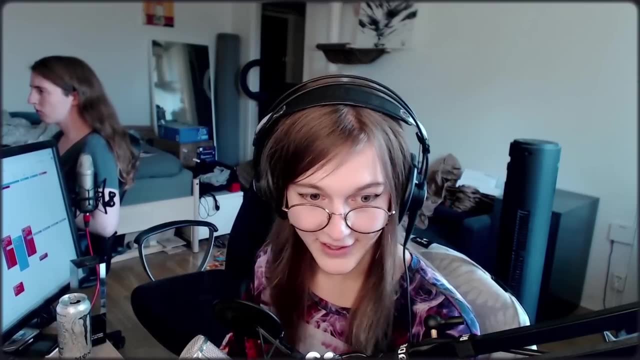 right, Because, again, my goal is for you to learn what these things are. I don't care if you do the assignment or don't do the assignment, or copy code, I don't care, But I want you to learn. I want you to learn the things that are important to you. 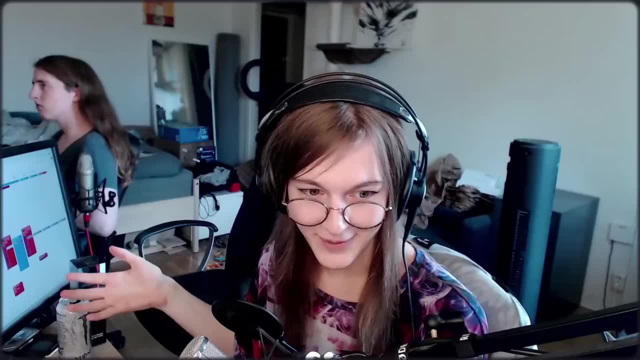 But then again, I'm not going to do this. I'm not going to do this. I'm going to do the grades. Krister probably cares if you copy or cheat or whatever, and if you do them at all. Okay, All right. 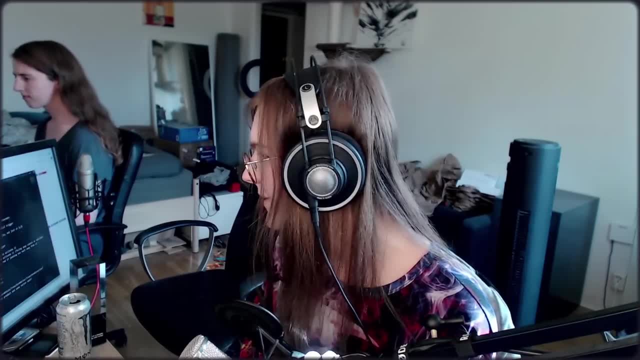 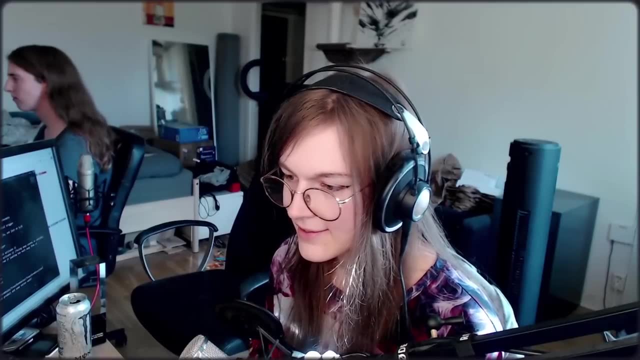 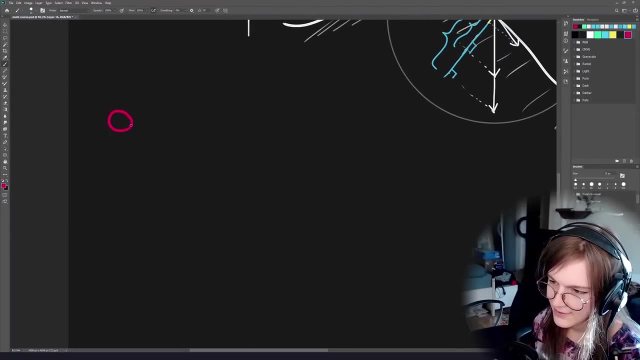 I got the assignments And here we go. I'm going to draw these so that it's very clear what they're doing And I'm going to post both the pictures and the text for it. Assignment number one: Yeah, I think the date for these assignments. 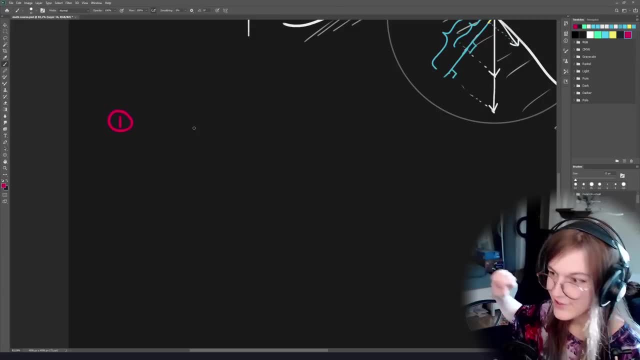 It's probably going to be much later, as in, you don't have to do them tomorrow. If you do them tomorrow, that's going to be good, because then I'm going to cover these assignments at some point, And so it's probably good if you've done them before that. if you want to like maximize. 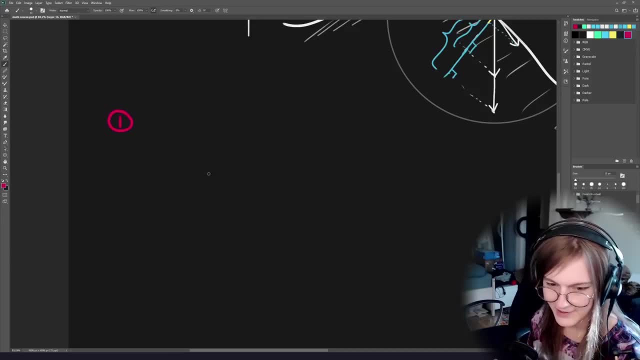 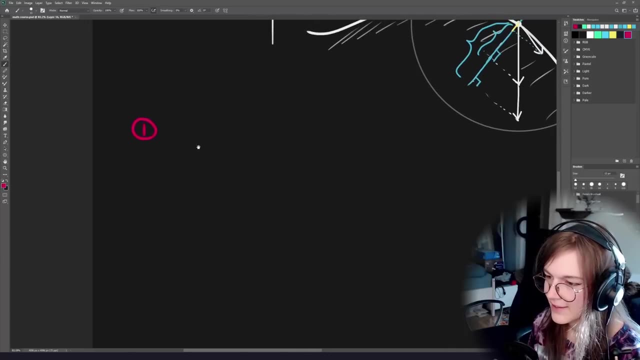 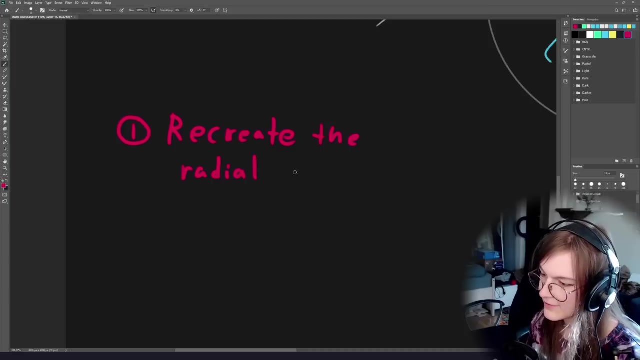 your learning. But if you're stressed, then I mean, don't stress yourself out. Okay, Cool. First assignment: Zoop. Okay, Okay. So we're going to create the radial trigger. So this is the thing we made on stream. 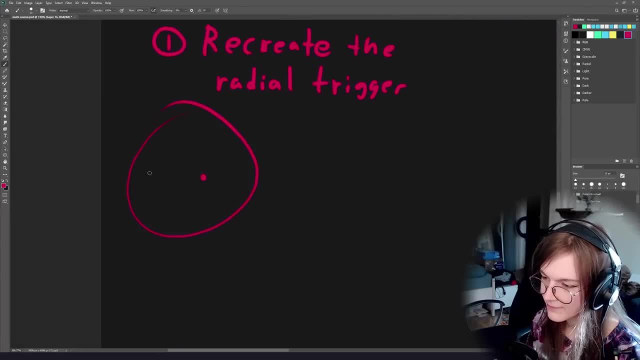 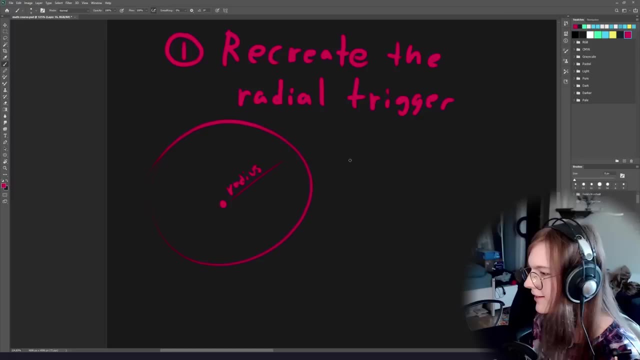 We had a trigger that had some radius. right There we go, It's got a radius And then we want to detect whether or not a point is a point. Okay, So we're going to create a point and then we're going to say, okay, this point is inside. 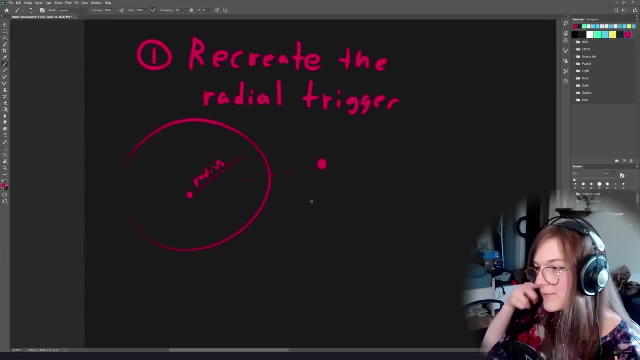 or outside Right Based on this trigger, And the trigger should be able to be anywhere. You need to be able to move the trigger around, You need to be able to change the radius And it should still be able to detect whether or not this point is inside or outside. 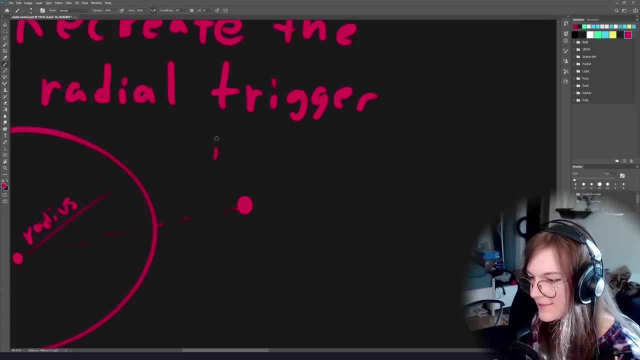 Right. So that's all you need to do: really Like it's inside versus outside, And you can do all of this in Androgyzmus. You don't have to make like an actual update loop or whatever. 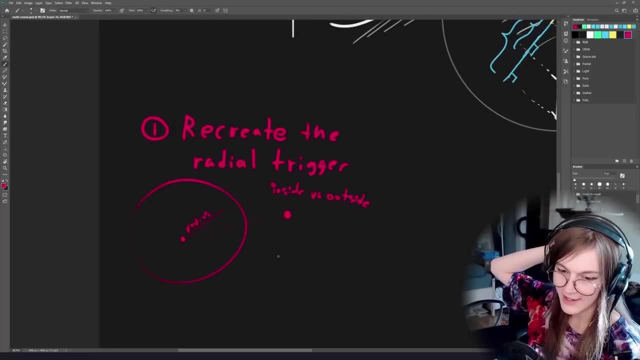 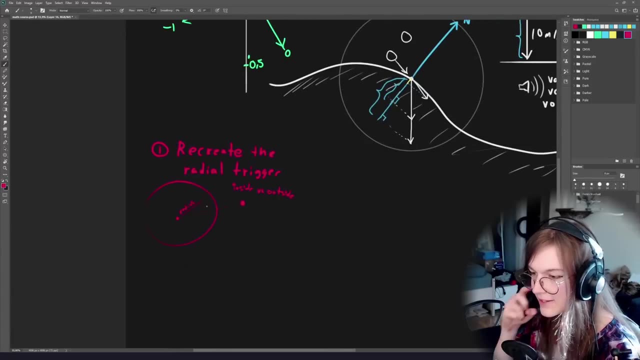 Just do it in Androgyzmus. The point is I want you to like, try this out yourself and make sure that you've actually like you can do the concepts that we've been talking about Right. So recreate the radial trigger is the first assignment. 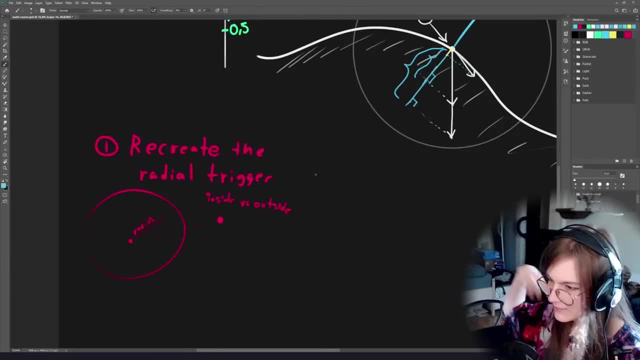 Can it be moved and seen only? Yes, You don't have to animate anything, It doesn't have to be in play mode, Just the same way we did it on stream, Just to like make sure that you know the mathematical concepts. 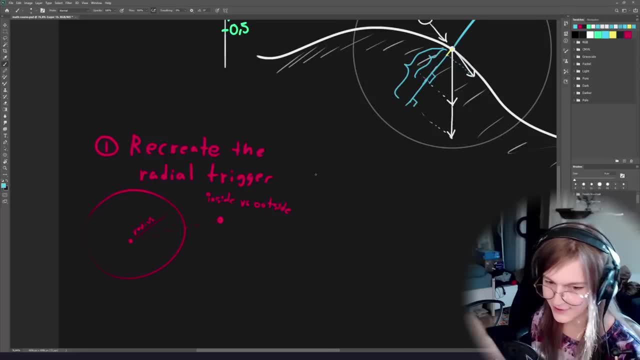 But like you don't have to involve yourself, You don't have to involve, like physics or rigid bodies or game play or anything like that- Just to make sure that, like you have the idea of detecting whether or not something. 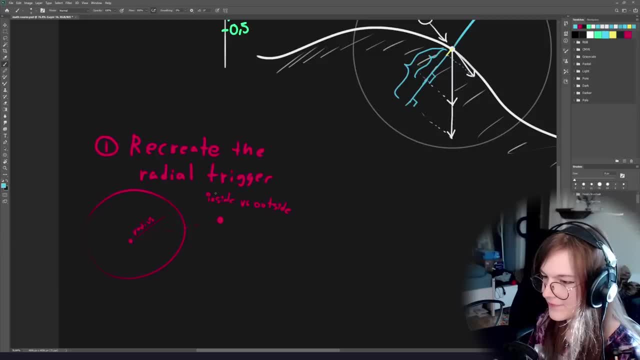 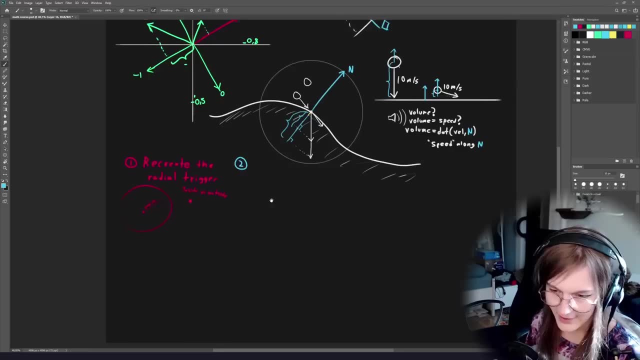 is closer to something or not, Right, Yeah, So that's one way of doing it, Or that's the first assignment. So assignment number two: So previously we the radial trigger kind of checked, like you know. are you inside of? 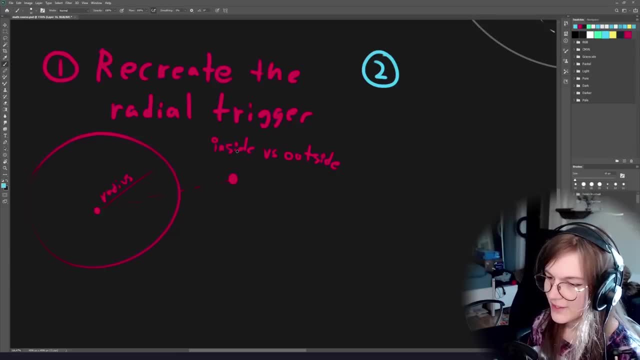 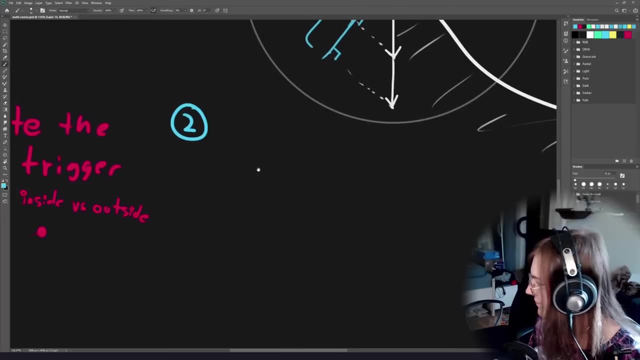 a trigger or outside of a trigger, Right, And that is B. It's based on the radius. But now I want you to make another trigger. I feel like I had a name for this. Actually, I just renamed it. There we go. 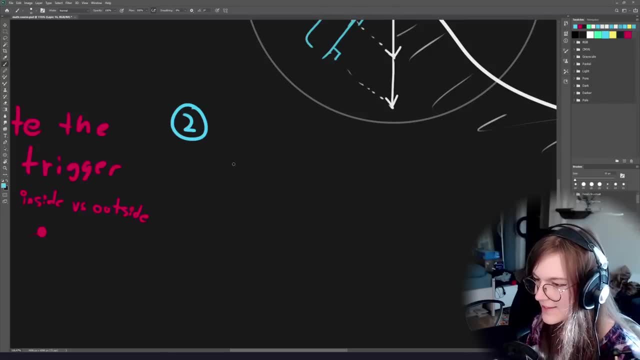 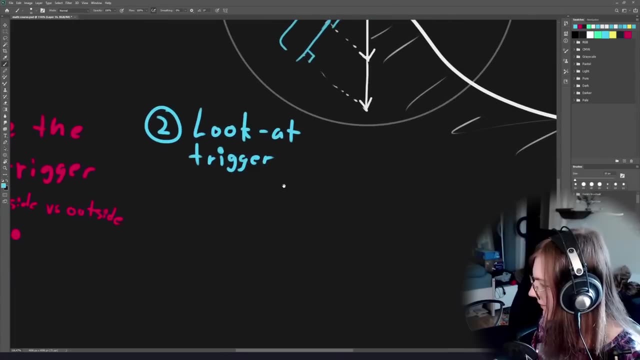 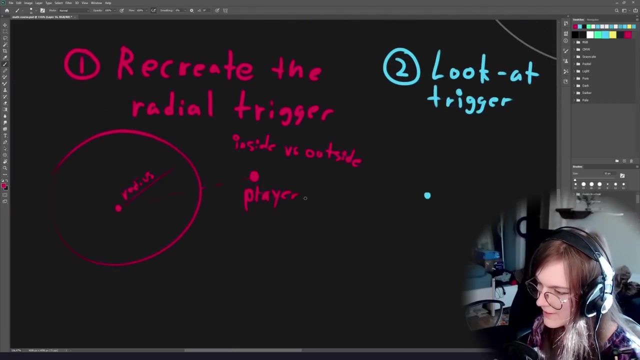 That's how rebellious I am. So the next one is that I want you to make a look at trigger, Okay. So basically you have a similar thing here. You have a actually let's name this player, There we go. Player objects. 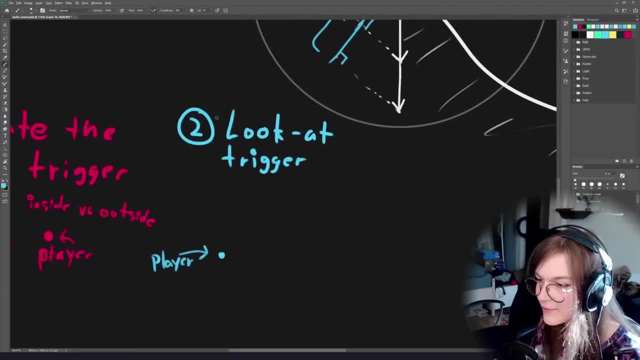 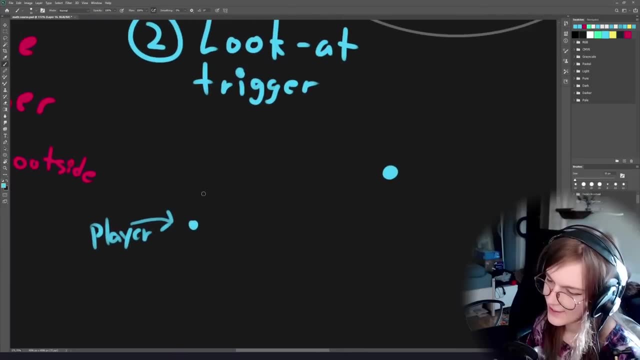 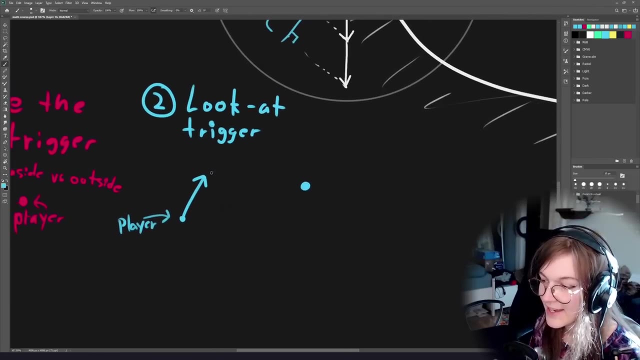 Another player, Cool. So then we want a look at trigger. So in this case, if you have the trigger at some point and then the player is looking in some direction, we want to be able to detect if you are looking toward this trigger. 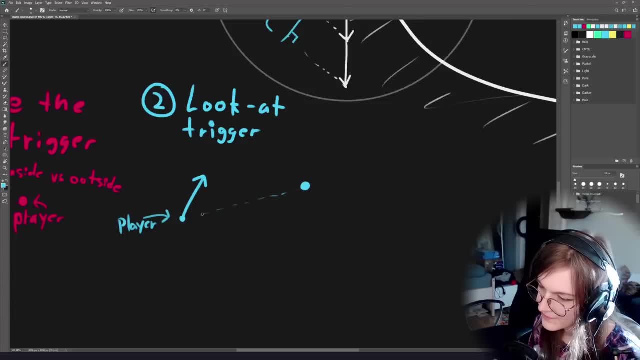 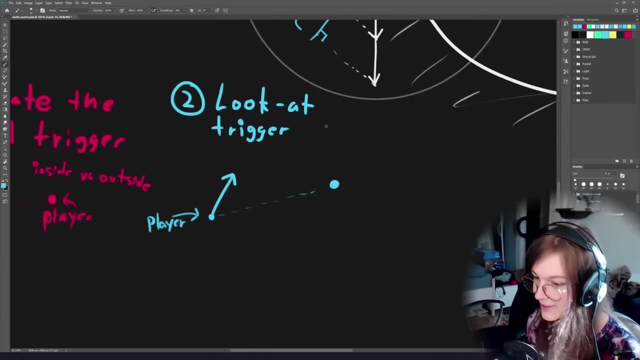 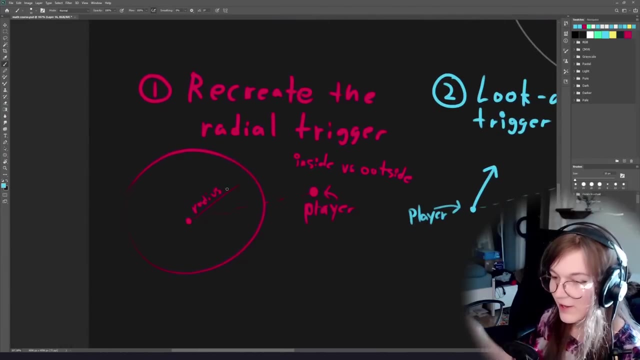 So if you are looking at this trigger, you want it to be true. If you're looking away from it, you want it to be false. So this one should also. you know, this one has a radius that you can modify to set the. 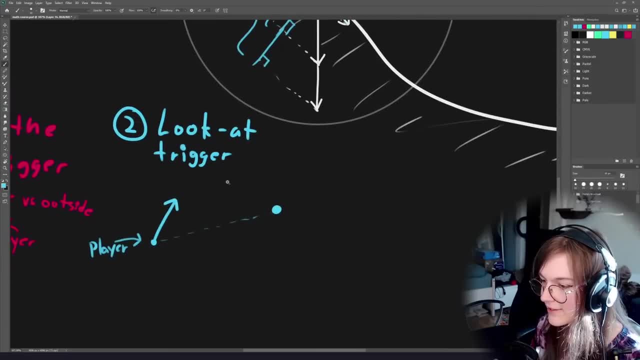 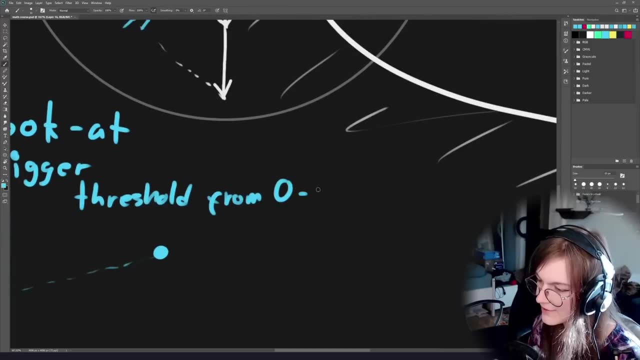 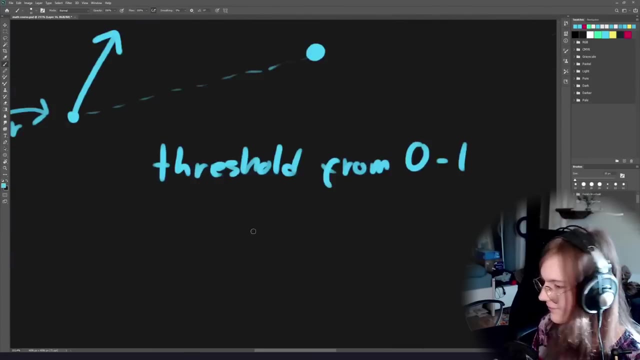 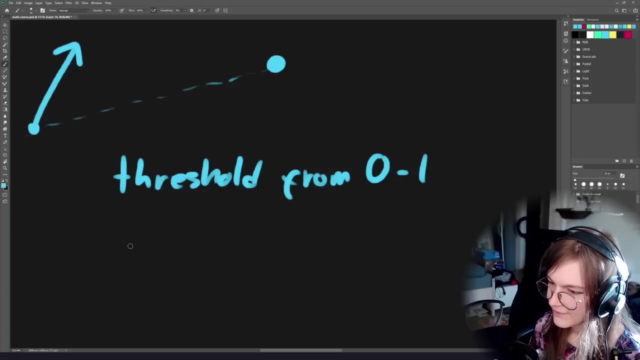 threshold of this, The look at trigger, should also have a threshold from zero to one. So So, let's see- actually let me move this down because I need to clarify a few things- All right, so threshold from 0 to 1.. And if the threshold is 1,. 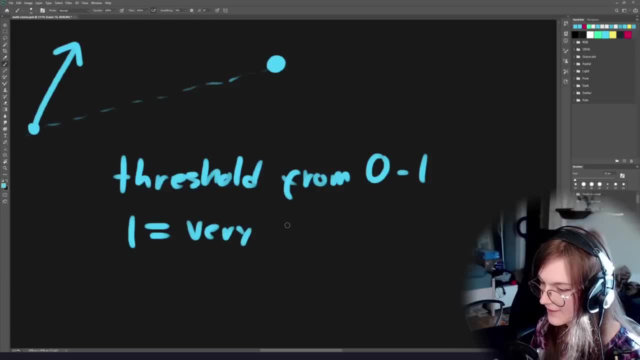 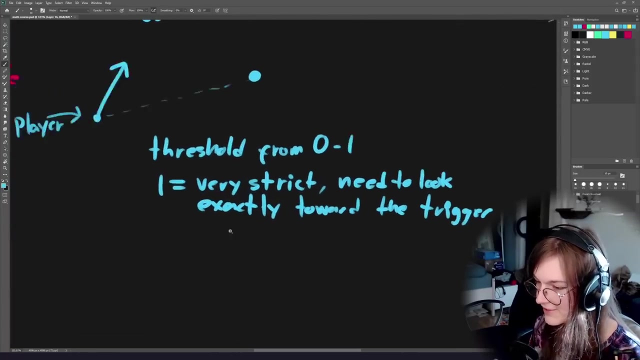 that means that it's going to be very strict? Probably impossibly so, because you're probably never in practice because of, like, floating point imprecision. All right, so 1 is super strict And this is a floating point value. You can set it to 0.5 and 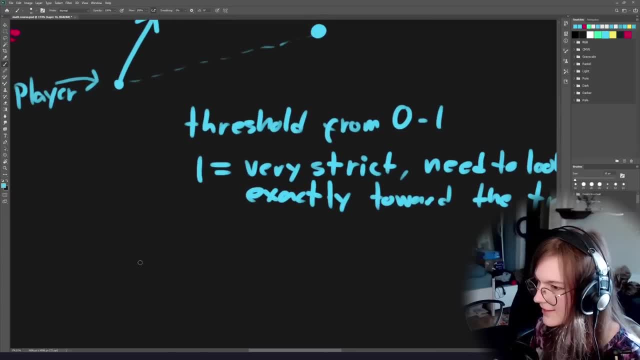 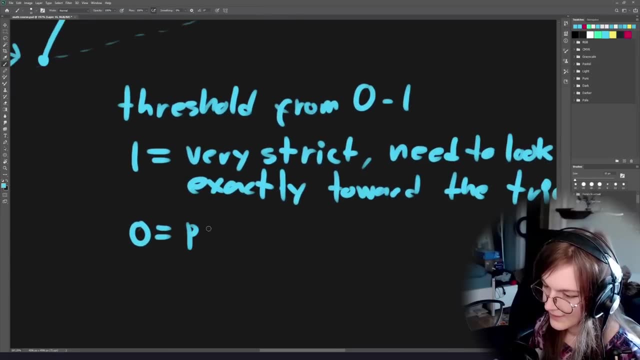 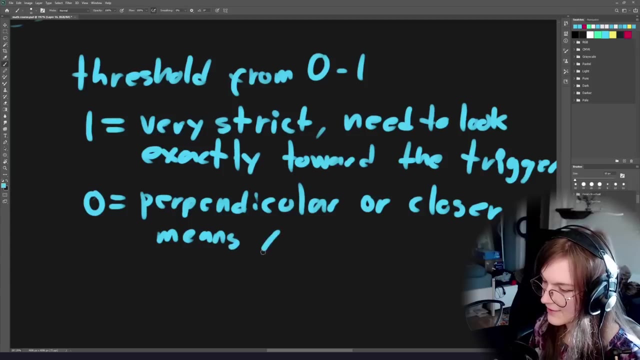 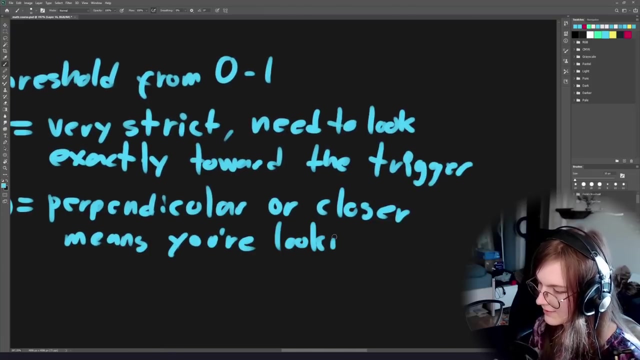 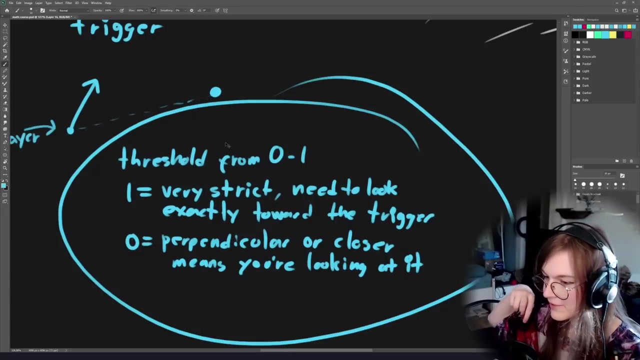 everything All right. And then we: if it's set to 0, that means that so perpendicular or closer means you're going to look at it. There we go. So this is the threshold, So you should be able to. if this is set to 1, you have to look like exactly at the thing And it's going to count. 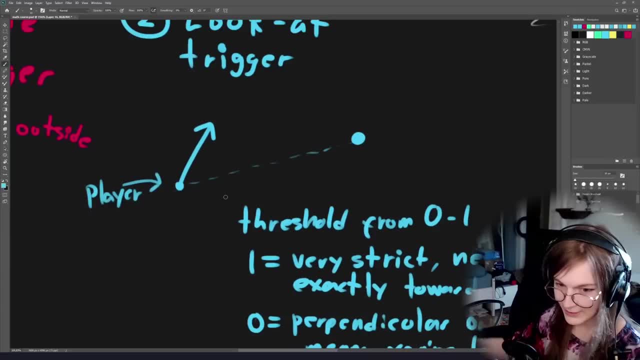 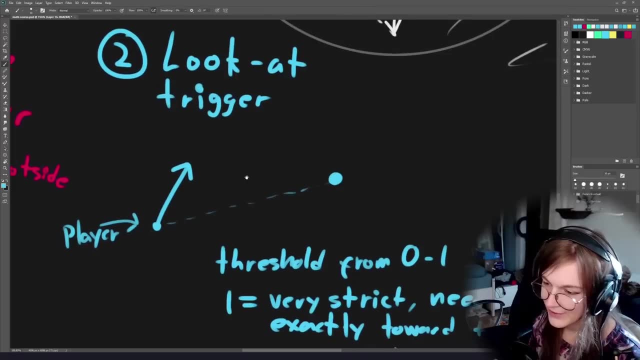 as triggered. only if you look exactly at it, Because of floating point precision, that's going to be like pretty much impossible, never going to happen. But if you set it to like 0.5, it should allow you to look a little bit away and still count. 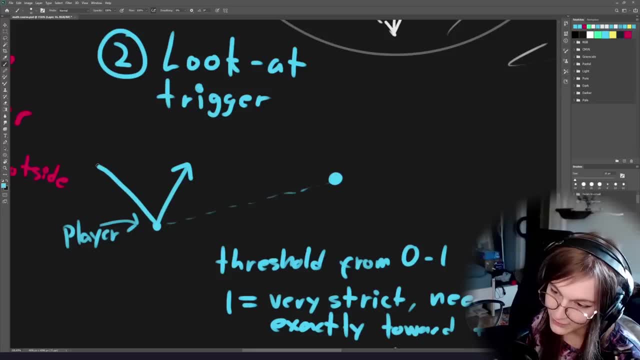 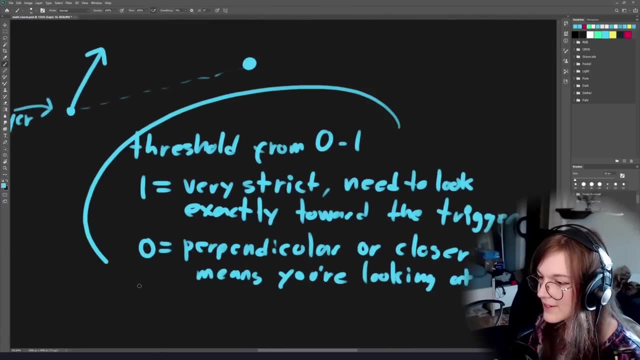 as looking at this thing, But then as soon as you are looking away from it like this, that should not count as looking at it right. So, basically, this threshold should set how sensitive it is. If it's a 1, it's hypersensitive. you need to look exactly at the point. 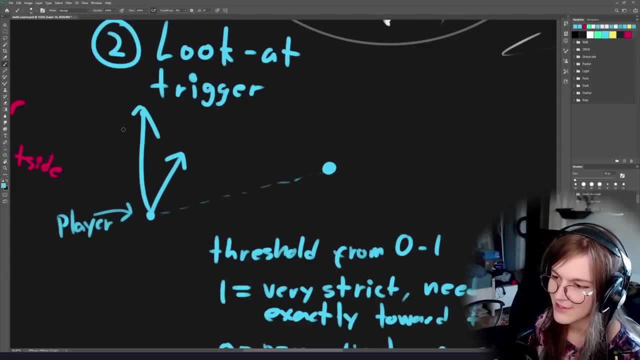 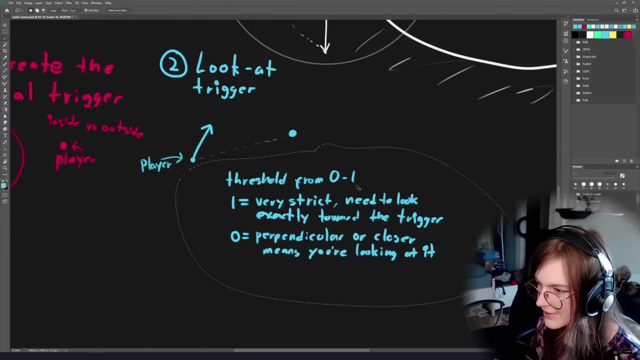 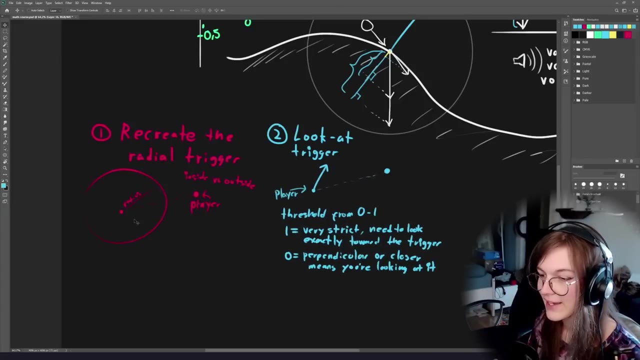 If it's 0, it's not very sensitive at all. If you look in this direction, it's going to count as looking at the thing, right? Yeah, that's about. that's about it. for for number two, To clarify, we haven't talked about angles yet, So we're this doesn't involve angles. 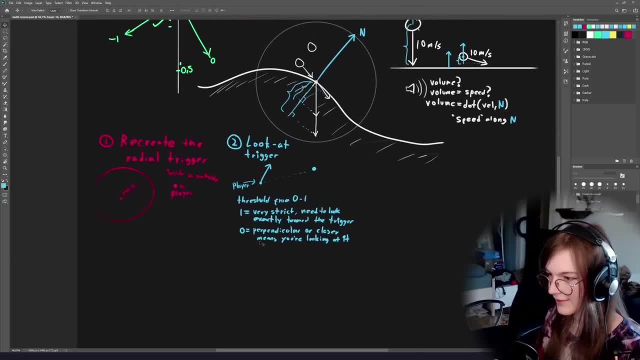 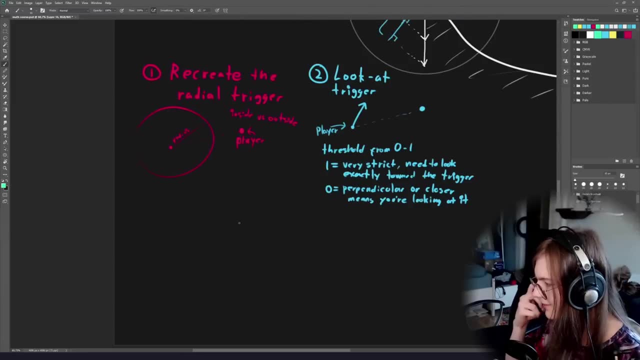 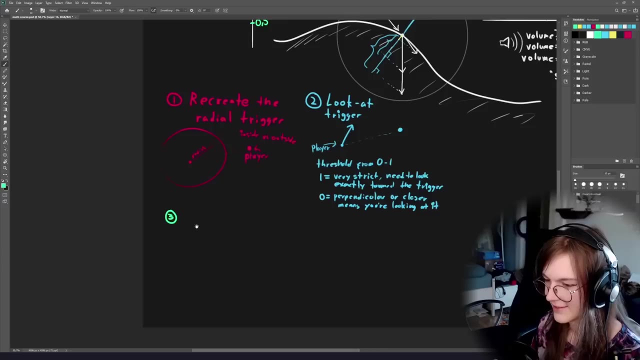 None of this is anglebakes. This is still just vectors. All right, And let's do the third one. Still just vectors. Yeah, angles don't exist. You've never heard of angles. This one is smaller, Okay, heck, I'm trying to figure out how to draw this one without 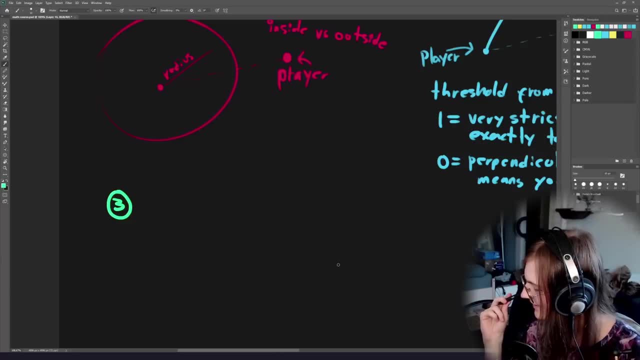 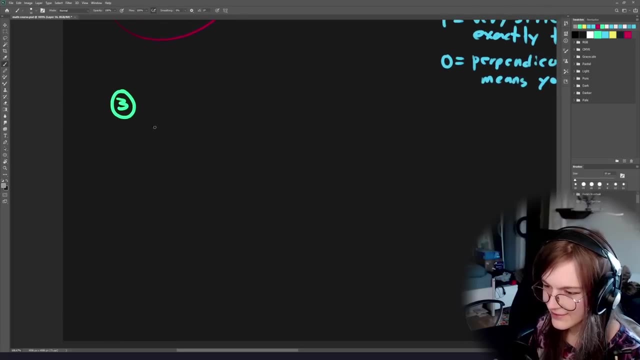 spoiling the solution, Because this is kind of difficult. So this is the one we're going sort of toward concepts we haven't talked about yet, But that's a little teaser thing or something. So let's say: this is the origin of the world, Like, this is 0, 0. And then you have an object. 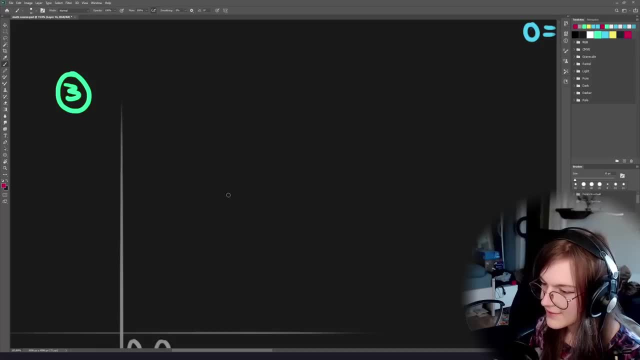 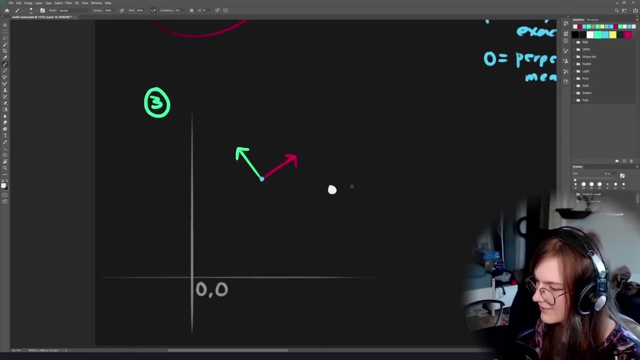 in Unity that has some some orientation, right. So usually Unity, you would have this gizmo that looks something like this, And then you'd have the z axis pointing toward the camera And then let's say: you have a point, There we go, Okay. and then you have this object. let's call it object. 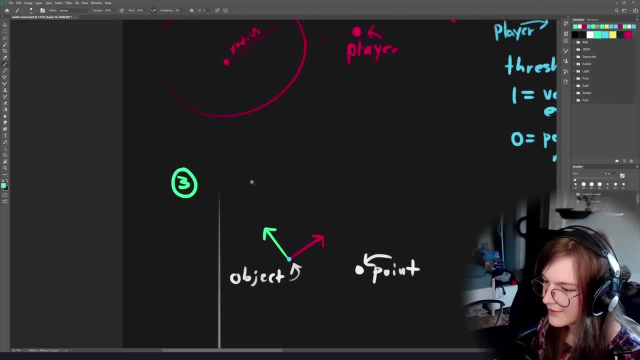 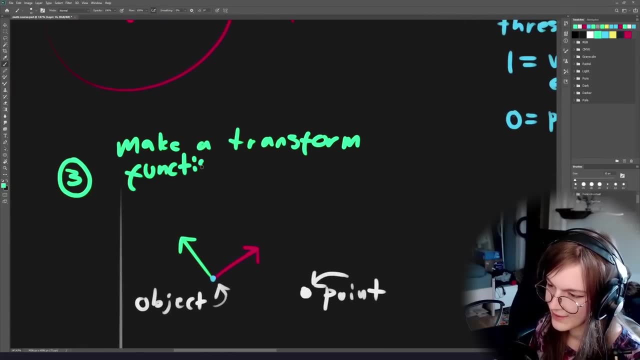 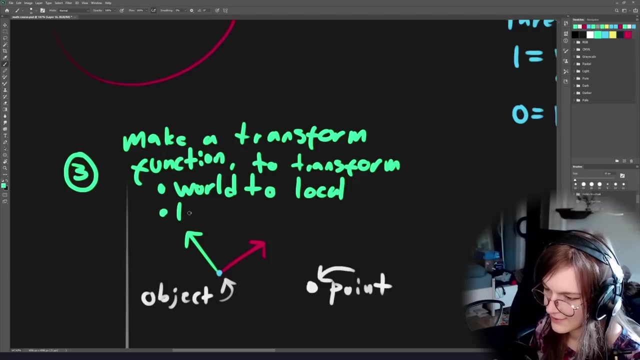 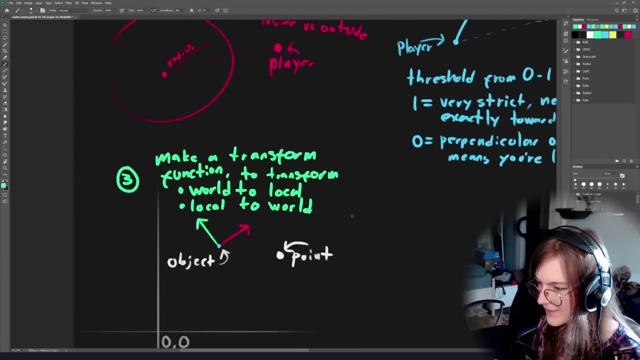 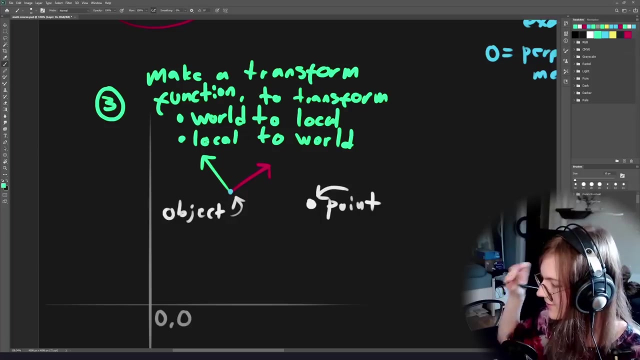 So this one is: I want you to make a transform function to transform from world to local and local to world. Cool, Okay. so the goal is I want you to have a transform in the scene that has some rotation and a position, And I want you to write a function. 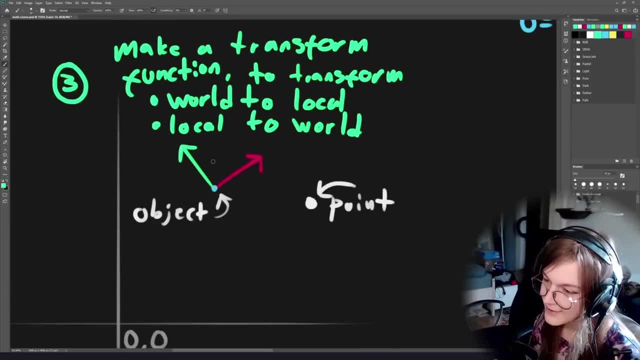 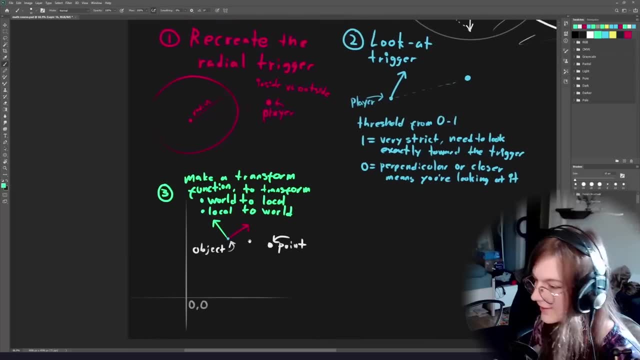 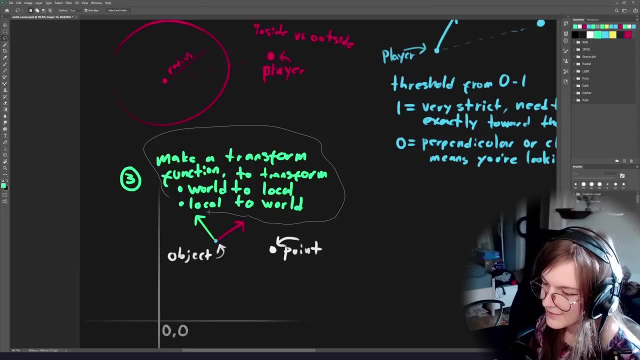 that can transform this point either into local space of this object or from local space of this object to world space. We haven't talked about spaces yet, So that's why this one is a little bit of a curveball, But I'm sure you sort of understand the concept of what it means for something to be. 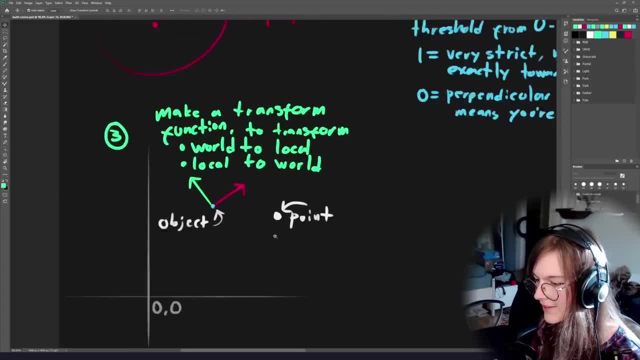 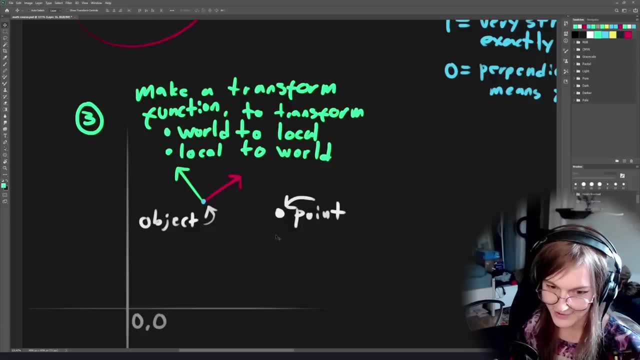 local space or world space. So that's what I want you to do, And you're not allowed to use Unity's transform functions in order to transform this point. You're not allowed to use matrices, you're not allowed to use transform dot transform points, not allowed to use those, those don't exist. 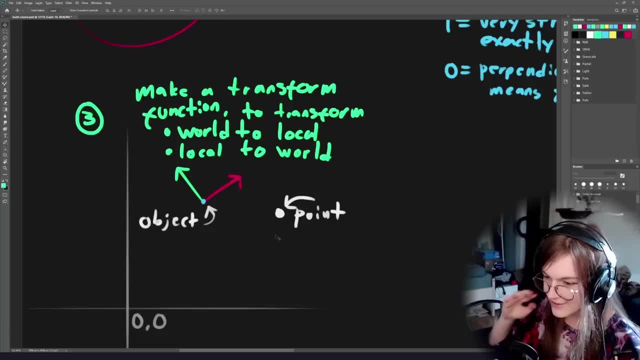 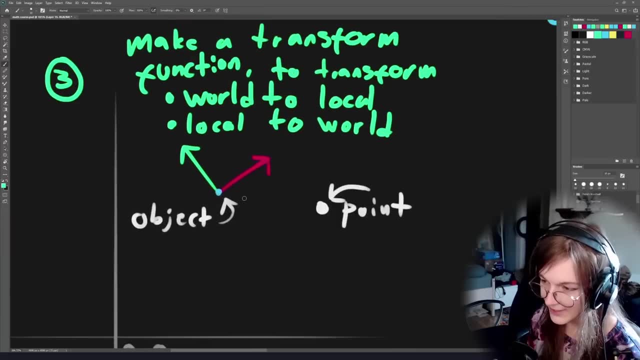 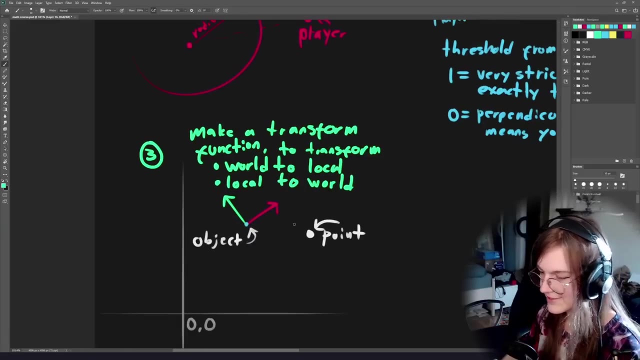 anymore. So so you need to do this using vector math and dot products. That's what you need to do, right? Yeah, you can still use transform dot, right, transform dot up to just get vectors and whatnot, But you're you're not allowed to use the transform functions. No, you don't need. 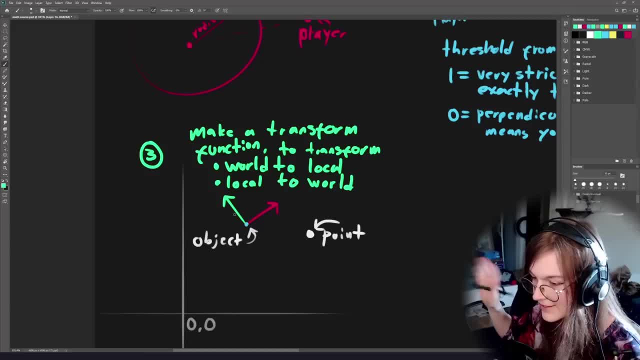 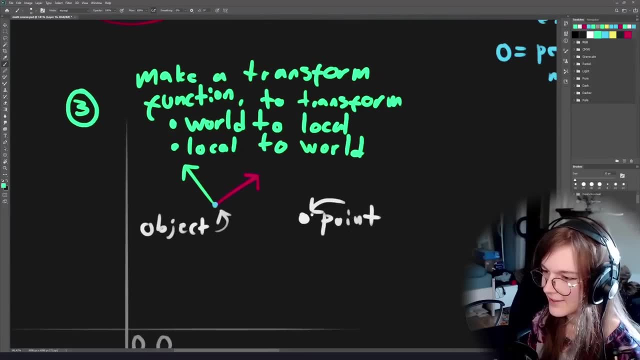 to use quaternions With. this is possible using only the things that we have talked about. Oh yeah, this is 2D only. We don't need to care about 3D yet. So, yeah, 2D only. I don't know where to fit. 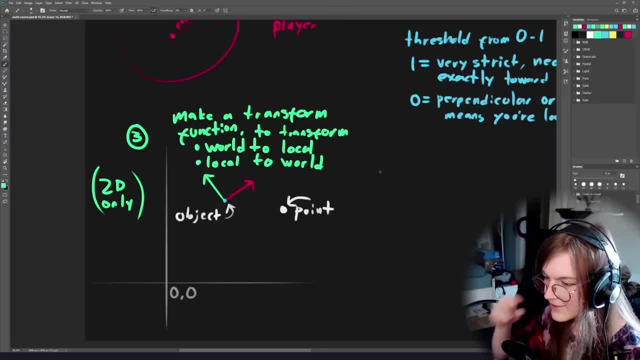 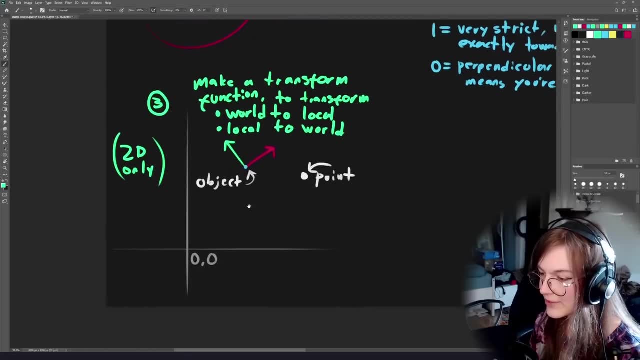 that in, I don't think I get the goal of this. You need to be able to transform a point from world space to local space, which means that you need to figure out where a point is. So if you look at this point, for instance, this is really hard to explain without spoiling the 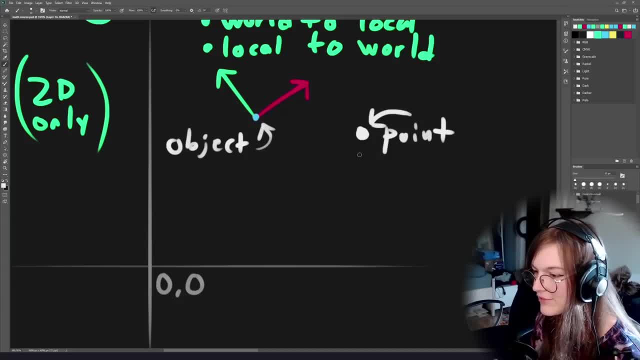 whole thing. If you look at this point here, if you consider the coordinate of this one in world space, well, it's this vector, right? And then you have an x-coordinate, you have a y-coordinate and so forth. But making a transform function means that you should be able to take this point. 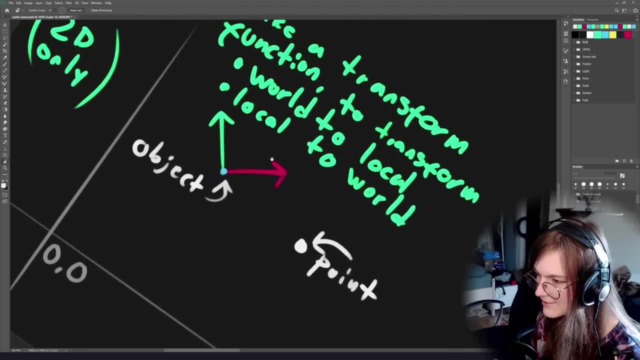 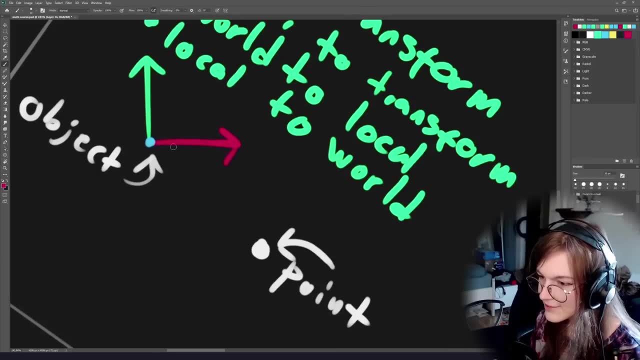 in world space and transform it to this space, As in I want it to be relative to this object. So now I want the x-coordinate and the vector and everything to be based on the local space of this thing, right here, right Yeah, And it should take rotation into account, So it's not just position You can ignore scale. 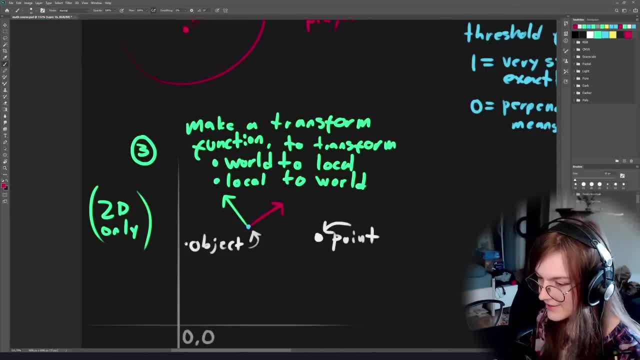 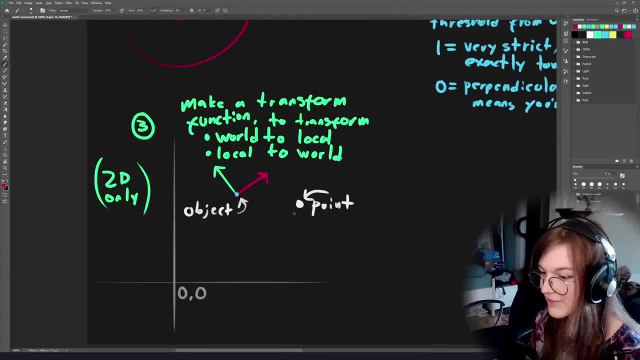 Scale doesn't matter, But it has to take rotation into account, And you can do this using only the concepts that we've been talking about. You don't have to do anything outside of that. In fact, you're not allowed to use matrices or the transform dot, transform point functions. 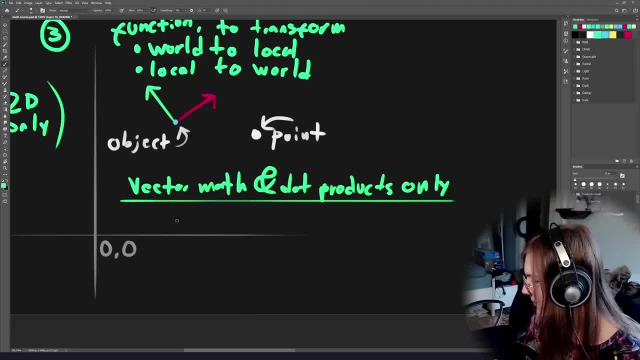 You need to do this with vector math and dot products. If I move the point to the position it would be under the new appearance. If I still have to move point B in world space, you mostly You just need to get the coordinates How you make it in the scene or how you move them around. 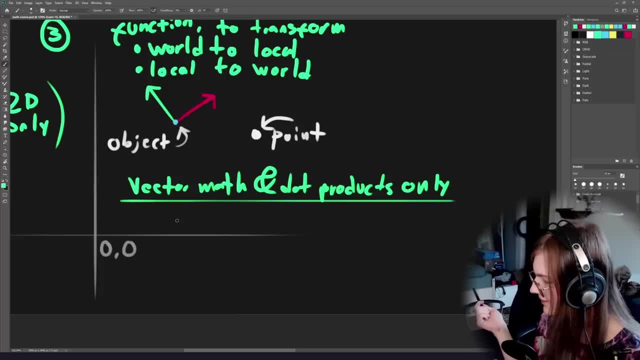 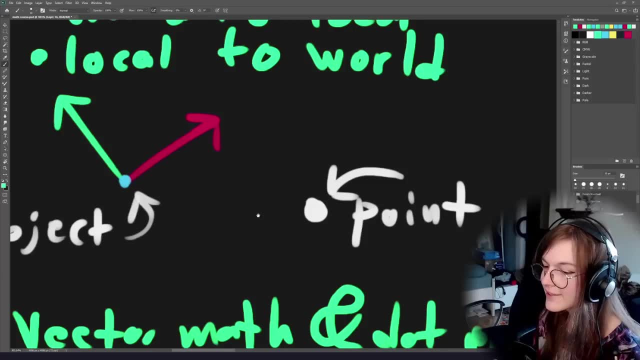 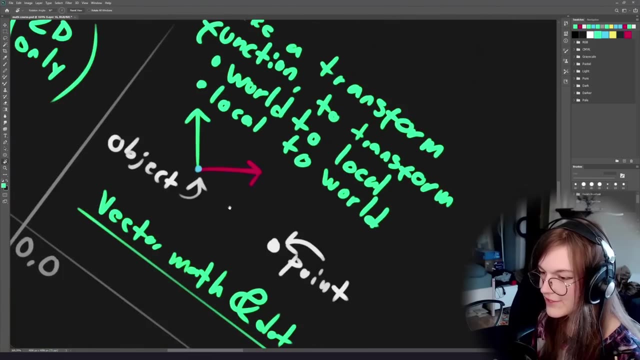 doesn't really matter. You just need to be able to get those coordinates. But how you visualize that or whatever, is a separate thing. You need to be able to get a point relative to a different space. Yeah, So what I mean by that is that if you ignore these lines that I used to draw, 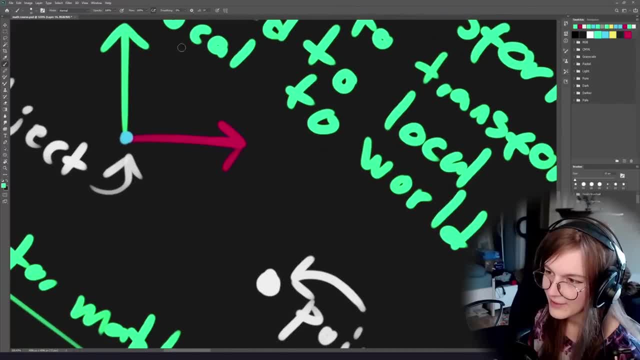 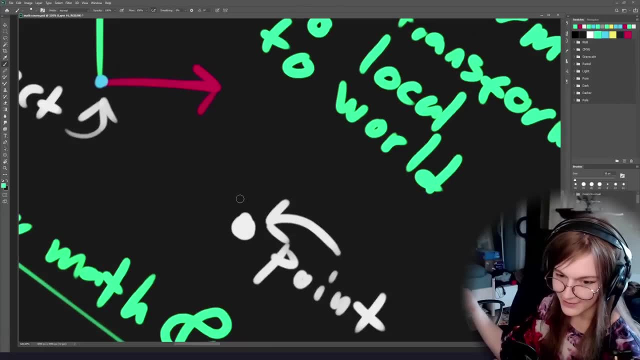 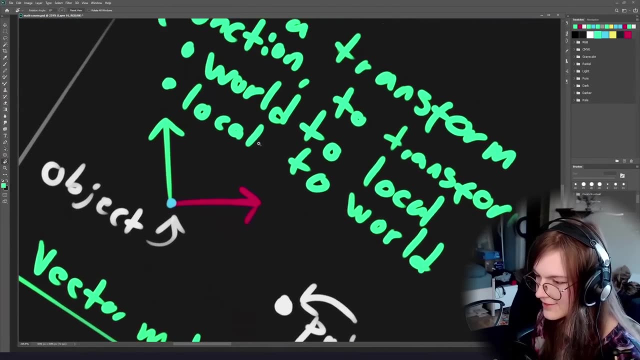 you just need the coordinates of this one If you pretend that Whoops Pretend that this right here is world space or whatever, Because that's kind of what you do, right, But yeah, Basically you want to get this point relative to this space, That's. 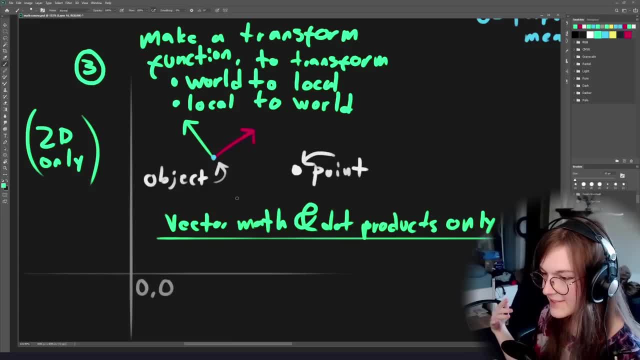 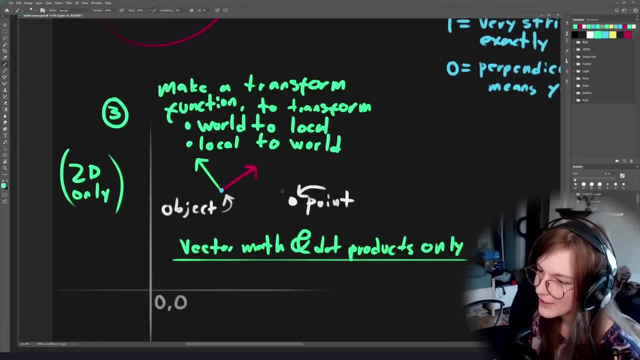 it And also the other way around. Oh, and just parenting objects and getting their location kind of defeats the purpose of it. And the reason I call this a curveball is because we haven't talked about space transformation yet. That's the only reason. Otherwise,